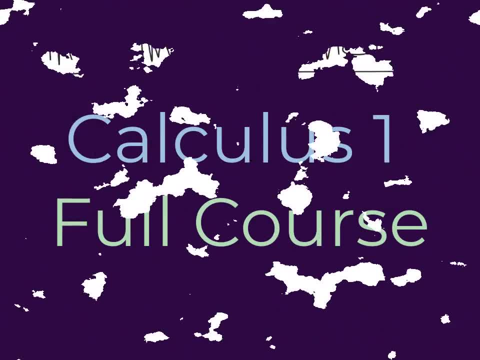 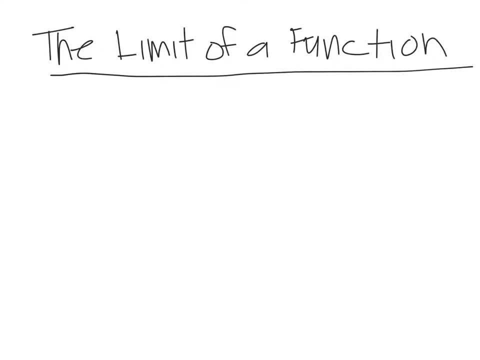 Today we're going to talk about the limit of a function. When we have a limit of a function, we write the following: The limit as x approaches some value a of f of x equals l. In words, this becomes the following: The limit of f of x as x approaches a. 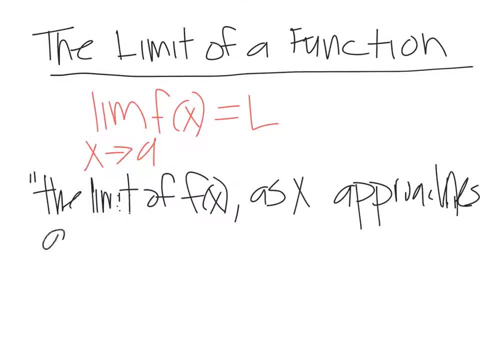 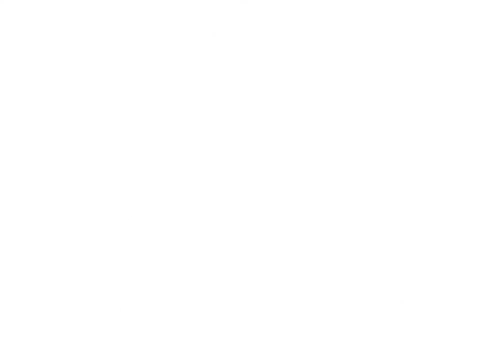 is l. We could also write this as f approaches l, as your x value approaches a. So let's do an example. Let's compute the limit as x approaches 1 of our function function. we'll call this function x minus 1 over x squared minus 1.. Well, what? 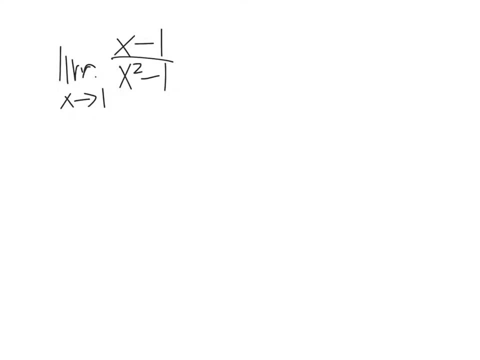 we can do is we can pick some values of x and plug it into our function and see what happens as x gets closer to 1.. So let's create a table. we'll have a column for our x value and a column for our f of x. So if x were 0.5, our f of x would: 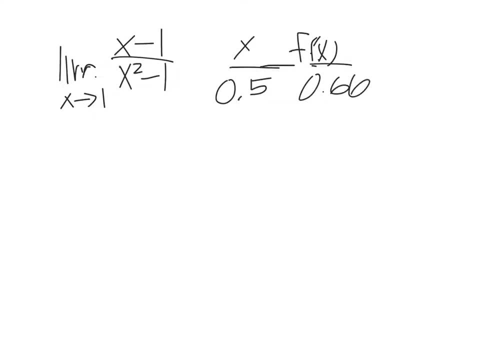 be 0.667 and actually going on forever. If x were 0.9, our f of x is 0.526.. If x were 0.99,, our f of x is 0.5025.. If x is 0.999, our f of x is 0.50025.. 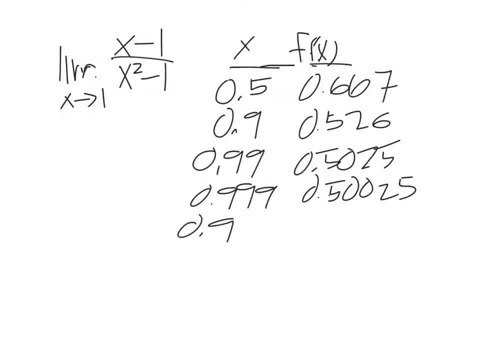 And if our x was 0.9999, our f of x is going to be 0.50025.. So you might notice a pattern, As our x value is going towards 1, our f of x value is going towards another number. 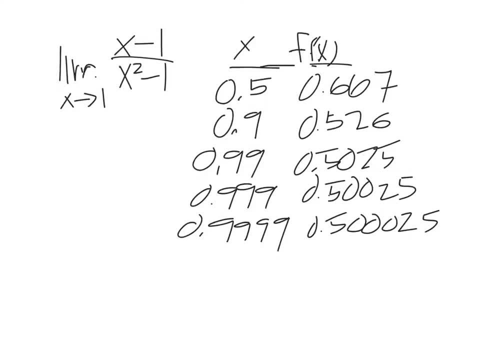 And we'll just confirm this and we'll check out when x is a little bit greater than 1.. So let's start from the other way, For our x value is 1.5, what's the f of x value? Well, that case is 0.4.. 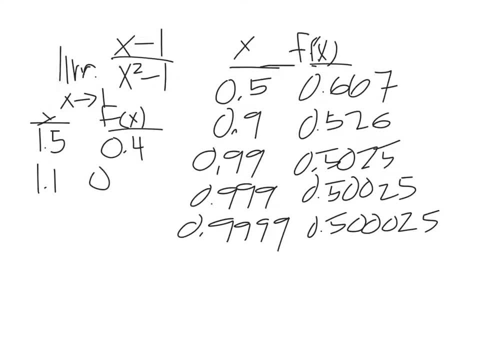 When x is 1.1, we have it's 0.476.. When it's 1.01, it's 0.4975.. When it's 1.001, it's 0.4975.. And, as you see, it is getting closer to 1.. 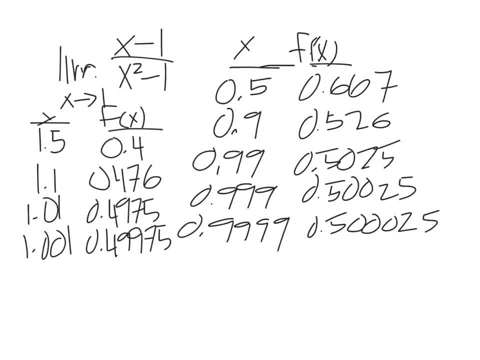 So therefore, we can conclude that as our x value gets closer and closer to 1, the limit, as x goes to 1, of x minus 1 over x squared minus 1, is equal to- excuse me, not 1, it's equal to 0.5.. 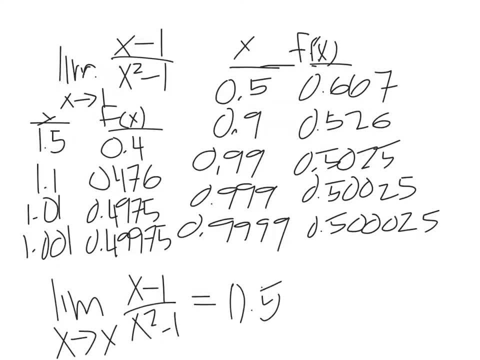 And if we were to actually graph this function, y equals x minus 1 over x squared minus 1,, what we get is the following graph. It looks something like this, where we have a hole right here when x is 1, but the value of that hole is at 0.5.. 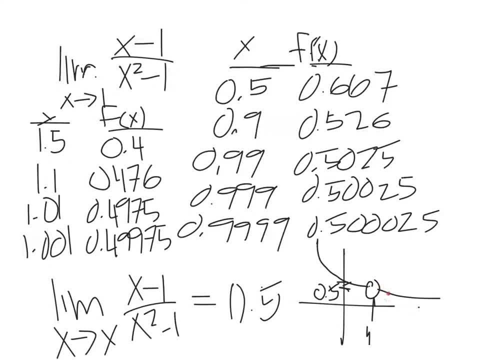 So even though there's a hole, so the function does not exist at that point, it's still the limit That function goes all the way towards it, Everything points towards it. It just doesn't include that point. So limit is just saying where do all the indications say the function is going towards? 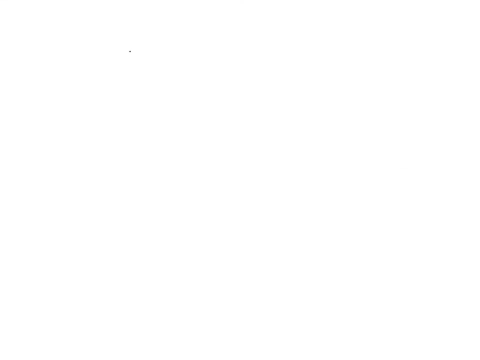 So if we were to look at a graph, we might say that if we have some graph that looks like this: if right here, that's our a of our function, f of x, that's the limit The function approaches, or as X approaches a, so we just look and we see as X gets closer to a. 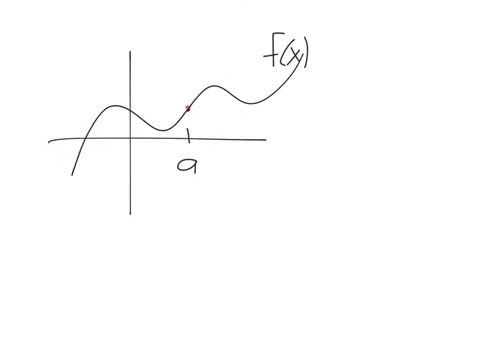 What is the value of the function and that limit is whatever this point is. But sometimes we're concerned only about what happens as we approach a From a certain side, from either the left side or from the right side, When we want to write the limit as X approaches a from just one side. 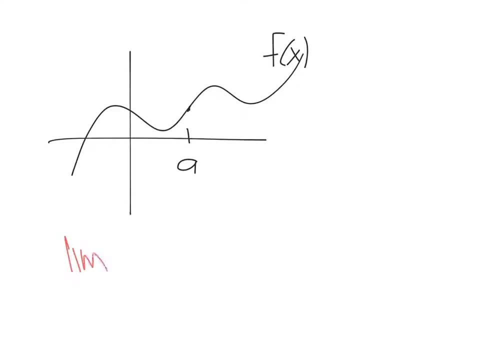 We write it as the following: the limit of f of X as X approaches a, and if we're going from the left side we write a negative sign. Then we say this equals L. in words, we write The limit of f of X as X Approaches a from the right or, excuse me, from the left. 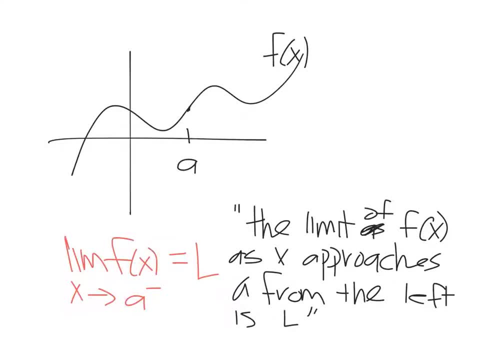 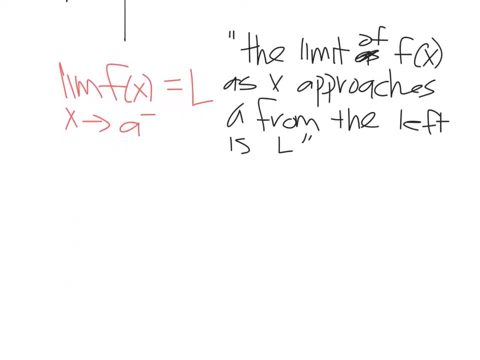 is L now Say. Similarly, you could write the right hand limit, and the right hand limit would just be written instead of the limit of f of x as x approaches a from the right side. we just use a plus instead of a minus, but it means the limit of f of x as x approaches a from the right side is. 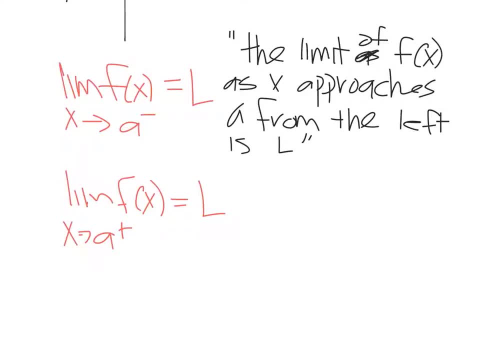 l. so we have the limit. we have the limit where it approaches from the left side and the limit where it approaches from the right side, and so now we put all this together, all the different limits we've learned, and we have the following: we have given the limit as x approaches a. 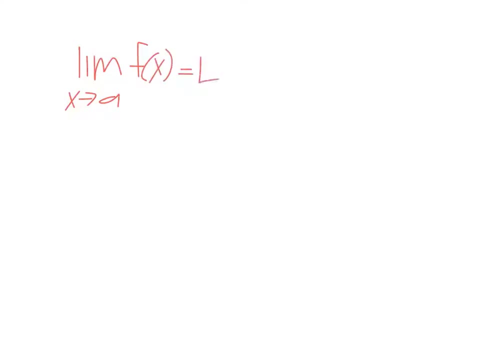 of f of x equals l. we have- this is true if and only if we have the other, the following: the limit as x approaches a from the left hand side of f of x equals l and the limit of f of x as x approaches a from the right hand side. 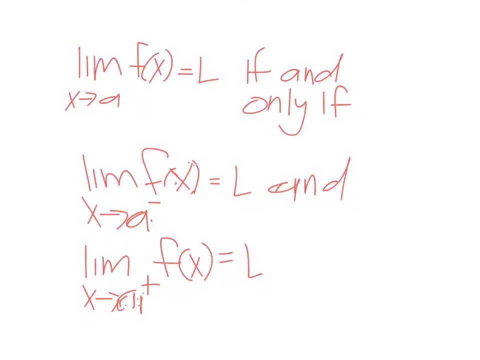 of f of x equals l. so what we have is we have just the limit of f of x. as x approaches, a equals some value, l. that is true only if we have both the left hand limit and the right hand limit equaling the same thing of f of x is equal to the left hand limit by l. 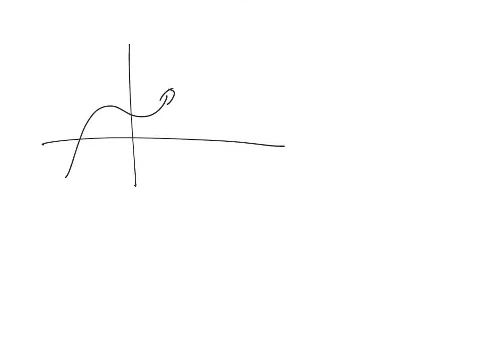 let's do an example. say, we have some function that looks like this and it does something like that, and then we have another gap right here, but it goes right there. so let's put this at one, two, three and let's have one, two, three gone. let's move this thing. 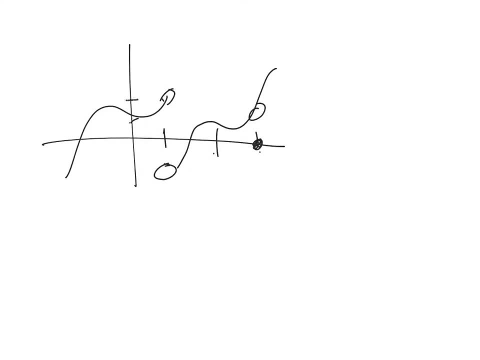 to the right this way, and let's try an example of this again. so this is the forward arrow, or våraoector, or what we call454,. we're gonna put our right hand down. let's grab and first put the right trick, but let's take it right down once we've done our left index finger and left. 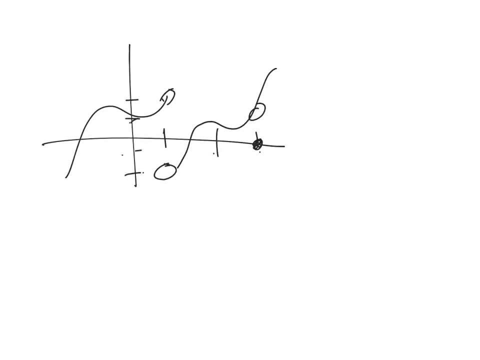 two and negative one, negative two. So this is our function: f of x. Let's determine what the limit of f of x is when x approaches one from the left side and the limit of f of x as x approaches one from the right side. 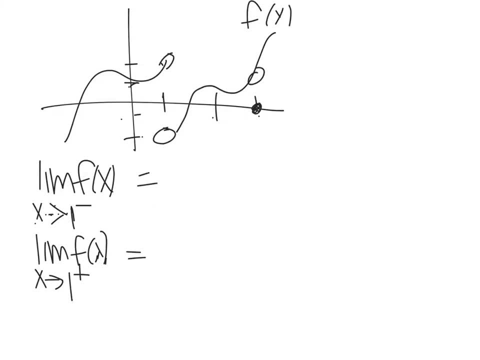 and give myself a little bit more room- and the limit of f of x, as x approaches just one. What is this? Well, if we look at this, and as x approaches one from the left side, this is the value one. 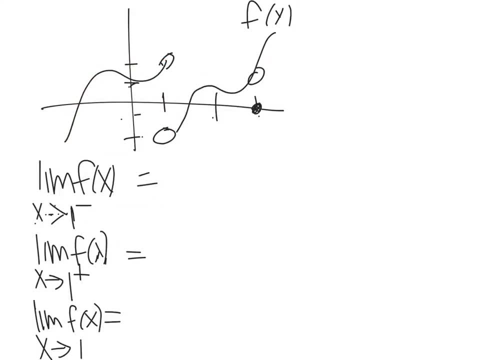 what does the function look like as you approach one? Well, if we're approaching one from the left side, it goes right here to the value of two. So we have our answer for this. first one is two. What about as it approaches one from the right side? 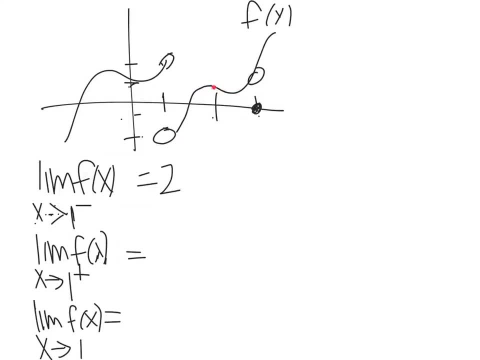 Well, from the right side, we're over here, So we're approaching one from the right, and it goes down to negative two. So now we've said: what's the limit as x approaches one? Well, the limit only equals a number. 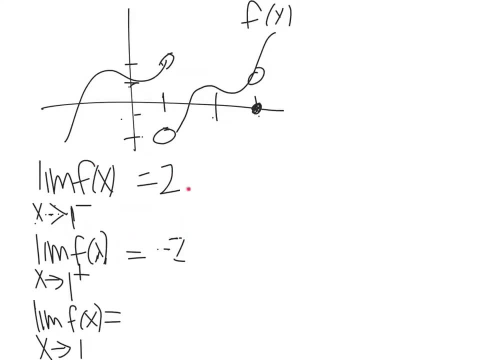 if, and only if, these two limits are equal. but these two limits are different. Since they're different, we can say that the limit does not exist. Now let's compute the limit as x approaches three. So we'll do three things. 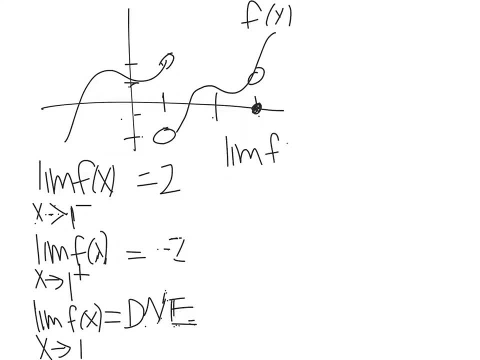 We'll find the limit of f of x as x approaches three from the left side, the limit of f of x as x approaches three from the right side, and the limit of f of x as x approaches three- Well, as x approaches three from the left side. 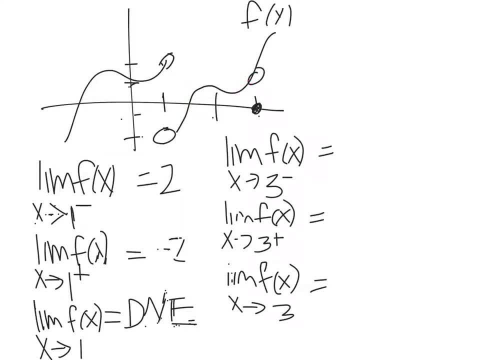 we're going and we come right here, So that would be two. So, as x approaches three, we're going right here. As x approaches 3 from the right side, we're coming up down here and we hit, and that would also be- excuse me, not 2,, 1, it would be 1 and it's also 1, right here. 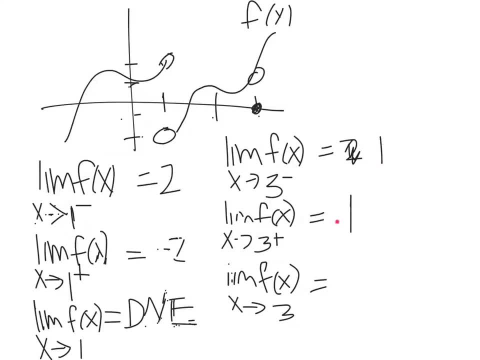 And finally, since we have the left and right hand limits are both equal to 1, the limit as x approaches 3 is just 1.. But note what is f. The value at 3 is actually 0. So the actual value of f equals 0 doesn't necessarily have to equal the limit. 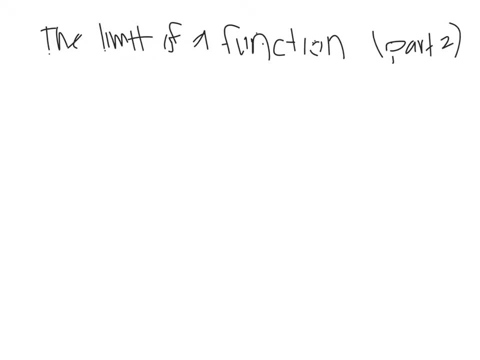 Now, sometimes the limit of a function doesn't equal an actual value. An example of that might look like: if our function does something like this, It goes all the way up to infinity, and from the right side it also goes all the way up to infinity. 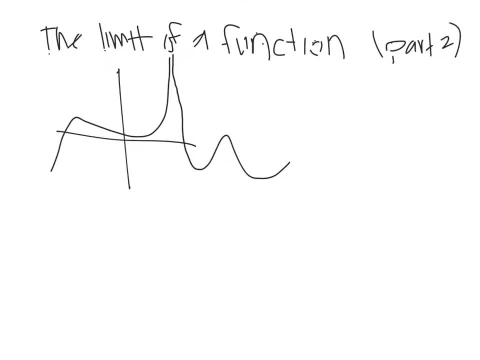 So if it goes up to infinity, we have the following: We write it as the limit as x approaches some value, a of f is equal to infinity. Similarly, it might go down to negative infinity And we would write: the limit as x approaches: a of f is negative infinity. 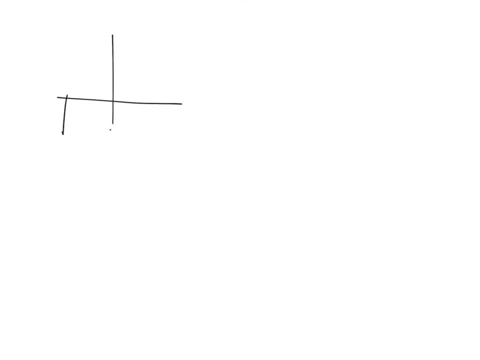 So we might even have something like this: We might have a graph that does this and it goes all the way up to infinity and it doesn't actually quite touch this line, It just goes arbitrarily close And gets very large. So this was the limit. as x approaches some value a from the left side of the function, 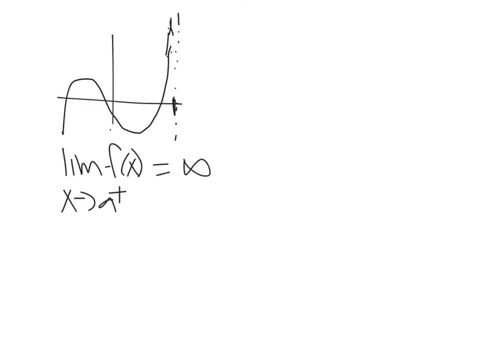 f, and that's going to be infinity. So this, right here, is the point a and this is our function f. We might also have, say, go down to negative infinity, in which case it might look like this: So that's our point a and this is f. 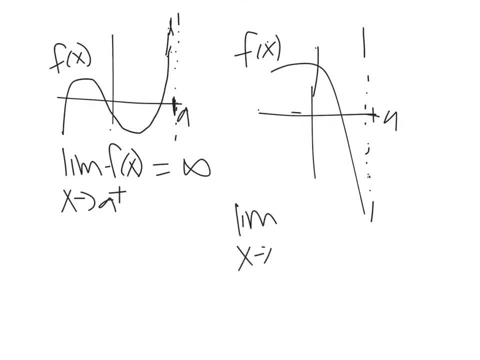 And so this is the limit, as x goes to a. oops, I've been writing the wrong sign- f goes to a from the left side of f. So here we have f equals, in this case, negative infinity. Now you may recall that these points from algebra, these values, are actually what we 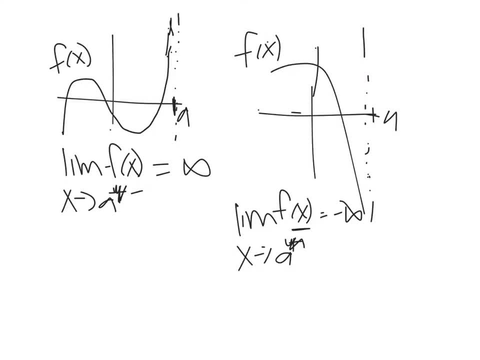 call vertical asymptotes of functions. So we have a definition that says the vertical line x equals a, equals f. And there is an interesting way of doing this: We can take the depth of the line f and take the length of the line x plus a and multiply. 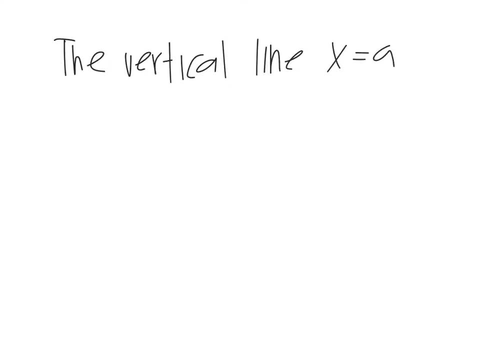 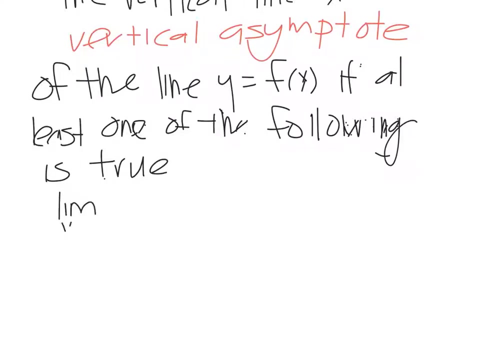 the length of the line x. Let's see what we call a vertical asymptote of the line y equals f of x, if at least one of the following is true, and what we'll have is: we have the limit as x approaches a from the left side of f of x is infinity. 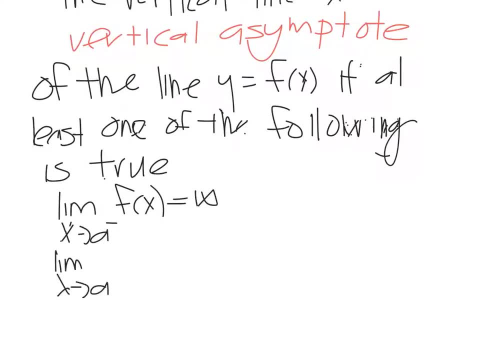 the limit as x approaches a from the right side of f of x is infinity, or the limit as x approaches a of f of x is infinity. or the limit as x approaches a from the right side of f of x is negative infinity. or the limit as x approaches a from the left side of f of x. 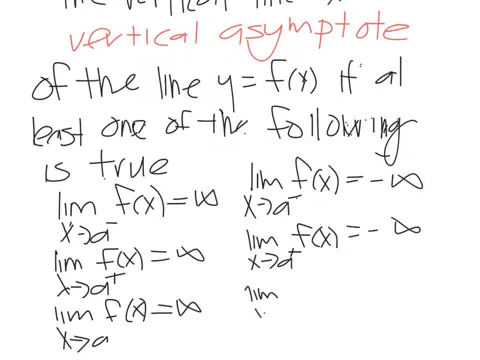 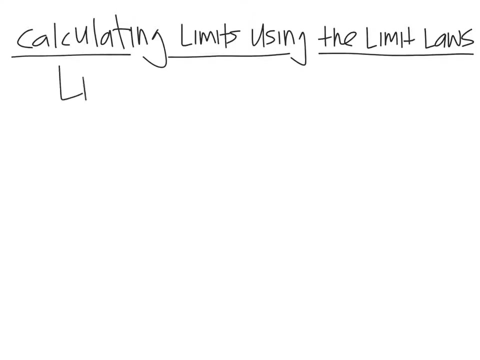 is negative infinity, or the limit as x approaches a of f of x is negative infinity. so if any of these cases happen, then we have what we call a vertical asymptote. now that we know what limits are, we're going to calculate limits and we're going to use the limit laws. 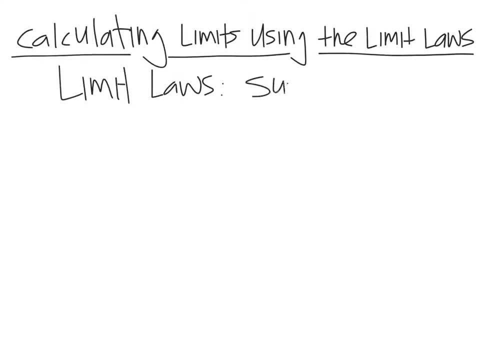 to do this. so first we're going to suppose that c is constant and we'll also suppose that the limits exist, for exists for the following: The limit as x approaches a of f of x and the limit as x approaches a of g of x. So if these two limits exist, then we're going to have the following: 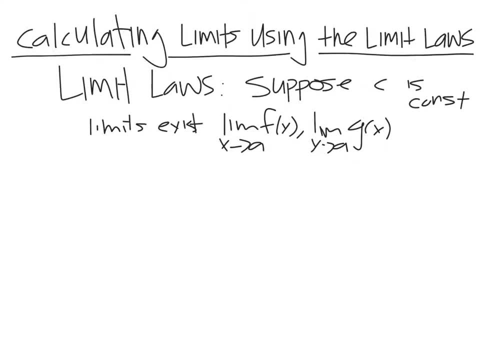 We have first: 1. The limit as x approaches a of the quantity f of x plus g of x is equal to the limit as x approaches a of f of x, plus the limit as x approaches a of g of x. So this is the sum law where we take the limit of the sum of two functions is the sum of each of their limits. 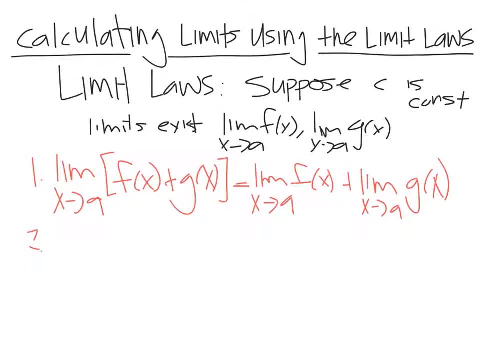 Similarly, we have the difference law, which says that if we're taking the limit as x approaches a of the quantity f of x minus g of x, That's equal to the limit as x approaches a of f of x, minus the limit as x approaches a of g of x. 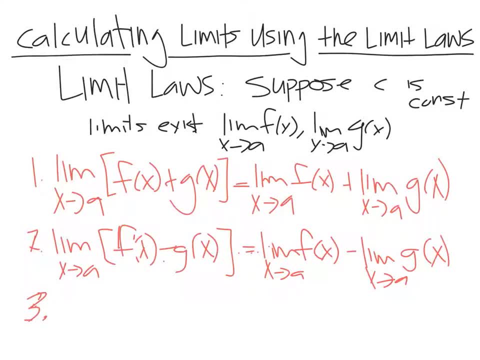 The next thing, 3, we have if we're dealing with a constant multiple. So the limit As x approaches a of some constant c times our function f of x. This is just equal to the constant times the limit as x approaches a of f of x. 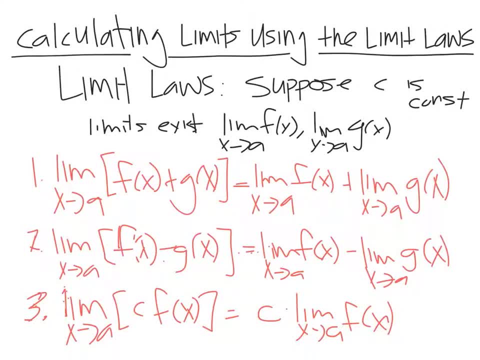 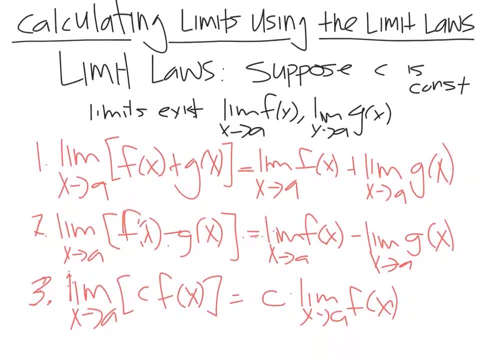 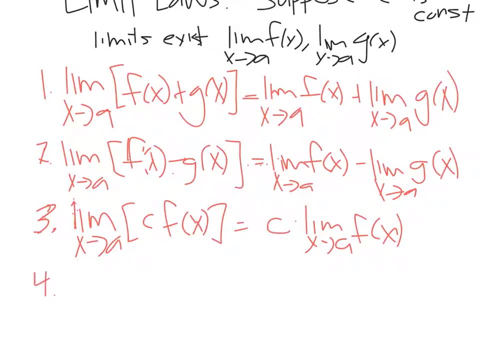 So if we have some constant, All we need to do is just Multiply that constant by the limit of the function. Now We have two more, So number 4. This is going to be the product. So if we have the limit, 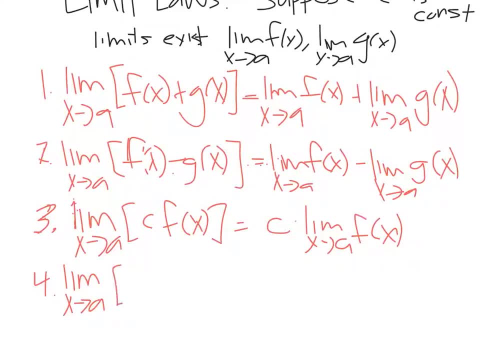 As x approaches a For the product of two functions, f of x times g of x, This is equal to The limit as x approaches a Of f of x Times The limit as x approaches a Of g of x. 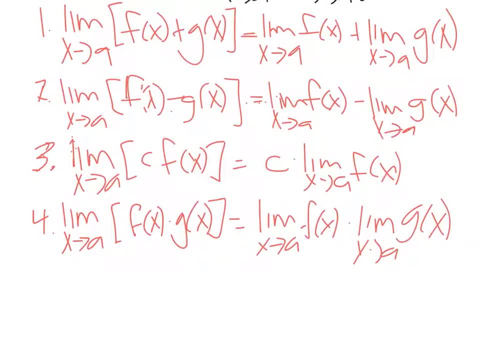 And finally, We have the fifth Law that we're going to go over right now, And this is going to be The quotient law, And this says that The limit As x approaches a Of the quantity f of x. 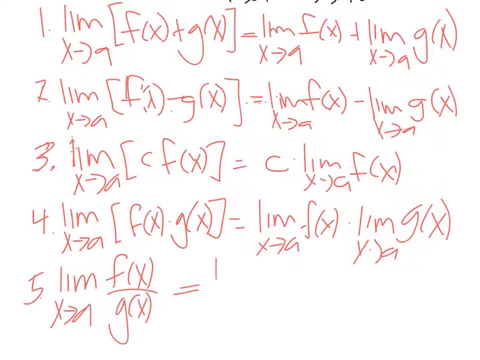 Over g of x Is equal to The limit As x approaches a Of f of x, Divided by The limit As x approaches a Of g of x, But This is provided That the limit As x approaches a. 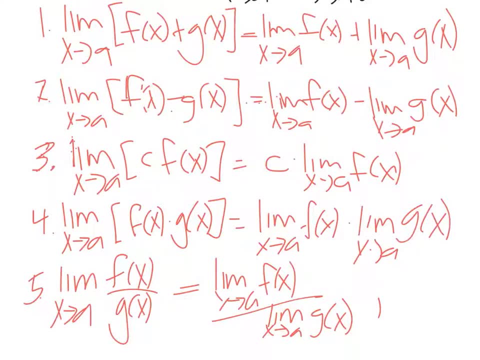 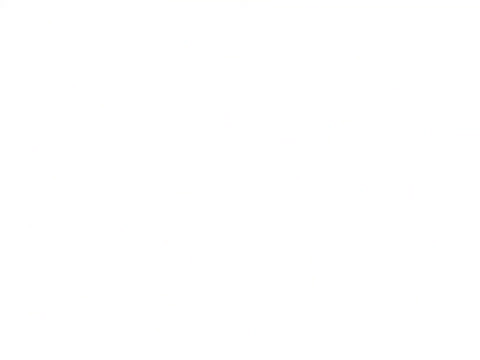 Of g of x Is not equal to zero, Because then we'd be dividing by zero. So this is: If The limit As x approaches a Of g of x Is not Zero. So, for example, If I told you: 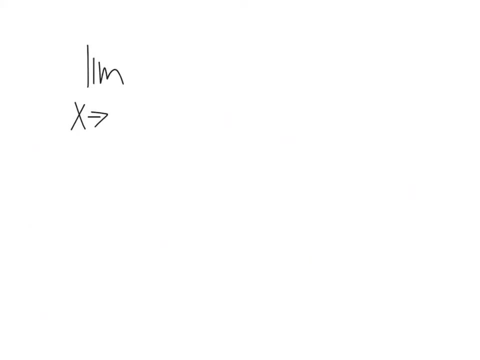 that the limit as x approaches 3 of f of x is 2 and the limit as x approaches 3 of g of x is negative 4, then if we were to calculate the limit as x approaches 3 of f of x plus 2 g of x, we can: 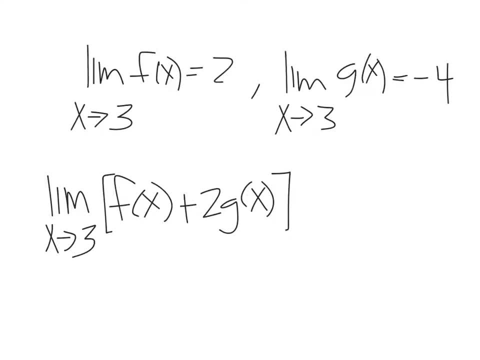 use the law of limits. so what we have here first of all is addition, so we could separate this into the limit as x approaches 3 of f of x is 2 and the limit as x approaches 3 of g of x is 2 and the. 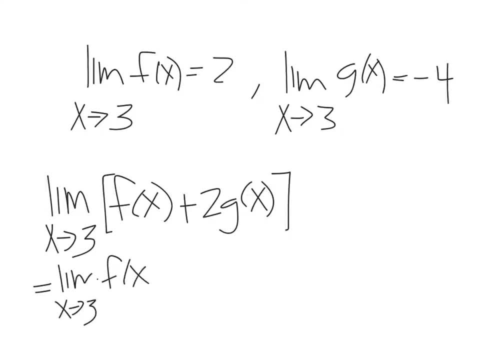 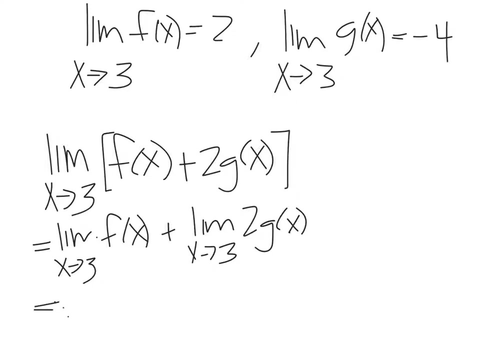 limit as x approaches 3 of f of x, plus the limit as x approaches 3 of 2 g of x. but notice, right here, 2 is a constant, and so by using the constant we can pull the constant in front, and so this we get is the limit. 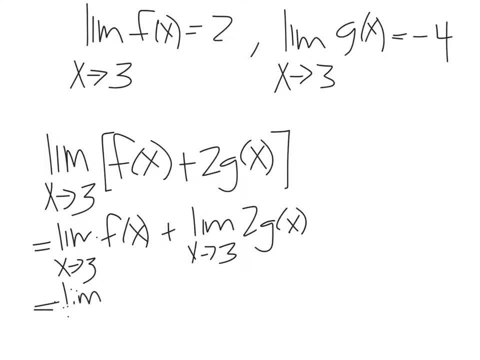 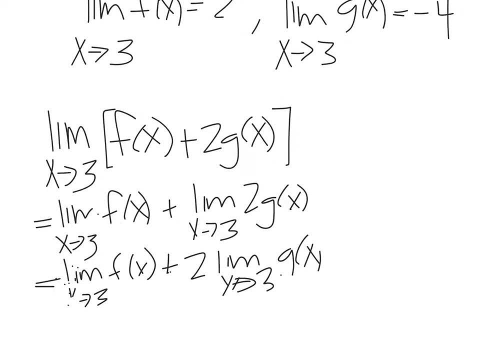 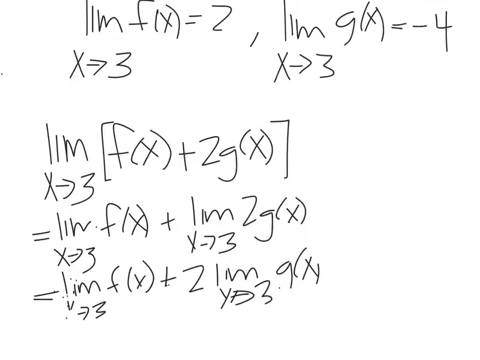 as x approaches 3 of f of x, plus 2 times the limit as X approaches 3 of g of x, and we know that the element as X approaches 3 of f of x is going to be 2 from right up here and the limit as x. 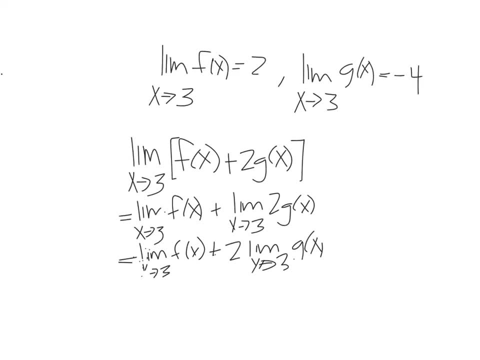 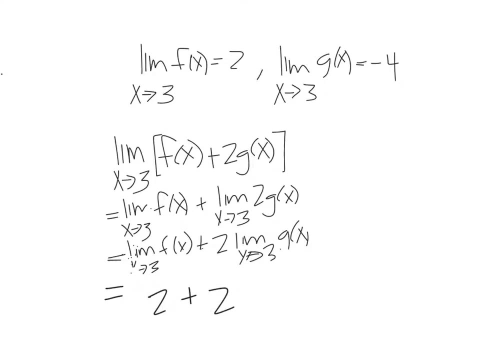 approaches. let me just make it a little bit smaller. So we have this: first limit is 2 plus 2 times negative 4.. So we have this is equal to negative 6.. So there are a couple more limit laws that we have. So number 6: this is the limit as x approaches a of the quantity of f of x raised. 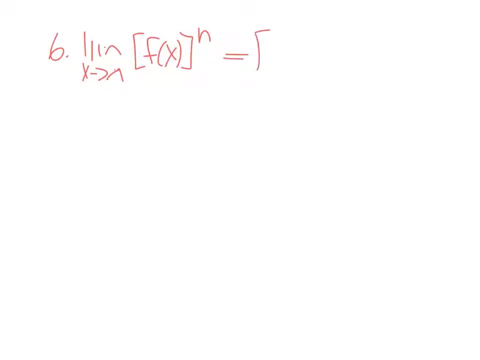 to the power n is going to be the same as the limit as x approaches a of f, of x all raised to the power n. this is the case where n is some positive integer. we also have the limit as X approaches a of just some constant C. well, that's just going to be C, because 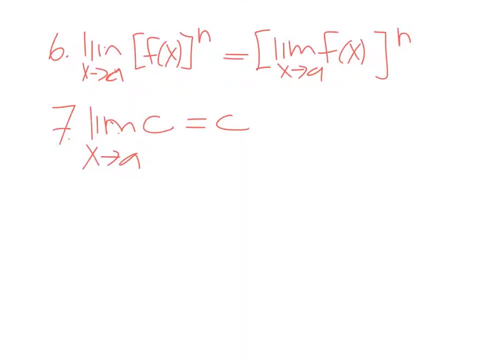 it's constant, it never changes. it's always going to be C. number eight: we have the limit as X approaches a of X is equal to. well. this is pretty intuitive as well. well, if X approaches a, then the limit of X should just be a, since X is going towards a. we also have, for nine, the limit as: 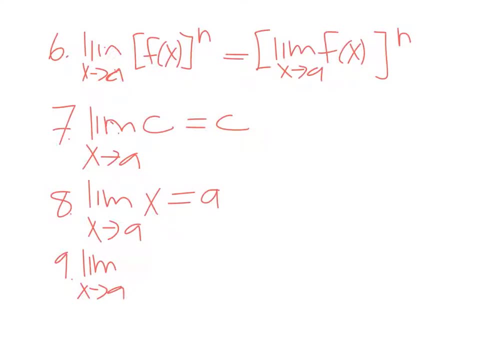 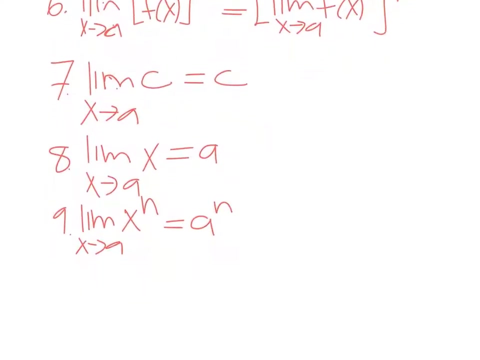 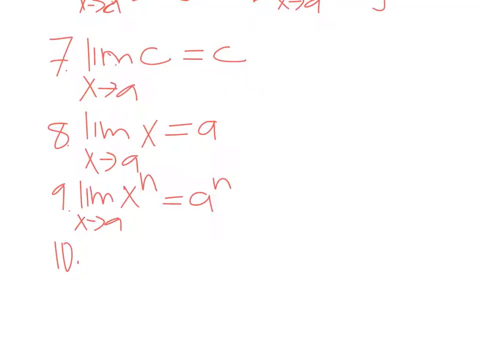 X approaches a of X to the power n is equal to a to the power n. and this is just for some positive integer n, number 10, we have the limit as X approaches a of the nth root of a to the nth root of X, this should equal the nth root of a, where again a our. 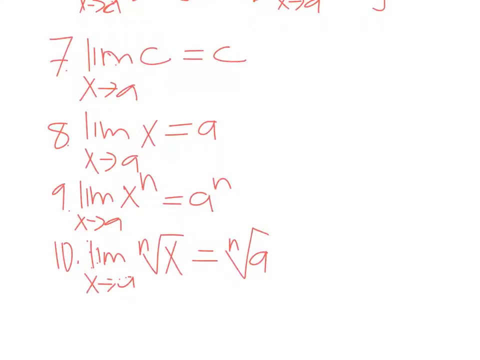 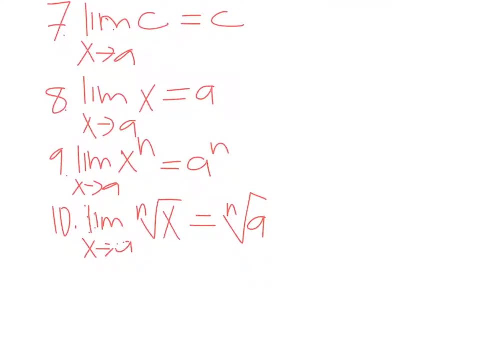 n is a positive integer and we're going to assume that a is also positive. and next we have number 11 and this law says that the limit as x approaches a of the nth root of f of x is equal to the nth root of the limit as x approaches a of f of x. and again, if n. 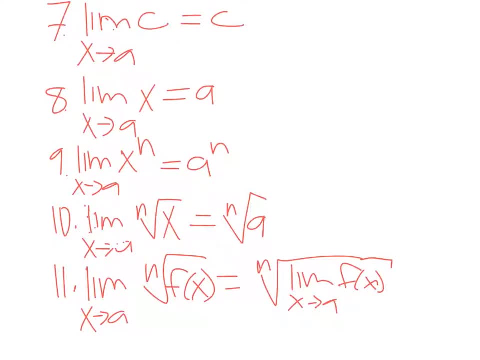 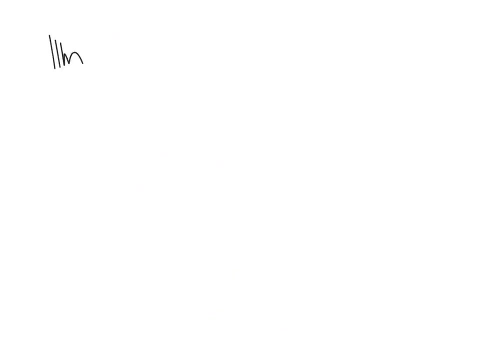 is even. we're going to assume that what's in the radical is positive. so let's do an example. let's calculate the limit as x goes to 5 of 2x squared minus 3x plus 4, while we have three things going on. we're adding and subtracting, so we can separate this into three limits. 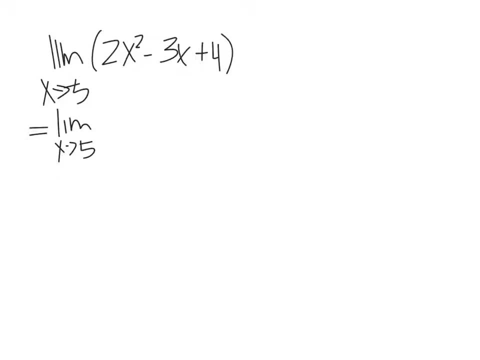 the limit as x goes to 5 of 2x squared, minus the limit as x goes to 5 of 3x, plus the limit as x goes to 5 of 4. now for this first one. right here we have we're multiplying by a constant, so we can pull. 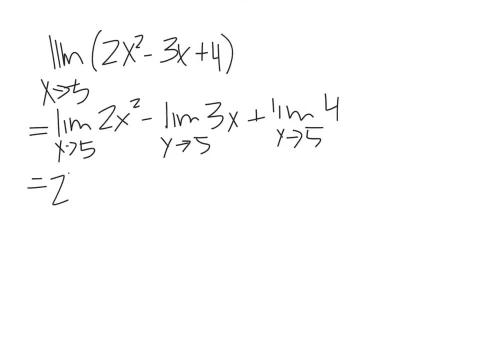 that out, this becomes 2 times the limit as x goes to 5 of 3x plus 4 of x squared minus. we also have a constant 3, so we can pull that out 3 times the limit as x goes to 5 of x plus and the limit of a constant 4 is a constant. so this is just going. 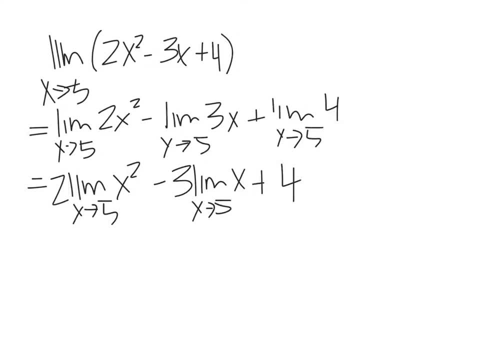 to be 4. we already found that part. now what we have, x squared. that can be rewritten as the following: so this is going to be 2 times the limit as x goes to 5 of x, quantity squared minus 3. and then now the limit as x goes to 5 of x is just going to be 5. 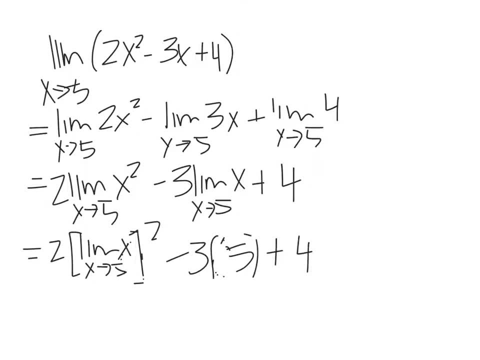 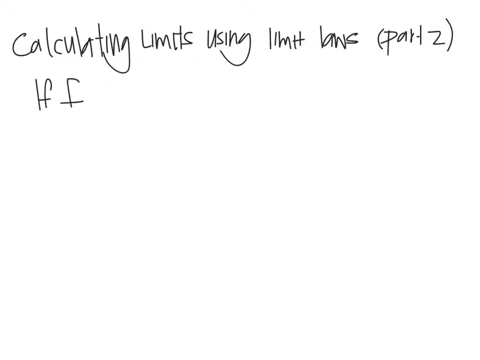 and then we have plus 4, and so the limit right here inside is going to be 5. so we write that now as 2 times 5 squared minus 15 plus 4, and we get this is equal to 39. now we have a property, and this says that if f is a polynomial or a rational function, 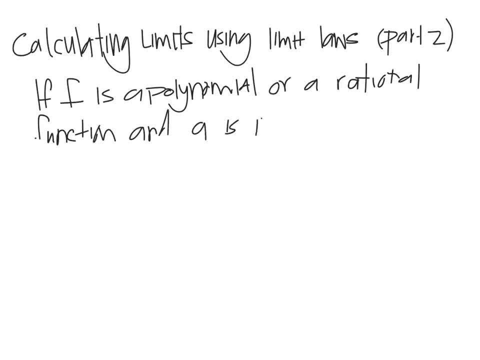 and the value a is in the domain of f, then we have the following: then the limit as x goes to a of f of x is just simply f of a. now this relates to something we call continuous at the point a, but we'll talk about that later. 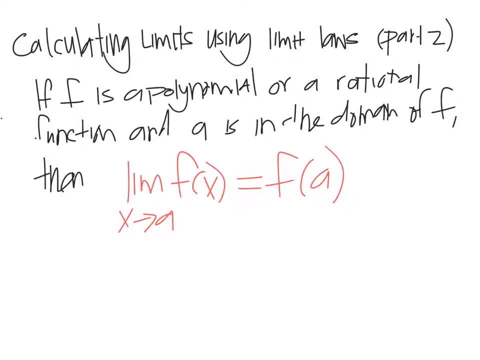 many times we can use this direct substitution and we'll make life easy, but sometimes we cannot. so, for example, if we're trying to find the limit as x approaches, 1 of x squared minus 1 over x minus 1, what can we do? if we plug 1 right into this, we would get 1 squared minus 1 over 1 minus 1, and so 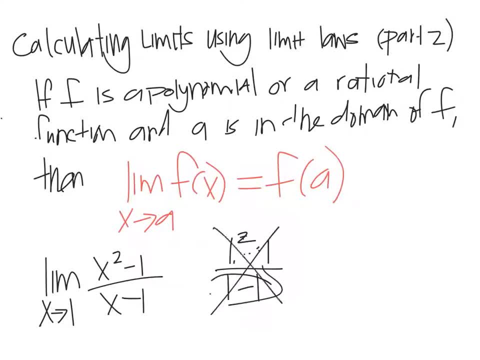 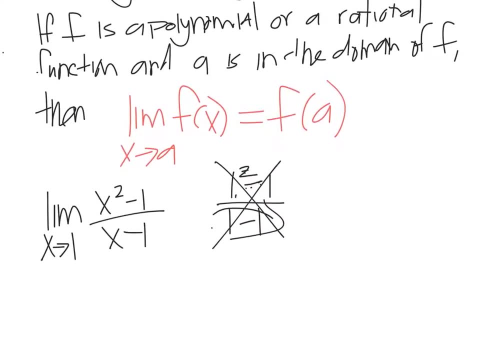 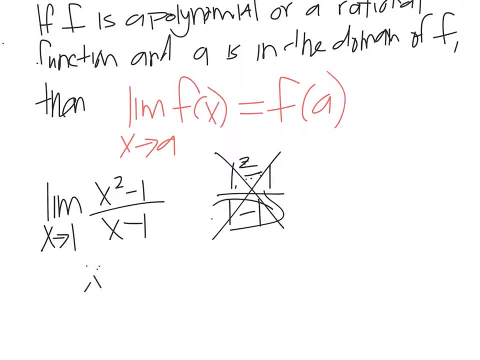 we'd be dividing by 0 and we cannot do that. so we know that 1 is not in the domain. but if we were to simplify this, we simplified the expression and we rewrote it as x squared minus one. instead, we wrote it as x minus one times x plus one when we divide. 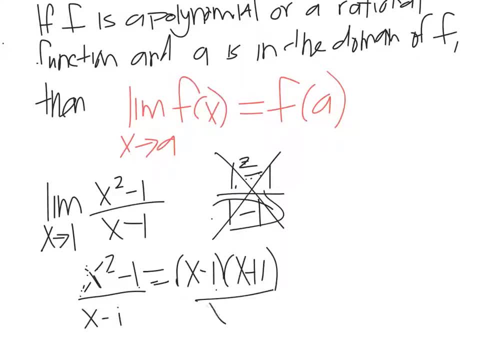 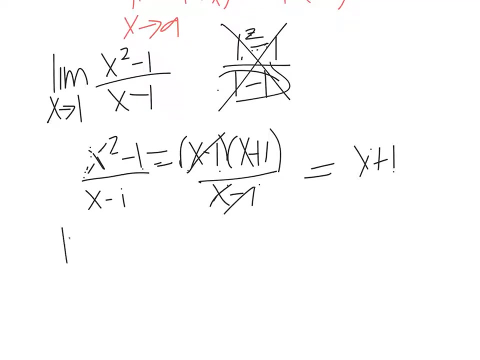 it by x minus one and we divide it by x minus one, we see that we cancel and this is just x plus one. So if we were to then plug that in, what we get is the following: we get the limit, as x goes to one of x plus one, and this is a polynomial, so we can straight substitute, and so this: 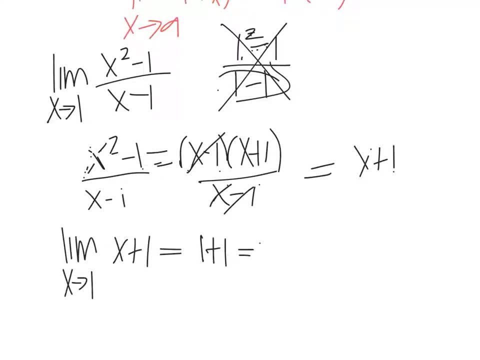 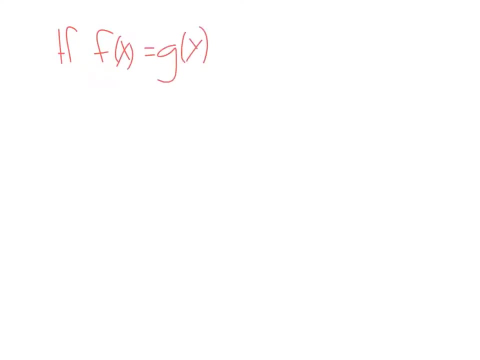 becomes one plus one, which is two. We also have another property, and this says that if f of x equals g of x, when x is not equal to a, then regardless, if it's not equal to a, we know that the limit as x goes to a. 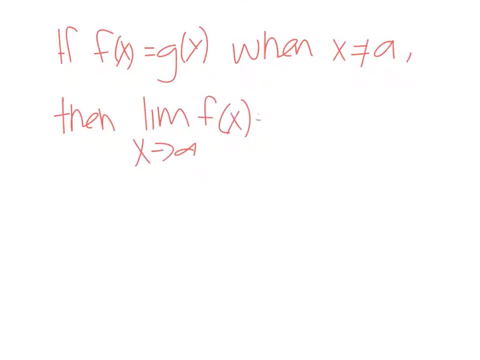 of f of x equals the limit as x goes to a of g of x, provided that limit exists. So an example of what this might look like is if we have, say, two functions and one function looks like this: This is our f of x. 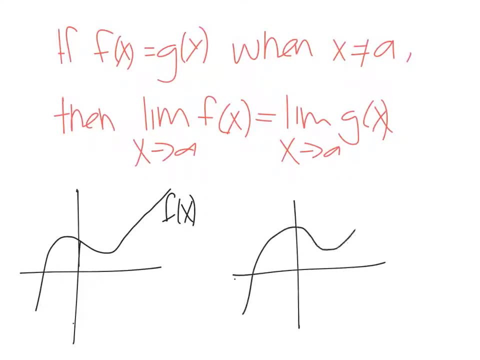 And then we have a second function that looks like this: So this is our point a and our g of x, and these two functions are the same everywhere, except at the point a. At the point a, g of x has a value up here, but doesn't really matter, because their limits. 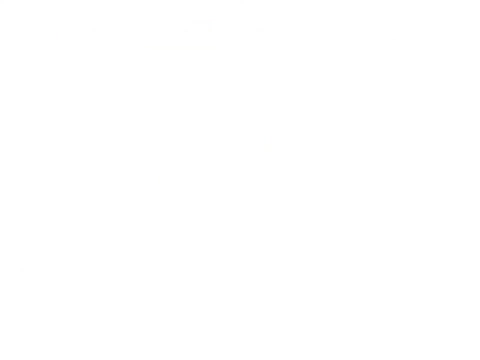 are both going to point down here. Now we have a theorem, And this theorem states that the limit as x approaches a of f of x equals l if, and only if, the limit as x approaches a from the left side of f of x of x equals L, and that equals the limit as x approaches a from the right side of f of. 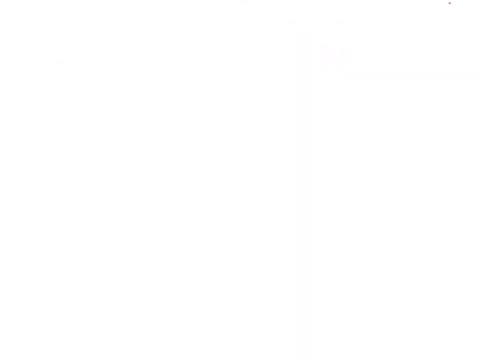 x. We have another theorem that states the following: That if f of x is less than or equal to g of x when x is near a, and this except for when, possibly, it's equal to a and the limits of f and g both exist as x approaches a, then we have the following: 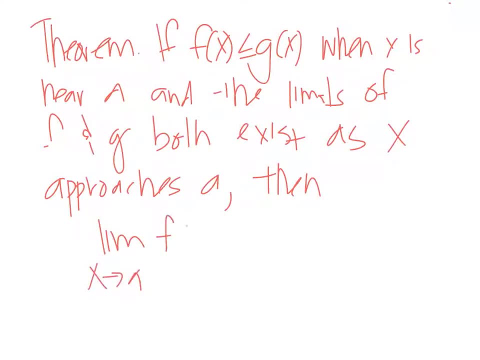 The limit as x approaches a of f of x is less than or equal to the limit as x approaches a. That's the limit. We have another theorem that states the following: That if f of x is less than or equal to g of x when x approaches a, and this except for, 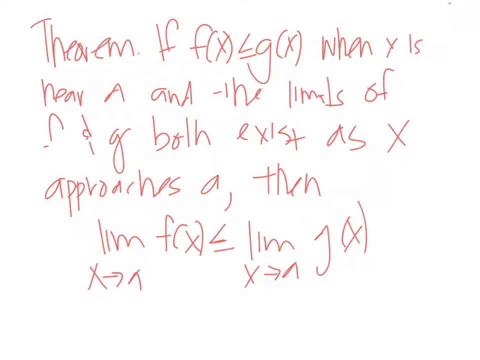 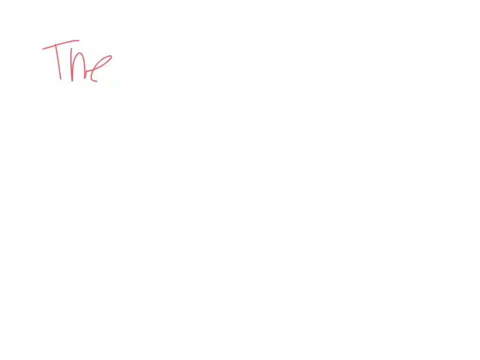 of g, of x, and this should be sort of intuitive. if one function is less than the other, then the limit of that function is less than or equal to the limit of the of that one. and the last theorem we're going to talk about is one that actually has a name, and this is called. 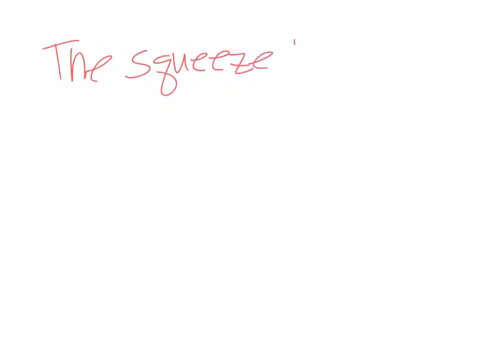 the squeeze theorem and this says: given three functions, and if the functions f of x is less than or equal to g of x is less than or equal to h of x, when x is near a, except possibly possibly at a, and if x is near a, except possibly possibly at a, and if 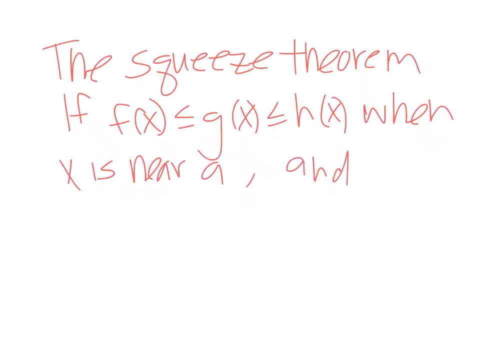 we have that the limit as x approaches a of f of x equals the limit as x approaches a of h of x equals some value: l. then the limit as x approaches a of g of x is l. so what this is saying is that if we have three functions- f, g and h- where f is less than g, 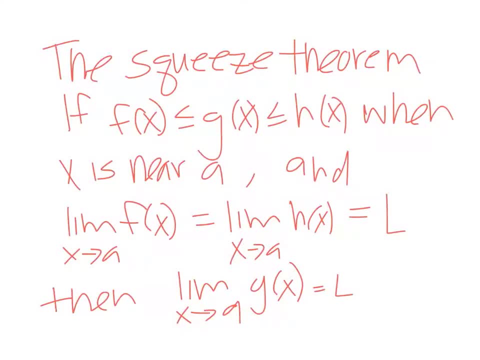 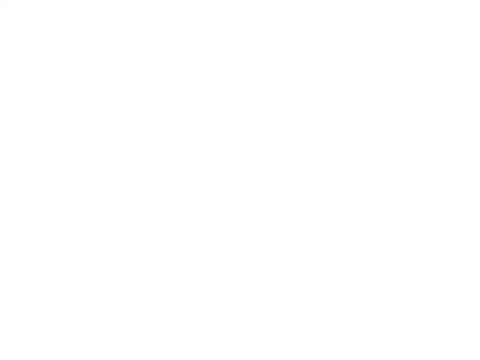 is less than h and if the limit, as x goes to a of f of x, equals h of x, then that means that we're squeezing g of x, the limit, to be the same value. so let's do an example, let's try. and we're squeezing g of x, the limit, to be the same value. so let's try and. 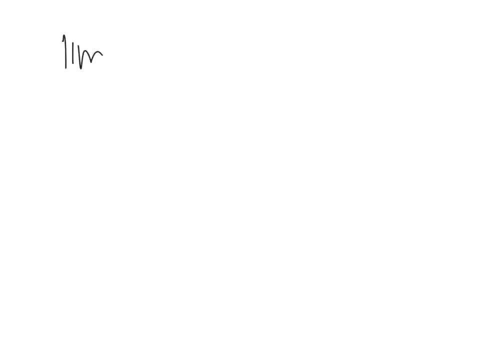 and show that the limit as x approaches 0 of x squared times, sine of 1 over x is equal to 0, well, we cannot reuse the following. we cannot write it as the limit as x goes to 0 of x squared times, the limit as x goes to 0 of sine of 1 over x, because 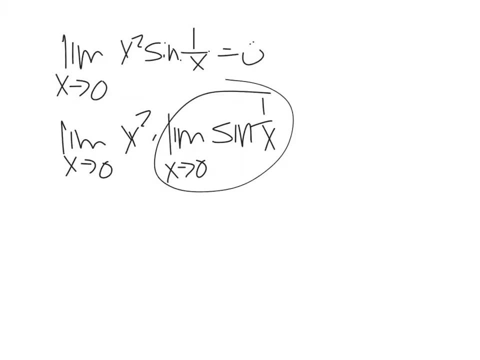 this does not exist. so what we'll do is we now look at x squared times: sine of 1 over x. now we know that sine of 1 over x- sine of anything- really- will vary between negative 1 and 1, and so therefore we can bound this by just saying that negative x squared. 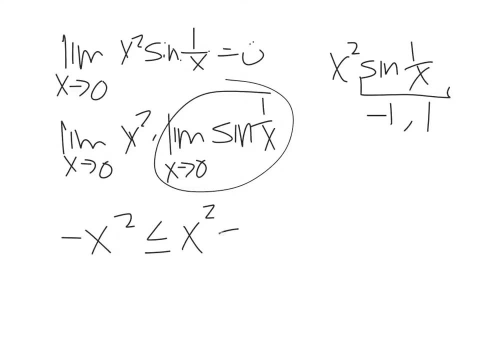 and is less than or equal to x squared times, sine of 1 over x is less than or equal to positive x squared, because we know that sine of 1 over x varies between negative 1- that's where we get this- and positive 1, and so now, applying the squeeze theorem, what we get is we're going to. 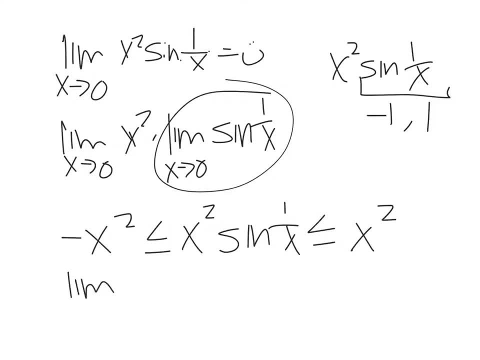 find the limit, as x goes to 0, of negative x squared. well, that, right there, as it goes to 0 is just simply 0, and the limit, as x goes to 0 of positive x squared is also 0, and so therefore, we know by the squeeze. 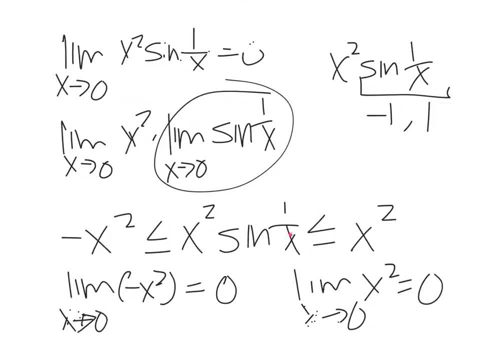 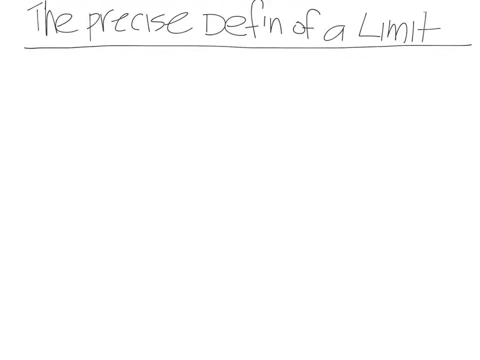 theorem that if we have something like this, we're all. between then, we conclude that the limit of x goes to zero. of x squared sine of 1 over x is 0. today I wanted to talk about precise definitions of a limit, so we can begin by the same. let f be a function. 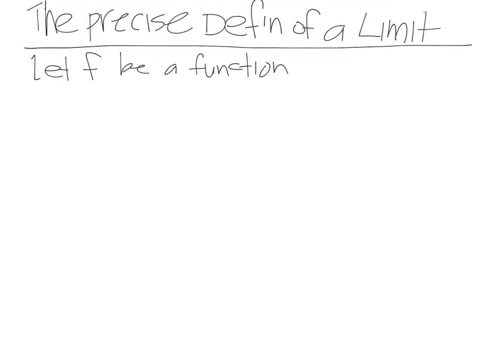 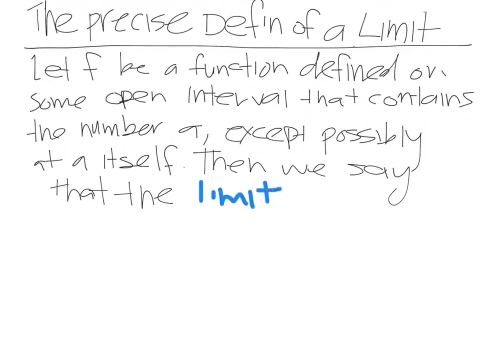 function defined on some open interval that contains the number A, except possibly at A itself. Then we say that the- I'm going to change my font right here- that the limit of A, f of x, as x approaches A is L, and we write the following: 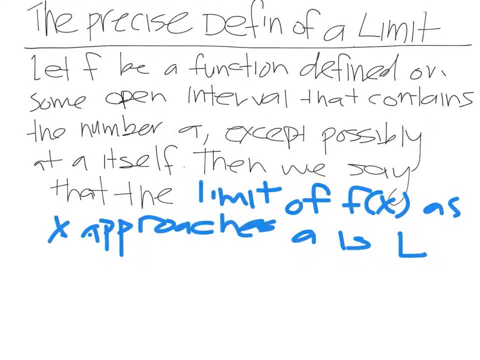 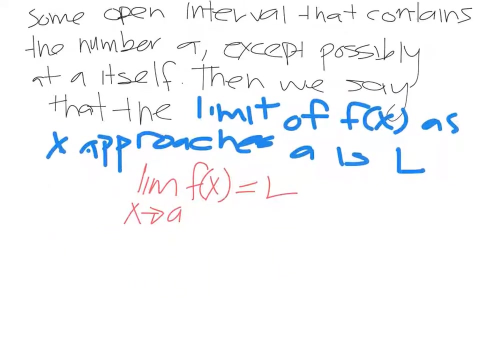 We write the limit as x approaches A of f, of x equals L. So we have this if- let me move this up a little bit. So we have this. if the following: If for every number- we're going to just call this number epsilon. 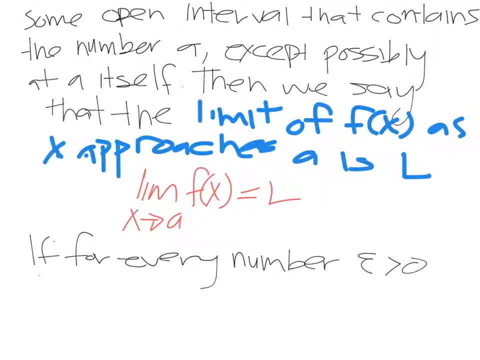 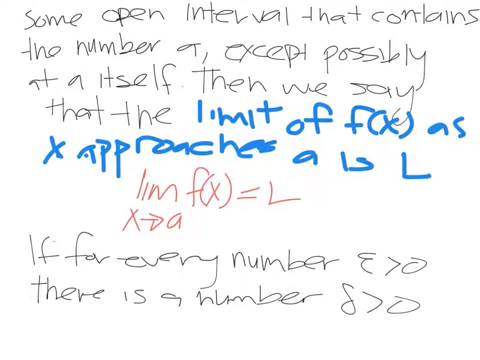 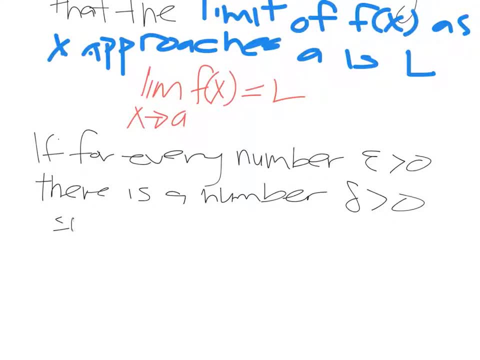 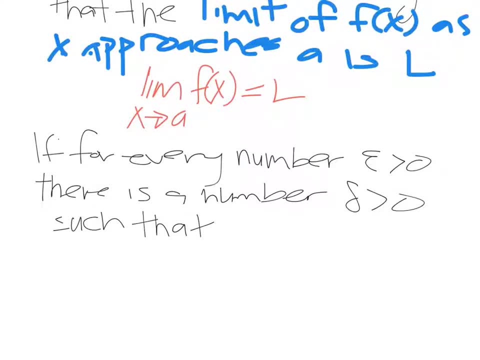 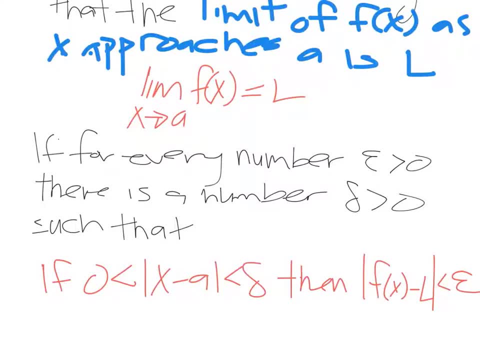 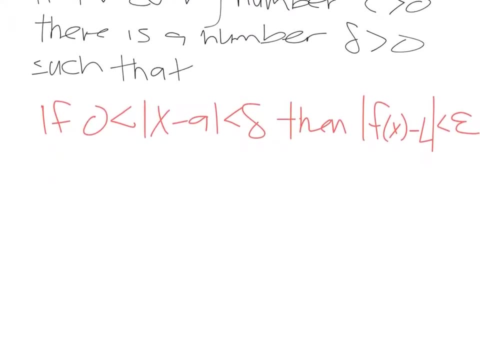 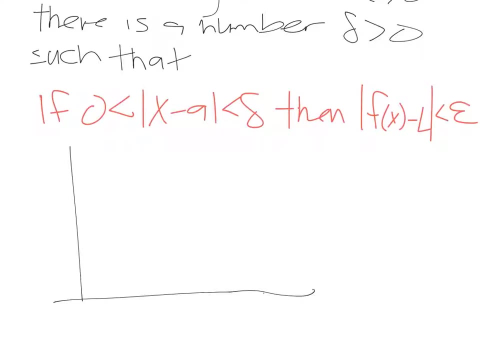 then we have that the distance between f and l is less than epsilon. Graphically, what this looks like would be the following: So if we have our graph, we have x and y, then we have some function like this. this would be our f of x. 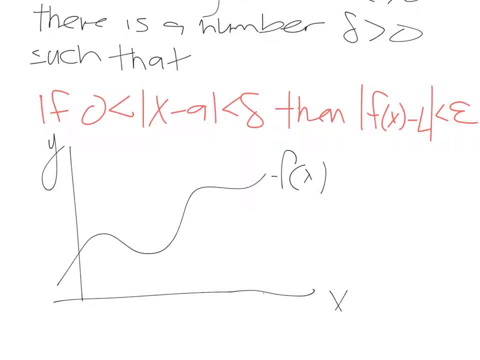 And if we had some arbitrary x point, excuse me, I meant a. So if we had some arbitrary x point, excuse me, I meant a. So if we have some arbitrary value a and it goes right here, and if that's what the 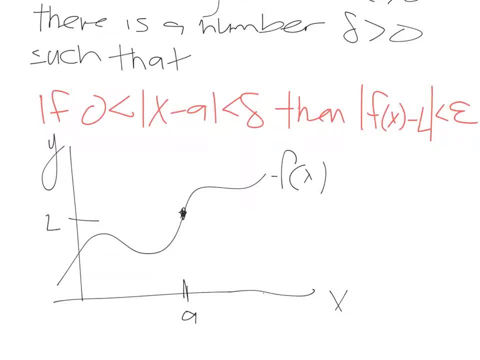 limit would be, and that limit is l, then what this says is that if we're given some epsilon- so let's just say epsilon looks something like this: This has a length of epsilon, and then we also have another length epsilon going down. 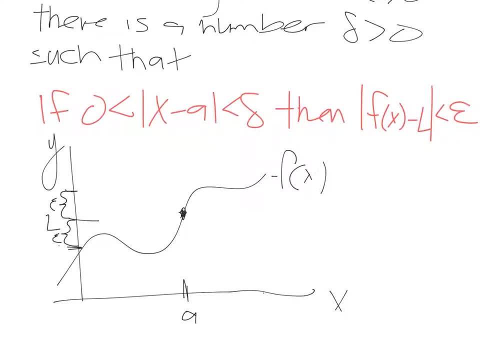 So this upper bound right here goes from the point l and we add epsilon. so this is really l plus epsilon, and then this lower point right here is l minus epsilon. So we have a region. We start at l and we basically say: if we go just a little bit up or a little bit below, 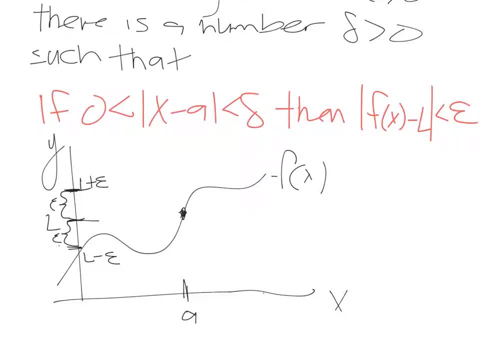 that's what epsilon says. If there's an epsilon like that, what we can say is that there's going to exist some sort of delta, such that the difference between your a value and your delta value or, excuse me- and your actual x value will be within that delta. 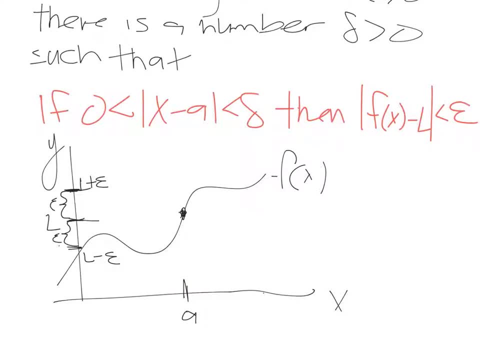 So go ahead and extend this line from here. we extend it right there, we'll bring that down over here. again up here we'll extend and then we'll bring that down. So as long as we're within this region for our x value. 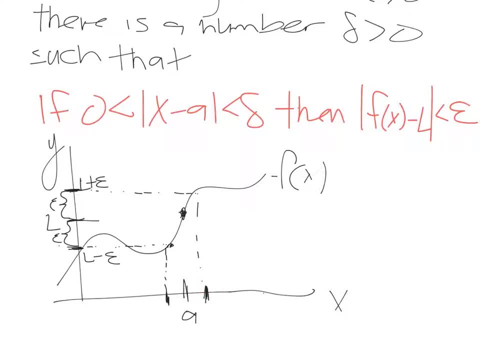 then this satisfies. So what do I mean? First of all, I'll go ahead and label the delta. We have delta here and here, and then this point right here is going to be a plus delta, and then over here would be a minus delta. 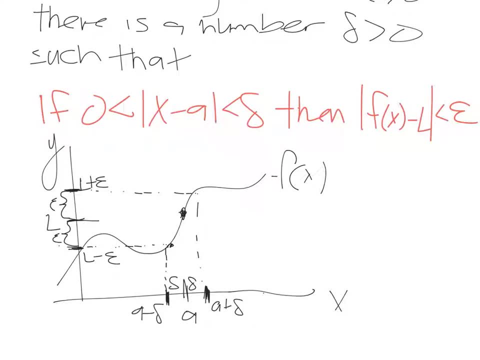 So, looking at this definition, and this says that as long as our x value is the difference between our x value and a is less than delta, So we're somewhere in this region. So if our x value is close enough over here, then our y value will fall within this region. 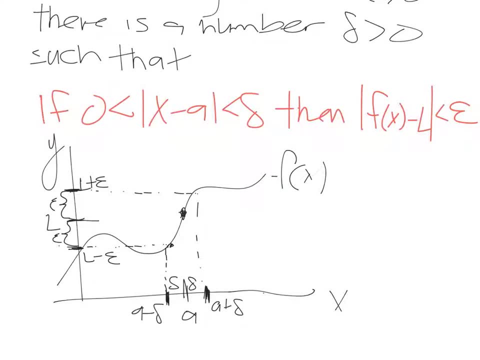 And that's what it means for something to be continuous. If your x value is close enough, then your y value is going to be close enough, and that will happen as we get arbitrarily small. So let's go ahead and do that. 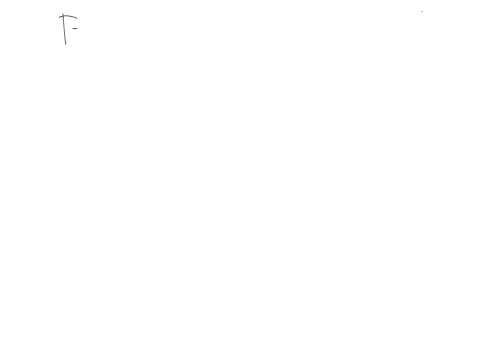 So let's go ahead and do that. So let's go ahead and do that. So let's do an example. Let's find a number, delta, such that if 0 is less than x, minus 3 is less than delta. 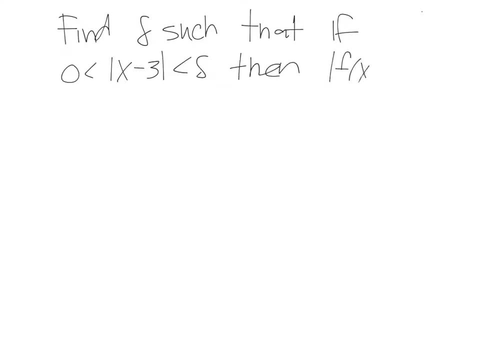 then we'll have that the absolute value of f of x minus 2 is less than 0.. 0.5.. So we need to find what delta is. So let's go ahead and graph this, And I'm giving you the graph. 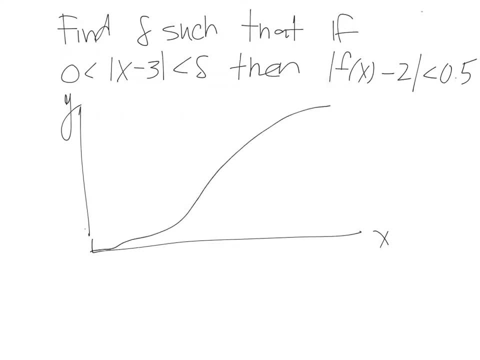 So the graph will look something like this, And so we have the point where x is 3.. That would be over here, and the y value for that would be 2, so I'm getting all this by looking right over here. 3 and 2. 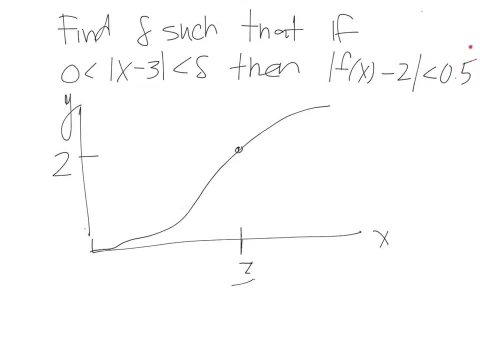 and then our epsilon, how far we're varying in the y direction, is 0.5, and so we would have at 2.5 up there and 1.5 down here, and if I were to follow that over here and then all the way down, 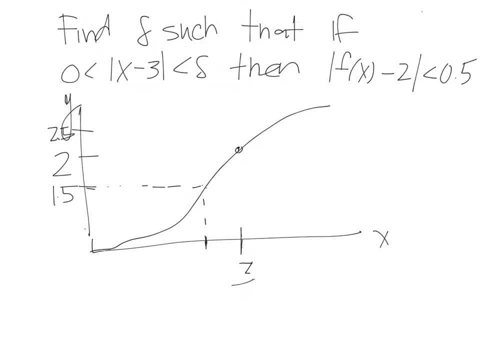 what I would get down here is the value 2.6 and then, following this all the way to here and down, I get the value 3.8. so notice that these are different lengths: the length between here and here and the length between here and here. 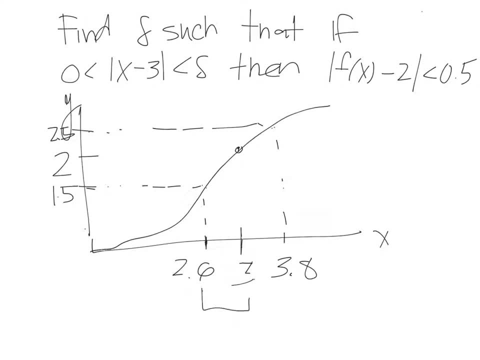 so the length between 2.6 and 3 and the length between 2.6 and 3, and the length between 2.6 and 3 is 0.4, and then the length between 3 and 3.8 is. 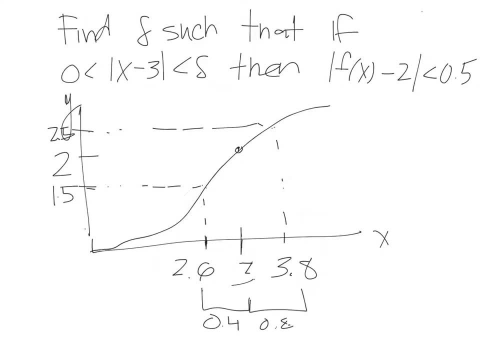 0.8. so what would our delta be? what we need to do is find a delta that guarantees if we're within that width- so if we're in some region, then the y values will also be in that region. so what we want to do is we want to pick the smallest. 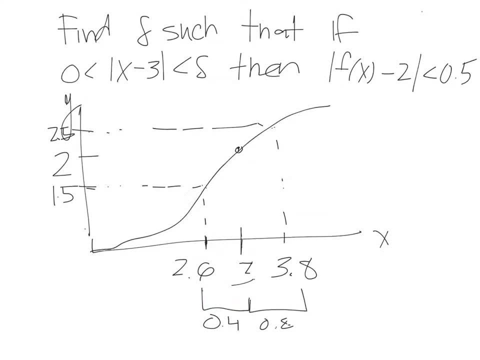 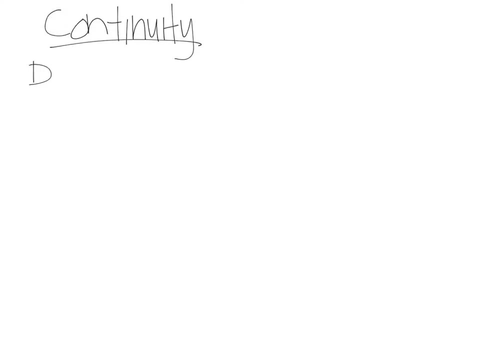 region and that's what our delta would be. so we would say delta is equal to 0.4. in this section we're going to talk about continuity, so we'll begin with definition. definition a function, f is what we say. is what we say: continuous at a number a. 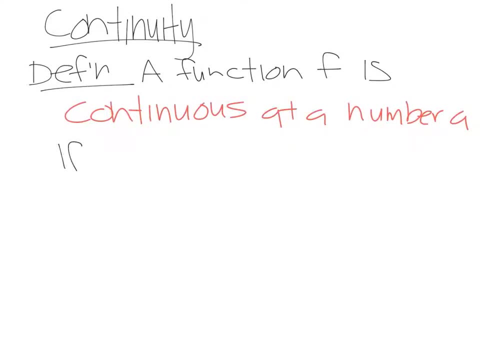 if the following: the limit as x approaches a of f of x equals f of a. so it's continuous. if the limit is equal, the limit as x goes to a is equal to f. at that point. a notice that we're assuming three things. first of all, that f of a is in fact defined. 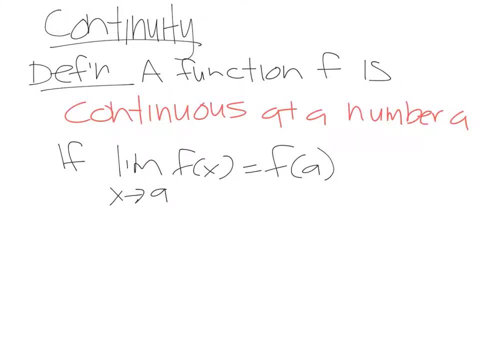 meaning it's in the domain. second, that the limit as x goes to a of f of x exists. and finally, we're assuming that the limit as x goes to a of f of x is equal to f of a. we also have, as another definition: 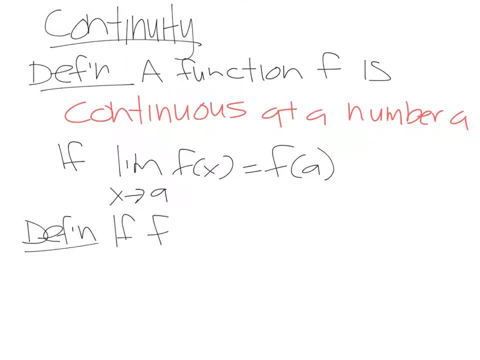 if f is defined as near a, we say f is discontinuous at the point a. if if is not, is not continuous, is not continuous at a meaning right here that the limit as x goes to a of f of x does not in fact equal f of a. so this Puisque describes this method we're using: using f of a to characterize f of x and that f of x as a slight difference: incity of x, that limit as x goes to a of a is not in fact equal f of a, meaning right here that the limit as x goes to a of f of x does not in fact does not in fact, equal foa. 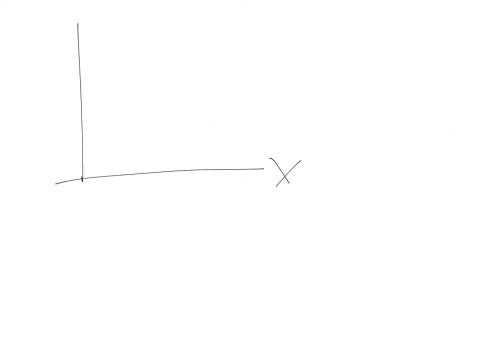 so improvement. both points. well, at the point a: if, if, So, if we have a graph that looks something like this: this is continuous at all these points, except right here, at this value. It's not continuous, so it's discontinuous, right here. 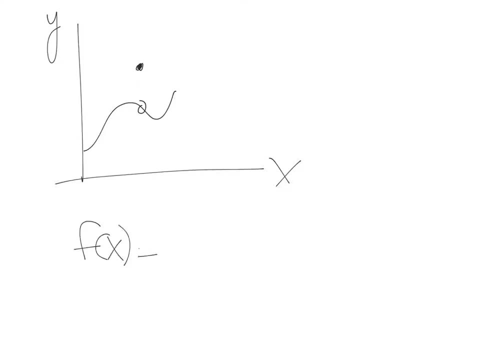 We might even have a function. say f of x is equal to x squared minus x minus 2 divided by x minus 2.. Well, if x is equal to 2, we'd have 0 in the denominator, and that's not possible. 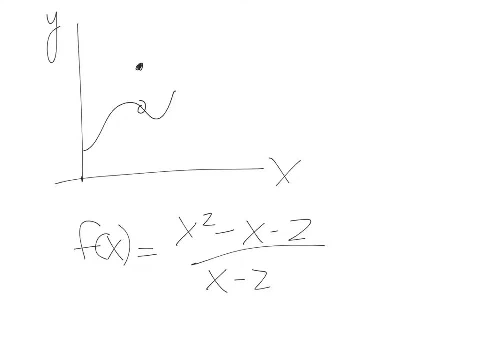 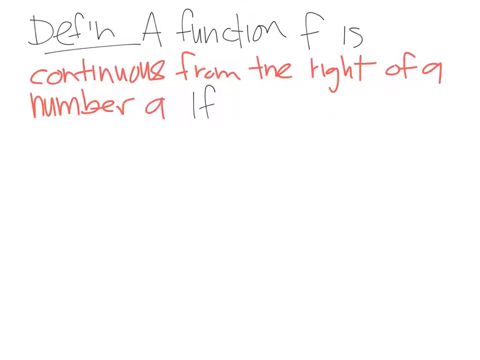 So x cannot equal 2.. Therefore it's discontinuous. at that point x equals 2.. Okay, Now we have another definition, and this definition says that a function f is continuous from the right to the left. So we have a function f of a number a if we have the following: 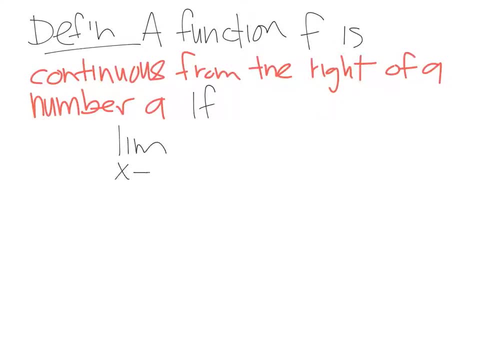 The limit as x approaches a from the right side of f of x is equal to f squared minus 2.. F of a, F of a, F of a And f is what we say with the next definition: F is continuous. F is continuous. 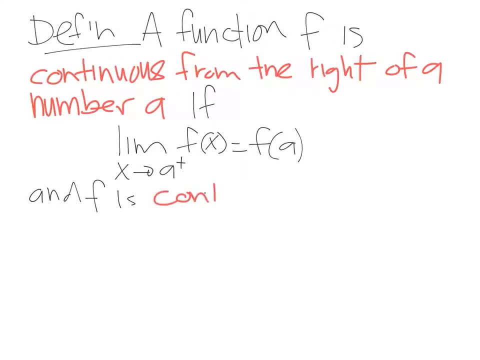 From the left of f, From the left, From the left, From the left And from the left, And from the left From the left, a number a. if we have that, the limit as x approaches a from the left side of f is equal. 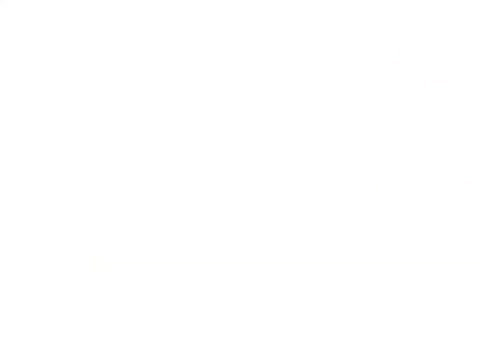 to f of a. so, graphically, what this might look like is, if we have a graph like this and we have something like that, and that's our point a, this is our function. f of X. well, if we look at f of X from the right side, it is equal to f of X is equal to the right-hand limit, and so, therefore, 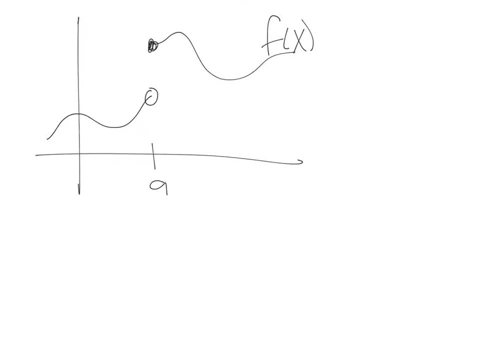 this graph would be continuous from the right at some number, at this number a. similarly, if we had a graph that looked like something to this effect: well, there and then below- we do that- then this would be continuous from the left of some number a. we have another definition, and this states that a function f is continuous. 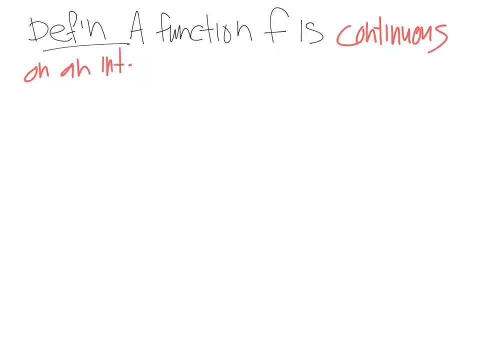 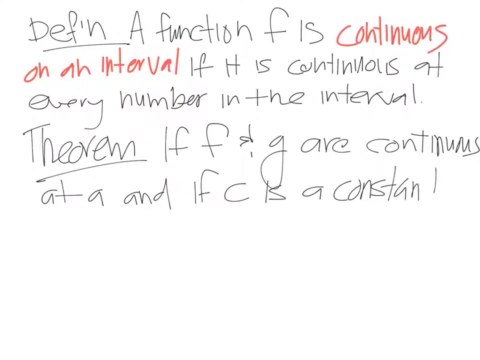 on an interval if it is continuous at every number in a, the interval. now we have a theorem. this theorem states that if f and G are continuous at the point a and if the value C is a constant, then the following functions are also continuous at a. f and g are continuous at a. 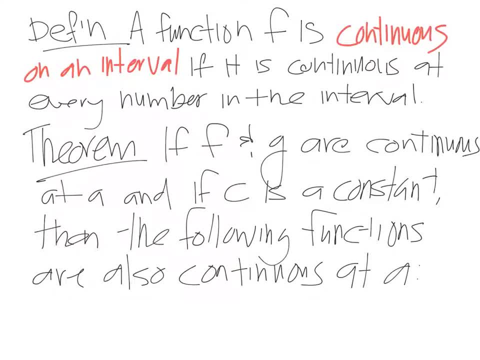 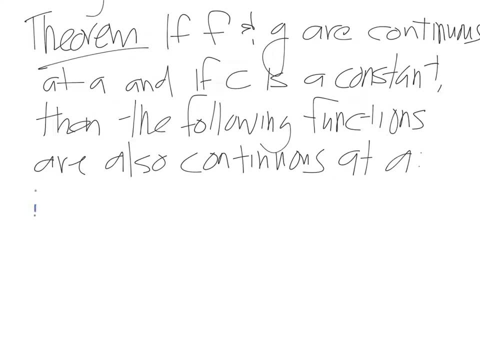 let's get back to our equation for continuous in: 1, f plus g will also be continuous. 2, f minus g will be continuous. 3, the constant c times f is continuous. 4, we have the product f times g and 5, we have the quotient f divided. 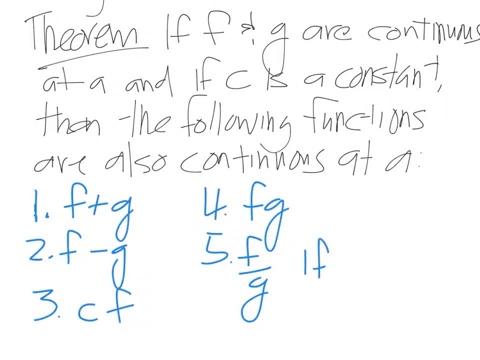 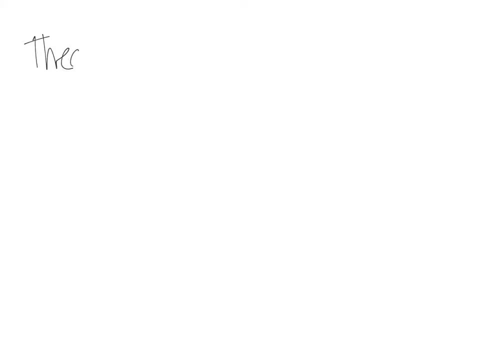 by g is also continuous, and this is if we assume that the denominator g evaluated at the point a is not 0.. Now we have another theorem, And this theorem states two things: a- any polynomial is continuous everywhere. that 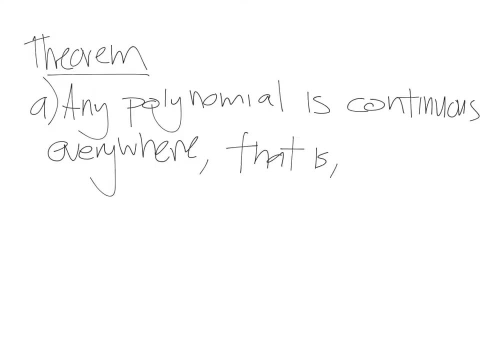 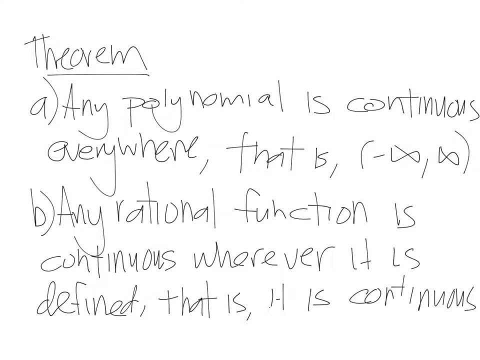 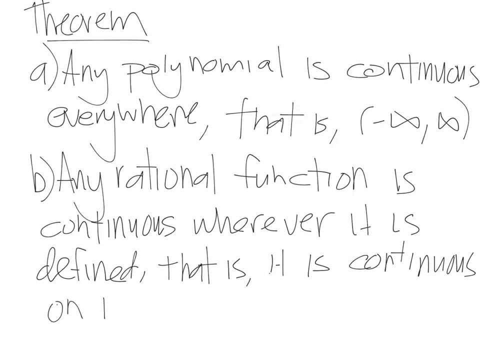 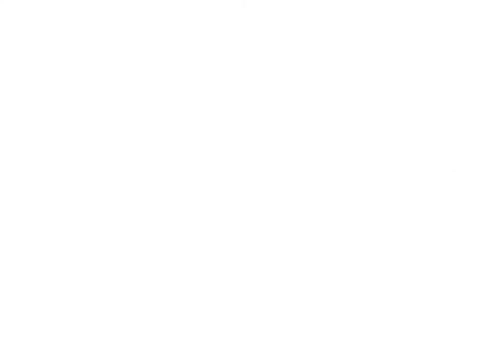 is is continuous from 0. From negative infinity to infinity on the interval. Second part of the theorem states that any rational function is continuous wherever it is continuous, That is, it is continuous on its domain. So let's take a look at an example. 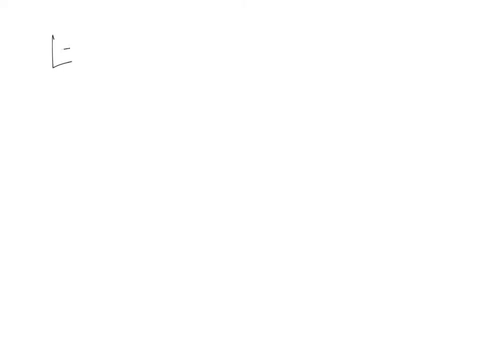 Find the limit as x approaches negative, 2 of the quantity x cubed plus 2x squared, minus 1, all over 5 minus 2x squared. Well, this is a rational function. and taking a look at this rational function, what's its? 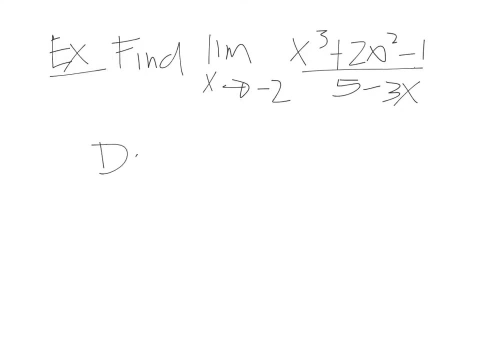 domain, Well, the domain of this is all real numbers, except when the denominator is 0, so, except when x equals 0. Okay, Okay, Okay, Okay, Okay, By 5 thirds. And if we look here, we found this limit: when x goes to negative, 2, well, negative. 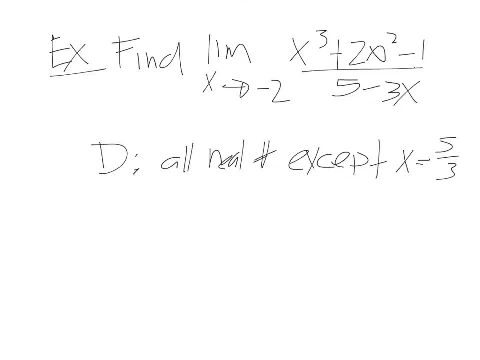 2 is in the domain. So now what we can do with this limit is that if we define the function f of x to be this whole x cubed plus 2x, squared minus 1.. divided by 5 minus 3x, and if we're trying to calculate the limit as x goes to negative 2, 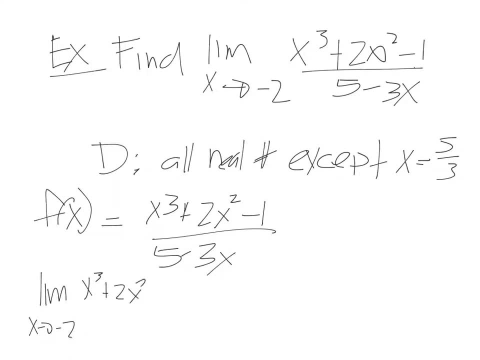 of x cubed plus 2x, squared minus 1 over 5 minus 3x. this is just the same as the limit, as x goes to negative 2 of f of x, but we know that negative 2 is in the domain of this. 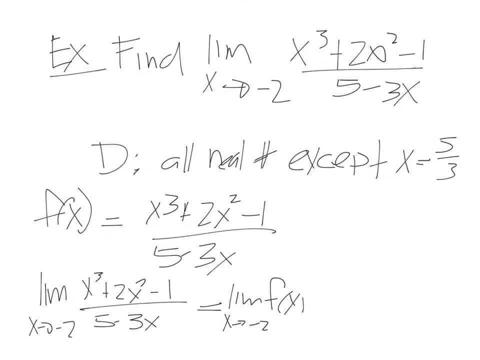 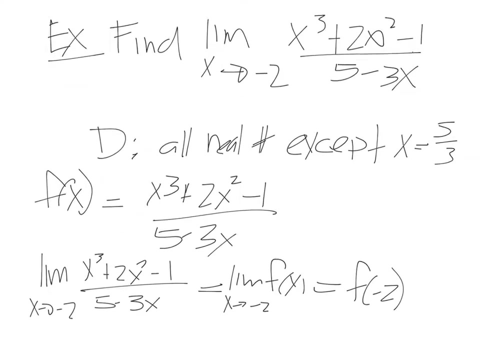 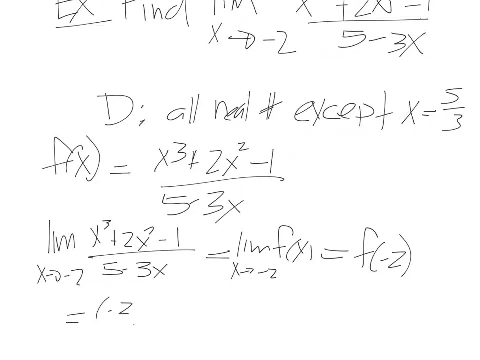 function f of x, because the only thing that's not in the domain is 5 thirds. so therefore we can write it as just simply f of negative 2.. And what is f of negative 2?? Well, we plug that in and that would be negative 2 quantity cubed plus 2 times negative 2 squared. 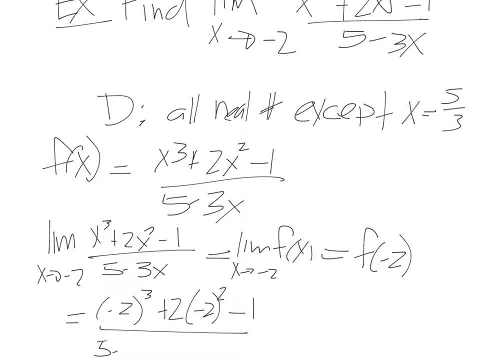 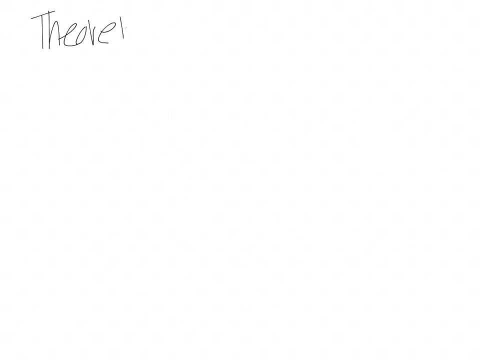 minus 1, all over 5, minus 3 times negative 2, and, simplifying this, what we get is negative 1 over 11.. We next have a theorem that states the following: The following types of functions are continuous at every number in their domains: 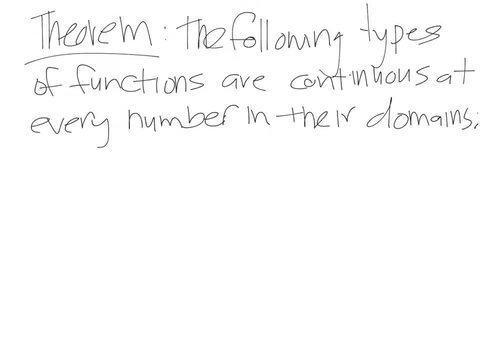 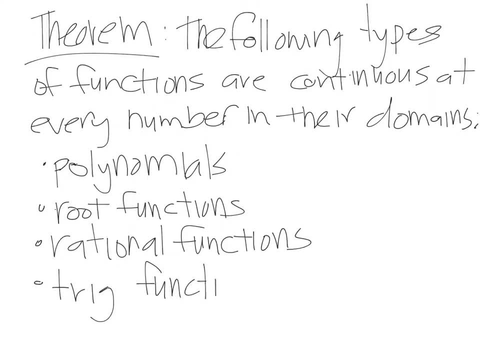 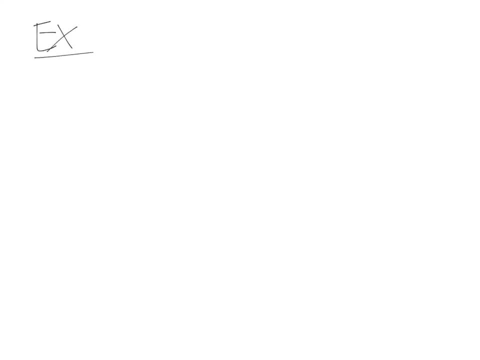 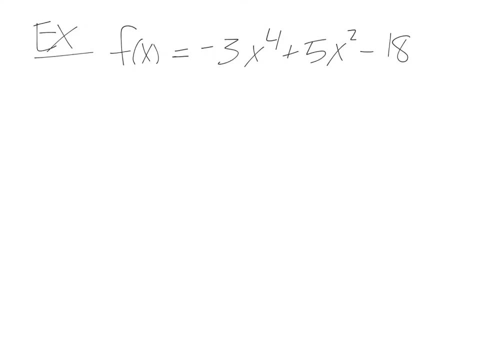 and so, because it's a polynomial, it's defined everywhere and so it's continuous everywhere by this previous theorem. so it is continuous on the interval. so continuous on the interval, negative infinity to positive infinity. what about you do another example, and let's call this g of x and let's do a rational function. so let's do 3x squared, minus 7x plus 11 divided. 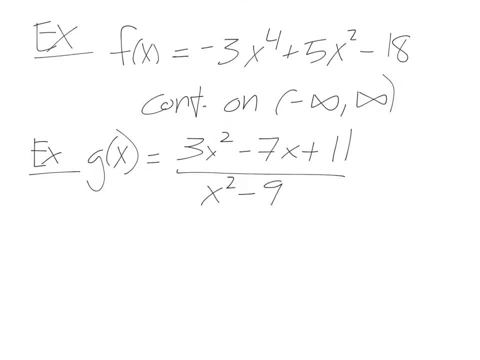 by x squared minus 9. well, we want it to be. it'll be continuous anywhere in its domain, so it's the domain of this. well, since we're dividing by something, we can't have the denominator equal 0, and so the domain is all numbers in, except when X is 3 or negative 3. 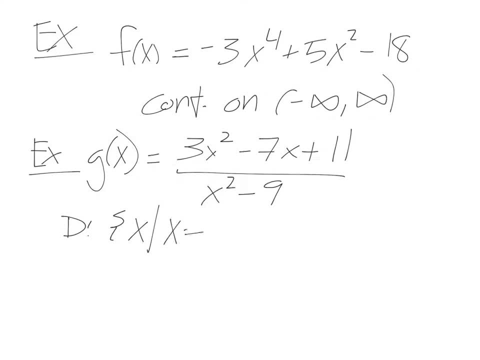 so all values X, such that X cannot equal plus or minus 3, and therefore it would be continuous for every number, except for positive or negative 3. so we would write that as negative infinity to negative 3, negative 3 to 3 and then 3, all the way on. 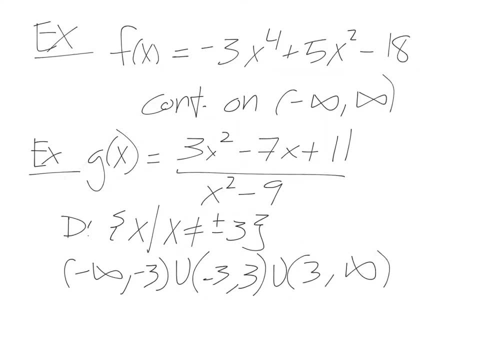 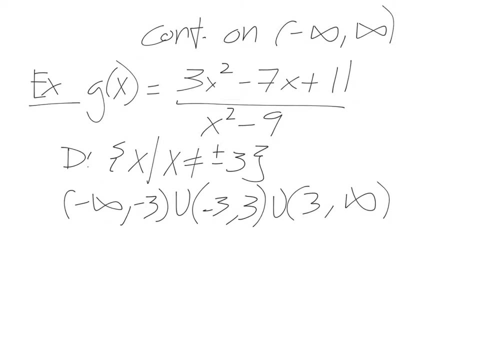 to infinity. this includes all numbers except for 3 and negative 3. and finally, we'll do one more example, and so here we have fg. we'll call this function h of x, and so h of x is the square root of x plus x plus 1 over. 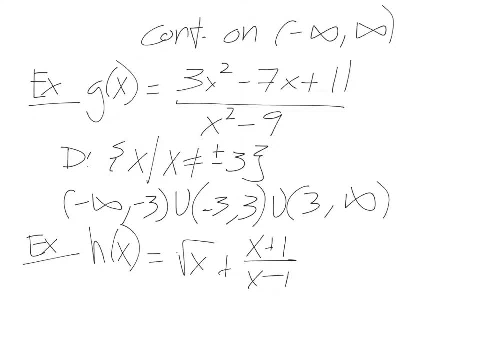 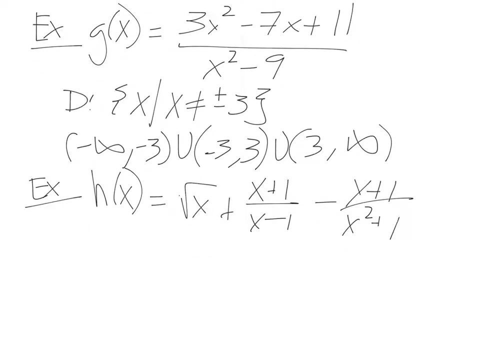 x minus 1 minus x plus 1 over x squared plus 1. and so well, what is the domain for this function? what we see here is we have. we can break this down into three smaller functions by our previous theorem. if we define, let's say: 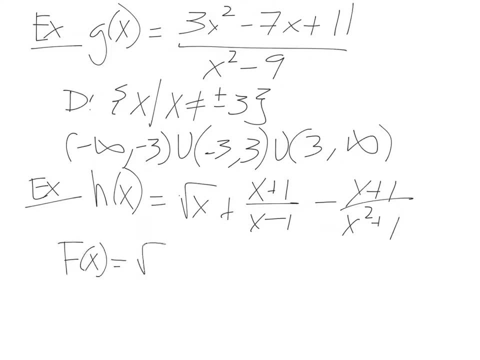 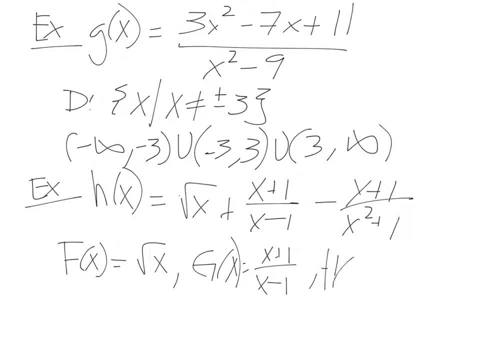 to be x plus 1 over x minus 1. capital h of x is x plus 1 divided by x squared plus 1. then we just need to figure out what are the domains for each of these. well, the domain for f of x, capital f of x. 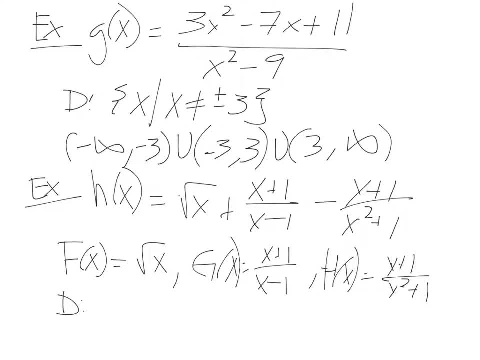 is all real numbers greater than or equal to 0. greater than or equal to 0. we cannot have 0 in the square root. so this is 0 to infinity. the domain for the second one, it's all real numbers except for negative 1, so really this is negative infinity. 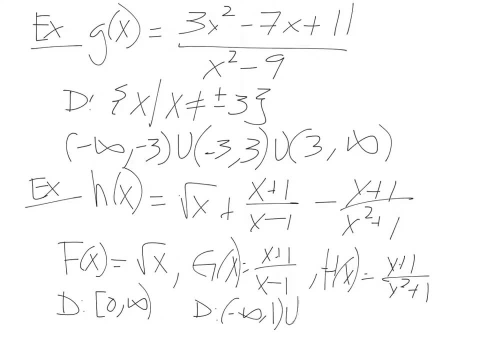 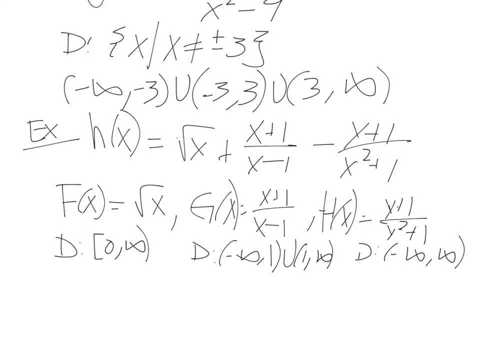 or positive 1. so negative infinity to 1, union 1 to infinity. and this last one it includes. we would never be divided by 0, so our domain is all real numbers, negative infinity to infinity. so we have these three, combining them, what we end up with 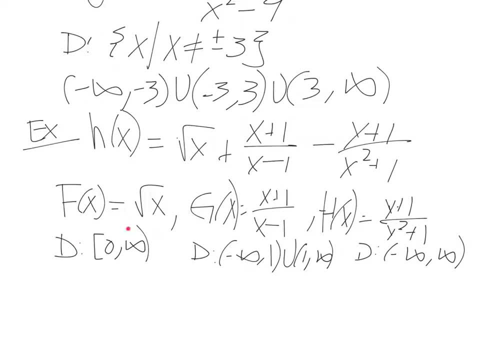 is, we have to make sure that it's not negative, so we have to include this. but we also know that it cannot include the point 1, so we get for our our domain and therefore the interval where it's continuous is 0 and therefore we have to include the point 1. 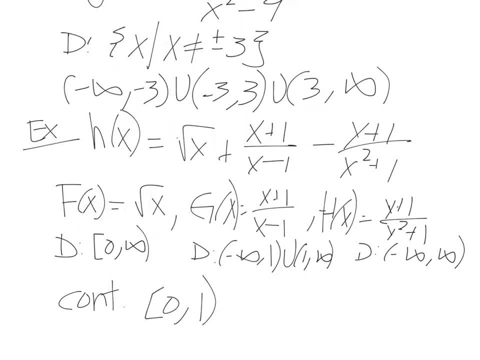 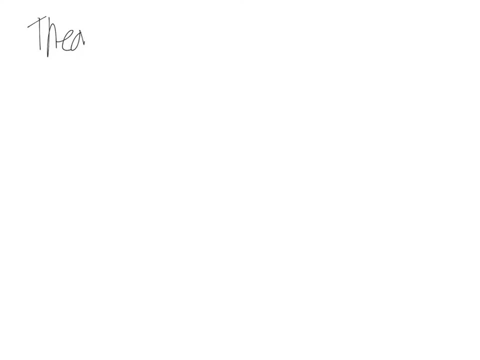 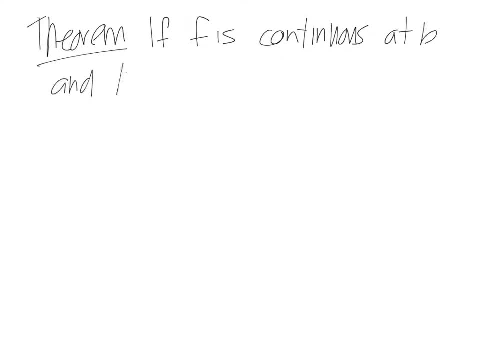 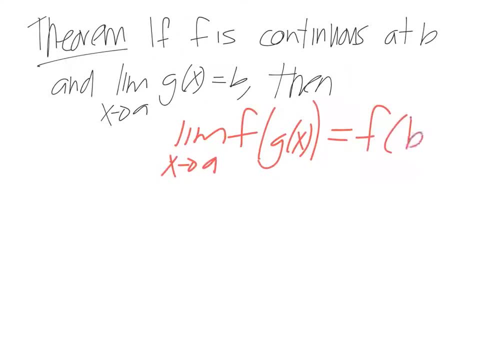 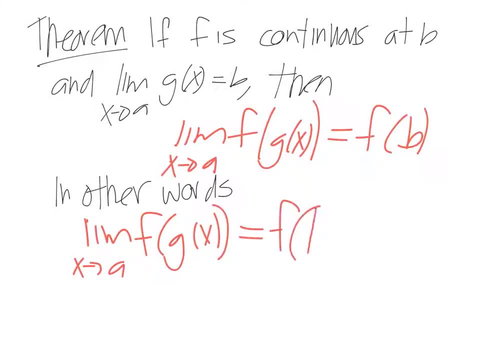 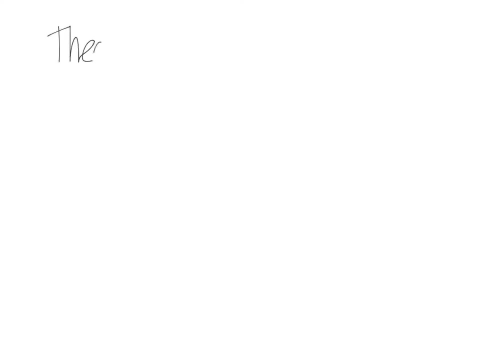 of f of g of x of f of g of x of f of g of x. this is equal to f of the limit as x approaches a of g of x. we have another theorem, and this theorem states that if g is continuous at the point a, 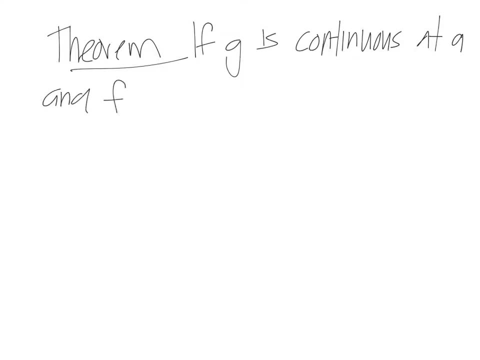 at the point a of g of x and our function f is also continuous at the point g of a. then composite function given by a function of g of a and f of g of x equals f of g of x. This is continuous at a. 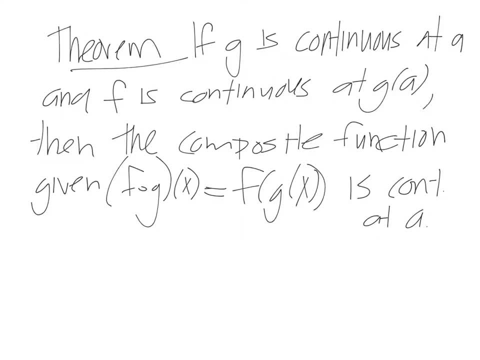 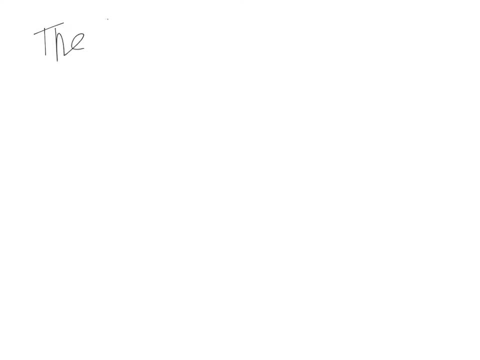 And finally we have one last theorem left to go. So this theorem is a big theorem and it has a name. This is called the Intermediate Value Theorem. And what this Intermediate Value Theorem says is: suppose f is continuous on g of x. 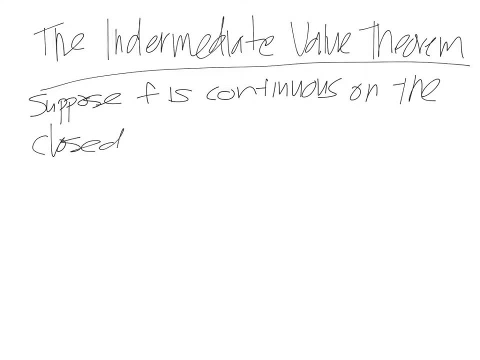 With the Gross 멋 ability. f of x is continuous on the closed interval a to b And let capital N be any number between f of x and cancelled degrees. Any number between f of n and closed interval. any number between f of x and closed interval. 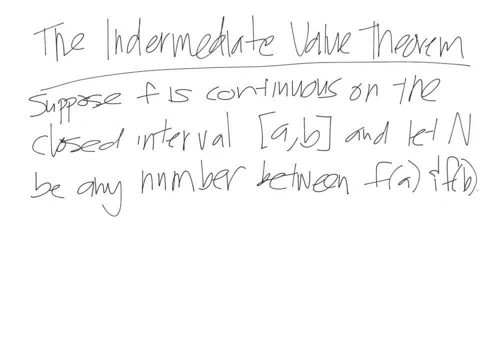 and closed interval f of a and f of b. where f of a does not equal f of b, Then there exists a number c in the interval a to b, such that f of c equals n. So I'm going to actually draw this out for you. 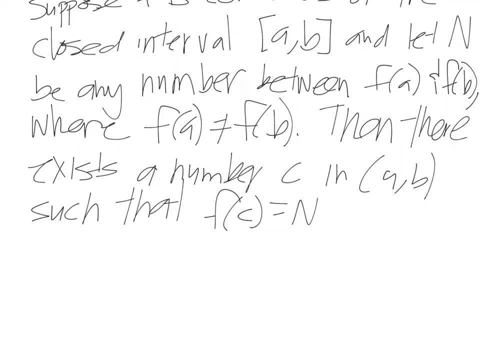 So that it might be a little bit more clear. So we're going to have an axis, so we have x, we have y, we have our function f of x. So if we have a point a right here and then over here we have the point b, 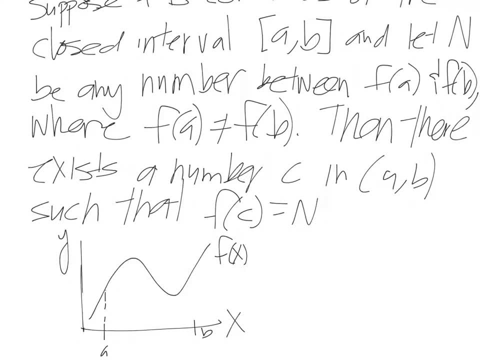 Okay, So we bring this up, we get f of a, we have f of b right here, and then we're assuming that n capital N is between f of a and f of b, So let's call that n, right there. 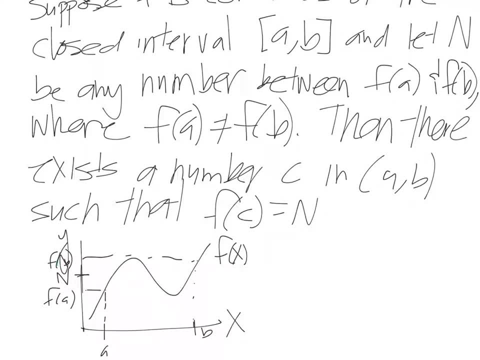 What this says is that there exists some point c where c falls somewhere between a and b, such that f at that value is equal to c. Well, looking right here, right there, that's one possible value for c, and we'll call that. 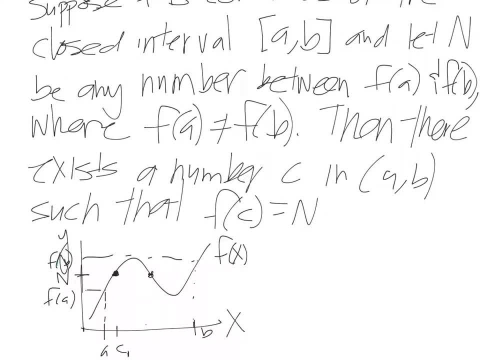 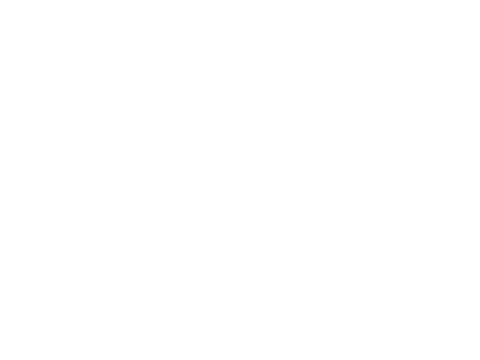 c1, because we have another point that could have been c, or even another point that could have been c. But as long as there's one, Okay, Okay, Okay, Okay. The intermediate value theorem is used often when you're trying to find the root or show. 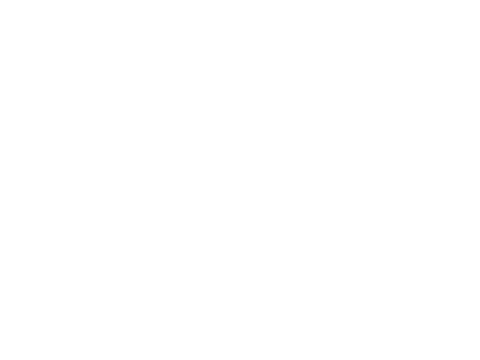 at least that a root of an equation exists. So if we have some function, f of x is equal to 4x. cubed minus 6x. squared plus 3x minus 2 equals 0.. And I asked you to show that there. 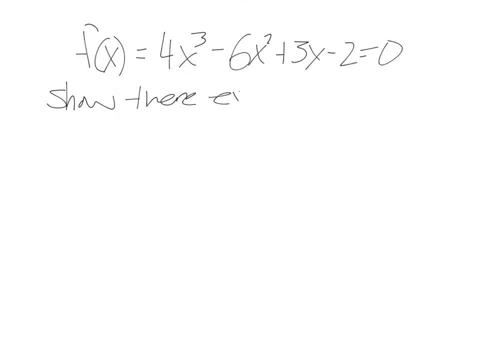 is, exists a root, or in other words a zero, between 1 and 2, what we would first do is calculate what is f of 1.. Well, f of 1, plugging this in, we get 4 times 1 cubed minus 6 times 1 squared plus 3 times. 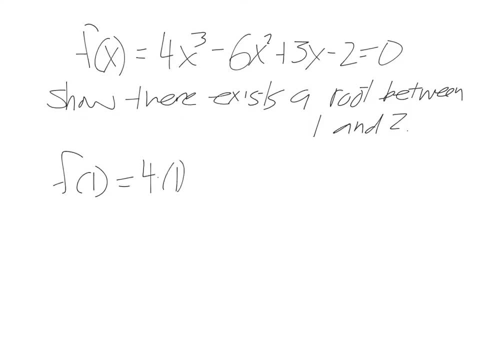 1 minus 2.. So 4 times 1 cubed minus 6 times 1 squared, plus 3 times 1 minus 2, that's a minus And we end up with this as negative 1.. And we all know negative 1 to be less than 0.. 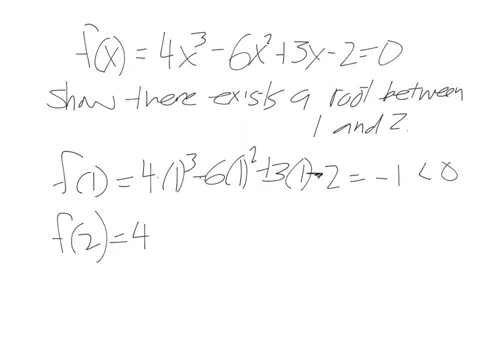 F of 2,. well, this is 4 times 2 cubed minus 6 times 2 squared, Plus 3 times 2 minus 2.. And this is 12, which is greater than 0.. And so that capital N that we dealt with, we know that we'll call that capital N, the. 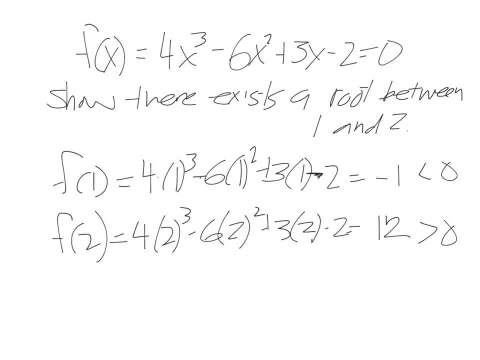 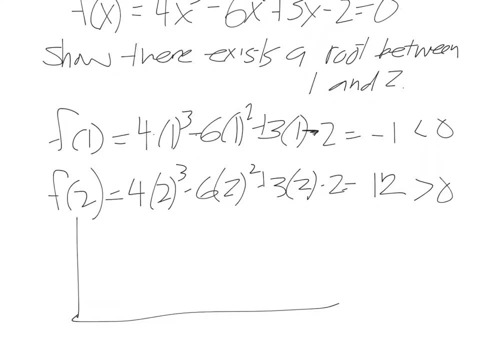 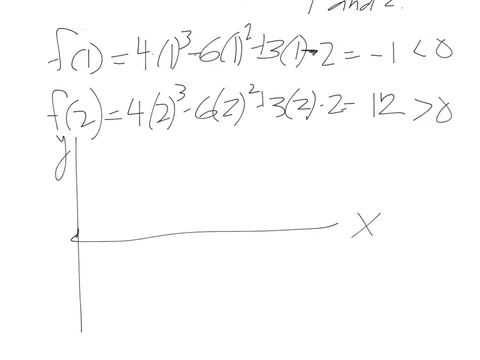 point 0.. So what we have is something like this: Okay, Okay, So we have something like this. So this is our x-axis and this is the y-axis, And we know, when x is 1, we're negative. we're somewhere down here below the axis. 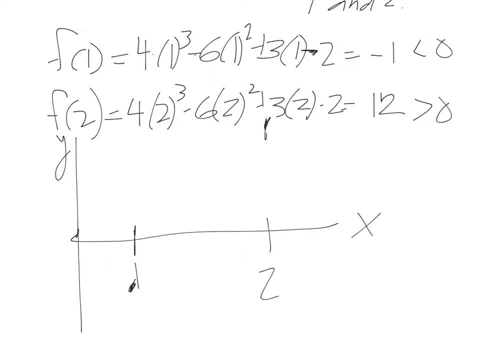 But then when x is 2, we're above the axis, And this is a polynomial function, so we know it's continuous. So in order to get from below the axis to above the axis, you have to cross somewhere between 1 and 2.. 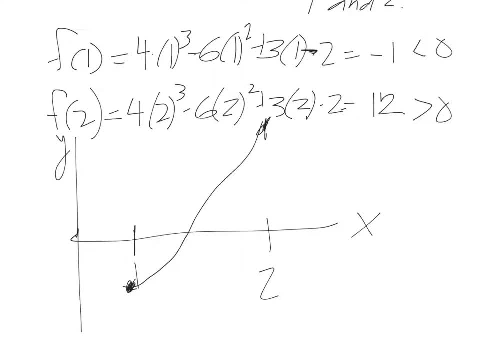 To get from below to above, you have to cross the axis. Now I'm not saying exactly where it is. All this says is that it crosses the axis somewhere between negative 1 and 2.. Who knows, It might cross many times. 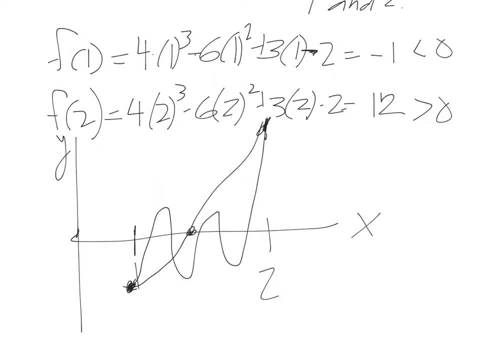 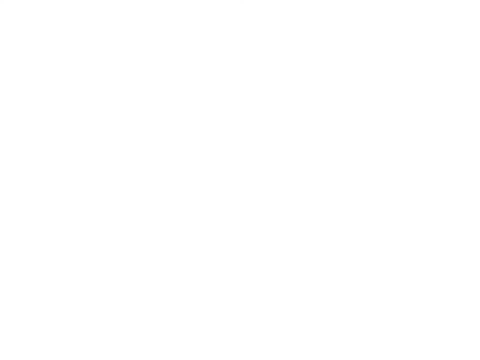 But we're just trying to show that there exists at least one crossing in that interval. Now we're going to shift gears a little bit and talk about volatilities. So we're going to say that f is the position of an object. Now when you think of velocities, you might think about, you know, moving in a car. 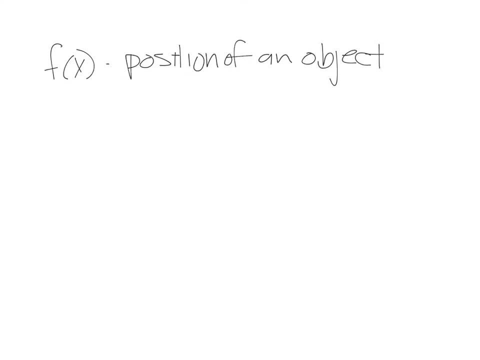 And the speed limit is given by miles per hour or distance over time. so we would say that the average 1. Velocity is equal to displacements over time, which in this case would be f of a plus h minus f of a all over time. 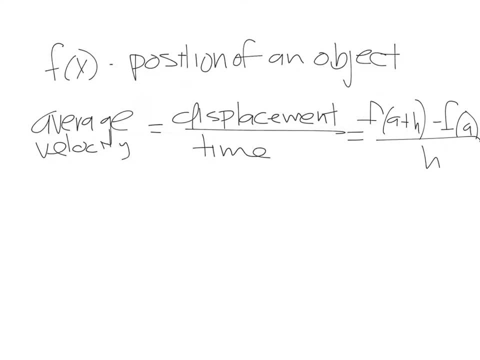 H: 1. 1., 1., 1., 1., 1. 1.. But, as you know, if you're driving in the car, your speed or your velocity changes constantly, And so if you want to find the instantaneous velocity, we're going to say that, the instantaneous 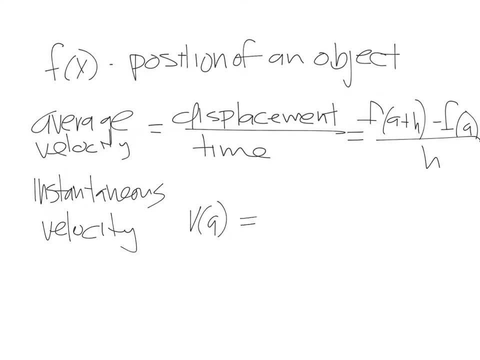 velocity is given by v and that's going to be, as time gets, smaller and smaller, So not averaged over your whole time span, but almost instantly. So as you change the time it becomes very, very small, or the limit as that gets closer. 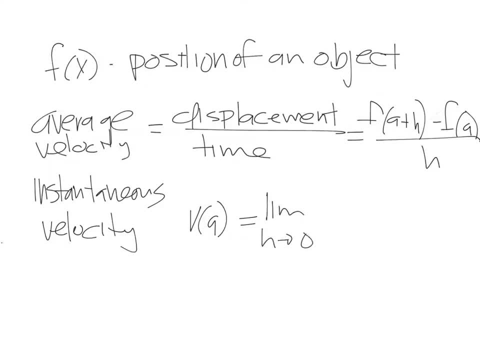 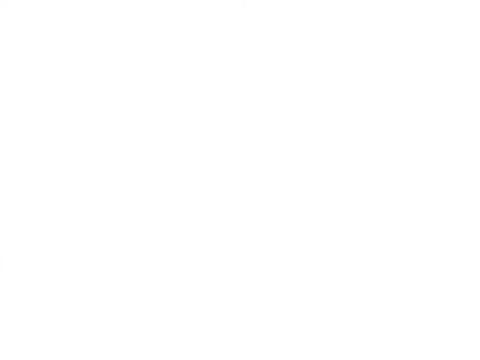 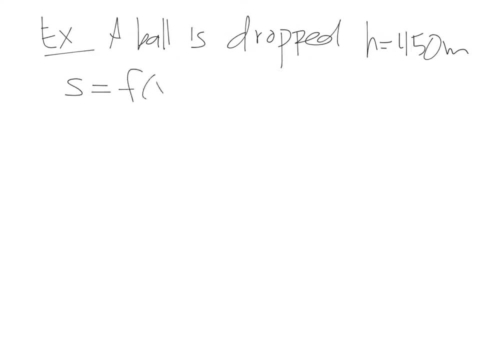 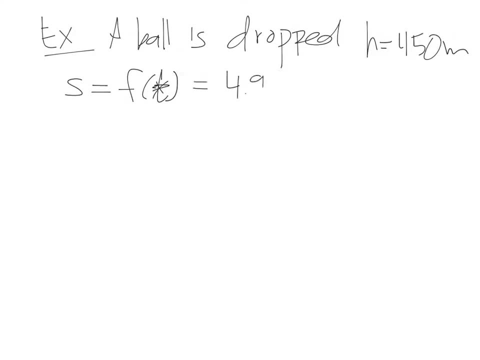 or f of x or f of t, rather, or f of x or f of t, rather, for time, for time, for time, And this is 4.9 times t squared, And this is 4.9 times t squared. 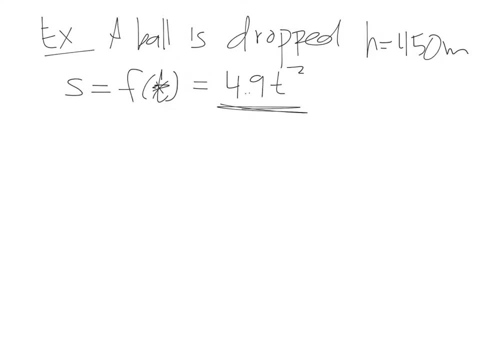 And this is 4.9 times t squared. So this right here is something, So this right here is something, So this right here is something that we will be given, that we will be given that we will be given Now to find the velocity. 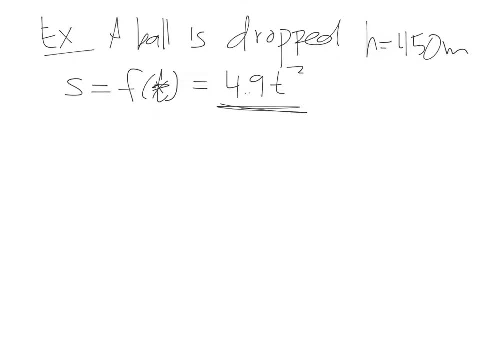 Now to find the velocity. Now to find the velocity after 5 seconds, after 5 seconds, after 5 seconds. we need to figure out the velocity, we need to figure out the velocity. we need to figure out the velocity. v of t is going to be the limit. 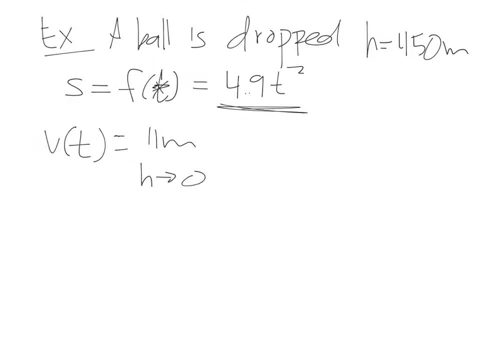 v of t is going to be the limit. v of t is going to be the limit, as h goes to 0 of our f of t plus h. as h goes to 0 of our f of t plus h. as h goes to 0 of our f of t plus h minus f of t divided by h. 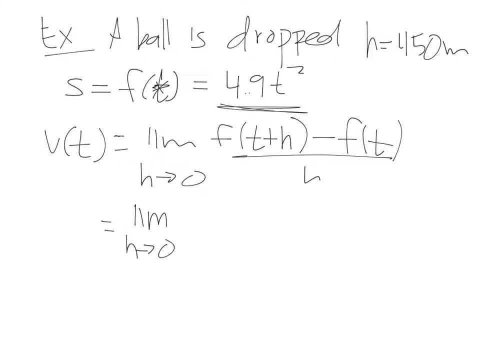 minus f of t divided by h, minus f of t divided by h. So this is the limit. So this is the limit. So this is the limit. as h goes to 0, of f of t, as h goes to 0, of f of t. 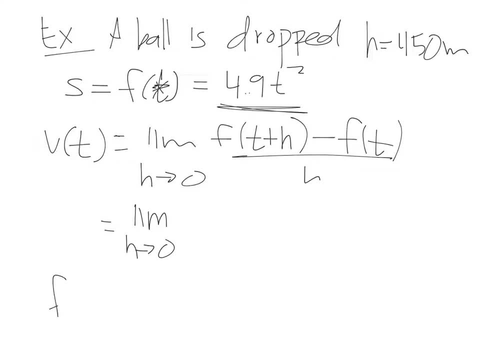 as h goes to 0, of f of t plus h plus h plus h. So again, we'll do that right down here. So again, we'll do that right down here. So again, we'll do that right down here. So this is f of t plus h. 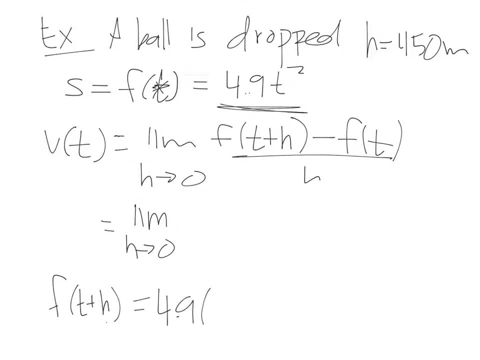 So this is f of t plus h. So this is f of t plus h, which is going to be 4.9 times, which is going to be 4.9 times, which is going to be 4.9 times the input squared. 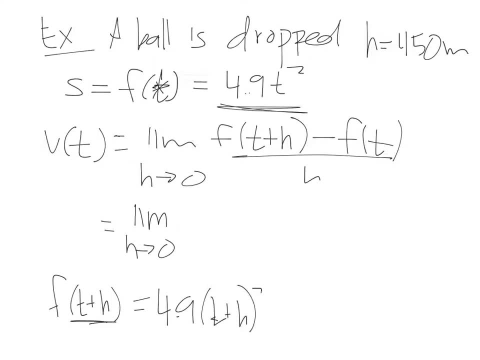 the input squared. the input squared So 4.9 times t plus h. So 4.9 times t plus h, So 4.9 times t plus h. quantity squared: quantity squared: quantity squared, which is equal to 4.9 times t squared. 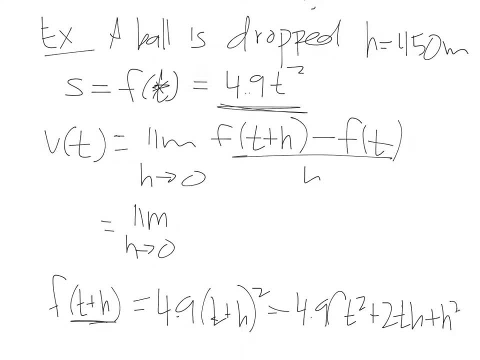 which is equal to 4.9 times t squared, which is equal to 4.9 times t squared plus 2th plus h squared, plus 2th plus h squared, plus 2th plus h squared. So plugging that in, we get. 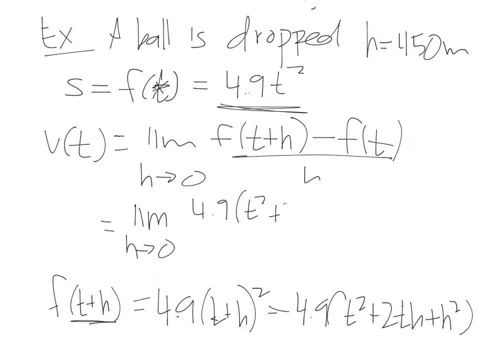 So plugging that in, we get. So plugging that in, we get 4.9 times the quantity t squared. 4.9 times the quantity t squared. 4.9 times the quantity t squared plus 2th, plus h squared. 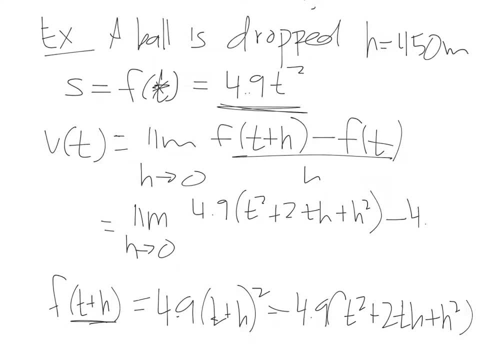 plus 2th plus h squared, plus 2th plus h squared, then minus f of t, which is then minus f of t, which is then minus f of t, which is 4.9 times t squared all over h. 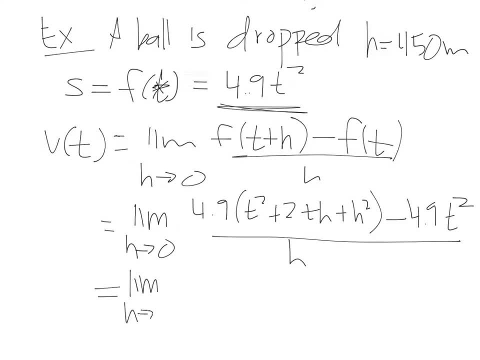 4.9 times t, squared all over h. 4.9 times t squared all over h. So this becomes the limit, So this becomes the limit, So this becomes the limit, as h goes to 0, and everything has. as h goes to 0, and everything has. 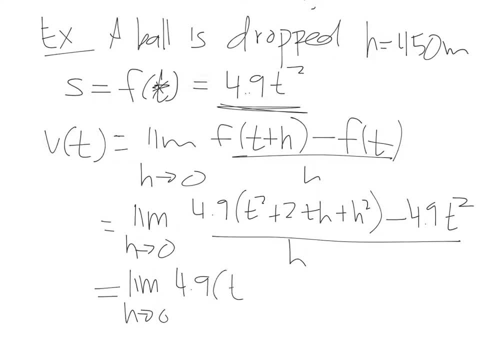 as h goes to 0, and everything has 4.9, so I can factor out 4.9- 4.9,. so I can factor out 4.9- 4.9, so I can factor out 4.9 from the numerator, and so we get. 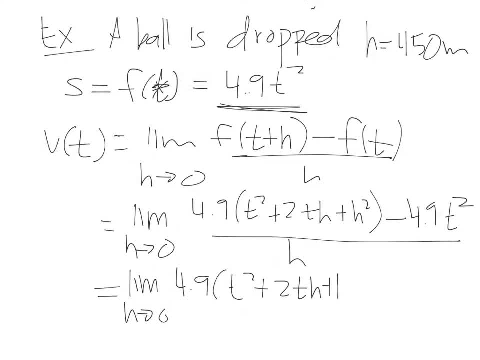 from the numerator, and so we get from the numerator, and so we get t squared plus 2th plus h squared. t squared plus 2th plus h squared. t squared plus 2th plus h squared minus, since we factored out the 4.9,. 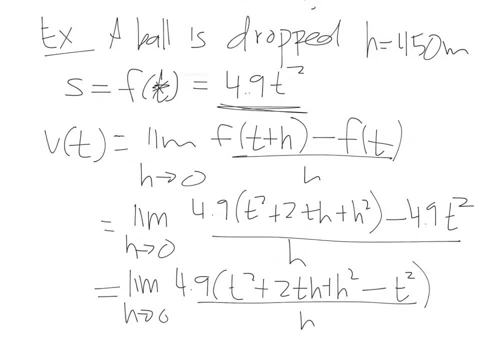 minus, since we factored out the 4.9,. minus since we factored out the 4.9,. we're just left t squared over here. we're just left t squared over here. we're just left t squared over here, all over h, and now our t squareds. 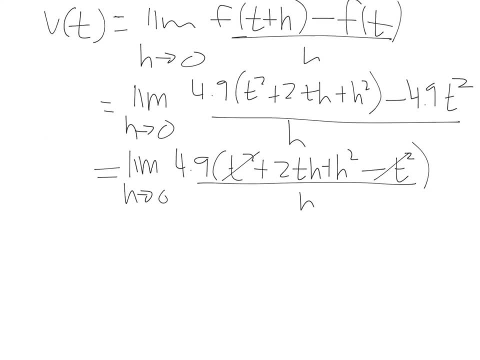 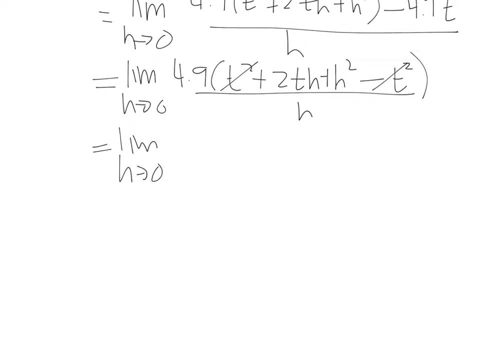 all over h, and now our t squareds. all over h, and now our t squareds- cancel. so moving this up. we get cancel. so moving this up, we get cancel. so moving this up. we get the limit as h goes to 0 and notice. 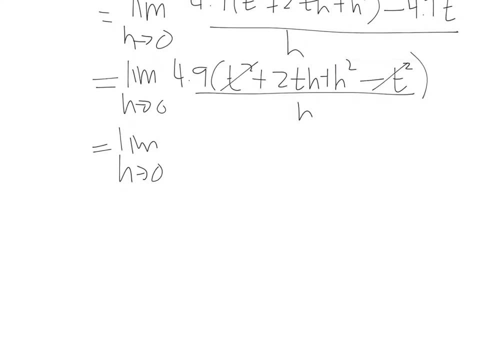 the limit as h goes to 0 and notice the limit as h goes to 0 and notice that each term has an h in it, that each term has an h in it, that each term has an h in it, so we can factor out the h. 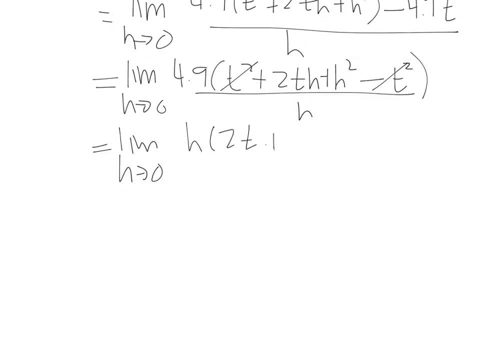 so we can factor out the h. so we can factor out the h. so we get h times the quantity. so we get h times the quantity. so we get h times the quantity 2t plus h, 2t plus h, 2t plus h, all over h, and our h is now cancel. 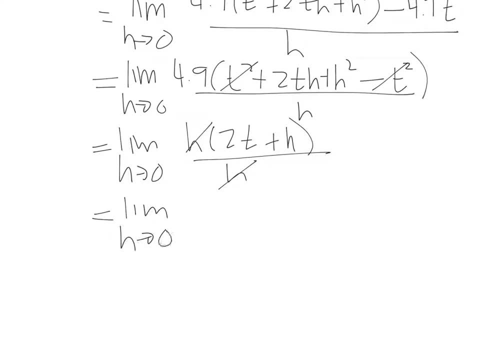 all over h and our h is now cancel. all over h and our h is now cancel. and so this is the limit. and so this is the limit, as h goes to 0 of 2t plus h. and now, since we don't have an h in the denominator, because we had an h, 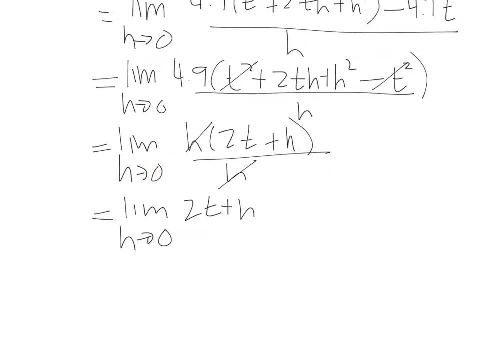 denominator over here. we couldn't evaluate it when h went to 0 because we'd be dividing by 0, but we don't have that problem anymore. so this is just 2t plus 0, or just 2t. excuse me, i forgot. we had the 4.9 this whole time, so this is 4.9 times all this. 4.9 times all that. 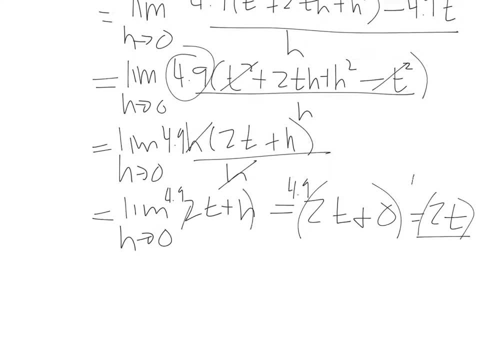 4.9 times all that and 4.9 times all of that, which means this is going to be 9.8 times t. so this is a progressive property and as we solved this last category we get, v of t is 9.8 times t, and if we're 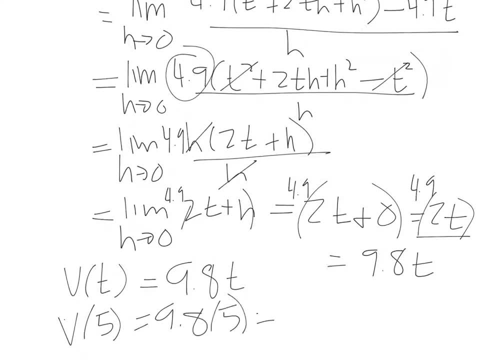 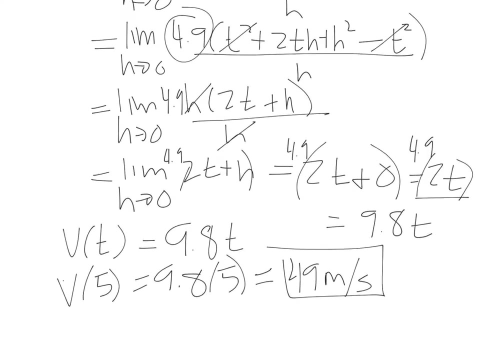 trying to find the velocity after the ball dropping for five seconds. this is 9.8 times five. plugging this in, we get that this is going to be 49 and we're doing in meters per second. What is the time when the ball hits the ground? 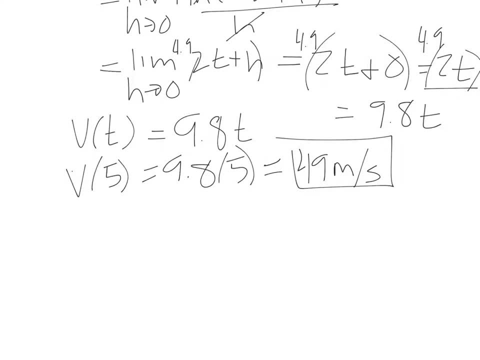 Well, we would need to figure out time. So recall the position vector is gonna be: f of t is equal to 4.9 t squared. That's a t, not an x. So f of t is 4.9 t squared. 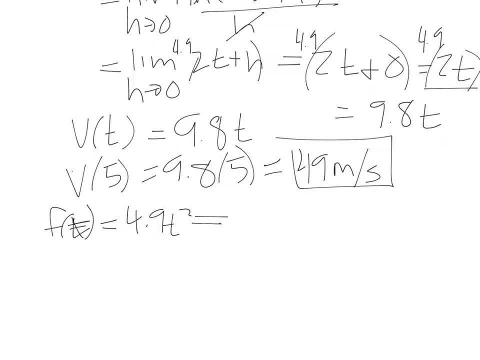 We wanted the position to be on the ground, so it will have traveled 450 meters, And so this is just a problem that we can solve, And so we solve this. we get t squared is 450 over 4.9, which means that t is approximately 9.6 seconds. 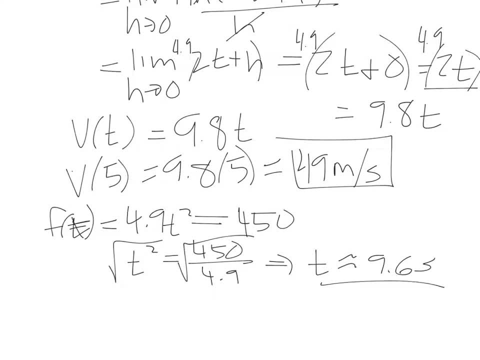 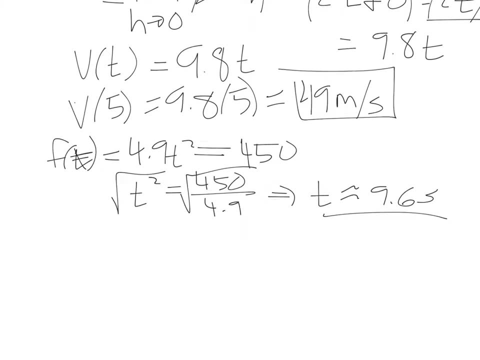 by taking the square root of both the square root and the square root. So it hits the ground after 9.6 seconds. Well, what's the speed when it hits the ground? What's its velocity? Well, the velocity when it hits the ground. 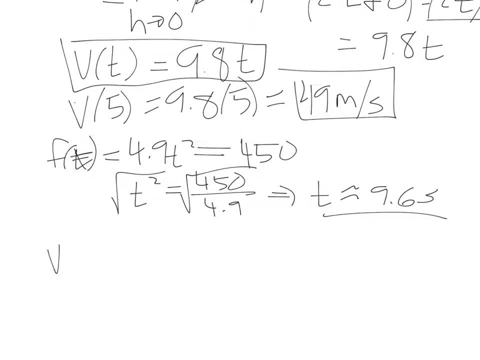 we just use this formula that we found: V of t is 9.8 times our time, 9.6.. And so we get that this is about 98 meters per second. So if you drop the ball at 450 meters above the ground, 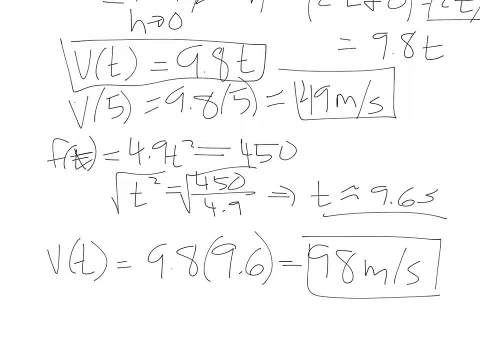 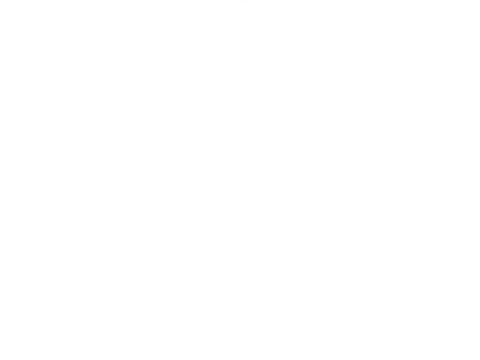 and you let it fall. when it hits the ground, it'll be traveling and hitting the ground. excuse me, this is 94 meters per second. It'll hit the ground at 94 meters per second. Now we have another definition And we say that the derivative 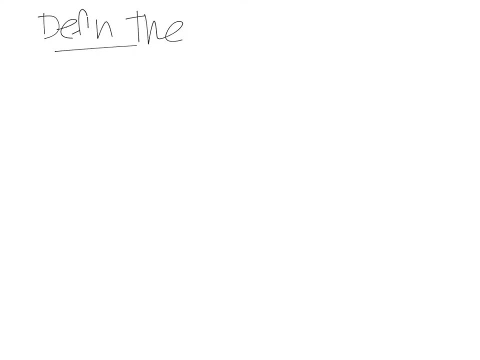 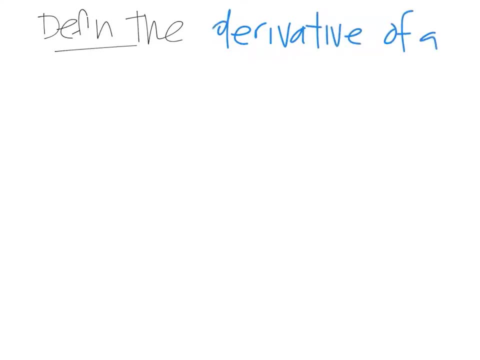 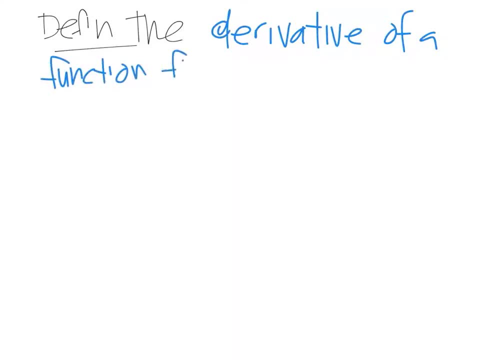 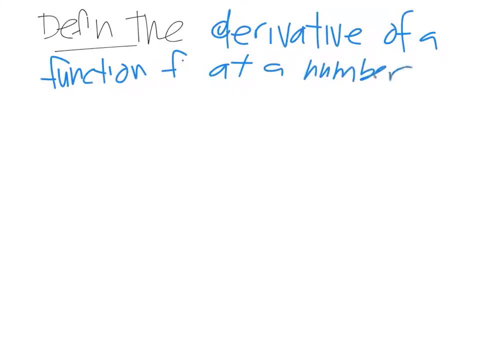 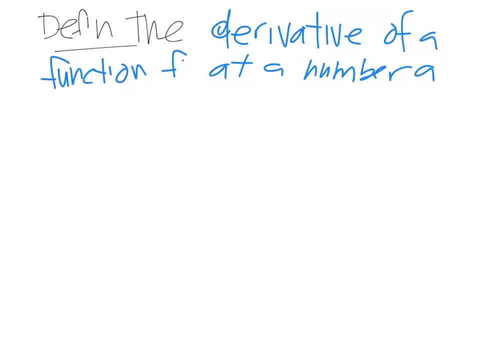 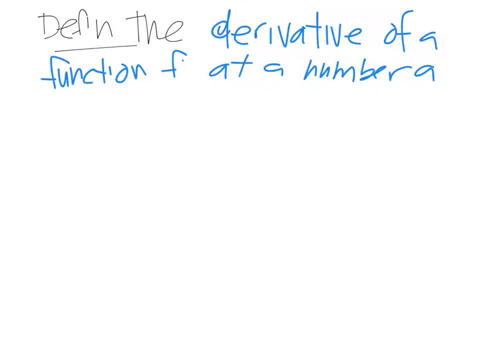 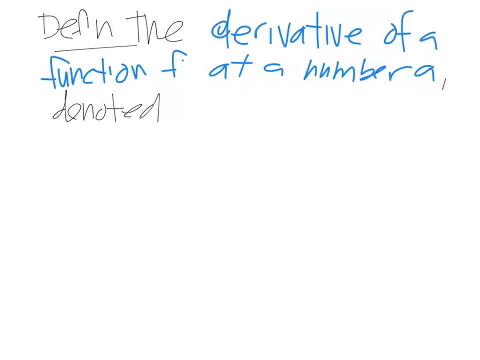 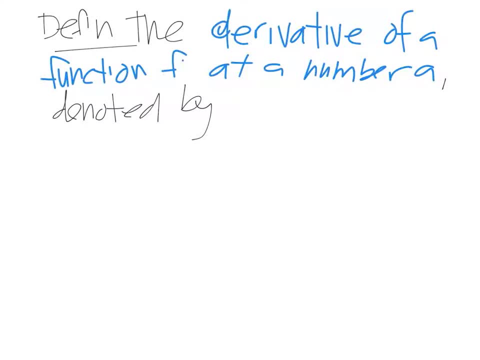 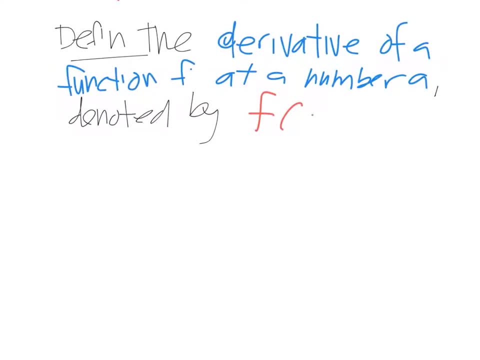 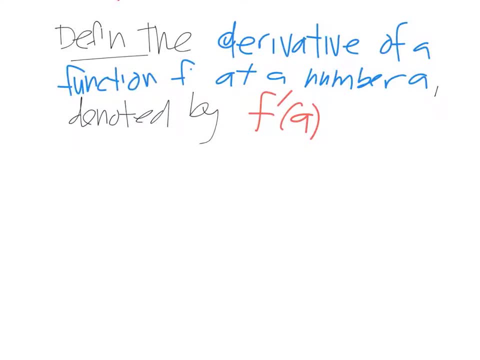 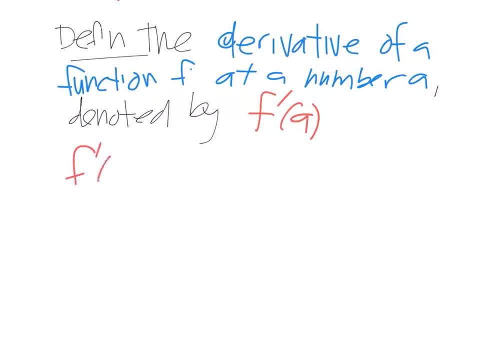 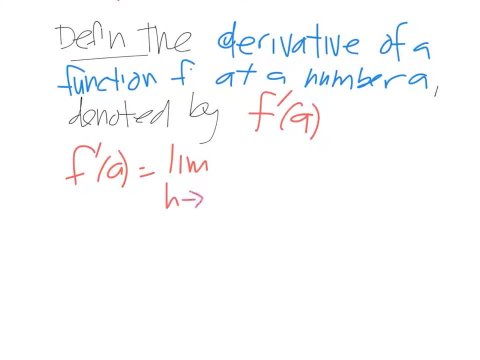 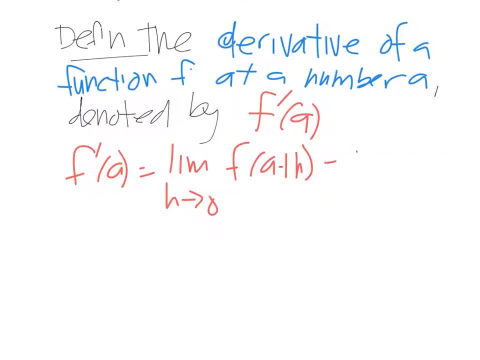 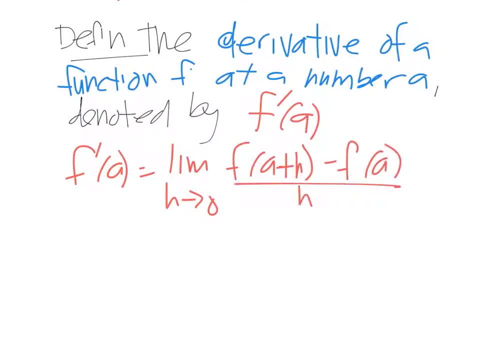 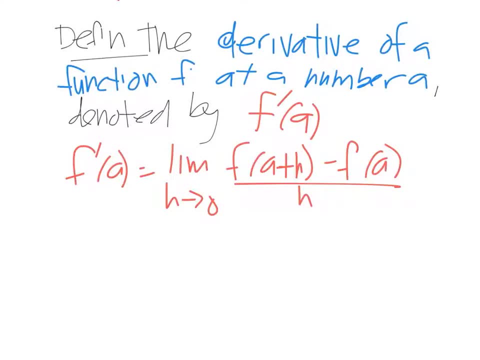 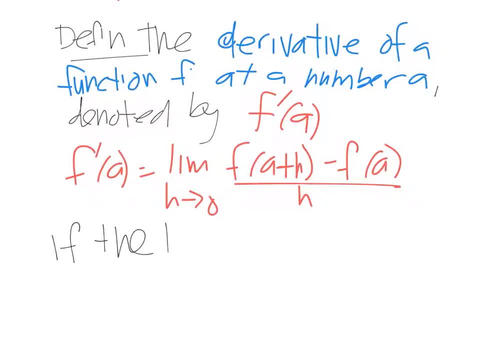 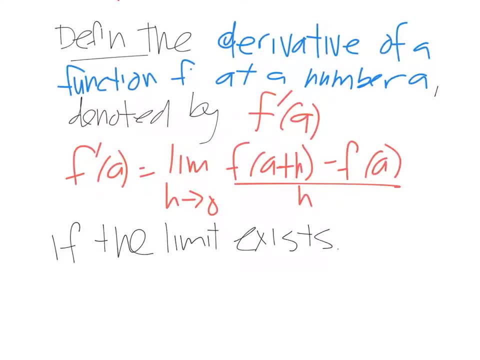 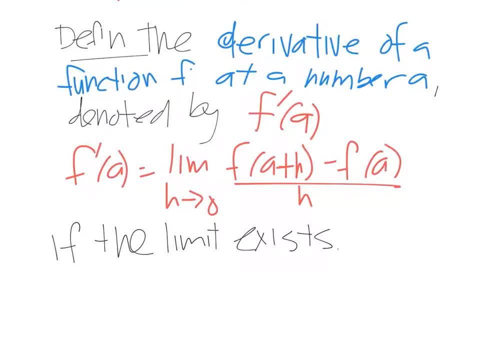 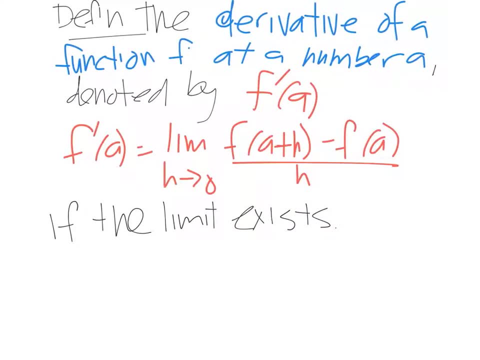 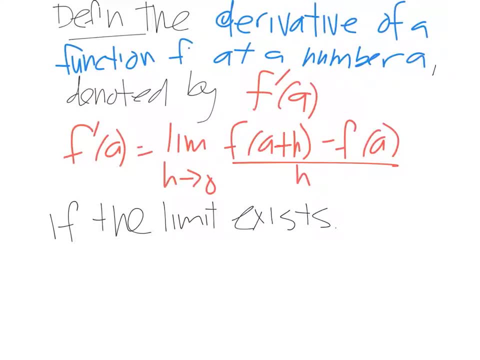 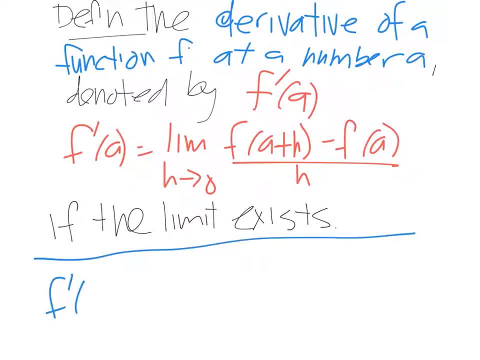 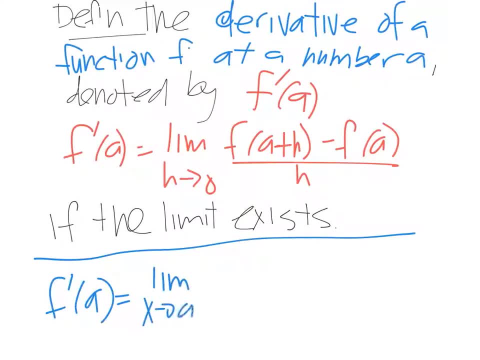 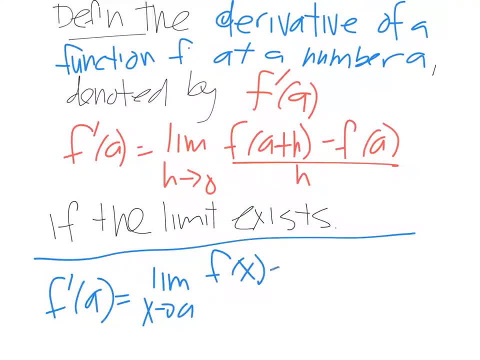 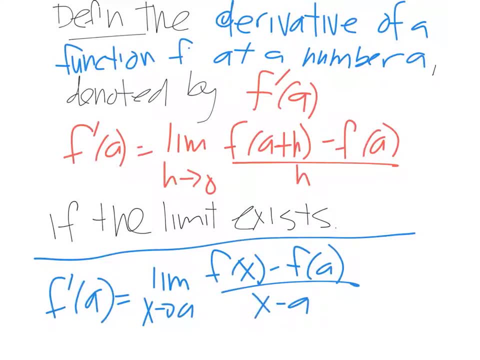 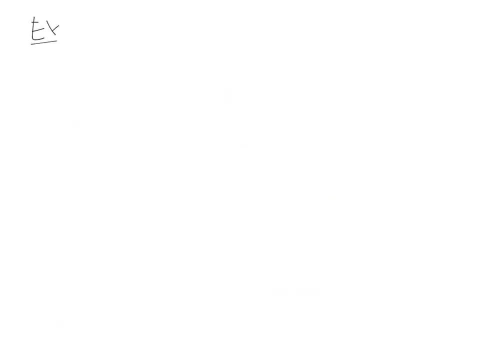 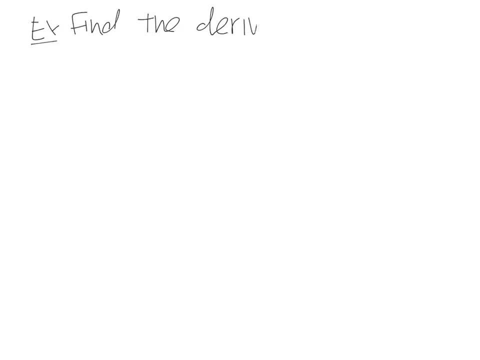 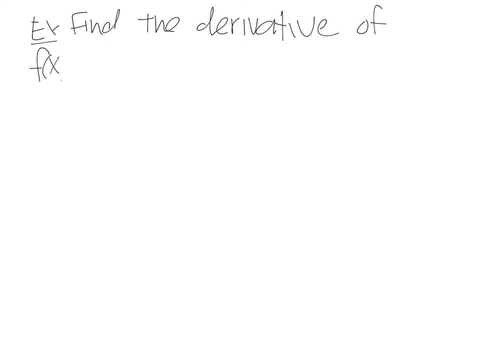 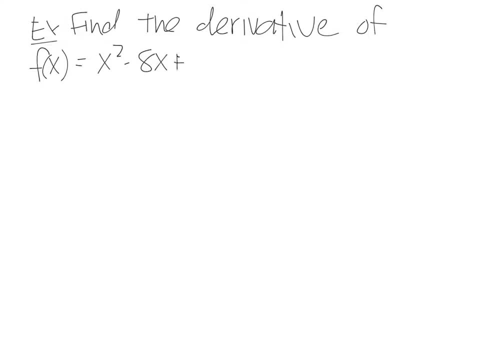 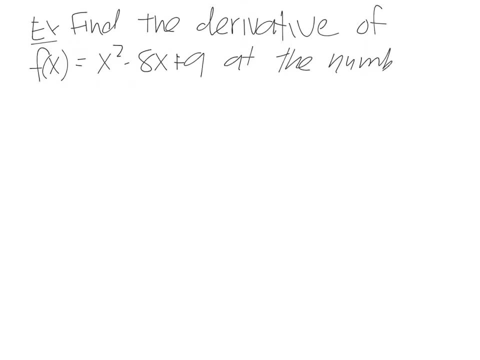 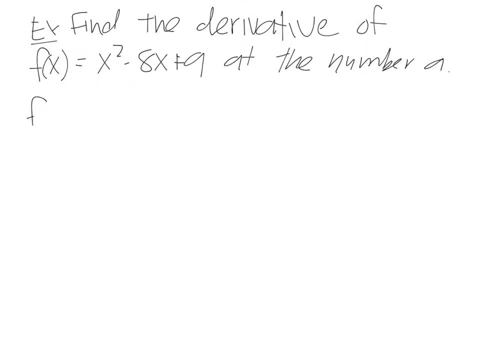 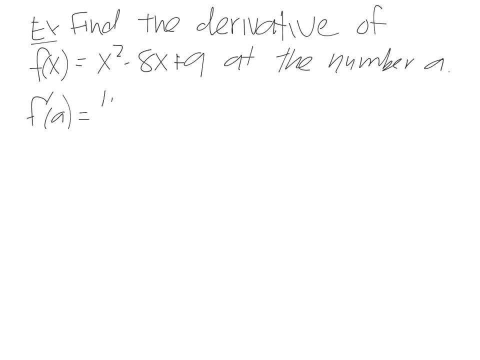 the derivative of a function f at a number e. the derivative of a function f at a number e. That is the limit, as h goes to 0 of f of a plus h minus f of a all over h. So let's figure out what's f of a plus h. 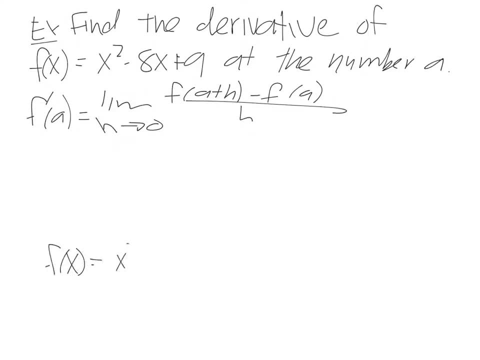 So if f of x is x squared minus 8x plus 9, f of a plus h is going to be a plus h squared minus 8 times a plus h plus 9, which is a squared plus 2ah plus h squared minus 8a minus. 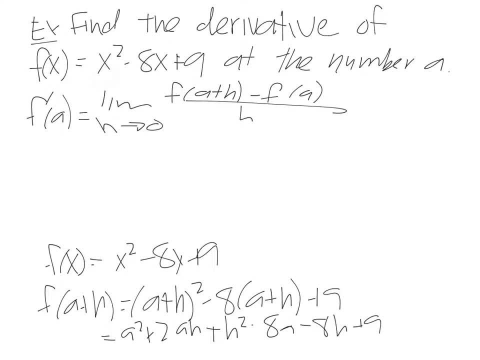 8h. So we have, this is the limit. h goes to 0 of a squared plus 2ah, plus h squared minus 8a, minus 8h, minus 9, and we're subtracting f of a. so this would be minus x squared minus. 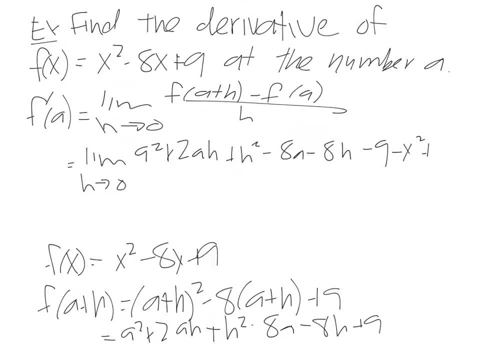 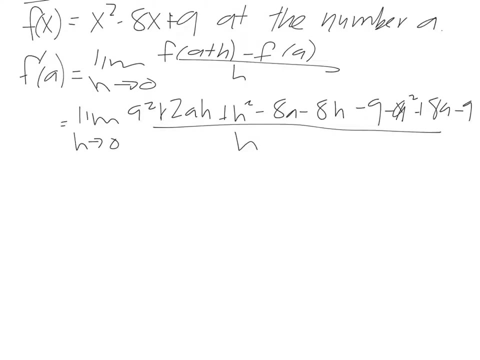 a negative. so this is going to be plus or, excuse me, not a, Not x. it should be a squared plus 8a minus 9, and this is going to be all over h. So simplifying we get. let's see, we have our. oops, this should be a plus 9,, not a. 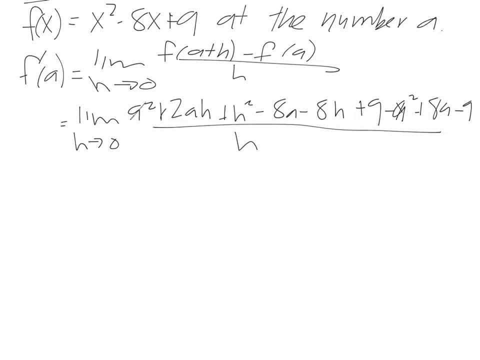 minus 9.. Okay, so now we have our a squared and our minus a squared cancels Our plus 9 and our minus 9 cancels, so we get the limit, as h goes to 0, of 2ah plus. 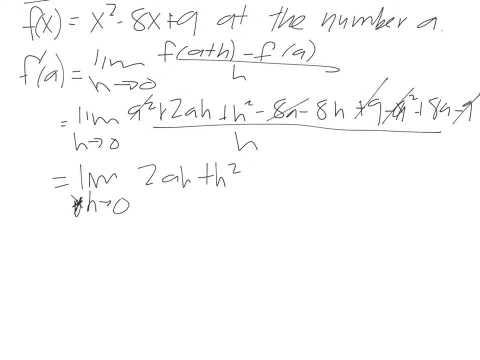 h squared and then our negative 8a and our positive 8a also cancel. so minus 8h and that's it all divided by h. Now, if you notice, everything has an h in it, so we can cancel out our h's. 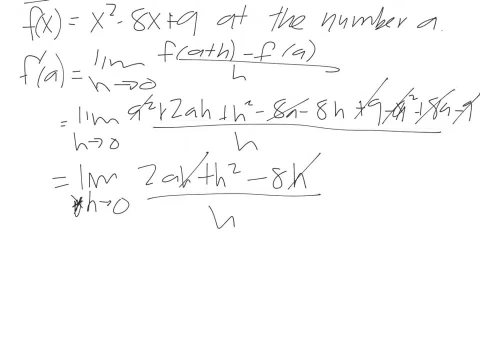 That h cancels, that h cancels and the h squared just becomes the power of 1, and then we divide the h in the denominator. So this is now the limit, as h goes to 0, of 2a plus h minus 8, and we can now evaluate. 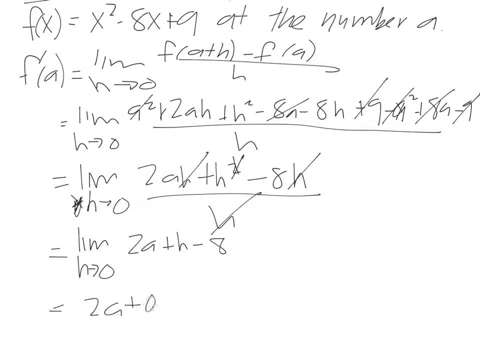 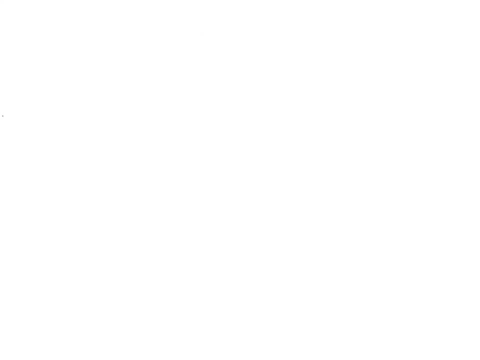 this limit when h is 0, so this is 2a plus 0 minus 8, or 2a minus 8.. So this is the limit, Okay, And this is equal to our derivative evaluated at the point a. 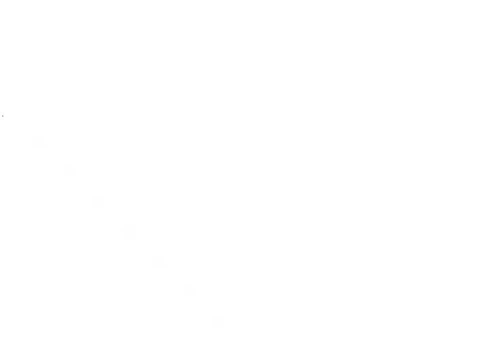 So now we have another way of expressing the tangent line and we say that the tangent line to the function y is equal to f of x at the point a comma f of x. f of x is the line through the point a comma f of a, whose slope is equal to, is equal. 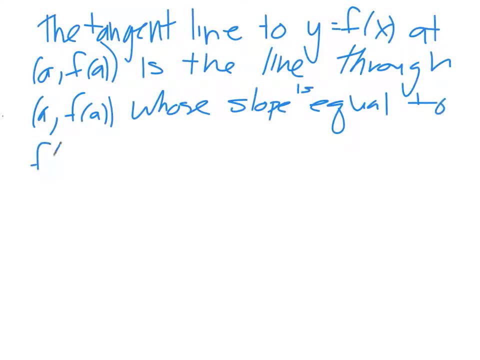 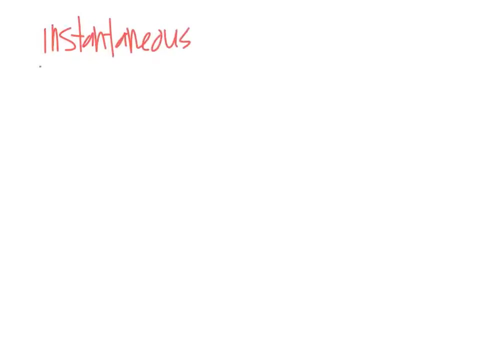 to the derivative f prime of a. So this is f prime of a. So this is f prime of a. Now we have something called the instantaneous rate of change, and this instantaneous rate of change is equal to the limit, as delta x goes to 0.. 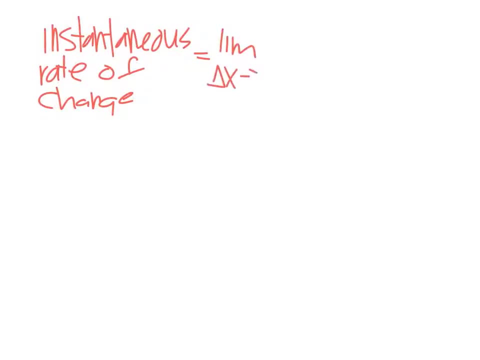 So this is f prime of a. So this is f prime of a. So this is f prime of a. So delta x goes to 0 of delta y over delta x. So rate of change: the change of y over change in x, just like our slopes. 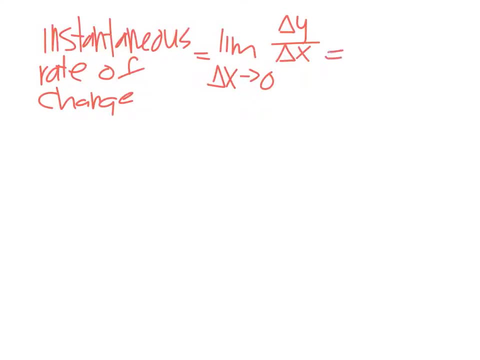 So this is one way of writing it, Or we could re-write it as the limit, as say, your point x2 goes to your point x1 of f of x2 minus f of x1, over x2 minus f of x1.. Okay. 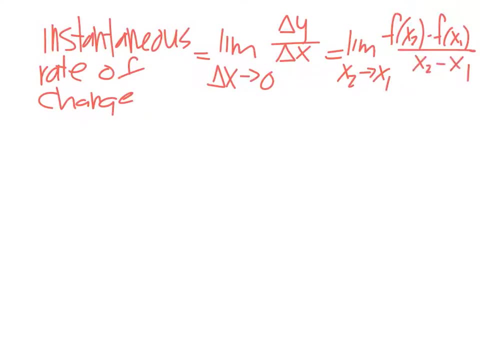 Okay, minus x1. and this is if something we have like delta x is given two points, and that's really our x2 minus our x1, and then our delta y is y2 minus y1. so we had some sort of curve like this and we had x1, x2. that would be f of x1, f of x2, or we can just say that this length 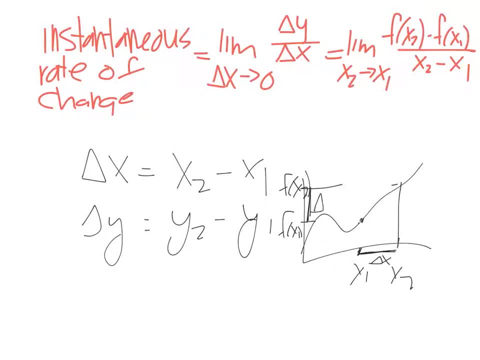 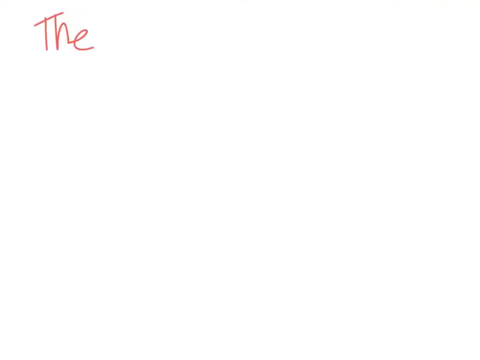 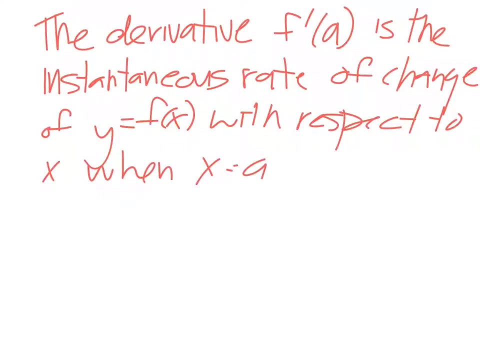 is delta x, that length is delta y, and so, finally, we have one last thing in this section, and this is the derivative f. prime at e is the instantaneous rate of change. of y equals f with respect to x when x is equal to a. In this section we'll talk about derivatives and rates of change, but before we start, we'll 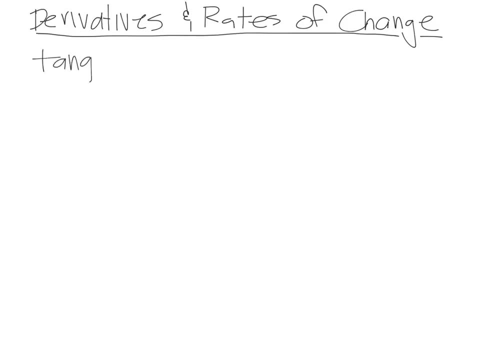 talk about something called a tangent. A tangent line is some sort of line that touches a curve, but it doesn't cross the curve, and so we should assume that this tangent line will have the same direction as the curve and right at that point of contact. 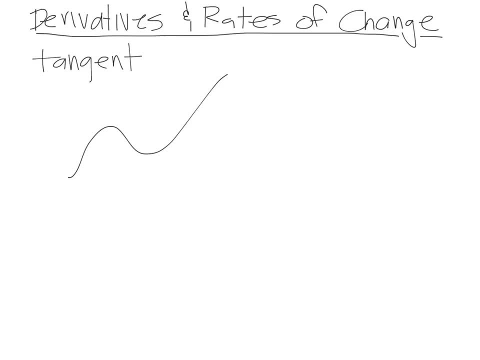 So, for example, if we have a curve that looks something like this, the tangent right here at that point should be a line that touches right here And has that same direction. If we had, the tangent point down here is going downward, and so the tangent line would look: 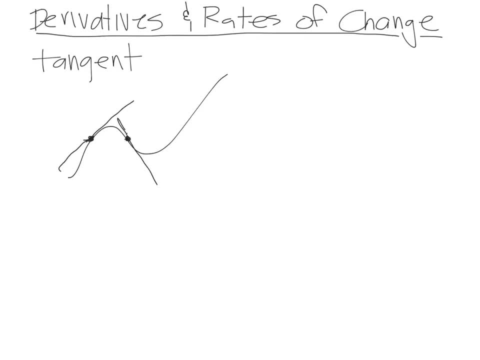 something like this. So if we were to have some curve, that looks something like this: we have x and our y axis, and then we have some point right here. we call this point a and if this is our function f, This value would be f. 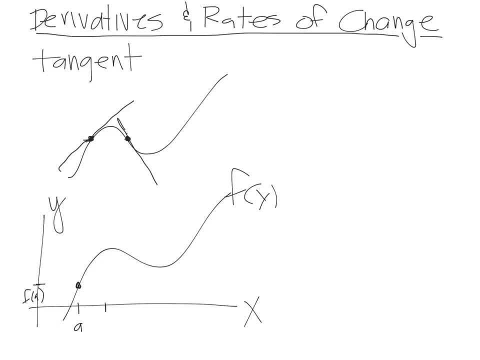 Now if we picked some arbitrary value, x, lets just say some x values over here, and then we had- this would be our f, evaluated at that x value. We have two points Now if we're trying to find the tangent line right here, we're trying to find the tangent. 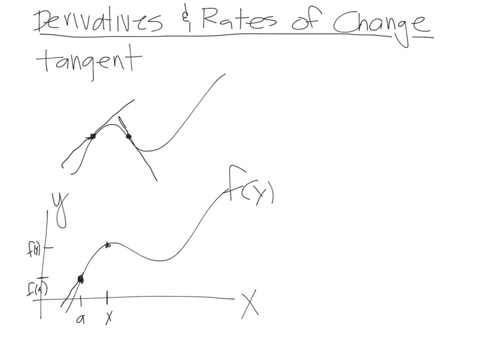 line right here. We want the tangent line to go through here and have something like that. So right there is, we have a straight line. Well, if we want to find the equation of a line, what we need is we need to figure out what's the slope. 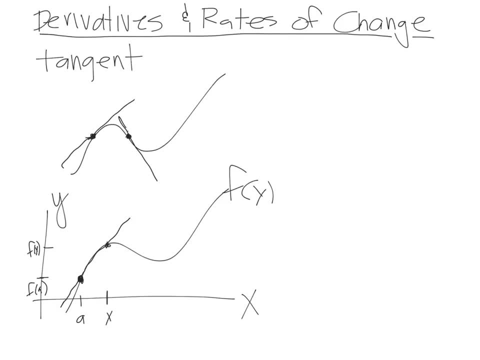 So now we know the equation of a slope is: m is the change in height over. so the change in the y value over the change in the x value. The change in the y value is f of x minus f of a and the change in the x value is x minus a. 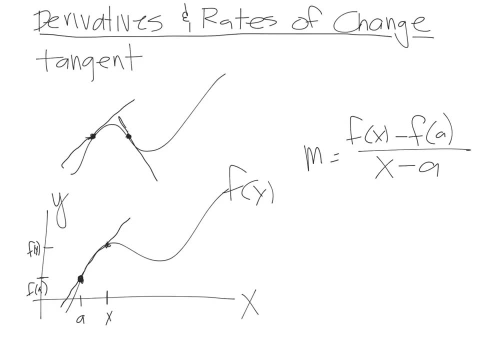 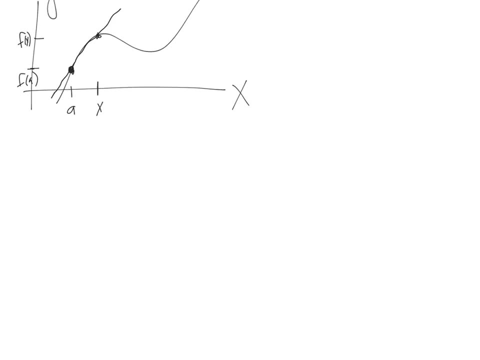 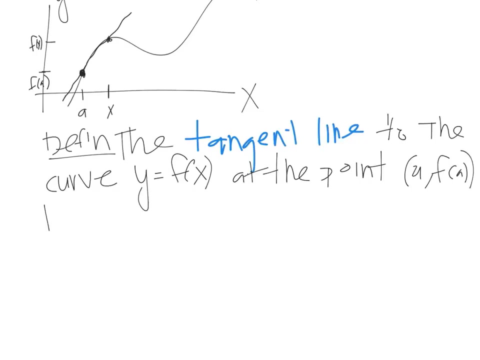 That's our slope, just rise over, run. So now we'll have our first definition, and this definition will say the following: The tangent line to the curve y equals f of x at the point a comma. f of a is the line through our point. 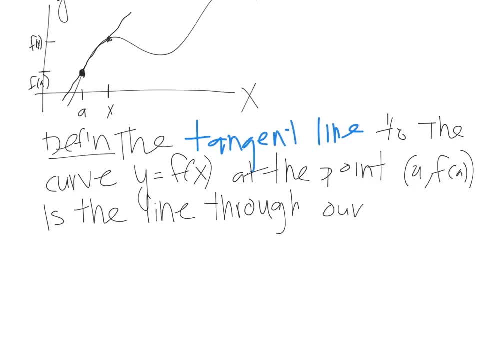 through our point with slope m equals. Now, taking a look at this, we pick some arbitrary x, but this is somewhat accurate. but if our point were way out here, maybe let's say over here, that's not a really good representation of what the slope looks like. 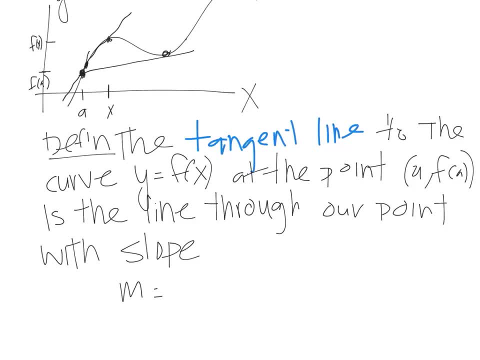 So what we want is: we want as close as possible to pick our x value to get a more accurate slope. So if we want it to be as close as possible, we take the limit as x approaches a. so we want x to be very, very close to a. 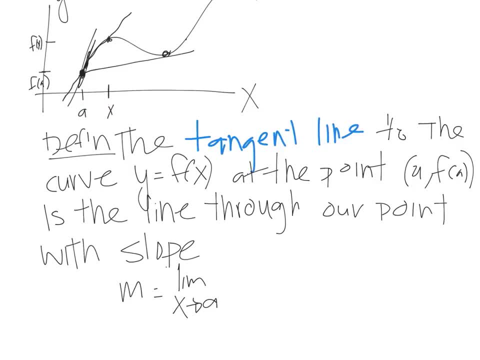 So we're taking x as it gets closer and closer to a. So we want this limit of f of x minus f of a divided by x minus a, Provided the limit of f of x minus f of a divided by x minus a. 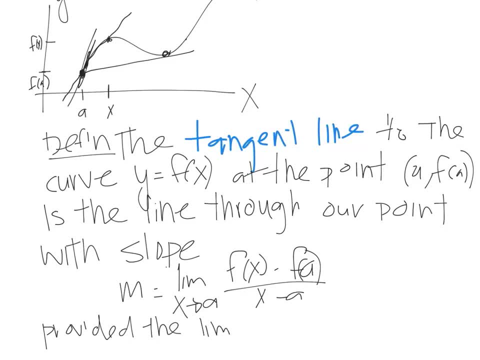 Provided the limit of f, of x minus f, of a divided by x minus a. That's really nothing right now in terms of its dimension, But you see, this one here has the perfecting function and it shows that this matrix of great-. 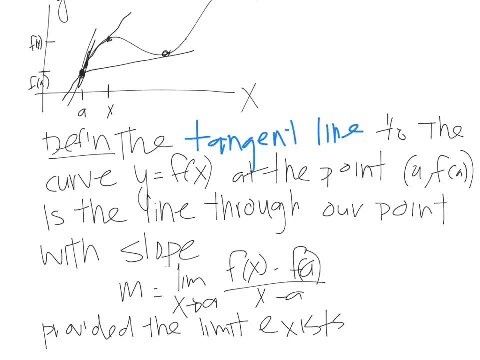 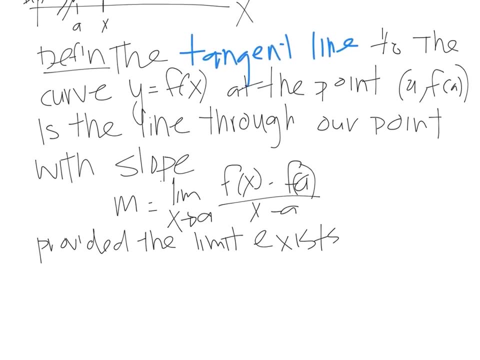 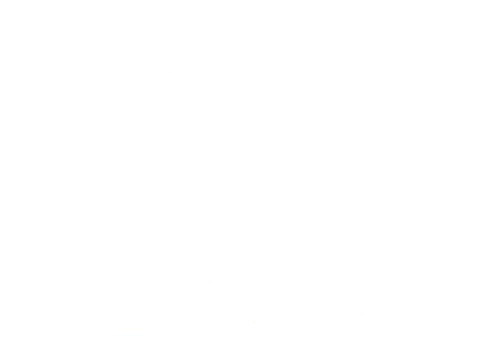 week-є exists. So that's the definition of a tangent line. Sometimes we will actually call a tangent line, or rather the slope of a tangent line, the slope of the curve. So let's do an example. So find the equation of the tangent line to the curve: y equals x squared plus 3 at the. 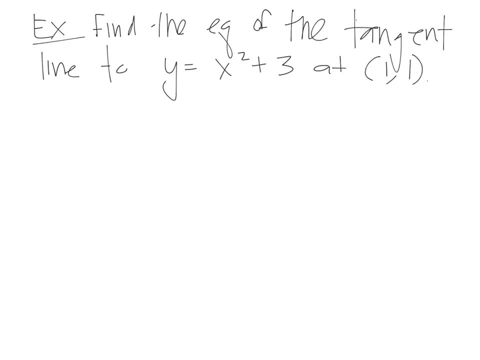 point 1, comma 1.. So what we want to do is find the equation of a line. When we find the equation of the line, one of the forms we can use would be: y minus y1 equals m times the quantity x minus x1.. 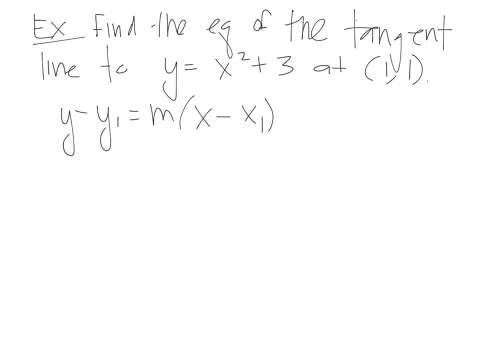 This is called the point slope formula, because we have our point x1, y1 and we have our slope m. Well, we already know our point, that's 1 comma 1, so substituting we get y minus 1 equals m times x minus 1.. So all we need to do is figure out what m is, and we'll be done, So let's go ahead. 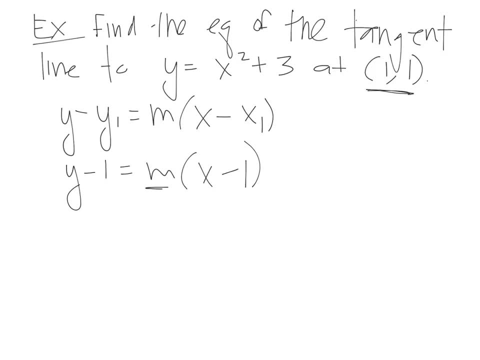 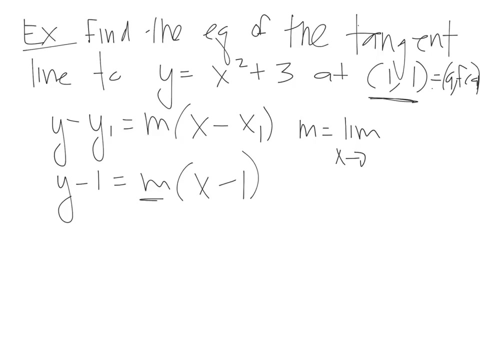 and do that. So remember the definition for the slope is going to be given: m is the limit as x approaches the slope, Which is our a value. and remember this: 1 comma 1, that's really our a comma f of a. So this is the limit as x approaches 1, really the x value of the point we're doing, of the. 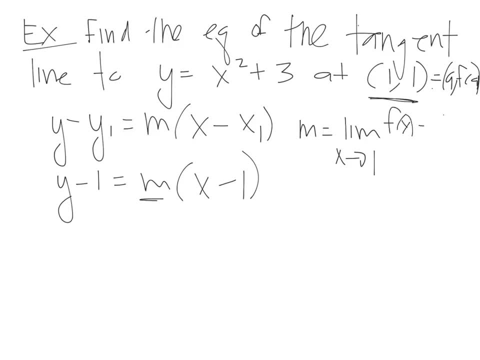 quantity f of x minus f of 1, divided by x minus 1.. Well, Let's Substitute What's f of x, f of x. well, that's right here. so that's going to be so. we take the limit as x approaches. 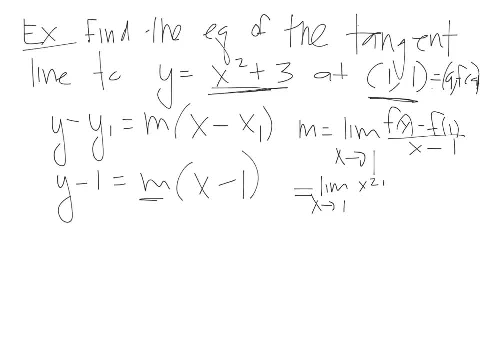 1 of x squared plus 3 minus- I'll put these in parenthesis: minus what's f of 1. We'll plug in 1 for x, we get 1 squared plus 3. All over x minus 1.. If I take out the parenthesis, 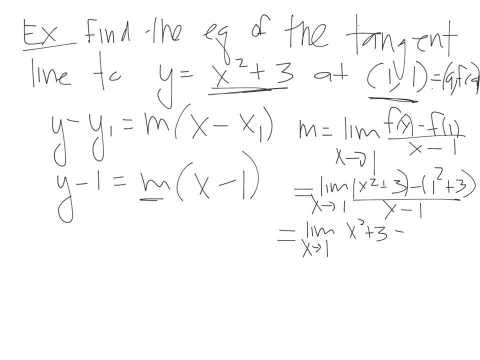 We get. this is x squared plus 3 minus 1, because 1 squared is just 1 minus 3.. All over, x minus 1 and our 3 and minus 3 cancel, And so we're left with the limit, as x approaches, 1, of x squared minus 1 over x minus 1.. 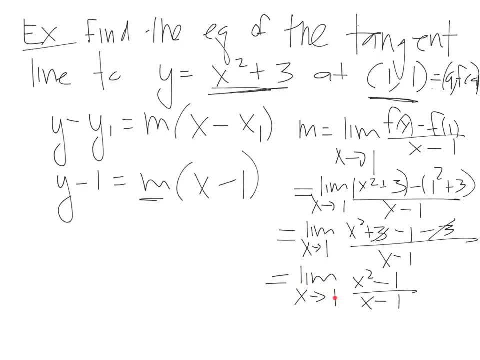 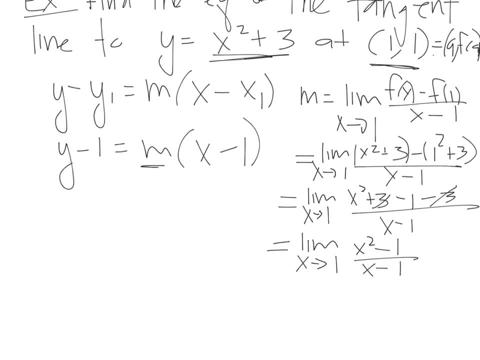 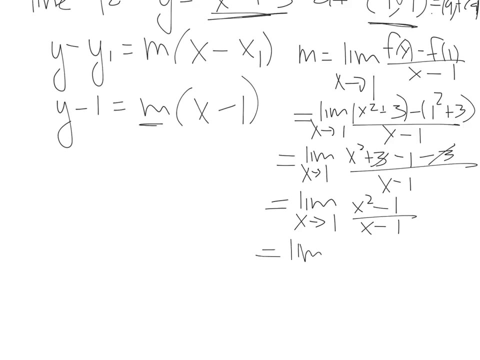 Now We can't just plug this right into the limit, because if we plugged in 1 we'd be dividing by 0 right here. But you might have noticed that x squared minus 1 can be reduced. So we now can write this as limit as x minus 1. x squared minus 1 becomes x minus 1 times. 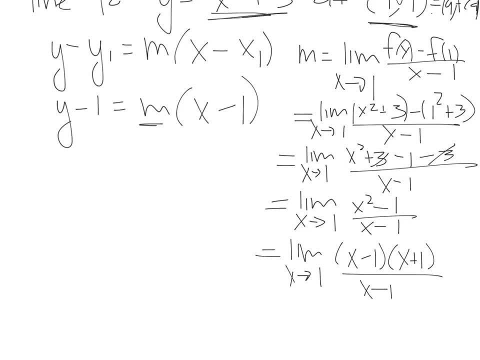 x plus 1 divided by x minus 1, and now we can cancel. So this is the limit, as x approaches 1, of just the quantity x plus 1.. And now we can plug in 1 in for x, And so we're left with: this is just going to be 1 plus 1, which is 2.. 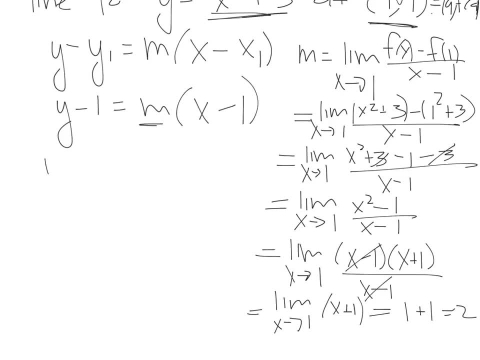 So our slope is: 2. Plugging it back into the formula. so we get y is the y minus 1 is equal to 2 times the quantity x minus 1.. Okay, Y minus 1.. And so this is our answer. 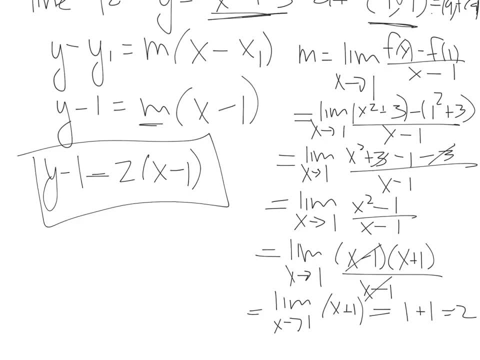 Now, this is a perfectly acceptable answer for me, But if you turn it in on the homework, it, depending on the format, it may not be acceptable. But if you turn it in for quiz or test, this is fine. But I'm going to simplify it just as an exercise. 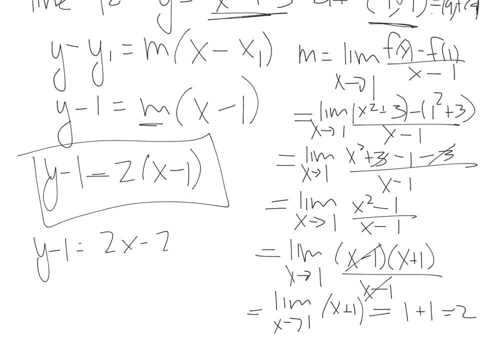 So this is going to be: y minus 1 equals 2x minus 2.. I just distributed and now I add 1 to both sides And so we get y. That's a pretty easy one, But this is going to be: x minus 1 equals 2x minus 1.. 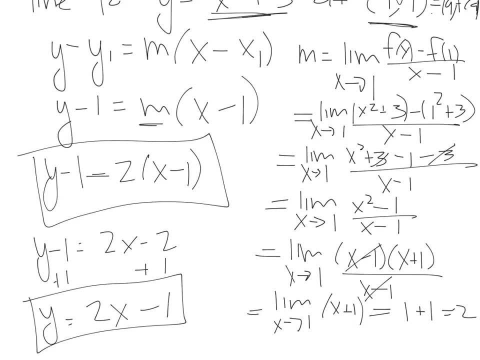 Now, the way that this works is that this is just going to be a process. It's written in different forms, so we're just going to write it in different forms. So it's just going to be this, right, And then we're going to add x. 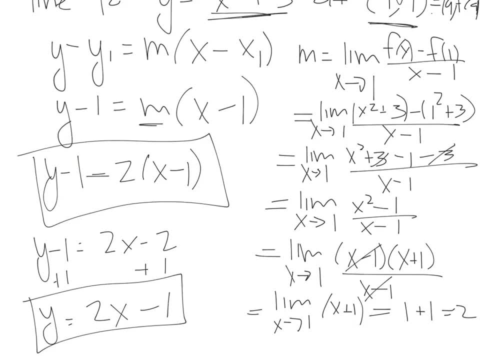 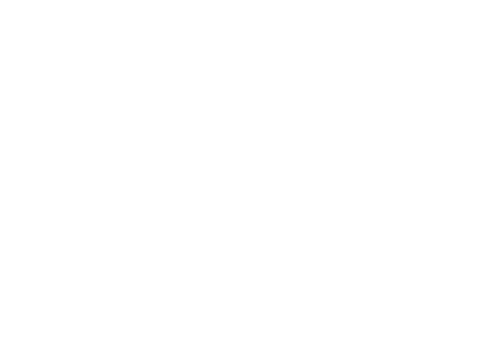 Two of these is equal to 2x minus 1.. Both of these represent the same line. It's just written in different forms. Now, sometimes it might be easier to write, given our curve, something like this where we had our point. 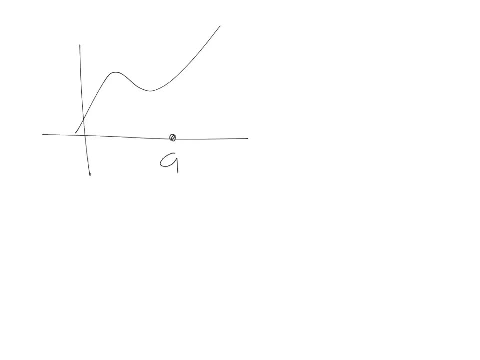 Let's say A, And so that would be our f of A. And then what that would be is: let's say a, So that would be our f of a. Let's say a, And so that would be our f of a. 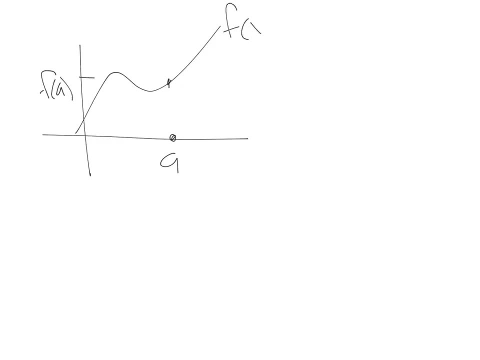 So that would be our f of a, our f of a. that'll be our function, instead of having some point x out here, what we could do. so I'm going to erase that x. instead of having a point x like that, what we can write is: let's just: 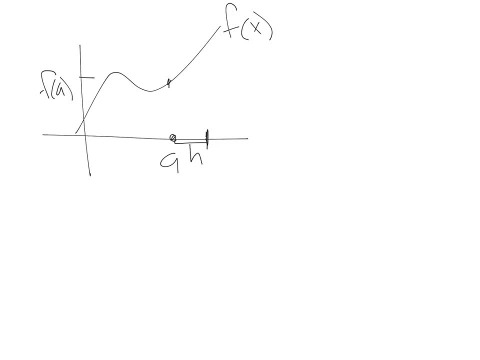 say this distance right here would be h. so we say we're just h, distance apart from a, which means that the value of that point would be a plus h and then the y value would be f of a plus h. so now we're just dealing with how far we are away from a. so instead of some value x, we're just 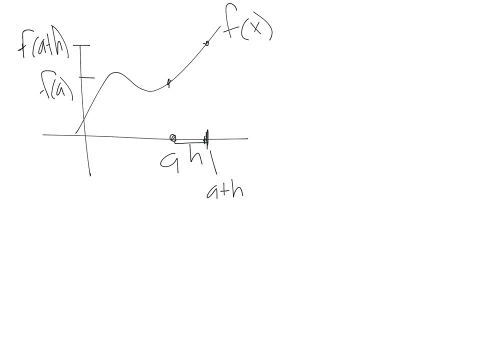 saying that a plus h, or we're just going h away from a. so using this notion we can rewrite the value of that point a plus h, and then the y value would be f of a plus h. so now we're just the equation for the slope of the line. this is going to be: x is or m is equal to the limit, as 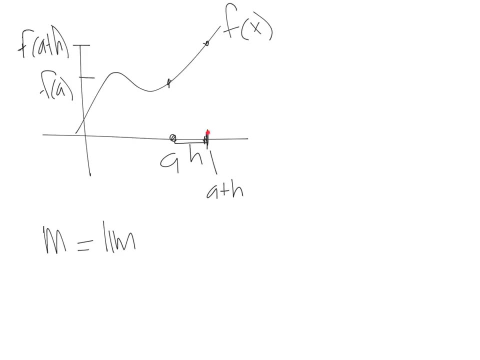 well, what we're taking before is the limit, as the value x was going towards a. so really, what that's saying is that the limit of this gap is getting smaller and smaller. so we can say this is the limit. as h approaches zero of well, the limit is just the slope. so the change in your y value, the 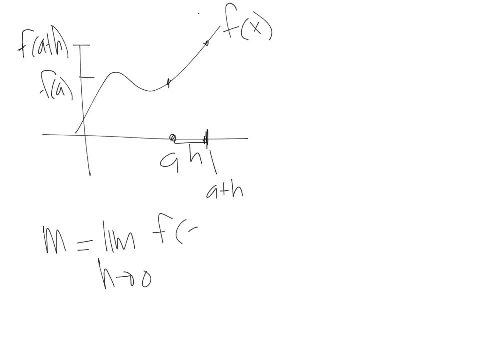 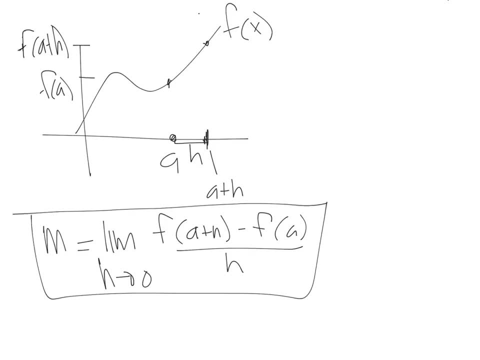 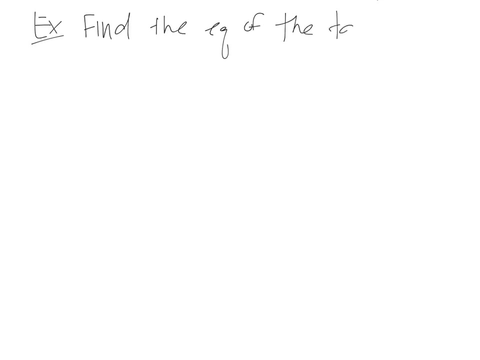 slope. so this is another way of rewriting what we learned on the other side. so let's do an example. find the equation of the tangent line to the equation. y is equal to three over x at the point three comma one. okay, so this three over x, that's our f of x. so let's begin. we wanted to find the. 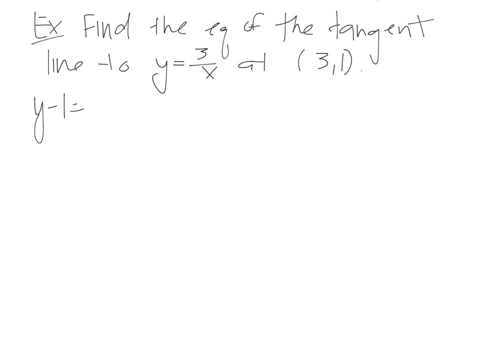 equation of a line. so that's going to be: y minus one is equal to m times x minus three. and now we need to find our slope, m. so that's going to be: m is equal to the limit, as h goes to zero, of f of a. 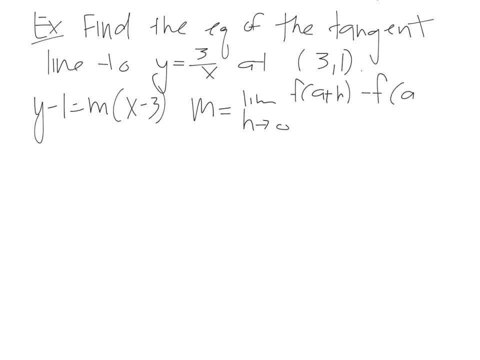 plus h minus f of a divided by h. now notice: we can't plug in zero for h right now because we'll be dividing by zero, which is not something we can do. so we will start simplifying. so this is limit, as h goes to zero f of a plus h. well, 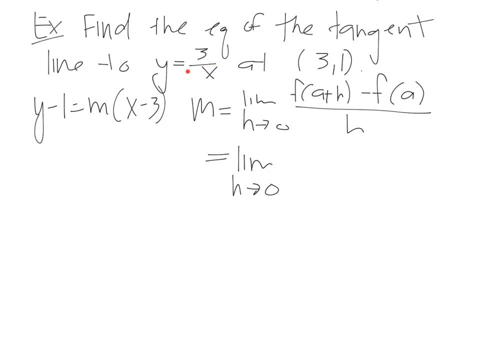 what happens if you plug in a plus h into this function? that's really just your x values. so this becomes three over a plus h. minus f of a is three over a. so just take a little note right here: if your f of x is three over x, 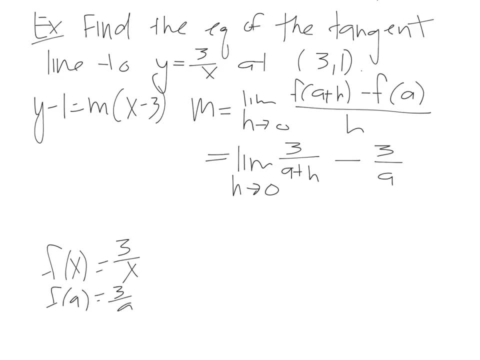 f of a is three over a. all we're doing is just simply taking whatever is the input and writing it wherever their x was. so in our case we had: this is f of a plus h. m of f over a plus h. okay, this is t. this becomes three over a plus h. the same way you might treat. 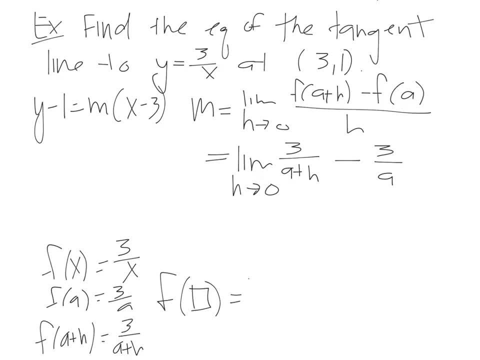 something like: if this is just a box, this is just 3 over that box, whatever goes inside gets replaced. and now, continuing back here, this is all divided by h. well, what we have is we're subtracting two fractions, and when we work with fractions, we want to find a common denominator. so what we're doing is: 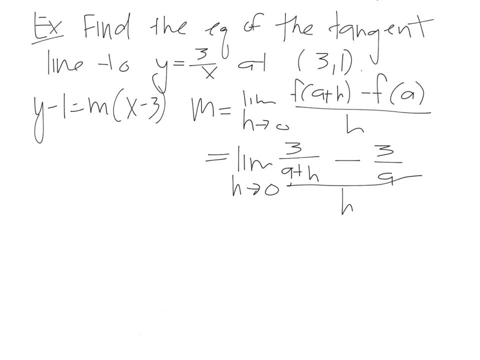 we're subtracting two fractions and when we work with fractions, we want to find a common denominator, and when we work with fractions, we want to find a common denominator, common denominator. So this becomes the limit, as h goes to 0 of 3 over a plus h. 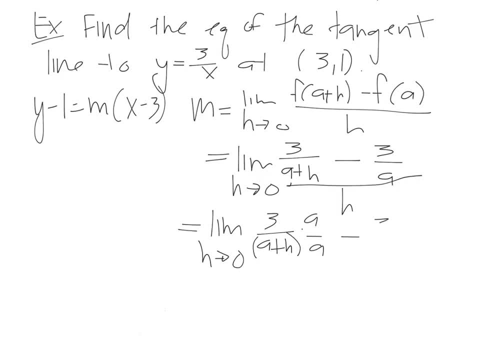 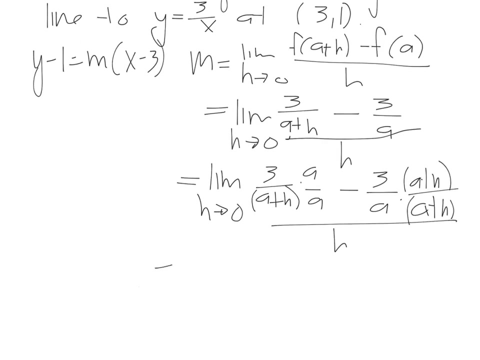 times a over a minus 3 over a times a plus h over a plus h all over h, which simplifies to the limit as h goes to 0 of 3a minus 3a minus 3h all over a times a plus h all over h. So what I did there was I just distributed this right there, So we get 3a. 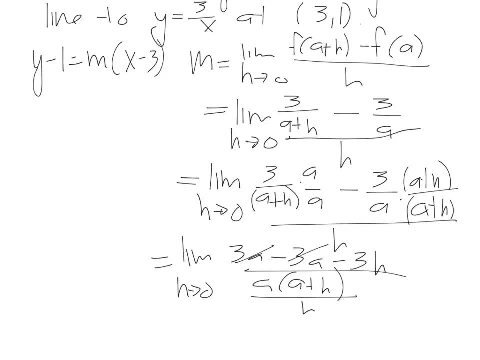 minus 3a, That cancels, and so we end up with the limit, as h goes to 0, of negative 3h divided by a times a plus h, and this is all over h, and so if we're dividing by h, let me just pull. 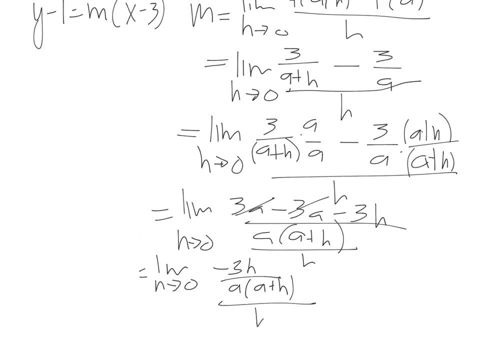 this up again. So this is all going to be over h. And now remember that our a value was 3.. That was the x value of the point, So, plugging that in, let me go ahead and just give myself a little bit. 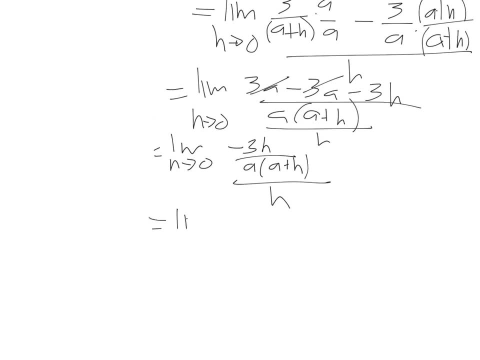 more space again. So, plugging that in, we get the limit, as h goes to 0, of negative 3h divided by 3 times 3 plus h. So this is all going to be over h. And now remember that our a value was 3.. That was. the x value of the point. So, plugging that in, let me go ahead and just give myself a little bit more space again. So plugging that in, let me go ahead and just give myself a little bit more space again. So plugging that in, let me go ahead and just give myself. a little bit more space again. Alright, so now the final bar. our h. that was 4a, n. separating 1t and 4h, It's W in here. there is negative one plus h, All over h. So if we're dividing by h, it's the same. 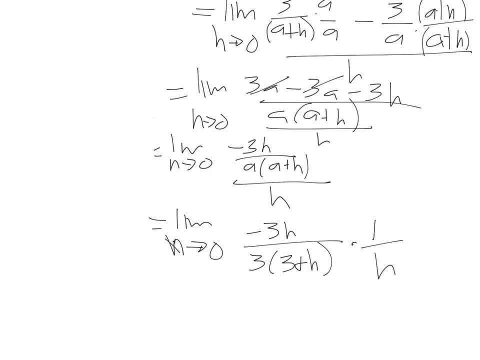 as multiplying by 1 over h. So we have something like that. And now our h's will cancel, Those hs cancel. So we take the limit as h goes to 0 of and then also our 3s cancel. So this is just negative one over 3 plus h. And now we take the limit as h goes to 0. And this 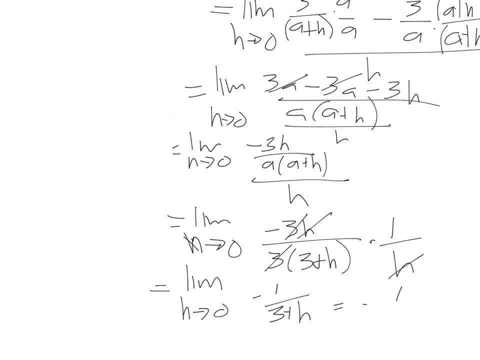 becomes negative one plus h, These three are going to cancel. So the integral where the over- excuse me- negative 1 over 3 plus 0 or just negative 1 third. So that's our slope. going back up here, filling it in, we get. 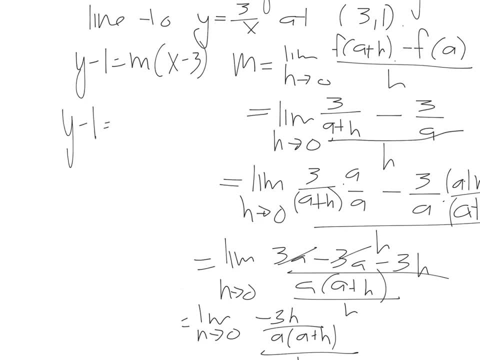 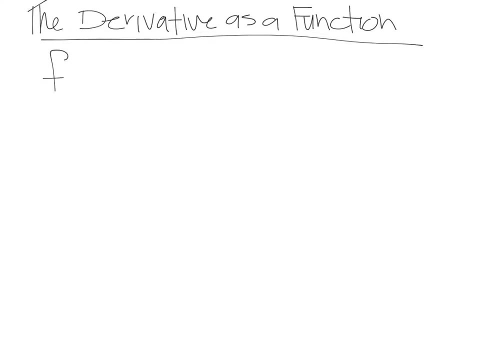 our equation is: y minus 1 is equal to negative 1. third, x minus 3, and that's our answer. previously we talked about the derivative of a function at a point. f, prime of a is equal to the limit as h approaches 0 of f of a plus h. 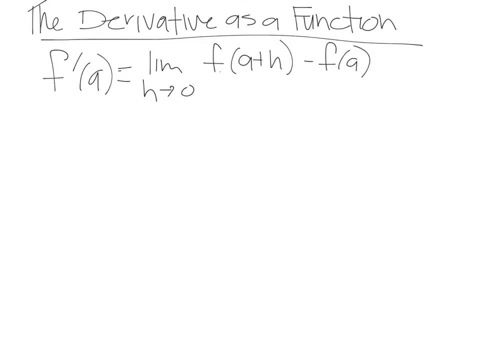 minus f of a divided by h. but now in this section, instead of just talking about the derivative at a single point, we'll think of the derivative as an equation, and so we will have, instead of at a single point, at some arbitrary value, x or some input value of x. 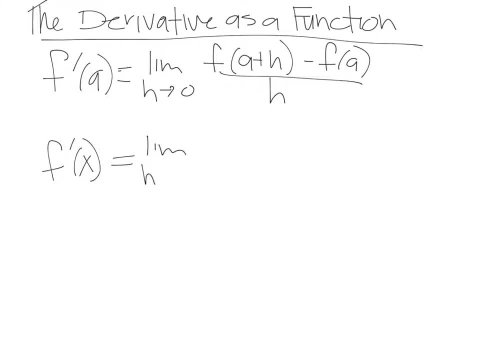 f prime of x is equal to the limit, as h goes to 0 of f of x plus h minus f of x. excuse me, f of x all over h. so this is the formula for the derivative at any point x, or as a function of x, rather. 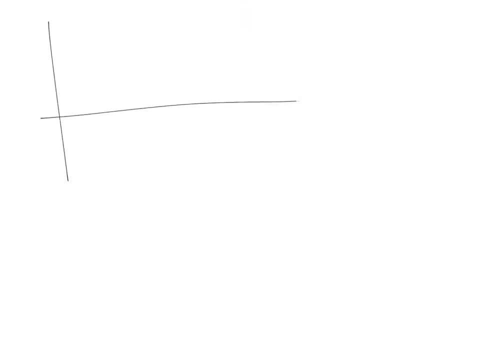 now, let's say we have the graph of some function and the graph might look like this: so this is x, y and this is our function: f of x, f of x. if we wanted to graph the derivative of this function, what would that look like? so we want to find: 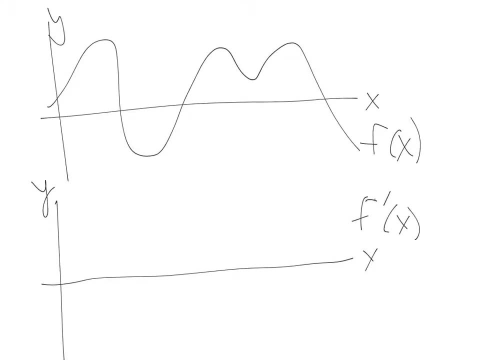 f, prime of x, or remember the derivative is really the slope of the line at each point. so let's examine the slopes. well, we have a positive slope going up here, then it becomes negative and positive and negative and positive and negative. But when it goes from positive to negative, right here at this peak, it is zero slope. 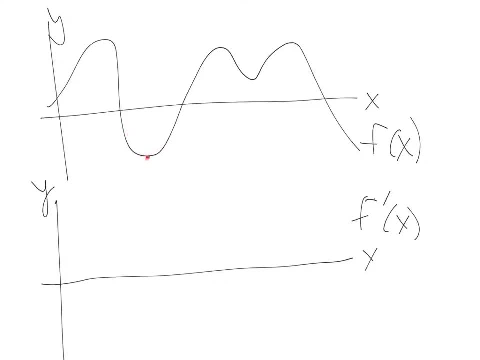 And same thing down here. If you're going from a negative to positive, you pass zero. So right here is the zero slope, zero, slope, zero and zero, So we can fill in all those gaps. So this point right here gets translated down to here: zero. 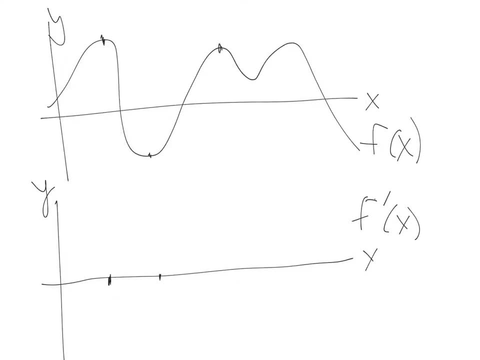 This point is also zero. This point becomes zero, This point is also zero, And then here that's also zero. So now we have three points for our derivative. Now, looking back over here, we have a positive slope. Positive slope means it's going to be above the axis. 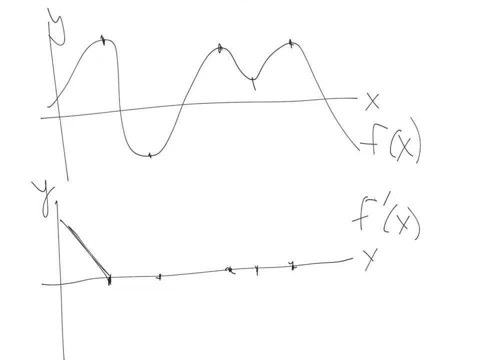 Positive means we're above, so we're some value above the axis. Now, looking over here, it's a negative slope, so we will be below the axis. So we're going to come down negative and then we go back up To zero. 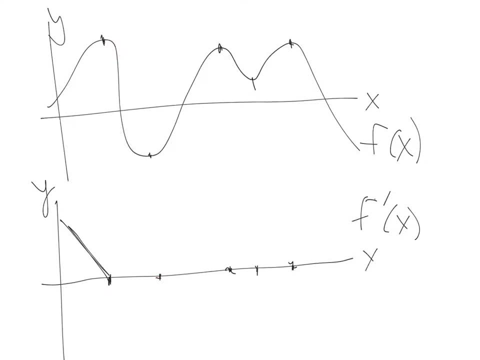 And if you look right here, this slope right here is a negative, but it's not too steep. Over here it's a very steep and then it's not too steep. So if it's not too steep, it's a smaller number. 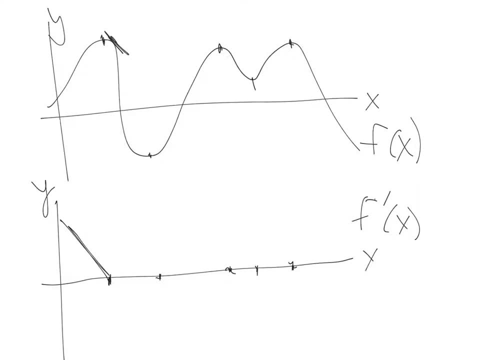 So not too steep right here means negative, but just a small negative. So something like this: Very steep over here is negative and a large negative, And then over here we have a negative, But it's not that much of a negative, so it's smaller. 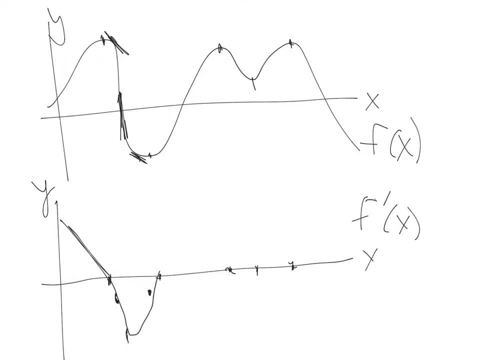 So we might have it looking something like that: And same thing, as we go over here We're going to be increasing, so it's a positive slope. The slope is not too big right here. It's a small positive. It's a bigger positive and then it goes back to a small positive. 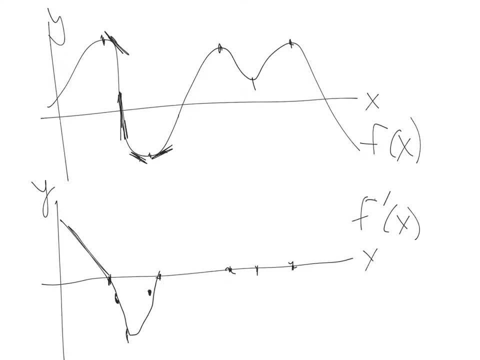 So let me just draw that in. So it's a small positive, A bigger positive and then a smaller positive. So small positive, big positive and a small positive, And our graph might look something like that. And then same thing in this section right here. 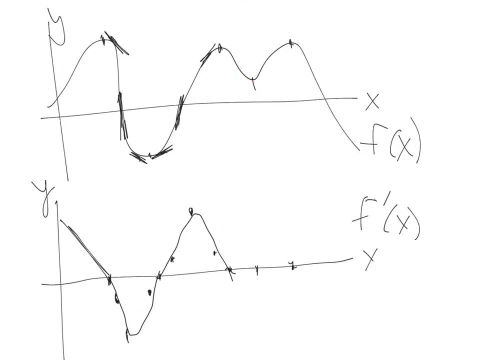 Small positive. it becomes steeper and then not as steep. So, excuse me, all negative, So negative back up, And then over here we have positive, So it goes positive and back down And then finally this is all going to be negative. 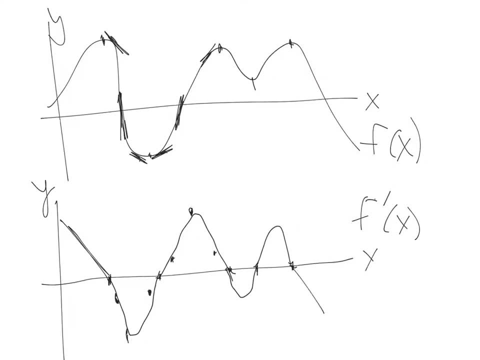 And so we're going to be negative, And this is sort of a sketch of what the derivative might look like. Really, what we do is we first look at what are the zeros And that's these peaks, And we can tell all those points. 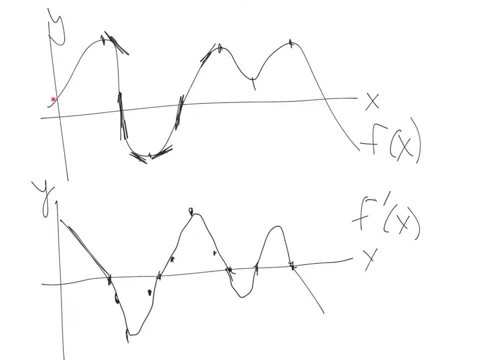 The zeros tell us when it crosses the axis And then the slope tells you: if it's positive, then you're above the axis. If it's a negative slope, then you're below the axis. Now let's do it again. For example, if we're given f of x is equal to x cubed minus x, let's find the formula. 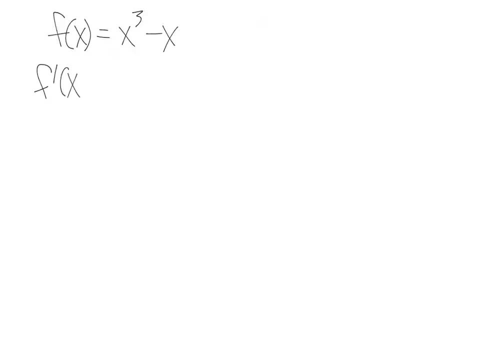 for the derivative f prime of x is equal to the limit, as h goes to zero, of the following: f of x plus h minus f of x all over h. So this is the limit, as h goes to zero, of f prime of x. 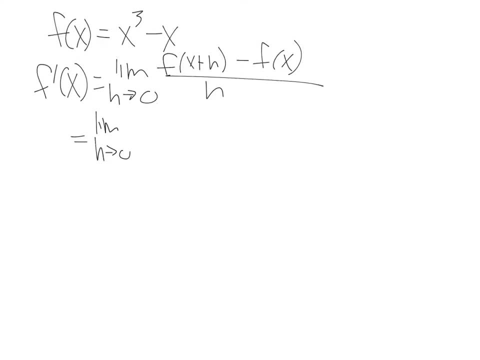 So this is the limit as h goes to zero of f prime of x. So this is the limit as h goes to zero of f prime of x. Well, we need to figure out what's f of x plus h. Well, that would be the following: 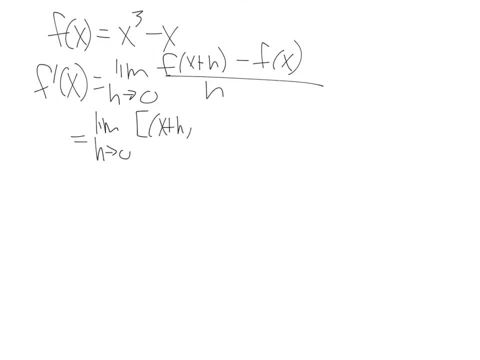 This would be x plus h. quantity cubed minus x plus h. all minus x. cubed minus x. all over h. Now notice we have x plus h. quantity cubed f plus h can be squared plus that. I'm already going to tell you what that is. 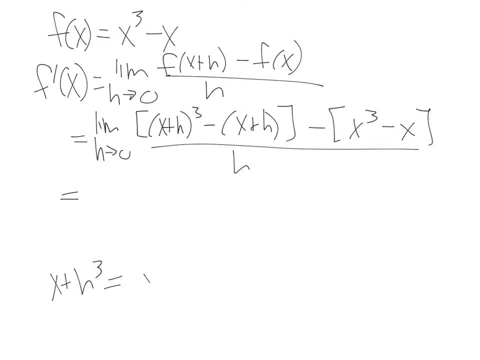 You can calculate it yourself. but x plus h quantity cubed is x cubed plus 3x squared h plus 3xh squared plus h cubed, And you can find that on your own just by multiplying it out. So we have the. 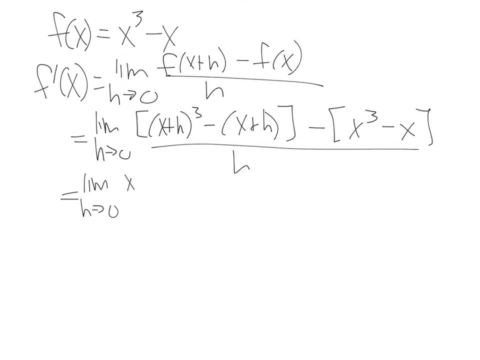 limit, as h goes to zero of x cubed plus three x cubed, is x cubed minus h, squared plus three x squared plus three x squared squared h plus 3xh squared plus h cubed minus x. minus h minus x cubed. and then 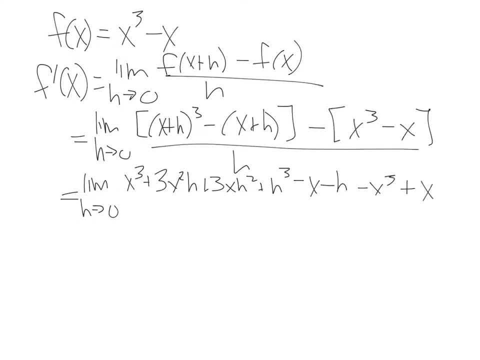 a minus, and negative means we have a plus x. This is all going to be divided by h, and so we can cancel some things. our x cubes cancel, and then our x's will also cancel. So we're left with the limit, as h goes to 0, of 3x squared h plus 3xh squared plus. 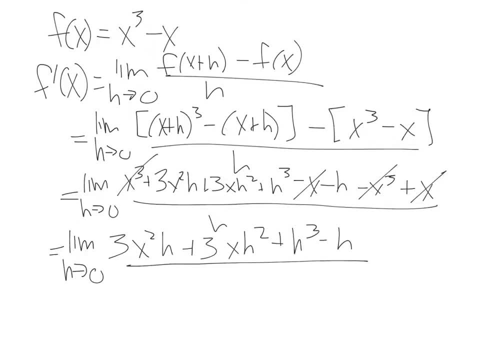 h cubed minus h, all divided by h. Now notice, everything has an h, so we can start cancelling our h's. This h cancels this h squared becomes h, just to the power of 1, this h cubed becomes h. 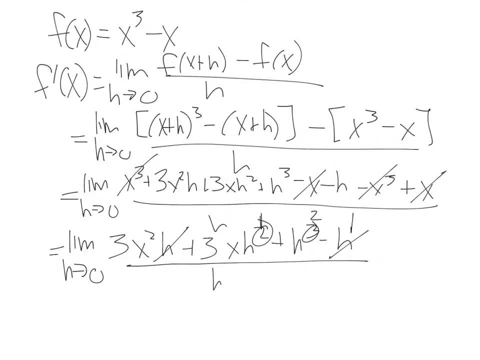 squared and this h cancels. And when we do this we cancel. Divide h divided by h, you're just left with 1, and then we cancel out our denominator. So this becomes the limit, as h goes to 0, of 3x squared plus 3xh to the power 1, plus. 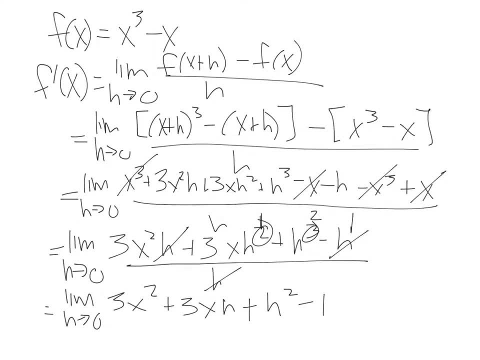 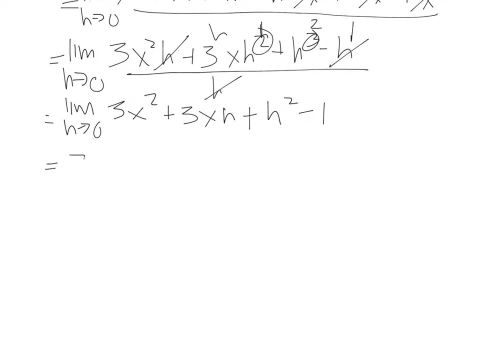 h squared minus 1.. We can evaluate this now, and so we get: this is equal to 3x squared plus 3x squared times 0, because we're evaluating when h is 0, plus 0, squared minus 1, or 3x squared. 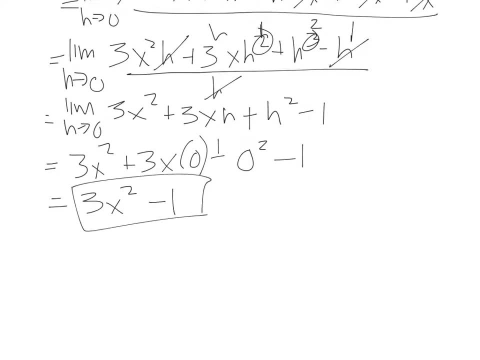 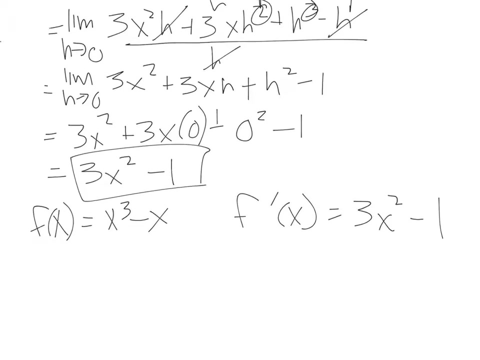 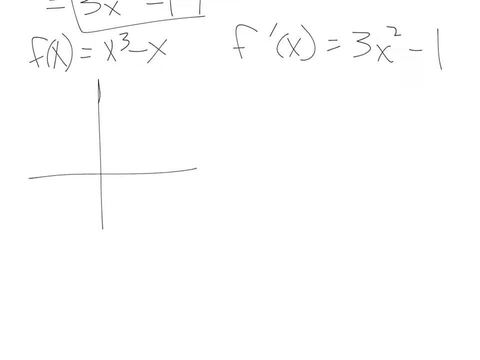 minus 1.. And that's our answer. So if we're given the function, f of x is equal to x cubed minus x, the derivative f prime of x is 3x squared minus 1.. And so if we're to graph this, what this looks like is the following: the cubic function. 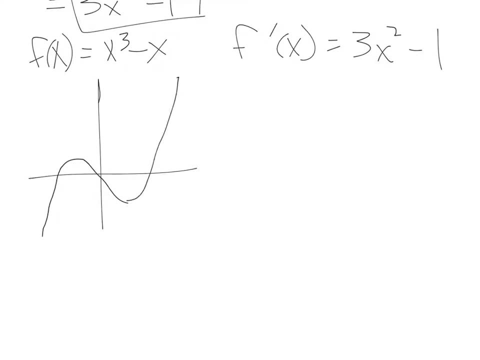 x cubed minus x looks something like this: The graph of the derivative f prime of x is a parabola, so if we were to graph that below we would see. well, right here It's a maximum. it has a slope of 0.. 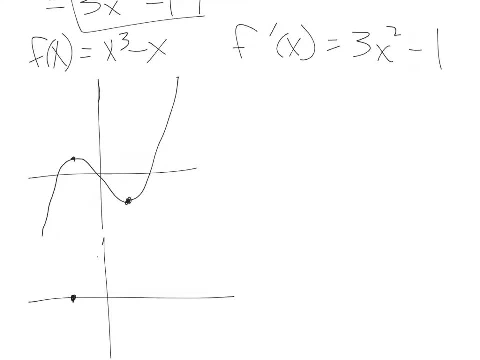 So that's where it crosses and we also have a minimum, another slope of 0, it's right here. And then we see over here we have a positive slope and another positive slope, so we're going to be above the axis like this and like this. 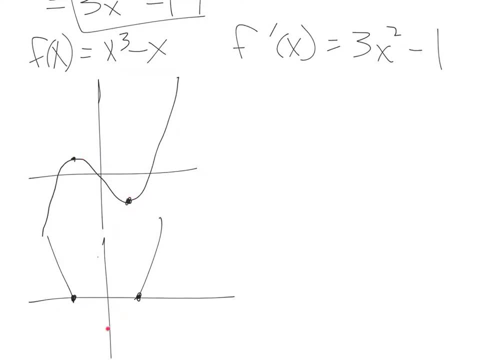 And then we see in the middle we have a negative slope, so we'll be below the axis. we start off at a small negative. it becomes steeper and then becomes a smaller negative. So small negative, steeper means it's a larger number and then back to a smaller number. 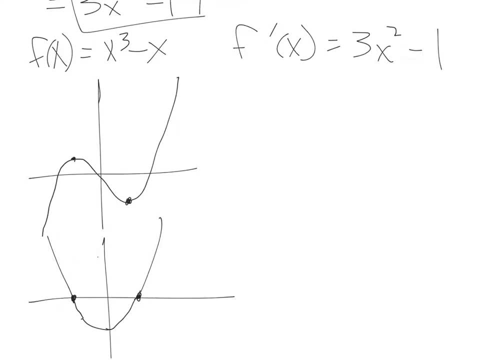 and that's exactly what this is. This is a parabola, And so you can see the difference between f of x and f prime of x. Let's do another example. If we have our function, f of x is equal to x cubed minus x cubed minus x cubed. 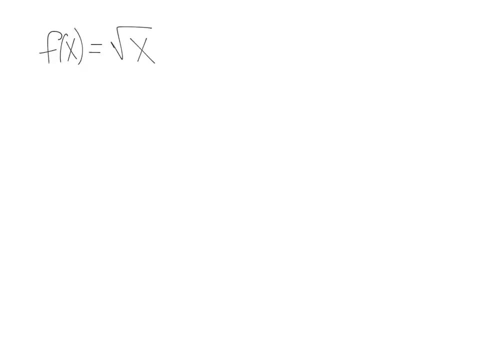 f prime of x. If f of x is the square root of x, what's the derivative of the function? Well, to find that we get: f prime of x is equal to the limit, as h goes to 0, of f of. 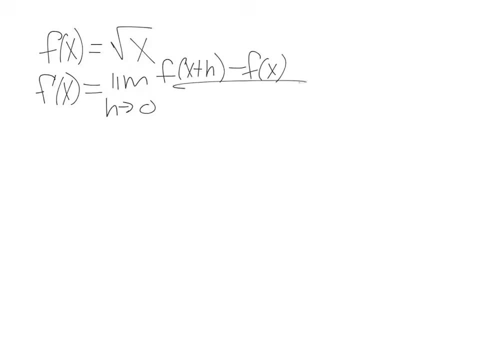 x plus h minus f, of x all over h. So we get the limit, as h goes to 0, of the square root of x plus h minus the square root of x All divided by h. Well, what can we do in a situation like this? 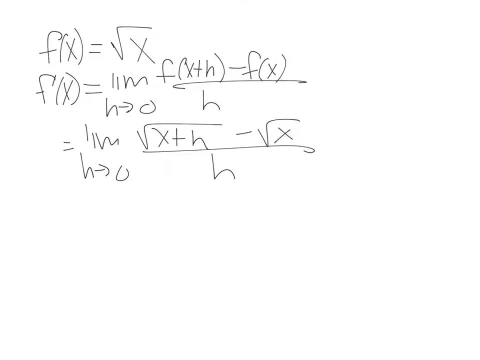 When you see the subtracting two different square roots, the first thing you want to think about is rationalizing the numerator, And what I mean by that is by multiplying by the conjugate. So we multiply by almost the same thing, but instead of it being minus-ing, we add the. 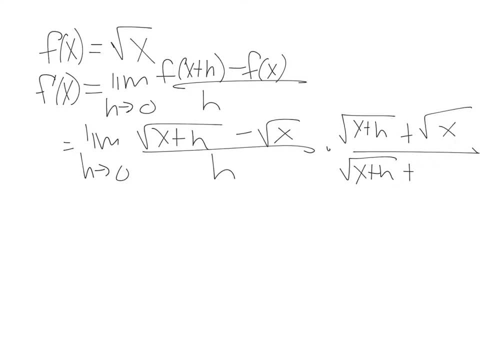 two. So we multiply by almost the same thing, but instead of it being minus-ing, we add the two. So we multiply by almost the same thing, but instead of it being minus-ing, we add the two. So we get square root of x plus h, plus the square root of x over the square root of. 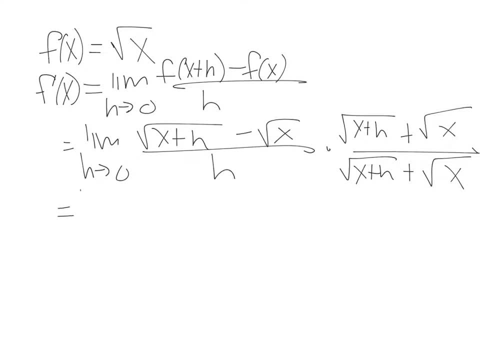 x plus h plus the square root of x. So what this does is this simplifies the numerator. We have two things multiplied by each other. So, for example, if we had a minus b times a plus b, that's the difference of squares. 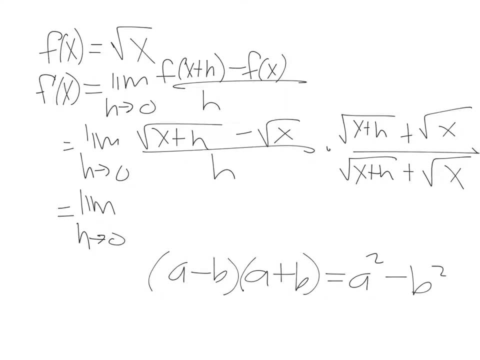 and this becomes a squared. So if we had a minus b squared, well, if each of these are the square root, what we would have is the square root of x plus h squared. So the square root of x plus h quantity squared is just going to be x plus h. 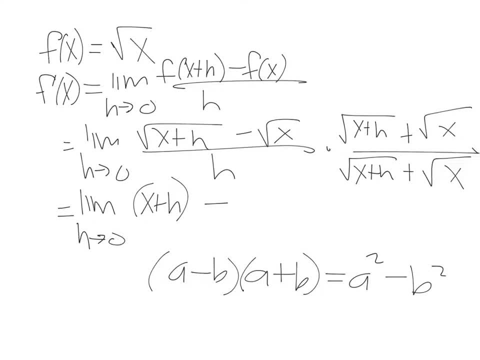 And then minus the square root of x, quantity squared just is going to be x, And then our denominator would be h times this whole thing on the right square root of x plus h plus square root of x. But we can simplify this and so we get the limit as h goes to zero. 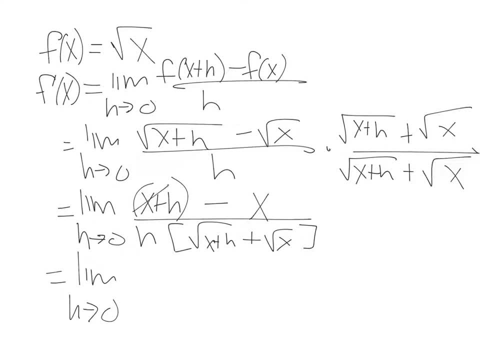 Well, the numerator is x plus h minus x, so our x's will cancel and we're just left with h on the numerator divided by h times the quantity squared, So the square root of x plus h plus the square root of x. 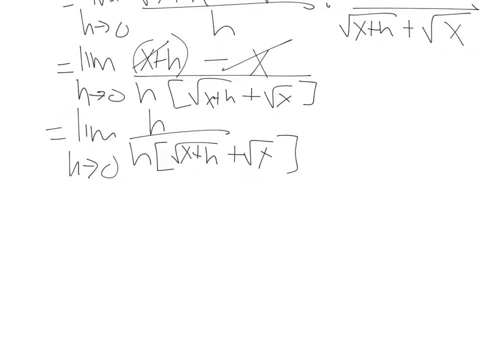 And now notice they both have an h in it in the numerator and denominator and that cancels. so we're left with the limit, as h goes to zero, of one over the quantity x plus h, square root of x plus h plus square root of x. 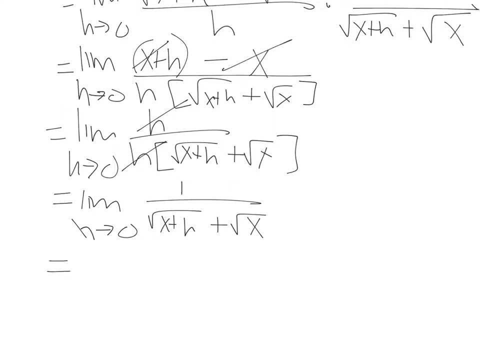 Now we can evaluate it when h is zero, And so this is one over the quantity x plus h plus square root of x plus h plus square root of x. So this is one over the square root of x plus zero plus the square root of x. 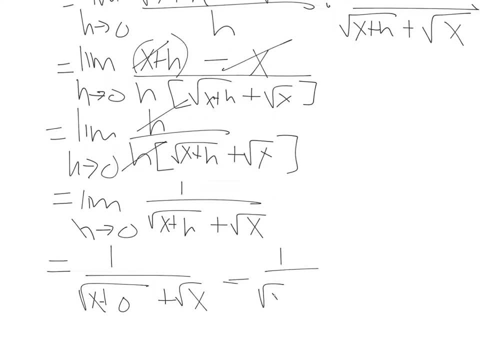 So this is one over square root of x plus square root of x, which is one over two square root of x. So the key to this problem was recognizing if we had two square roots, you would multiply it by the conjugate and rationalize the numerator. 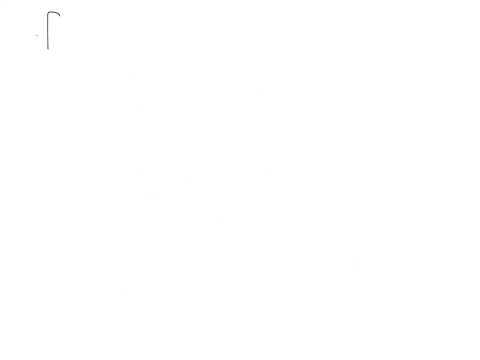 So we'll do another one. Thanks, We'll do another example where, if we're given f of x is x divided by x minus one, the derivative f prime of x is going to be the limit, as h goes to zero, of f of x plus h minus f. 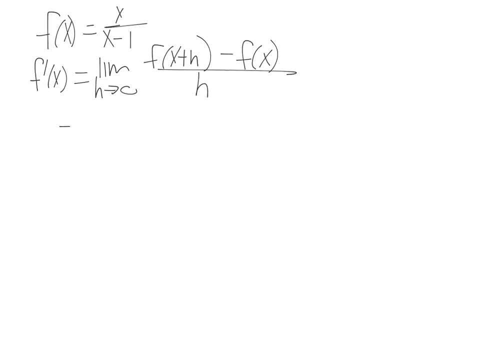 of x all over h. So this is the limit as h goes to zero. So f of x plus h becomes x plus h divided by x plus h, minus one minus x over x, minus one all over h. So we're subtracting two fractions. 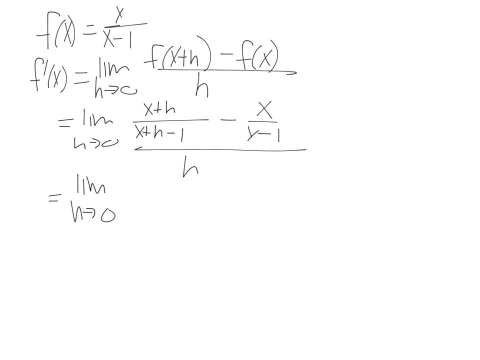 So what we want to do is find a common denominator, And so that common denominator is going to be x plus h minus one times x minus one. And so in order to make this first fraction have that denominator, we need to multiply it by x minus one over x minus one. 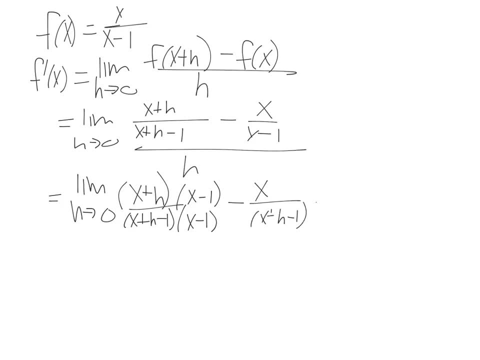 And then the second one. what we need to do is multiply it by x plus h minus one over x plus h minus one, And again this is all still over h. So we have the limit as h goes to zero, and now we'll distribute and multiply this out. 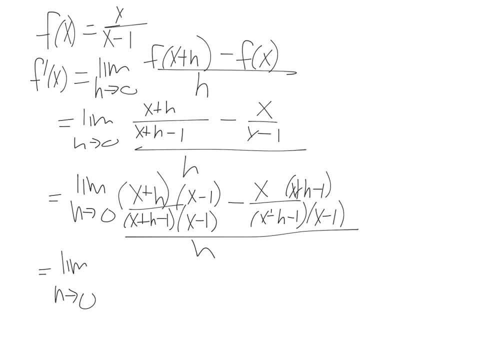 so we get the following: We get x squared plus x, h minus x minus h. We get x squared plus x, h minus x minus h, h minus x squared minus x, h plus x, all over the common denominator of x plus h minus one times x minus one, and since we have, we're dividing by another h, it's the same as multiplying. 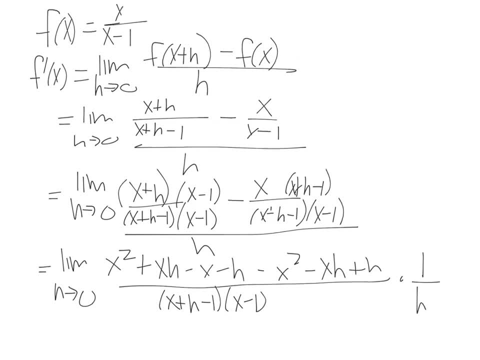 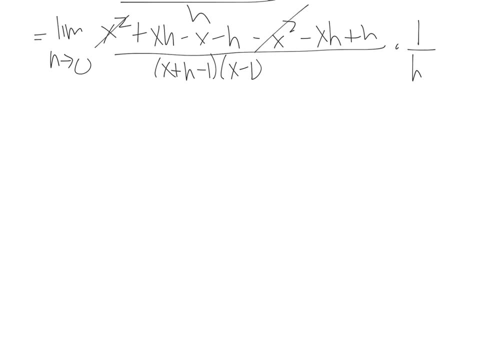 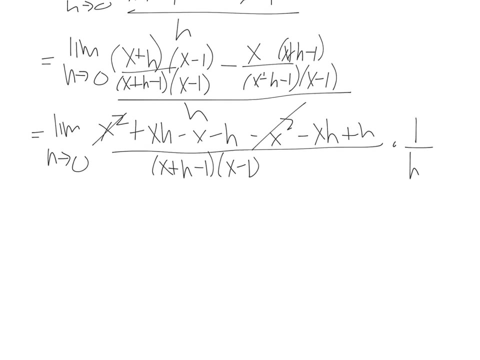 by the reciprocal multiplying by one over h, And so we can start cancelling Our x squareds. cancel, and I think I made a mistake somewhere. oh, yes, right here. So what we had this should be x squared minus x h Instead of this. 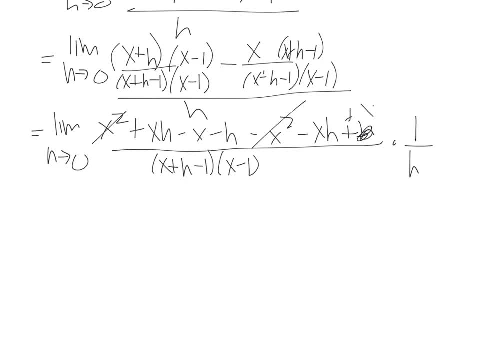 This was. This was being an H. this should have been a plus X, So we had X times 1, or minus X times negative. 1 will give us a plus X, So there's the mistake that I had. So now we have our negative X. 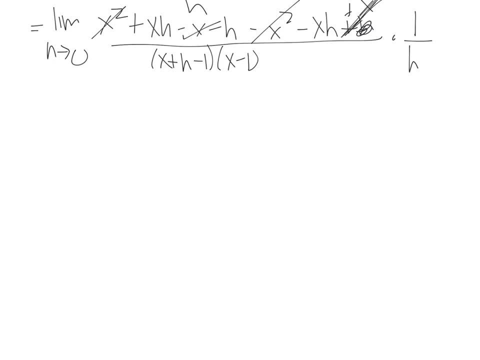 and this X right here cancels, and so we're left with the limit, as H goes to 0, of XH minus H minus XH. Oh, and those XHs will also cancel too, so rather we're just left. 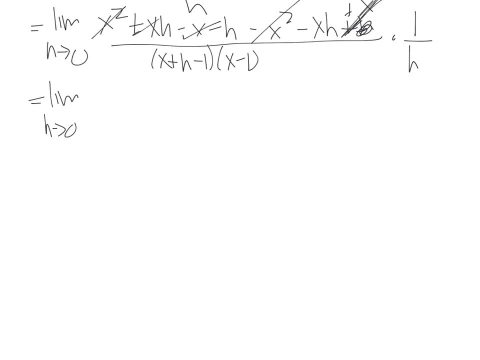 with. so these cancel. so we're just left with minus H over X, plus H minus 1 over X minus 1.. Now that means our Hs will cancel and we're left with the limit, as H goes to 0, of negative. 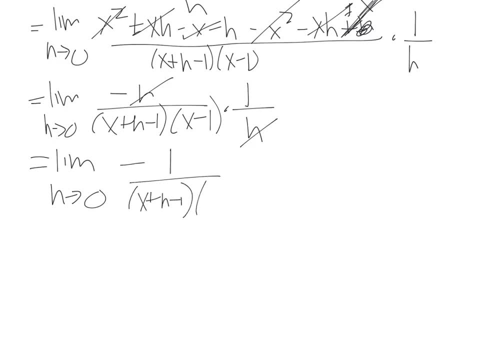 1 over X plus H minus 1 times X minus 1, evaluating the limit when H is 0, we get this is negative 1 over X plus 0 minus 1 times X minus 1.. Well, this term is just X minus 1, so this is negative 1 over X minus 1. quantity squared. 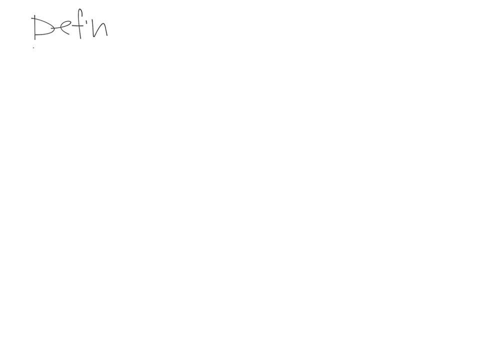 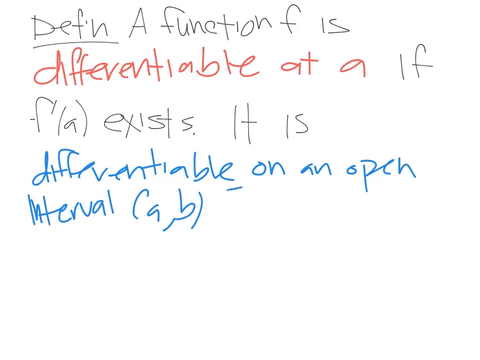 Now we have a definition and this definition says that a function, f, is differentiable. pertinent, Okay, Perfect, at A. if f' of A exists, then we say it is differentiable on the open interval. or on an open interval, say this interval is from A to B, or really it could also be from A. 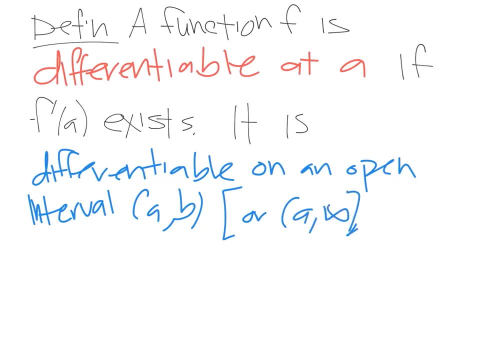 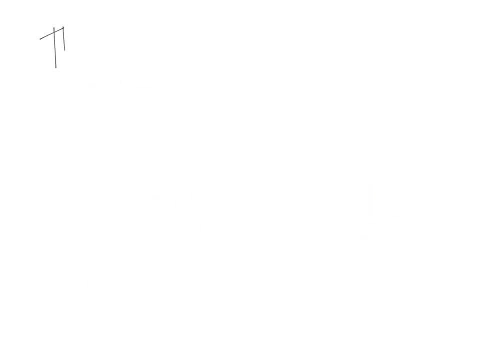 to infinity, or let's say negative infinity to A, or even negative infinity to positive infinity. So on some interval We have it's differentiable. if it is differentiable at every number. on the interval, We now have a theorem, and this theorem states the following: 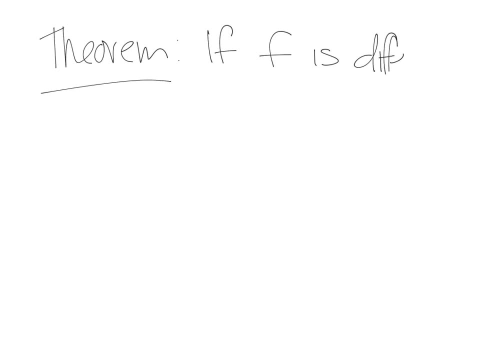 If f is differentiable at the point A, then f is continuous at the point B. So now you might ask yourself: when would a function not be differentiable? We'll talk about that in a minute. Now, when can a function not be differentiable? 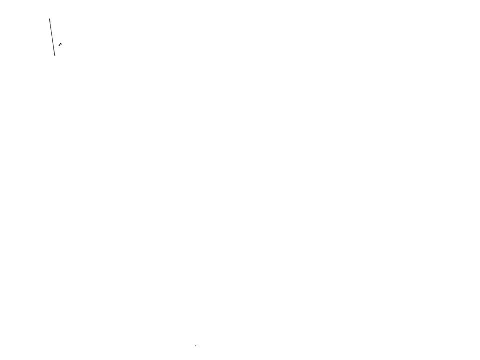 There are three possibilities. The first possibility is that something called a corner exists, and what that means is that you might have a smooth curve And then all of a sudden it goes right here and it goes just straight down. Not smooth, just a little kink in the curve. 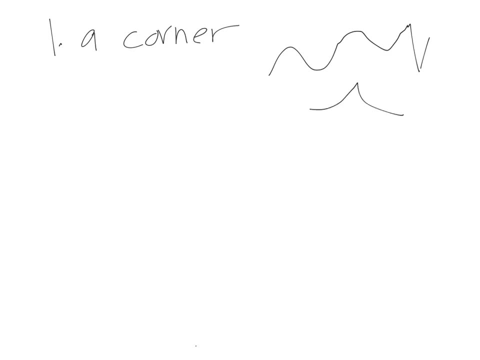 Something like that and like that. When you see that in the graph it is continuous but it's not smooth, There's a little corner happening. So the first thing is a corner. The second thing is that if we have a discontinuity, 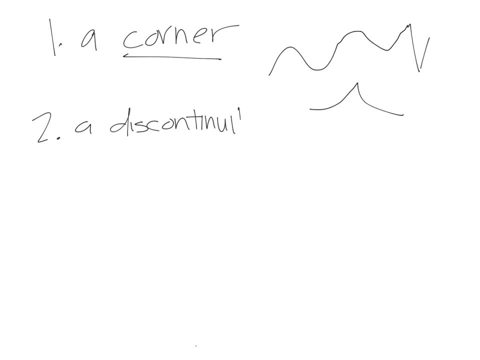 Discontinuity, Discontinuity, Discontinuity, Discontinuity Meaning. we might have the graph that looks like this, and then it continues like that. It's not continuous at that point, right here, and so it is not differentiable at that point. 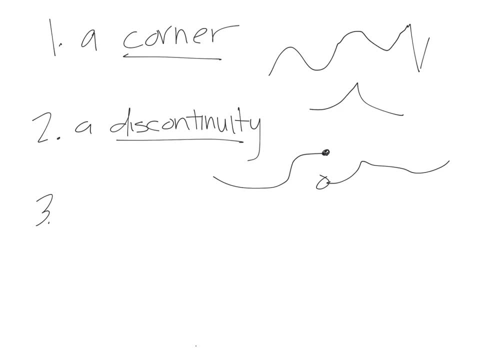 Now the third possibility is that if there is a vertical tangent line, Meaning that the limit as x approaches a of f, prime of x is equal to infinity, or the vertical tangent line is at the point x equals a. Now we found that, given a function f, we can find its derivative by, and we denote it that 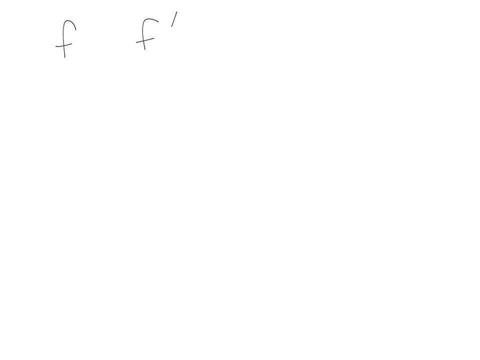 way, But the derivative is a function in itself. We can take the derivative of the derivative, In which case, if we have f prime and we take its derivative, we could write it like this: And this is what we would say: is the second derivative of f. 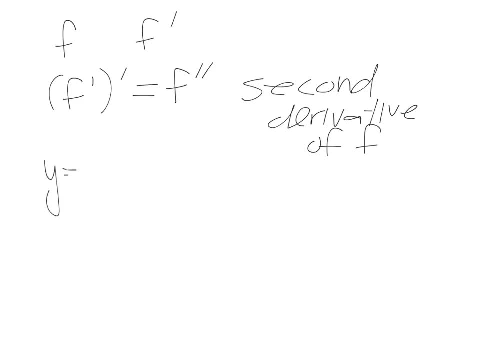 And so another way of writing this: If we have that y, If we have that y is equal to our function f of x, The derivative d dx of the following: dy dx is equal to d squared, y over dx squared. This is a notation used by Leibniz. 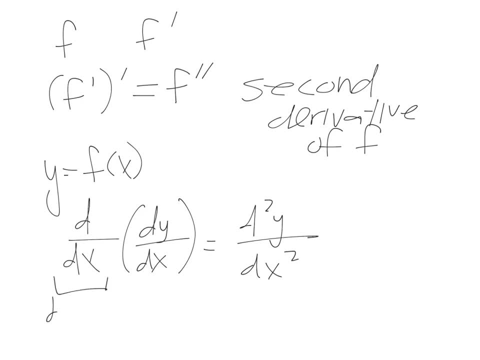 So this first term, This is really saying the derivative of The derivative of The derivative of. This is another way of writing the first derivative. So instead of writing f, prime of x, we could have written it as dy, dx, And then this term over here. 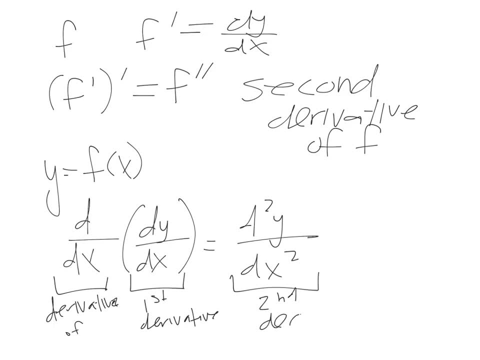 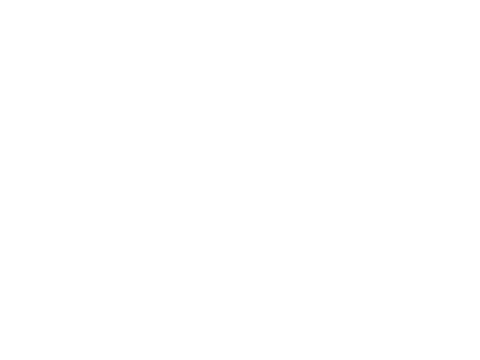 This is what we call the second derivative. Similarly we can calculate the third derivative, So y triple prime is can also be written as f triple prime of x, Which means we're taking the derivative d- dx of the second derivative. So d squared, y dx squared. 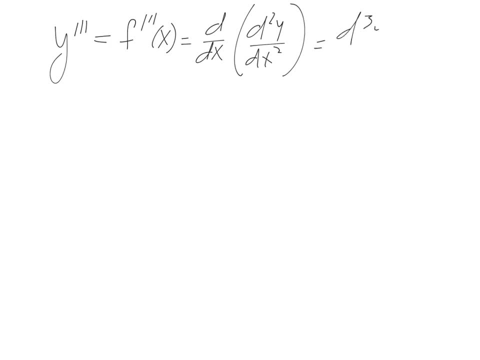 And what that comes out to Is d cubed y. And then we have the second derivative, So d squared, y, dx squared. Now, these are just ways of writing the same thing. You might see it as just the triple prime, Or you might see it like this: 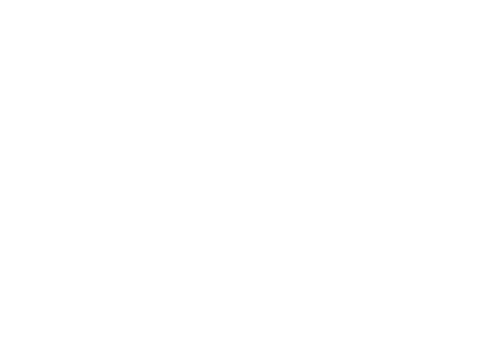 But it just all means the same thing: The third derivative. So let's do an example: If we're given, f of x is equal to x cubed minus x. Find the first, second and third derivatives. Find the first, second and third derivatives. 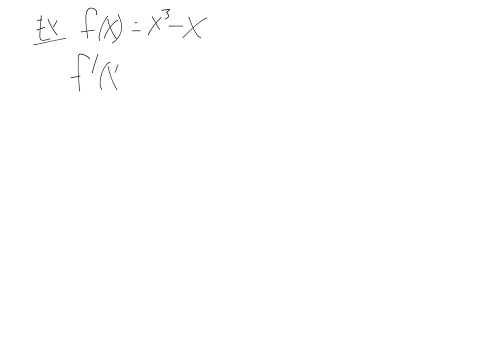 From the earlier video we found that the first derivative, f prime of x, is equal to 3x squared minus 1.. So to find the second derivative, f double prime of x, we just need to take the derivative of this Of the first derivative. 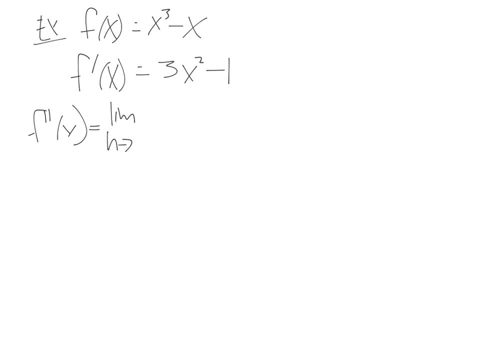 So this is equal to the limit, as h goes to zero, of f prime of x plus h minus f prime of x all over h. So we have the limit, as h goes to zero, of three times the quantity x plus h squared minus 1 minus 3x squared minus 1, all over h. 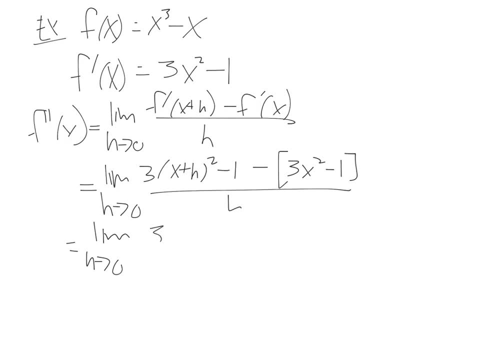 So we get the limit, as h goes to zero, of 3x squared minus h. F prime of x, F prime of x squared minus 1 over h, squared plus 6xh plus 3h squared minus 1, minus 3x squared plus 1, all over h. 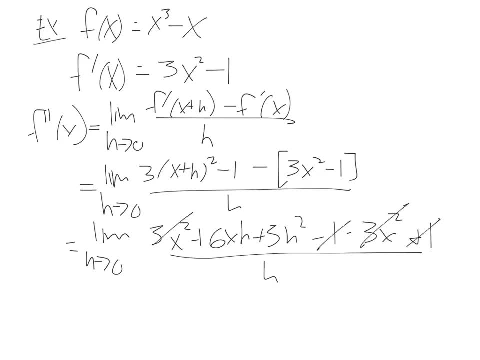 Now our 1's will cancel and our 3x squared's will also cancel, leaving us with the limit- as h goes to 0, of 6xh plus 3h squared all over h, And now we can cancel our h's and our h squared's cancel. 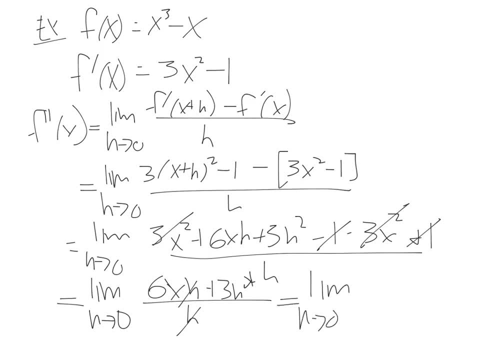 So this is the limit, as h goes to 0,, of 6x plus 3h. And now evaluating that, when h is 0, we get this is 6x plus 3 times h squared minus. 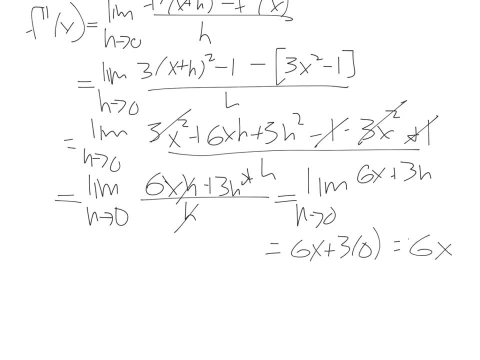 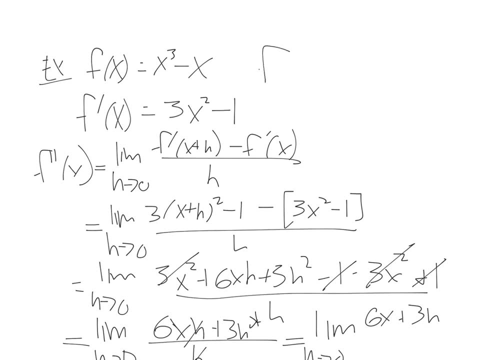 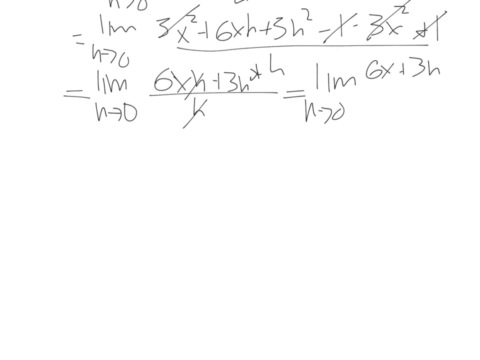 3h, squared times zero or just 6x. So filling that in up here, we get that the second derivative, f double prime of x, is 6x. And then finally, to find the third derivative, we get f triple. 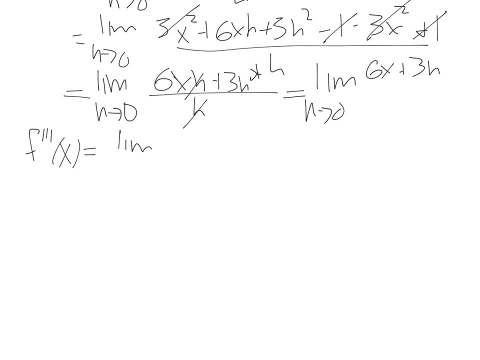 prime of x is the limit, as h goes to zero, of the second derivative of f of x plus h, minus the second derivative of f of x all over h, which is the limit, as x goes to zero of remember, the derivative is just 6x. so 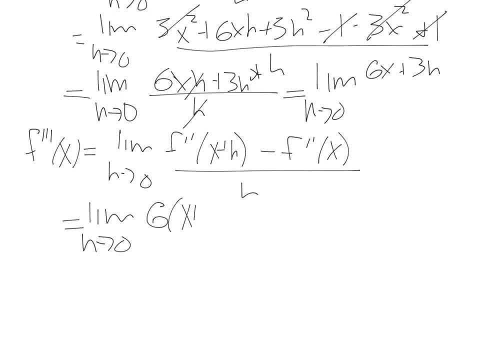 so we have this is going to be 6 times x plus h minus 6x all over h. so we get the limit, as h goes to zero, of 6x plus 6h minus 6x over h and our 6x's cancel. so this is the limit. 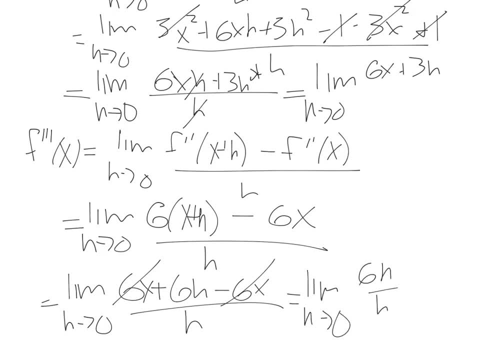 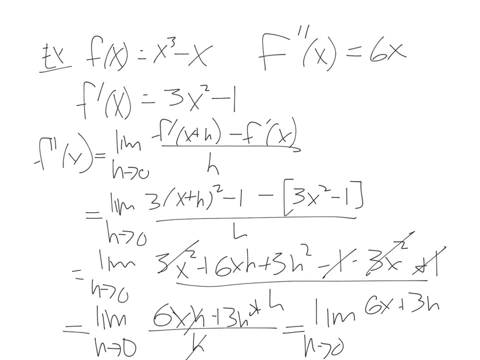 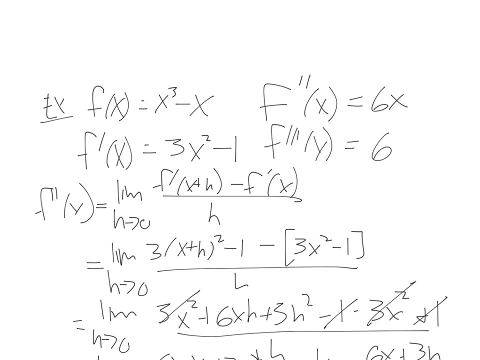 as h goes to zero of 6h over h, which cancels, and that is just 6.. So, oops, moving all the way back up to the top, there we go. moving all the way to the top, we get. our third derivative is just 6, so we had our function f of x, our first. 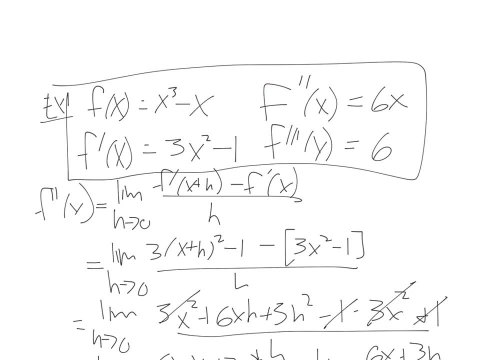 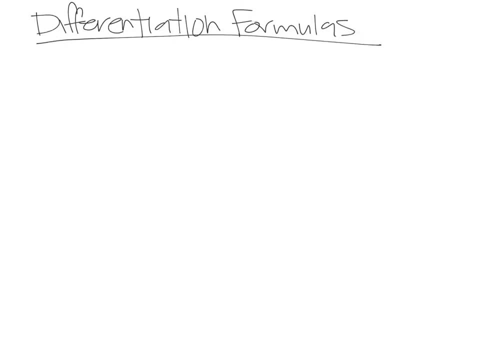 derivative, our second derivative and our third derivative. Now that you're familiar with finding the derivative of a function using the limit definition, we're now going to go over some formulas that will make your life a little bit easier. So first of all recall, if we have f of x, is some constant like f of x is equal to 3,. 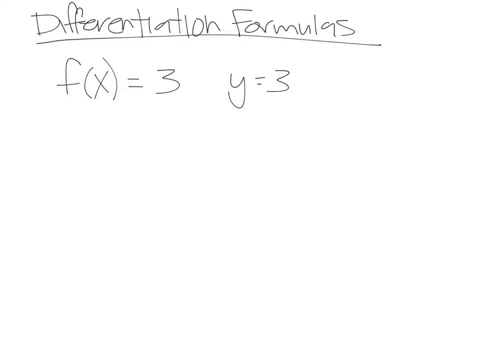 that's the line: y equals 3, and that's a horizontal line. Well, what's the slope of that horizontal line? The slope of that horizontal line is 0.. So the derivative of f, of x equals, or f prime, rather, is going to be 0.. 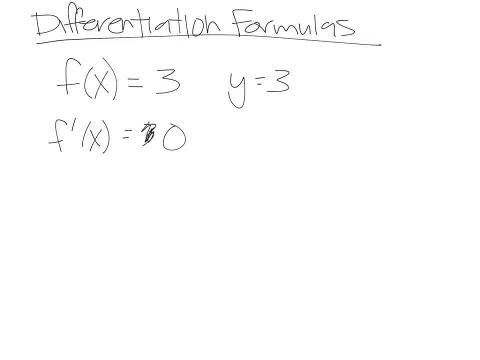 So any sort of constant function we're going to have is going to be 0. So the derivative of a constant function, f of x equals f. prime is going to be 0. So any sort of constant function will be d. dx of some constant is equal to 0.. 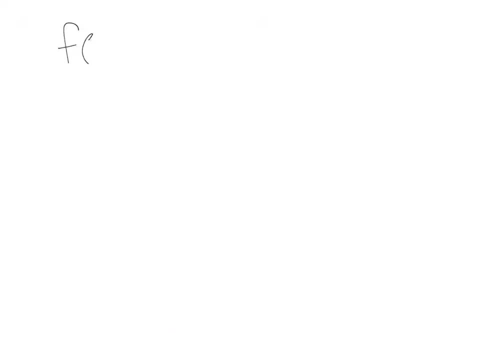 Next we'll take a look at what happens if we have our f of. x is just simply the line x. So really we're looking at the straight line: y equals x. Well, what's the slope of that line? The slope of that line is just 1.. 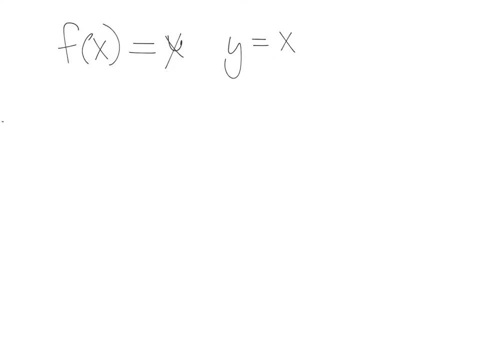 So we have that the derivative is going to be d. dx of x is just 1.. So this is now. we're starting to look at different powers. Now, what about the derivative of the function f of x equals x prime. So we'll take a look at the straight line. 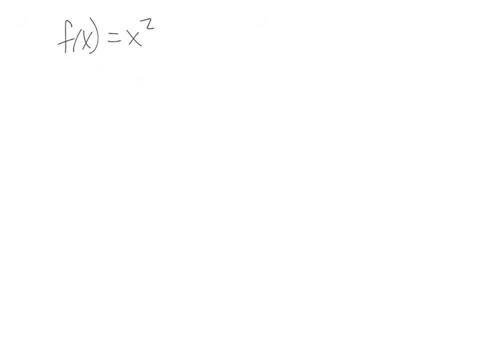 So we have that the derivative is going to be d. dx of x is just 1.. equals x squared. well, if we use the definition f, prime of x is equal to the limit as x, or rather, excuse me, as h approaches, zero of f of x plus h minus f of x all over h. so this is the limit. 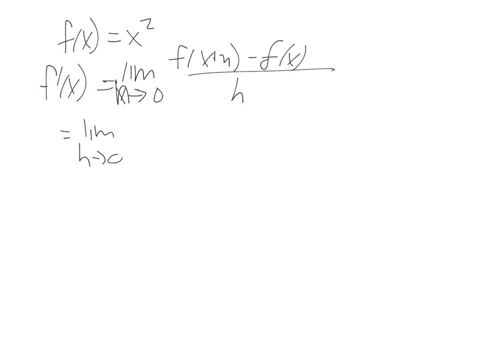 as h approaches zero, of x plus h, quantity squared minus x, squared all over h, which is the limit. as h approaches zero, x squared plus 2xh plus h, squared minus x, squared all over h, and we can cancel our x squareds. so this is the limit as h approaches zero. 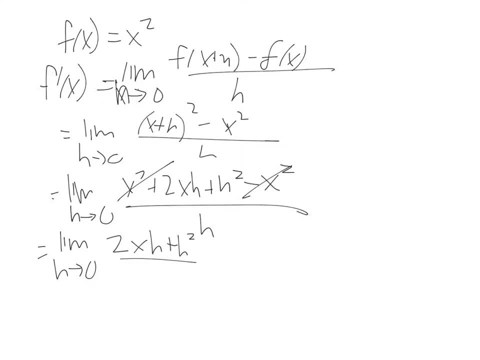 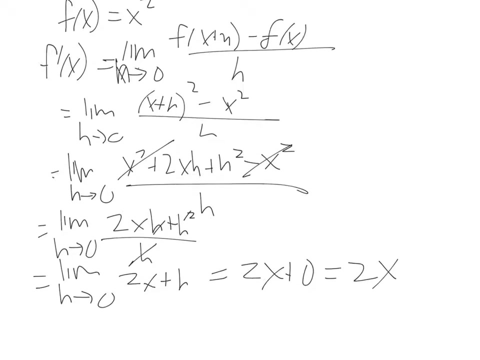 of 2xh plus h squared all over h and we can cancel our h's. so we're left with the limit as h approaches, 0 of 2x plus h. evaluating this when h is 0, we get this is 2x plus 0 or just 2x. so therefore we get that if our function is f of x. 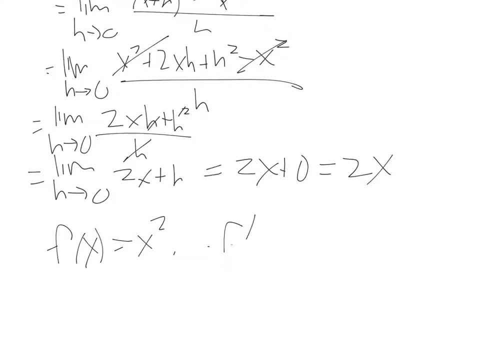 is x squared, the derivative f prime of x is 2x. it can also be shown that if your f of x is x cubed, the just the derivative of x. f prime of x is 3x squared and even if f of x is x to the 4, we get that the derivative of f is going to be. 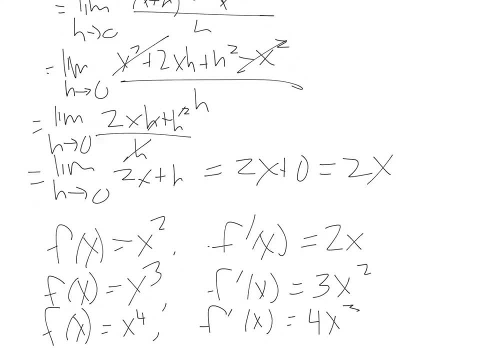 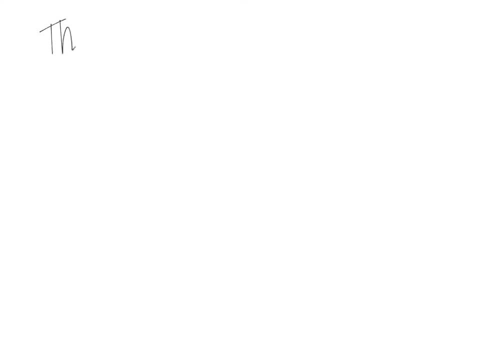 4x cubed and you might notice there's a pattern going on which leads us to the next rule. this is called the power rule, and the power rule says that if n is is a positive integer, then we have the following: then ddx, so the derivative of x to the nth power is just the power n times x. 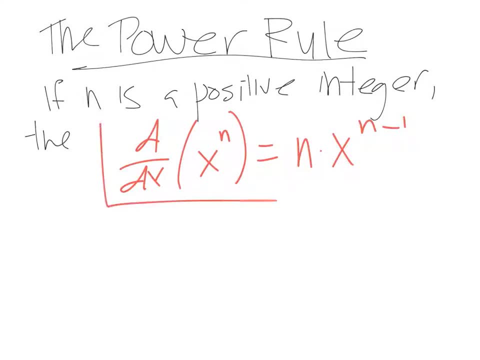 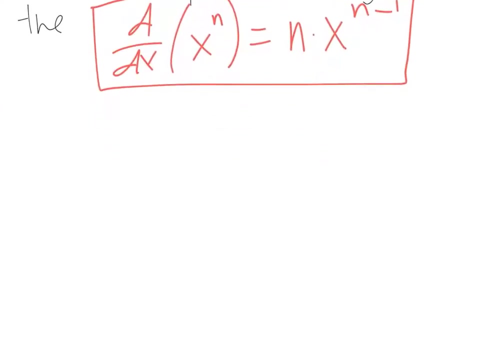 raised to the power minus 1. So if you know this formula, then you won't have to compute the limit or the derivative by using the limits. So let's do some examples. So let's calculate 3,. how about? h of t is equal to t to the 7th. and maybe how about k of t? or maybe let's use r. 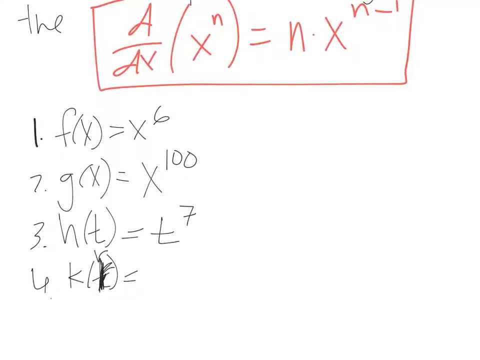 So k of r, let's use: r is equal to r cubed. So to find the derivative of each of these, we would have f prime of x, or you might see it written as d? dx of f or d? dx of x to the 6th. 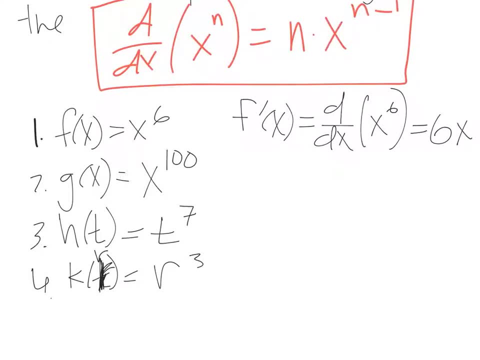 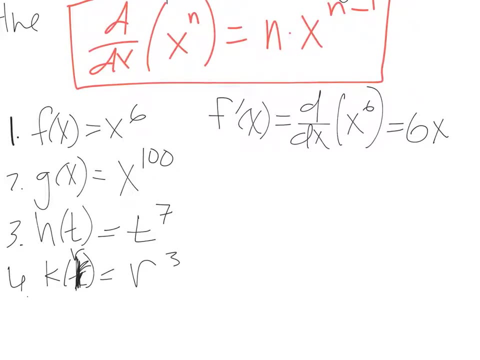 Well, we take the power 6, times x to the power minus 1.. I'll just slide this over a little bit to the power minus 1,. so x to the 6th minus 1, which is 6, x to the 5th. 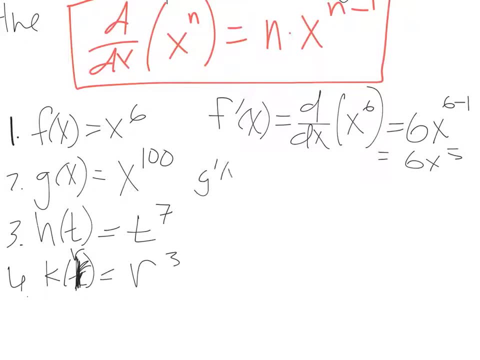 Same thing for our g. So g prime of x is d dx of x to the 100, which is going to be 100 times x to the 100 minus 1, or 100, x to the 99. The derivative of h. so h prime of t. well, since we're dealing with t instead of writing d dx, 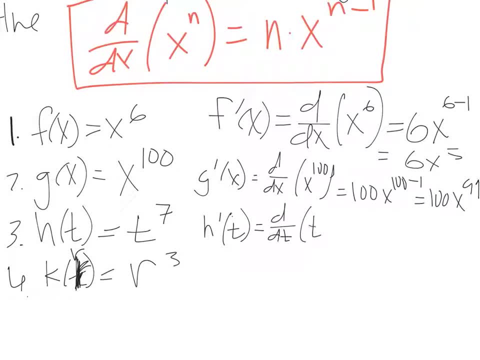 this would be d dt of t to the 7, and this is going to be 7 times t to the 7 minus 1, or 7t to the 7th. And finally, for our r, for our k, so the derivative of k with respect to r. 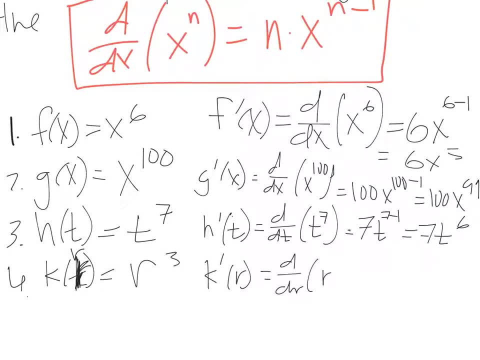 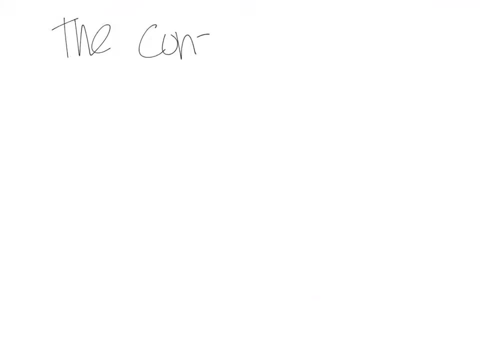 so d dr of r cubed is going to be 3r to the 3 minus 1, or 3r squared. The next rule we have is the constant multiple, And the constant multiple rule states the following: If c is a constant and then the function f is a differentiable function, 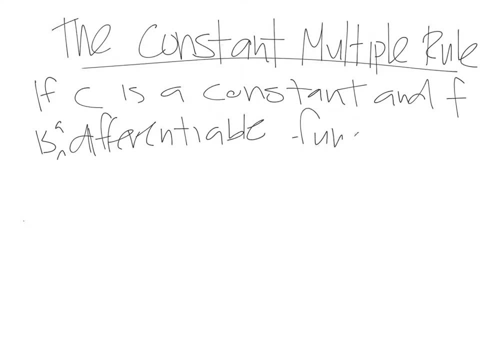 it's a differentiable function. then we have the following: We have that the derivative d dx of c times our function f of x is just equal to the constant c times the derivative of f of x. So we can actually pull the constant out in front. 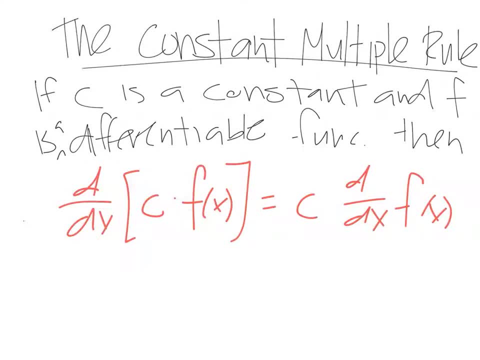 This way we don't need to compute a whole other derivative, We just take the constant in front and then we can figure out what the derivative of f of x is. So an example of this would be: if we have- we're trying to compute- the derivative of 5x to the 6th. 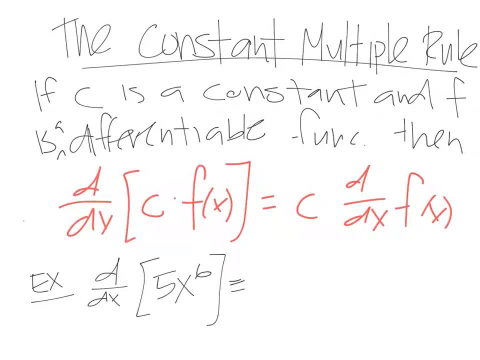 this is the same as computing 5 times the derivative of x to the 6th. This is the same as computing 5 times the derivative of x to the 6th, Because 5 is just a constant. we pulled it in front right here. 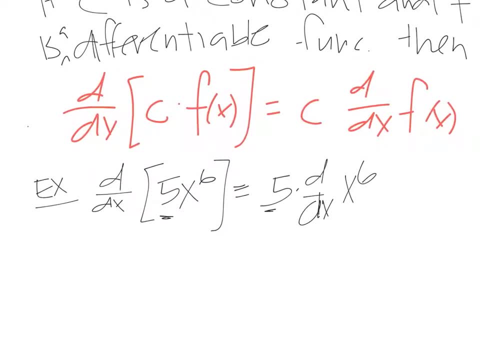 And now we know the derivative of x to the 6th by using the power rule, So this is going to be 5 times. the derivative of x to the 6th is 6,, x to the 6th minus 1, or x to the 5th. 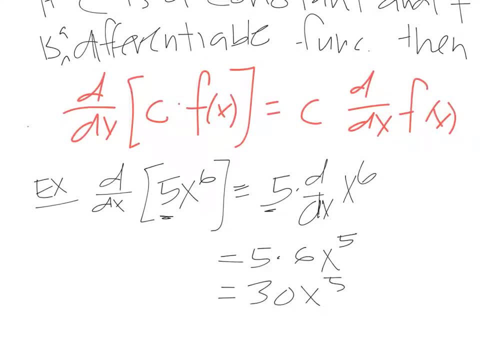 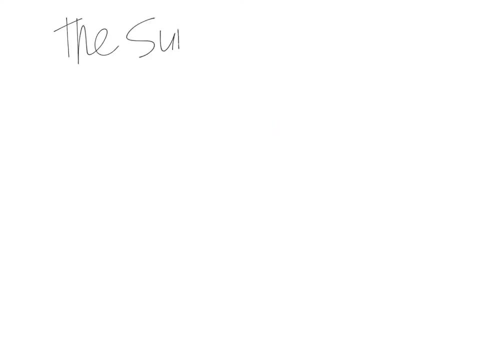 So we have? our answer is 30x to the 5th. The next rule that we have is called The sum rule, And the sum rule says that if we have two functions- f and g- and they are both differentiable, 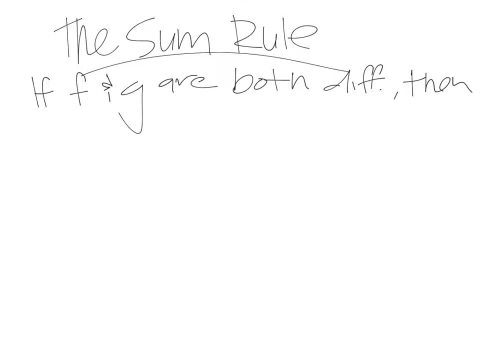 then what we have is the sum of the two, or the derivative of the sum of the two, d dx of f of x plus g of x, is equal to the sum of each of their derivatives: d dx of f of x plus d dx of g of x. 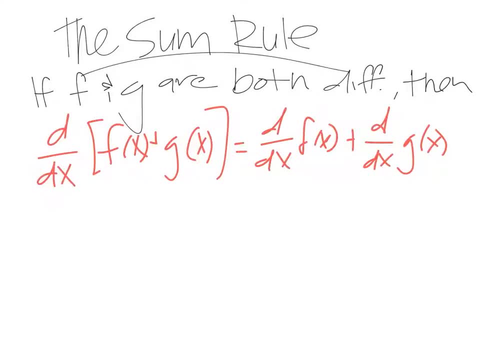 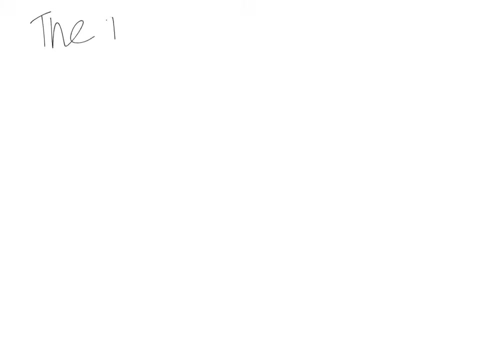 Another way you might write this, using the prime notation, is that f plus g prime is equal to f prime plus g prime. The next rule we have is the difference rule And this says, similar to the sum rule, that if f and g are both differentiable, 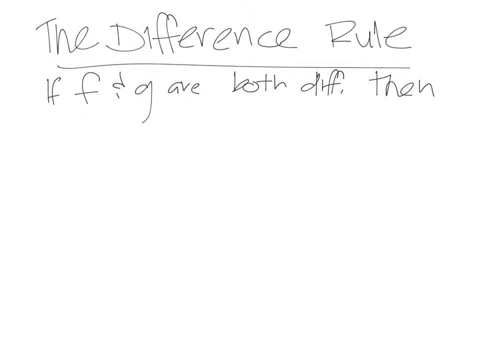 then we have that The derivative of the difference of the two is going to be the difference of the derivatives Meaning d dx of f of x minus g of x is equal to d dx of f of x minus d dx of g of x. 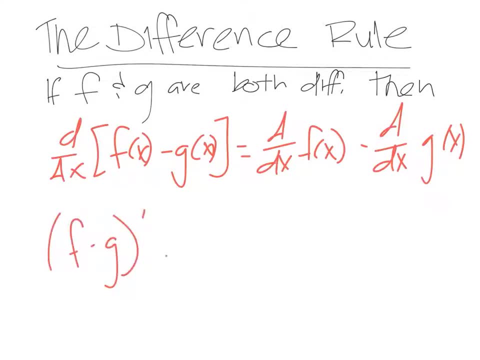 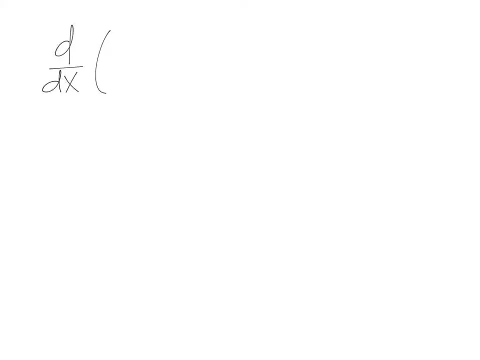 So in other words, if we take f minus g prime, this is f prime minus g prime. So if we did an example and we're trying to find the derivative of the following: 3x to the 7th minus 4x to the 5th plus 2x to the 4th minus 7x plus 2,. 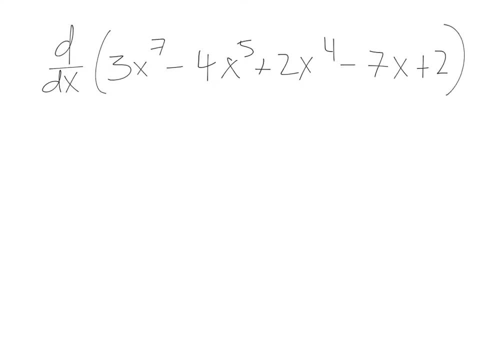 well, we can break this up into individual pieces. So this is going to be the derivative of 3x to the 7th, minus the derivative of 4x to the 5th, plus the derivative of 2x to the 4th minus the derivative of 7x. 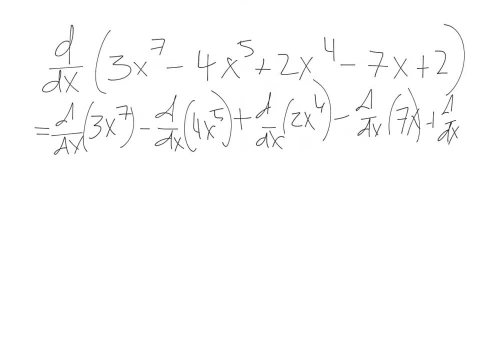 Plus the derivative of 2.. Well, this first one, the derivative of 3x to the 7th. well, 3 is a constant, so we can pull that out and that's 3 times the derivative of x to the 7.. 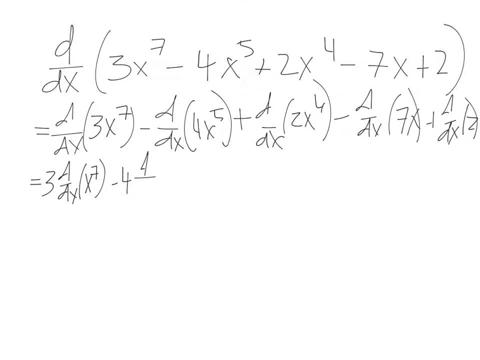 Minus, and then the next term. we can pull out 4, so we get the derivative of x to the 5th. Plus we can pull out 2, so we get the derivative of x to the 4th. Pull out 7 times the derivative of x. 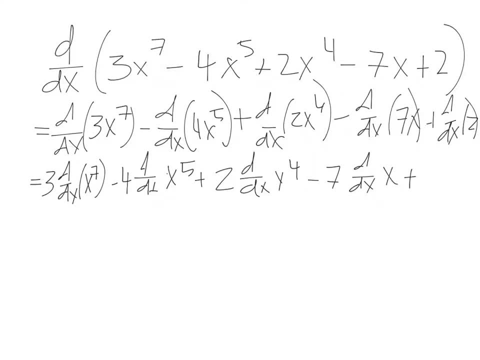 plus. well, the derivative of a constant is just 0. So we don't need to worry about that. Now, the derivative of x to the 7th is 7x to the 6th, because we took the power of 7 and subtracted 1.. 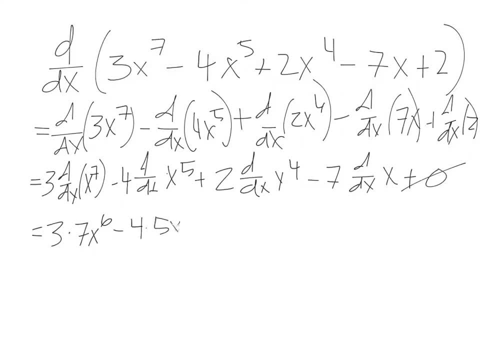 The derivative of x to the 5th is going to be 5x to the 4th and we get plus 2, and the derivative of x to the 4th is going to be 4x cubed And the derivative of x is just x. 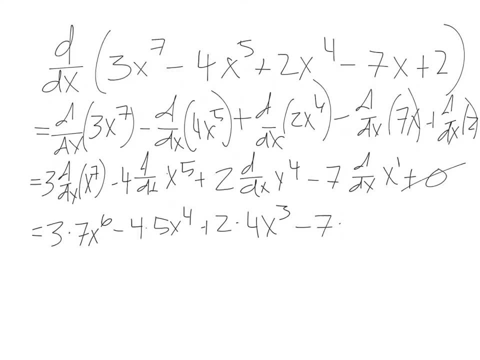 so really the derivative of x. think about it as x to the power of 1,, so that's 1 times x to the 1 minus 1, or well, 1 minus 1 is x to the 0, and anything to the 0 power is 1.. 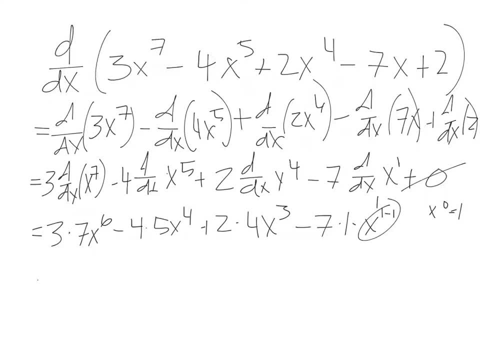 So this is just 1.. So here we have 21x to the 6th minus 20x to the 6th, x to the 4th plus 8x cubed minus 7.. And there's no x here, because it's really x to the 0 power. 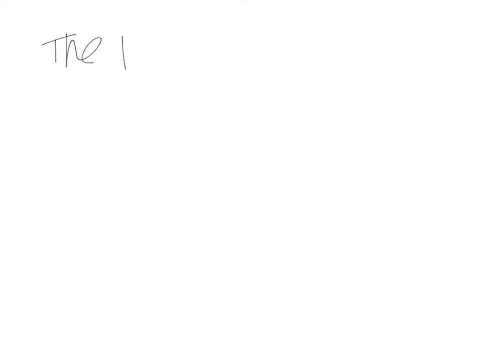 The next rule we have is called the product rule, And the product rule states the following: If we have two functions- f and g- and they are again both differentiable, then we have the following: Then we have the derivative dx. 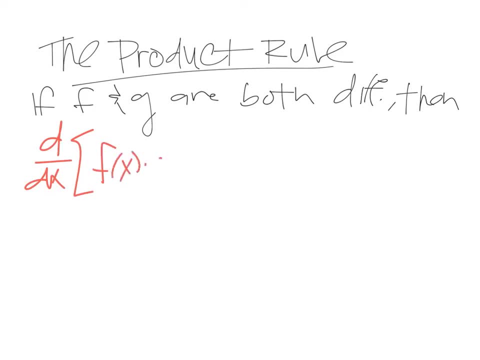 of the product: f of x times g of x. that's equal to. this is where it gets. it may not be as intuitive: f of x times the derivative of g of x, plus g of x times the derivative of f of x. 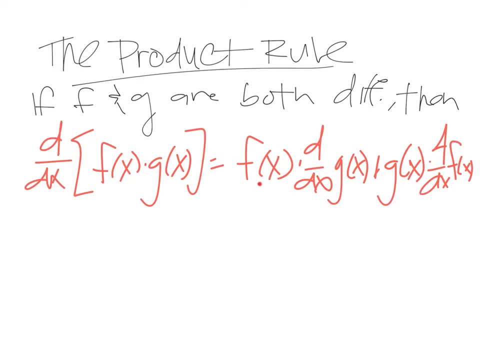 So if we have the derivative of the product, it's the first term times the derivative of the second plus the second times the derivative of the first. So let me write this in prime notation and this says that if we have f times g, 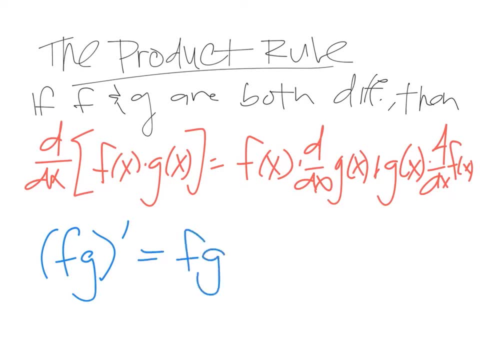 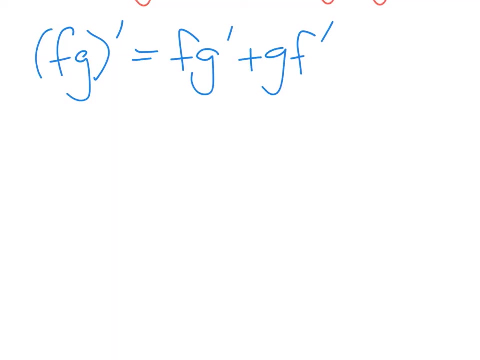 and the derivative of that. this is going to be f times g prime plus g times f prime. So let's do an example. Let's say we have some function like this. Let's say we have for function capital F of x. 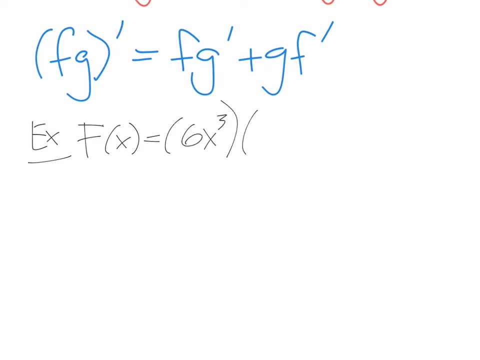 is going to be six x cubed times seven x to the fourth. Well, you can think of this as our f and this would be our g. So the derivative of capital F is going to be the first term. 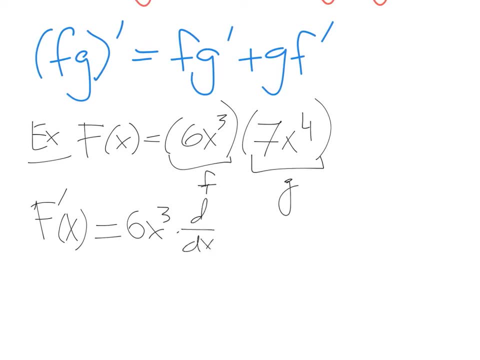 six x cubed times the derivative of the second term, seven x to the fourth, plus the second term, seven x to the fourth times the derivative of the first term, six x cubed. And now we can compute each of these. 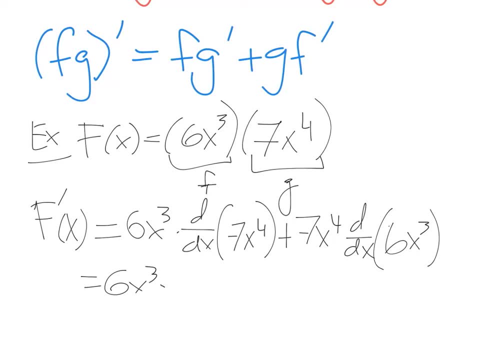 So this is going to be six x cubed times. the derivative of seven x to the fourth is going to be seven times. the derivative of x to the fourth is four times x cubed, because we're taking one less than the power. 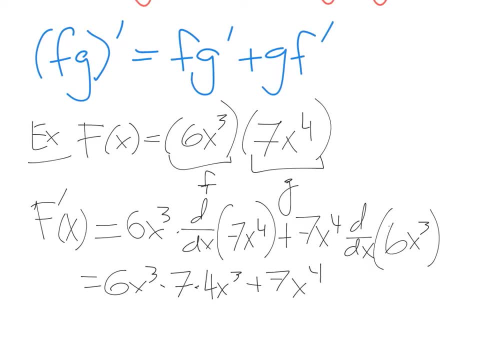 plus seven x to the fourth times six times. the derivative of x cubed is three x squared, And so, multiplying six times seven times four, we get 168, and then x cubed times x cubed. 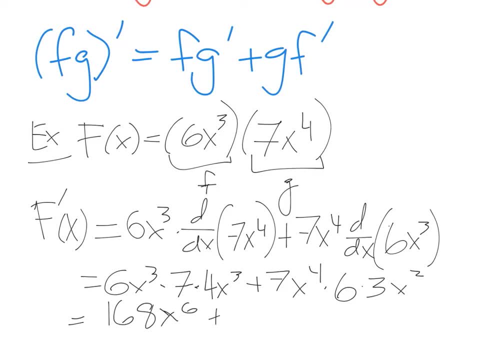 would give us x to the sixth plus, and then, multiplying out over here our seven and our six and our three, we get 126, and then x to the fourth times. x squared is also x to the sixth. 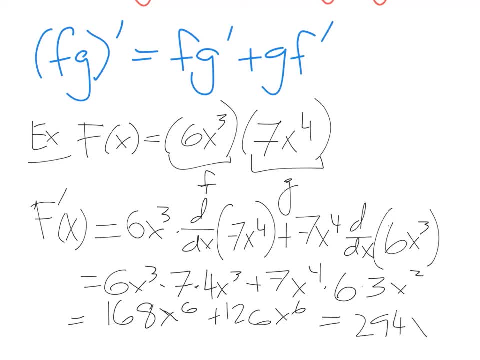 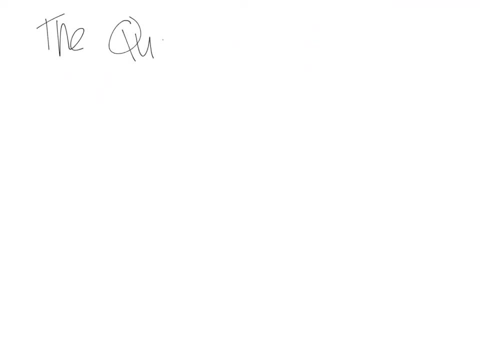 so this can simplify to 294, x to the sixth. The next rule is called the quotient rule. in this rule people can get confused, so let's go over this carefully. the derivative of the quotient. 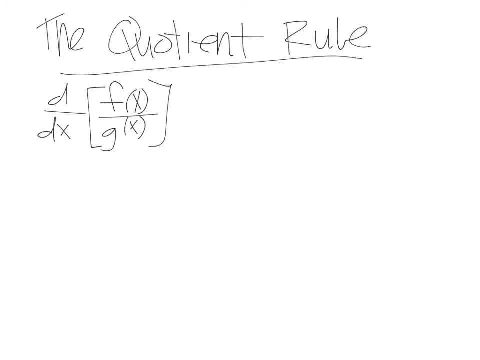 f of x divided by g of x, this is equal to the following: g of x times the derivative of f of x, minus f of x times the derivative of g of x, all divided by: 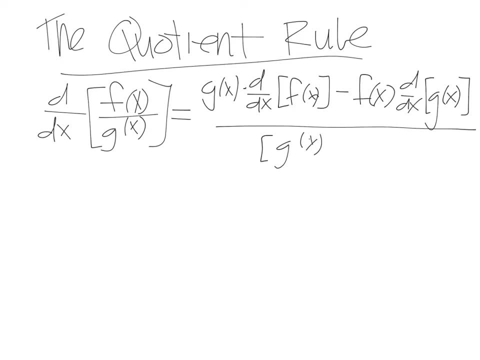 g of x, quantity squared. The difficult thing with this is knowing which one comes first. since we're subtracting, order does matter, so we need to make sure that we go in this order and then in prime notation. 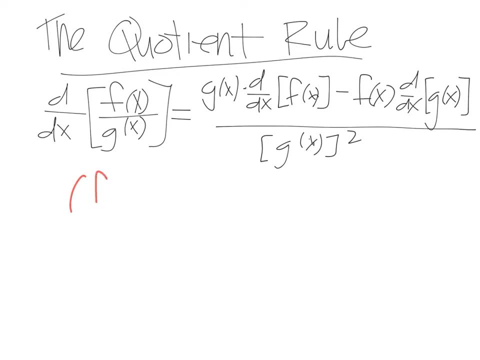 this is going to be rather not r, but f over g prime equals g times f prime, minus f times g prime over g squared. So doing an example for this we get, we'll do the following: 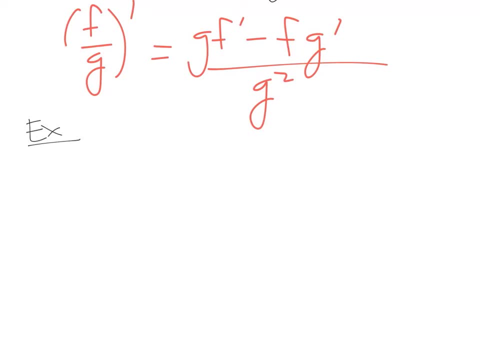 if we're given that our function- let's call this f- of x is equal to x squared plus x minus two divided by x cubed plus six, the derivative f prime of x is going to be the following: 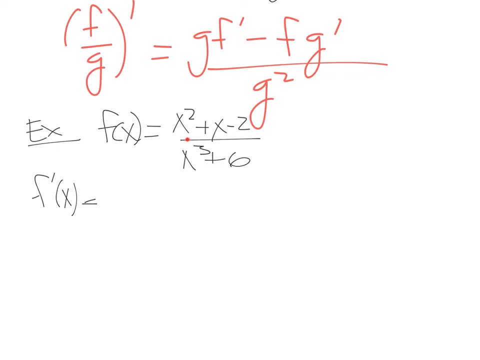 so we look at our numerator and our denominator. so we're going to take the denominator, which in this case is going to be x, cubed plus six times the derivative of the numerator minus. 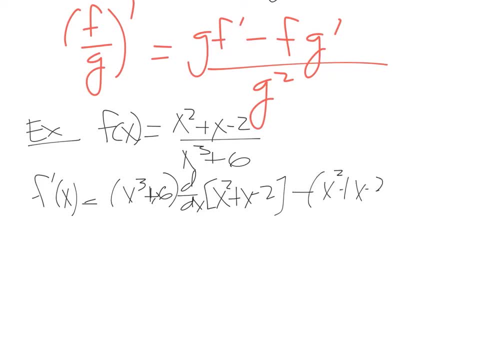 the numerator x squared plus x minus two times the derivative of the denominator x cubed plus six, all divided by the denominator squared. So this becomes x cubed plus six, the derivative of x squared. 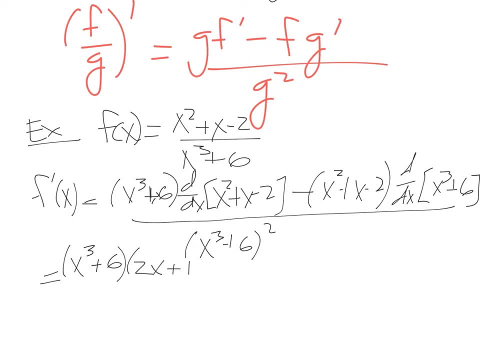 is going to be just two x. the derivative of x is one and the derivative of negative two is zero minus. we get x squared plus x minus two. so this is a plus minus two. 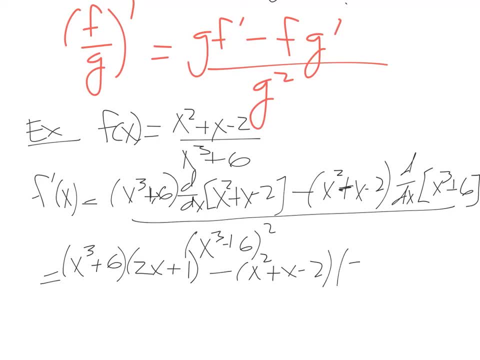 times, the derivative of x cubed is three x squared. the derivative of six is zero, all divided by x cubed plus six, quantity squared Moving along. we can distribute this: x cubed plus six. 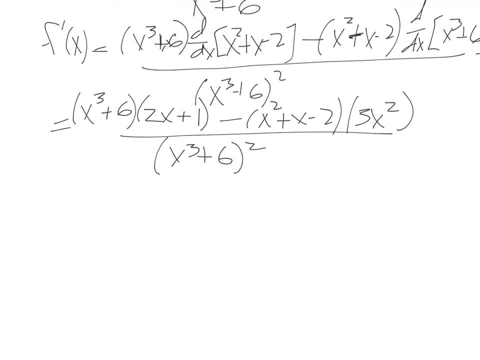 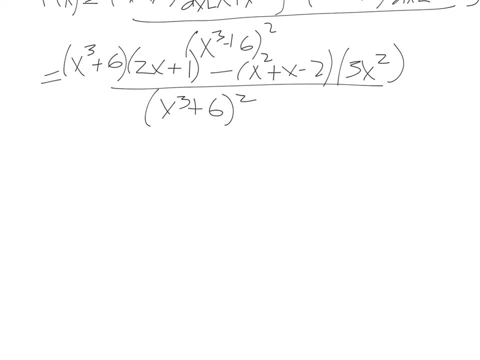 times two x squared plus x cubed, plus six quantity squared. Moving along, we can plus six times two x plus one, and so we get two x to the four plus x cubed. 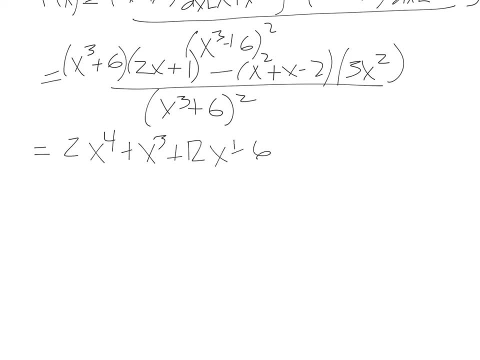 plus twelve x plus six minus three x to the four minus three x cubed plus six x squared, all divided by x, cubed plus six, quantity squared, So we get two x. 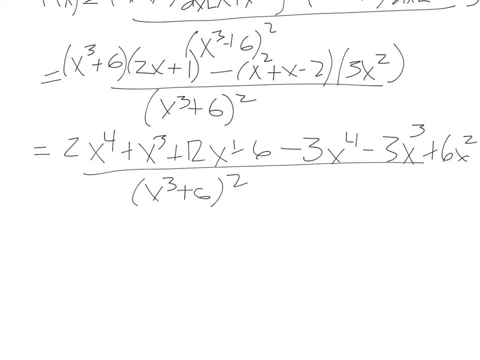 to the four plus three squared, And we can now start combining terms. so our x to the fours combine, and so we get, or we get- negative x to the four, our x. 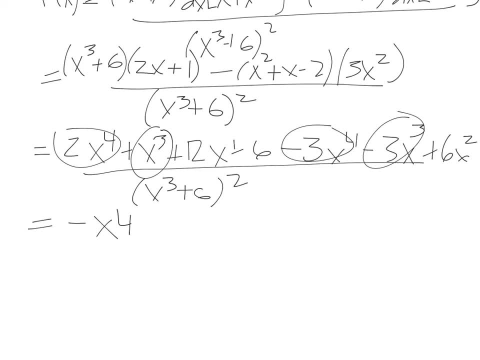 to the power three will combine, and so we get for that minus two x. cubed, we only have one x to the power one, so we get plus twelve x and then plus twelve x. 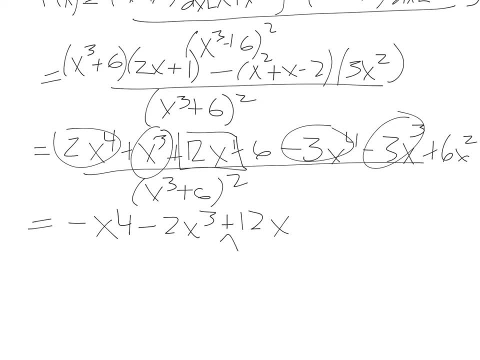 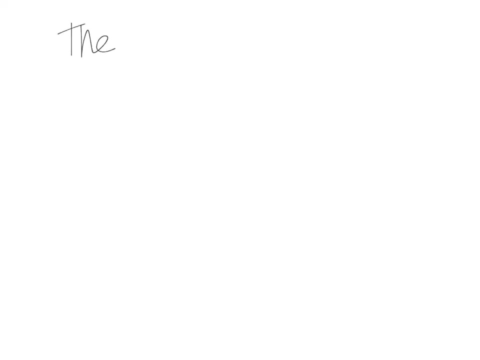 and then we have plus six, and this will all be divided by x, cubed plus six, quantity squared. This is the answer. Not nice, but it is the answer. And now we revisit the power rule. 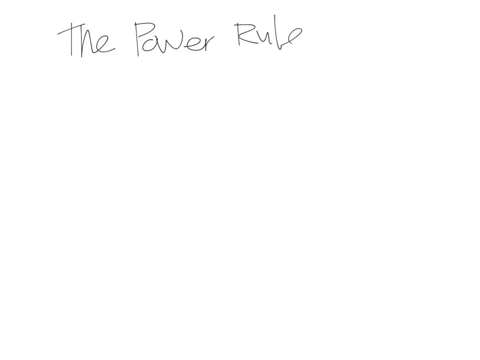 and the power rule will actually apply before. instead of just assuming n is a positive integer, we can assume if n is any real number, then we have the following: So then we have: 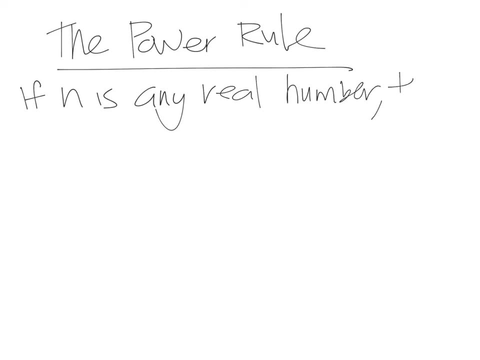 the following. So we have: n is any real number. then we get d dx of x to the power. n is n times x to the n minus one, And 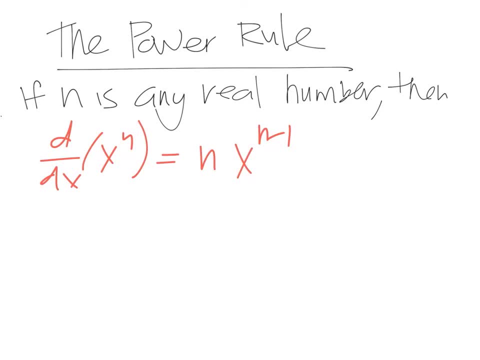 this works for any power, any value, n. So if we have, for example, the derivative of x to the pi, because pi is a number, three point one, four, one five, that's going to be. 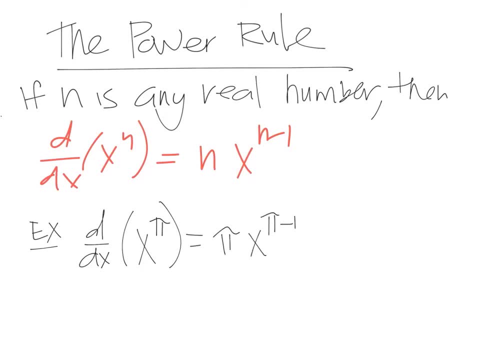 pi times x to the pi minus one. We may also have it as a fraction, So this might be the derivative of x to the one. half is going to be one half. x to the. 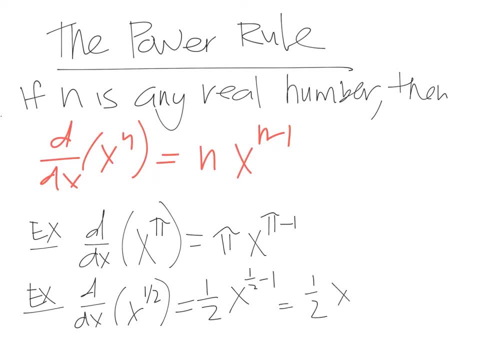 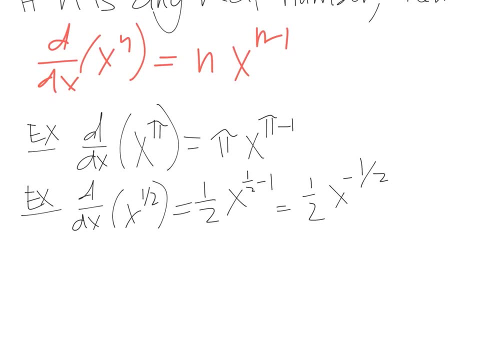 one half minus one or one half. x to the negative one half. What about if we have a negative number? Well, same thing applies. So the derivative of x to the negative three is going to be: 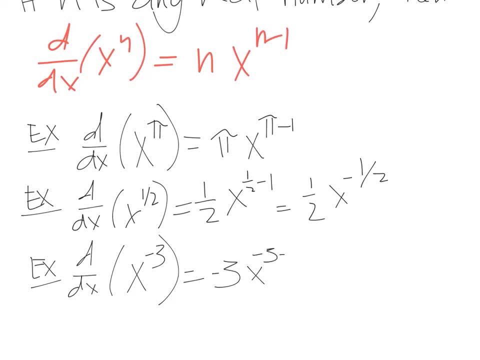 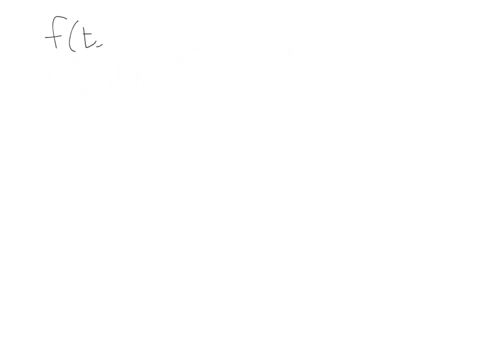 negative three x to the negative three, minus one, which is negative three x to the negative four. Now we'll do some examples. If we're given, f of t is the square root of t times a. 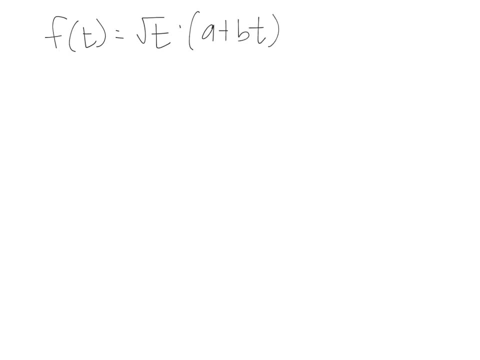 plus b times t. find the derivative. find f prime. Well, when computing derivatives and seeing square roots, the first thing I do is rewrite it as t to the power one half times a plus. 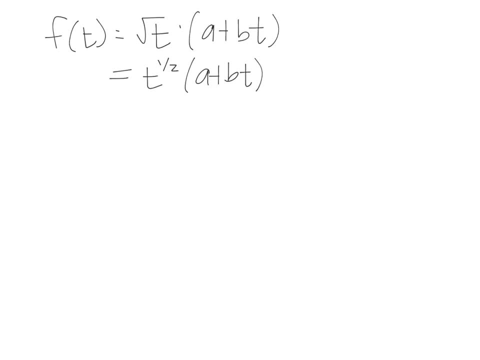 b, t, So you'll almost always want to write square roots and anything with a radical in terms of the power. So, calculating the derivative f prime of t, what we have is the product, And so 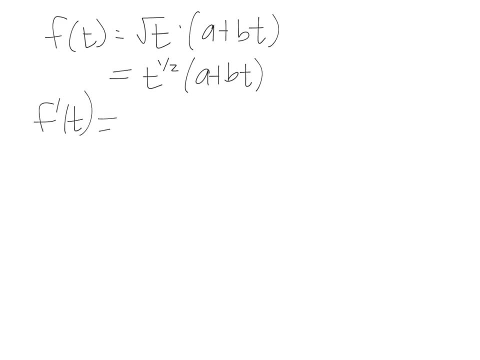 the derivative of the product is going to be the first term, t to the one half times the derivative of a plus b times t plus the second term, a plus b times. 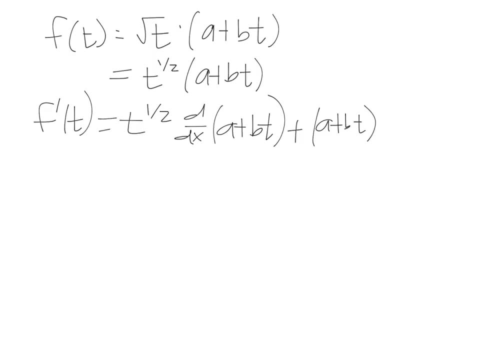 t times the derivative of the first term, which is a plus b, which is t to the one half. So this becomes t to the one half times the derivative of a. a is a constant. 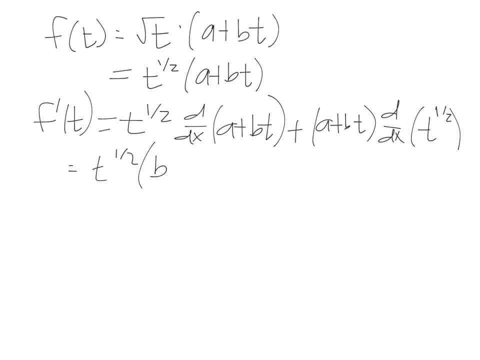 so that's zero derivative of b times t is just going to be b plus a plus b times t times. the derivative of this is one half t to the power, one half minus one. 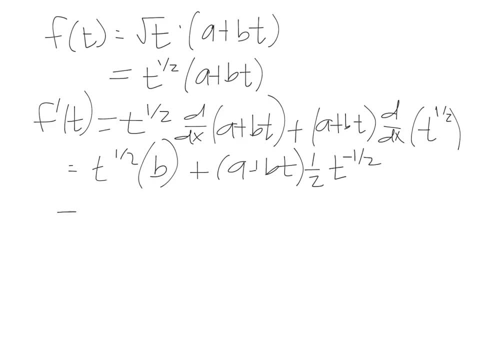 or negative one half. So we get b times t to the one half plus a plus bt. bt times one half t to the negative one half, And that's your answer. You can leave it like this. 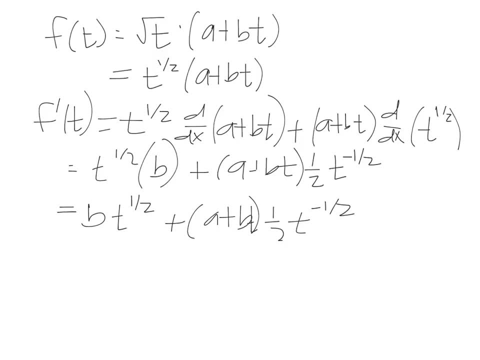 but if you feel more comfortable writing it back as a fraction or as a radical, you can do that b to the square root of t plus a plus bt times one half and t to the negative one half. 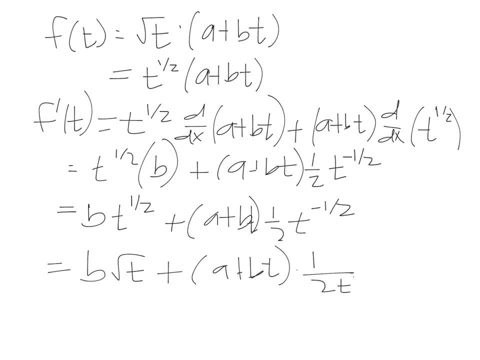 means it moves down to the bottom, and then that is just the square root of t. So we would have had divided by two times the square root of t And the final example that we'll go over today. 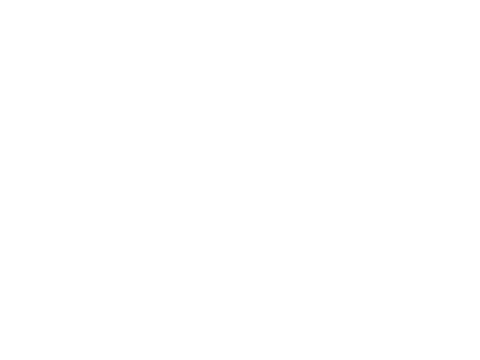 is going to be dealing with the quotient. So if we're given, y is equal to b plus a plus bt, plus a plus bt is equal to the square root of x divided by. 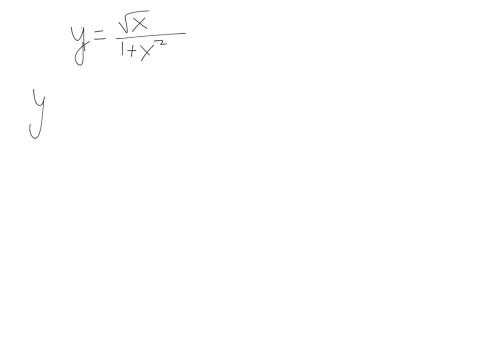 one plus x squared. if we wanted to find a derivative, that will be the following: The derivative is going to be the denominator one plus x squared times the derivative of the numerator. If you recall, if we had. 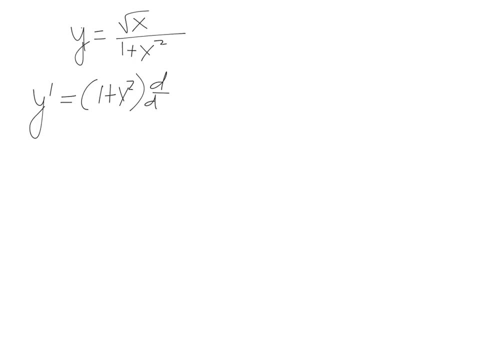 something like f over g plus a plus bt times the derivative of the numerator. If you recall, if we had g prime, the derivative of this is going to be g times f prime. 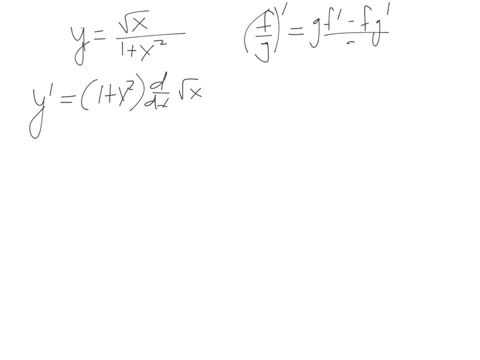 minus f, times g prime divided by g squared. So that's what we have right here. This is our g, this is going to be our derivative of f, and then, continuing on, we get: 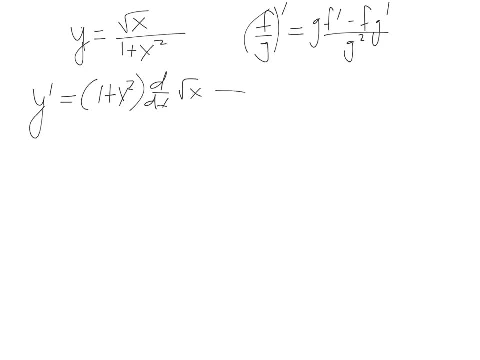 minus f, so minus our numerator, square root of x times the derivative of f, the derivative of the denominator one plus x squared. So this is going to be one plus x squared the derivative of x. 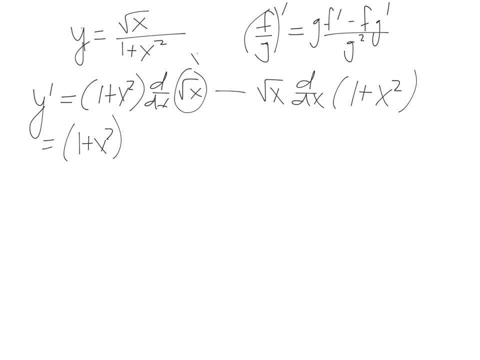 of a square root of. excuse me, the derivative of square root of x, which is really x to the one half, is one half x to the negative, one half minus, and I'm just going to rewrite square root. 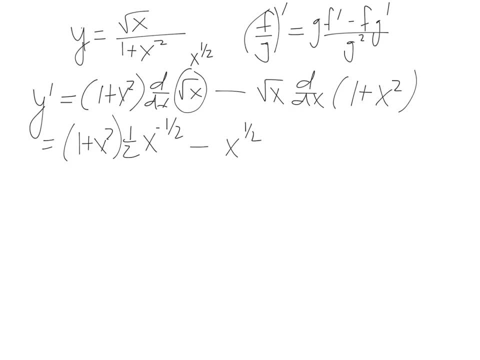 as x to the one half, the derivative of one plus x squared. well, the derivative of one is zero and the derivative of x squared is two x. Oops, I forgot that this whole thing is all going to be. 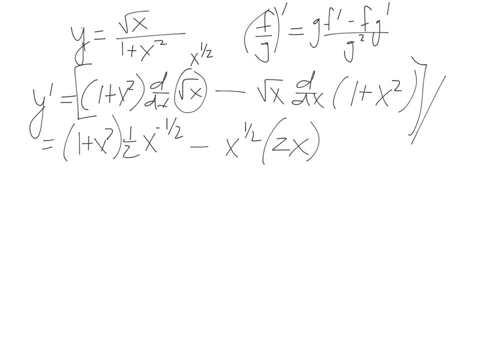 divided by the denominator squared, one plus x squared squared. So this is all divided by one plus x squared squared, And this is all divided by one plus x squared squared. 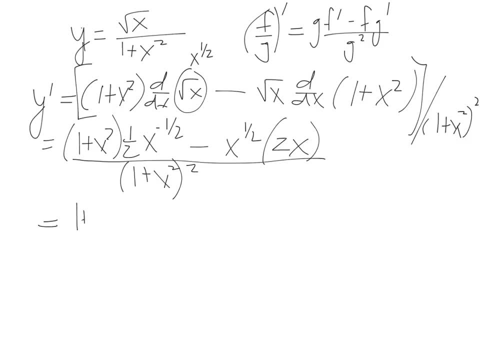 And so, simplifying this, we get one plus x squared times well, times one half, which is the same as saying divided by two. and, just like in the last example, x to the negative, one half can be written as: 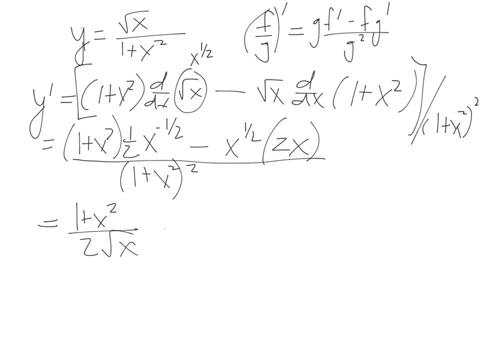 one over the square root of x minus. the next thing is square root x to the one half, or square root of x times two, x divided by one plus x squared, squared, And so here: 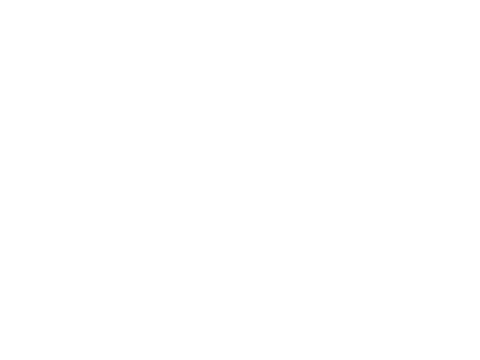 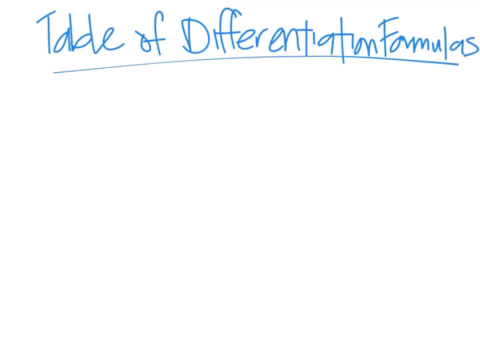 and, and, and, and, and, and, And. so we know we have a constant is just zero. So we have the derivative of a constant is just zero. We also have the derivative of x to some power n. 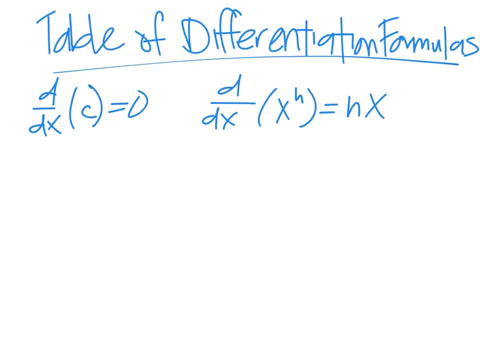 is just n times x to the power n minus one. You just subtract one f. the derivative of that is equal to c times the derivative of f. If we're adding two functions, we have f plus g in the derivative. this is the derivative. 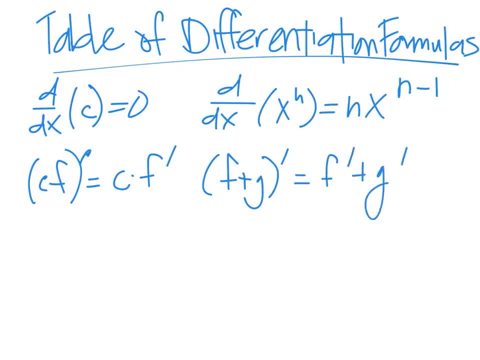 of f plus the derivative of g. If we are subtracting two functions, f minus g, that's going to be f, derivative of f minus derivative of g, and then we have the product. if we have f times g, that's just f times. 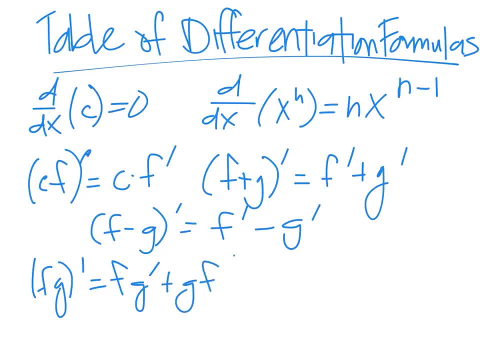 the derivative of g plus g times the derivative of f and finally the quotient. if we have f divided by g, the derivative of that whole thing is g times the derivative of f minus f times the derivative of g. So we have the derivative of g divided by g squared. 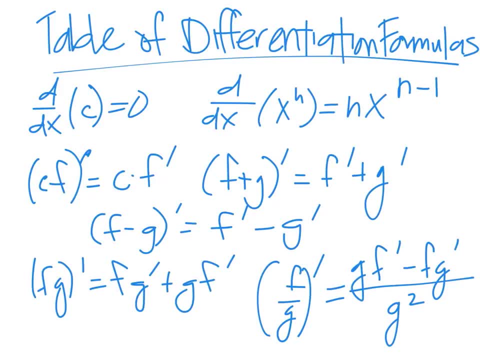 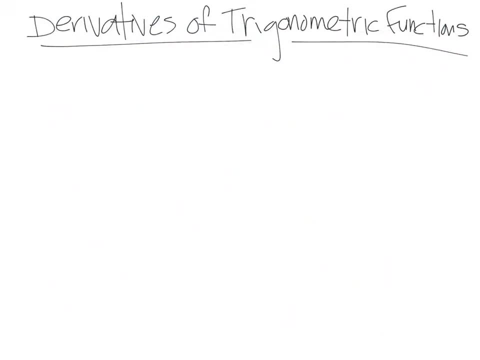 These are all very important formulas that you'll need in order to calculate derivatives. In this section we're going to talk about the derivatives of trigonometric functions, So recall what the graph of sine of x looks like. and sine of x starts at zero. it goes: 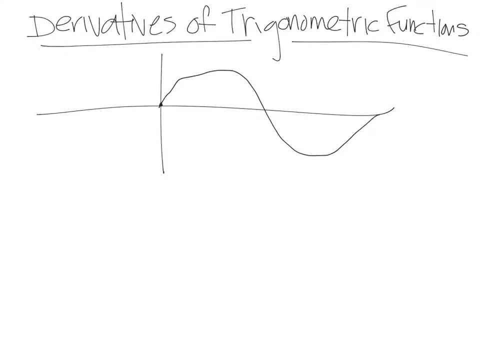 up, Comes back down, goes back up and repeats And same thing with this, And it has a period of 2pi halfway of. that would be pi. and then we fill out in the middle of all of these. this would be 3pi over 2, this would be pi over 2, and then negative. 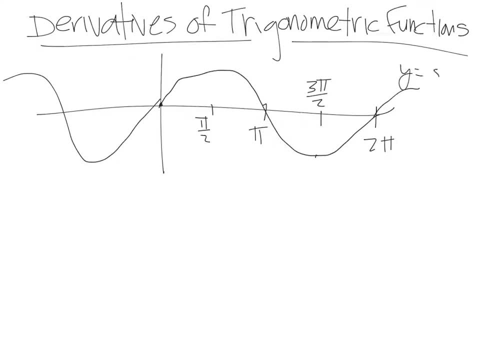 as well. So this is the graph of y equals sine of x, Subtitles by the Amaraorg community. Or let's call this: f of x is y equals sine of x. Now what would the graph of the derivative look like? 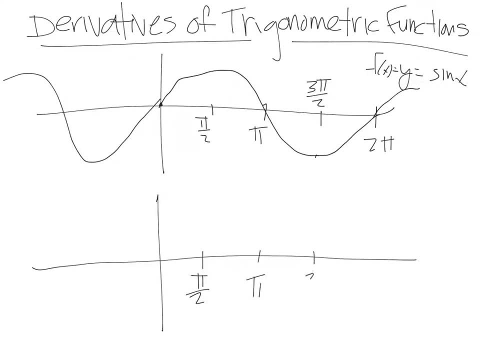 So, bringing all these down, we have pi, we have 3pi over 2, and 2pi. So the graph of y equals the derivative f prime of x. well, when we start by graphing the derivatives, we want to look at the maximums and minimums, because that means the slope. 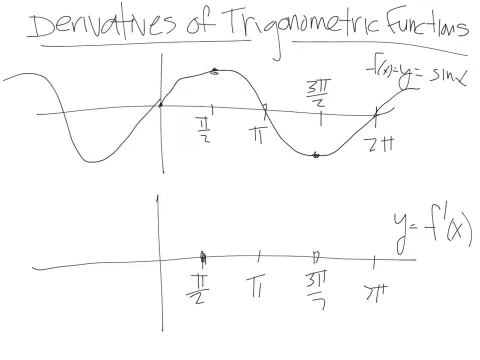 is zero and so it crosses right here on the axis. Now, looking over here, we have a positive slope, it's increasing, so it's positive, so we're going to be, it's going to be with a high positive value and it gets lower and 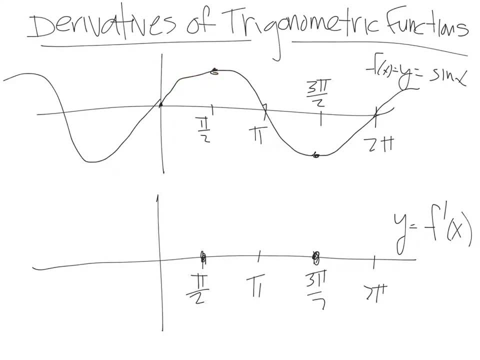 lower until we hit zero. So we have a high positive number and it gets smaller and smaller until you hit zero. So we're going to be- it's going to be- with a high positive value and it gets lower and lower until we hit zero. 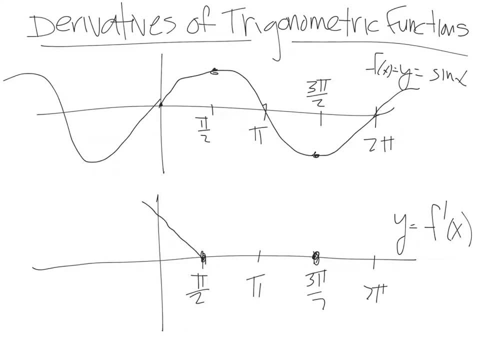 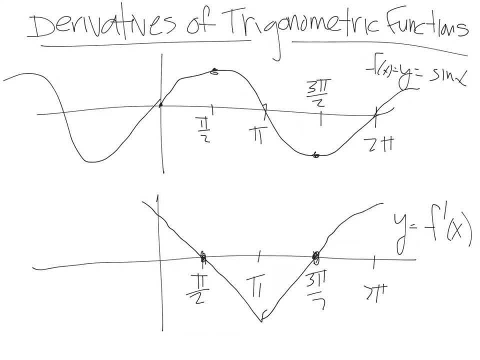 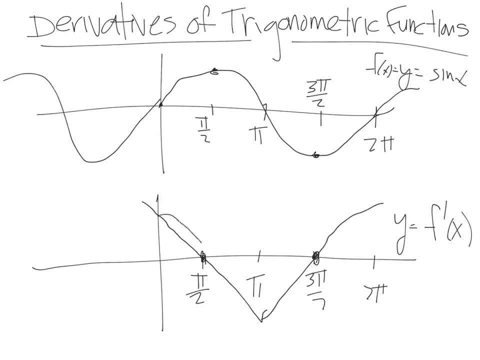 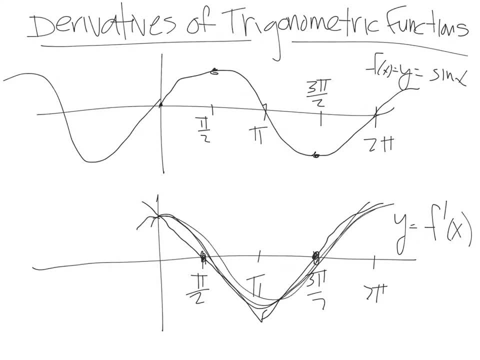 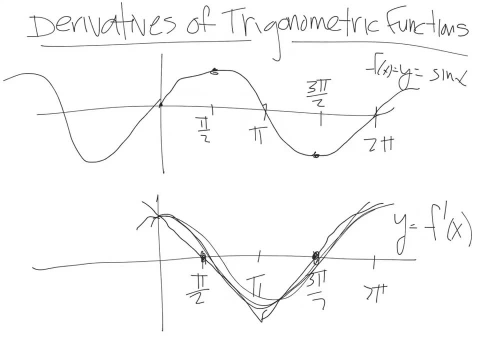 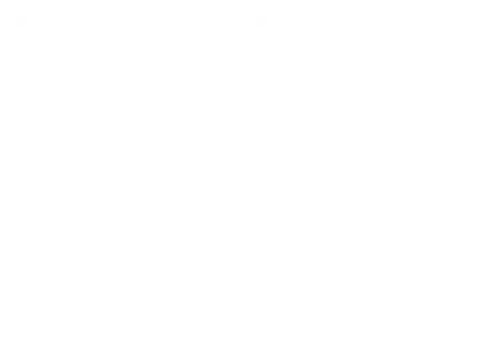 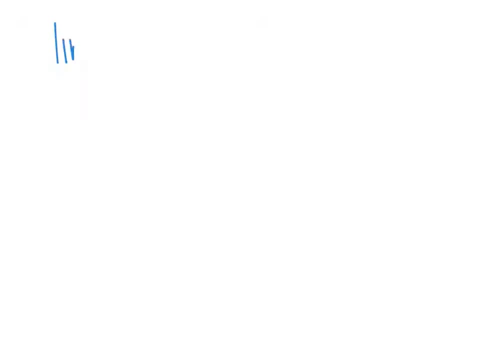 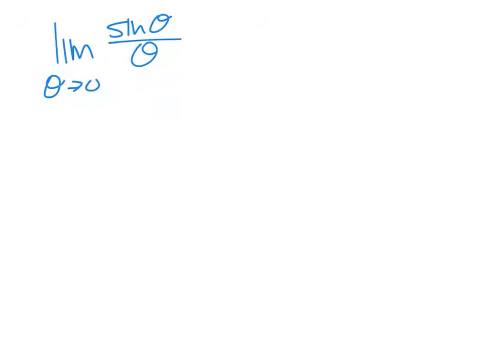 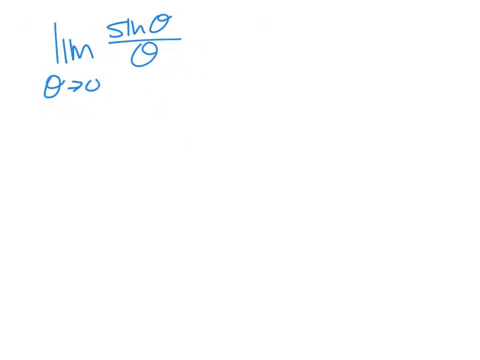 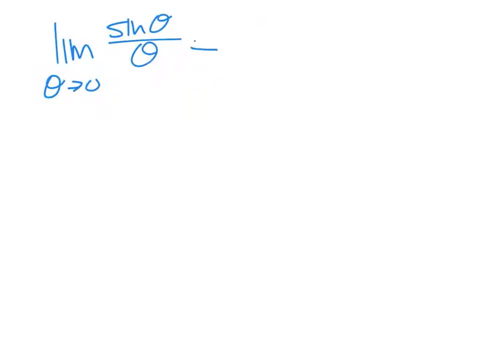 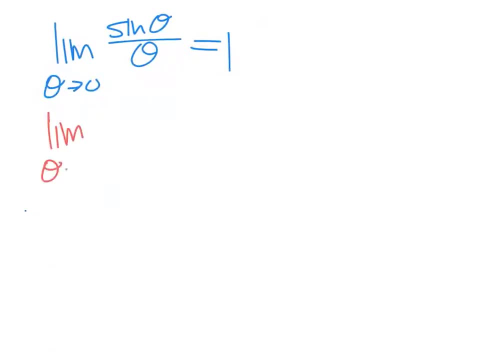 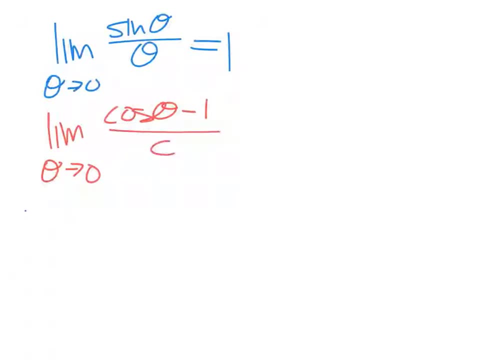 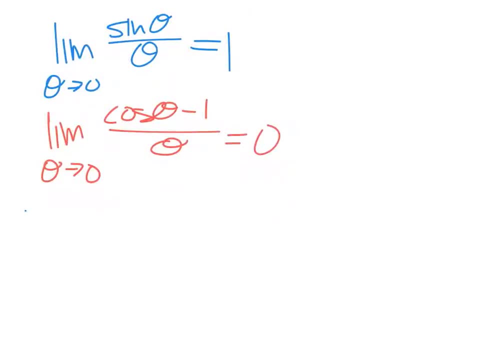 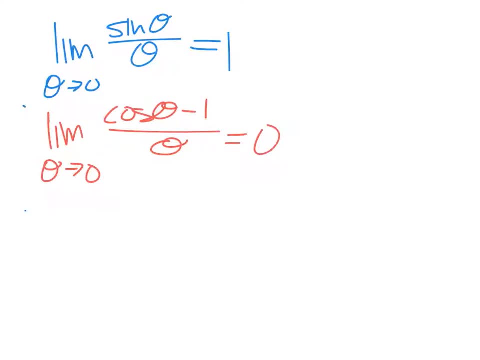 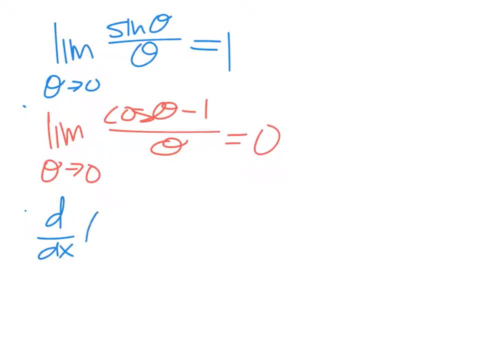 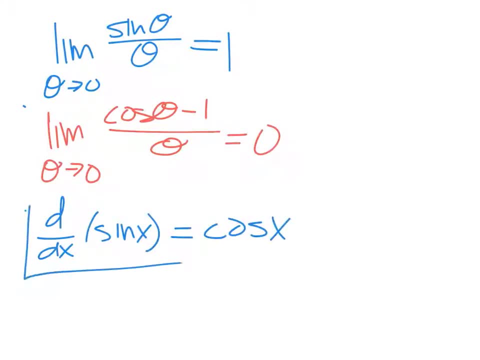 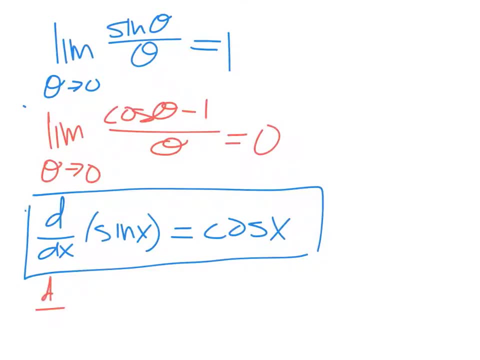 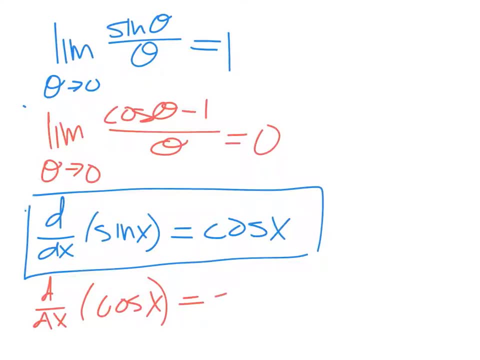 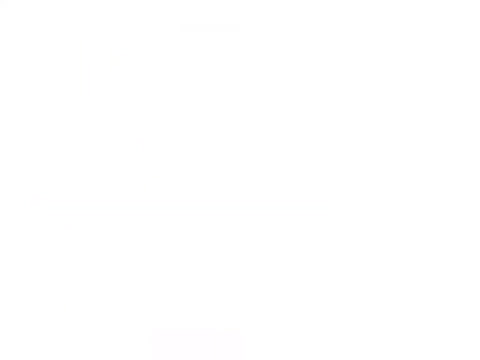 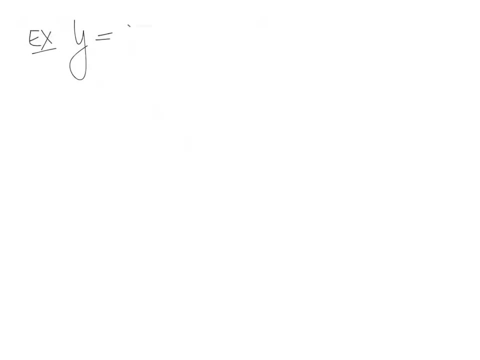 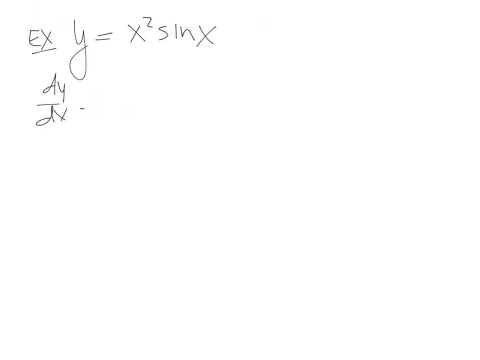 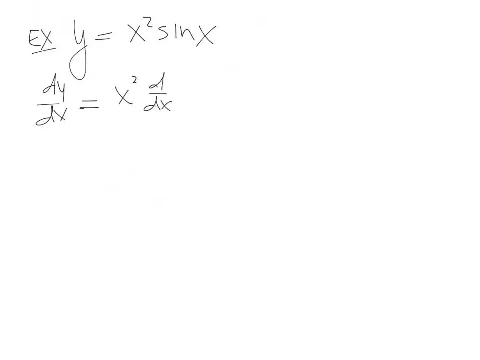 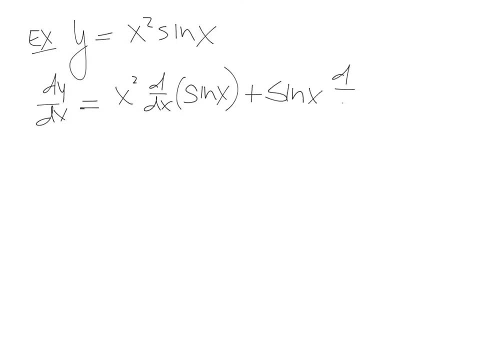 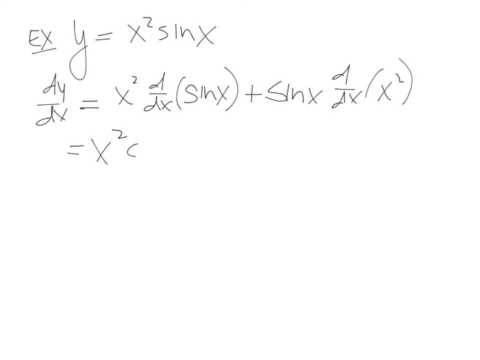 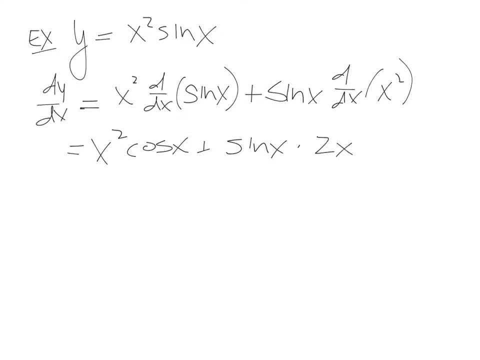 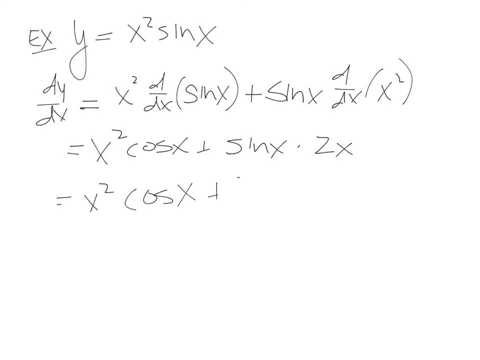 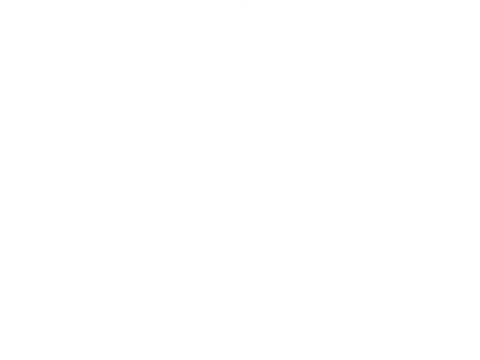 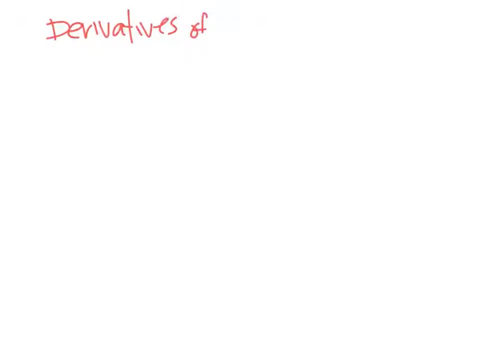 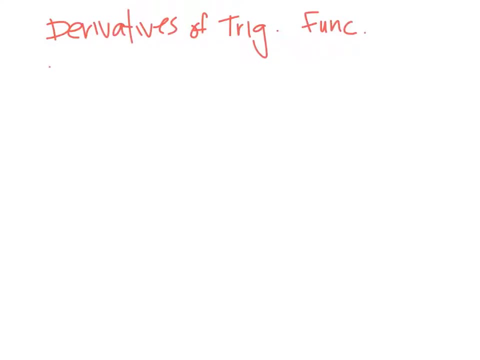 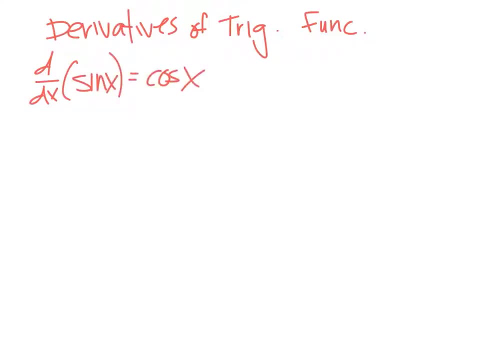 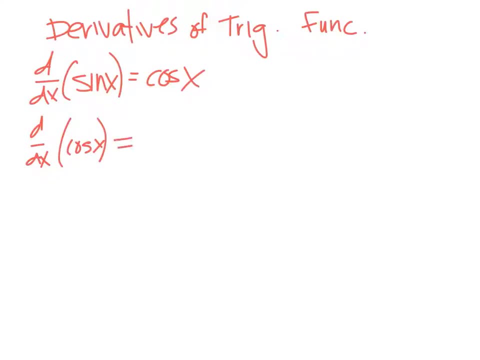 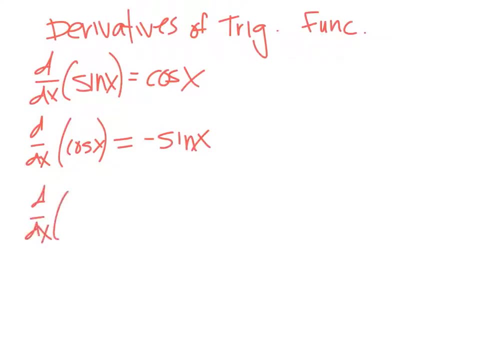 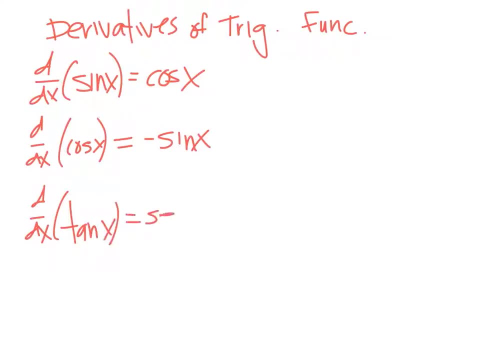 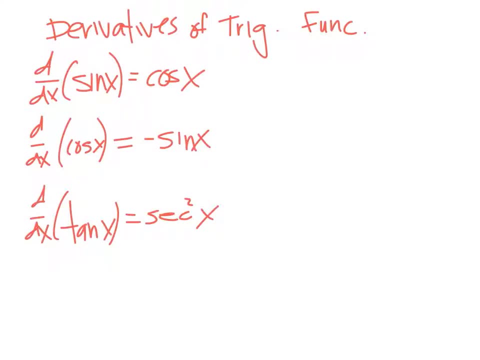 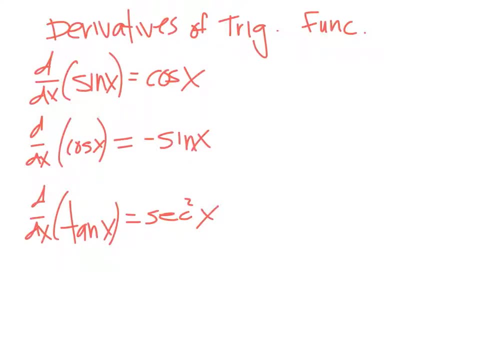 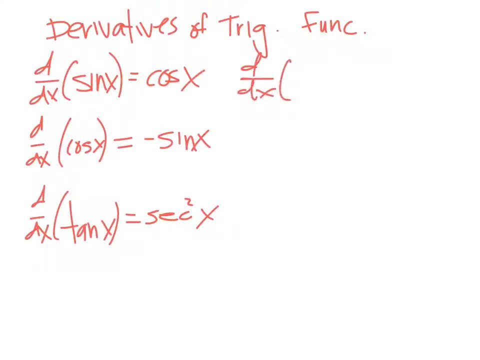 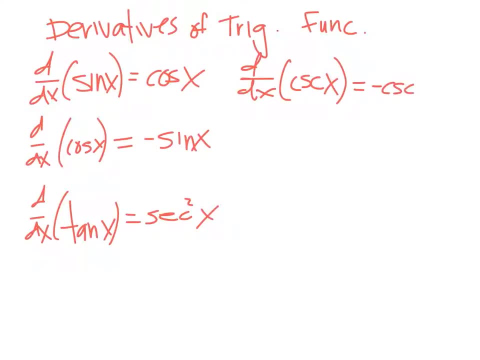 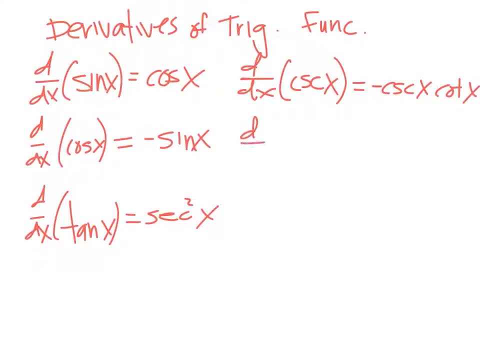 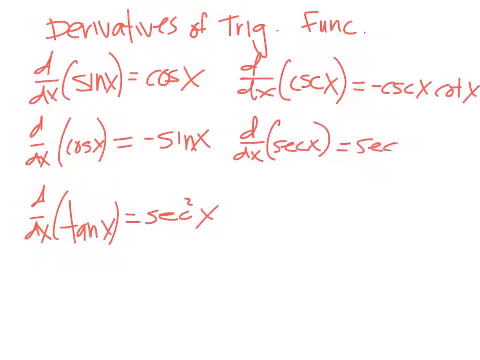 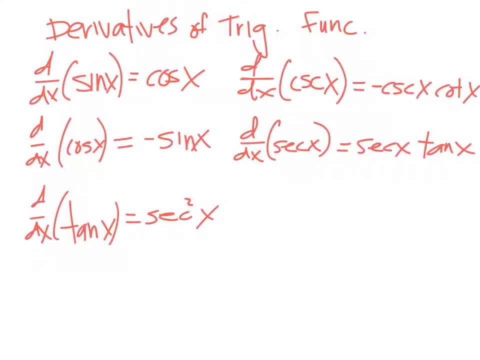 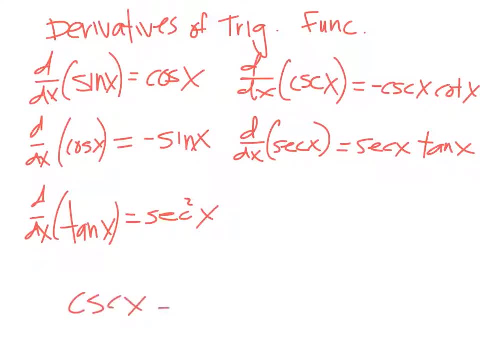 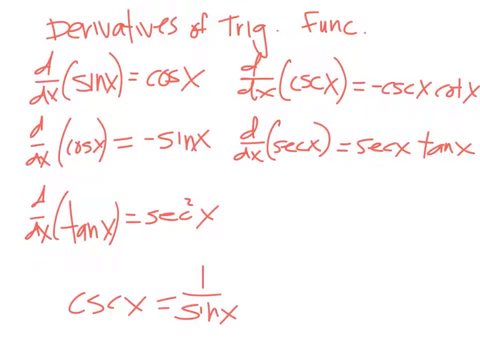 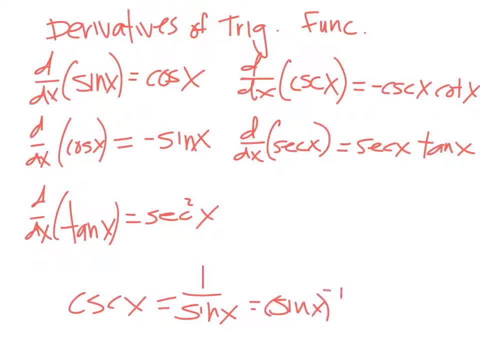 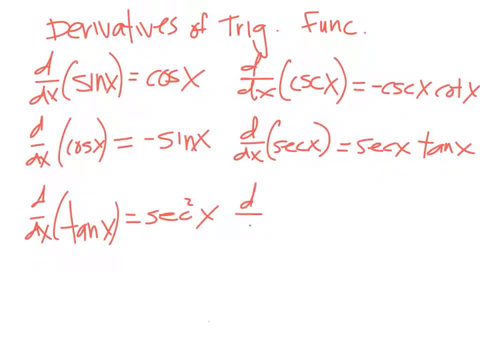 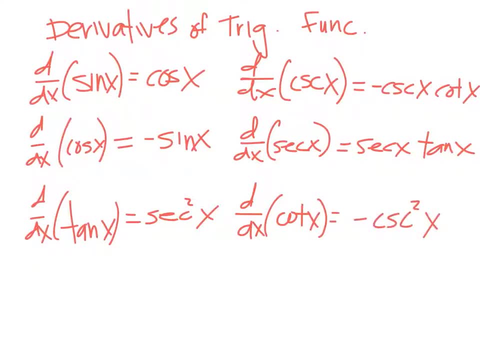 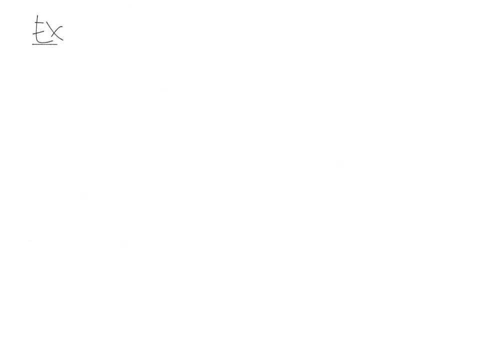 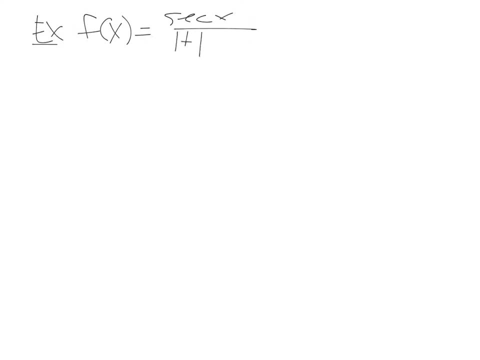 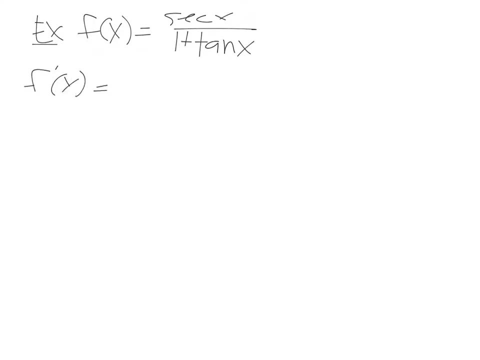 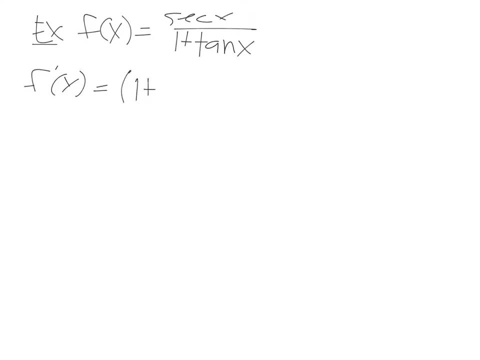 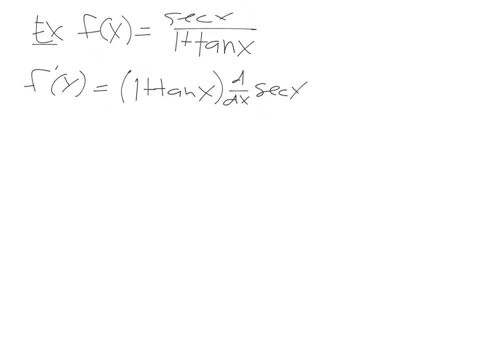 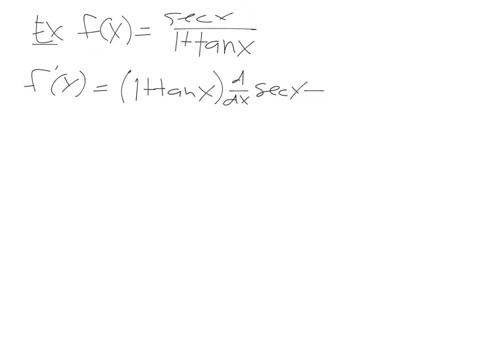 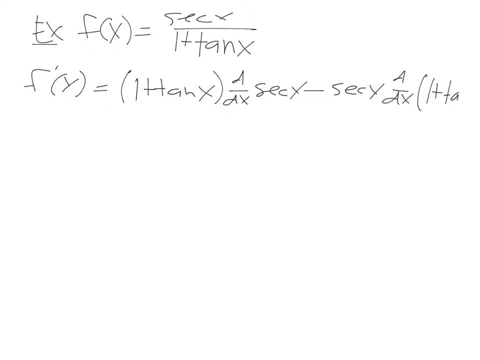 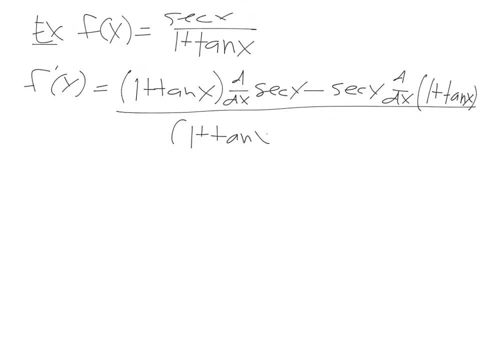 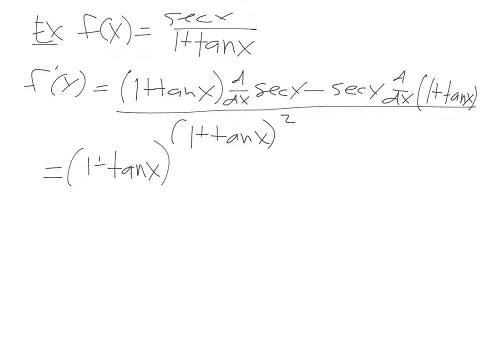 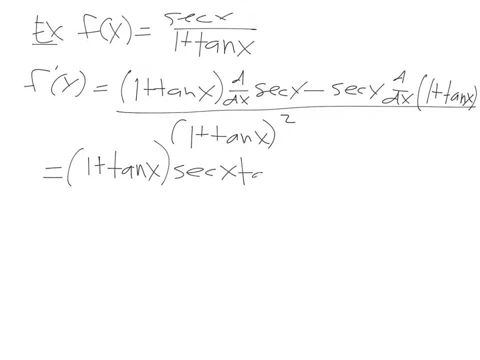 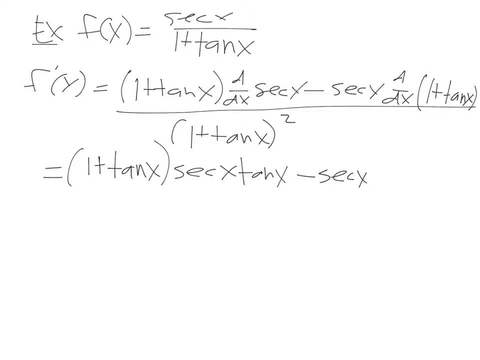 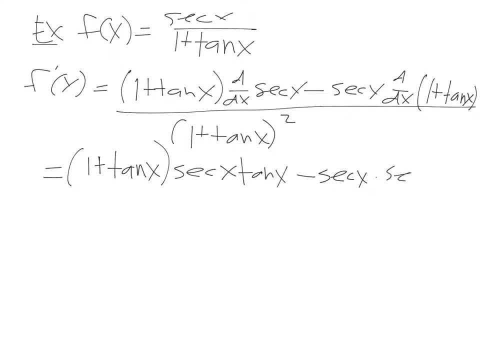 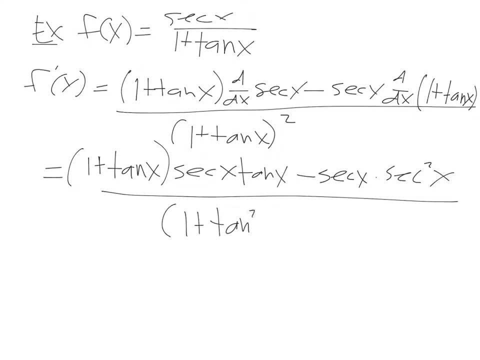 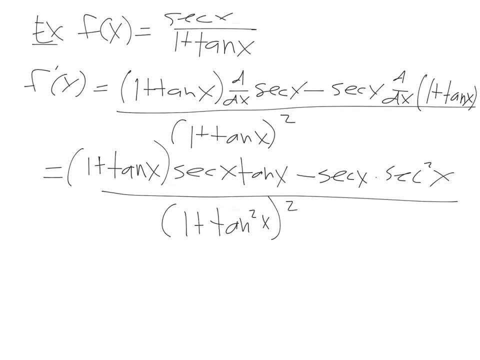 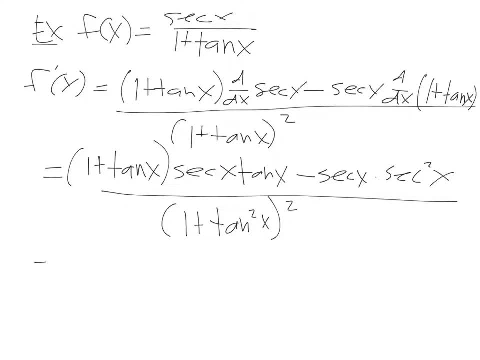 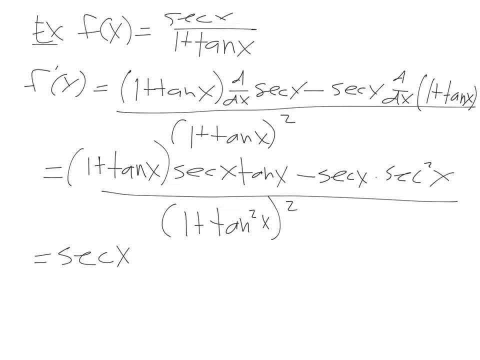 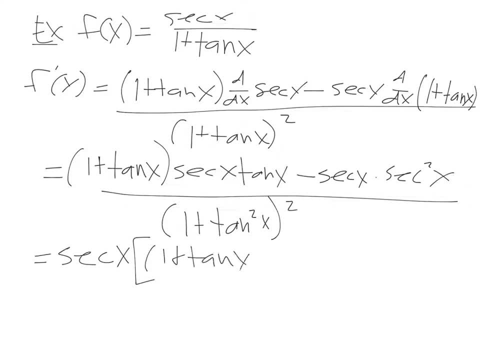 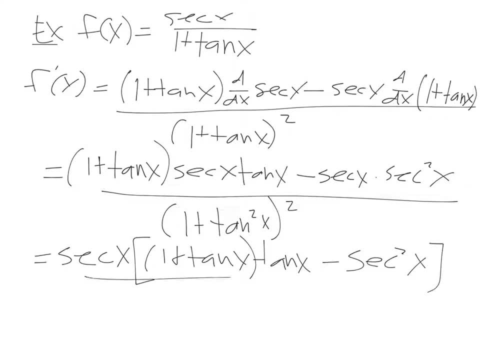 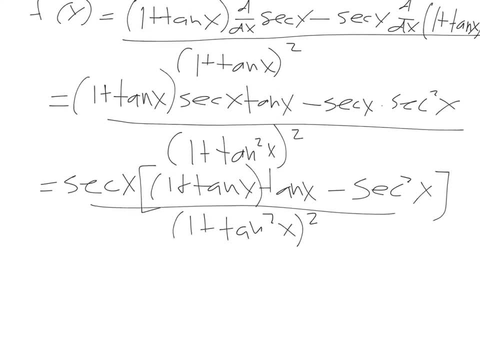 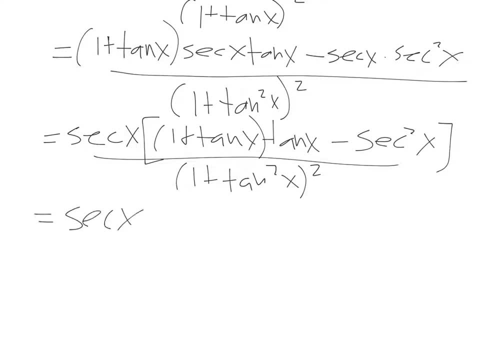 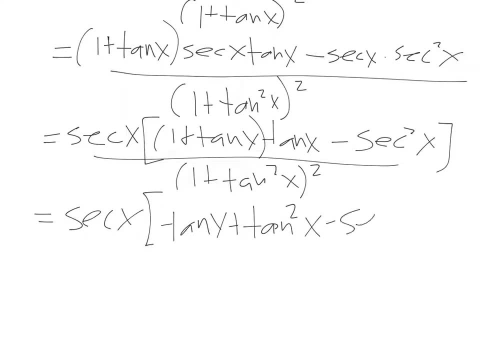 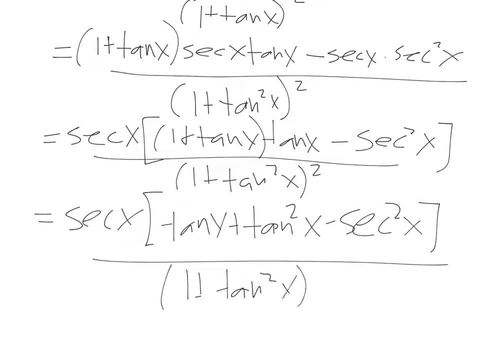 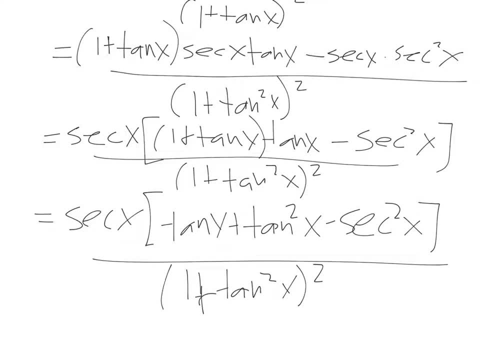 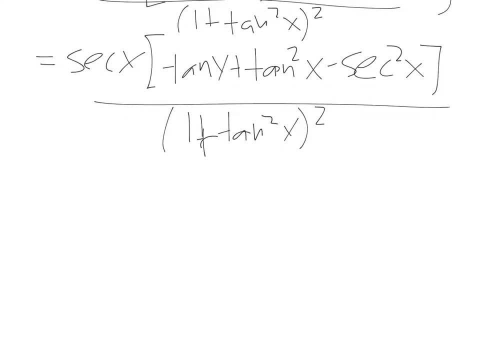 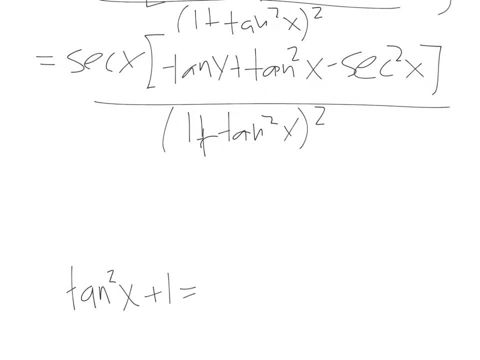 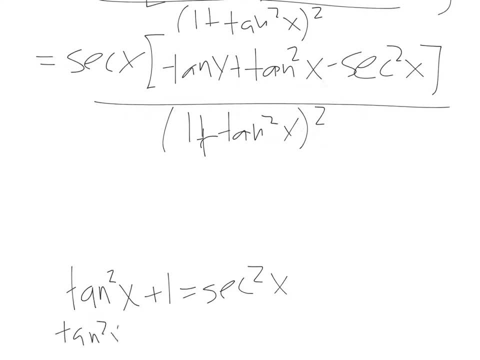 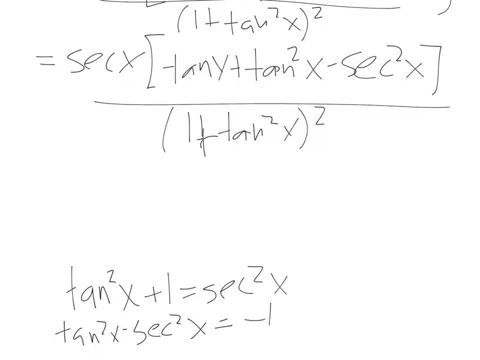 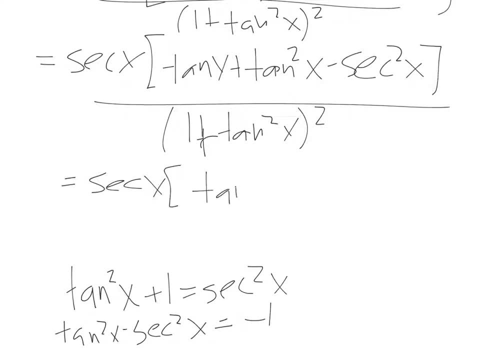 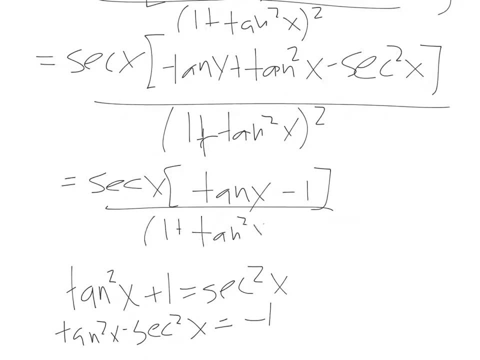 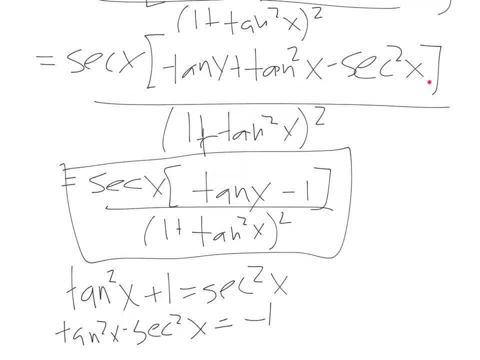 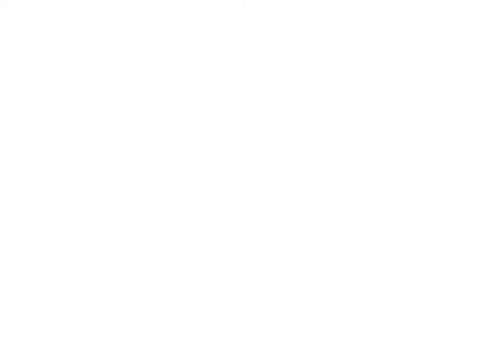 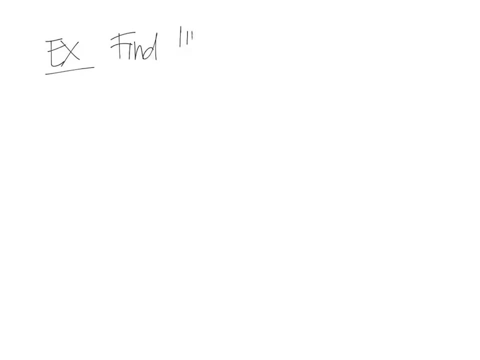 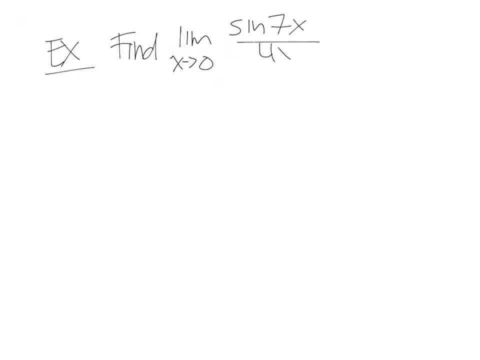 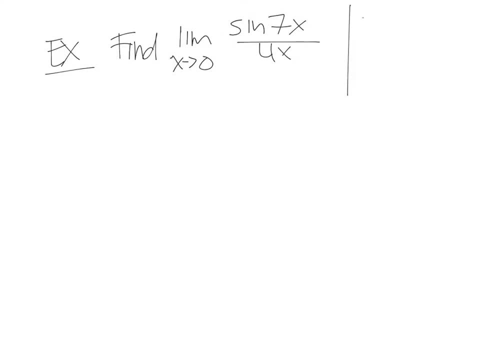 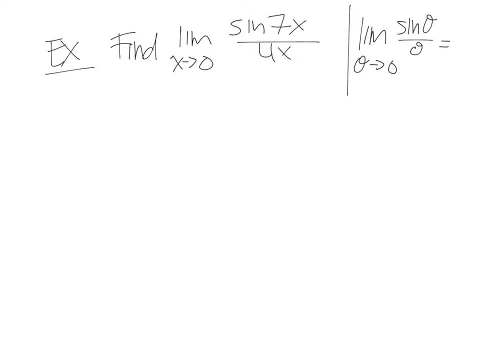 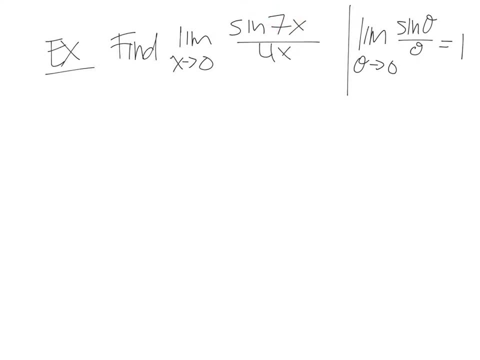 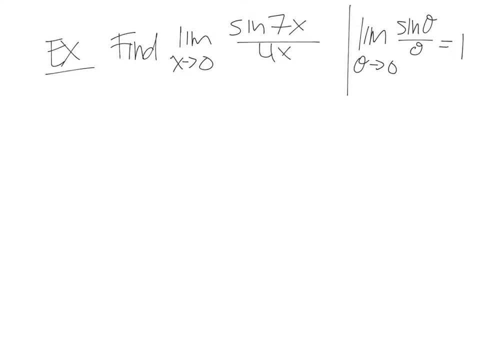 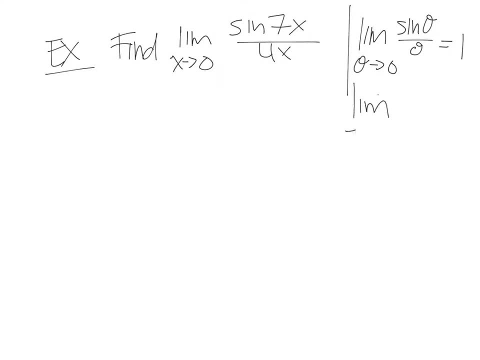 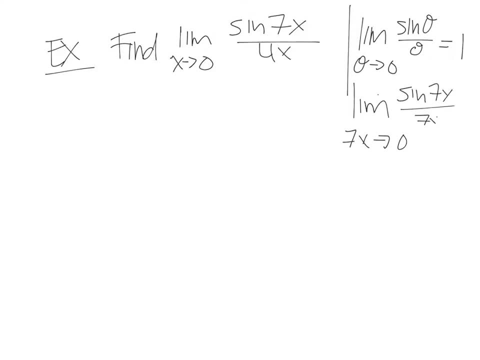 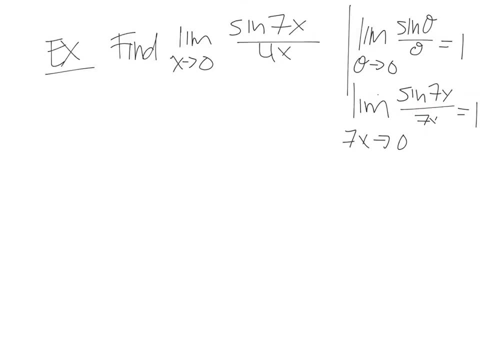 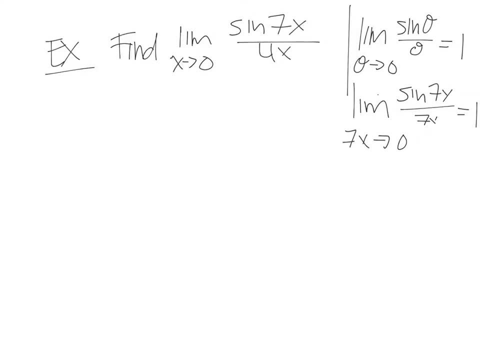 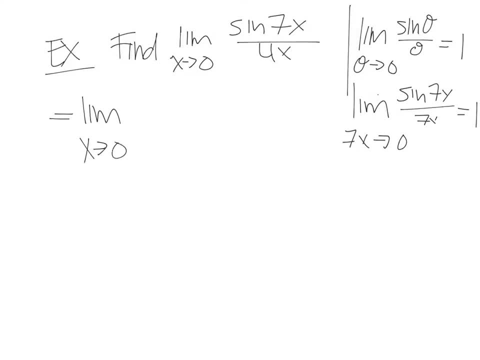 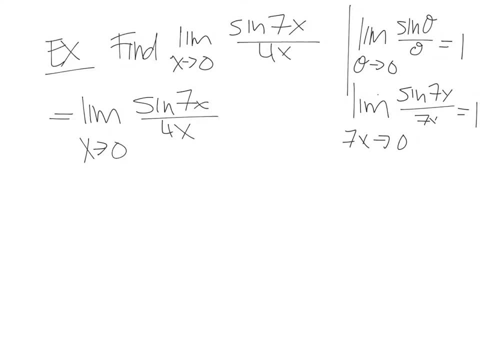 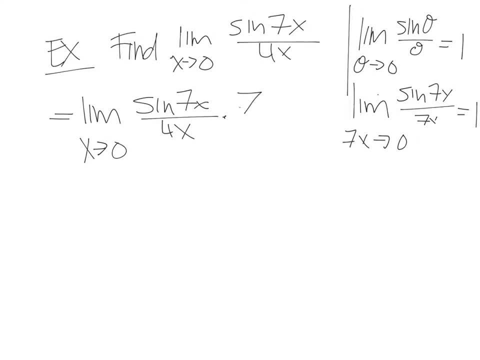 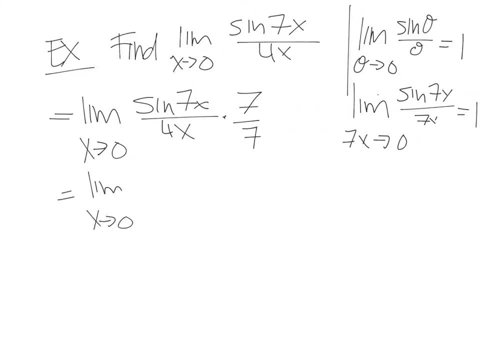 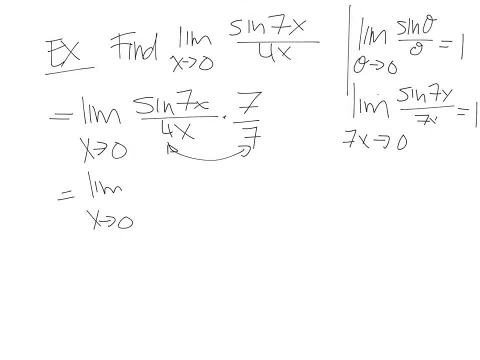 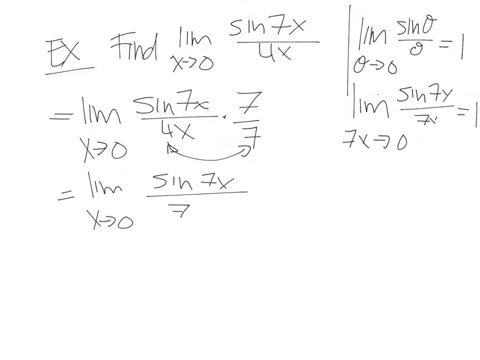 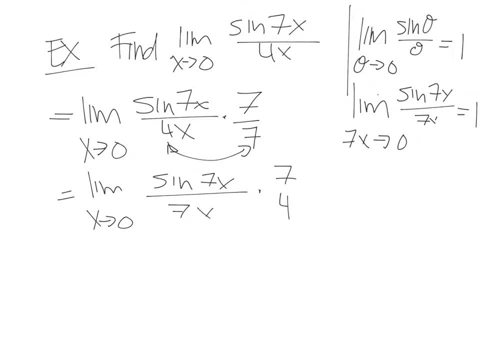 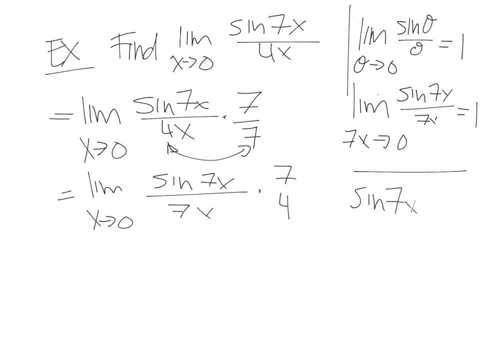 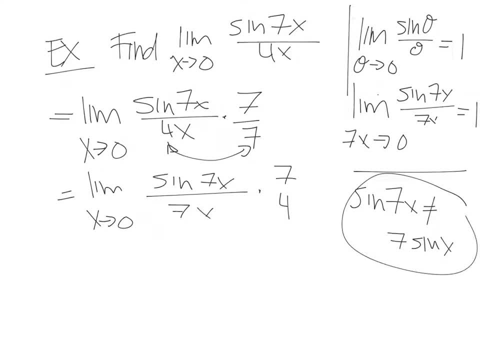 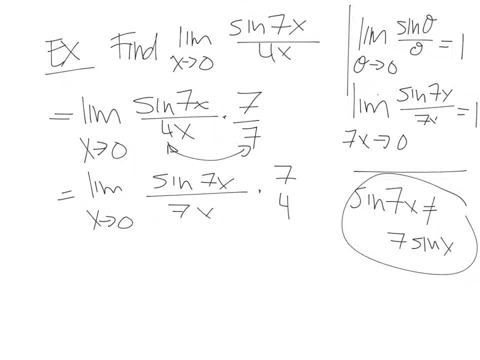 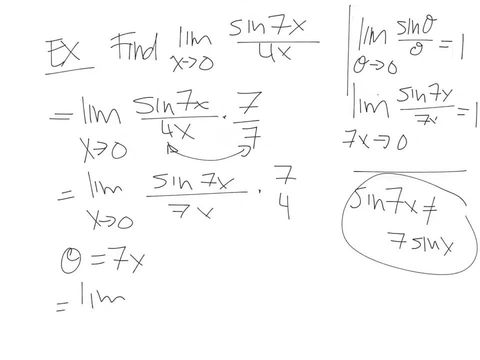 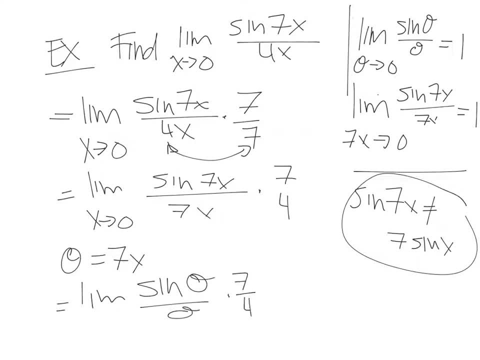 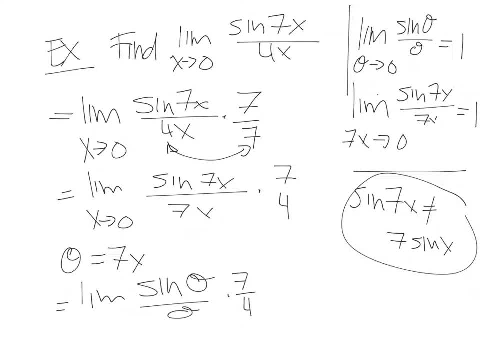 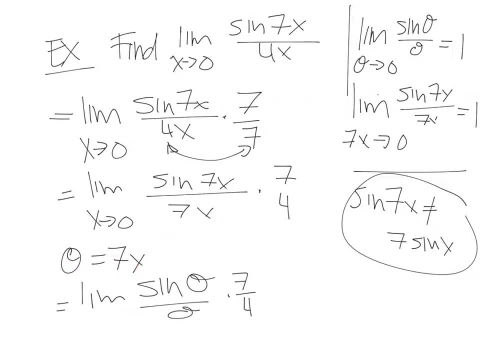 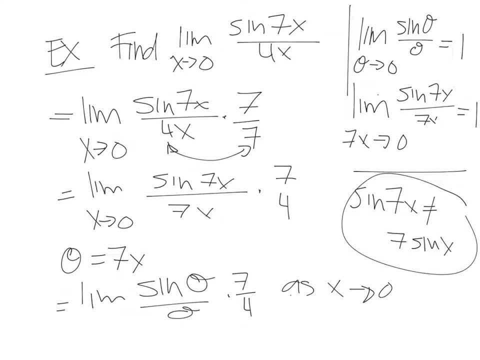 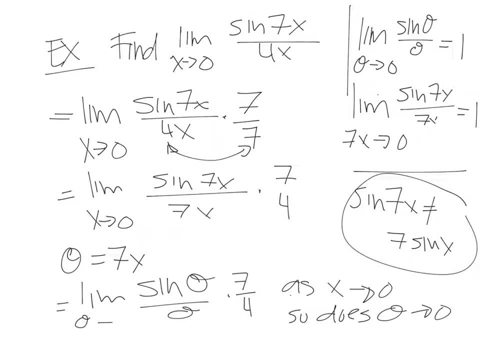 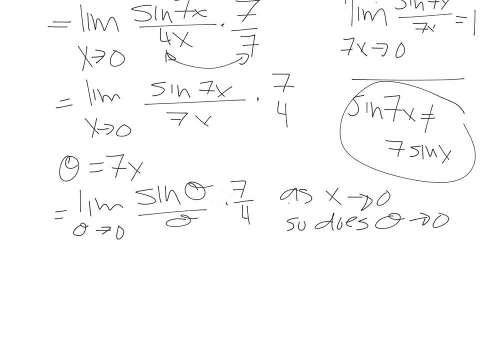 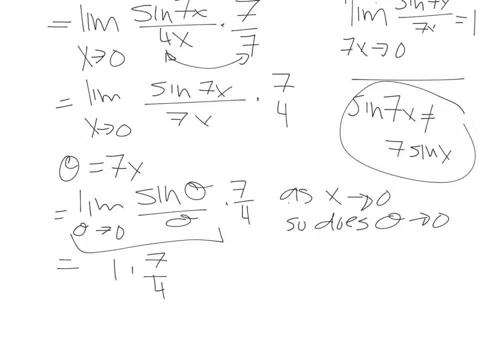 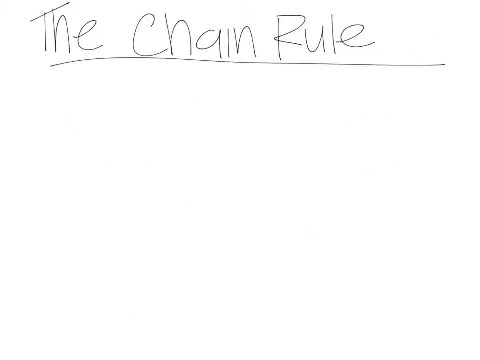 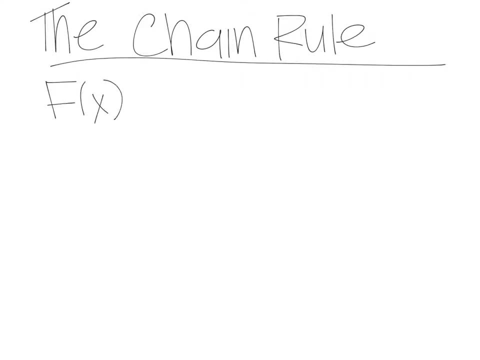 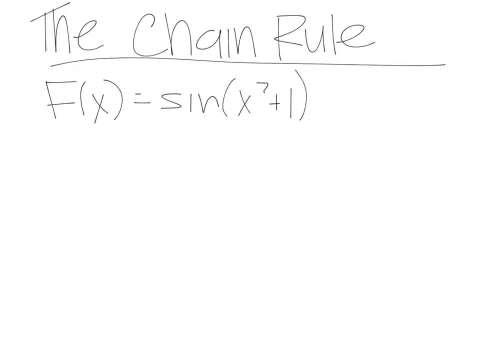 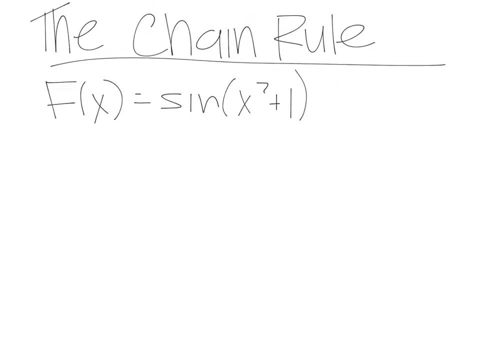 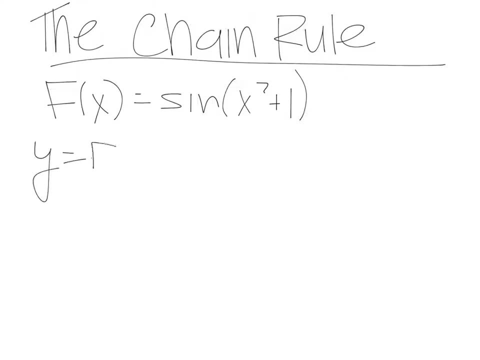 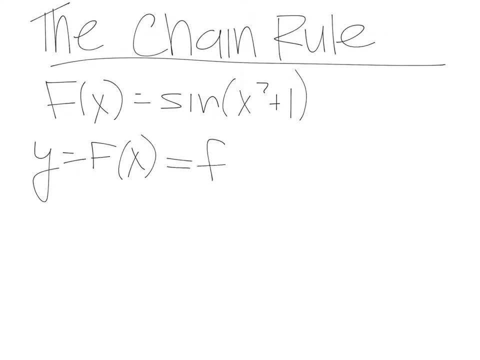 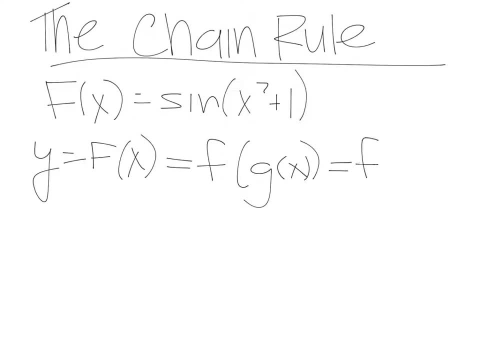 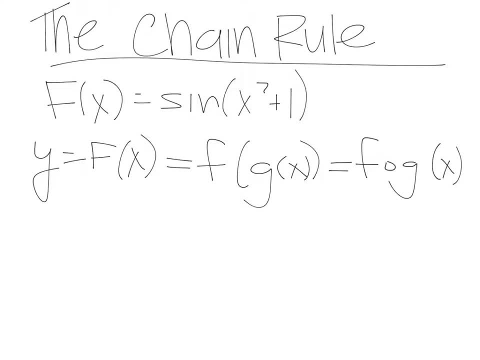 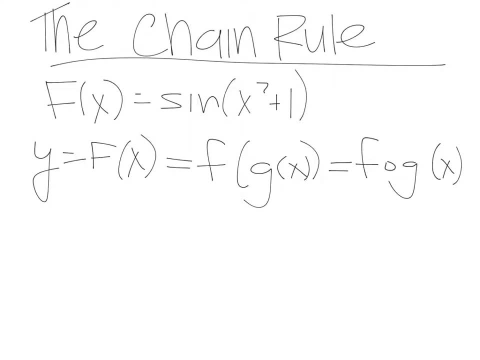 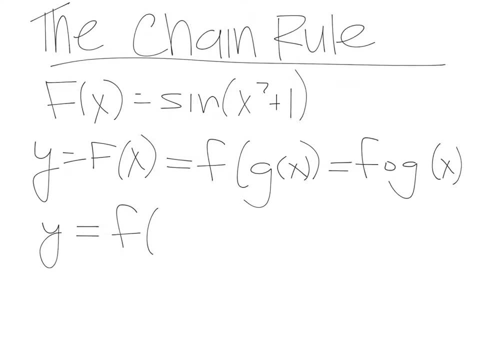 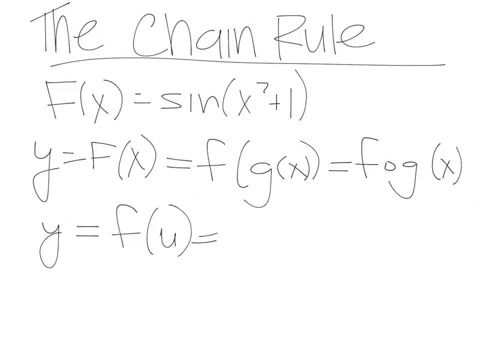 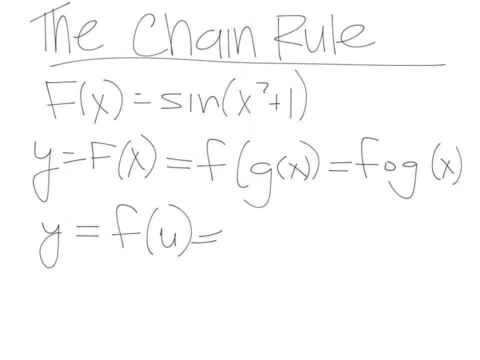 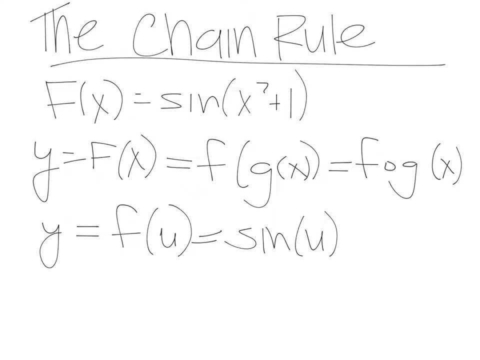 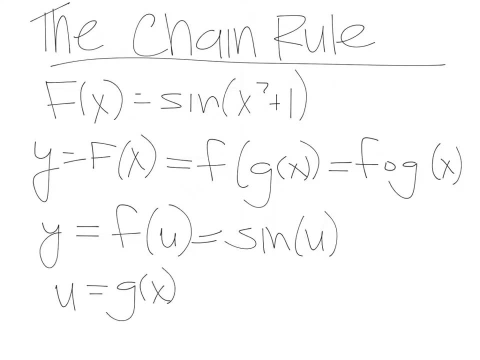 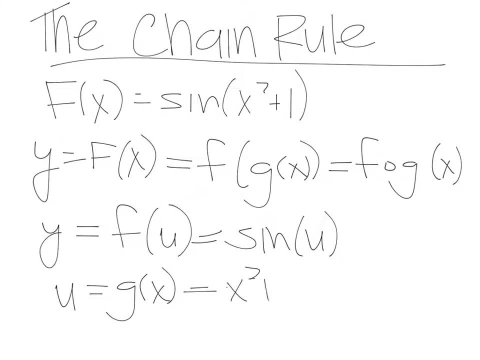 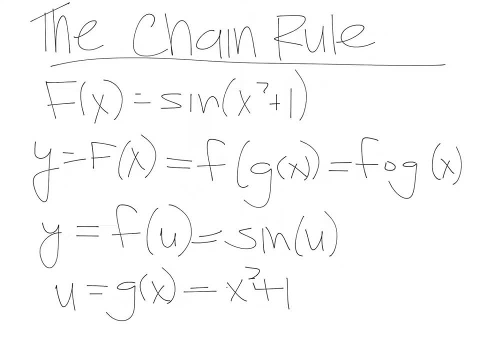 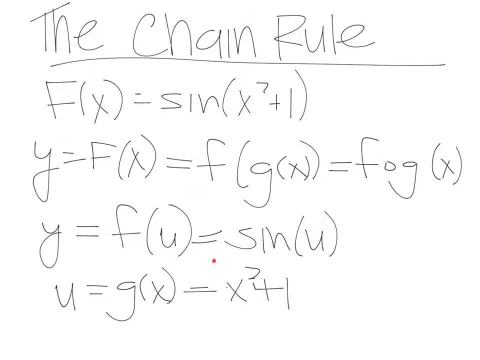 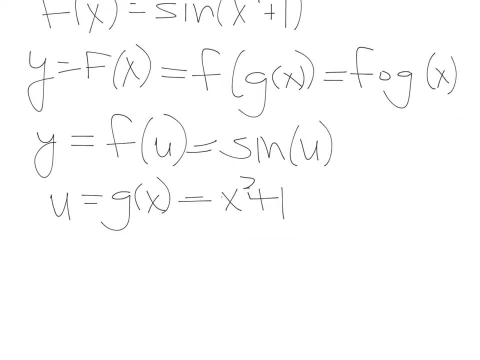 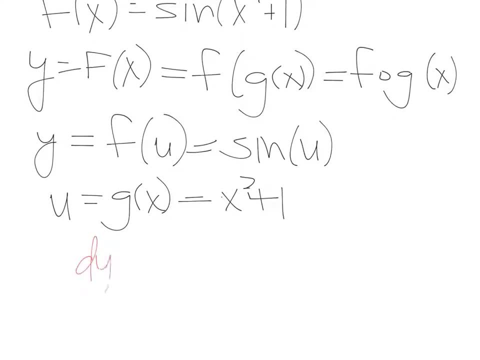 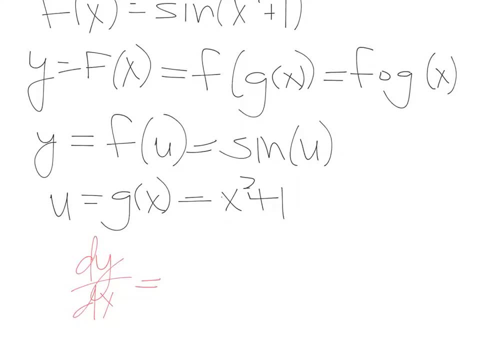 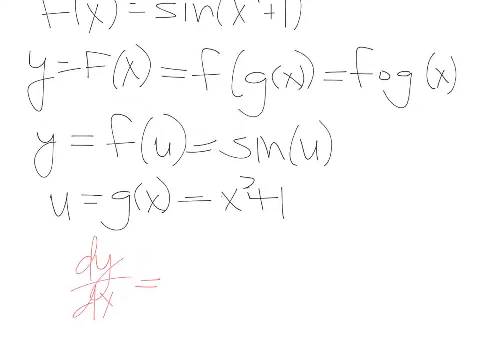 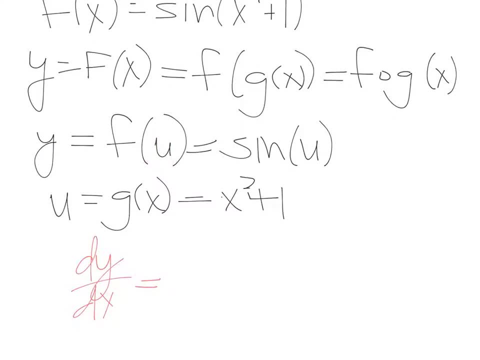 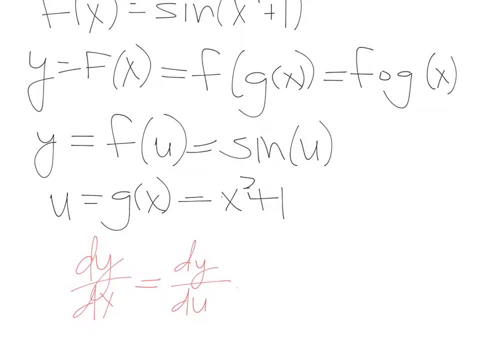 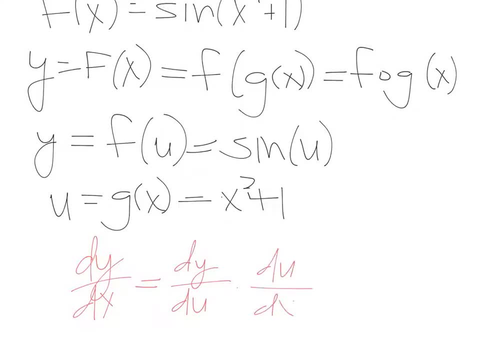 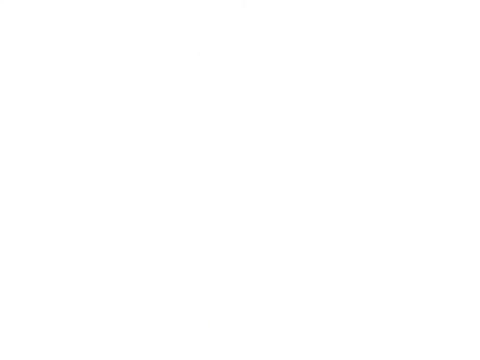 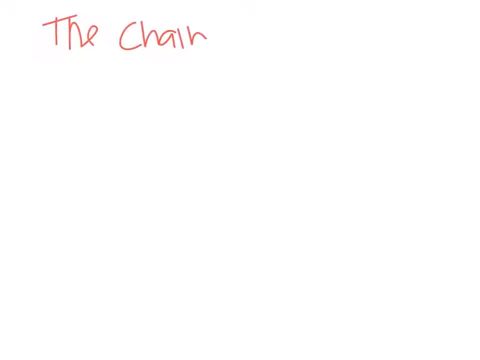 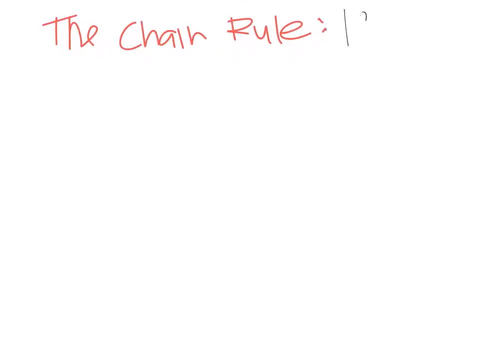 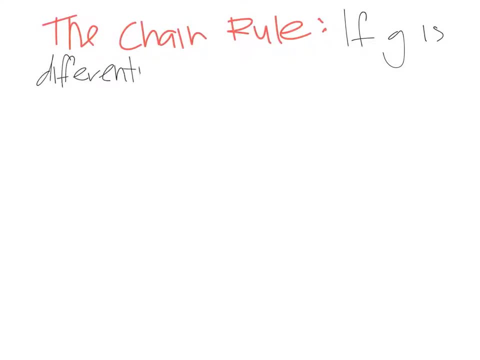 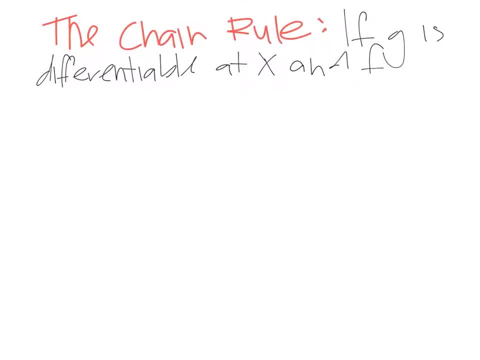 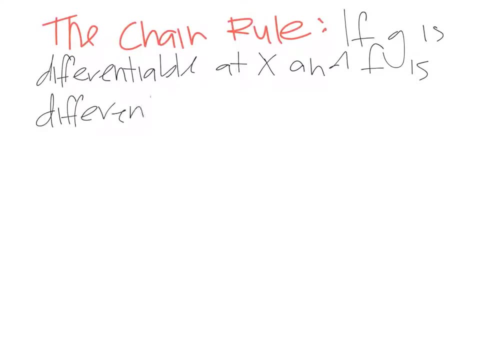 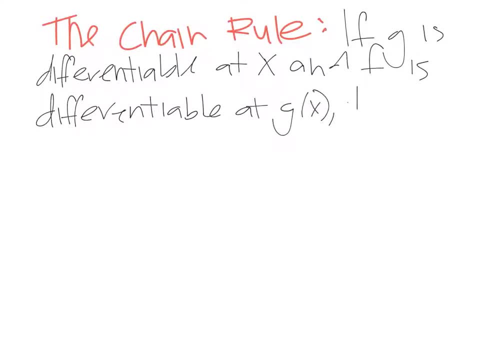 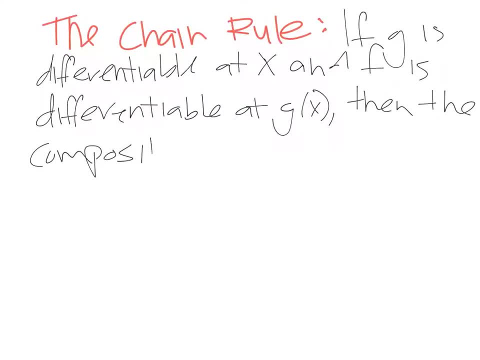 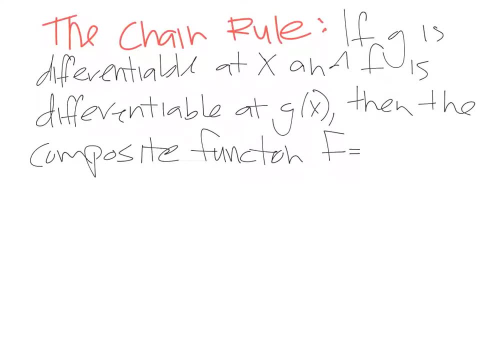 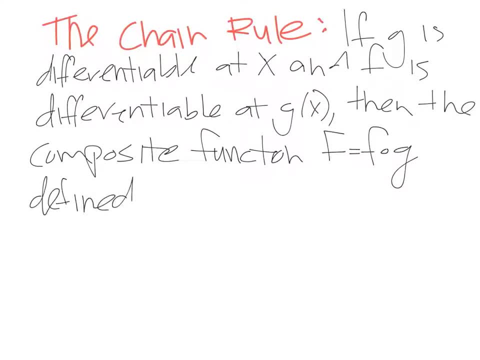 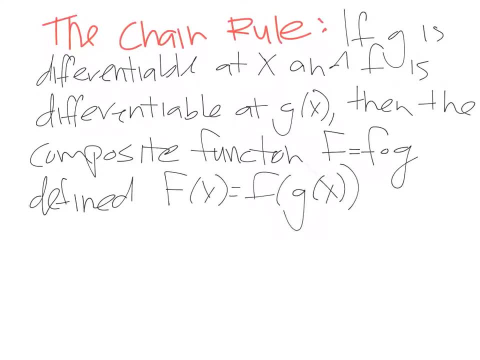 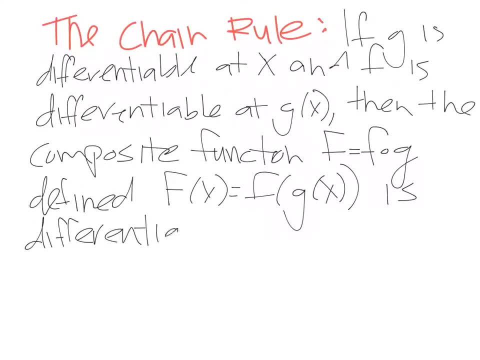 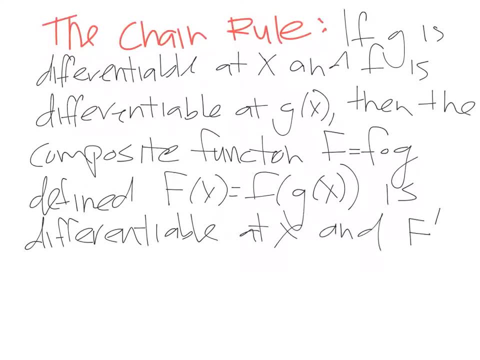 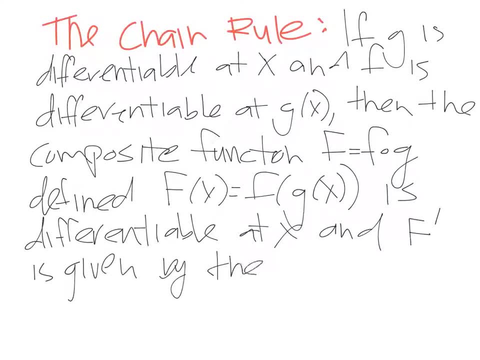 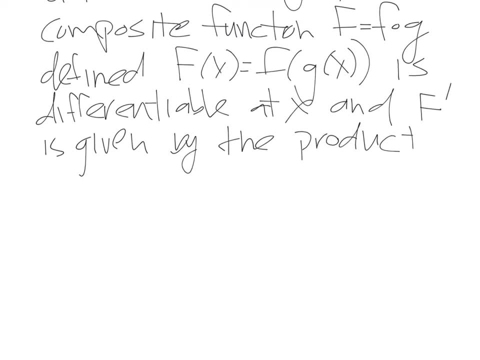 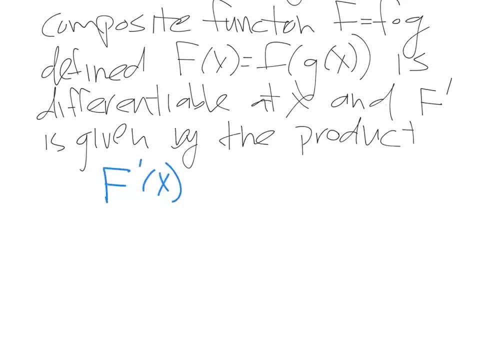 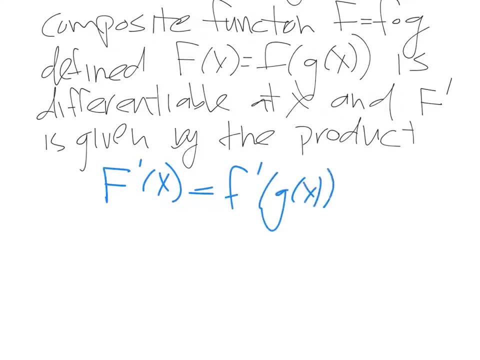 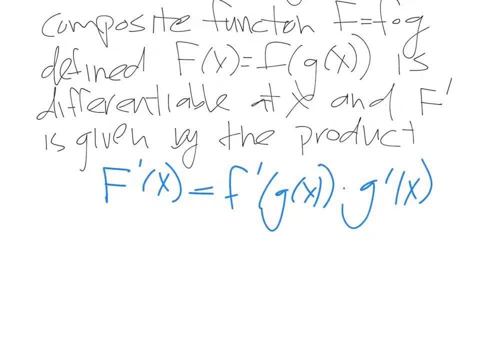 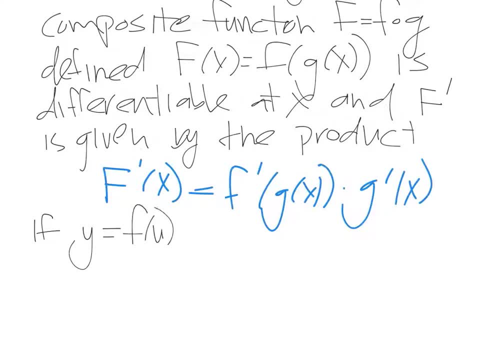 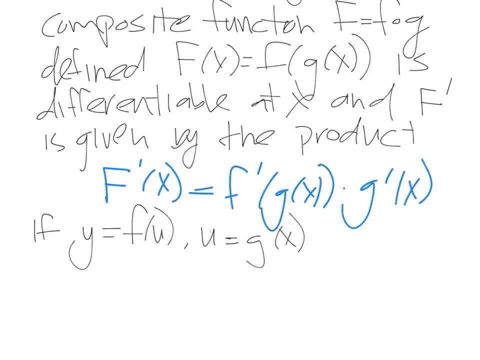 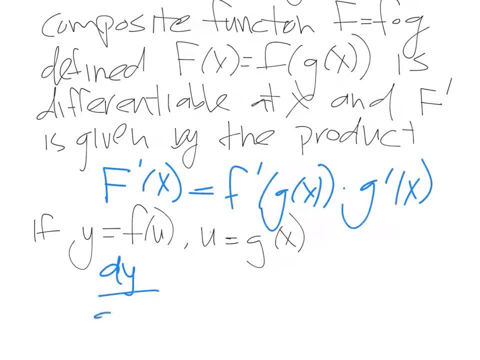 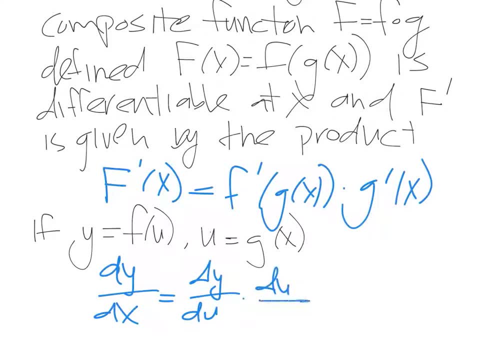 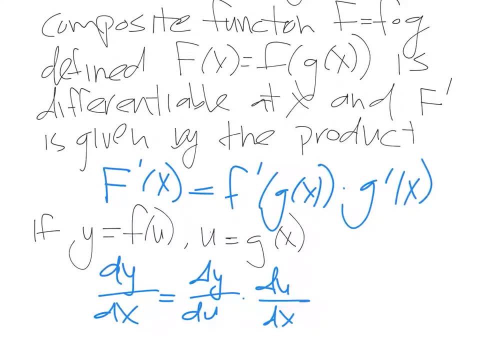 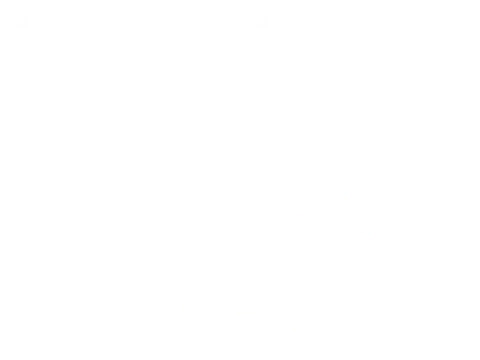 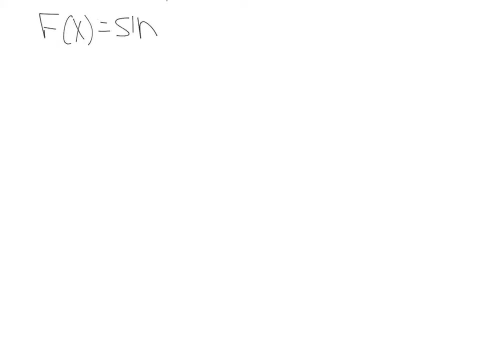 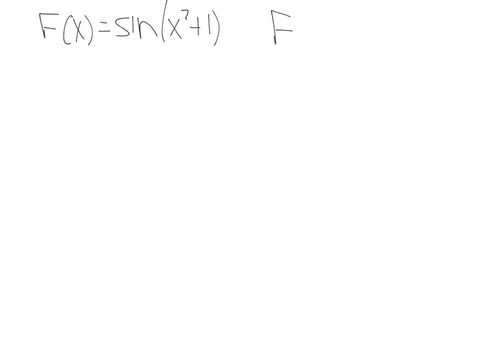 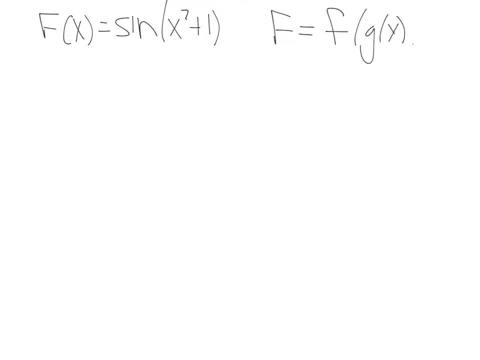 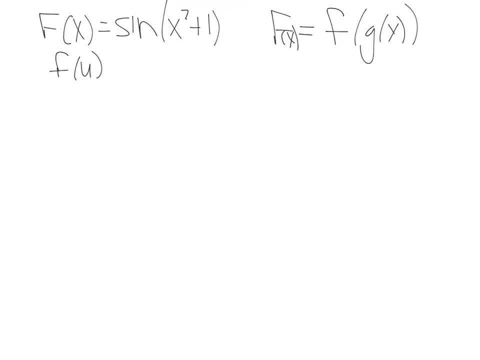 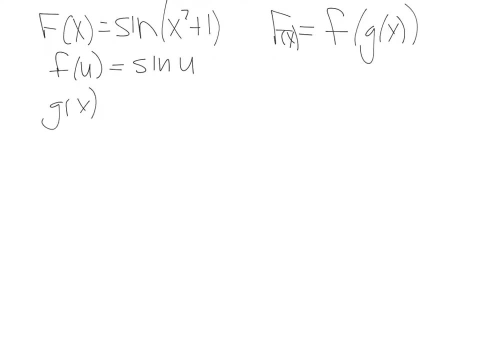 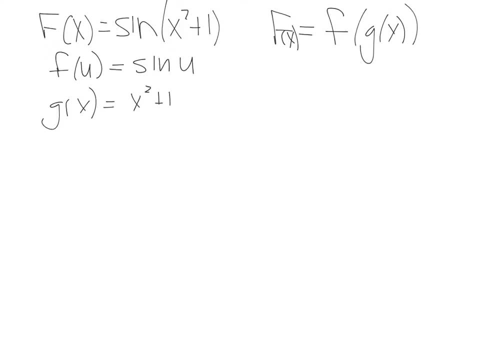 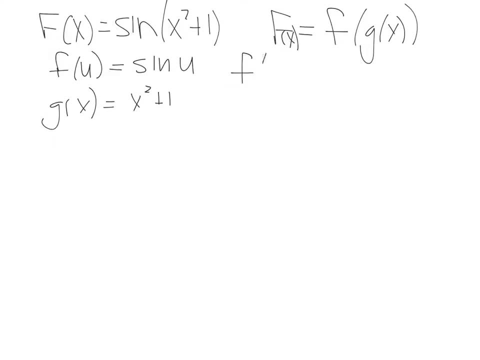 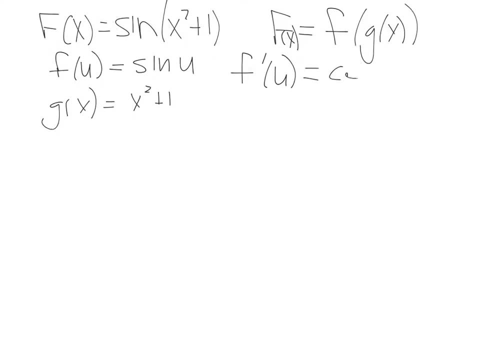 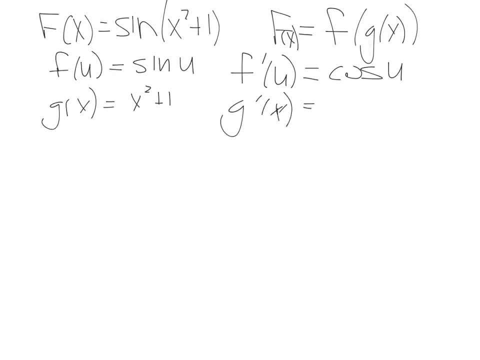 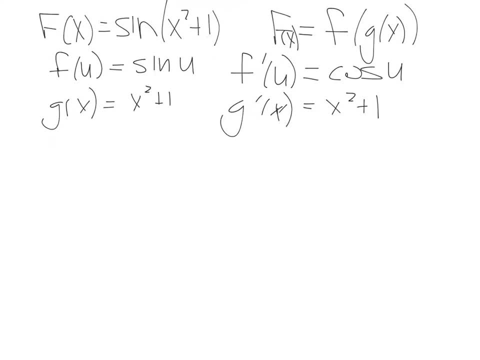 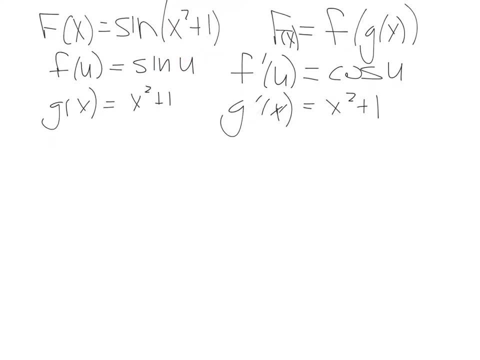 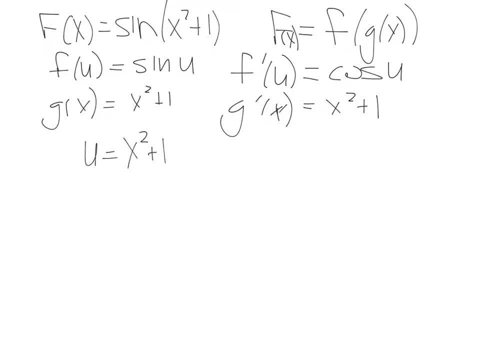 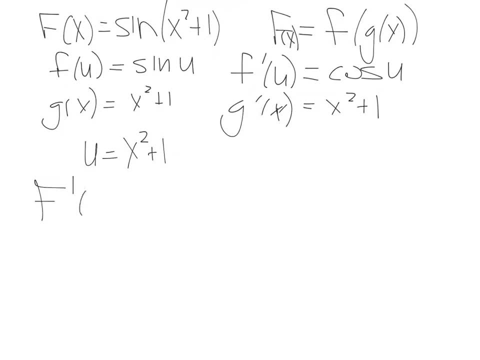 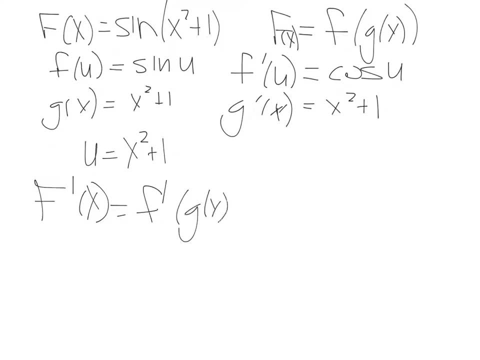 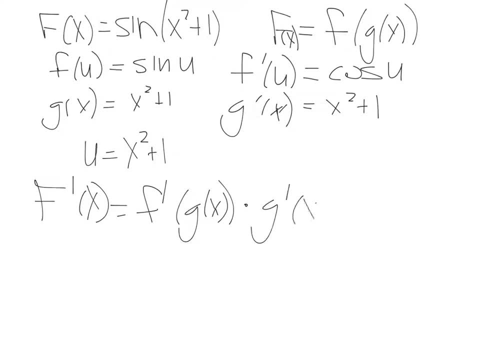 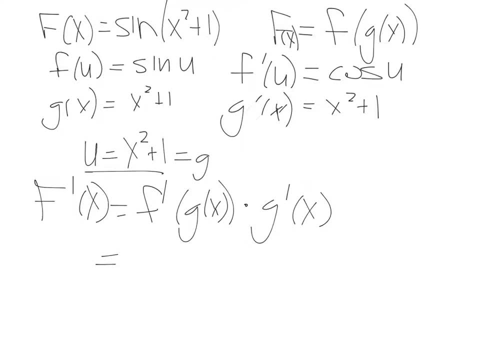 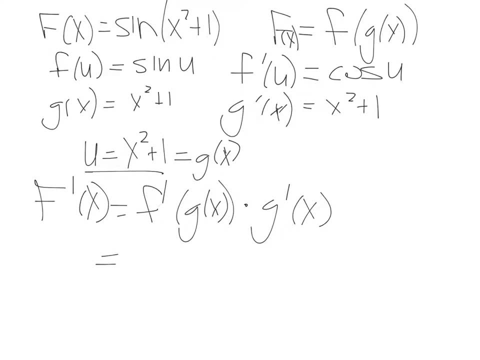 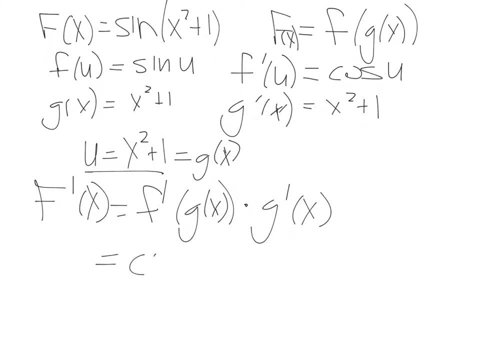 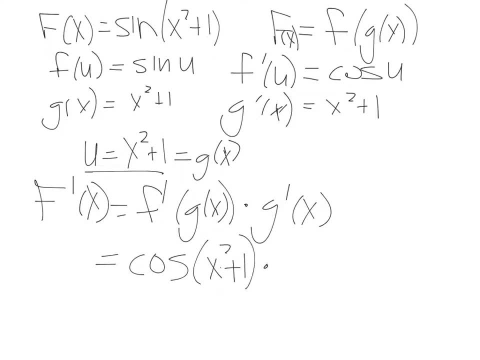 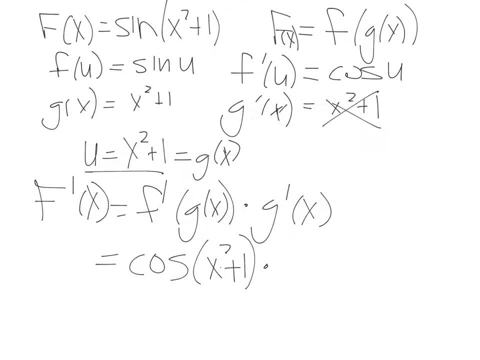 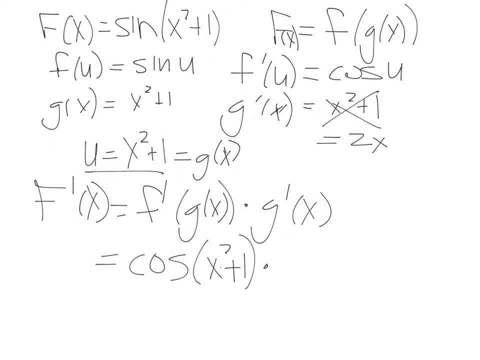 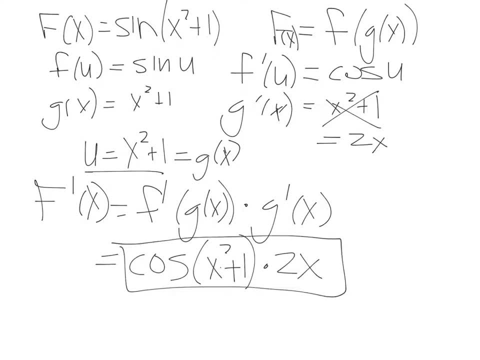 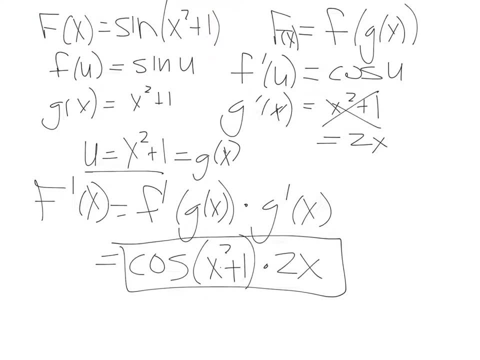 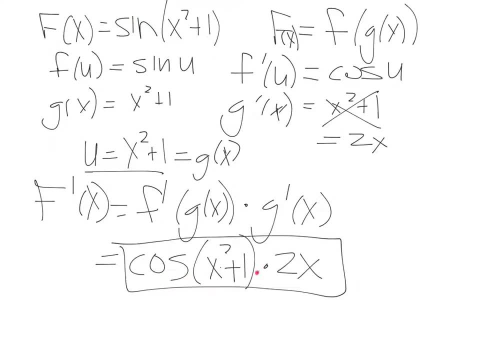 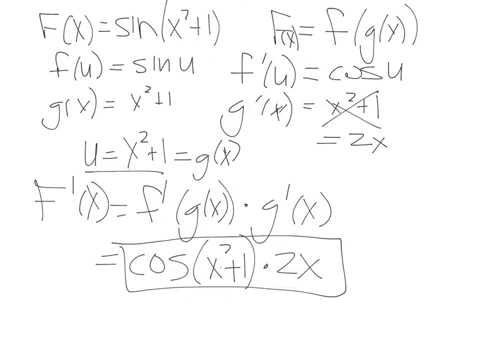 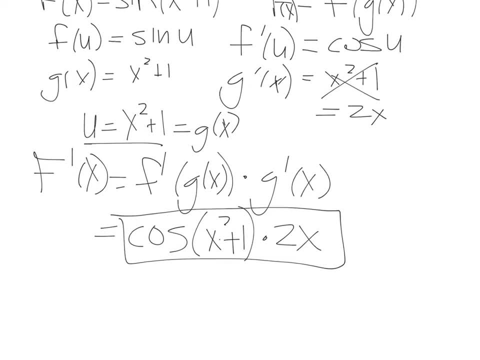 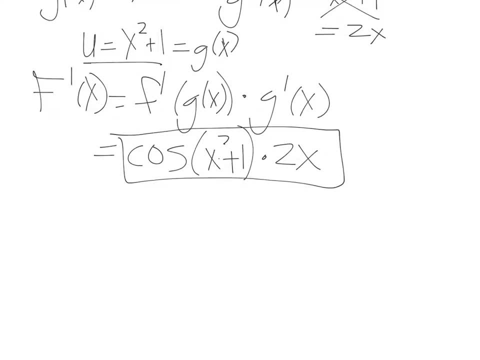 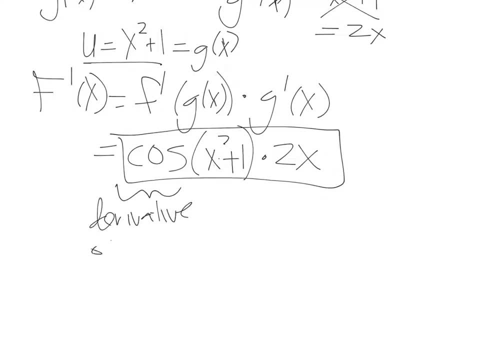 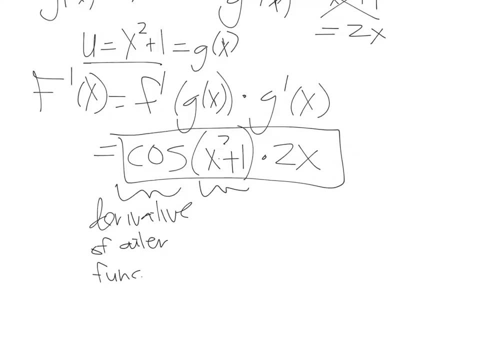 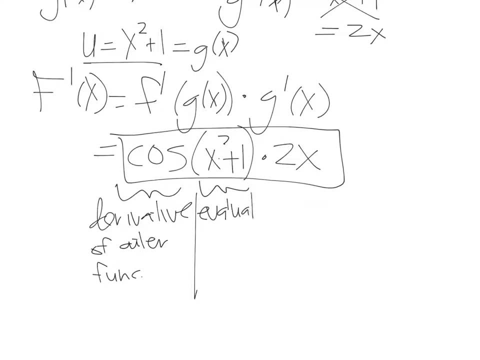 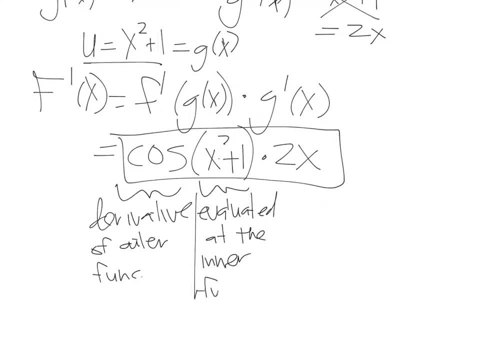 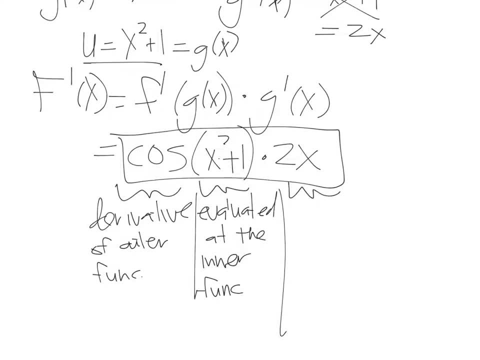 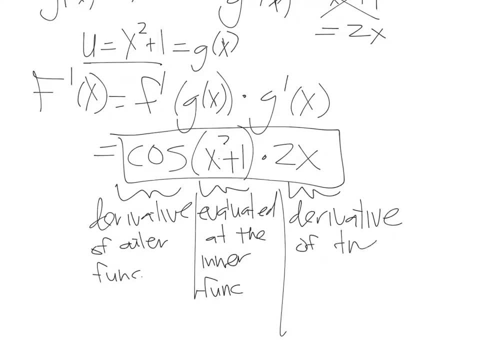 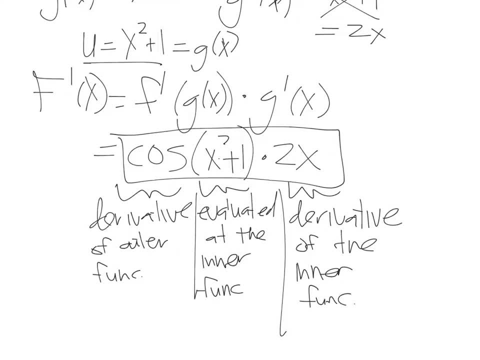 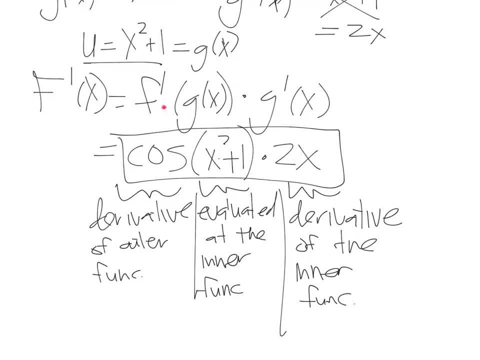 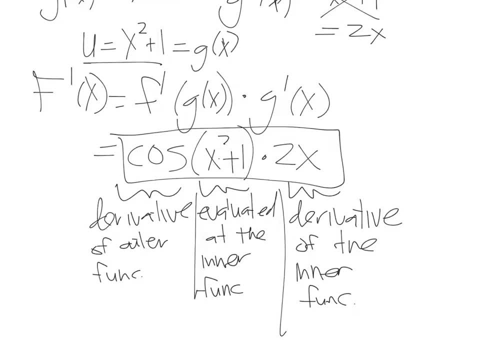 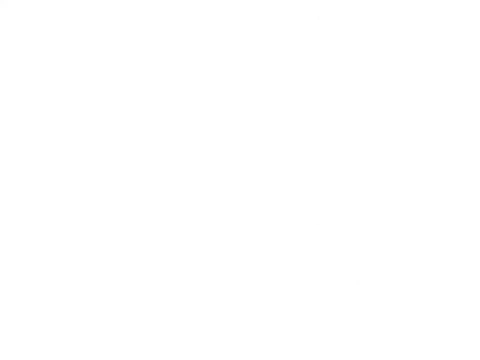 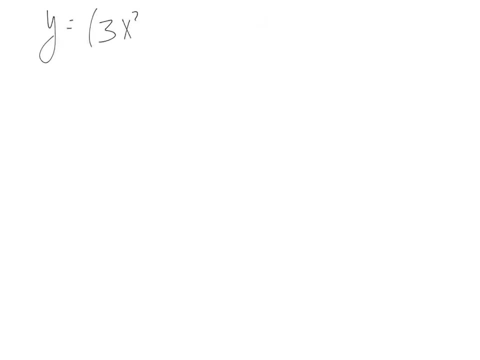 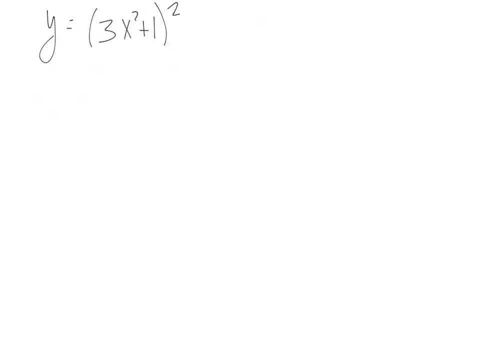 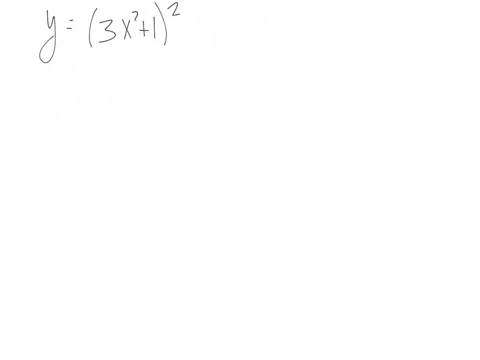 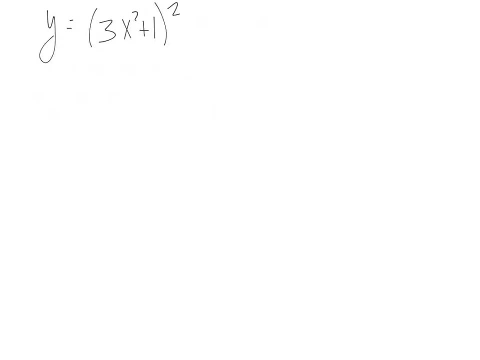 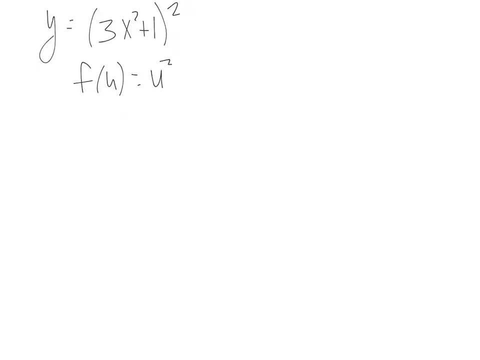 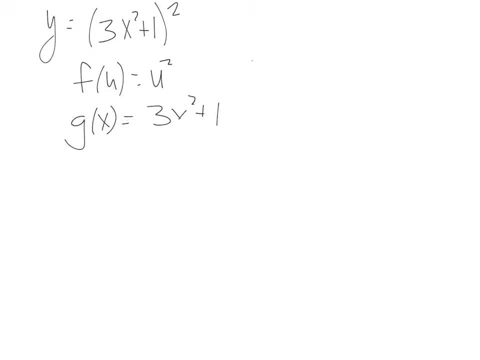 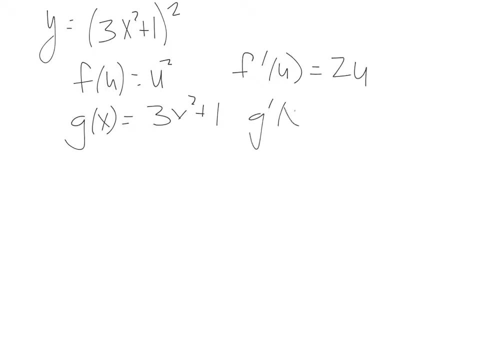 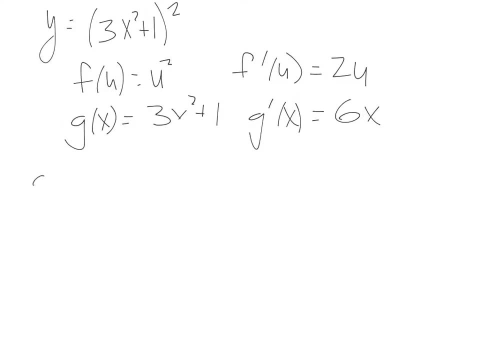 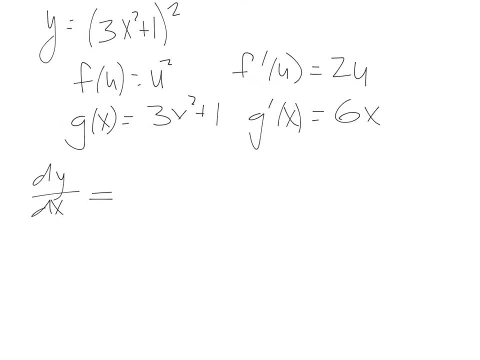 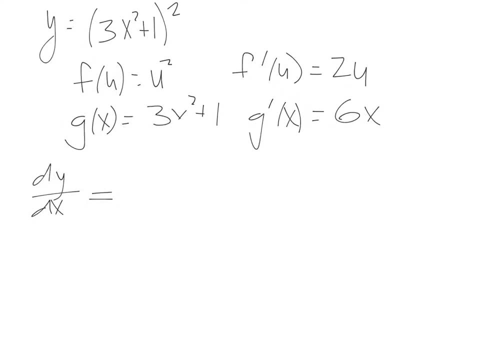 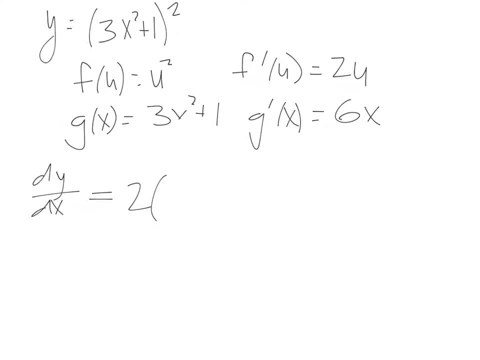 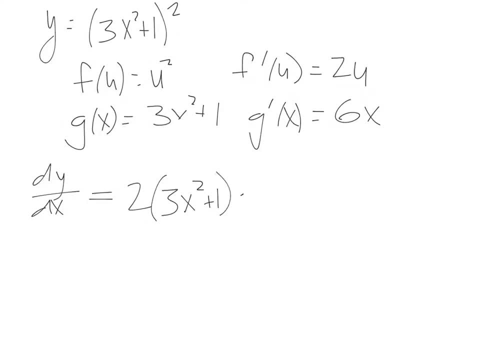 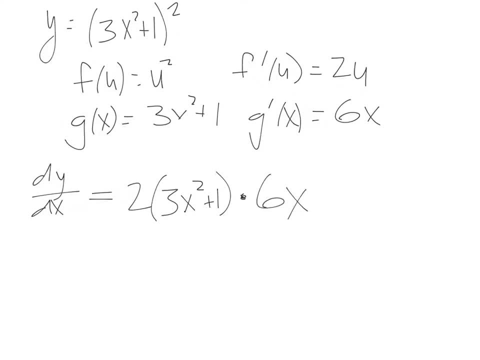 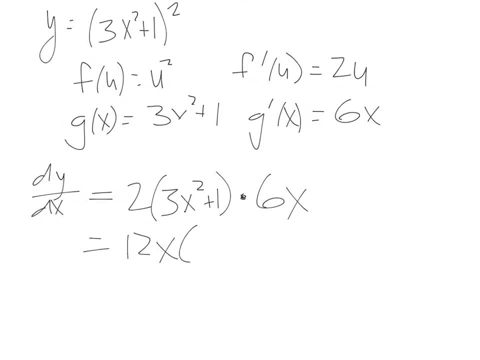 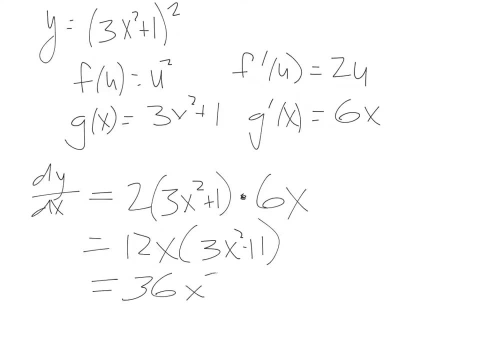 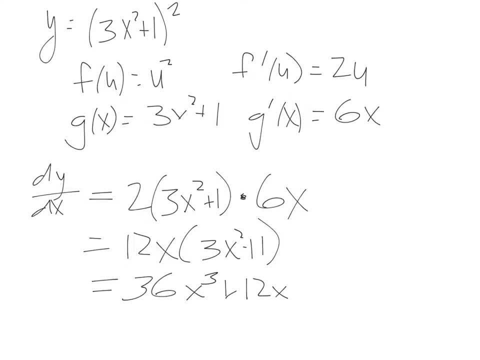 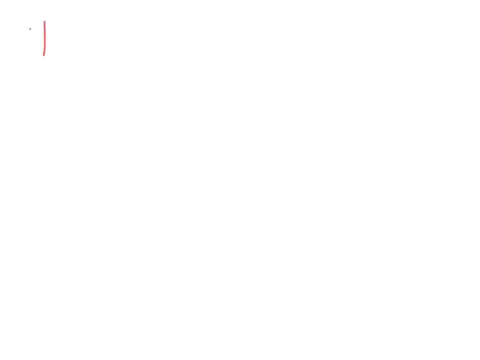 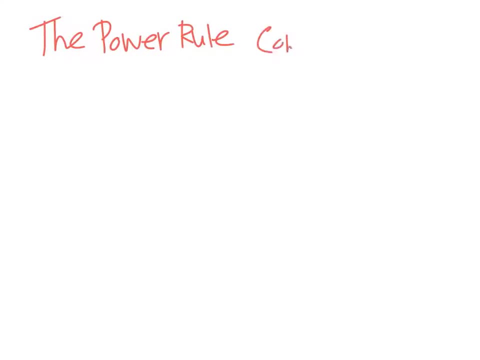 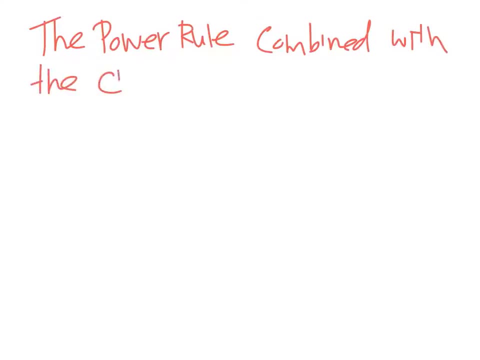 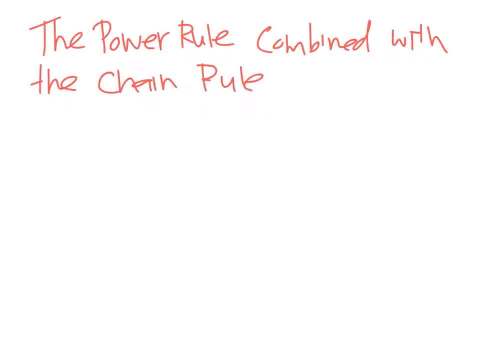 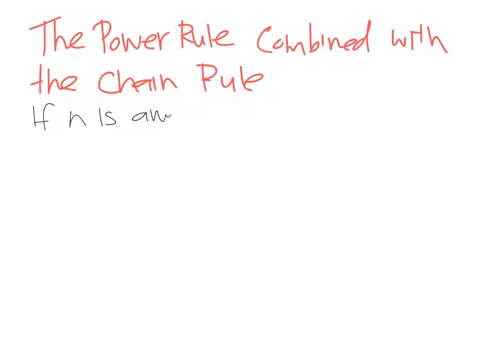 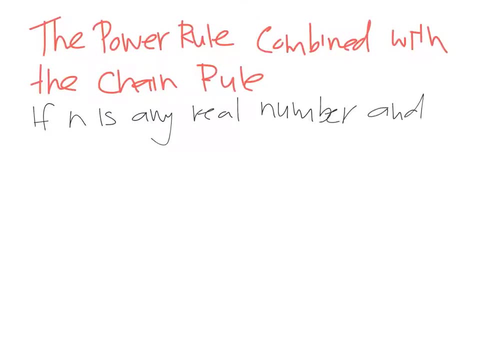 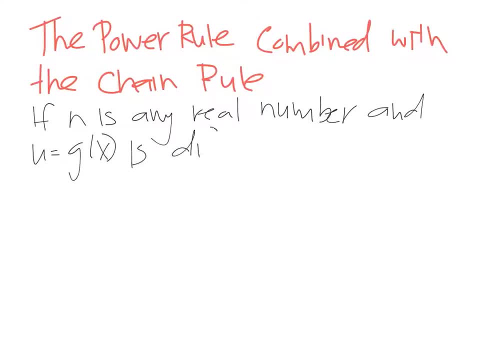 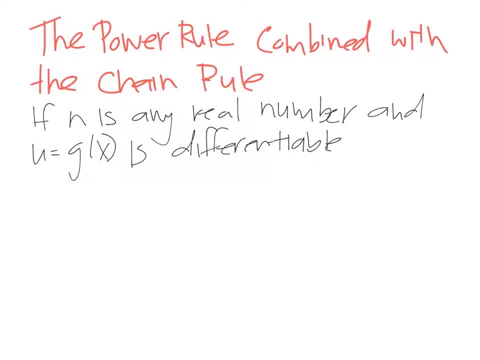 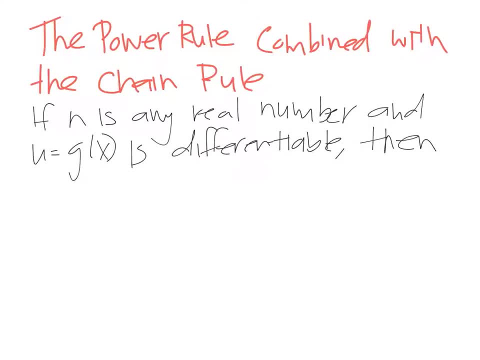 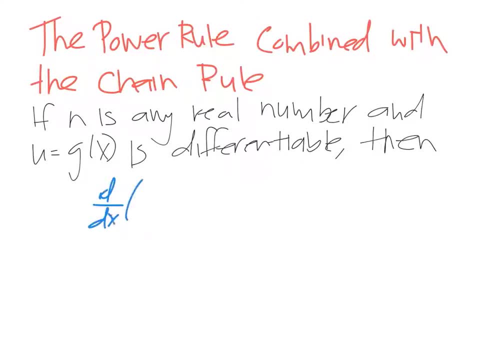 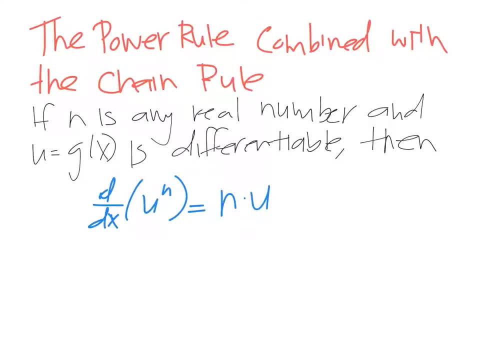 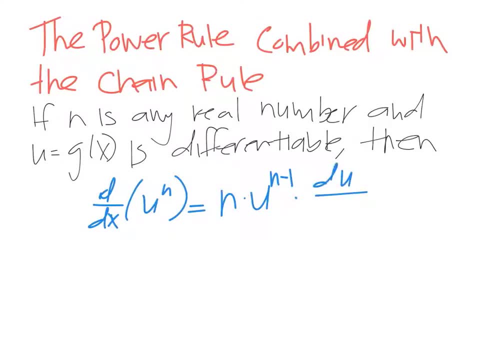 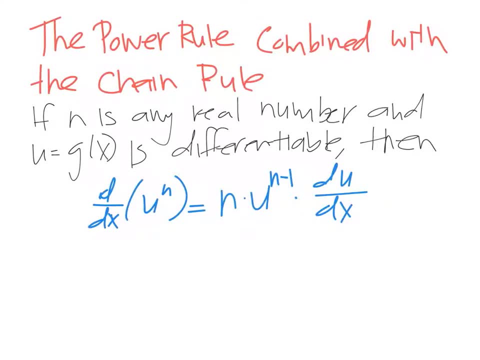 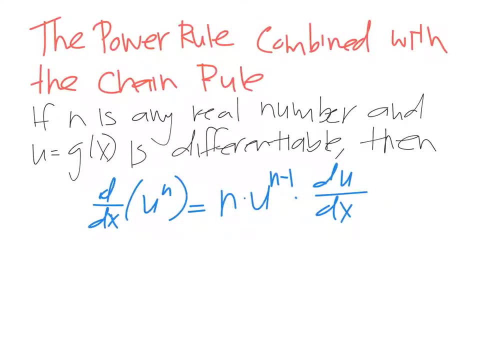 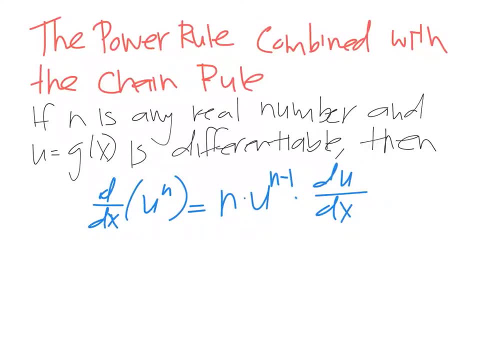 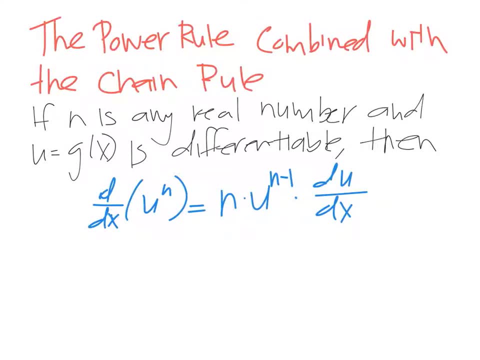 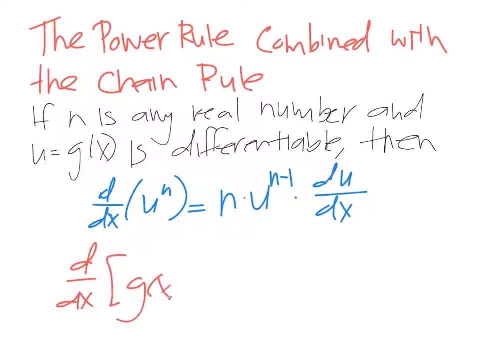 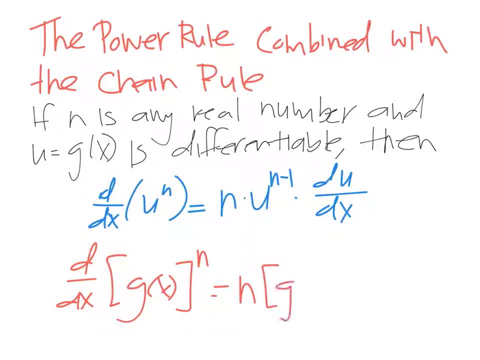 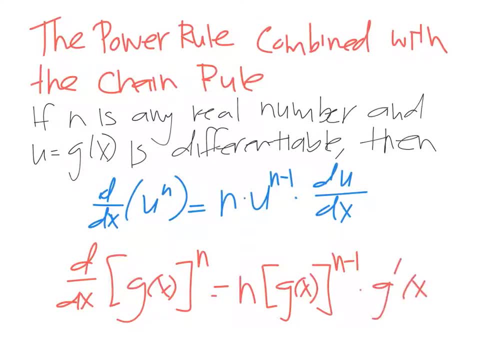 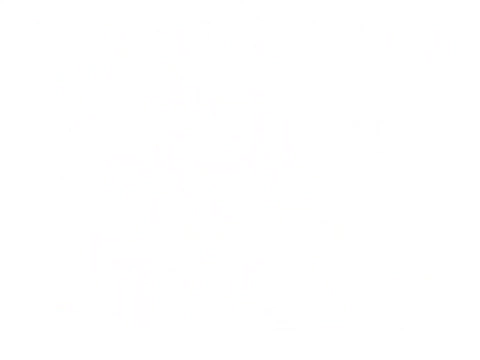 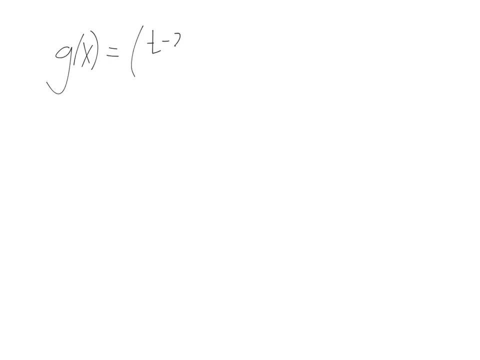 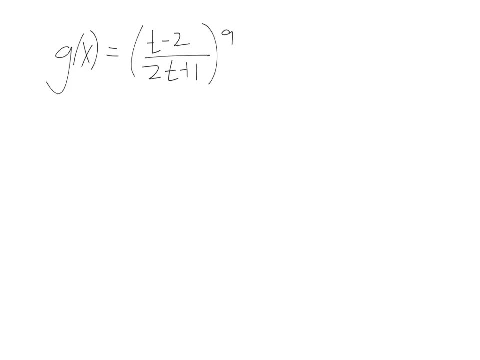 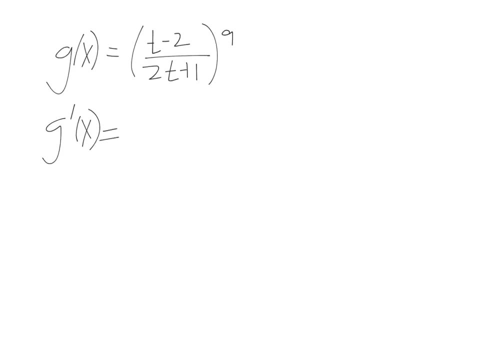 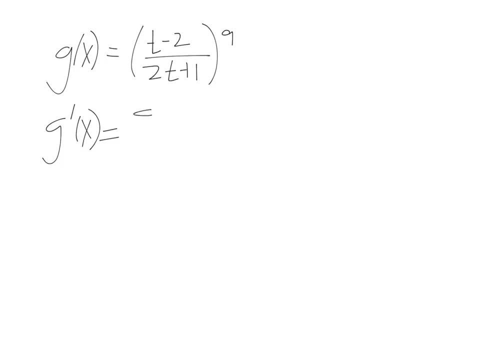 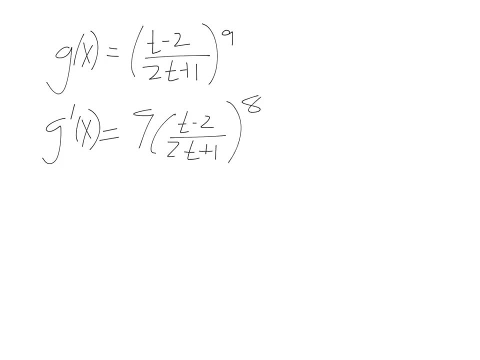 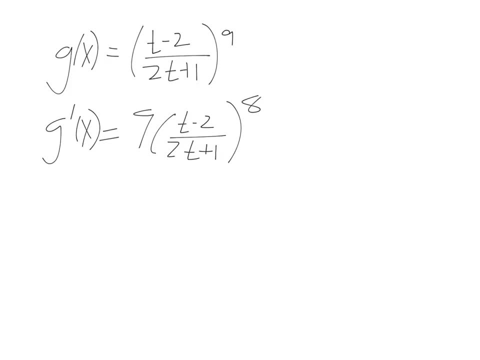 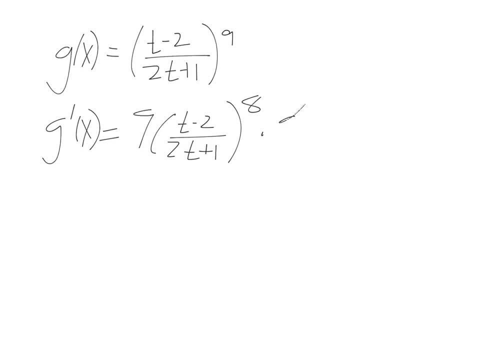 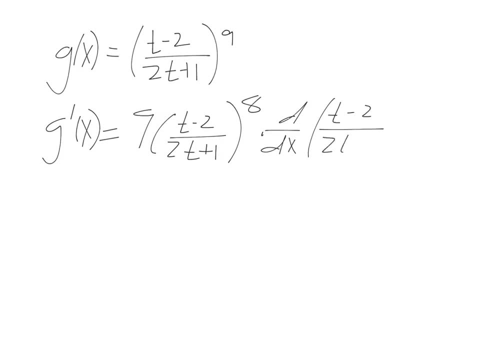 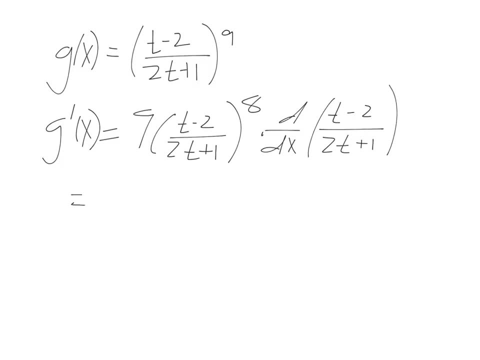 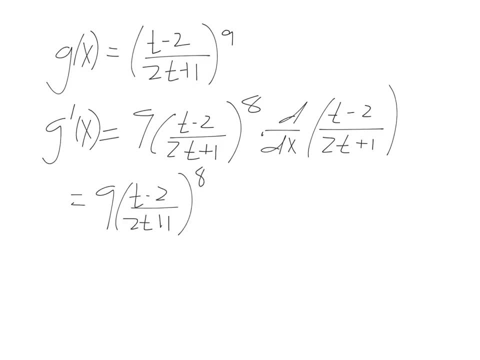 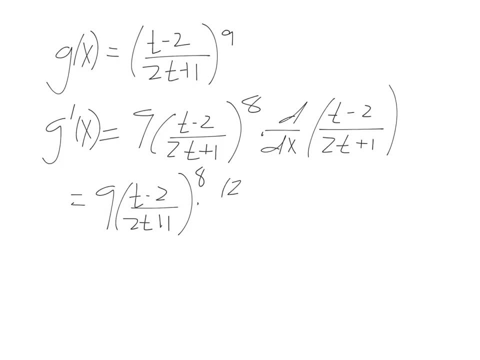 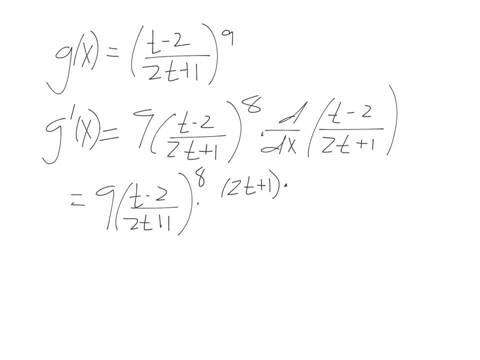 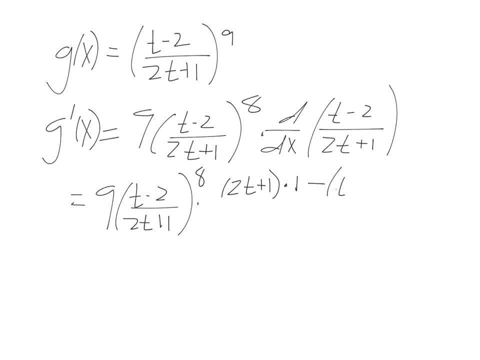 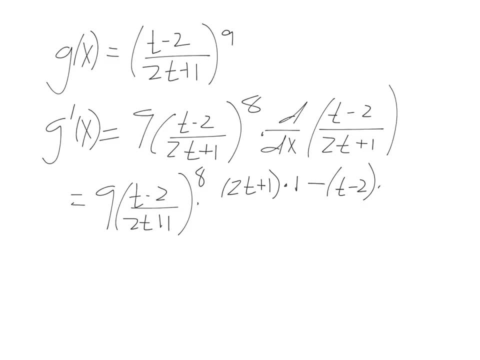 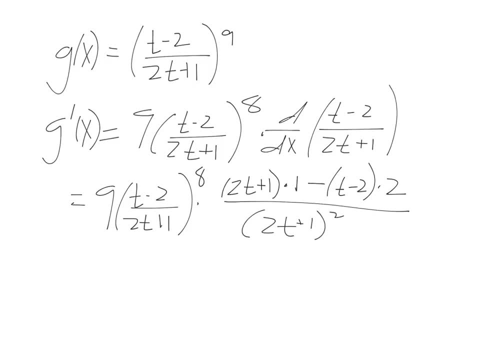 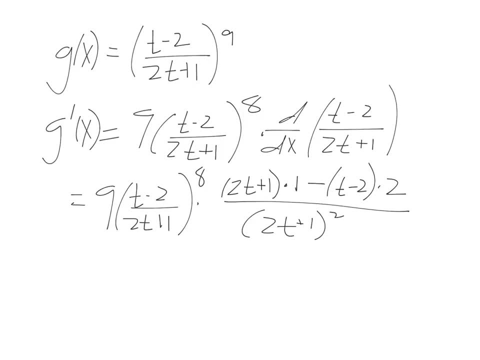 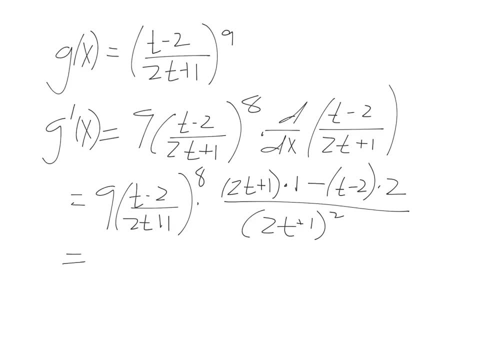 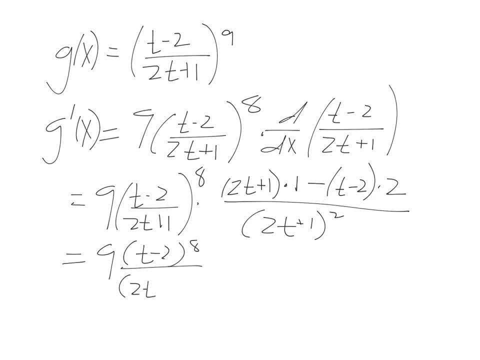 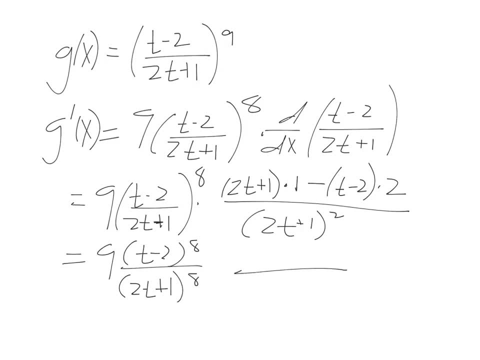 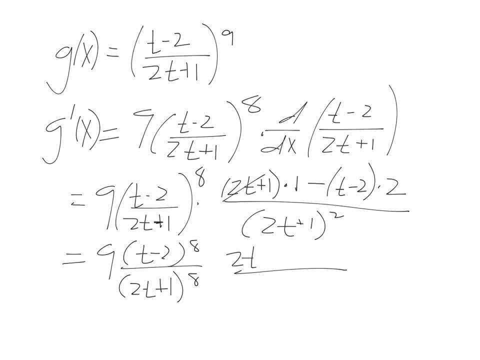 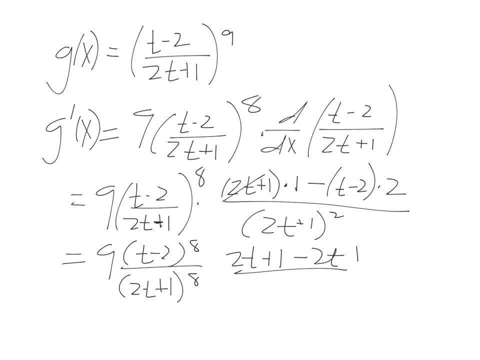 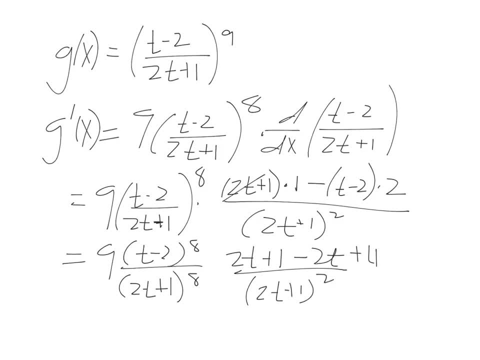 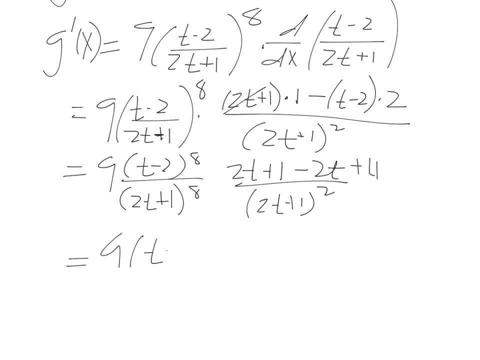 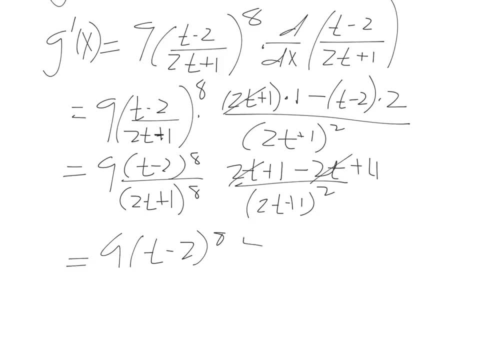 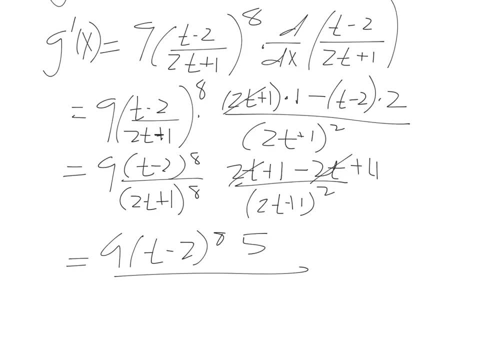 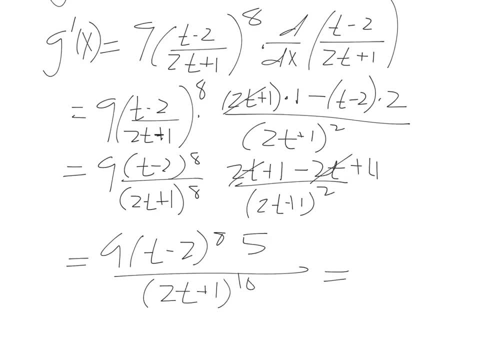 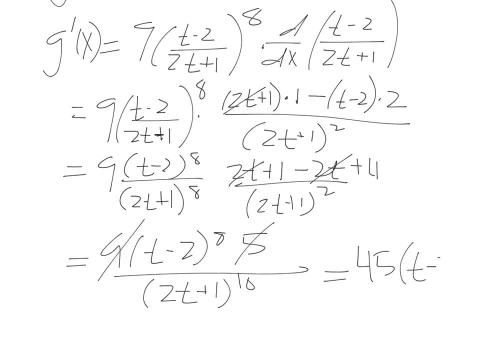 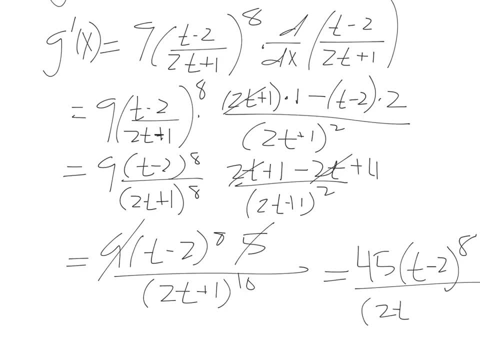 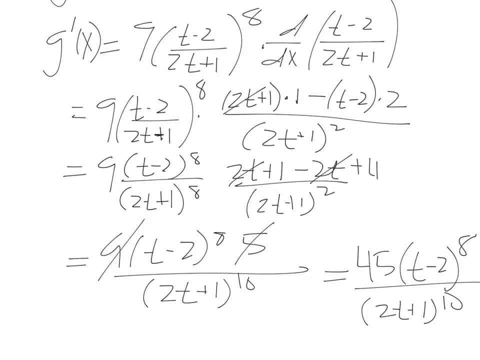 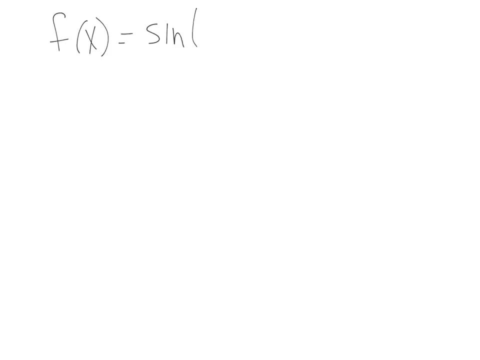 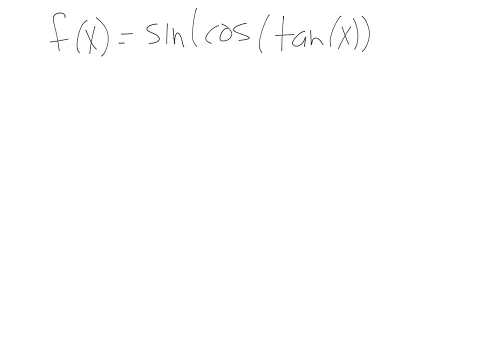 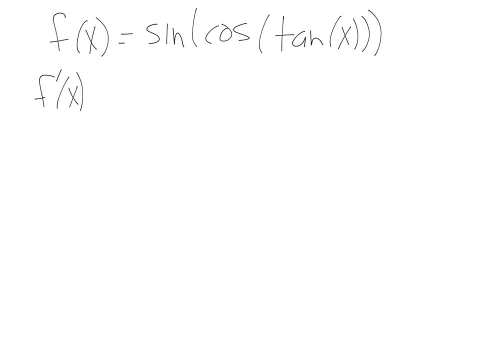 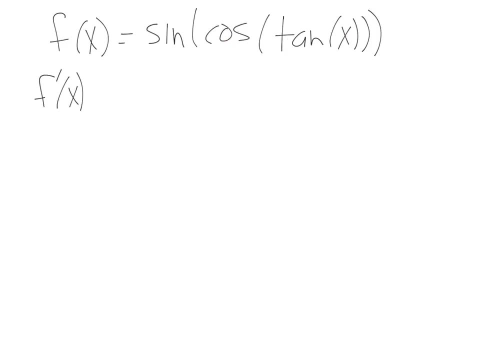 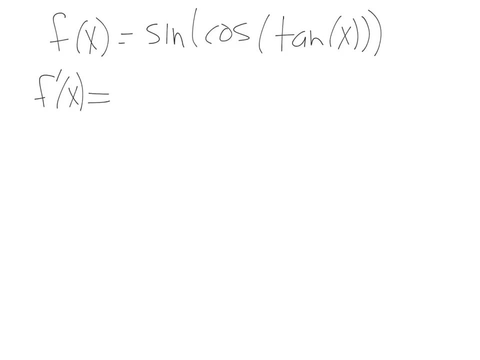 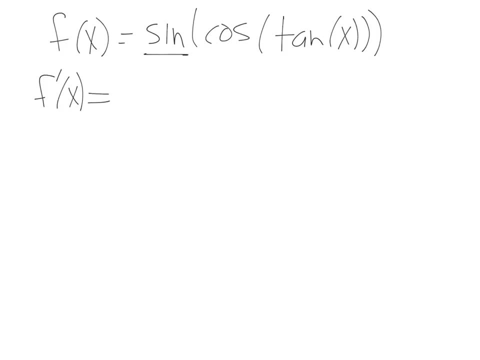 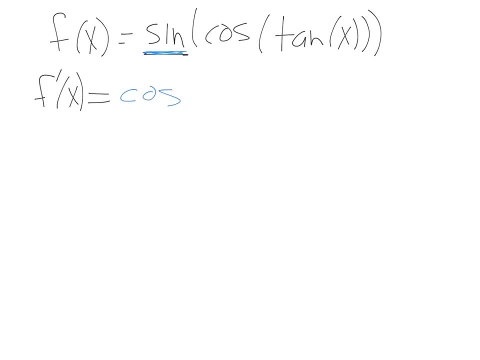 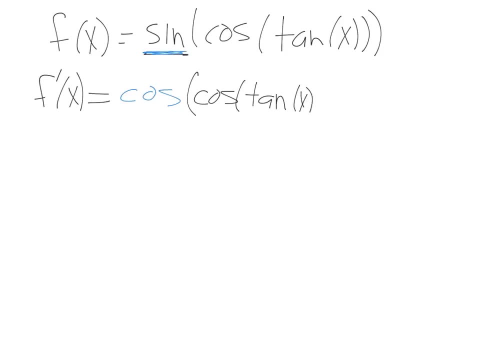 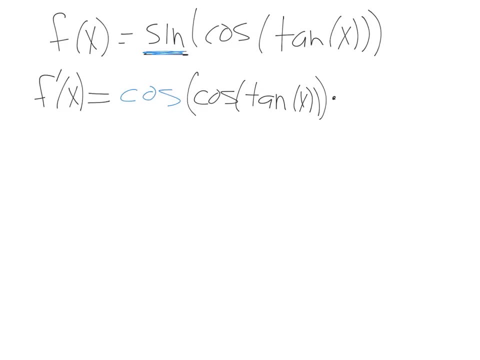 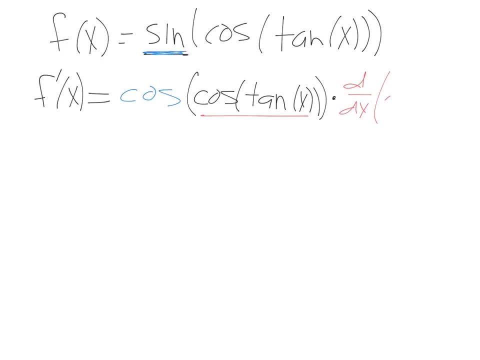 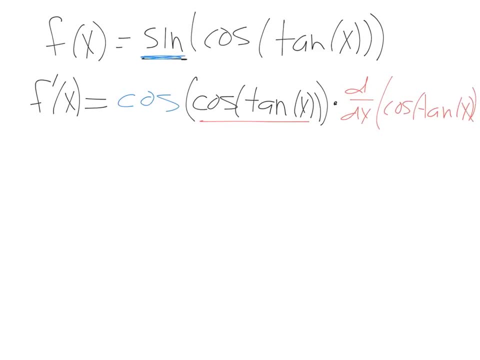 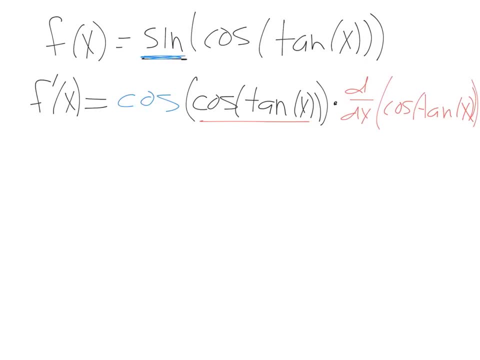 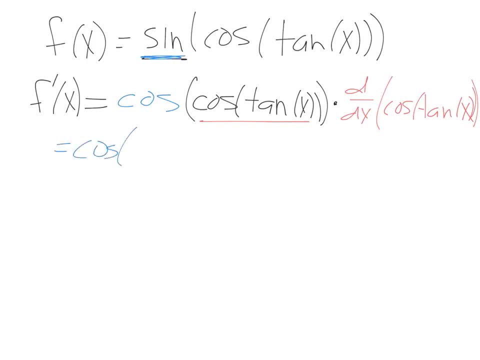 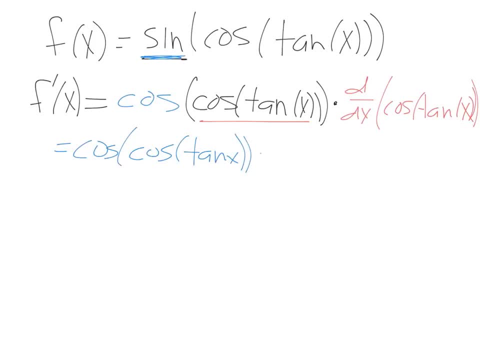 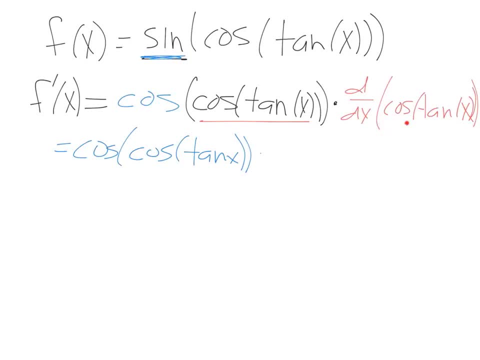 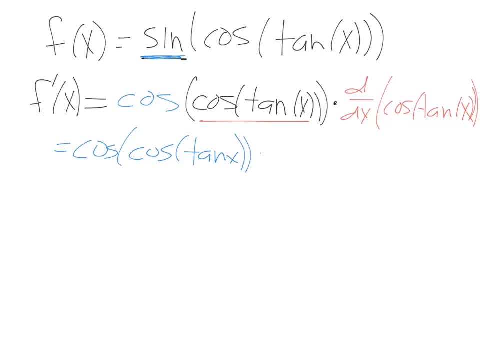 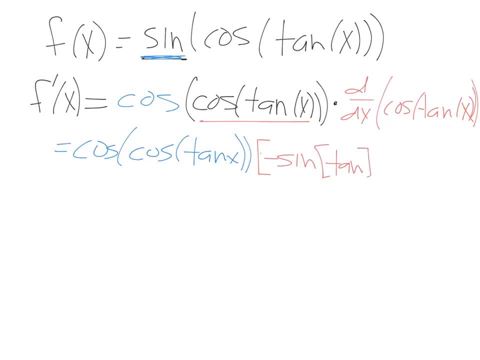 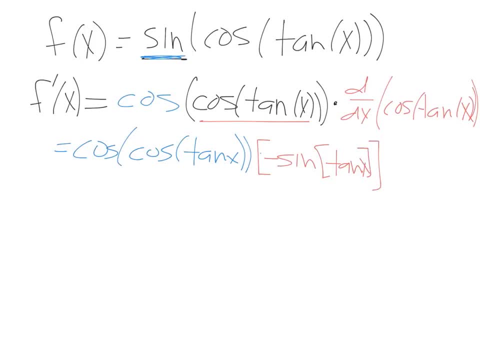 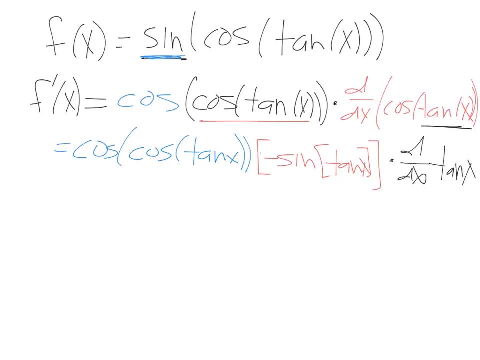 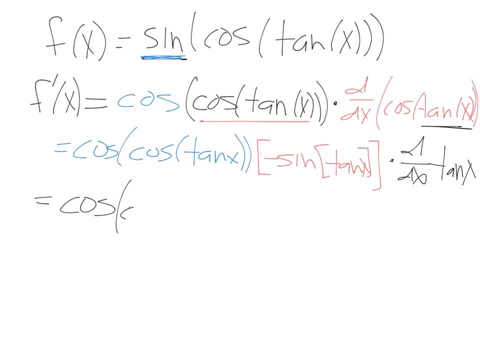 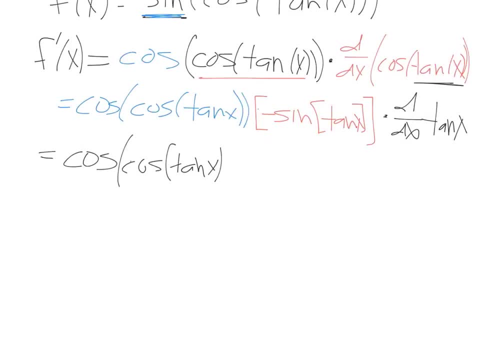 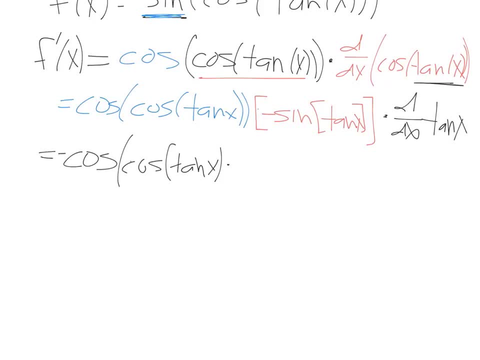 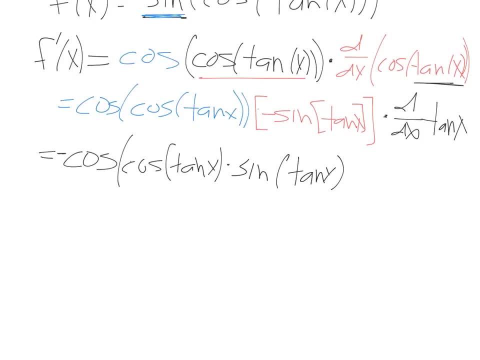 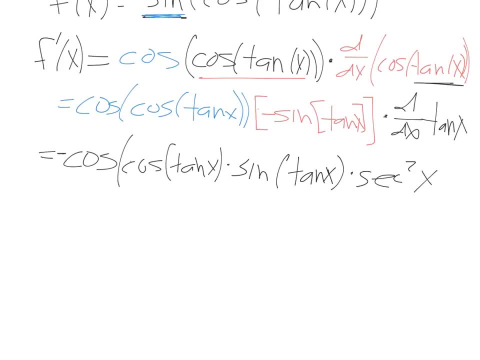 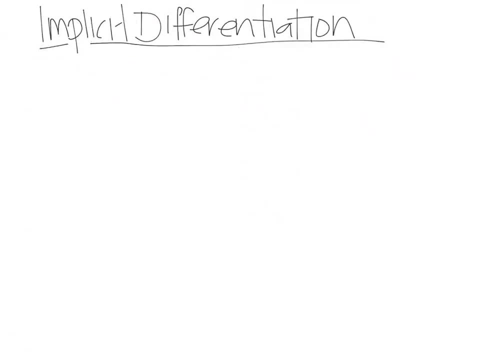 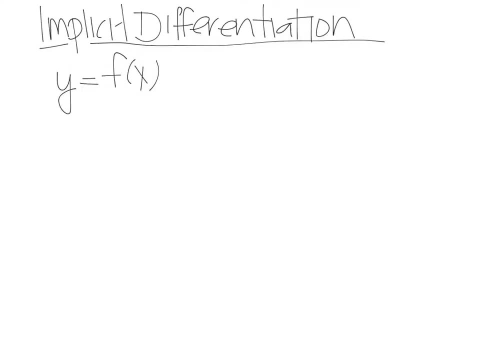 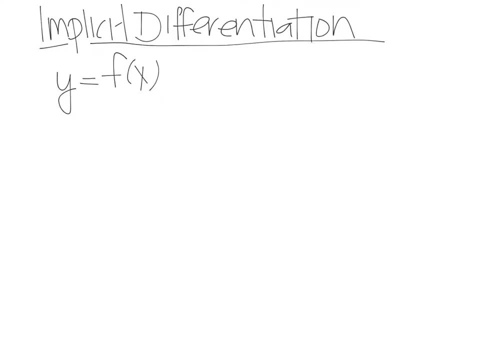 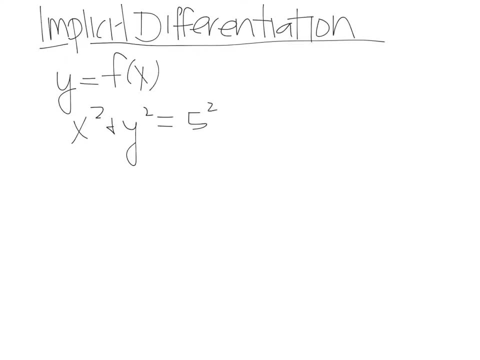 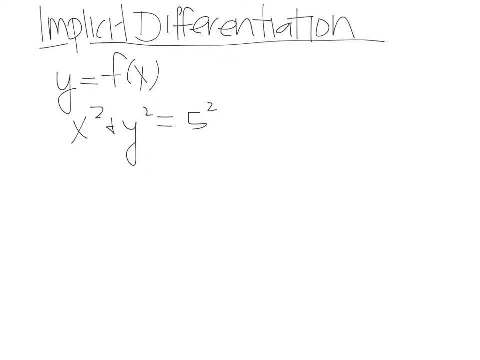 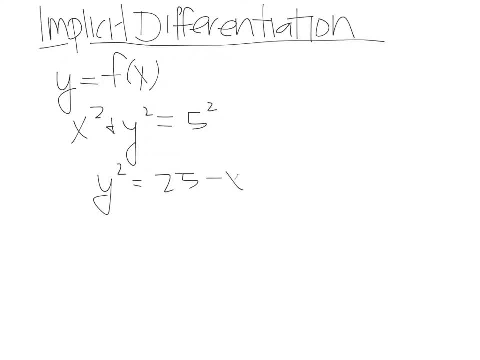 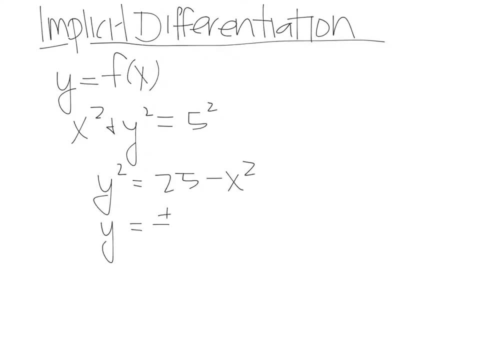 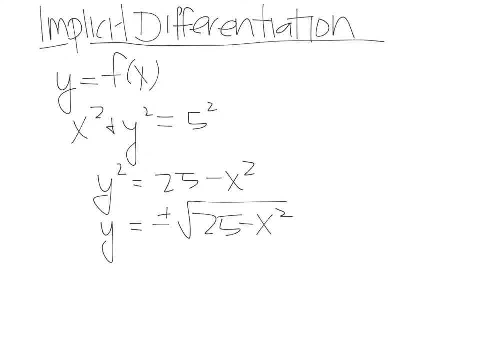 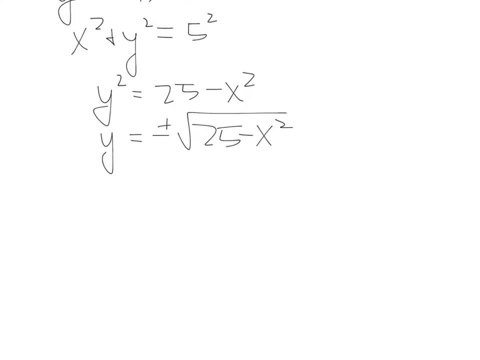 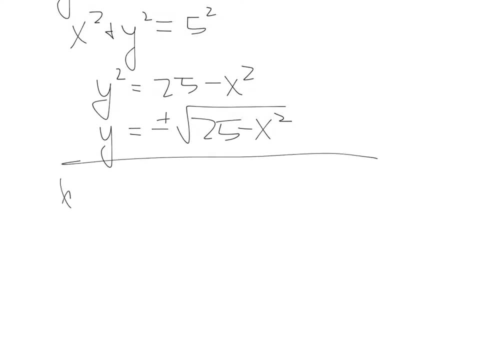 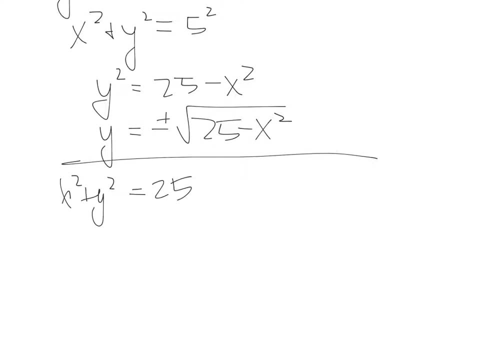 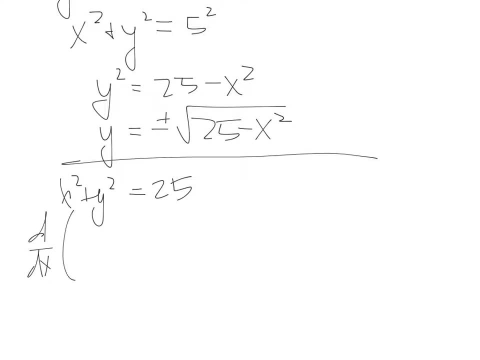 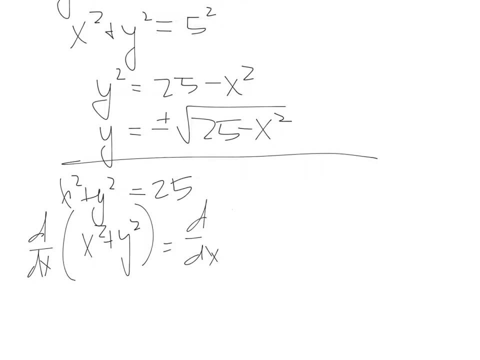 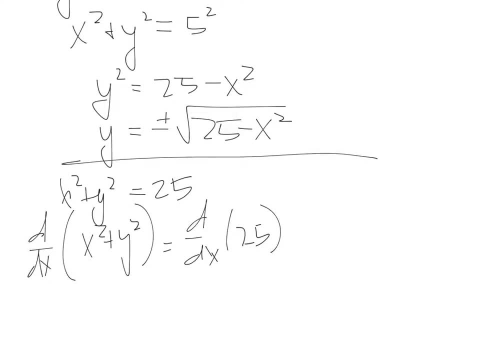 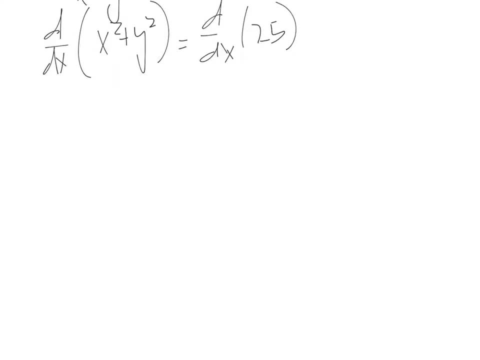 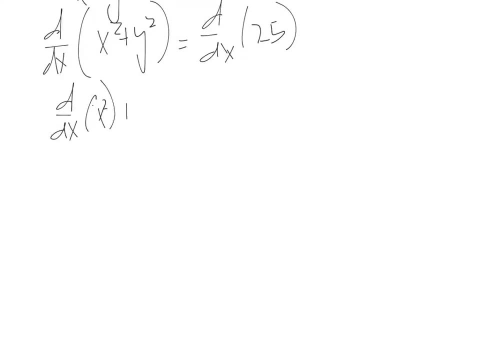 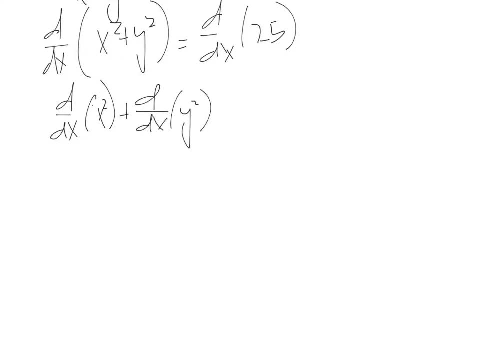 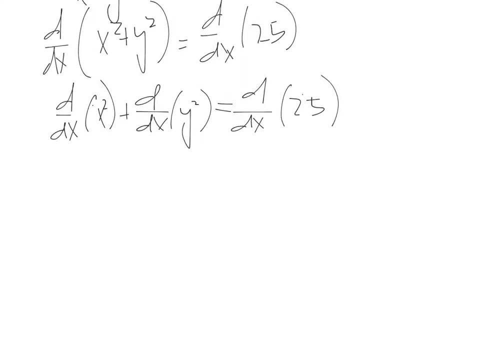 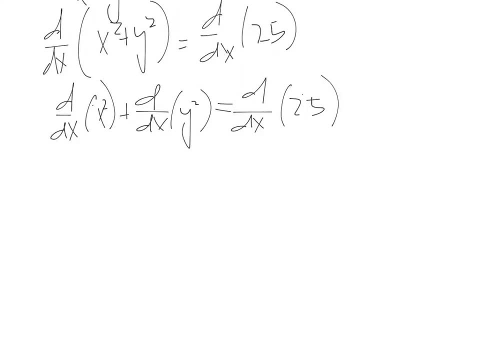 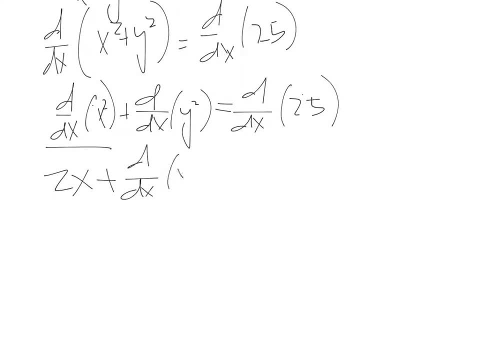 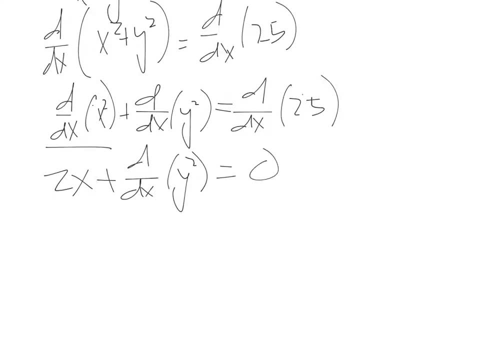 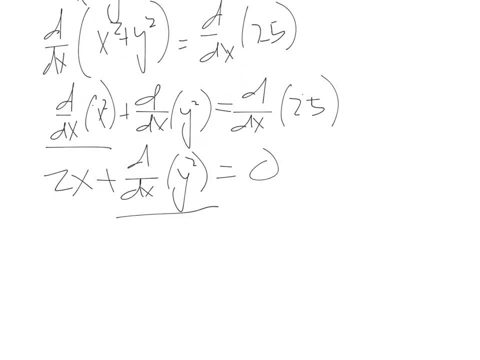 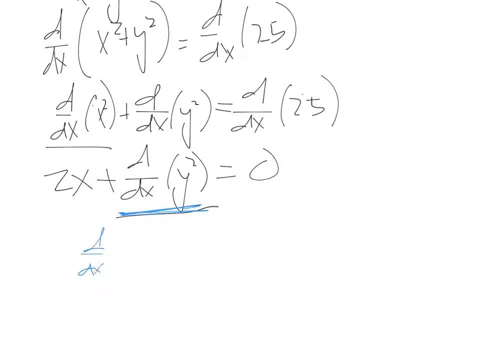 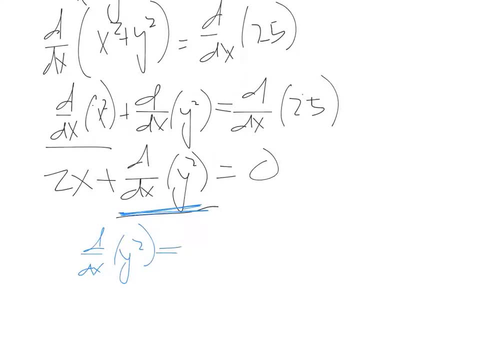 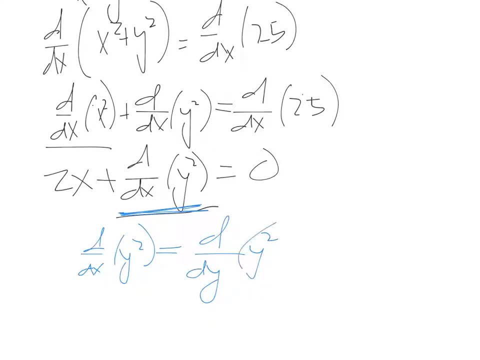 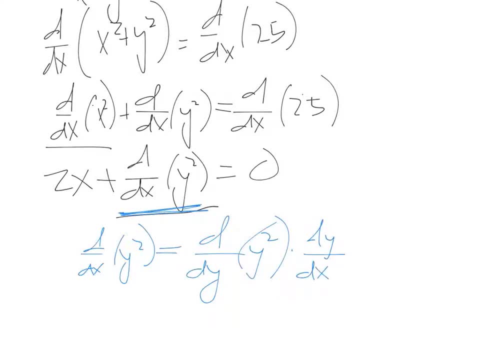 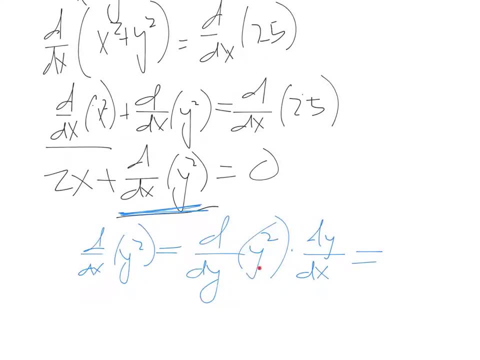 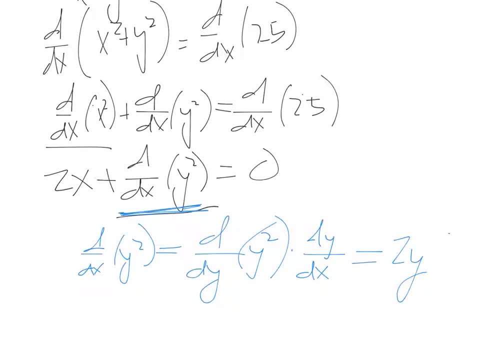 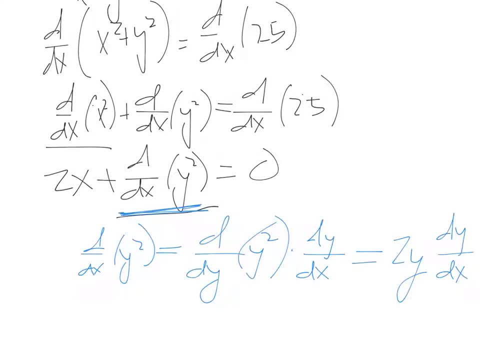 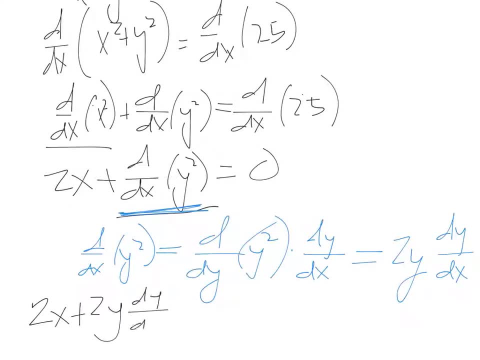 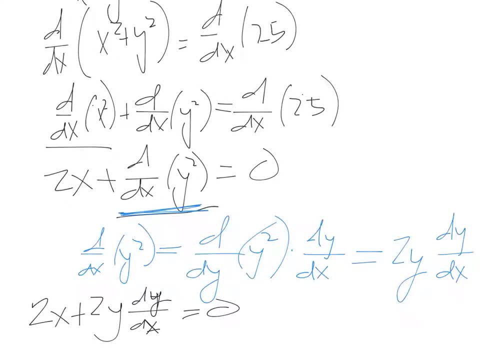 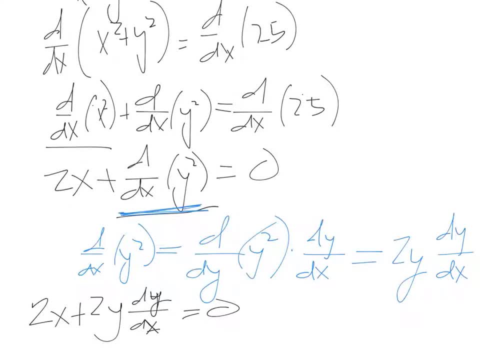 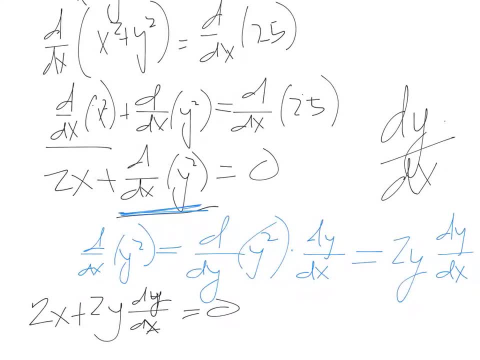 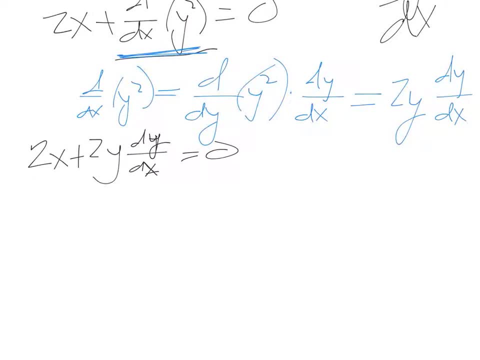 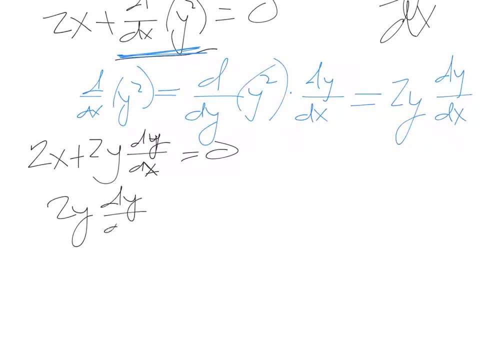 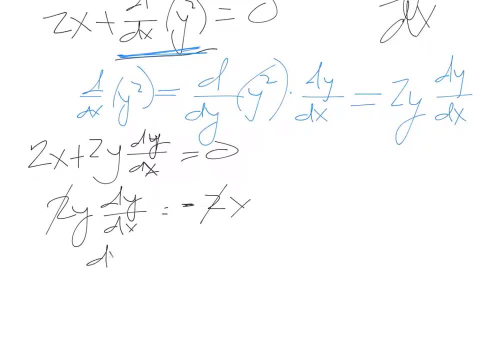 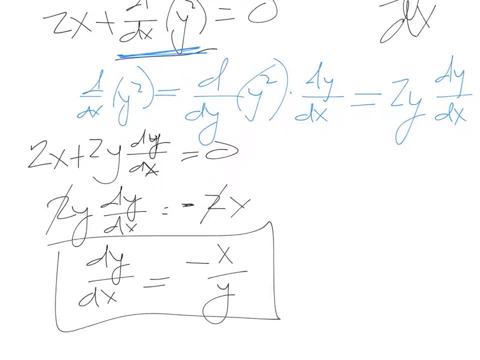 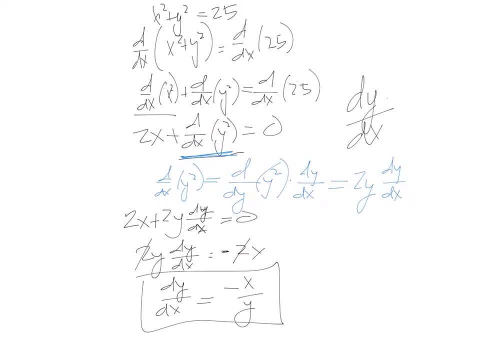 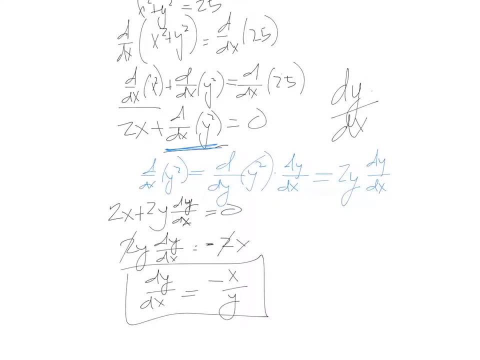 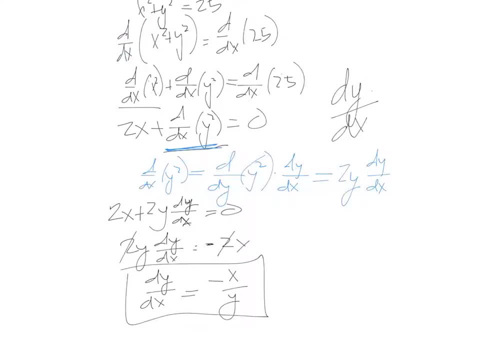 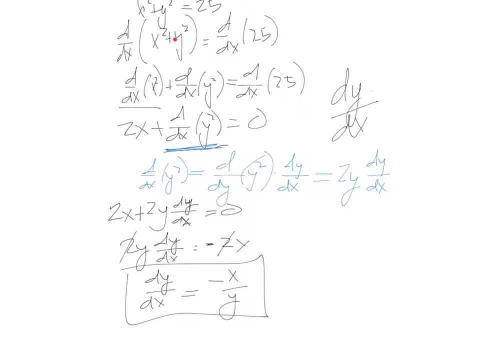 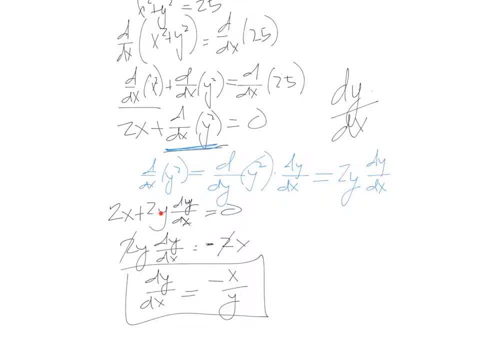 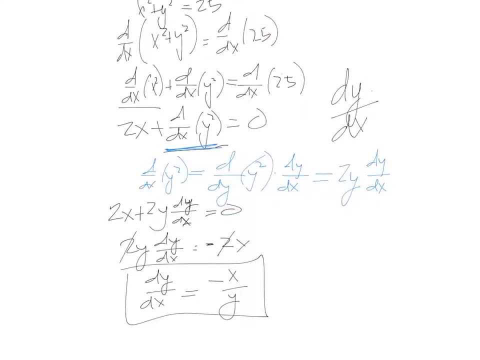 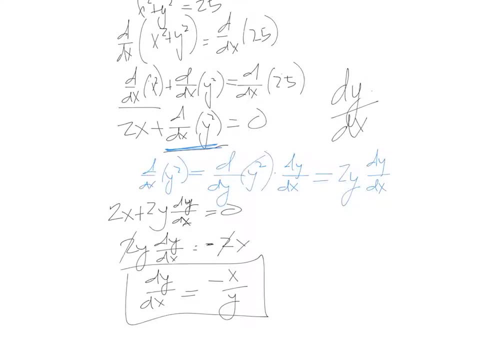 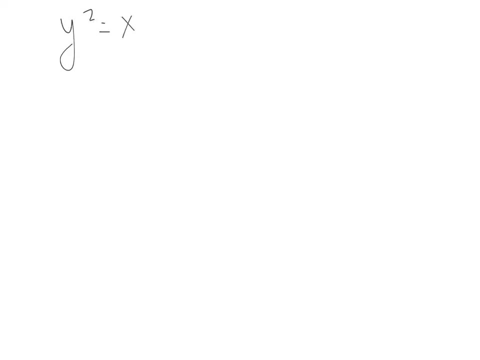 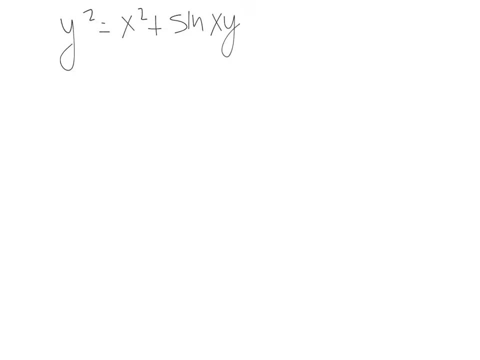 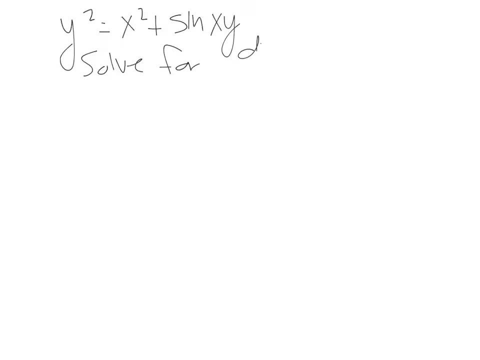 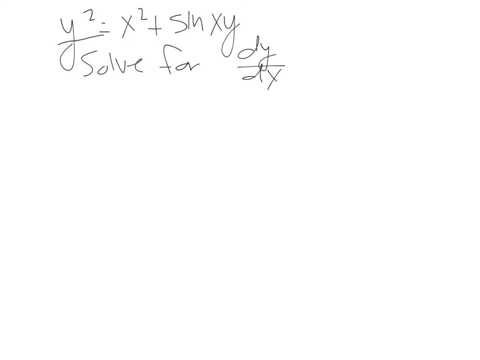 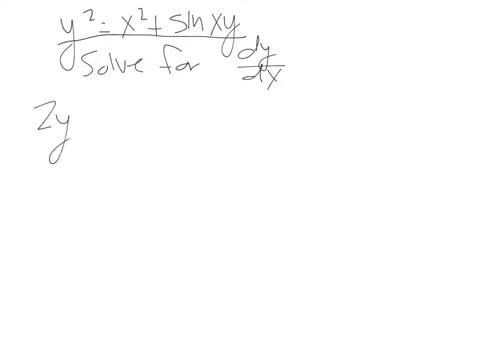 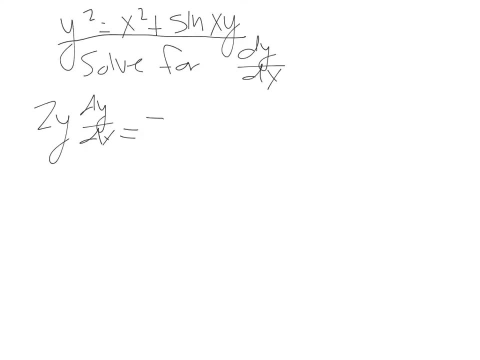 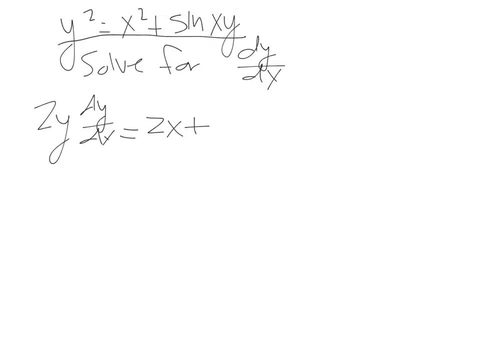 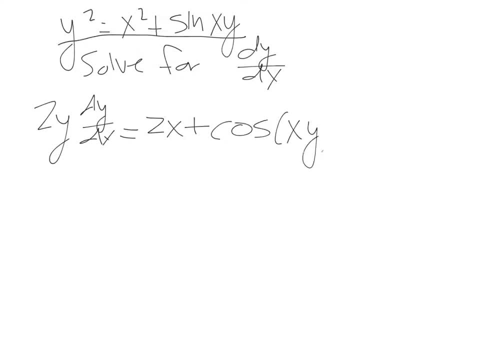 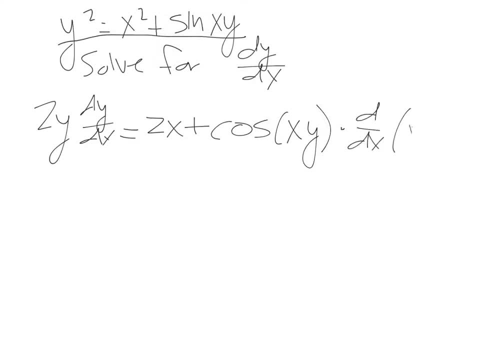 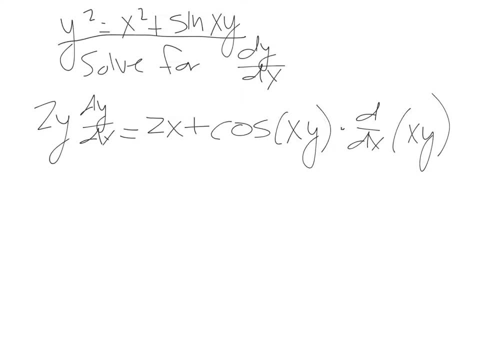 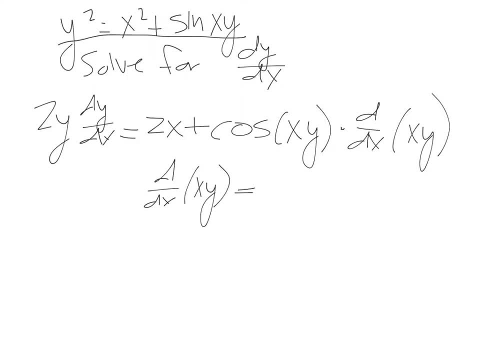 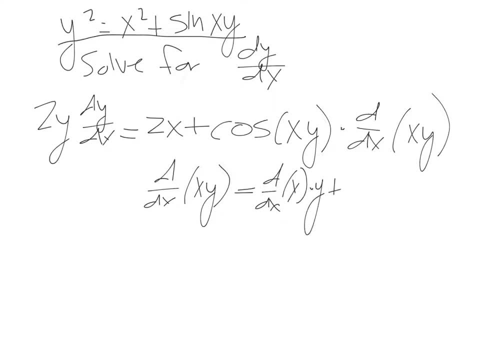 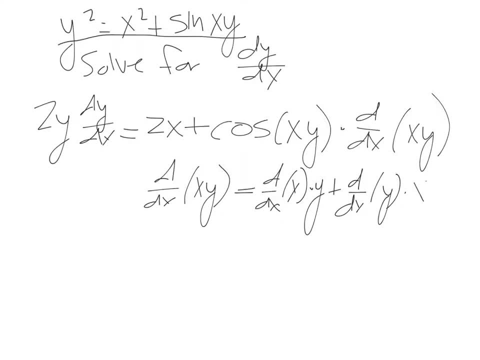 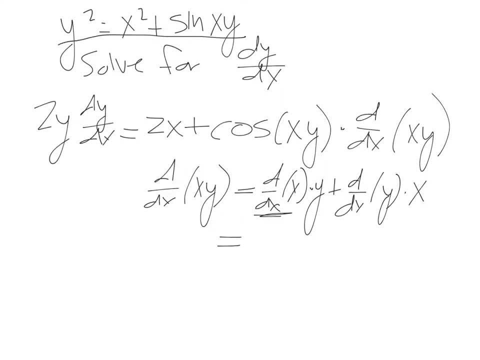 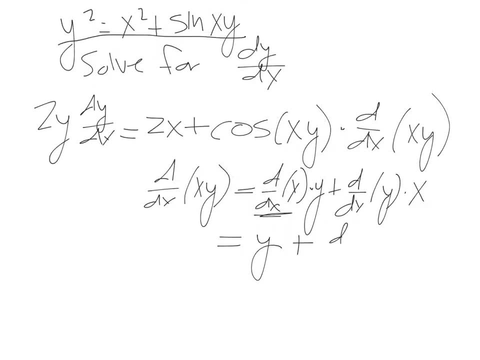 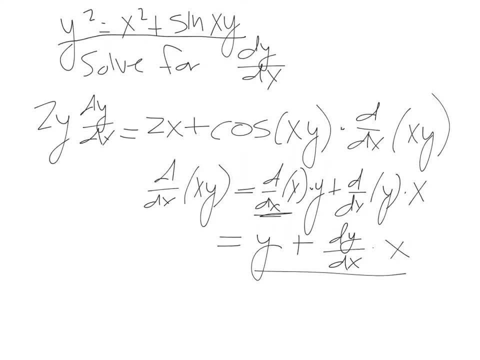 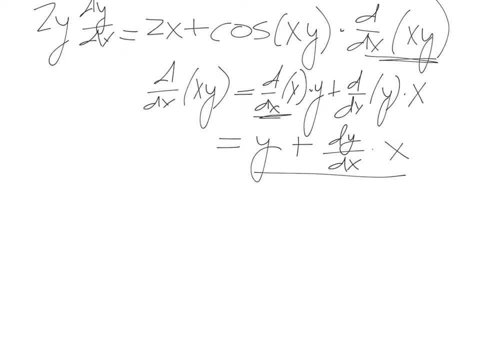 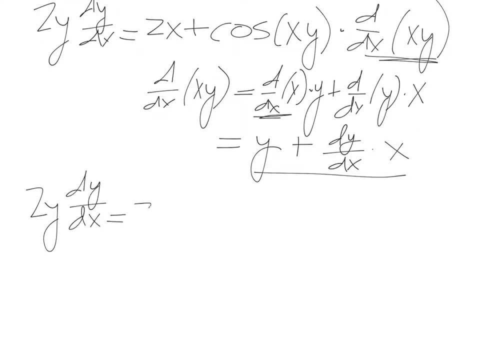 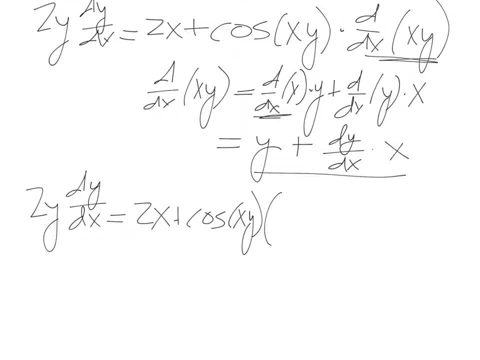 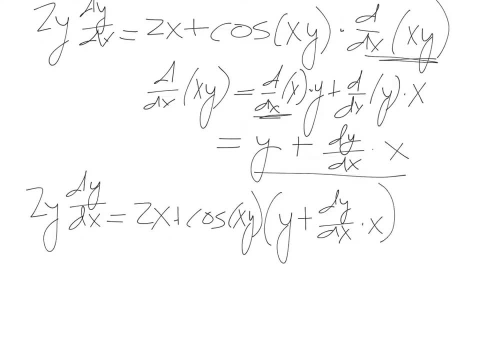 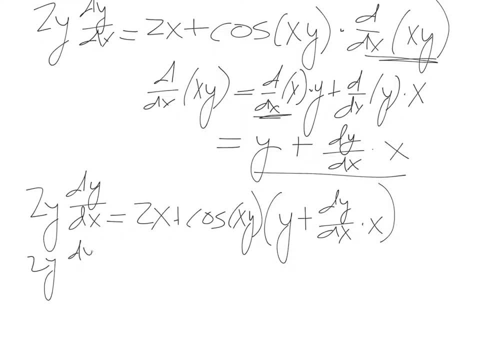 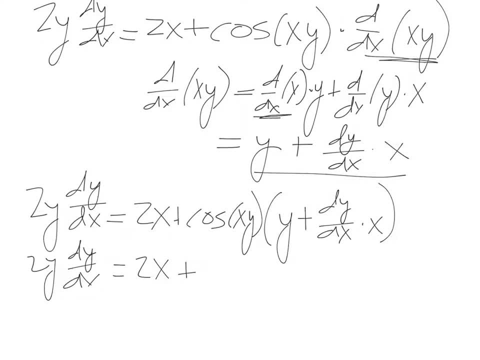 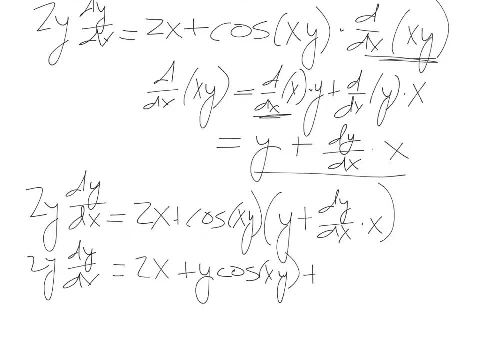 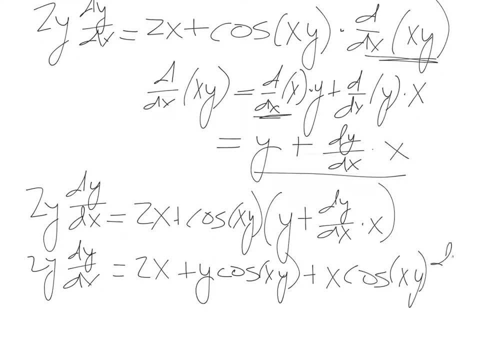 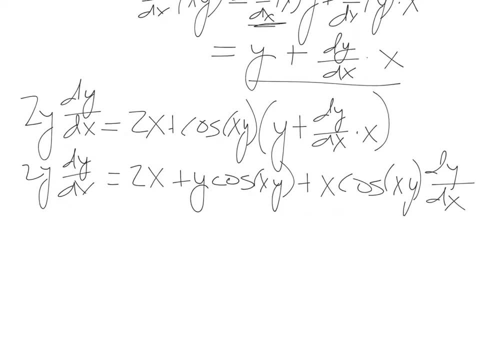 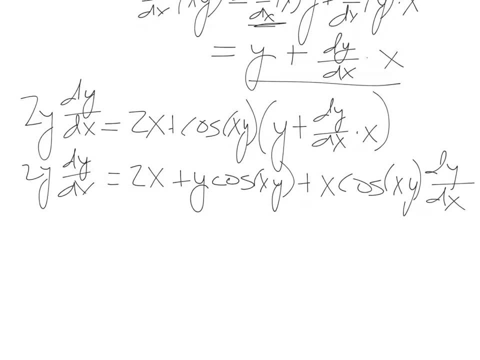 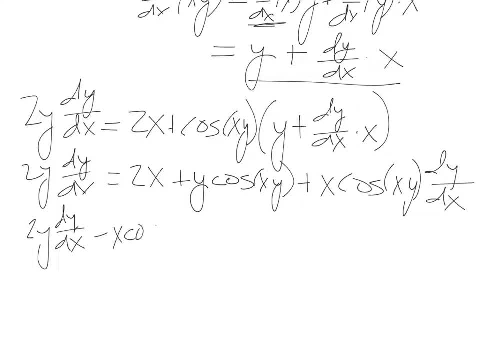 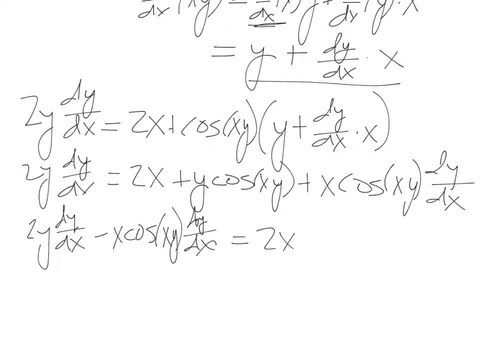 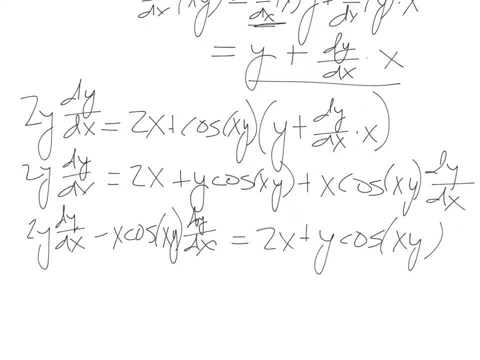 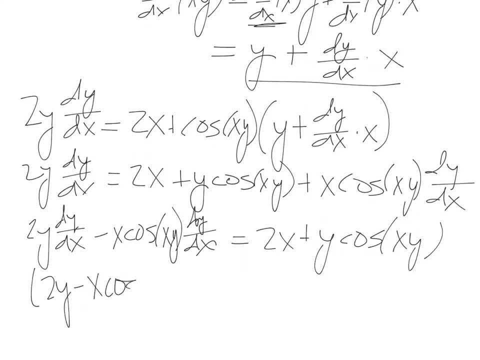 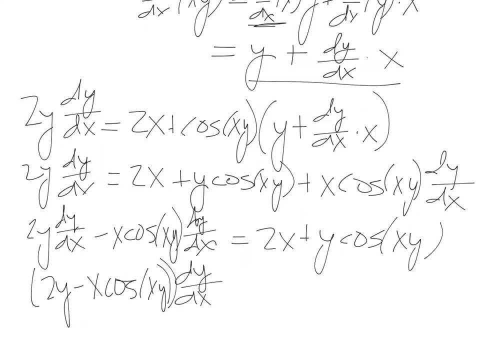 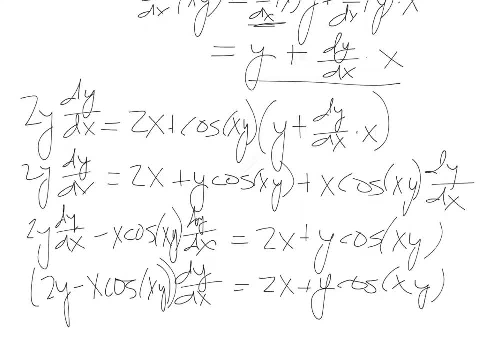 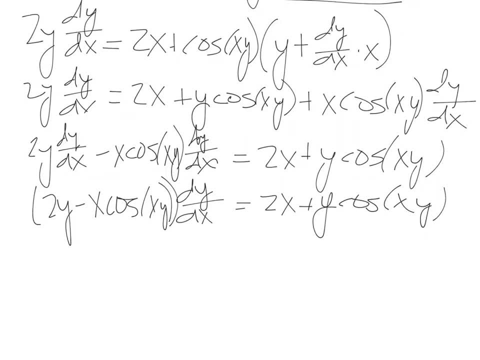 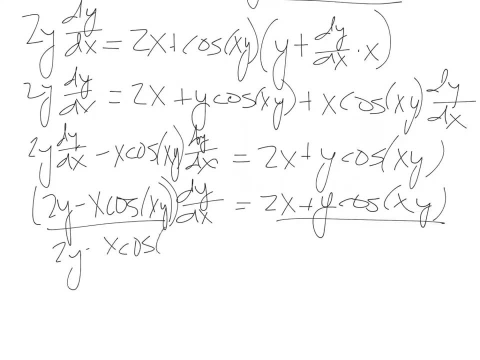 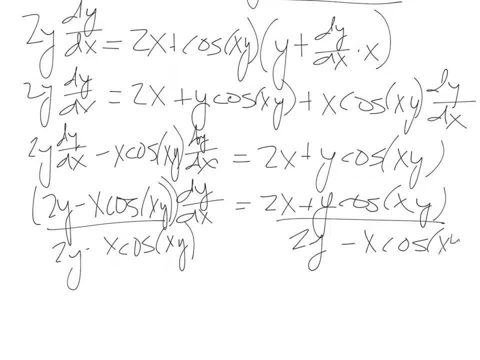 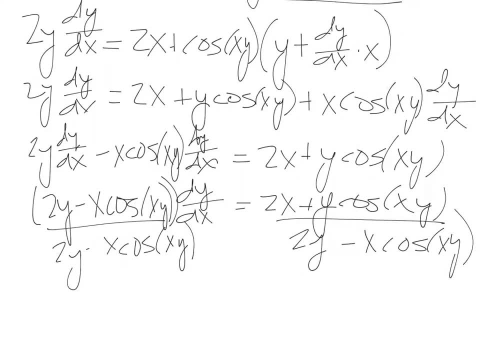 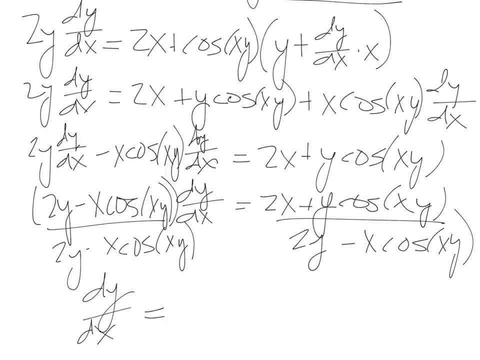 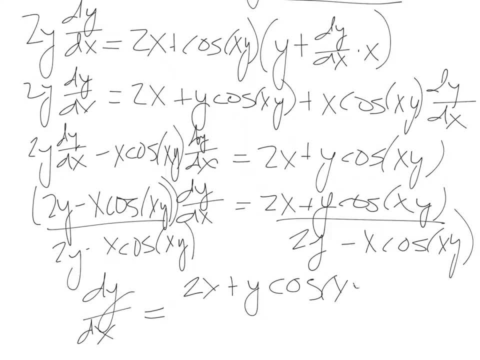 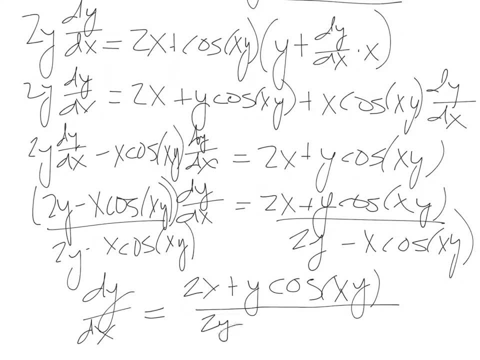 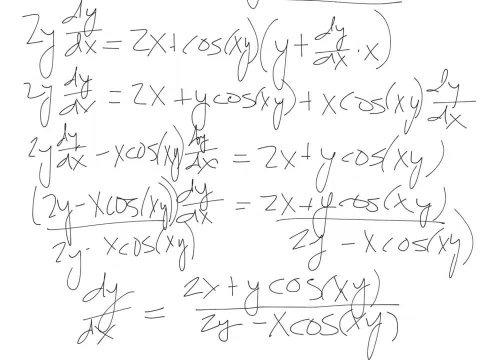 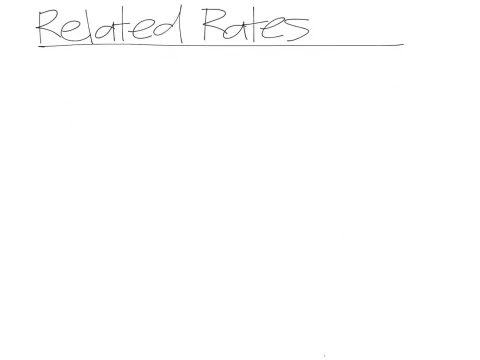 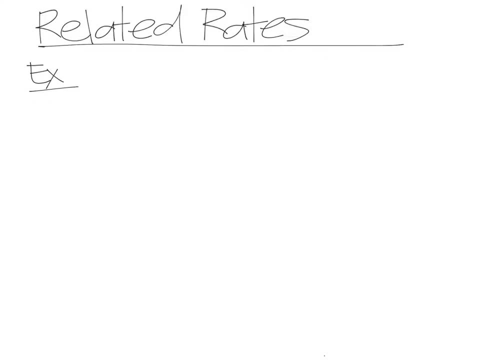 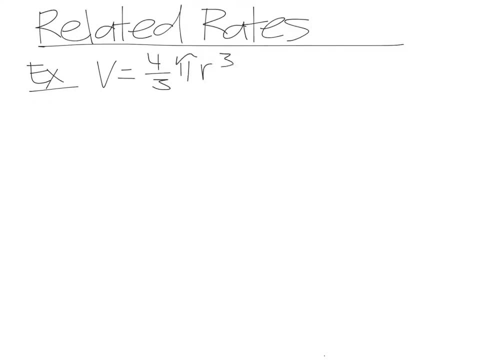 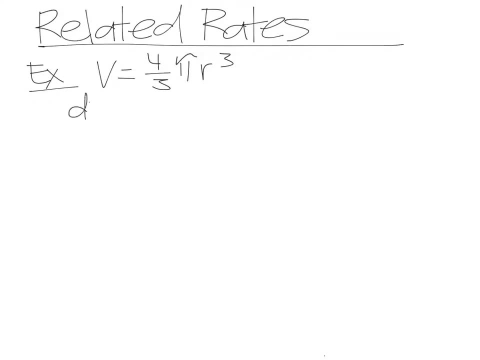 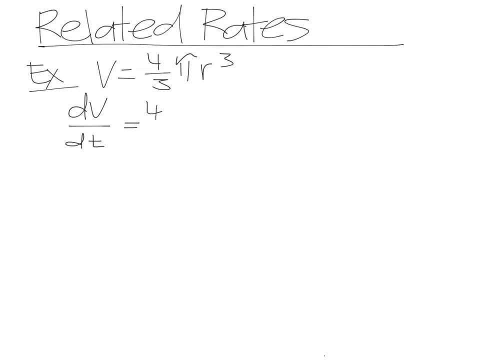 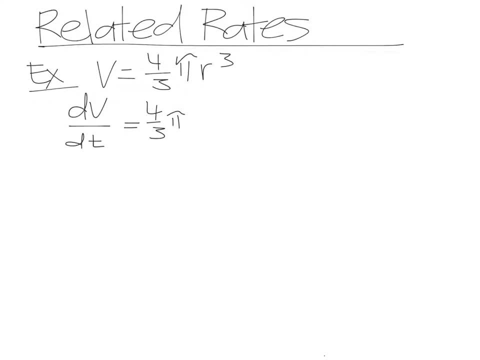 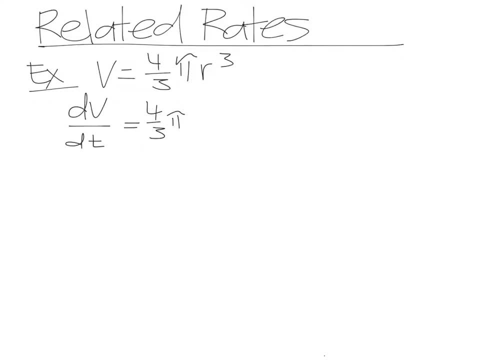 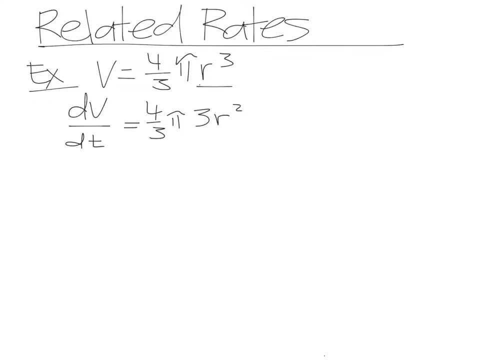 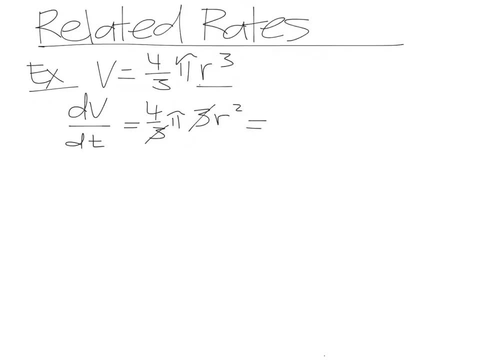 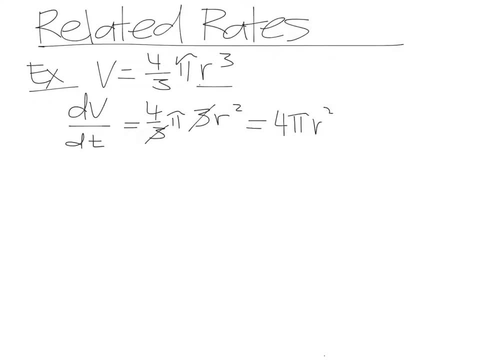 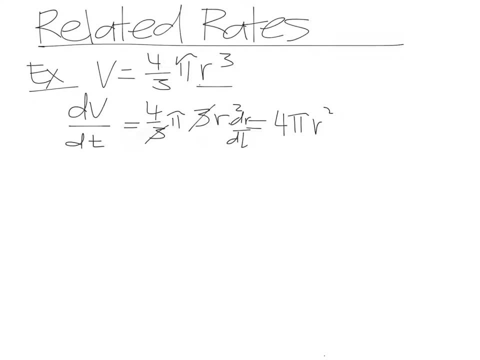 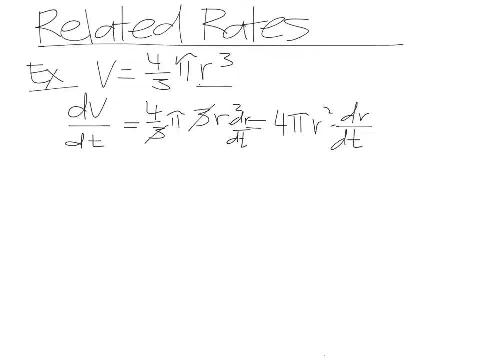 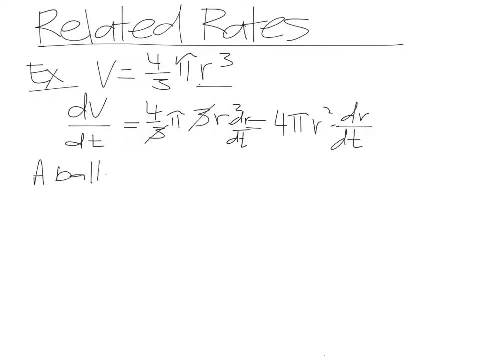 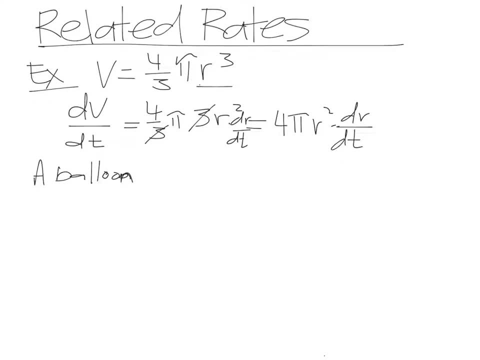 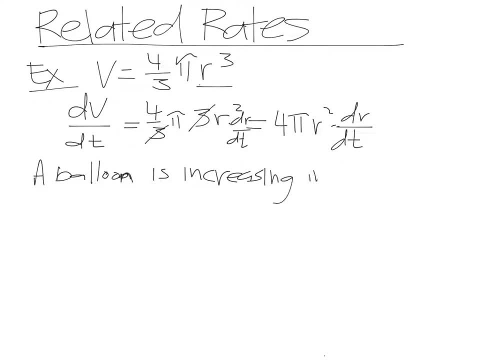 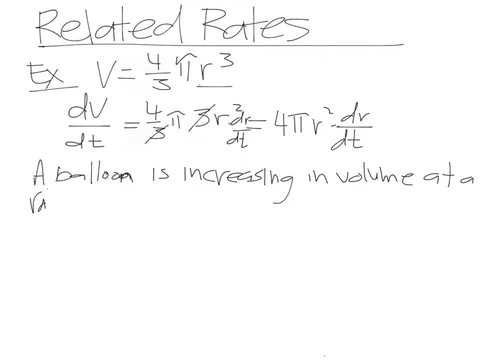 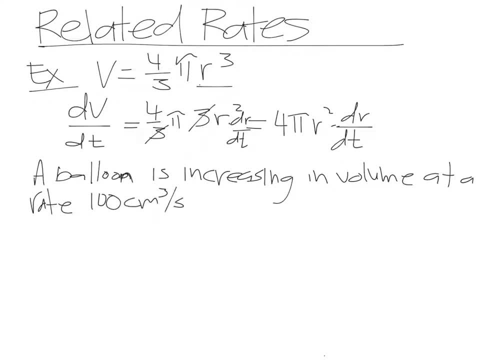 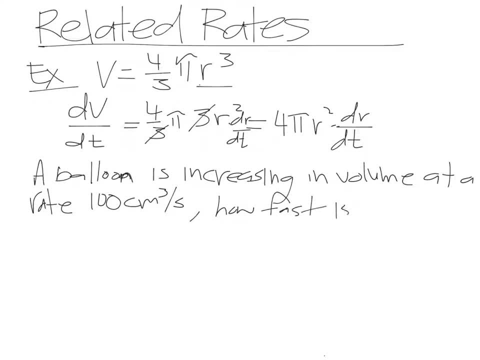 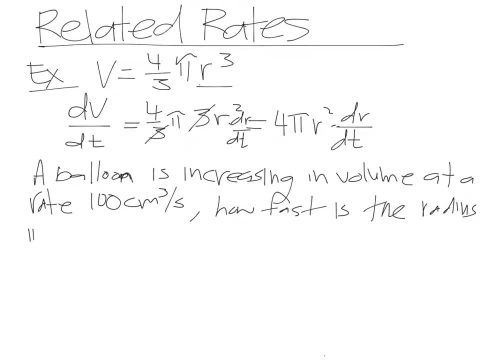 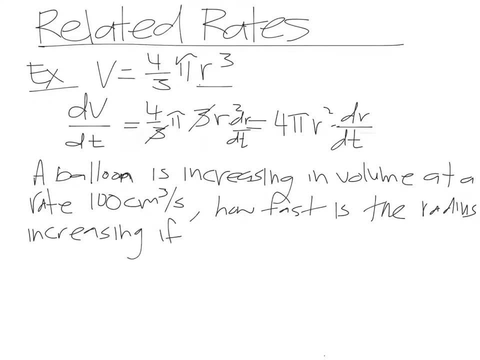 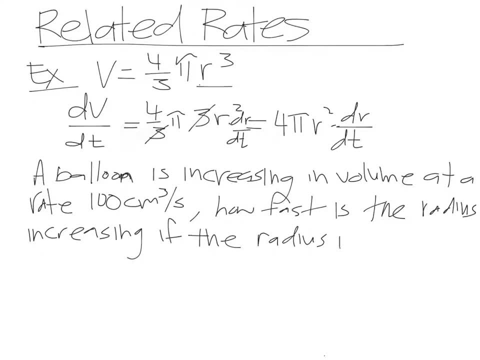 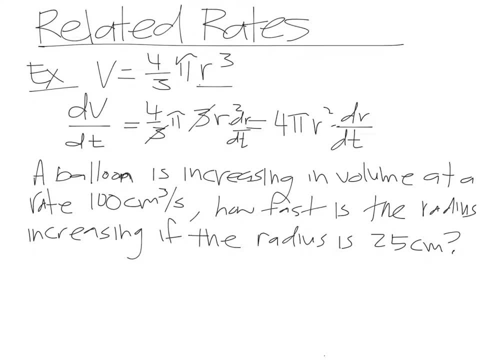 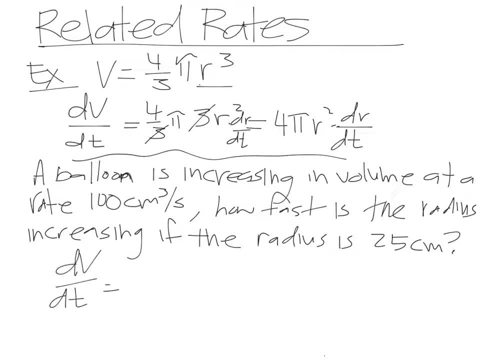 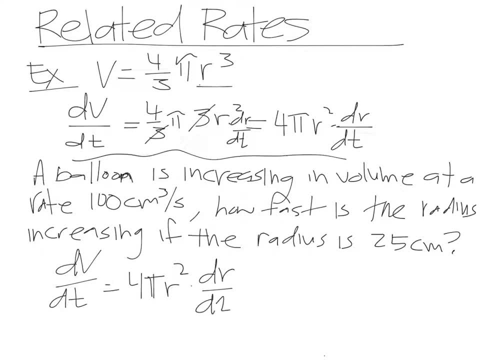 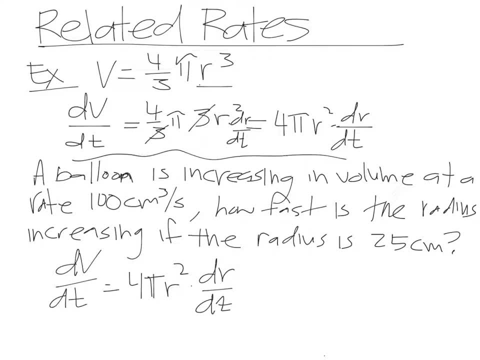 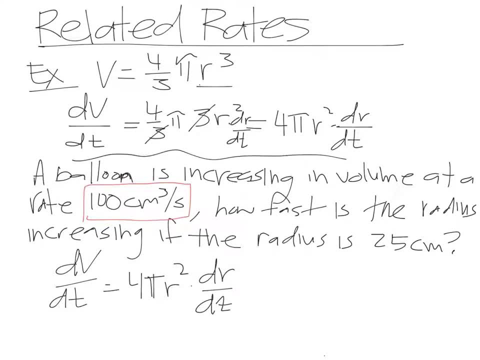 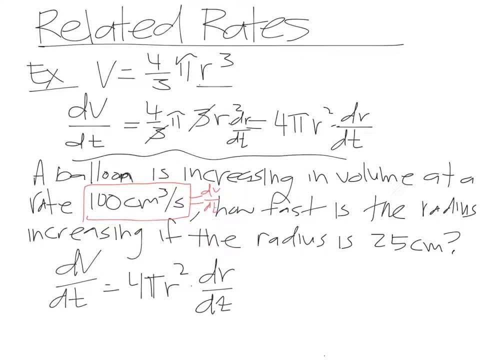 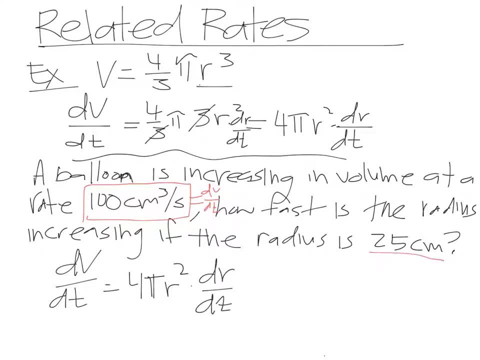 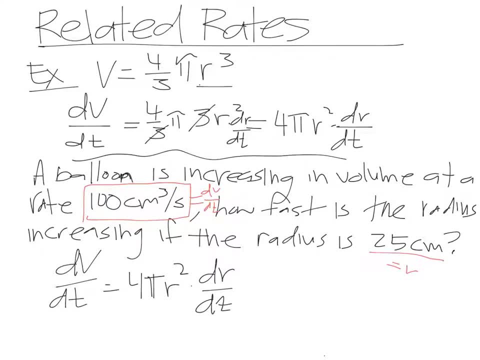 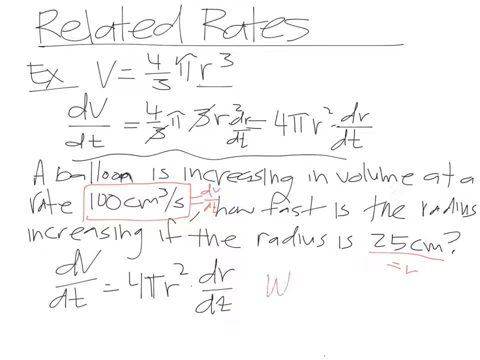 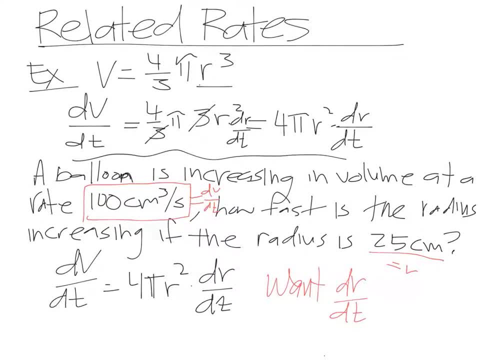 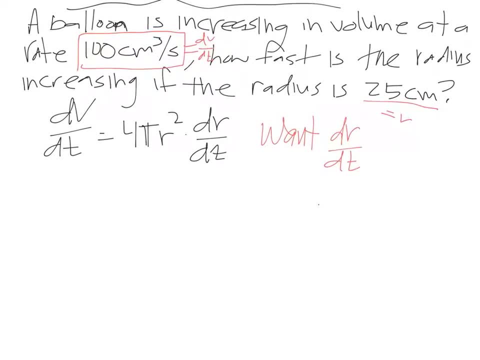 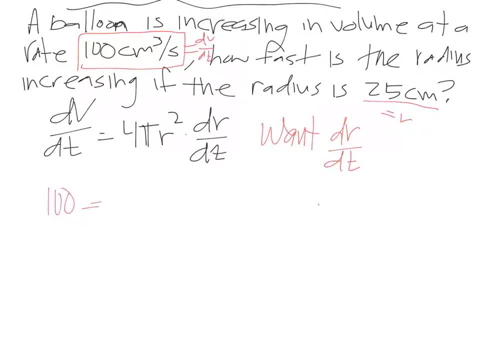 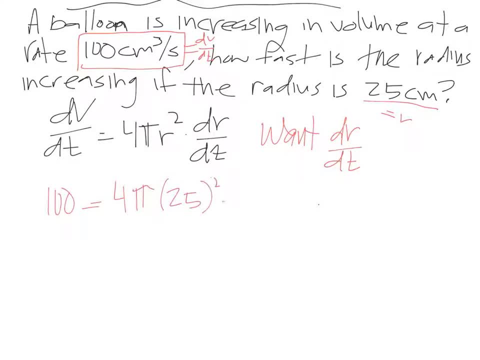 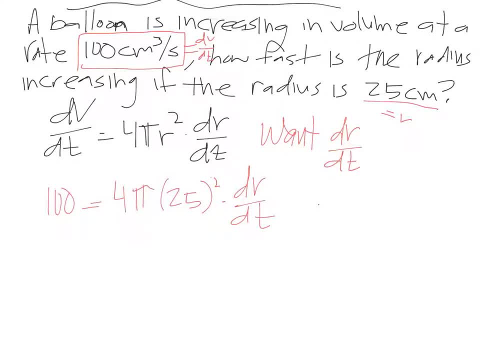 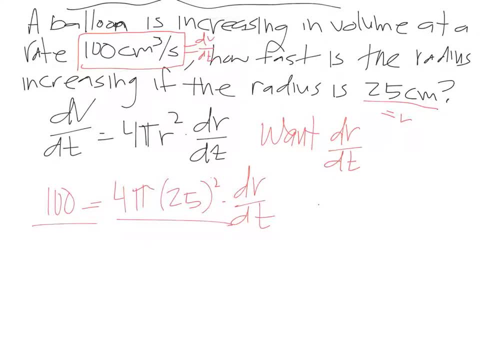 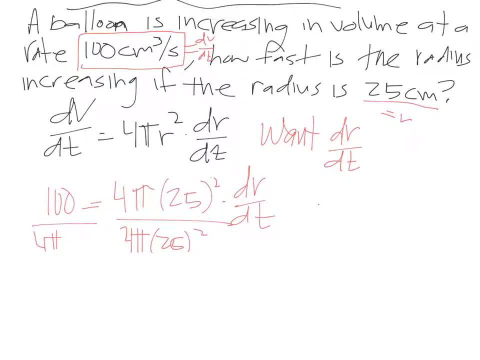 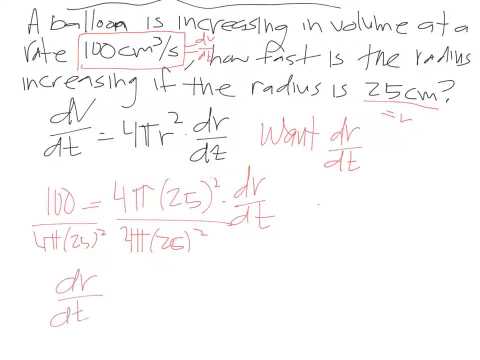 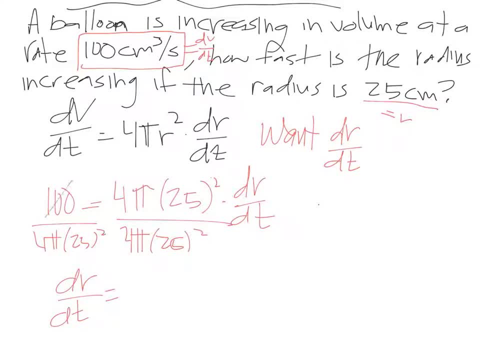 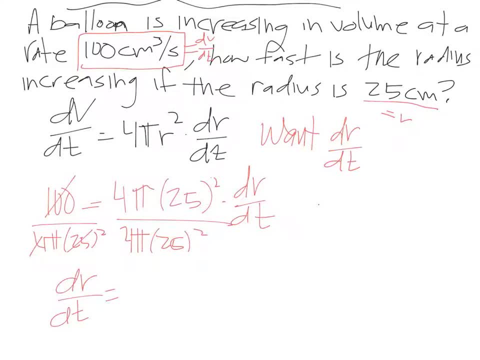 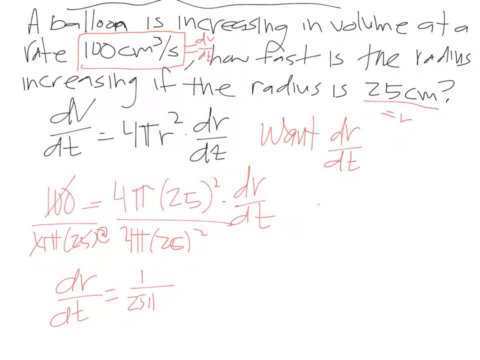 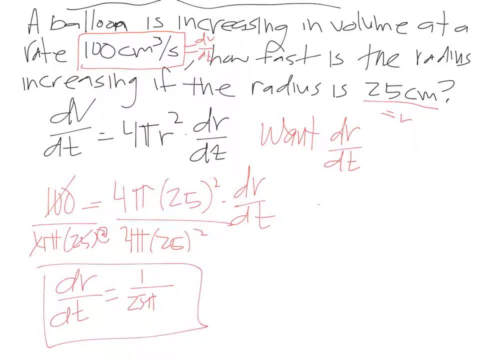 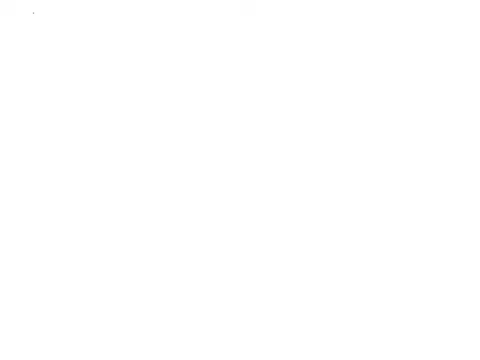 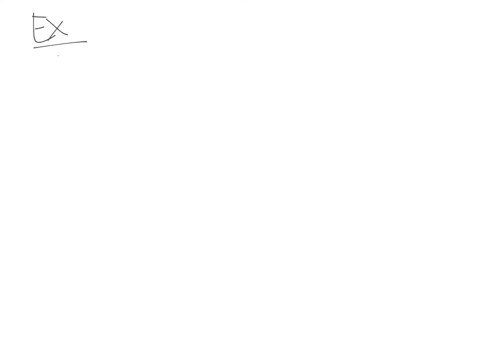 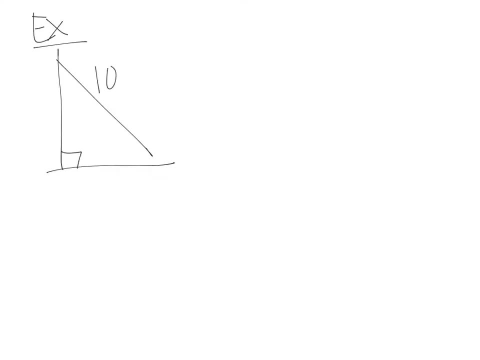 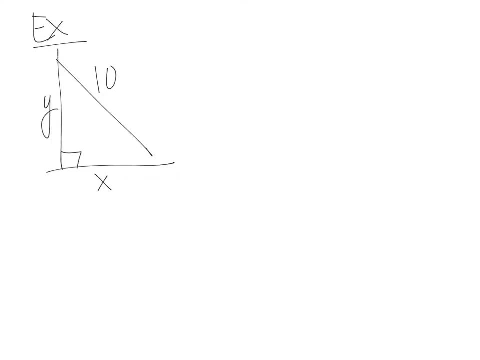 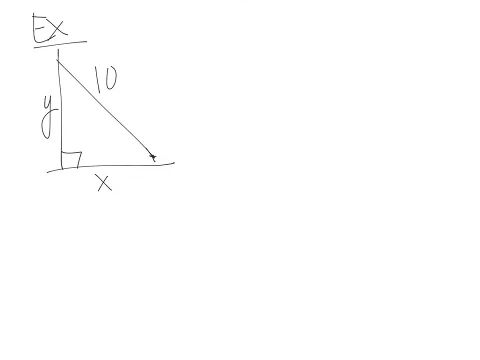 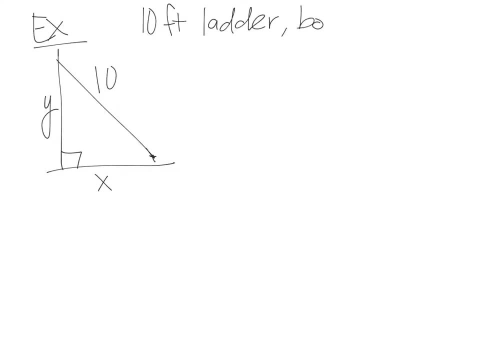 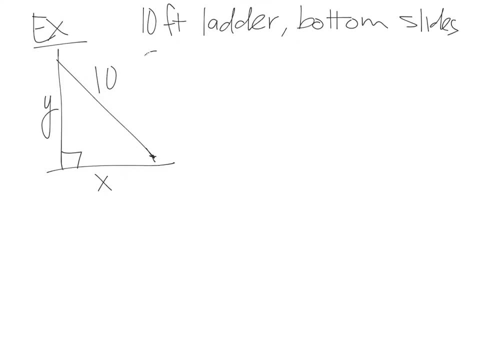 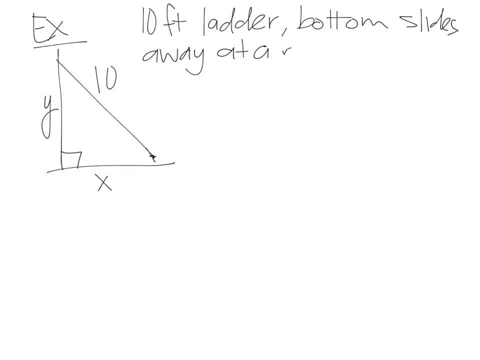 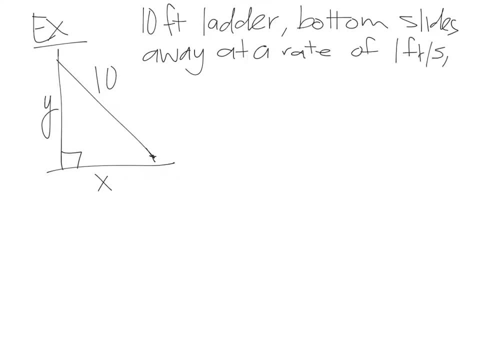 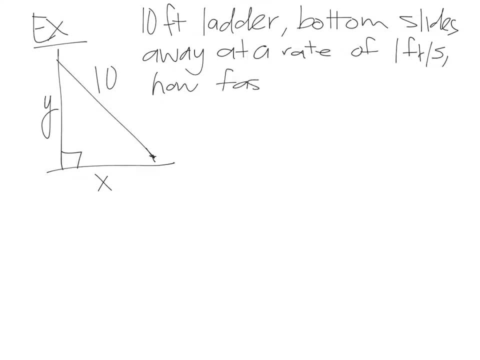 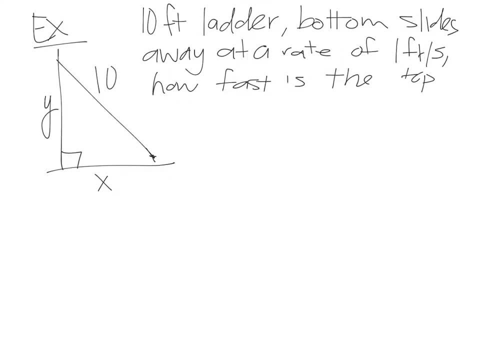 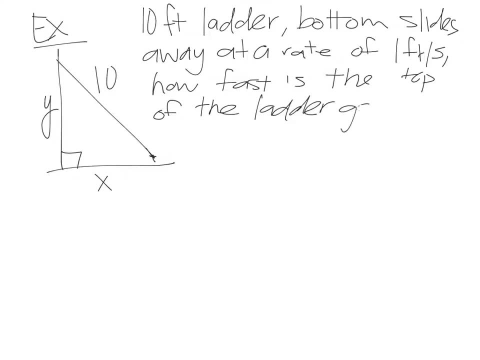 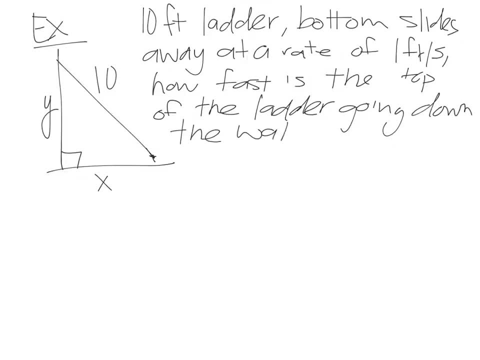 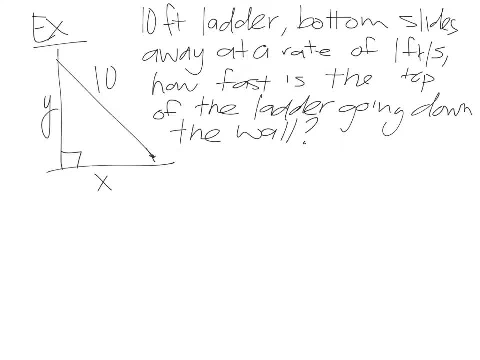 Subtitles by the Amaraorg community. Subtitles by the Amaraorg community. ladders going down the wall. in this case we don't have a nice equation like we did for the volume of a sphere, but that's alright. what do we have here? we? 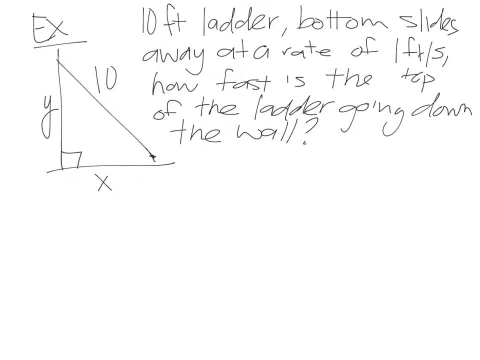 have a right triangle, so we can relate all the sides using the Pythagorean theorem, and that says that x squared plus y squared equals the hypotenuse squared, which is 10 squared. and now what are the pieces of information that we're given? it's going away from the wall at a rate of one foot per second. so 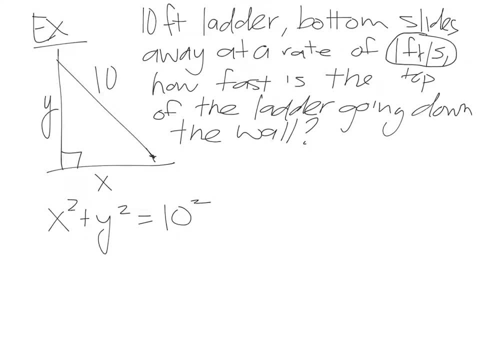 if it's going away. that's your X direction and the rate is changing. so this is your DX, DX, DT. and what are you trying to find? you're trying to find something and you're gonna try to find some data. so we're going to go here and 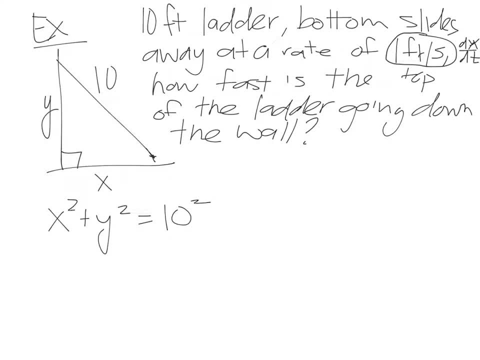 how fast is the ladder moving away from the wall? and so this is how fast the ladder is moving away from the wall. that would be, or moving down the wall, rather, that'd be your dy dt. and let's say we want to find this when we are six feet. 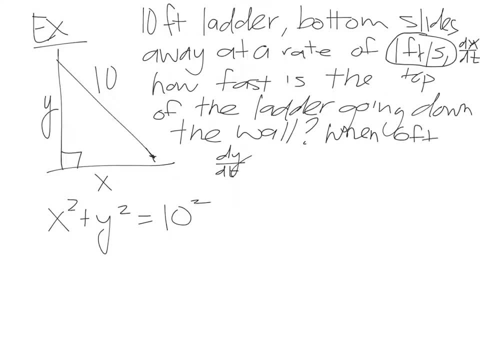 from the wall when we're six feet from the wall. so that's our X value. we want to find out when X, so that's where an X is six. so we can plug this in. first of all, let's take the derivative we're going to take. use the chain rule again. 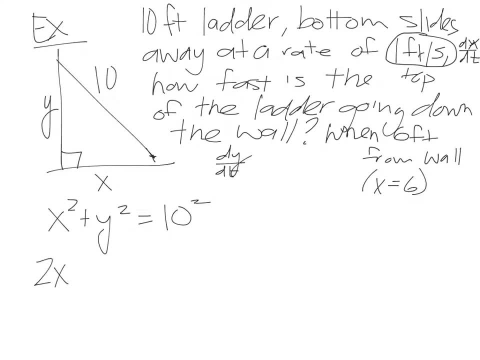 so we get 2x times the chain rule. DX DT plus 2y times dy dt is equal to. well, what's the derivative of 10 squared? or 100? since it's a constant number, that derivative is 0. so now plugging things in, we have to. our X value is 6, so 2 times 6 times dx dt, and we know dx dt is. 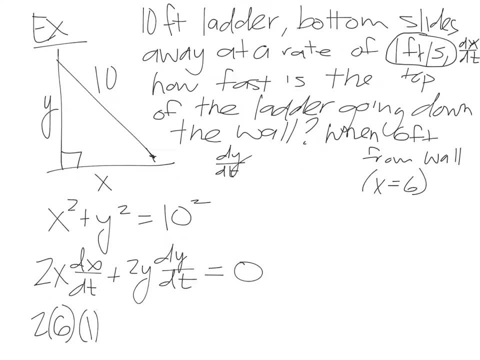 1 from up here plus 2. now, do we know our Y? no, we don't know our Y, but we can figure it out because of the Pythagorean theorem, if X is 6, we can figure out Y. so this is going to be 6 squared, because I was our X value plus Y squared is equal. 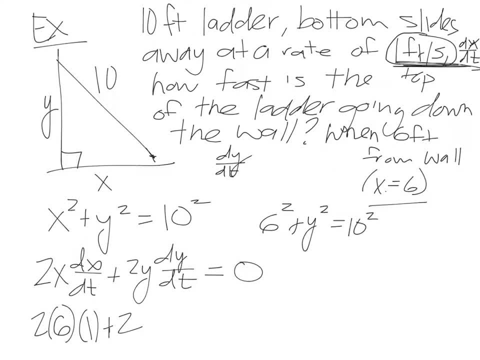 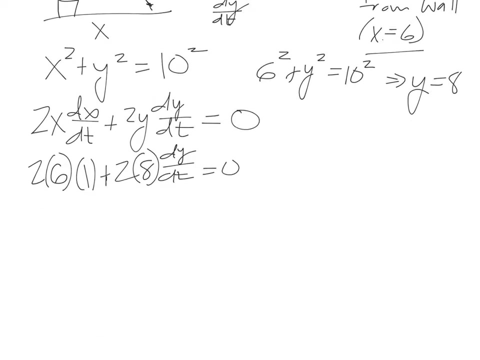 to 10 squared. now, solving this, or if you recognize this is a 3, 4 or 5 triangle, we end up with: Y is equal to 8, so this can be 2 times 8 times dy, dt equals 0, and so what we get is we get. 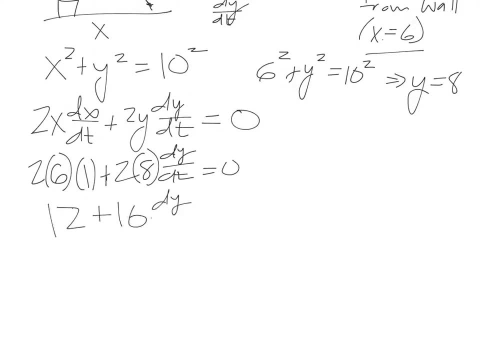 12 plus 16 dy dt equals 0. moving things around, we get that your dy dt is equal to negative 3 over 4 feet per second and that makes sense that there's a negative because you're moving downwards, your y value is increasing, is decreasing. that's our answer. 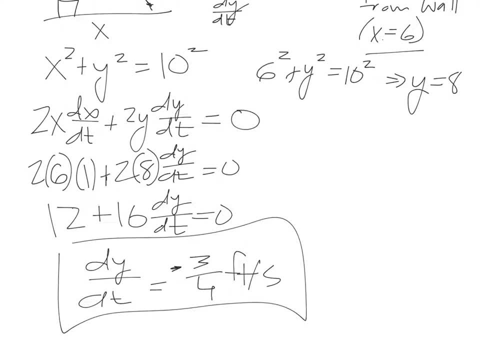 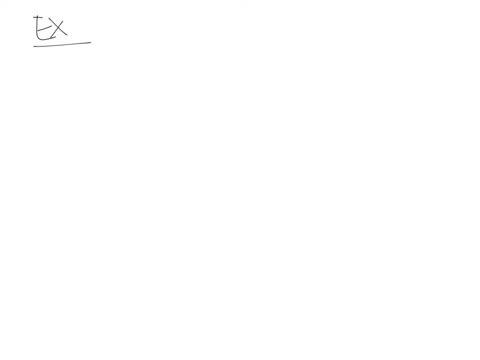 now let's see: we have water going into a tank that's in the shape of an inverted cone, so it looks something like this. so, so and so, given this, and we have water going into the tank at a rate of 9 cubic feet per minute. so, as it's going into 9 cubic feet per minute, and this tank, it has a height of 10 feet and the base of the radius is going to be 5 feet, so this tank right here is 10 feet tall. so 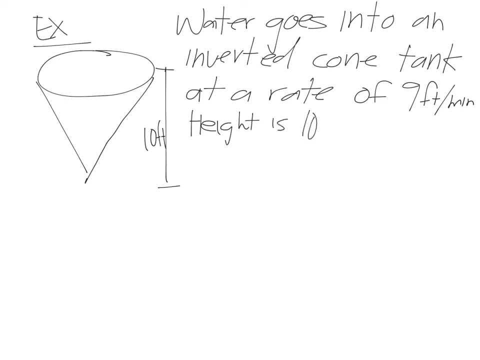 the height is 10 feet and then the the radius at the base that's going to be 5 feet. so right here, that radius is 5 feet. so if we add water to it, you know water micrometer come up at this level. it might not be all the way up, but the tank itself is 10 feet tall and has a radius of 5 feet. what I want to know is: how fast is the water rising? 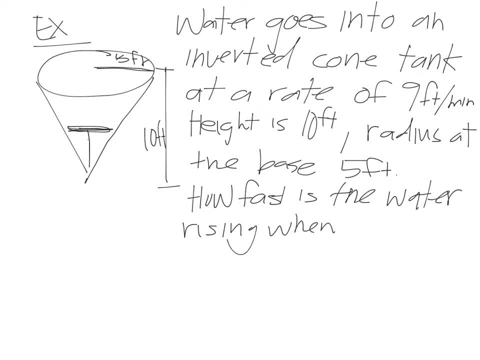 when the water in the tank is 6 feet deep. so if, when this height is going to be 6 feet, how high is the water changing? well, we need to do a couple of things here. first of all, what's the volume? what's the equation for the volume of a cylinder? that equation is going to be: v is equal to one third pi times your radius squared times your height, and so we'll let the radius be our b- x and then we'll let the height be y. so volume is one third pi times x times y. now, unlike the other problems that we have, that based on the ret704 data, we can add one. 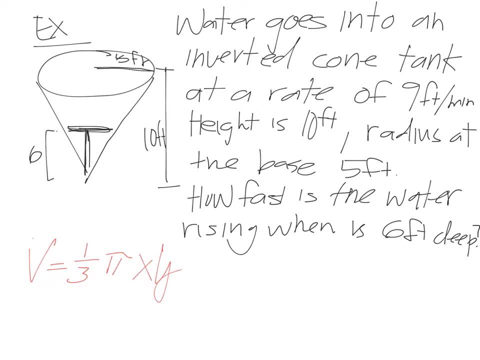 did? we only had two variables. we had V, and then we had something else. we didn't have X and Y. we didn't have V, X and Y, we only want two. is there a way that we can reduce this to just two variables? well, if you take a look at this, we actually 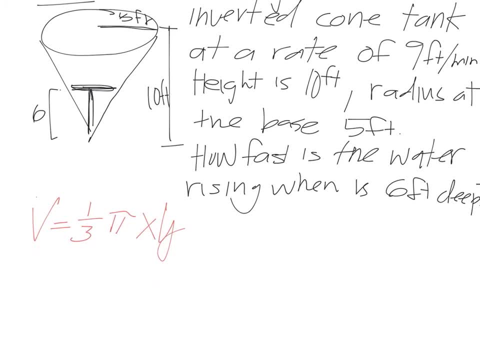 can, and this is by using similar triangles. so, taking a look at the triangles, we have one triangle like this, with a height of 10 and a radius of 5. if we look at the other triangle and we had some height, let's say Y- then we could. 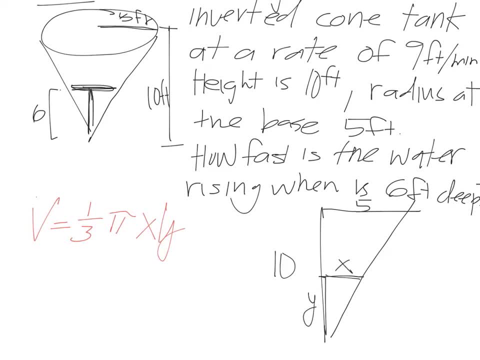 figure out that the X value or the radius would be some X value, and so, looking at these ratios, what we have is X over Y is equal to 5 over 10, or if we solve for X, X is equal to Y over 2, and so now we can actually plug this in for X, so the volume can now. 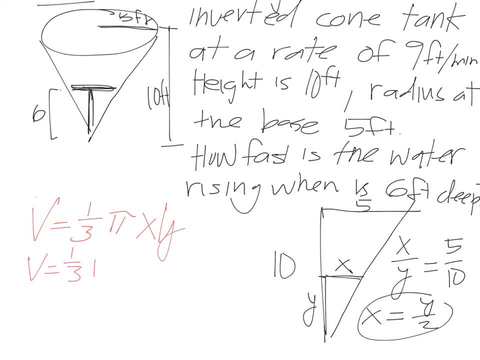 be expressed as one-third pi times. instead of X is going to be Y over 2 times Y, or in other words- excuse me, they should be: X squared the volume is one-third pi, the radius squared which. so this: this is really the area of a circle, so this: 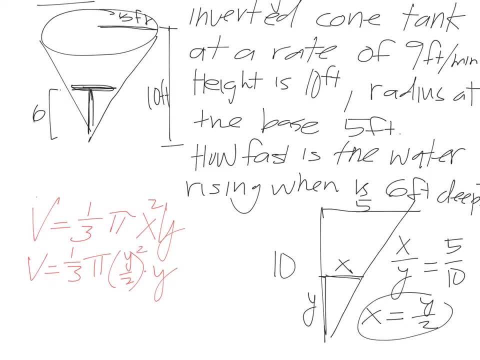 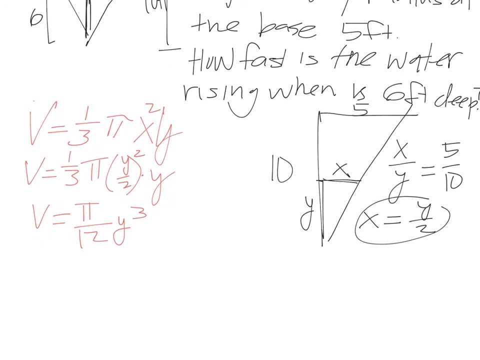 should be a squared right there. Okay, so volume is one-third pi times y over 2 quantity squared times y, Or volume is equal to pi over 12 times y cubed. And now we can calculate. finish this equation, or this problem. 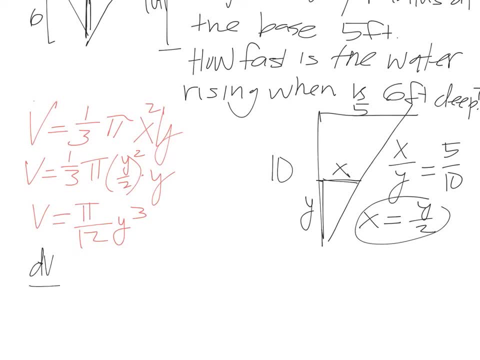 So, taking the derivative, we get dv dt is equal to pi over 12 times 3y squared. we're using the chain rule: times dy dt, Our 3 and our 12 cancel. So this is really pi over 4, y squared dy dt. 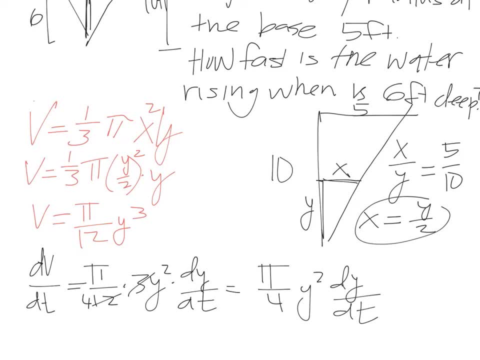 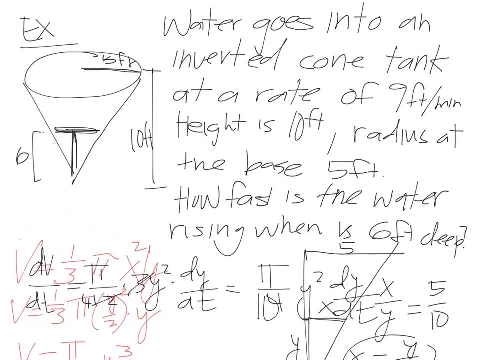 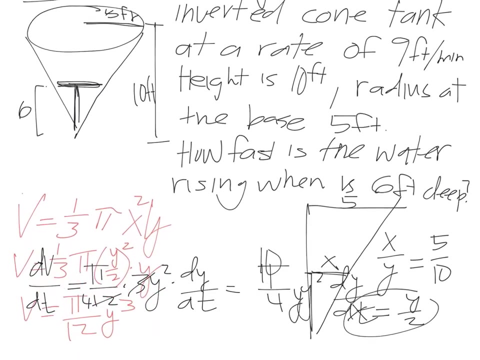 So if we look back at what the original question was stating, and that was we had water going in at a rate of 9 feet per minute, Then that should be cubic feet per minute, And we wanted to find when it was 6 feet deep. 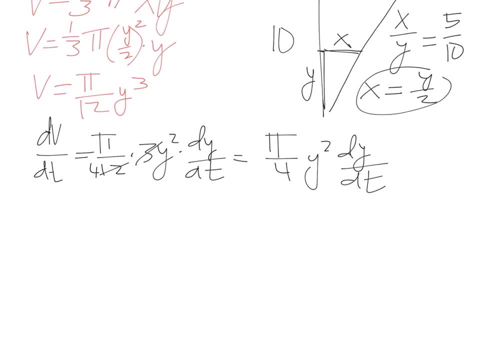 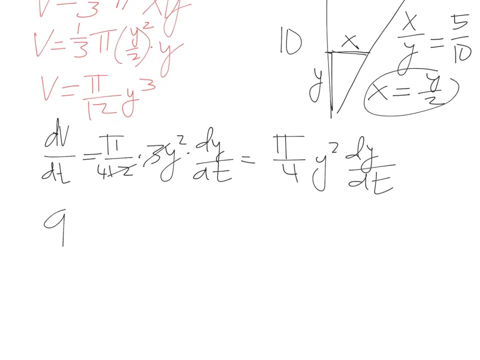 So that was when y is 6 feet, We'll have the following: So the change in volume, what was coming in, was 9.. So this should be 9, equals pi over 4, times the change in volume. 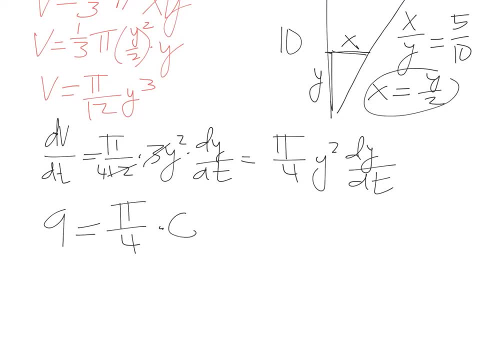 height, which was 6 squared times dy dt. 6 squared is 36 divided by 4. that, right there, simplifies to 9 and our 9s will now cancel. so we have 9 over here and 9 over here and they cancel. so we have: 1 is equal to pi times dy dt, solving for: 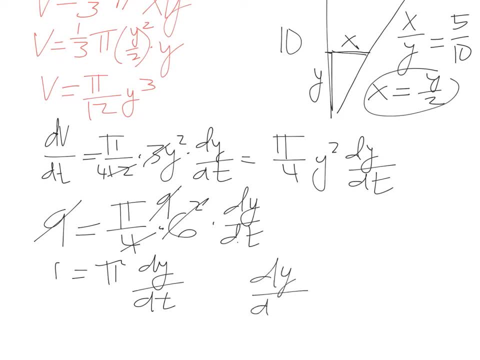 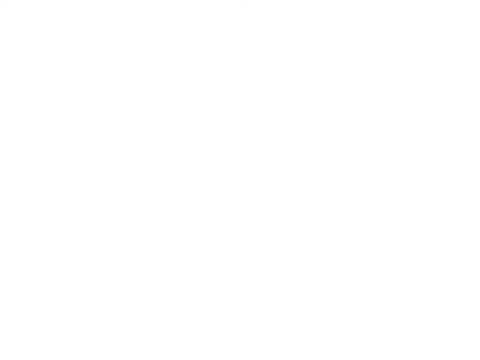 dy, dt we get that is just 1 over pi and then the rate- the units rather- is feet per minute. so there's a couple of strategies that we can use when dealing with these types of equations. the problems: the first is to read the problem carefully. the second thing: it really helps to draw a diagram, and this is: 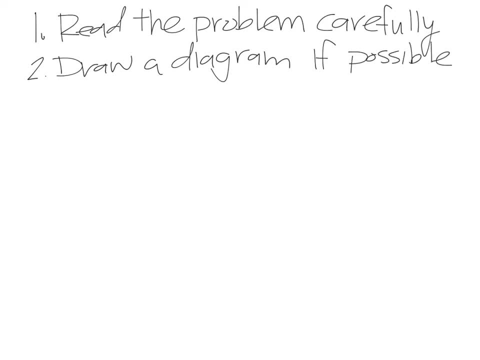 possible. The third thing is to introduce notation. So in the problems that we gave they didn't say dy dt is equal to so-and-so or solve for dx dt. They just said how? what is the? the change of height chain um the rate of the change. 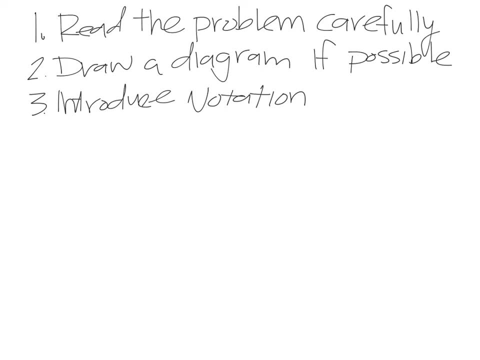 in height, and so we have to introduce our own notation to do that. So, introduce your notation, and then you assign symbols to all quantities that are functions of time. Then the next thing we do is we express the given information and the required information, or rather the required rate in terms of derivative. 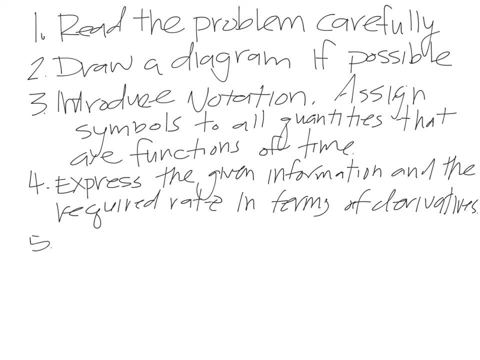 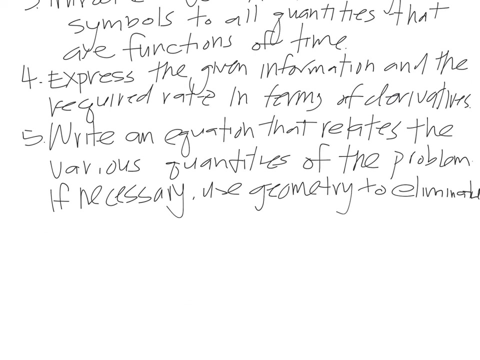 The fifth thing is to write an equation that relates the various quantities of the problem and, if necessary, use geometry to eliminate. to eliminate one of the variables, to eliminate one of the variables by substitution, and that's what we did in the last example. we had three things and we could substitute. we 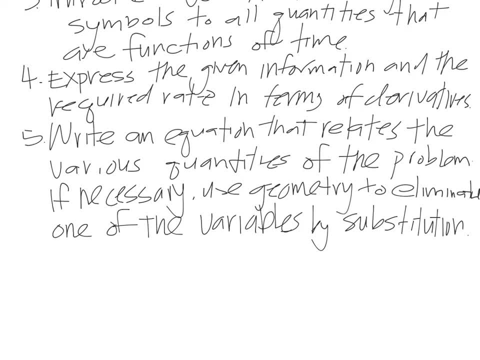 had v, x and y and when we found the ratio we could eliminate our x variable by substituting x was y over 2.. Number six: use the chain rule. Okay, we use the chain rule to differentiate both sides of the equation with respect to a certain function. 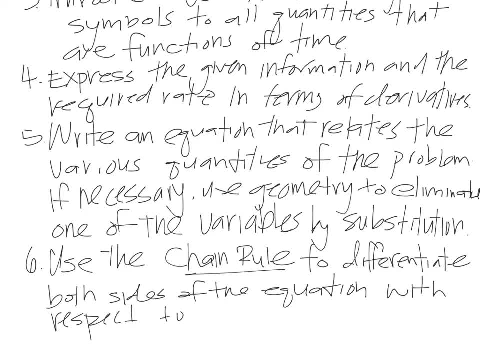 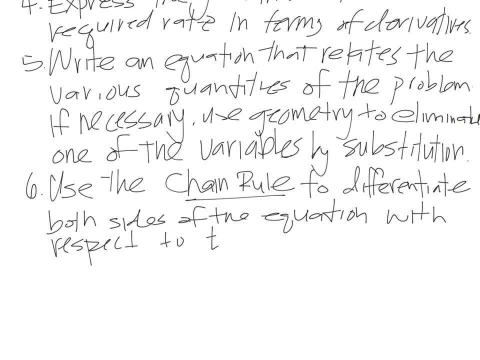 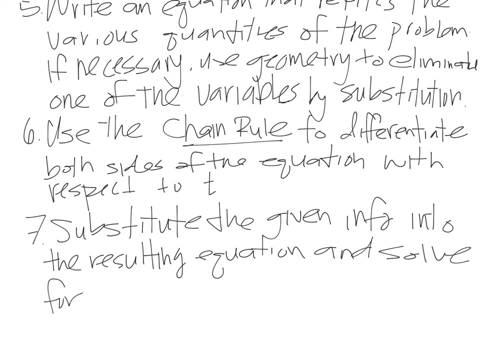 to our variable t and the last step for solving these types of problems. 7- substitute the given information into the resulting equation. 7- substitute the given information into the resulting equation and solve for the unknown rate, and so these steps will help you with your problem solving. on related rates. 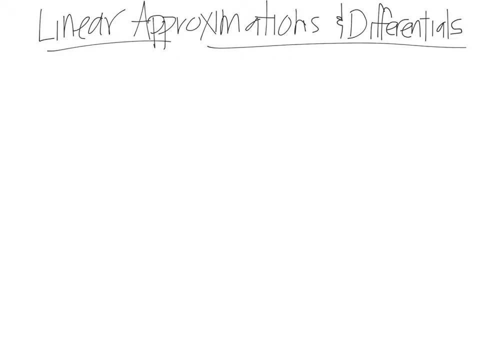 now today we're going to talk about linear approximations and differentials. now, if you recall, given some sort of curve like this, and this is the curve- y is equal to f of x, the tangent line at some point right over here, at some point a. so we'll say this is a comma f of a. 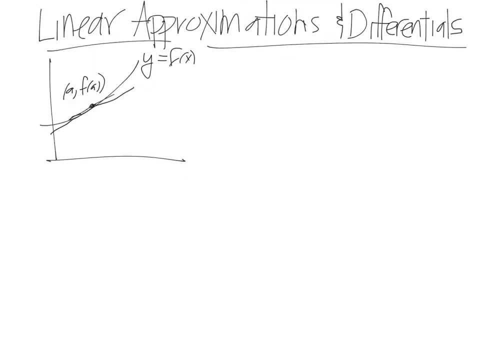 the tangent line is going to go right through the tangent line and it's going to go right through that and have the same slope. so the tangent line y is equal to- let's call this- l of x. now the point of this is that we might be able to calculate what f of a is. 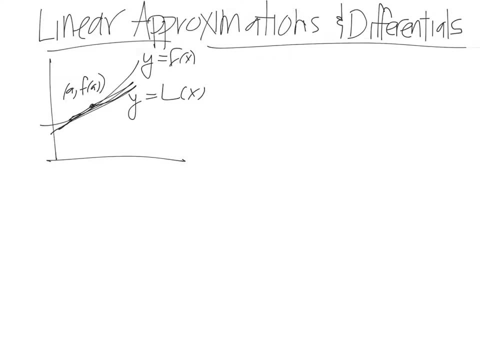 but we might not be able to calculate, or it might be very hard to figure out, what f of x is when x is really near a, and so what we can do is use this tangent line to help us approximate it, because the tangent line near when x is a. 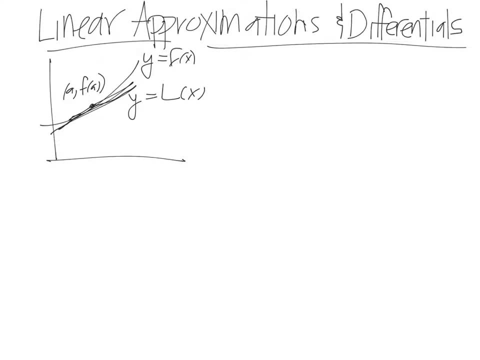 is a pretty good approximation to the curve. y equals f of x. so if you see, when we're here we're pretty close. as we get further away there's more of an error to where the y value is. but nearby it should be pretty close. but nearby it should be pretty close. 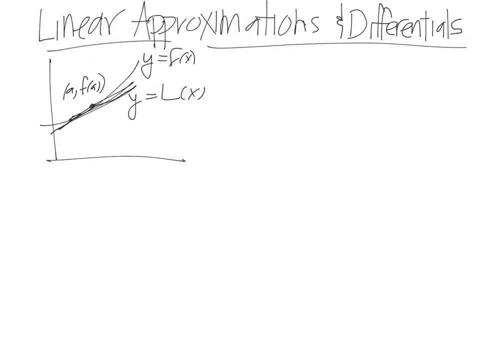 now, if you remember the equation of a line using the point slope formula, that is, y minus y1 is equal to m times the quantity x minus x1. if we move our y1 over, we have the equation: y is equal to y1 plus m times. 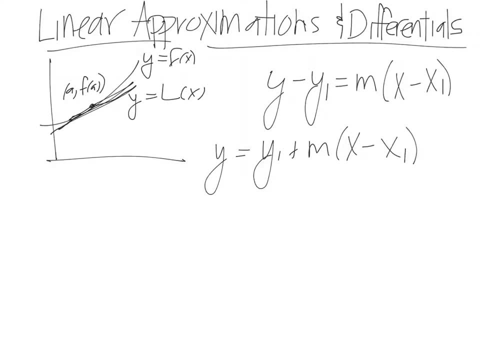 x minus x1. and this is, if we have some point x, x1, comma y1 and we have a slope that's going to be m. now, if the point that we have is this, point a, comma f of a, what we can do is our y1 value. 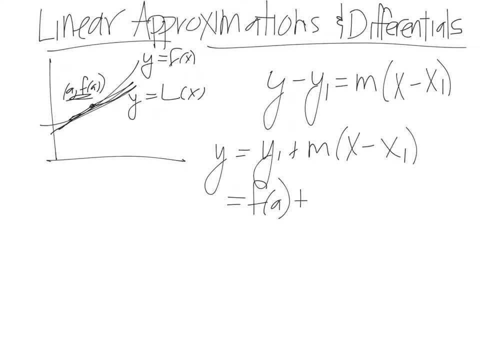 is f of a, and then our x1 value is our a. and what's the slope at that point? well, the slope is the derivative, so it's going to be f prime at a. so we have f of a plus f prime of a times the quantity. 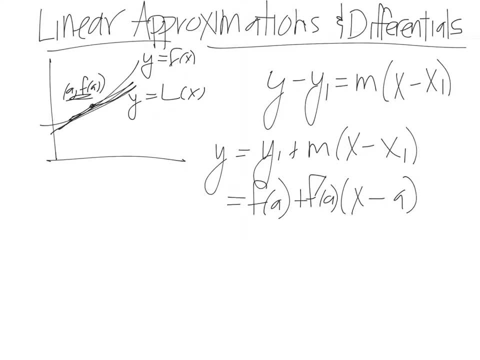 x minus a, and that is what our rather. that's going to be an approximation for f of x, for f of x, so let me rewrite that a little bit better. so the approximation, so the approximation f of x is approximately equal to some point f of a that we know. 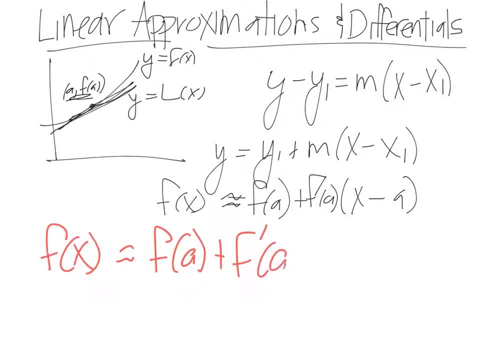 plus f, prime at a times, the quantity x minus a and again. to help you remember this formula rather than having to remember it from scratch, if you just think about the point slope formula, you'll be able to fill in the details. so this is what we call. 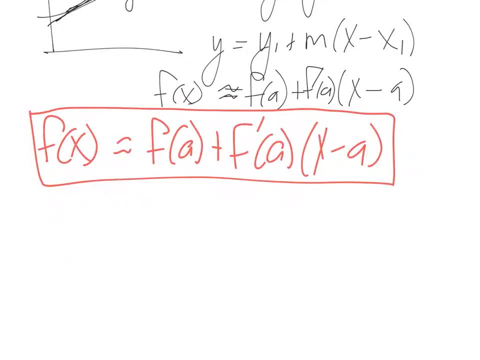 a linear approximation or the tangent line approximation. so this is the linear approximation or the tangent line approximation of f at the point a. and if we wrote: for the linear function, capital L of x is equal to f of a plus f, prime of a times the quantity. 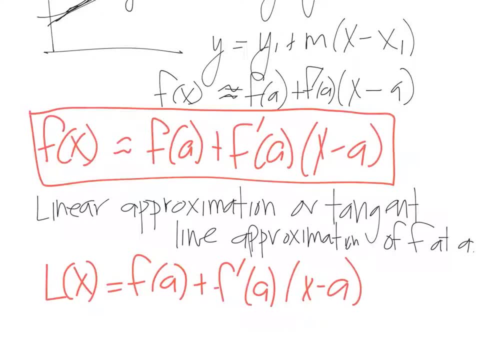 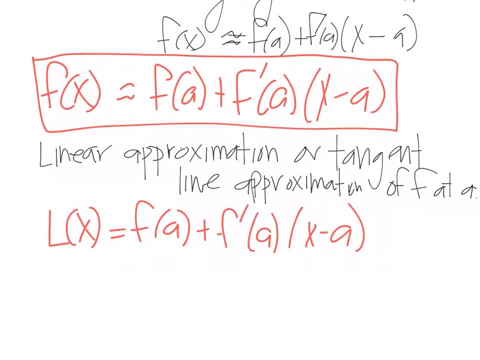 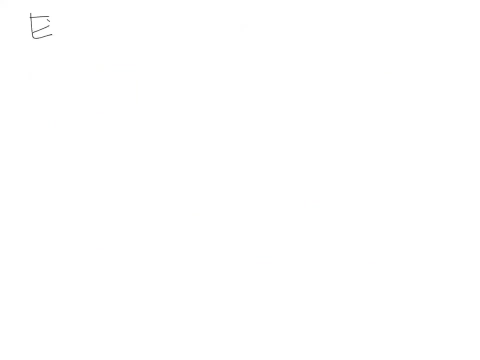 x minus a, and so, using this, this is what we call the linearization of f. at a point, x equals zero. so let's do an example. let's find the linearization of the function f of x is equal to the square root of one plus x. 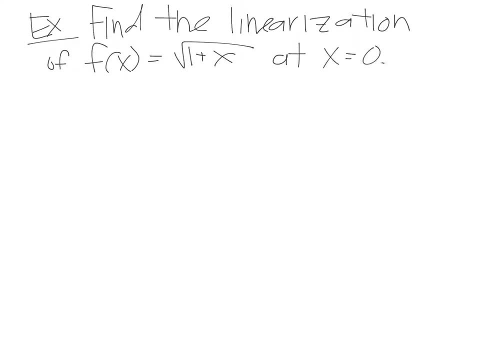 at the point x equals zero. so what we have here is a square root function and, yeah, we know some of the square roots, but do we know, for example, the square root of 1.2? well, we can approximate that using our linear approximation. so remember the formula. 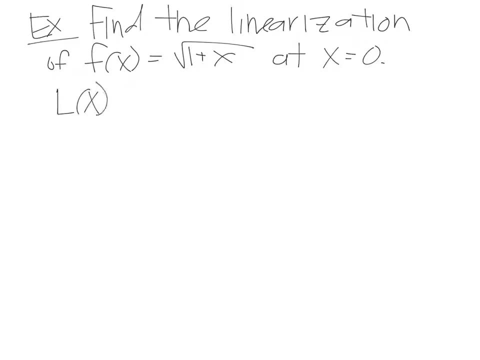 for the linear approximation L of x is equal to f of a plus f prime, at a times the quantity x minus a. so we're going to need this, but first of all, in order to do all that, we need to figure out certain things. so in this case, our a is zero. 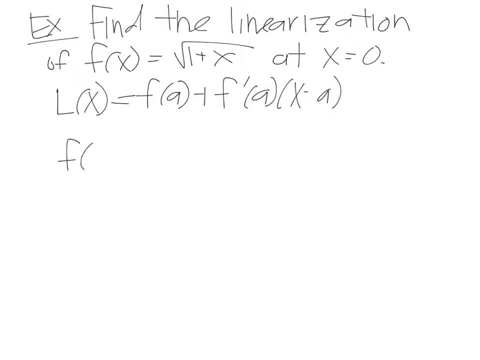 so we want to figure out what is f of zero. well, f of zero is going to be the square root of one plus zero, which is just one. and then we got to find the derivative, f prime at a or f prime of zero. so let's first figure out the derivative. 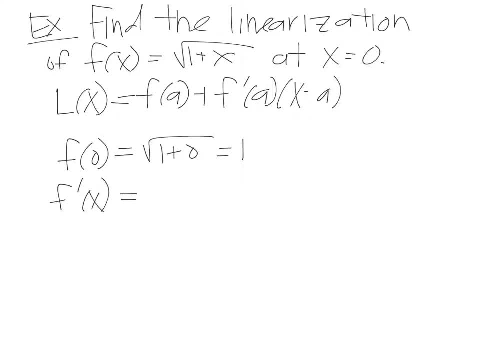 so the derivative of this- and remember our f of x, another way to write the square root- is one plus x to the power, one half. so this is going to be one half the quantity, one plus x to the negative, one half, or one over two times the square root. 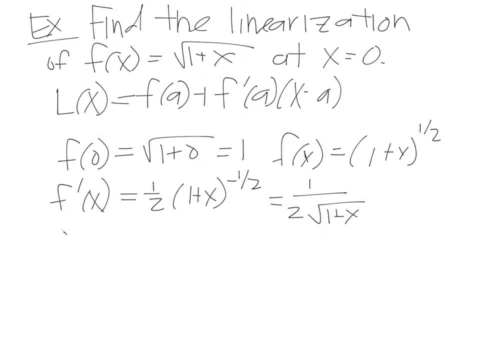 of one plus x and figuring out what this is, evaluating at zero our f prime at zero. this is one over two times the square root of one plus zero, or just simply one half. so now we have everything and we can plug it into the linearization and we get. 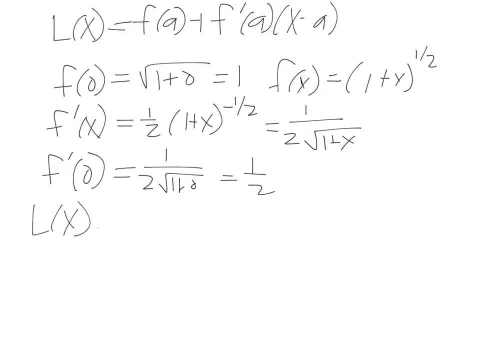 l of x is equal to f of zero plus f prime of zero times x minus zero. well, x minus zero, that's just x. so f prime of zero we get from right here is just one. so one plus f prime at zero. that's going to be right here. 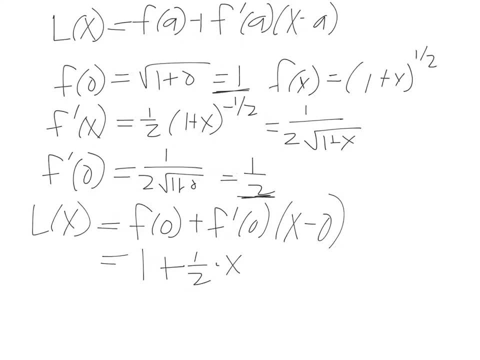 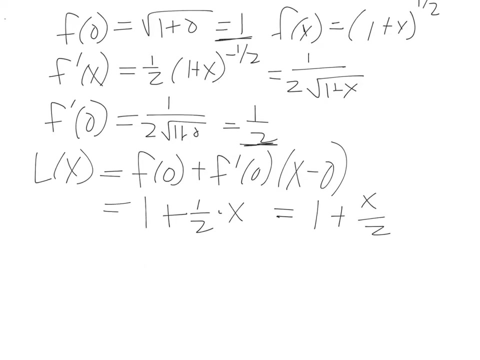 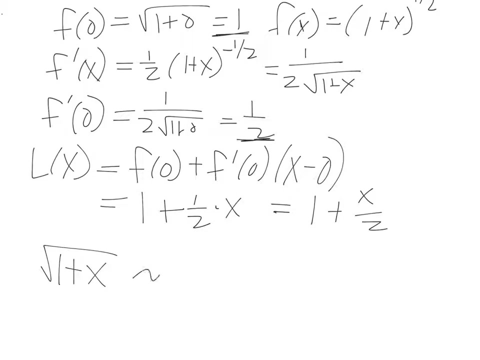 one half times x. so our linearization is just one plus x over two. so what this is saying? this is: the linear approximation for the square root of one plus x is approximately equal to one plus x over two. this is when x is near zero. so let's actually 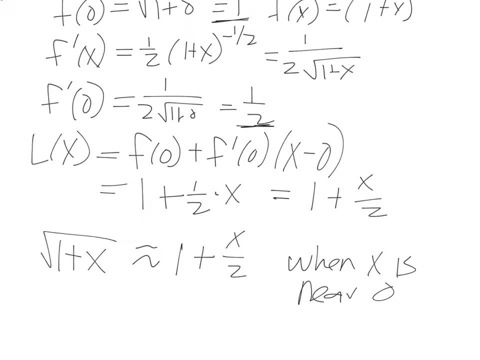 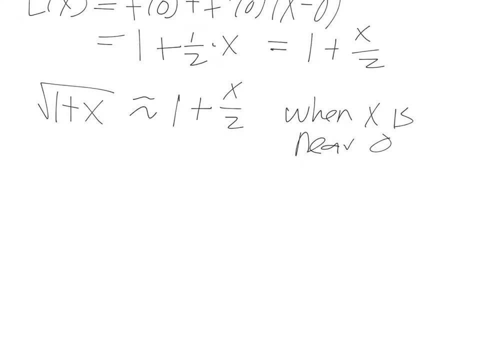 test this, let's see how accurate we are. so if we're, let's say, near zero, so, or when x is near zero, let's say when x is point two, so we're trying to find the square root of one plus zero, point two, which is the square root. 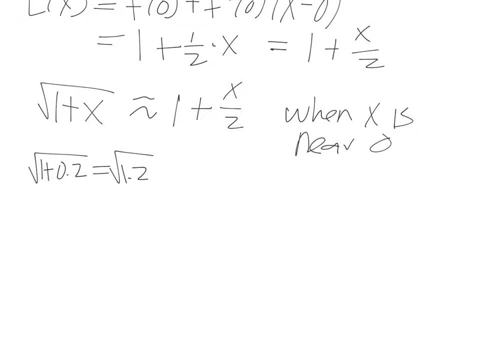 of one point two. now, according to the approximation- let me see if I can just move this down a little bit- there we go. so the approximation says the following approximation says that this should be one plus zero point two over two. that's what we said right here, in fact. 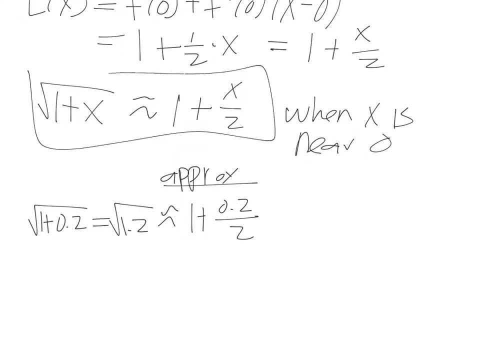 I'll box that. I'll box it right here. so this should be approximately one plus point two over two, and that is going to be one point one zero. now if you plug this in on your calculator, you find that the true value for this is one point. 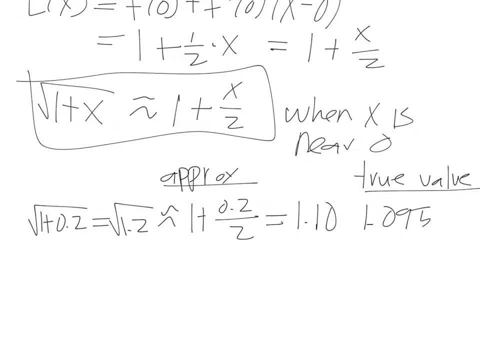 zero nine five four, four five. so we're close-ish. but let's see this really works well when we're near zero. so let's get a little bit closer to zero. let's say one plus zero point zero five. so we're taking the square root of one point zero five. 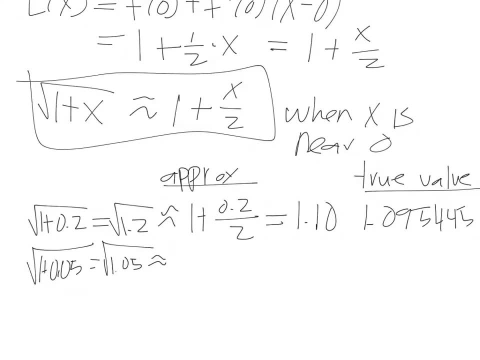 this is going to be, according to our linear approximation, one plus zero point zero, five over two, which gives us one point zero, two, five. and if we plug this on our calculator, what do we get? we get one point zero, two, four, six, nine, five. that's closer to the true value. 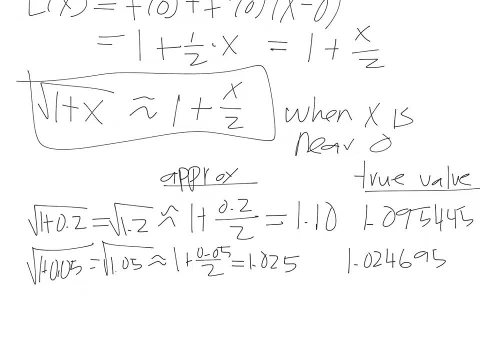 let's see if we can get better, let's get even closer to zero. so we're going to see one plus zero point zero, zero five. okay, so that's going to be one point zero zero five, which is approximately equal to one plus zero point zero zero five. 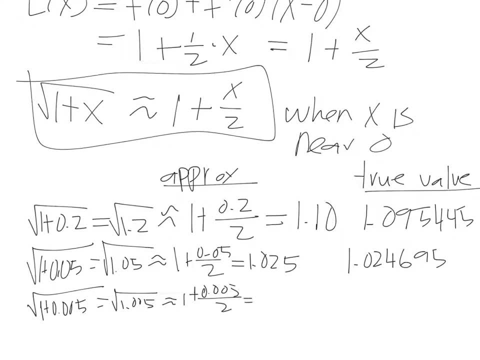 all over two and according to the linear approximation we get, this is one point zero, zero, two, five, zero. but the true value, if you use a calculator, this is one point zero, zero, two, four, nine, seven. we're getting closer and closer to the true value, the closer and closer. 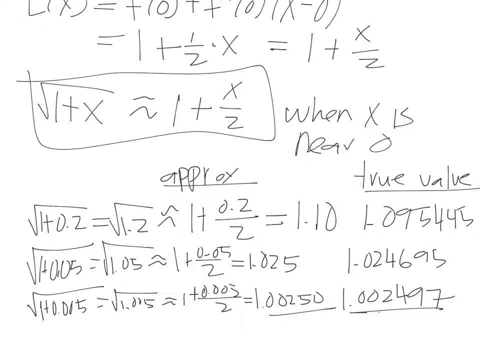 we get to zero, the closer that this number gets to zero. but this is just our linear approximation and that's what we use it for. we know how to take the square root of certain numbers, like when x is zero, and we can use that to find other values. 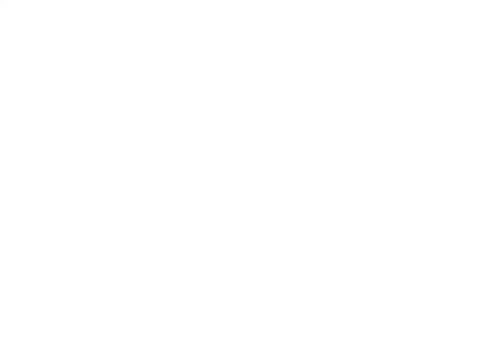 so if I said: find the linear approximation of f of x equals the square root of one plus x at the point x equals three, what we can do is the following: so three is really our a, and so we we want to find l of x at the point a equals. 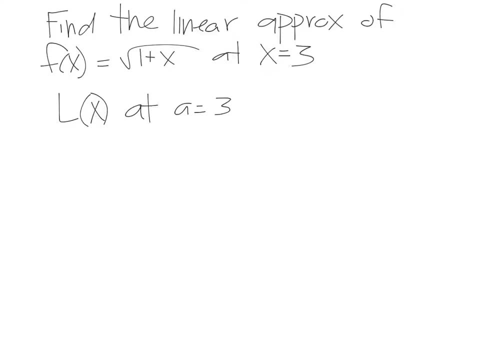 three. well, we need a couple of things. we need to figure out what is f of three. well, f of three is the square root of one plus three, which is the square root of four, or just two. we need to compute the derivative, and so we know the derivative over here. 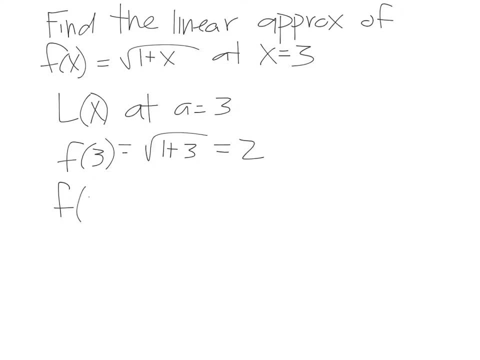 is going to be the derivative at three of f. remember we calculated the derivative on the other slide, so that was one over two times the square root of one plus a, so one plus three, and so this is going to be one fourth, so the linearization of x. 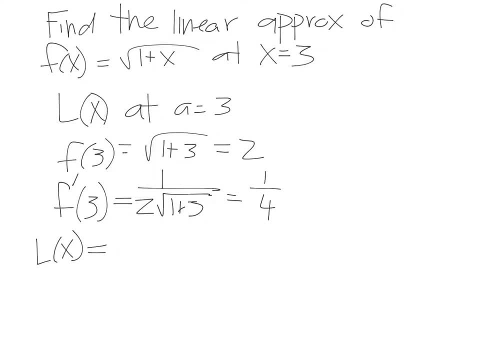 is going to be. remember l of x is going to be f of a plus f, prime of a times x minus a. so we get: l of x is f of a, which is two from right here, plus the derivative, which is going to be one. fourth times, 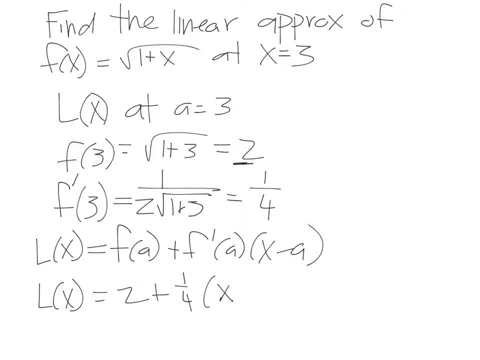 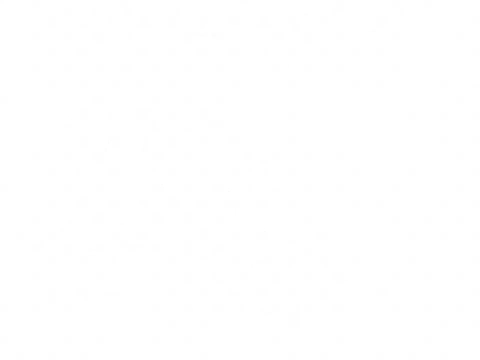 x minus a times x minus three. so that's our approximation, which, using some simplification, ends up being five fourths plus x over four. now we're going to show how to shift gears and talk about differentials. so let y equals f of x, and let this be. 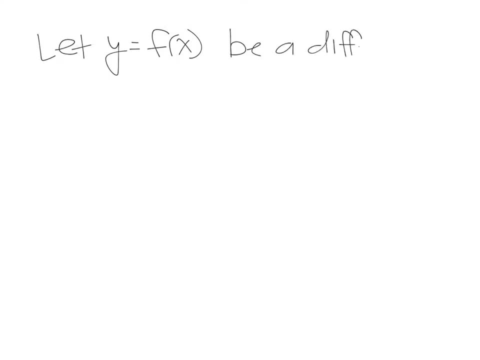 a differentiable function, then we say that the differential and the differential dx, this differential is an independent variable. and then we say that the differential dy, that is going to be a dependent variable. so the differential dy is a dependent variable, and so this is defined as the following: 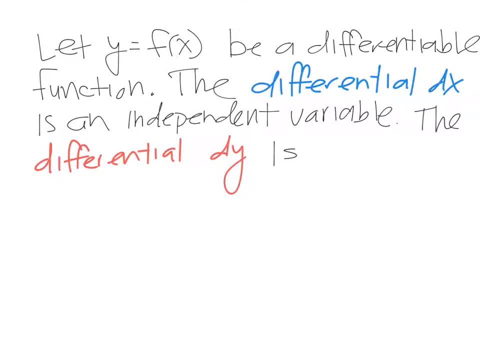 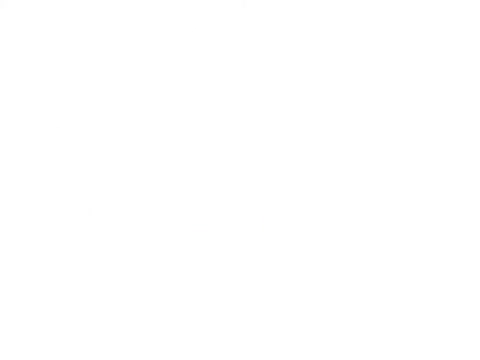 we're going to define it to be dependent, so it's going to have some sort of dx in it. so the derivative f prime times dx and that's why it's dependent, because it depends on whatever the x value is now geometrically what this looks like. 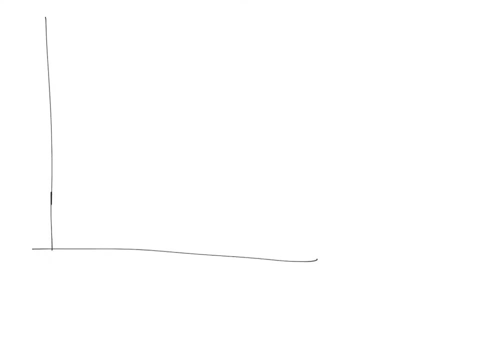 is the following: so if we have our curve, that's the curve y equals f of x, we have some point right here. we'll say that that point is p, and so that point corresponds to some x value, and then we're going to add some delta x to it. so this point 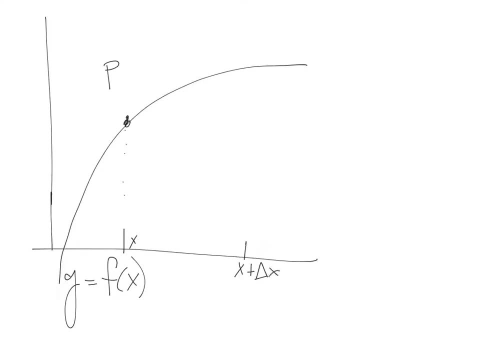 right here would be x plus delta x, go up to here and at some distance, delta x. we're right here. but if we approximated it at p and we had some linear approximation, or even the tangent line, as you may, it goes like that and it doesn't quite fit. 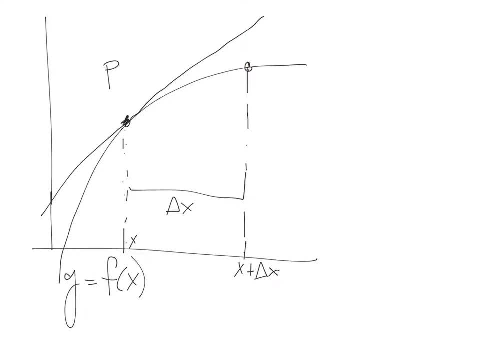 we have this error right there. so if we extended this all the way up and we call this our point r and we call this intersection q, then what we would have- and we'll maybe extend this over here, we'll call this the point s- so this distance that we have, 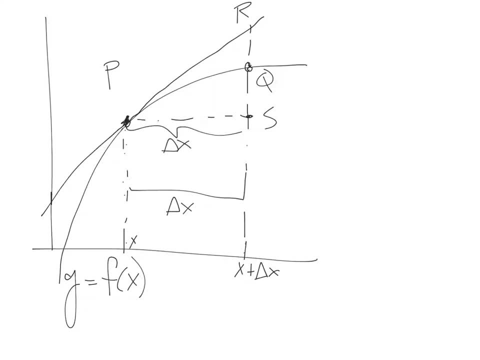 right. here is delta x, our change in the y value. this would be our delta y. now, if we're using differentials, our dx is going to be the same as our delta x, but if we're looking up here this big change in y that is dy. 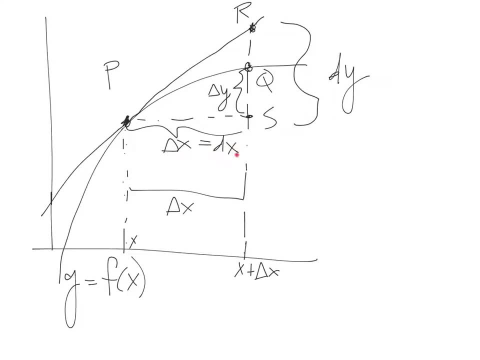 so our delta x is the same as dx, but our delta y is right here, and then the dy adds all this extra stuff up there. so if we were to express this in terms of an equation, what we get is: delta y is equal to f of x plus. 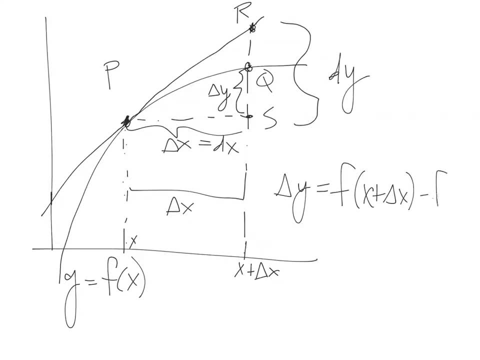 delta x minus f of x. so that's how we can get our delta y. it's just the y value right here: f of x plus delta x minus this height, which happens to be the same as f of x. now we know this is the slope, and so we know. 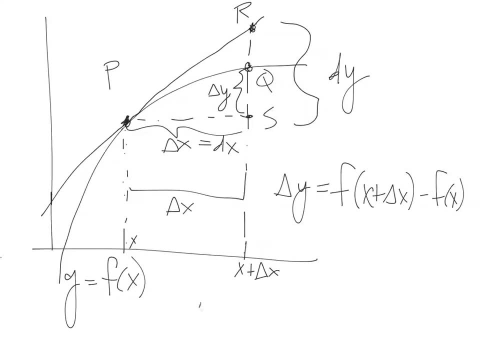 slope is rise over run. so the slope f prime of x is rise dy, dx, d, rise dy over dx, which means that rearranging this, we get dy is equal to our slope f prime of x times dx. and so here we have two equations that we can use for differentials. 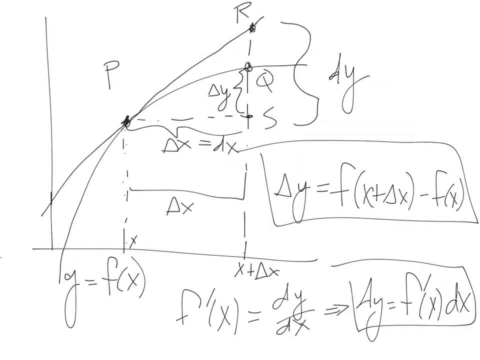 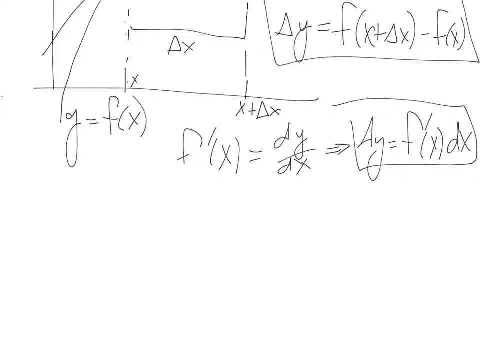 so I know this may seem confusing, so we're going to do an example using these two equations. I should probably have highlighted them, but I'll just underline them in a different color. ok, so example: we're going to compare our delta y and our dy if we're given. 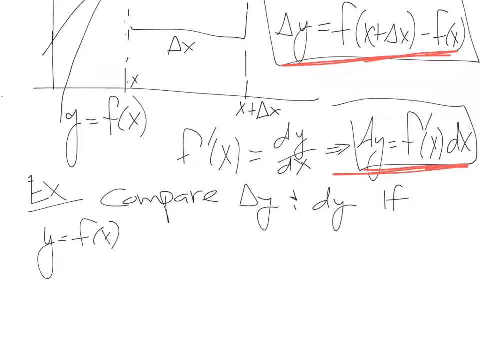 y equals f of x, which is the function x cubed plus x squared, minus 2x plus 1, and we're given that x changes from 2 to 2.05. so take a look at this equation, these two equations. I'm going to move the screen. 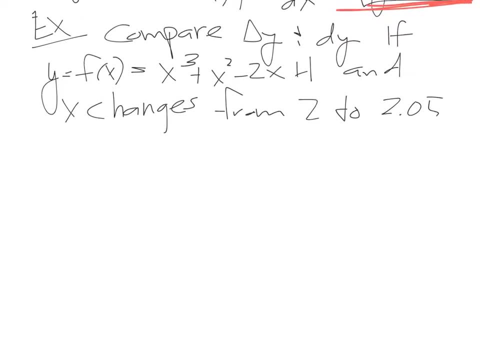 so you're not going to be able to use them anymore. ok, so let's begin. what we're going to have is: we want to figure out what is our delta y and what's our dy. to do that, what do we need? we need a couple of pieces of information. 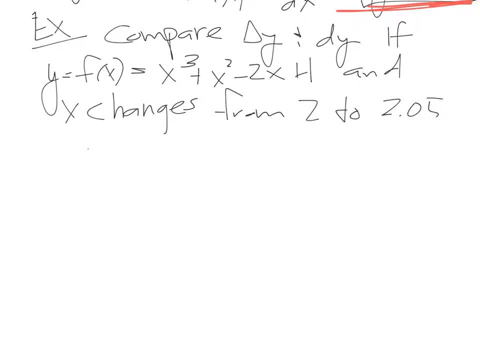 to find, to find delta y first. well, delta y, that was our f of x plus delta x, so that would have been our f of 2.05, and then we minus our f of x, minus f of 2, so let's figure out what's f of 2.5. 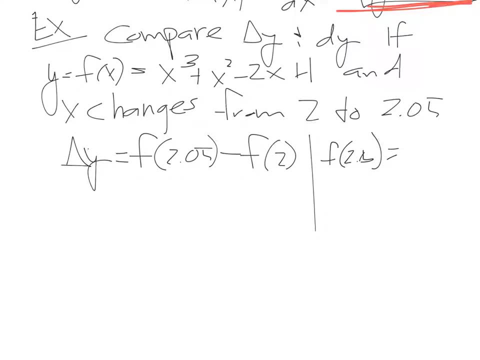 f of 2.5, plugging it in to this equation. I already did that, and so f of- excuse me, not 2.5, 2.05, f of 2.05 is 9.717625 and f of 2 comes out to just. 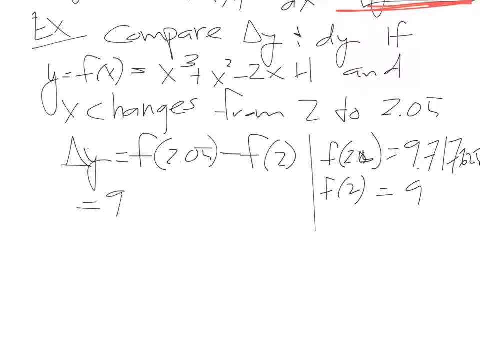 9. so our delta y is 9.717625 minus 9, which is 0.717625. that's our delta y. now we're going to find dy. so dy is given by the following: f prime of x times dx. so again on this side. 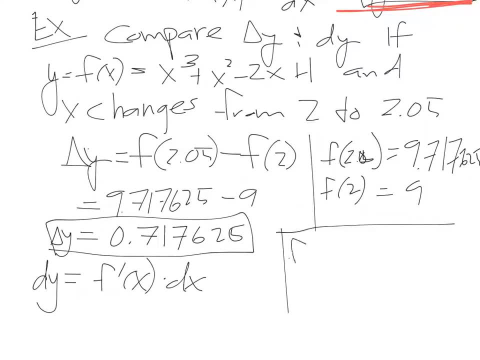 we need to figure out what's f prime of x. so f prime of x is the derivative of this whole thing. the derivative of x cubed is 3x squared plus the derivative of x squared is 2x and the derivative of negative 2x is negative 2. 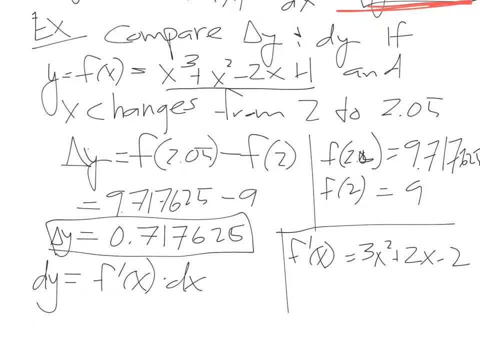 and the derivative of 1 is a constant, so it's 0, so that's f prime of x, so that's f prime of x, and so if we're doing this at, dy is equal to f prime of 2, and then our dx is our. 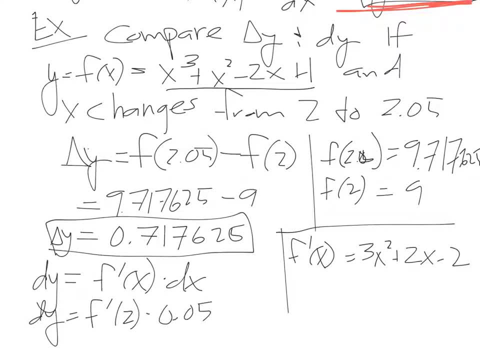 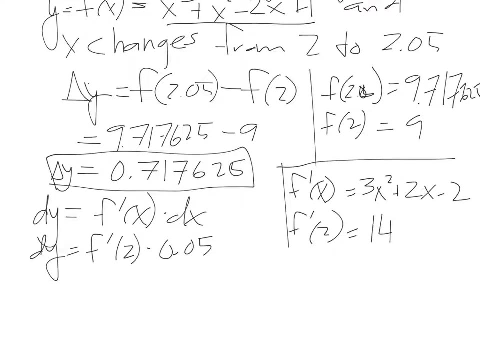 0.05. f prime of 2 is equal to the following 14, and so plugging in we get dy is 14 times 0.05, so we get our dy is going to be 0.7, 0.7 and you see these two. 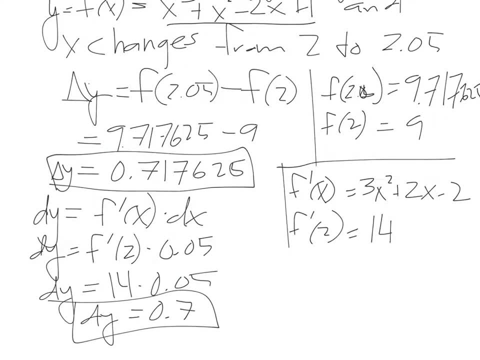 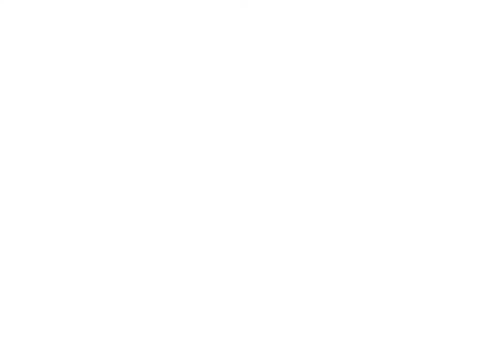 our delta y and our dy. they're in the same ballpark, but they are, in fact, different. now let's do one more example. in this last example, let's have the radius of a sphere, and this is actually going to be something that we might calculate, and this was measured. 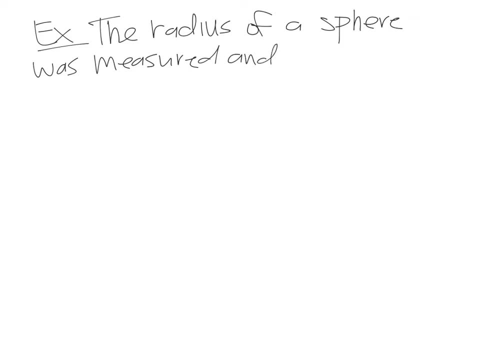 and found to be 21 centimeters, 21 centimeters. and when we measure this and when we measure this, it might have a possible, a possible error in the measurement, in the measurement of, of of at most 0.05 centimeters, 0.05 centimeters. 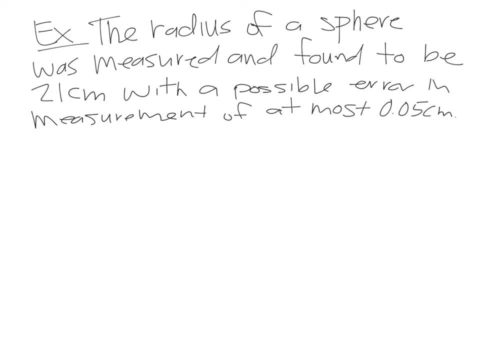 0.05 centimeters. so what is is the maximum error, the maximum error in using, in using the, the value, the value of the radius, of the radius, of the radius to compute, to compute the volume, the volume of of the sphere, the sphere. so what we did? 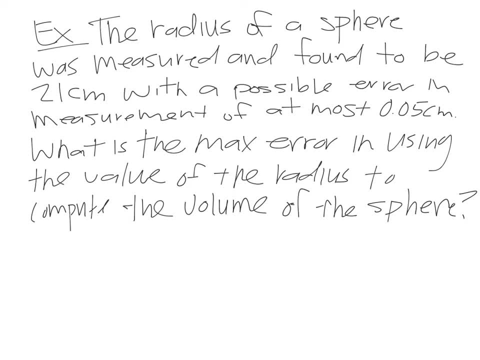 is, we measured the, the radius, but somehow, using the tools that we did, our tools might give us a maximum error of 0.05, or a possible error in our measurement of 0.05 centimeters. what's the maximum error that we could get when we compute? 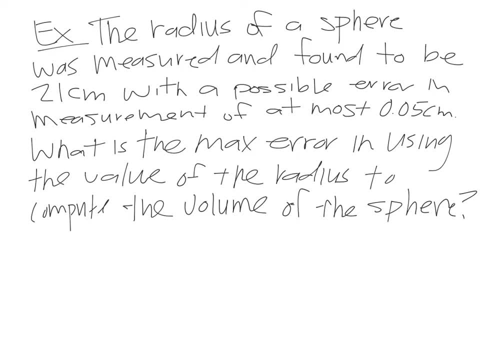 the volume. so the volume of a sphere v is equal to 4 thirds pi r cubed. if we let, if we let the dr equal, equal delta r, and this is going to be our and this is going to be our error in in the radius, then the corresponding 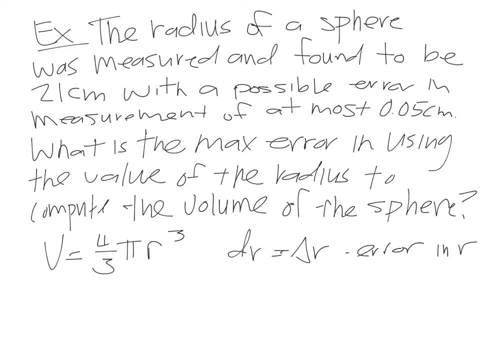 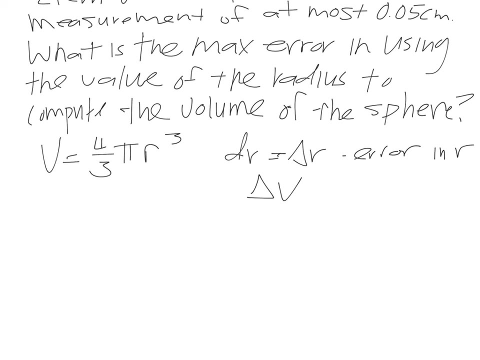 then the corresponding error in our volume would be this delta v and we can approximate our delta v. and we can approximate our delta v using the differential. so the differential taking the derivative we get dv is equal to the derivative over. here is using the power rule, we bring the 3 in front. 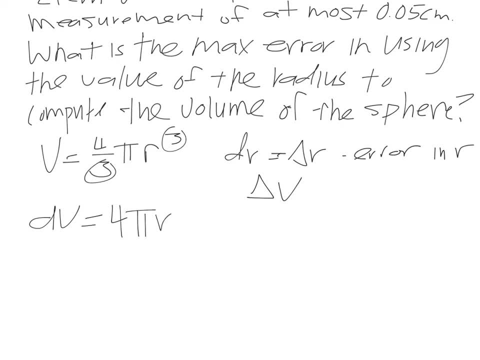 it cancels with that. so it's just 4 pi r squared times dr. and so if we're doing this, when the radius r is measured to be 21 and the possible error in r is measured to be 0.05, we get dv is 4 times pi. 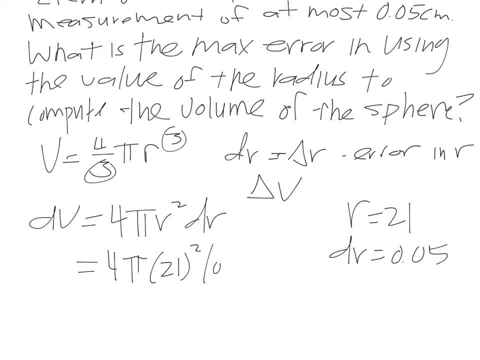 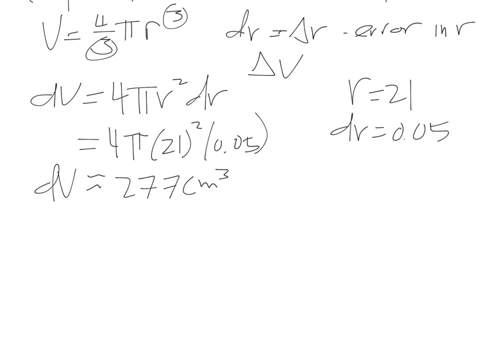 times 21, squared times 0.05, and so therefore we get our dv is approximately equal to 277, 277 cubic centimeters- cubic centimeters. so we computed the volume and the volume can be can have an error of 277 cubic centimeters. that might seem pretty big. 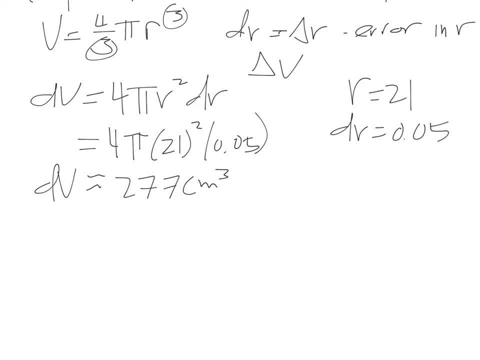 but it might not, because depending on the size of what we're dealing with. so this is something that we're going to, we take a look at and that's something that's called a relative error, and let me actually put a little color to this. so this is a relative error. 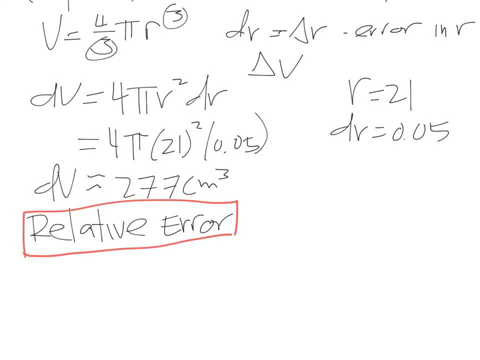 and the relative error is essentially the following: you take your error and you divide it by what the whole thing was. so we're going to take our delta v- let me just write this back in black. so we're going to take delta v and divide it by v. 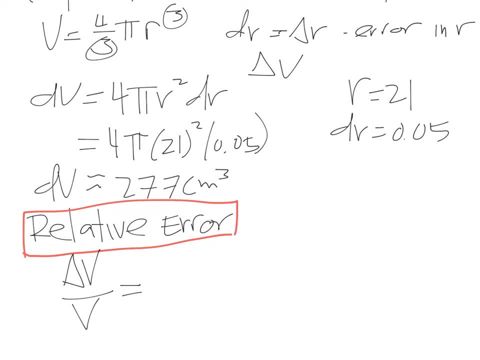 so how big is the error compared to the actual volume? and so maybe that's going to be approximately equal to dv over v, and so dv, which is dv, is 4 pi r squared times dr over 4 thirds pi r cubed, so that's 3 times dr. 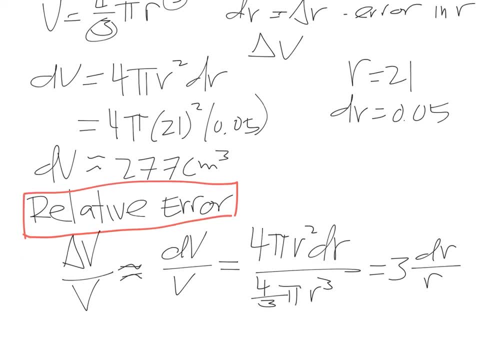 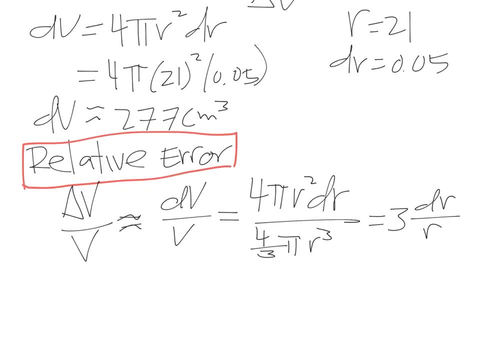 over r and so, looking at what we had, what we get, since we had our r and dr, is going to be 3 times 0.05 over 21, and that's approximately about 0.007- 0.007. and if we converted this, 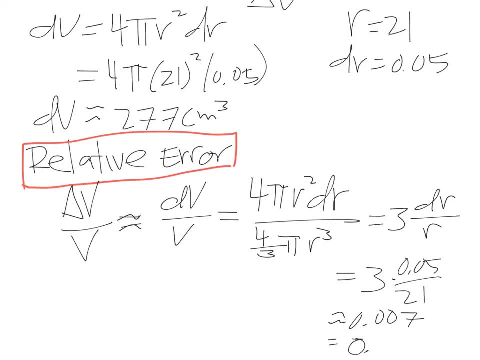 to a percent. this is 0.7 percent. that's pretty good. less than 1 percent, and this percentage that we call that's something that's called a percentage error. now, we could have solved this without this equation right here. all we needed to do was find: 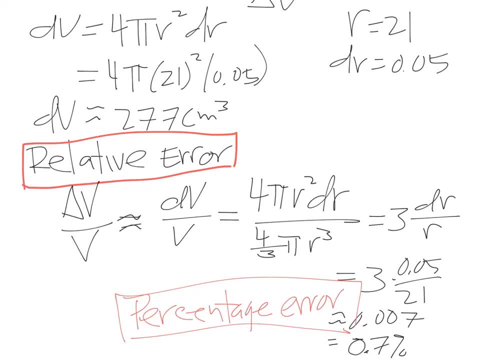 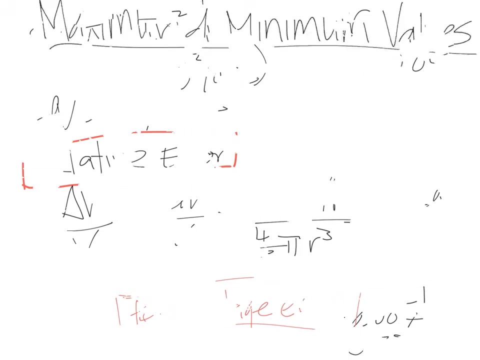 our error- divided by the total volume. so we could have taken 277 and if we knew what the volume was divided by the volume- in this case we didn't, but we could have actually computed it by the volume- is 4 thirds pi? r cubed. today we're going to talk about maximum. 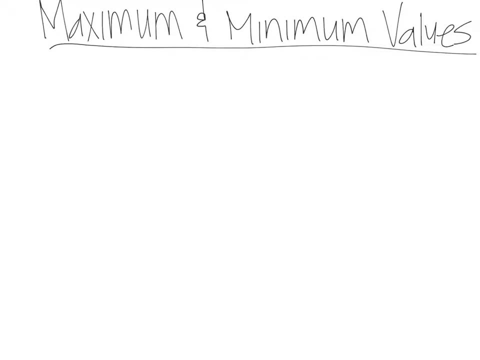 and minimum values. so we'll begin with definition. if we let c be a number in the domain of, and we'll call it domain d of a function f, then if we calculate f, evaluated at that point c, it's going to be called the following: it's going to be called: 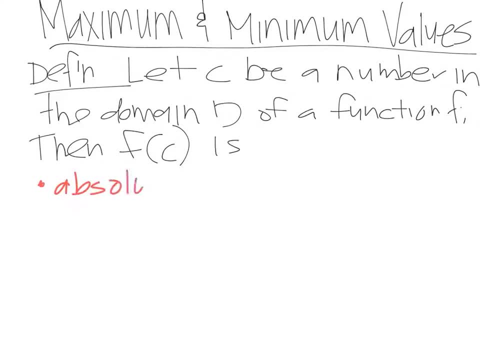 the absolute maximum is the absolute maximum value of the function f on d if f evaluated at c is greater than or equal to f for all x in your domain d. and then we say that the absolute minimum value is f of the function f on the domain d. 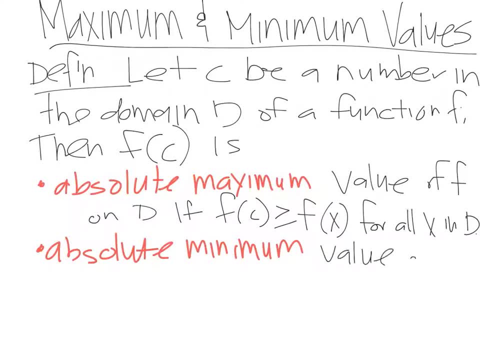 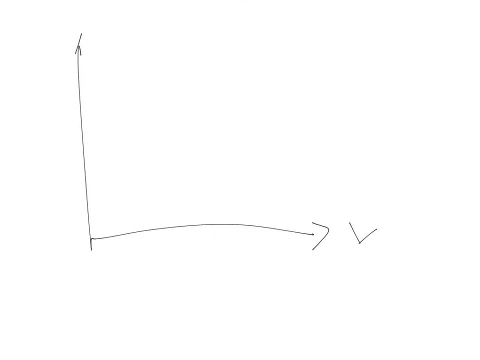 let's say, we have a graph and our domain is just going to be something like this and that's all we're dealing with. well, what is the absolute maximum value? This is because there is no value, an f of x value that's higher than that. 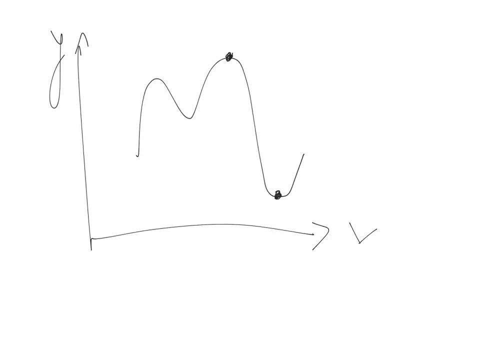 And then this would be the absolute minimum value, because there is no value that's lower than that. And so if we said like this is the point C and maybe this is the point D, then f of C is greater than or equal to f of x for every x that falls in this domain. 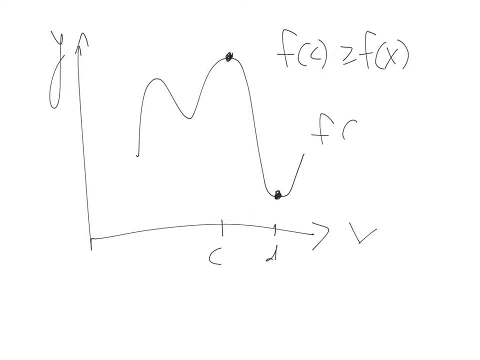 And similarly we would say: f of D is less than or equal to f of x for every x in the domain, and that's where this curve is our function. f of x: We have another definition And this definition begins with the number. f of C is one of the two following things: 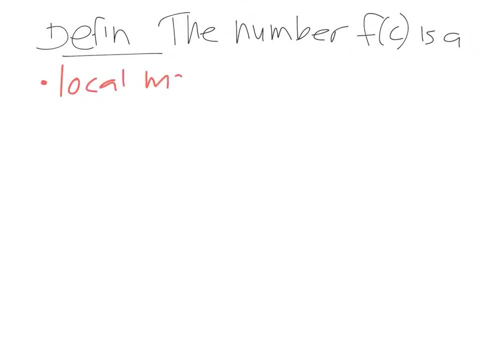 A local maxima or maximum value if we have the following: So it's local, So it's local, So it's local maximum value of our function: f. if f of C is greater than or equal to f of x. when x is near C. 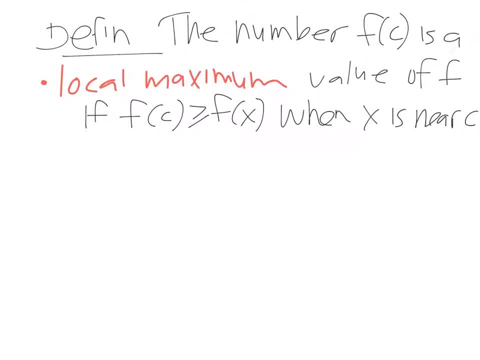 And then we have the second definition, that this says that it is a local, so it's local minimum value of our function f if f of C is less than or equal to f of x when x is near the point C. So 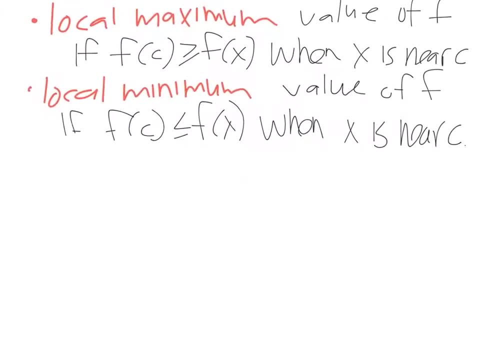 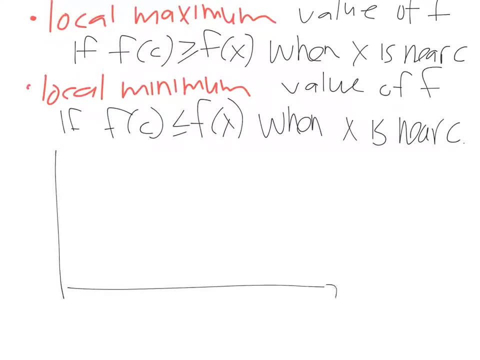 So what I mean by that is the following: so if we have our function- and let's say we're still our domain and we look to be something like this now, this point right here is the absolute minimum, because there's nothing else that's lower than. 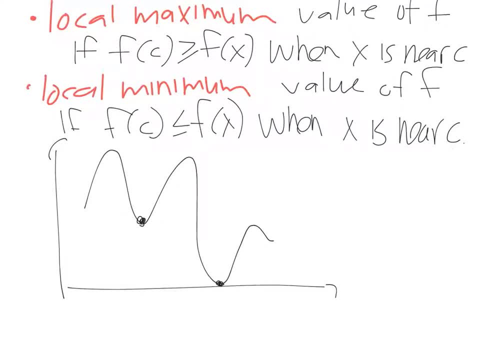 that. but this point right here is a local minimum, because if we're near that value, so we're near in terms of X direction- it's the lowest point near it. so this is a. this is a local minimum. this point up here is the absolute maximum. there's nothing else higher than that. but this is a local maximum and 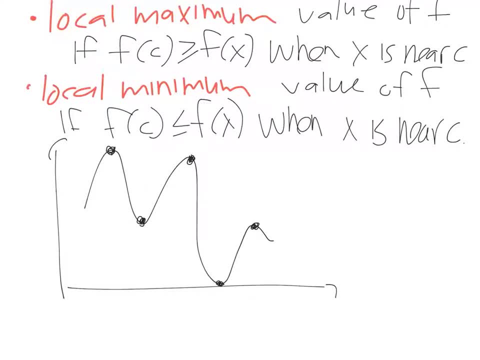 this is also a local maximum, because if you go near that, anywhere near here, there's nothing else greater than that. yes, if we pick the point over here, there is something greater. it's right here. if you pick the point right here, it's something greater. so none of those points are local. 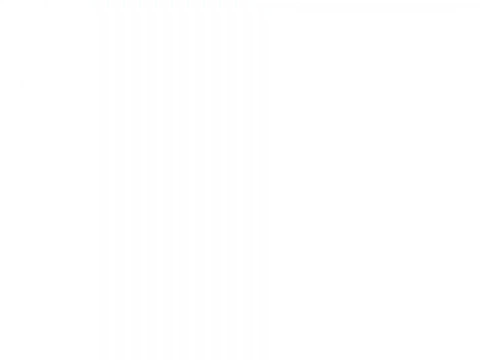 maximums. now we have a theorem, and this theorem is special and it has a name, and this is called the extreme value of theorem. the extreme value of theorem states the following: if our function F is going to be continuous on a closed interval, and this interval would be from: 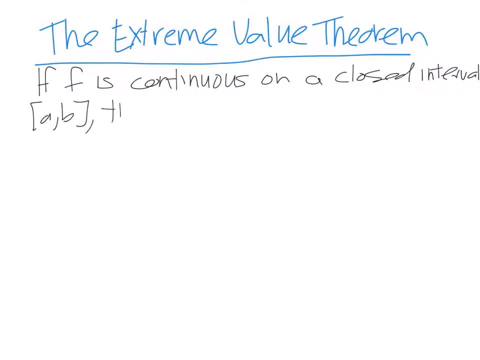 the point A to B, then the function F attains an absolute max value and we'll call that F of C and an absolute minimum value and And we'll call that point F of D. at some numbers C and D in the interval from A to B. 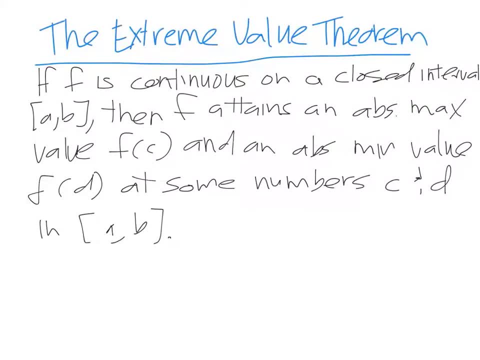 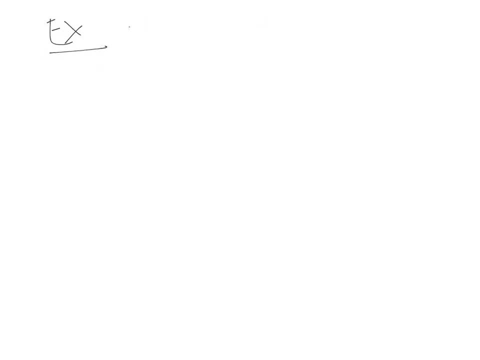 So where C and D are in the interval A to B. So let's take a look at a couple of examples. Y equals X squared. Well, that's a parabola, And so we know that the domain is going to be from negative infinity to positive infinity. 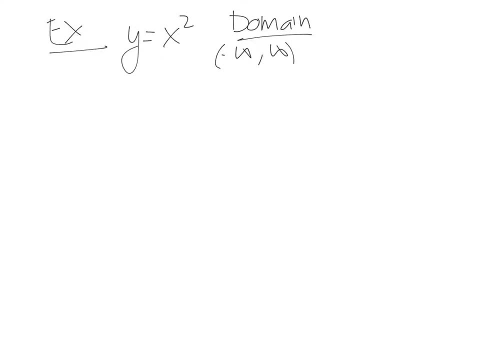 And so the absolute maxima is going to be none, Because that's a parabola that goes all the way up like this. So the absolute max There's going to be none, And the absolute min, Well, there is an absolute min. 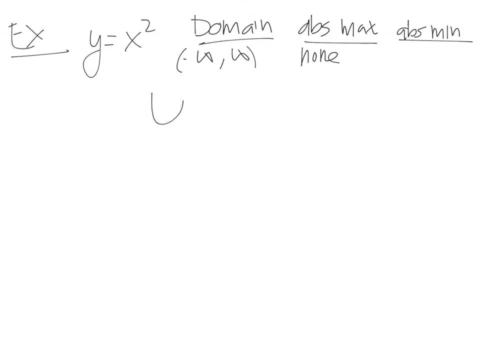 And that's going to be the absolute minimum value. So if we're asking for the value that's the Y value, It would be zero, And this is at: X equals zero. Now, if we're still looking at it, we're going to look at the function: Y equals X squared. 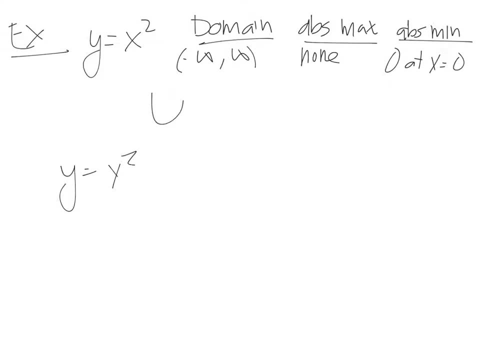 But our domain is not negative infinity to positive infinity. We're going to look at just from the point zero to two. So really, if we're looking at this curve, it maybe is at some point from here to here, So we're looking at just that curve. 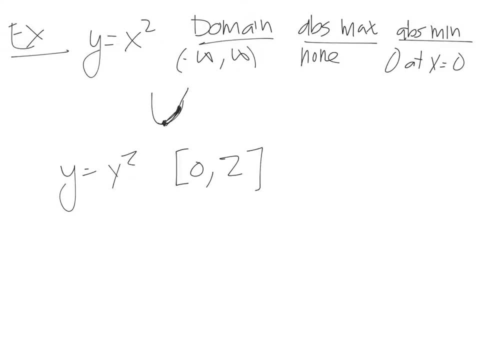 Then it does have a maximum value, And the maximum value is going to be right at the top when X is zero, And the maximum value is going to be when X is two. So the absolute max is when X equals two, And if you plugged in two into your function, 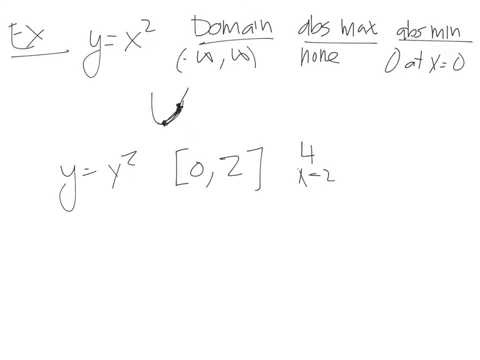 two squared is going to be four. So the absolute maximum value is four And the absolute minimum will still stay zero. And this is at. X is zero, And this is because of the extreme value theorem, since we had a closed interval And f of X equals X squared, that's continuous. 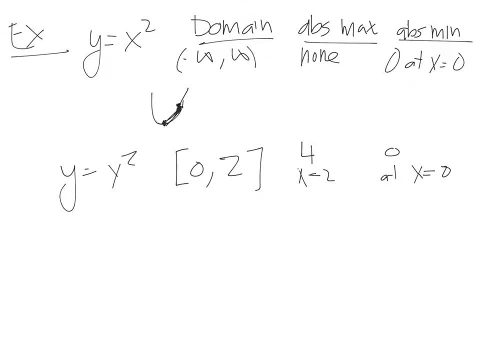 But if we weren't on a closed interval- and let's say we looked at some interval from zero to two- we include the point two but we don't include the endpoint zero- then what happens is the following: Well, two, we still have the maximum at two. 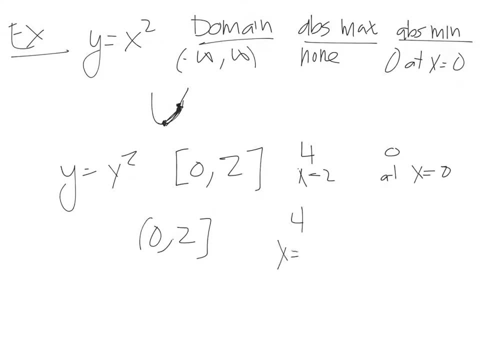 because we included the value two, So the maximum is four, And that's when X is two But zero is not included. So what's the lowest value we can get? We can start looking when X is, say, 0.1.. 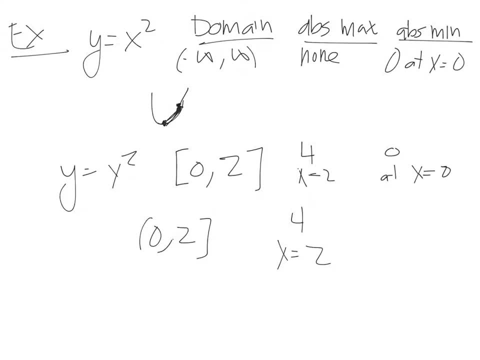 We can get closer to zero when X is 0.01.. We can still get closer when X is 0.001, and so forth. So we can get so close, but there is no exact value where we get the smallest. So in this case, there's no. 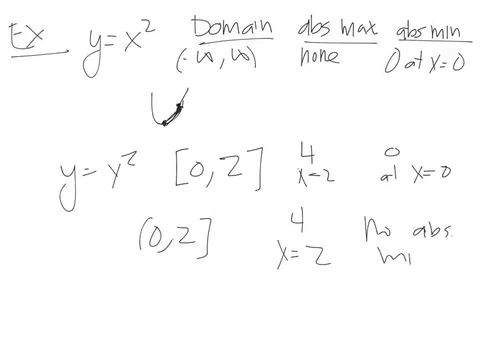 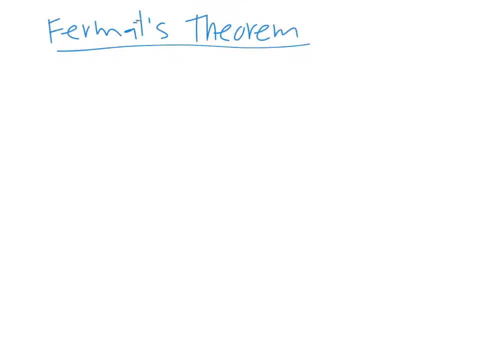 There's no absolute minimum. Now we have a theorem called Fermat's theorem, And Fermat's theorem states that if, If F Has A local Maximum Or Minimum At some point C And If the derivative of F at C, 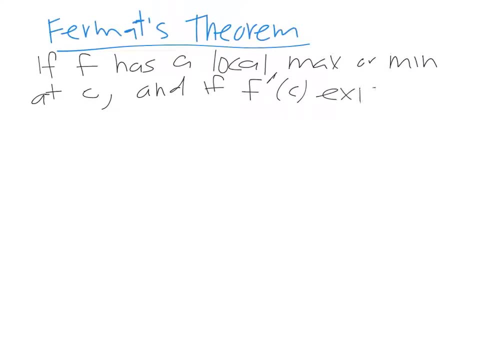 F prime of C Exists, Then The derivative of Of X At C Is Minimum At Some point. C And The, The derivative f prime of c, is equal to 0. Now I'm not going to prove it, but if you think about it it can sort of make sense. 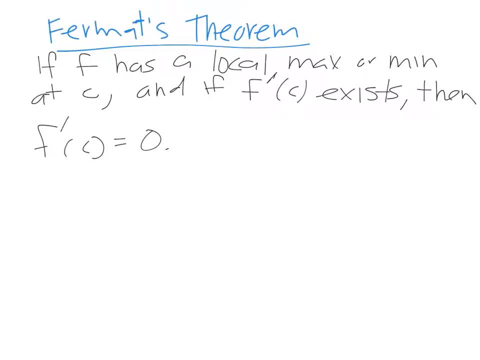 Taking a look at a curve, something like that, a curve like this, this point right here is a local maximum. What's the slope at that maximum? Well, over here, the slope is positive, and then this is also positive. Down here, the slope is negative and the slope is negative. 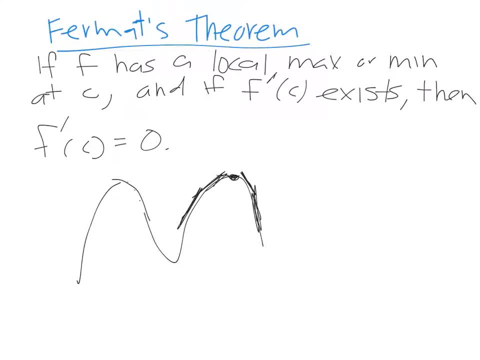 And so to go from a positive to a negative slope, right here, at that maximum value, the slope is 0.. And so the slope meaning the derivative of that function is 0.. And same thing for the minimum: We're going at a negative slope. 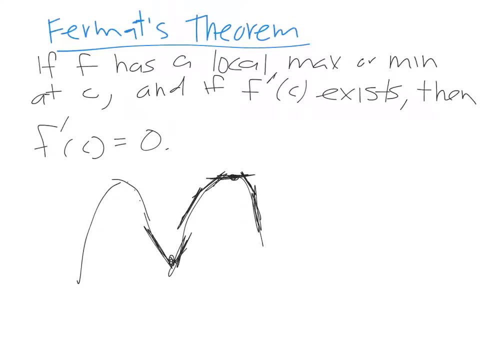 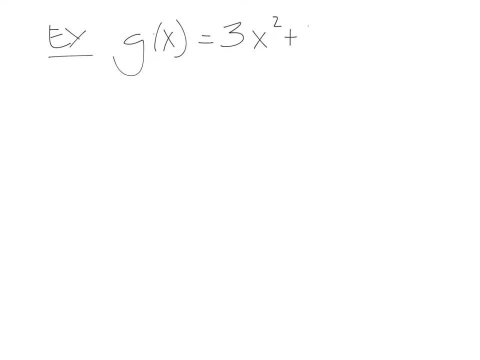 We have a negative slope And right at the minimum the slope is 0. So that's where we get this. f prime at c is equal to 0. So an example might be: if we have, the function g of x is equal to 3x squared plus 4x plus 9.. 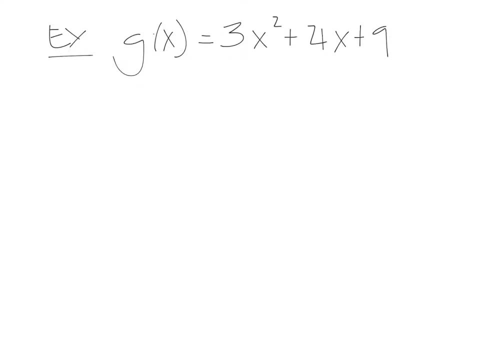 Find the local maximum and minimum. Well, in order to do that, we'll take the derivative g prime of x, and this is going to be 6x plus 4.. And we want to find when the derivative is equal to 0.. 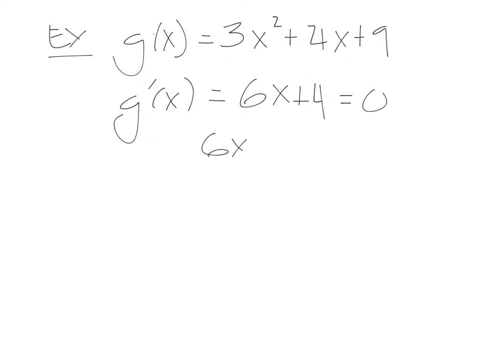 And so now we solve. So we get: 6x is equal to negative 4, or x is negative 4 over 6,, which is negative 2 thirds. Now that's the answer. So we plug in the x value and make sure when you're trying to find the local max or min. 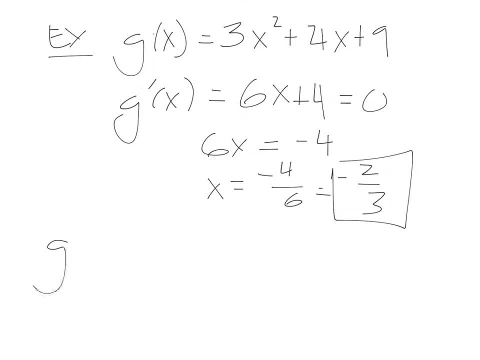 you want to find the y value, So we plug it back in. g of negative 2 thirds is equal to 3 times negative 2 thirds squared plus 4 times negative 2 thirds plus 9.. So this is going to be 3 times 4 ninths plus negative 2 thirds. 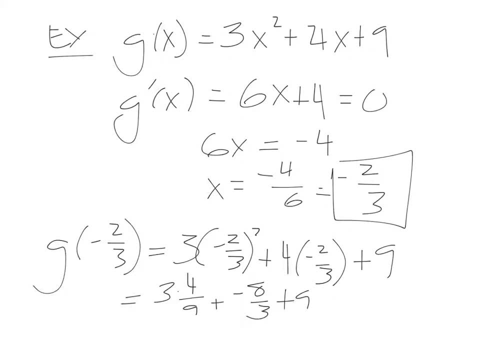 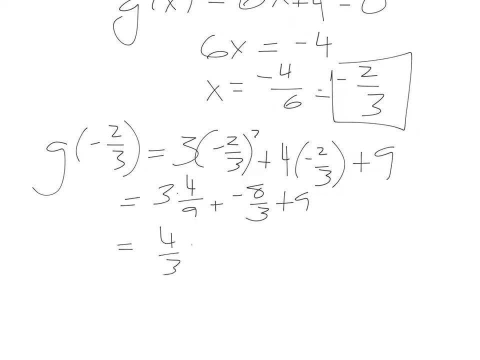 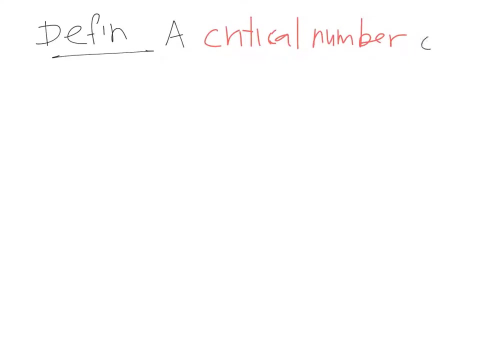 Negative: 8 thirds plus 9.. And this simplifies to 4 thirds minus 8 thirds plus 27 thirds, which is equal to 23 thirds. Next we have a definition. This definition states that a critical number of a function, f, is a number. 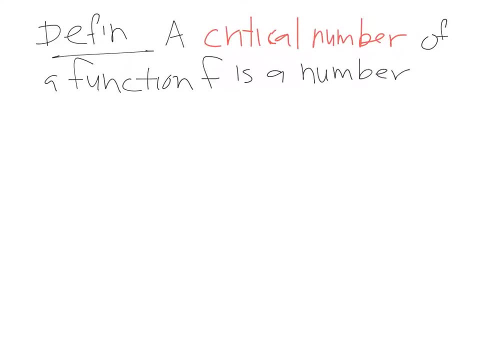 c, that's in the domain of f, such that either the derivative f prime at c is equal to 0, or f prime at c does not exist. So if a derivative is 0,, meaning it's going to be a local maximum or a local minimum. 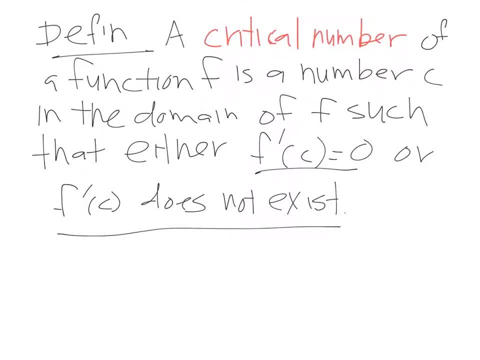 or if the derivative does not exist. that's a critical number. So let's do an example. Find the critical points for the function. h of x is equal to x to the 2nd power. x of x is equal to x to the 2th power. 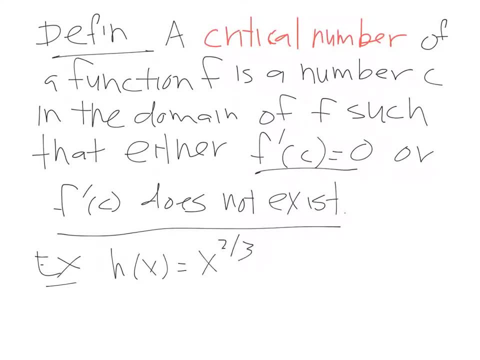 So let's do an example: equal to x to the two-thirds. Critical points are when the derivative is zero or the derivative doesn't exist. So let's calculate the derivative That is two-thirds x to the negative one-third, or this is going to be two over three times the cube root of x. Now the cube root can be negative. 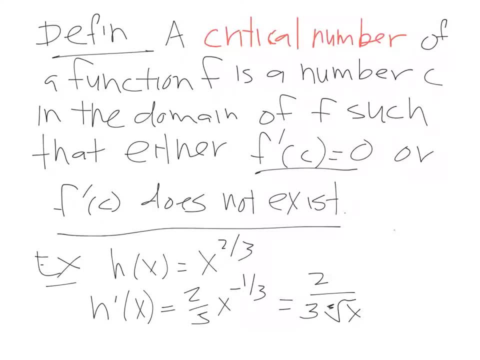 because you could take, for example, the cube root of negative 27 and that would be negative three, because negative three times negative, three times negative three is negative 27.. So that's fine, but we have something in the denominator and so we cannot have zero in the denominator. 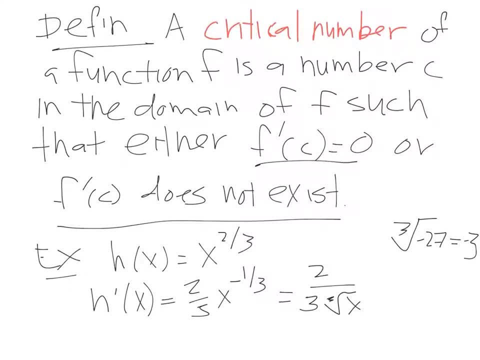 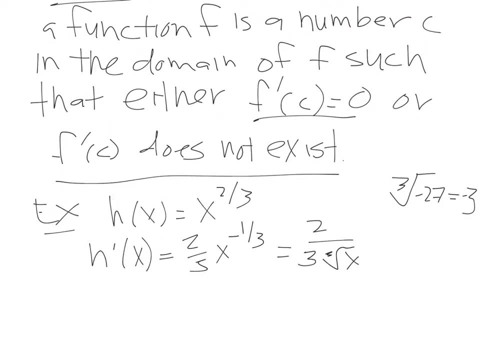 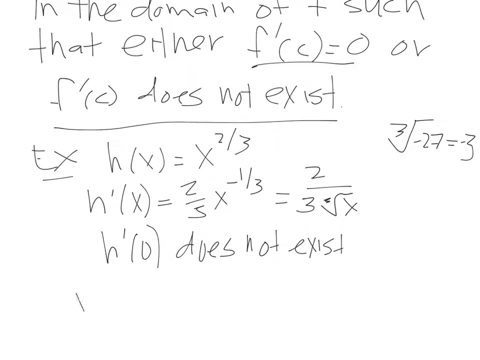 and so we know that if x were zero we could have a negative three times negative, three times negative three. Then we'd be dividing by zero. and so zero is our critical point, because h prime of zero does not exist. So our answer, x equals zero, is a critical point. 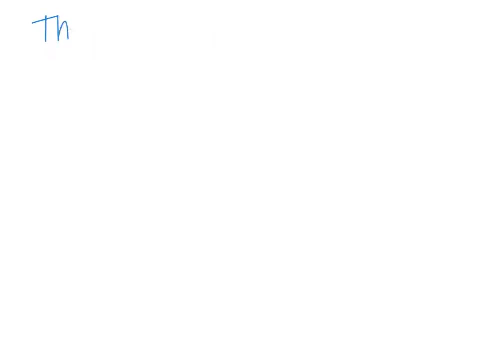 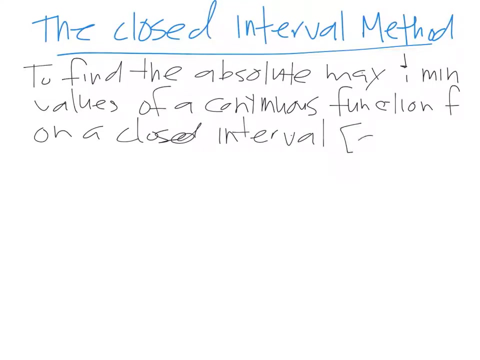 Now the last thing we're going to cover in this section is called the closed interval method. The closed interval method says to find the absolute maximum and minimum values of a continuous function on a closed interval from a to B. then we look at three steps. First, 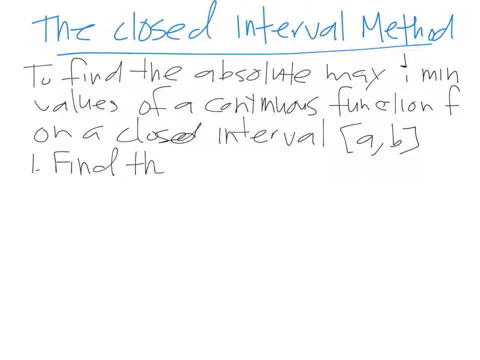 find the values of F at the critical points or the critical numbers of F in the open interval A to B. Then, step two, find the values of F at the end points of of the interval. And then the last step, step three. 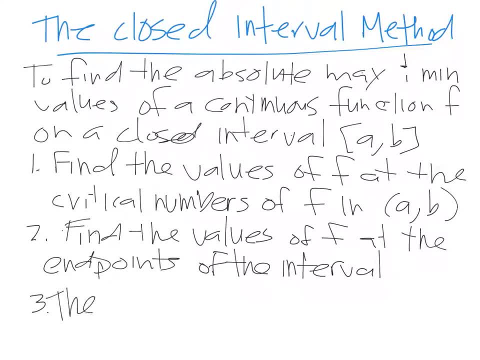 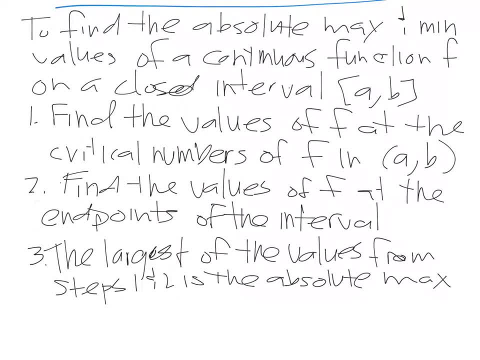 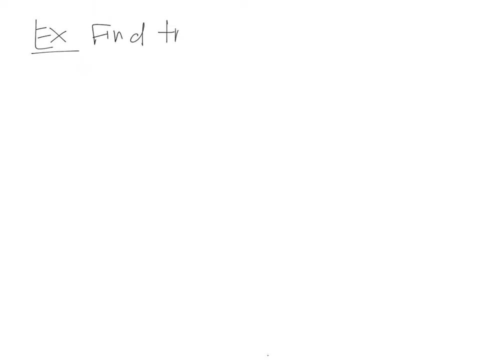 And, finally, the smallest of the values is the minimum or the absolute minimum. The smallest of the values is the absolute minimum, And so these are the steps to finding the absolute max and the absolute min. So we'll do one example And find the absolute max. 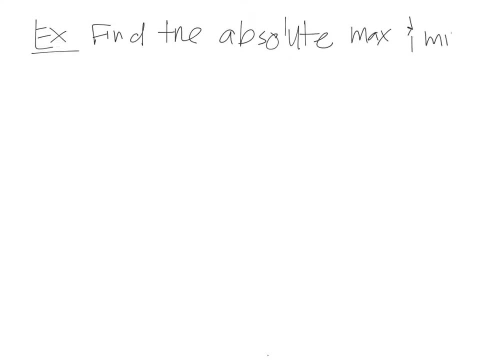 And min. So find the absolute max and min And we'll just say the values Meaning. the y value Of our function, f of x equals 8x minus x to the 4 on the closed interval negative 2 to 1.. 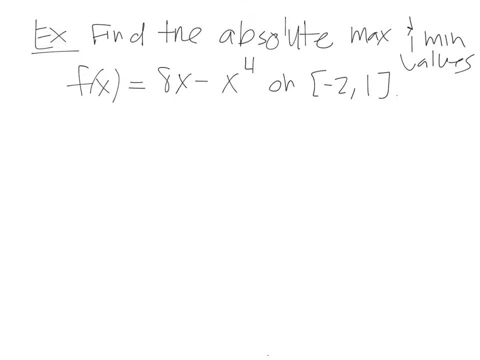 So What do we do? We first take the derivative f prime of x Equals 8 minus 4x cubed. We want to find the critical number. So we want to find when this is 0 or undefined. 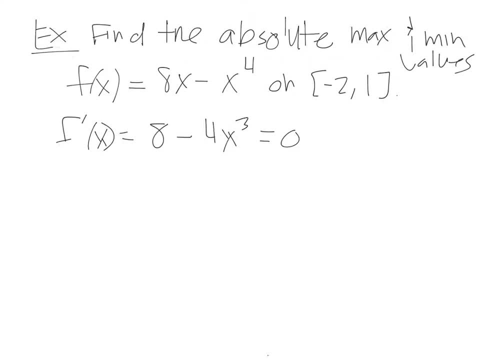 Well, this is going to be defined everywhere, So we'll just find out when it's 0.. If we add 4x cubed to both sides, We get 8.. Is equal to 4x cubed Or 2.? 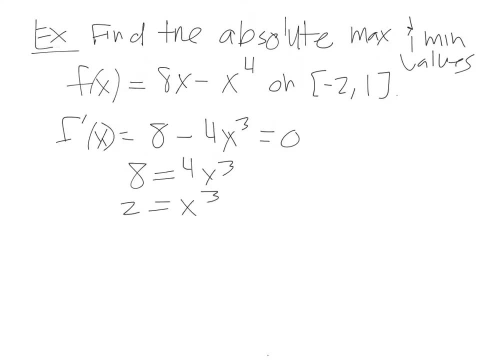 Is equal to x cubed, And so therefore, Taking the cube root, We get that x Is equal to the cube root Of 2.. And substituting in, We get our y value, f Of the cube root of 2.. 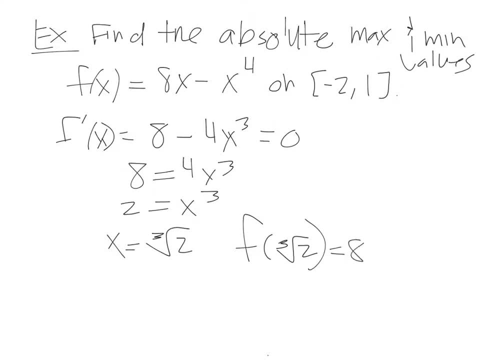 Is equal to 8.. Times the cube root of 2. Minus Cube root of 2. To the power of 4. And Plugging this on the calculator. This is about 7., 5., 6.. 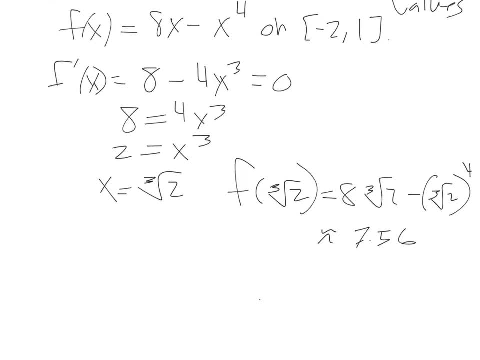 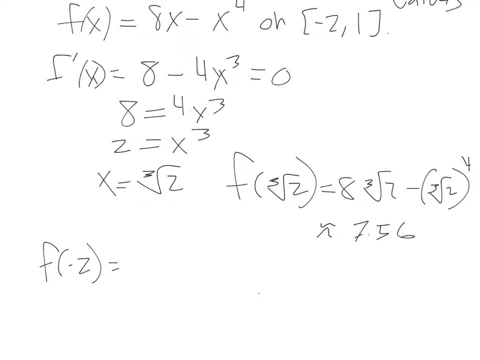 Now We need to check the endpoints, And so we're checking the endpoints f At negative 2. And f at 1. Well, f at negative 2. Is going to be 8 times Minus negative 2.. 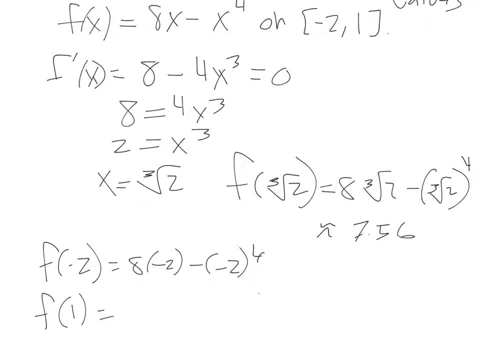 Minus negative 2 to the 4th, And that's going to be Negative 32. And f at 1 is going to be 8 times 1. Minus 1 to the 4th, Which is 7.. 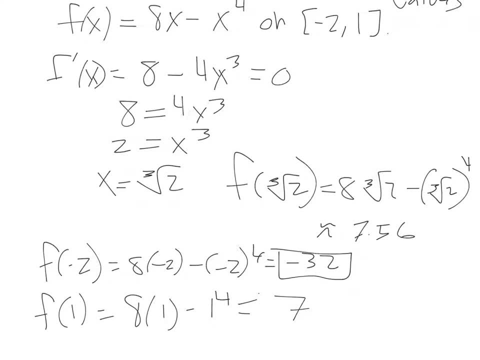 So what we have here Is that this is the minimum value. So this is the absolute Minimum. Now, the absolute maximum, This was a little trick Or a trick question. rather, 7.56 is greater than 7.. But remember, 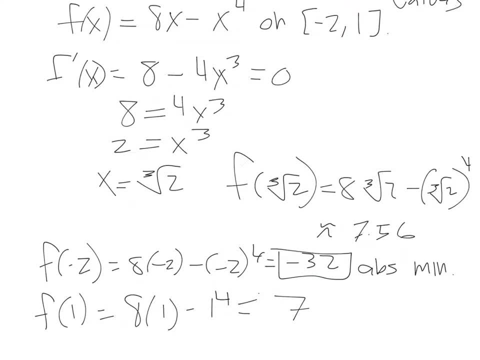 We said that our interval Had a maximum value Of 1.. What is the cube root of 2?? Well, The cube root of 2 is a little bit greater than 1.. It's about 1.26.. So 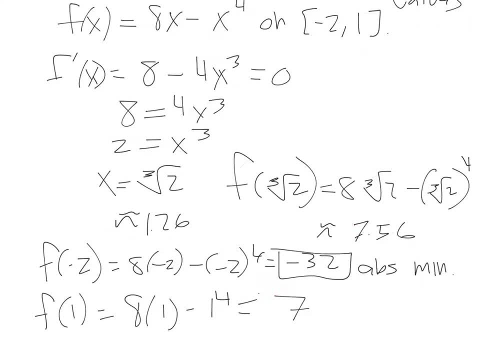 Even though This y value is greater than here, The x value didn't fall in Our domain, And so Our absolute maximum Was at 7.. So When you do problems, Make sure That your answer falls within the domain. 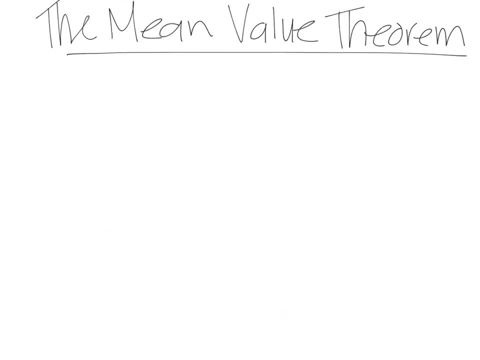 Today we're going to talk about the mean value theorem. We'll begin with a theorem, And this theorem is called Rolle's theorem. Rolle's theorem says the following: Let F Be a function That satisfies The following: 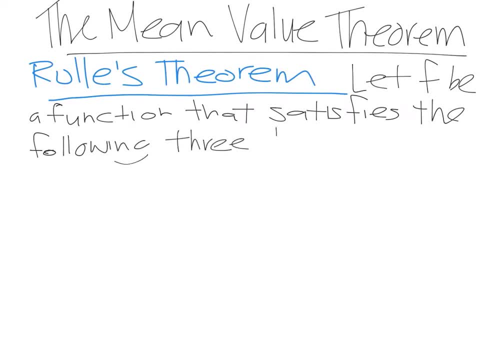 Three hypotheses To find out the mean value. Find out how, By using the curve And there's a number, this That will also help you Find out what the mean value Is. This Is The value, Is The. 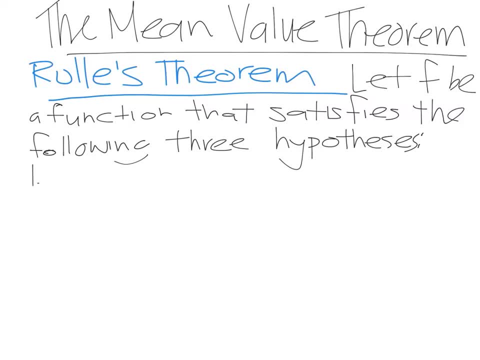 Complex Of The Sympathetic, The Sympathetic. The first one says No. The two of them Are Ek S, S Ul. that F is continuous on the closed interval A to B. The second criteria says: 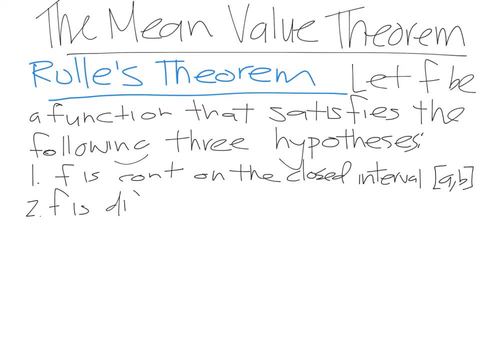 that F is differentiable on the open interval A to B. And then the third criteria states that F of A equals F of B. If all three of these things are met, Then we can conclude there is a number C that's in the interval A to B, so C falls. 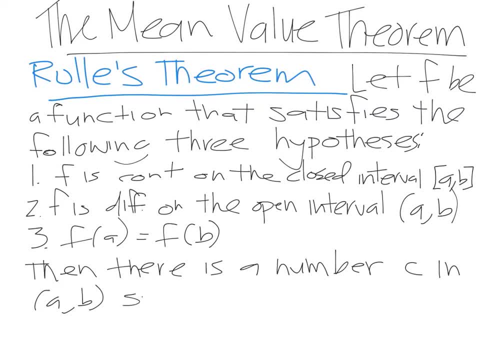 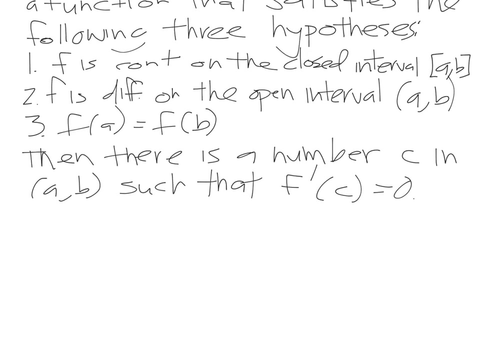 between A and B, but not on the endpoints, such that F prime of C is 0, meaning the derivative of F is 0.. F at the point C is equal to 0.. So what is this saying? Let's take a look at some examples. 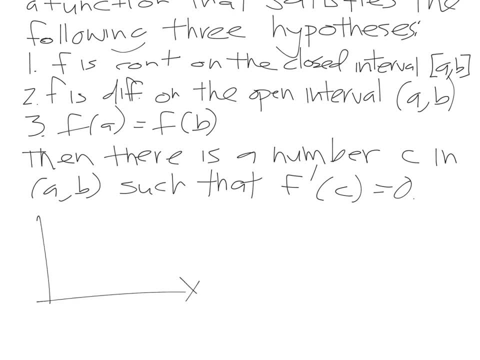 So if we have our function, and we have the point A and the point B and our function, F is a horizontal line. F of A equals F, prime of C. F of B equals F of B. It's differentiable on this function and it's continuous. 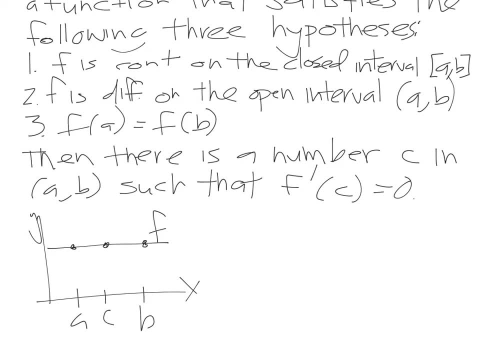 Then there's some point in the middle. let's say right here C, where F prime of C is 0, meaning the derivative is 0, so it has a slope of 0. And that's true because this is a horizontal line. 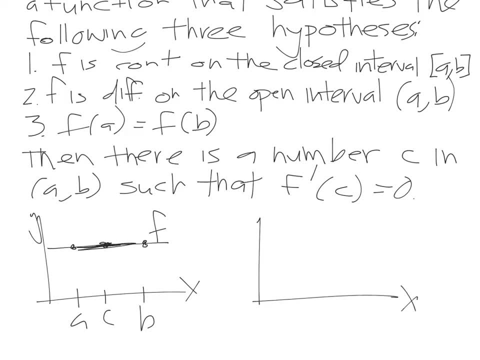 We could have another case that looks like the following: Let's say we have the point A over here, B over here, and our graph looks something like that: This is continuous, this is differentiable and F of A equals F of B, but this point right. 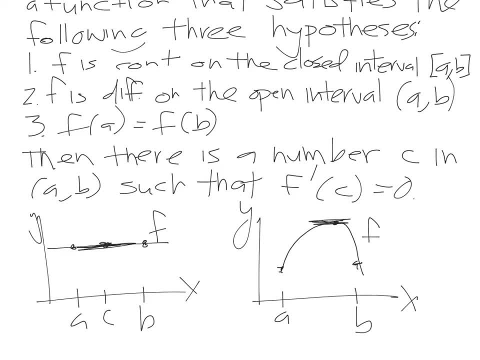 up here is horizontal, or it has a slope of 0.. F prime of C, so our C would be right. there is 0.. There's other cases. Let's take a look at this. Let's take a look at this. 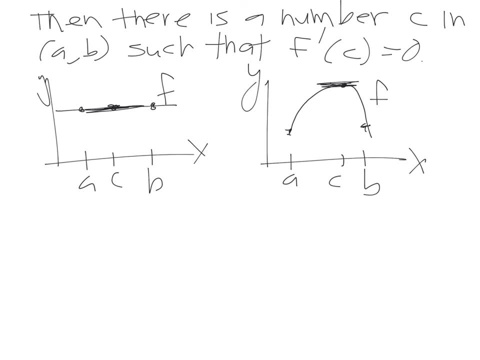 There's other cases that we might look at, And those cases might look something like: here's the point A, the point B: We might have F of A, F of B looks like that. we might have something like this: Now we'll have multiple places where we have F, prime at C is 0, so we could have this. 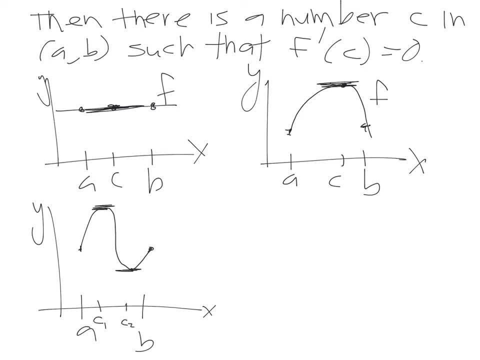 could be our C1, and that could be our C2.. But all we're saying is that there exists at least one point C And then finally we could just have for A and B. it would look like: oh, I just did that. 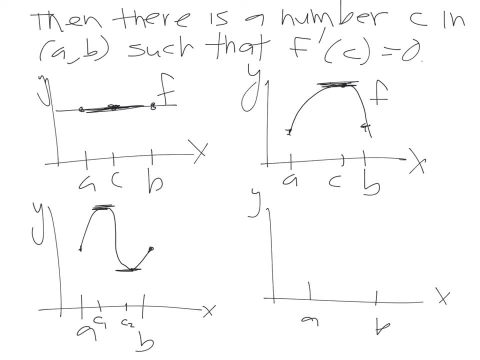 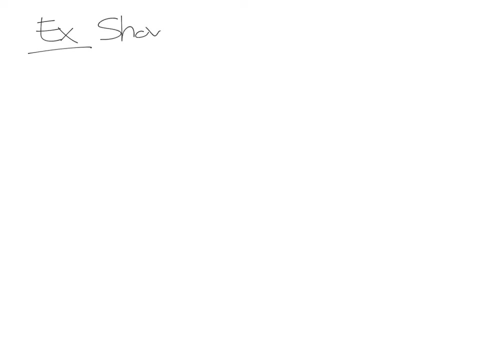 It would let me, it would look the other way, And so we have that one. So let's do an example. Let's show that the equation X cubed plus 3X plus 1 equals 0, has exactly one real solution. 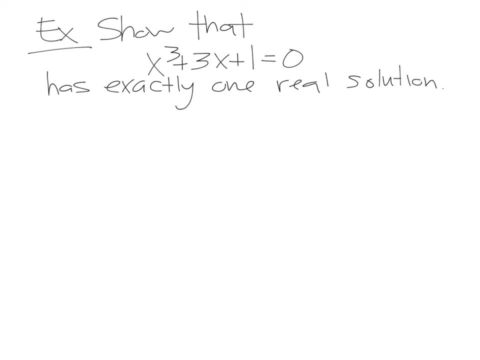 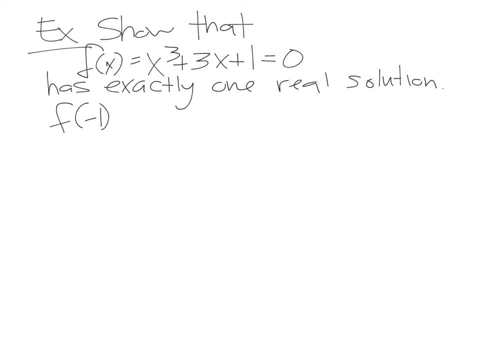 We're going to be able to do this. We're going to be able to do this, And so we're going to write the function F of X. notice that F of negative 1 is going to be negative 1, cubed plus 3 times negative 1 plus 1, which is negative 3.. 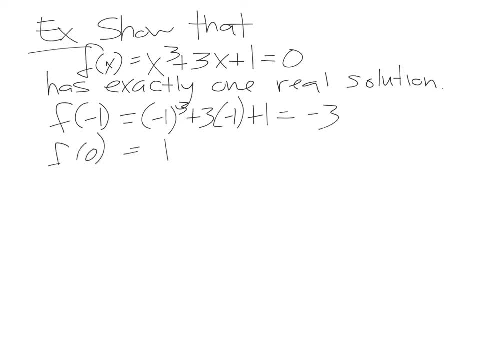 And F of zero. well, that's just going to be 1.. So we know we're crossing from negative to positive And the intermediate value theorem says that if you have something, that's going to be negative, negative and then it's going to be positive and it's a continuous function. 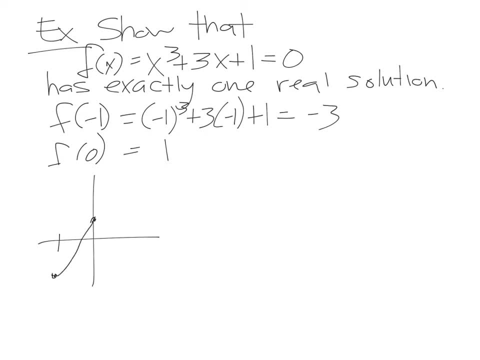 which this is. since it's a polynomial, it has to cross the axis. now I could cross multiple times, but now we're trying to show that it crosses just once. now, if it did cross more than once, we might have something where it would look like this: it crosses one time, crosses two times and then it goes back up, maybe even. 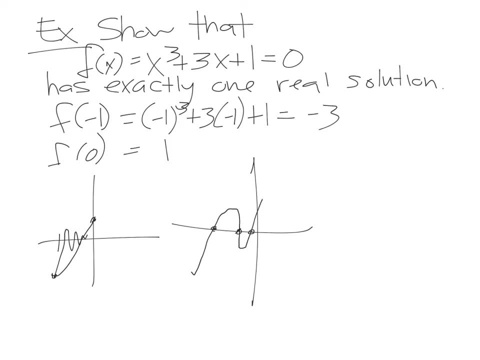 three times. but Rolle's theorem would say that if this were to happen, where we have these two values are equal, then we would have to have the derivative at some point is going to be zero. so let's calculate the derivative. derivative is going to be f. prime of X is 3x squared plus 3. but notice: 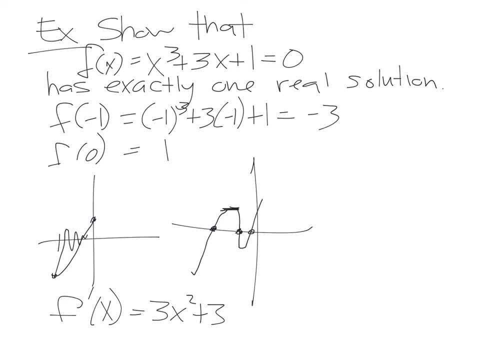 this is going to be f. prime of x is 3x squared plus 3. but notice, this is going to be f. prime of x is 3x squared plus 3, but notice, this can never be 0. this is always going to be greater than 0 because x squared is. 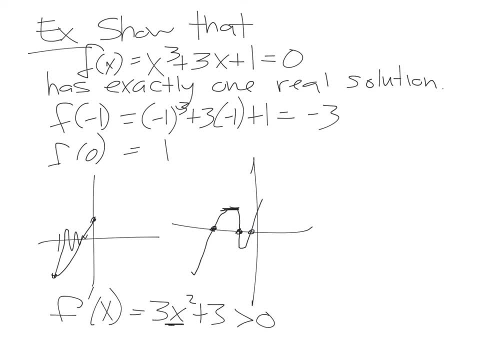 always a positive number, and if you add 3 to a positive number, it's always going to be positive. so there's never going to be the point when it's equal to 0, which means that we can't have. we can't satisfy a Rolle's theorem, and thus we 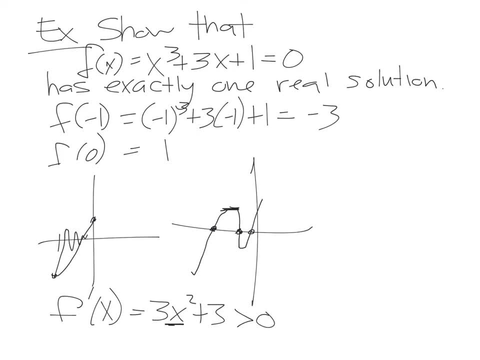 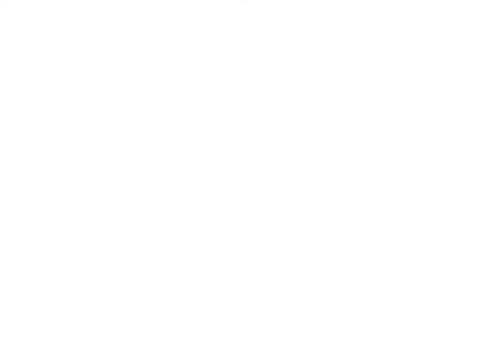 only have one zero. now the main point of Rolle's theorem is so that we can actually use it for the mean value theorem. now we go to the mean value theorem. the mean value theorem states the following: let f be a function that satisfies the following one: f is: 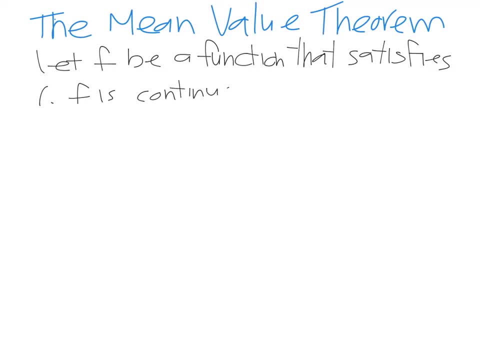 continuous on the closed interval and Sz a to B to f is differentiable on the open interval. 1. a to b, a to b, 2. if these two hypotheses are met, then there is a number C that's in the interval A to B, such that F prime of C is equal to F of B, minus F of A divided by B. 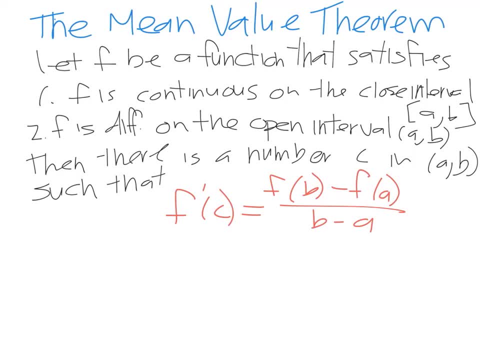 minus A, or we could write this equivalently as follows: you, if we multiplied out, we could have written it as: F of B minus F of A is equal to the derivative F prime of C times the quantity B minus A. so now, in order to think about this, 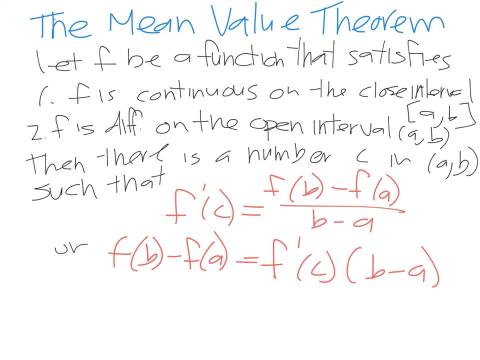 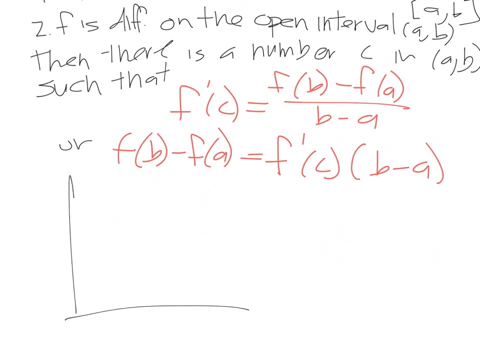 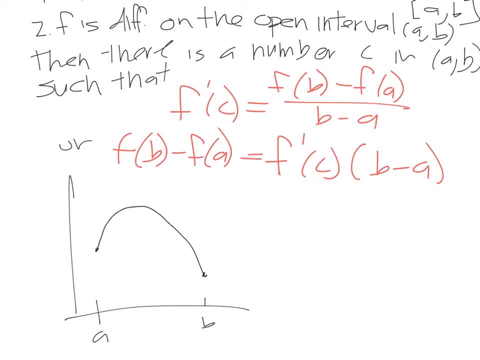 A and to get from A to B, connecting the slope from A to B, we have a line that looks like this with that slope, and we have a line that looks like this, and we have a line that looks like this: if we have a slope somewhere on this curve, we right here. the derivative is not the same, not right here. 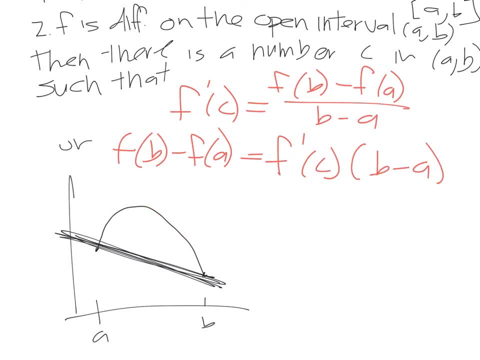 but maybe somewhere right there we have a derivative where the slope is going to be the same. we might also it might- have something else. say, we have some point A over here, some point B up there and the graph looks something like this: Connecting these two points. that's our slope. maybe we'll have a point right here as well. 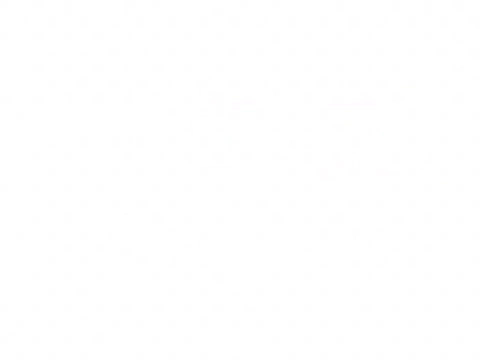 as a point right here. So let's do an example using the mean value theorem. Take a look at the function f of x equals x squared. Now we know this is a parabola, and a parabola is something like this: it crosses at the 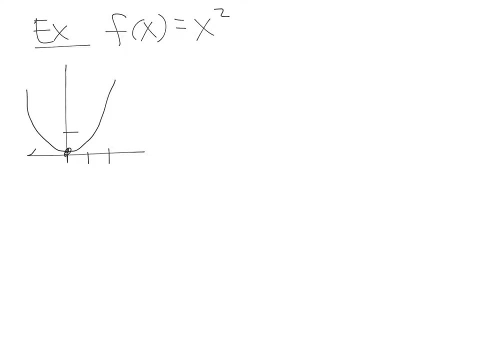 origin. at the point 1, it's at 1, at 2, it's 1, 2, 3, it's 2, squared, so it would be 4.. Let's take a look at the interval from 0 to 2.. 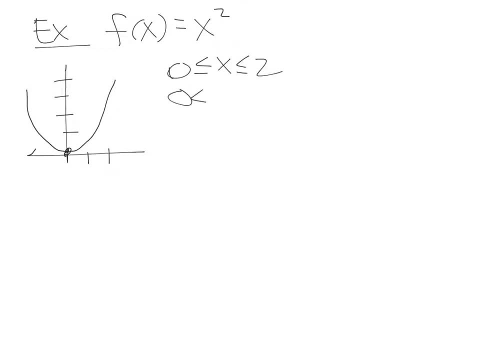 It's continuous from 0 to 2, it's differentiable on the open interval, 0 to 2.. So the mean value theorem says that there's some point C, such that 0 to 2 is 0.. f prime of C is equal to f of 2 minus f of 0, divided by 2 minus 0.. 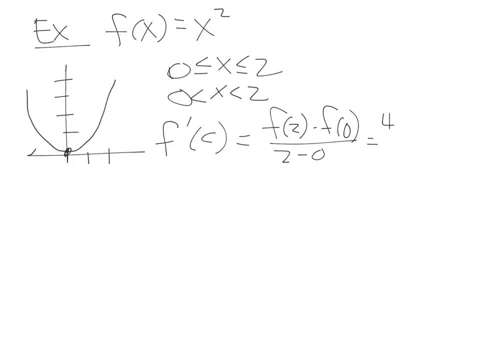 Well, f of 2 is 2 squared, so 4 minus 0 squared, or 0, over 2 minus 0, so this is going to be 2.. So we need to find that point C that exists. Well, what's the derivative? first of all, 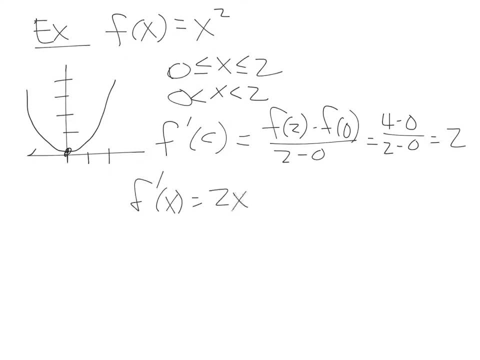 What's f prime of x? That would be 2.. So f prime of x is equal to x, And so if we wanted f prime of C to be equal to 2, then we get that C is equal to 1.. And we know that 1 is in this interval between 0 and 2.. 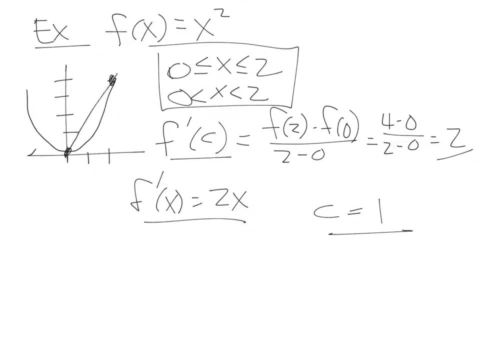 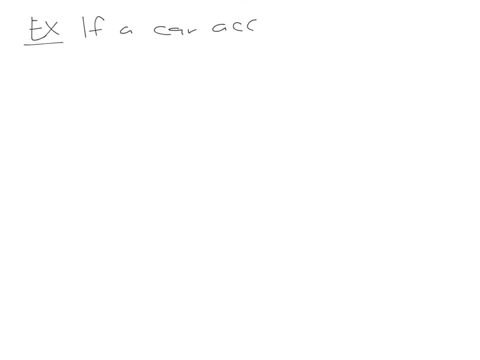 And so looking just at this graph where the line looks like this, Looks like that The slope right here at should also be that same slope. Now let's do a different type of example. Let's suppose that if a car accelerating From zero 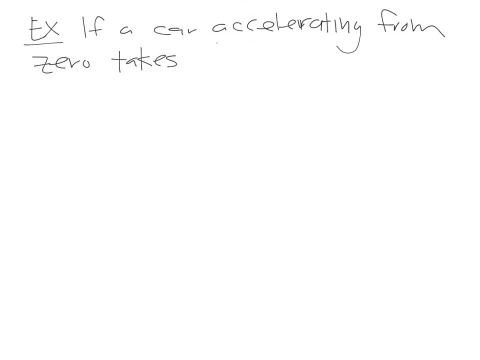 takes 8 seconds to go- 352 feet. its average velocity for the 8 second interval is going to be the distance- 352 feet divided by 8 seconds, and the units would be feet per second. So this is 44 feet per second. 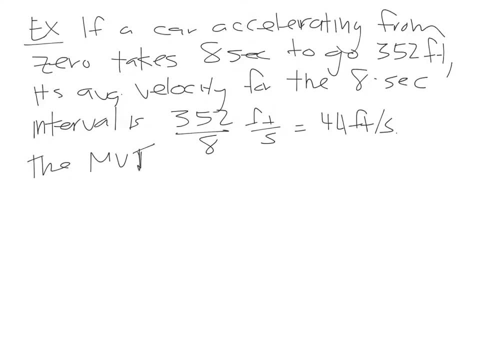 The mean value theorem, which I'm just going to abbreviate with its initials: MVT, says that at some point, that at some point during the acceleration, the speedometer must read exactly 44 feet per second, or 30 miles per hour, or 44 feet per second. 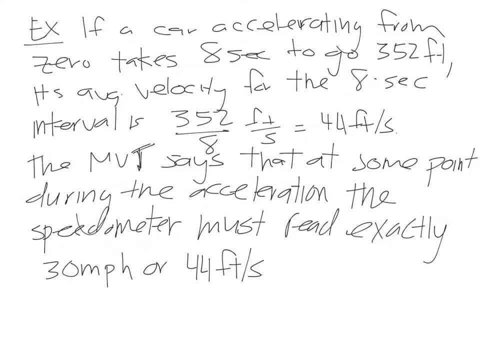 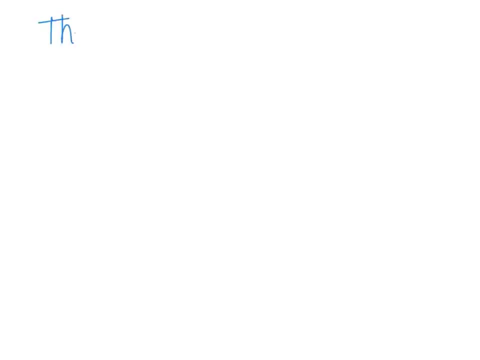 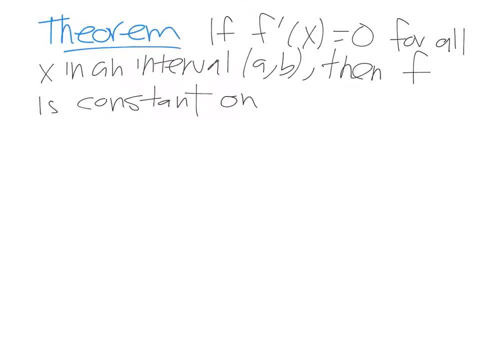 constant. Okay, on that interval a to b, if the derivative is zero for all that value, it's just a horizontal line. that's all this is saying. finally, we have a corollary. the corollary states the following: if f prime of x is equal to g prime of x, 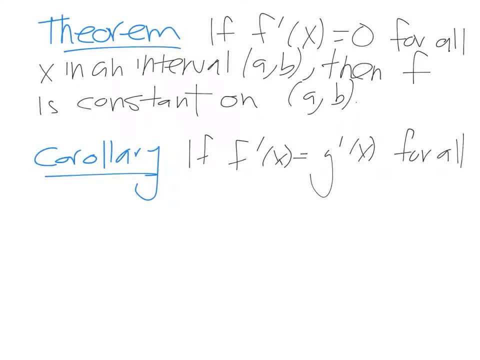 for all x in an interval a to b, then f minus g, f prime of x is equal to g. prime of x is constant on that interval a to b. in other words, that is f of x equals f of g plus some value c, where c is a constant. 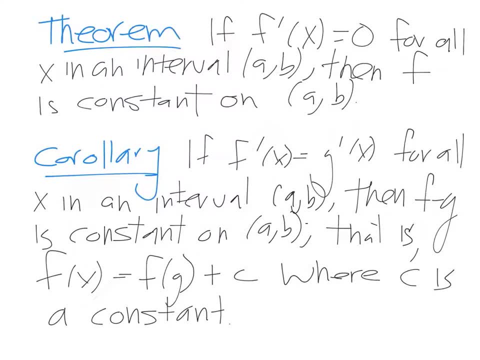 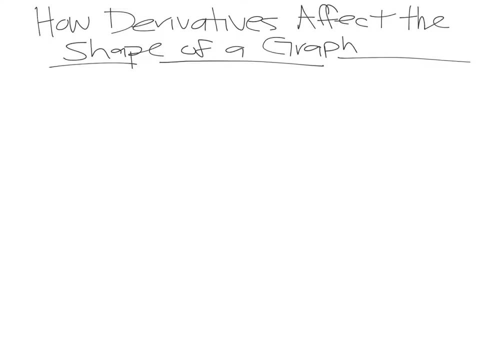 today. we're going to look at how the derivatives affect the shape of a graph. the first thing we'll look at is an increasing and decreasing test we'll look at. the first thing we'll look at is an increasing and decreasing test for the derivative. that's a constant. 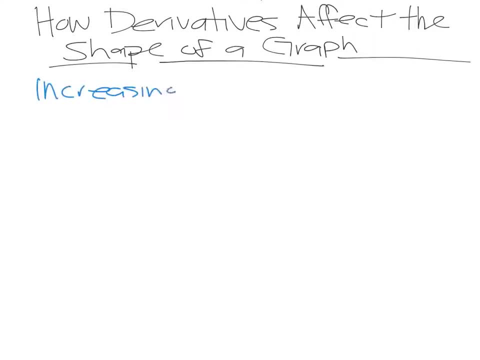 in any case you have to shift x and y to convert it's to c, it, GM, the derivative, and that's equal to g times x. This test says that if our derivative f prime of x is greater than 0 on an interval, then our function f is increasing on that interval. 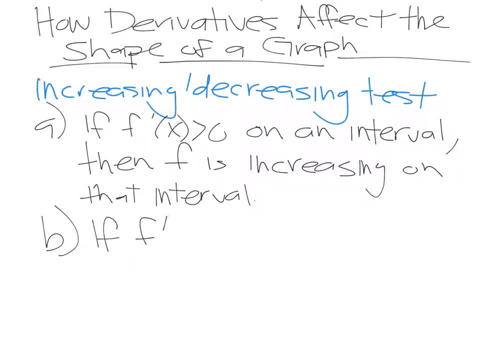 And then b, that if the derivative f prime of x is less than 0 on an interval, then f is decreasing on that interval. And so let's take a moment and think about this: If the derivative is greater than 0. That derivative is the slope, and if the slope is positive it's increasing. 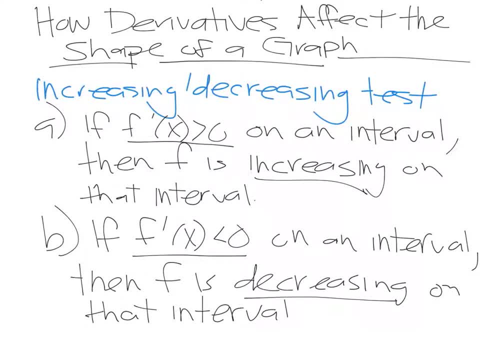 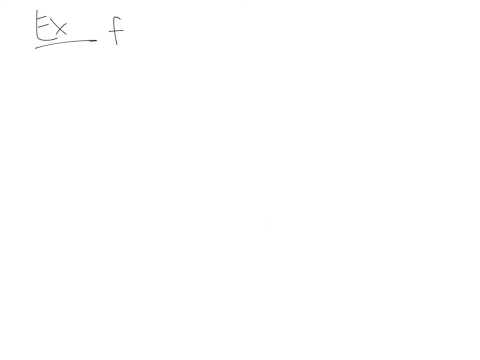 If the slope is negative, it's decreasing. So let's do an example. If we're given the function f of x is equal to x cubed minus 12x minus 5, identify the open intervals in which this function is increasing. 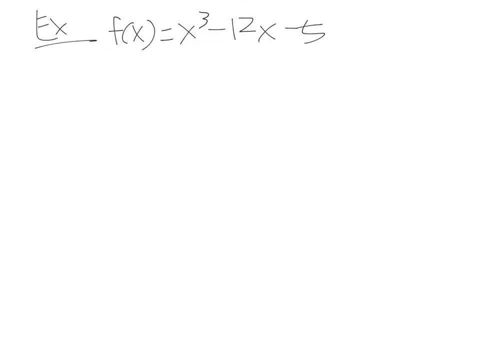 And the intervals in which it's decreasing. So we want to find increasing and the intervals where it's decreasing. If we have a function that say goes up, it increases and then it starts to decrease, that point where it changes, that's one of our critical points. 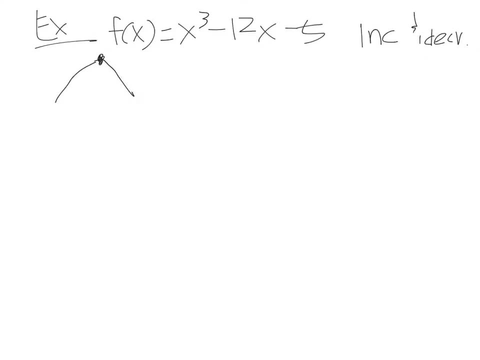 So let's first find the critical points, because then that will tell us where all of these different intervals are. We take the derivative f prime of x, so we get 3x squared minus 12.. That's our derivative. To find the critical points, we set the derivative equal to 0.. 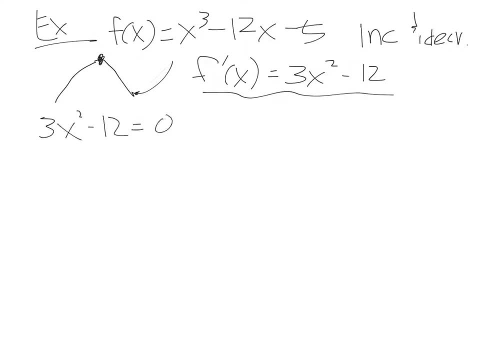 So we get: 3x squared minus 12 equals 0.. Solving for x, we get 3x squared equals 12.. x squared minus 12.. x squared equals 4.. Or x is equal to plus or minus 2.. 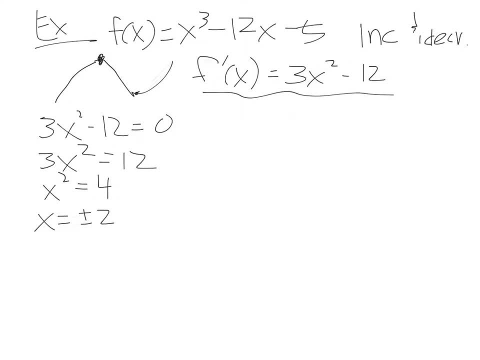 So we have two critical points at negative 2 and at 2.. So if we broke off and looked at this on a number line, we'd have negative 3, negative 2, negative 1, 0, 1, 2, 3, and so forth. 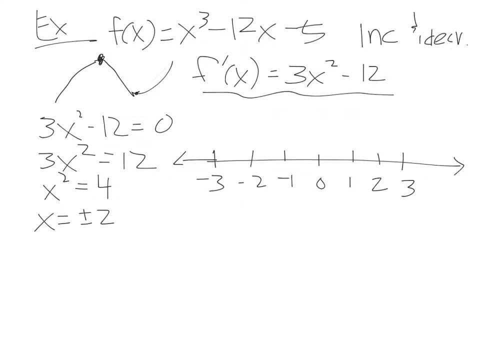 Off to positive and negative infinity. So we'd know we have a critical point at negative 2 and a critical point at positive 2. And since there aren't any other critical points, if we're on this side we're either all decreasing or all increasing. 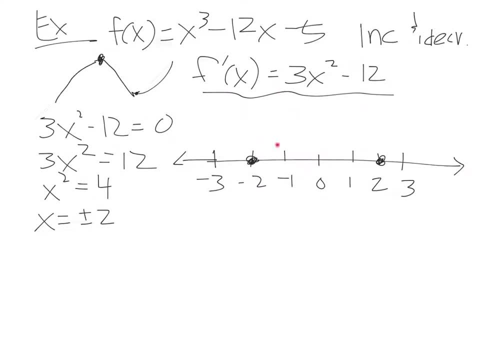 And in this interval all increasing or all decreasing, Because if we're to increase and then decrease again, going up to go down, you must have a local max or a local min. So we're all going to be the same in each of these intervals. 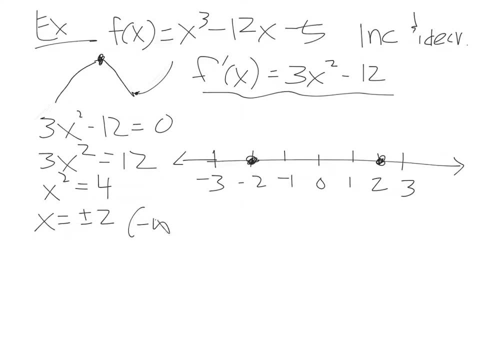 So we have the intervals negative infinity to negative 2, negative 2 to 2, and then 2 to infinity. Now we need to figure out if we're increasing or decreasing, And that is simply just plugging a number in each of these intervals into the derivative. 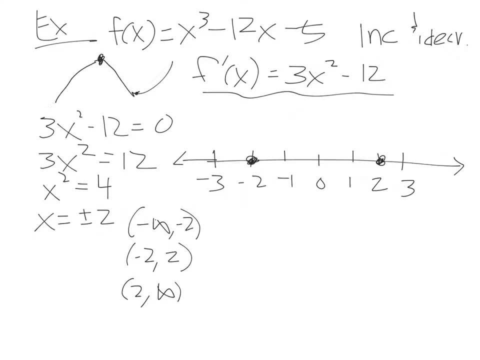 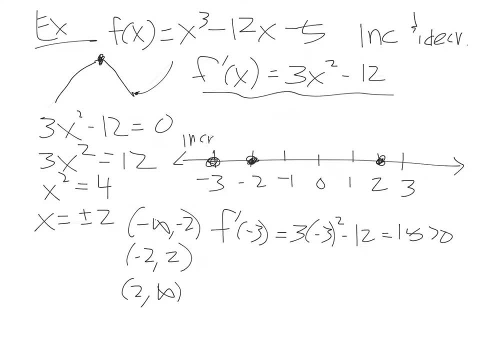 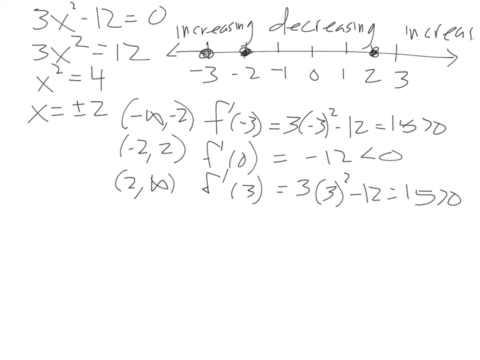 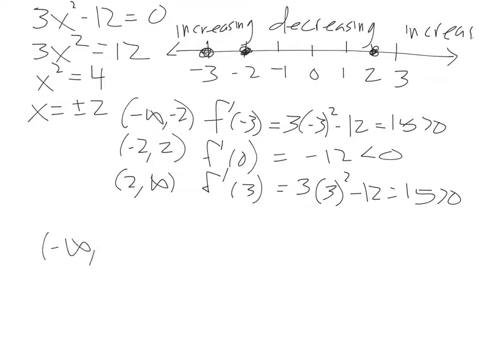 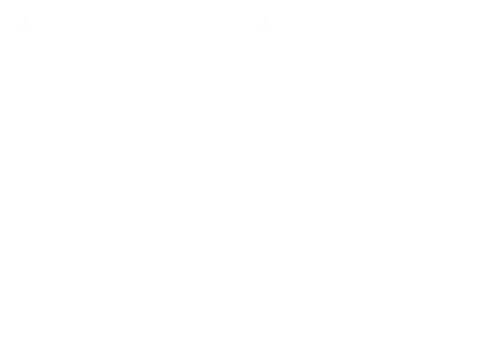 The next thing we'll look at is something called the first derivative test, And what this says is suppose that c is a. 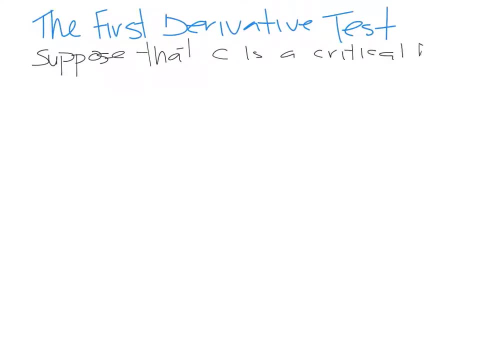 critical number of a continuous function, F. Then the first thing, A says that if F prime changes from positive to negative at the point C, then F has a local maximum at C. The second thing says that if F prime changes from negative to positive at the point C, then 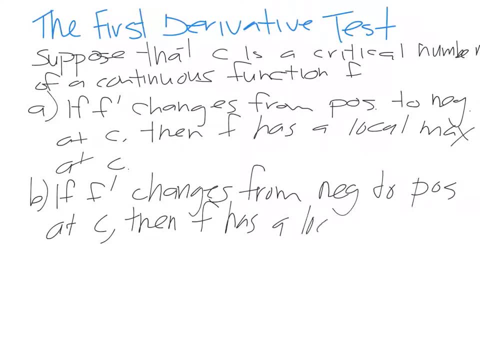 F has a local minimum at C, And so what these are saying is that if we're going from positive to negative, then we have a maximum. If we go from going down to a negative slope to a positive slope, we have a minimum, And then finally C. the third thing says that if F prime is positive, 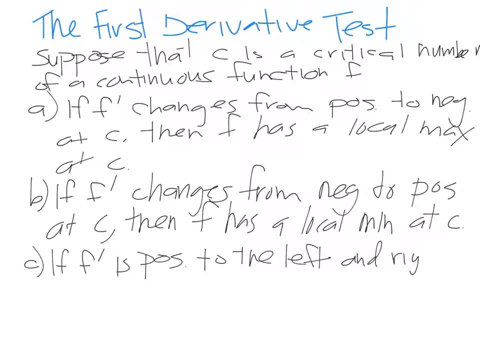 to the left And to the right of C, Or if it's negative To the left And right of C, Then F has Negative To the left And to the right Of C, Then F has No local. 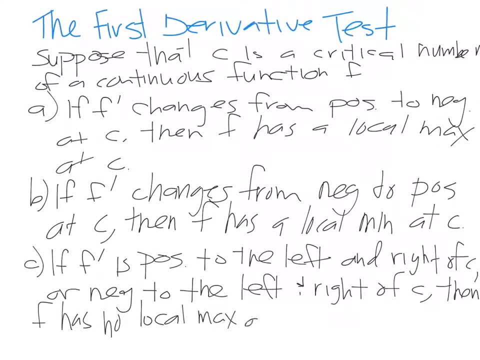 Maximum Or Minimum At C. So If the slope is Both Is positive On both sides of C Or negative on both sides of C, Then it's not a maximum or a minimum. So let's do an example. 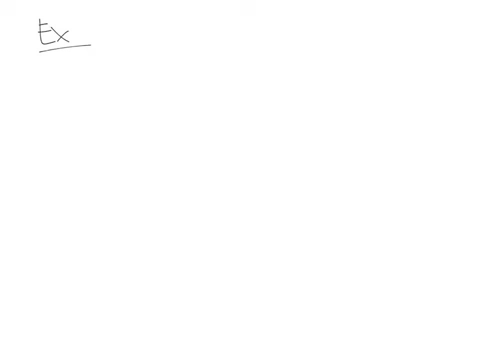 So let's do an example: Find The critical points Of F of X. Equals X to the one third power Times X minus four. Now we could use the product rule, Or what we could do Is just: 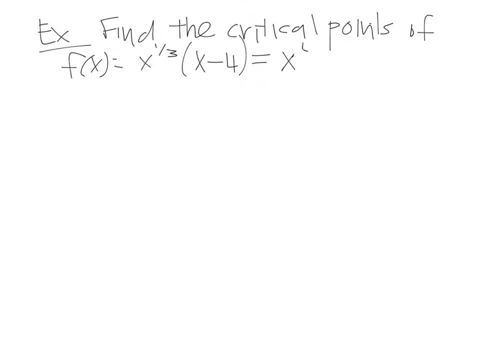 Multiply this out And this would be X To the four thirds power Minus four X to the one third power. Now, in addition to finding the critical points, Let's also identify the intervals Which F is increasing And decreasing. 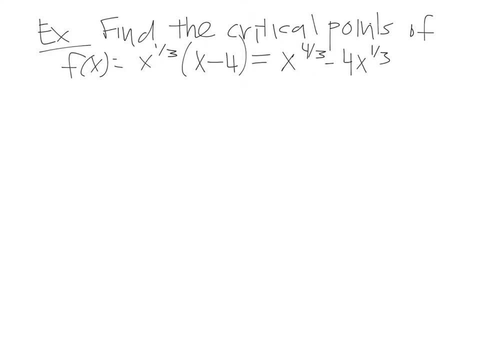 And find The function's local and absolute Extreme values Meaning the maximum and minimum. So the derivative F prime of X Is going to be four thirds X to the one third power, Minus Another four thirds X to the negative. 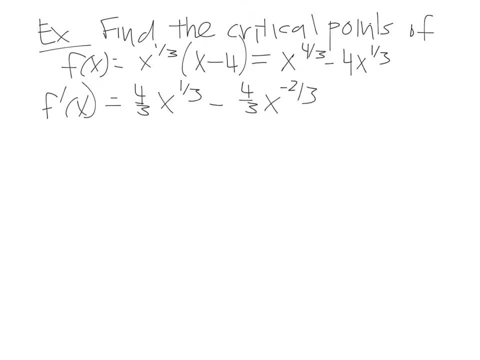 Two power, Or two thirds power, And I got this four thirds By multiplying four Times one third. So to find the critical points, We set the derivative Equal to zero And We set that equal to zero. And so now solving for this. 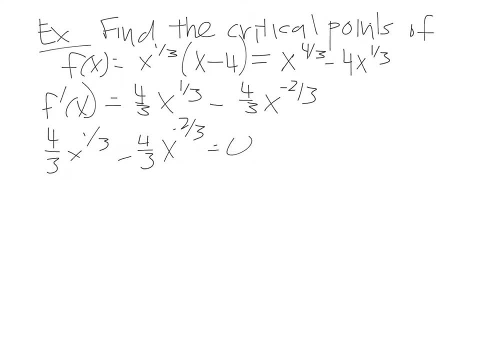 We can Get rid of the four thirds By, Let's say, Dividing everything by four thirds, And so we get X to the one third power Minus X to the negative. Two thirds power Equals zero. Now to solve this. 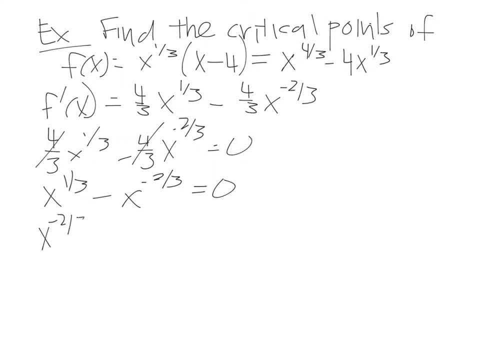 What we're going to do Is we're going to calculate X to the negative two thirds. So if we factored out X to the negative two thirds, From X to the one third, What we would get Would just be. 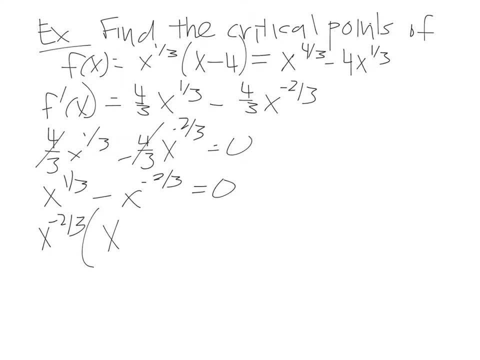 X, Because X to the one Times X to the negative, two thirds Is X to the one. third Minus one Equals zero. So this is X minus one Equals zero. So now, solving for X, We get: X is equal to one. 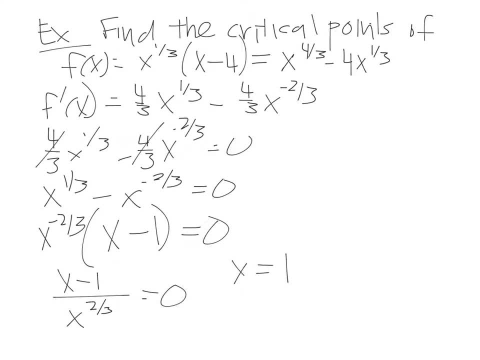 That's the zeros, But also note That we have an X in the denominator, And so that means That X Equals zero Is a critical point, Because a critical number Is when the derivative is zero Or the derivative Does not exist. 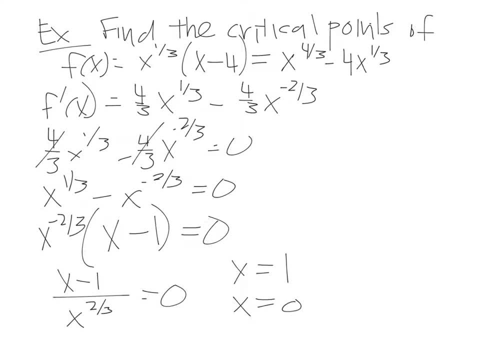 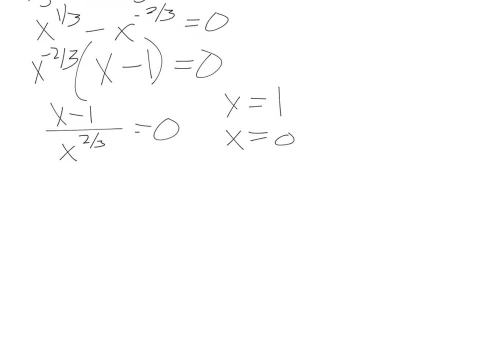 So these are our two Critical numbers. So now we're going to go ahead And make some space And we're going to draw The number line And that number line. So our numbers are zero and one. So we'll start with a point, less than that. 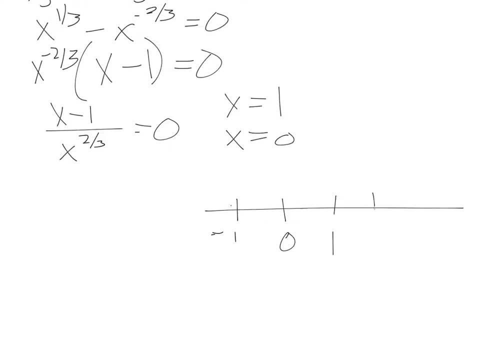 At negative one, Zero one, And we'll go ahead. one more to two. Remember our derivative Of X Is equal To four thirds Times X To the one third power Minus Four thirds X to the negative. 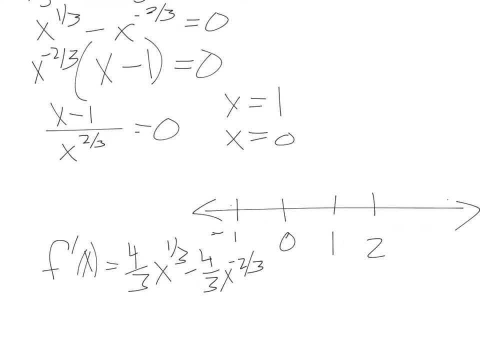 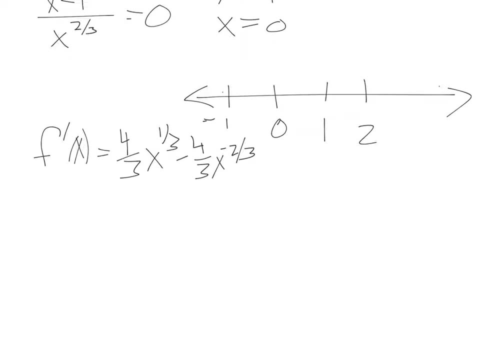 Two thirds power, And we're going to have Three intervals. The first interval Is going to be From negative infinity To zero. The second interval will be from Zero To one And then the third will be from one. 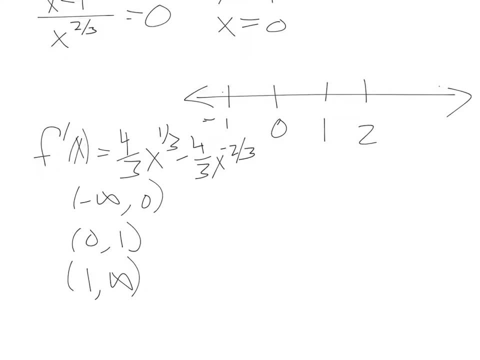 To infinity. So for this first interval We'll pick a point in that interval, Let's say negative one. So we'll check out F prime of negative one, And so we get Four thirds Times One third Minus four thirds. 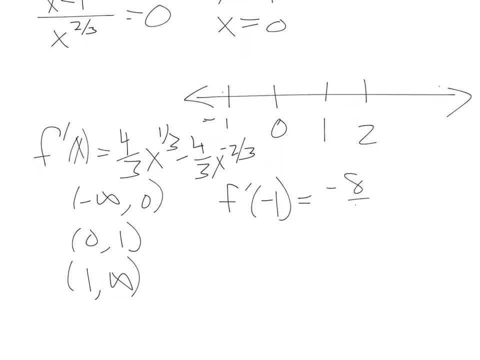 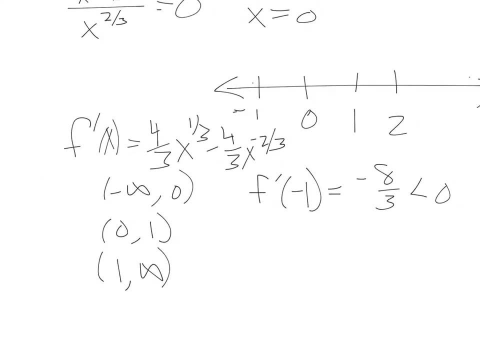 Times negative one to the negative two thirds, We get negative eight thirds, Which is negative. So on this interval right here We have, Since it's negative, It's decreasing, And then we'll pick a point Between zero and one. 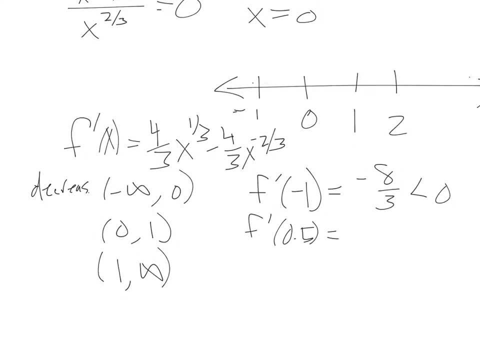 Let's just say, If we were to plug that in, We get that that is Also going to be negative. So this is Less than zero. And since it's less than zero, It's still Decreasing. So just because we have a critical point, 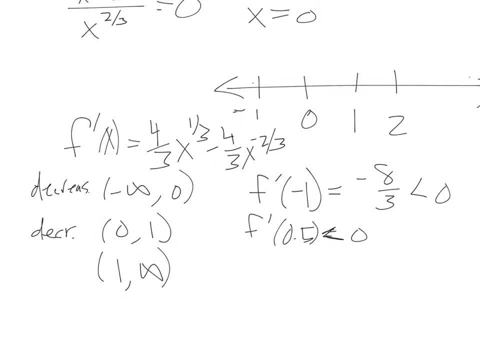 That doesn't necessarily mean That it's a max or min Or that it changes signs. And then, finally, We'll pick a point Two. If we were to plug this in on a calculator, We get that that is Greater than zero. 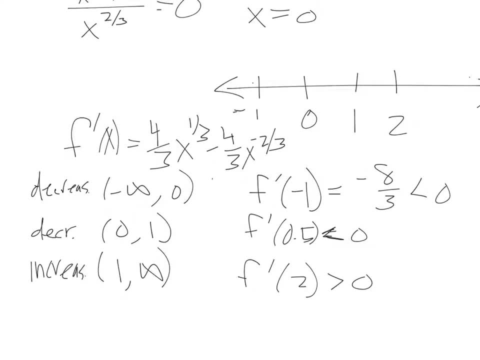 So it's increasing. So here we have The intervals Where it's increasing and decreasing, And we have A local max or min When it changes from increasing and decreasing. So right here, Where it changes from decreasing to increasing, We get that one. 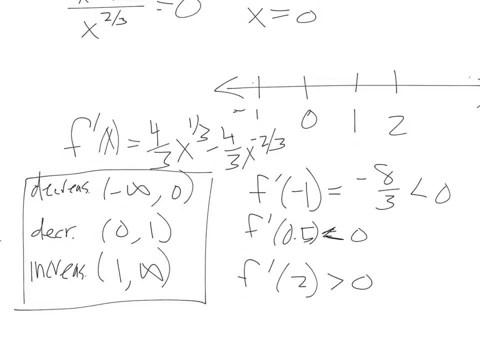 Is A local. It's going to be a max or min. So if you go from going down, Going up, We have a local minimum. So we have local Minimum At x equals one, And so the value of that. 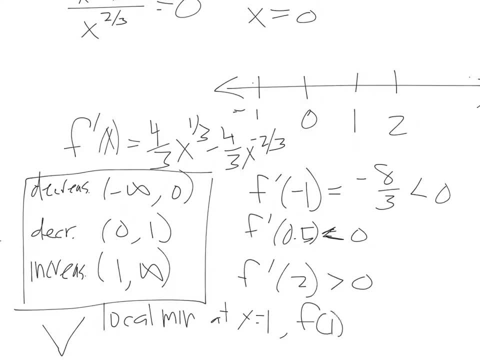 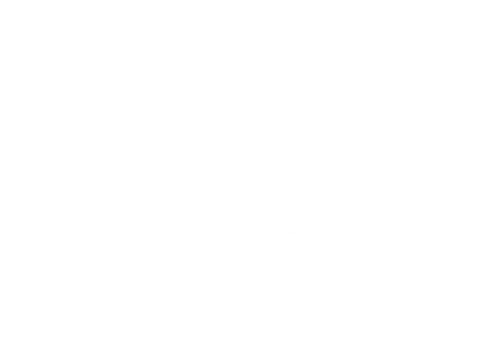 Plugging in F of one. What we get Is f of one is negative three. So that's The value Of the local minimum. So we've looked at What the first derivative tells us. Now we'll take a look. 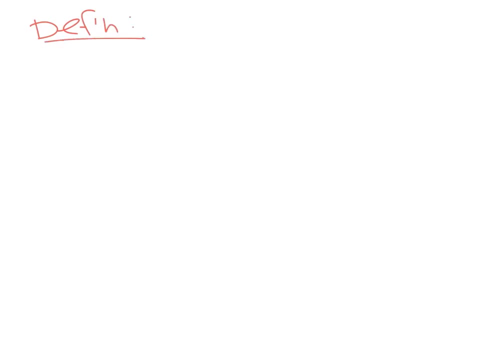 At what the second derivative Tells us. But first we'll begin with the definition. And this definition states That if The graph Of f Lies above All of its Tangents On an interval, Let's call this interval. 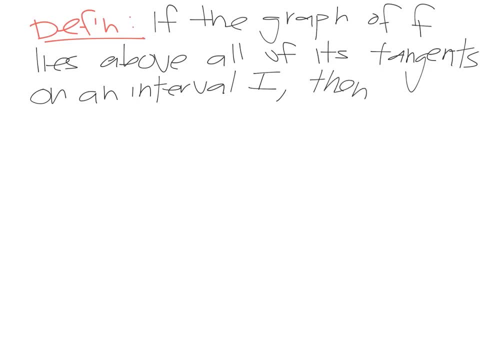 I. Then We say It's called Concave Upward On that Interval I. And then Similarly, If the graph Of f Lies Below All of its Tangents On an Interval 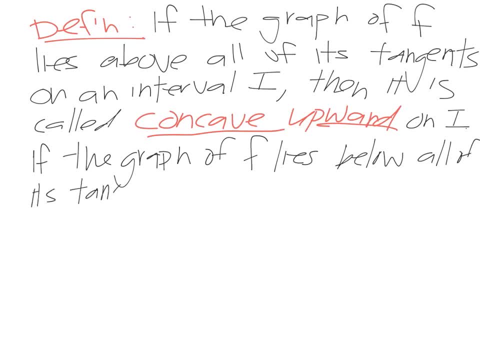 I Of f Lies Below All of its Tangents On an interval I. Then It is called Concave Downward On that interval I. So what does that even mean? So let's take a look. 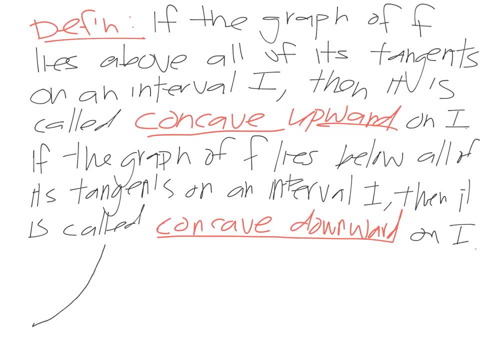 If it's concave up, If we have a graph that looks like this, And this is our graph f, Where are all the tangent lines? The tangent line goes this way. The tangent line goes this way. The tangent goes this way. 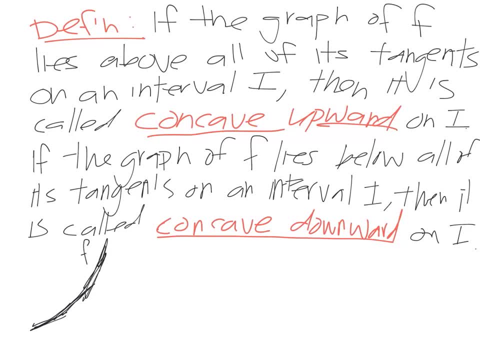 And this way And so forth, And each of those tangents f is going to be above the tangents. So Now, if we have a graph That goes like this, Let's call this graph g. We'll have a tangent that goes like this: 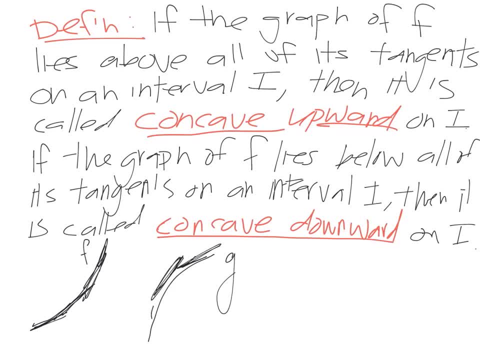 Tangent that goes like this Tangent that goes like this, And in each of these cases g, Our function is going to be below The tangents. And so This first one, This is concave up And this is concave. 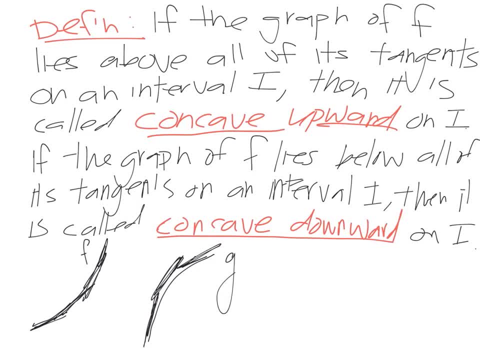 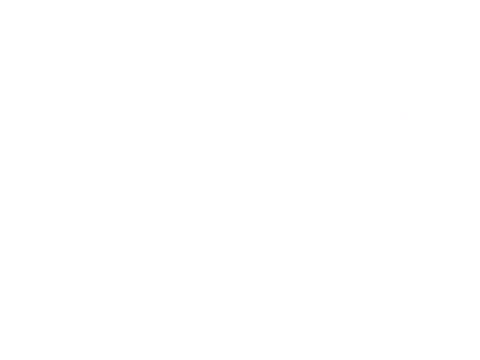 Down. So now we know What the definition of concavity is. Let's actually Figure out how we test for it. So The concavity test Goes as follows: We're going to A If you take the second derivative. 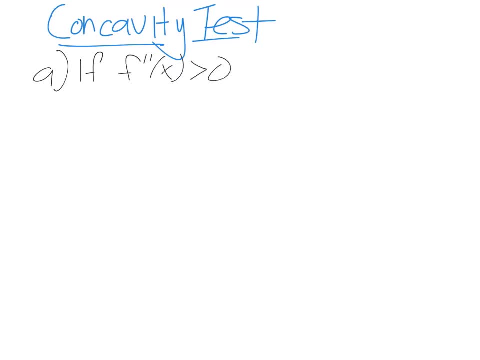 f, double prime of x, And if that derivative Is greater than zero For all x In that Interval i, Then The graph of f Is concave Upward On your interval i And then b. If 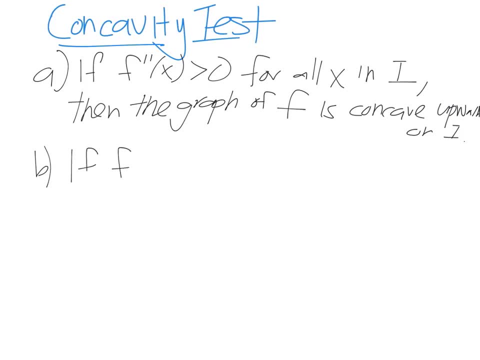 The second derivative of f Is less than zero For all x In the interval i, Then the graph Of f Is less than zero For all x In the interval i, Then the graph Of f Is concave. 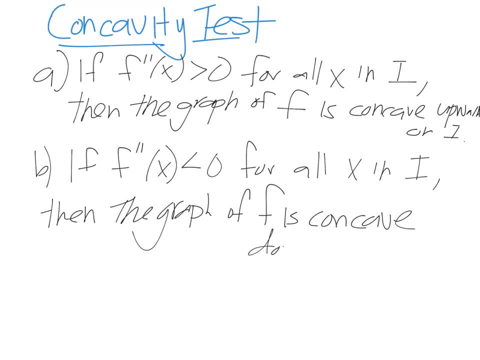 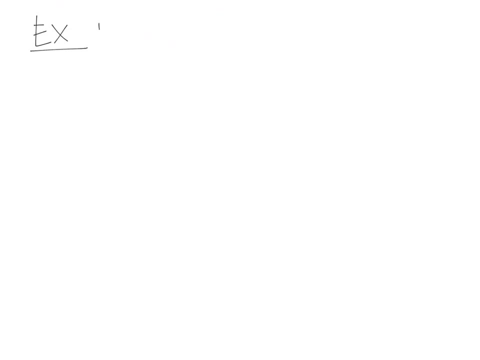 Downward On that Interval i. So let's do an example. If we have the curve Y Equals x cubed, Now that graph, You may Be familiar with that Because We have the curve Y And the cubic function. 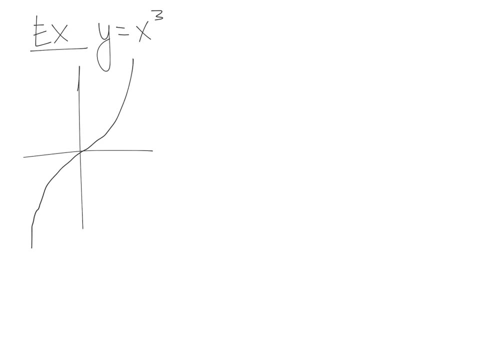 Looks something like this. So let's figure out When it's concave up And concave down. So if we call this our function f of x, First thing we do Is take the first derivative F, prime of x, So we get 3x squared. 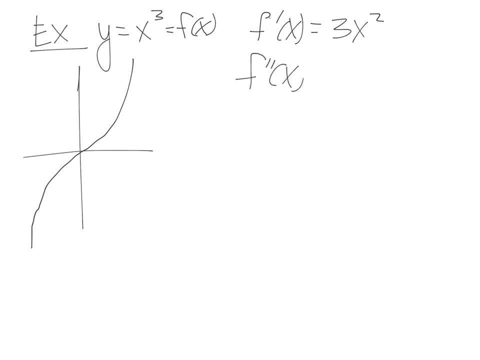 And then we take the second derivative, F, double prime of x, And so we get 6x. We want to find When this derivative Is going to be positive Or negative. Well, We know that This derivative Is going to be positive. 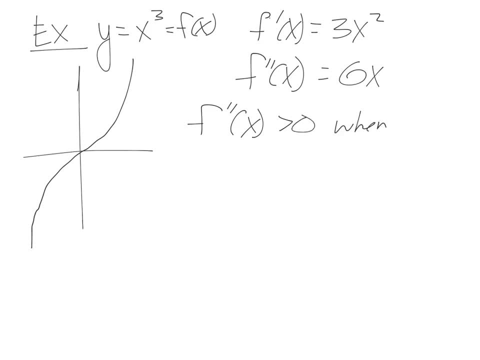 When X is going to be From zero To infinity. As long as x is positive, The second derivative is positive. Your second derivative Is negative When X is between Negative infinity And zero. So it's going to be concave up. 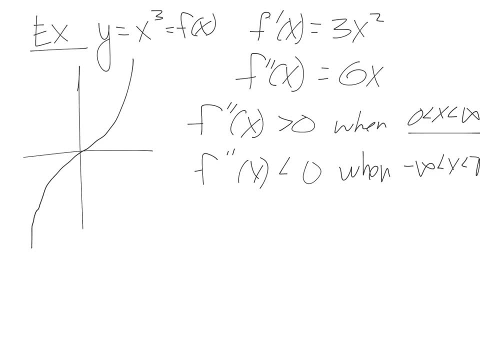 So that tells us, This is concave up, Concave up From zero to infinity, Concave down From negative infinity To zero. So if we look at here, From zero to infinity, We see it does have that Upward motion. 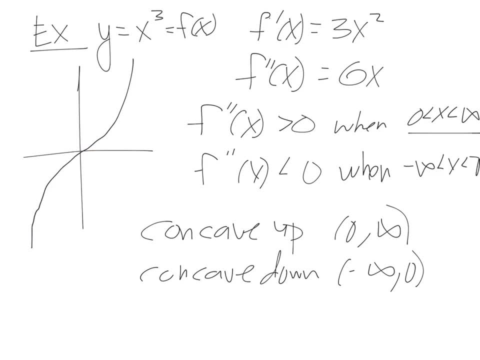 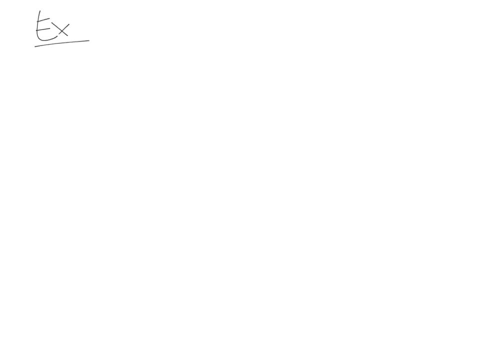 Or the upward appearance, And then we have that concave down From zero to negative infinity. We'll do another brief example, And this is: the curve F of x equals X squared. We know this is the parabola. So take the first derivative. 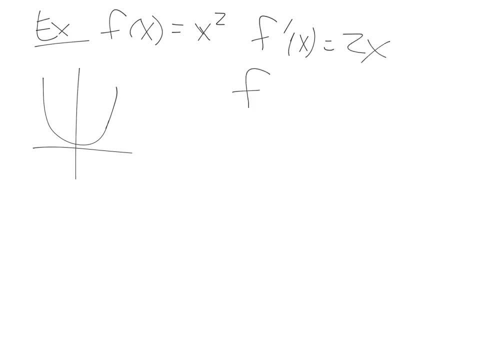 F prime of x Is two x, And the second derivative Is just going to be two. Well, we know, two Is always greater than zero. If that's always greater than zero, Then this curve is always Concave up, Meaning concave up. 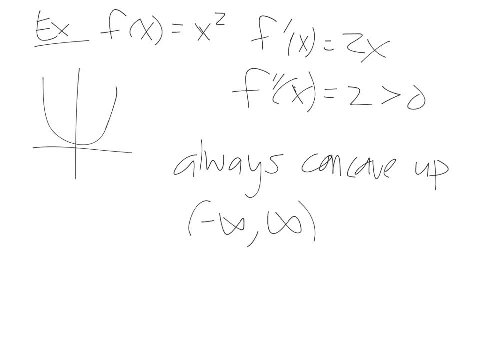 From the interval Negative infinity to infinity. And take a look at this: This curve is going to be Concave upwards. Now we have another definition, And what this definition states Is A point P On a curve, Y is equal to. 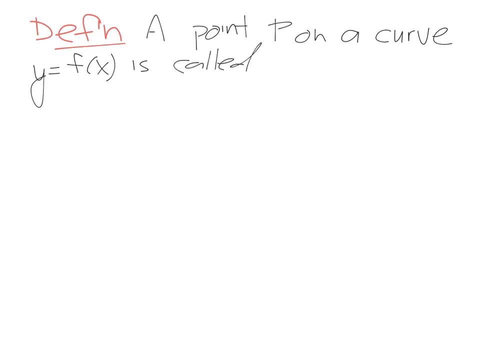 F of x Is called An inflection point If F Is continuous there. So at that point And The curve Changes From concave up To Concave down Or vice versa. So Or changes from. 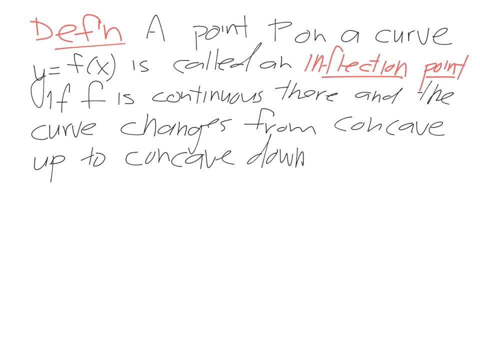 The curve To Concave down Or vice versa. So Or changes from Concave up To Concave, down To Concave up, So as long as the Concavity is changing, Then we have an inflection point. 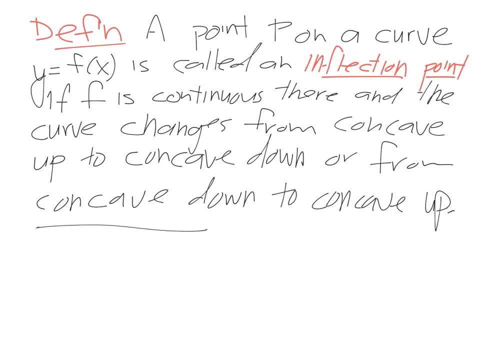 So now, If you recall from the example That we had just done, Where we had y Is equal to x, cubed At zero, The graph of this. It went like that. It went like this In this region, It was concave. 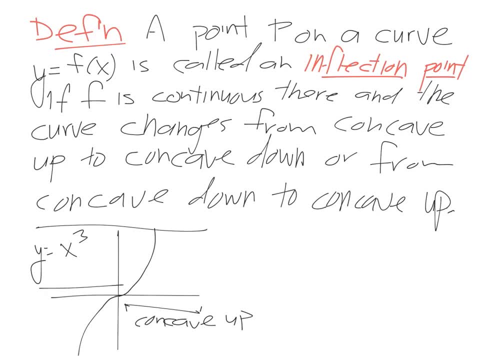 Up In this region It was Concave Down, And so that point where it changes From concave up to concave down, That Is the Inflection Point Right here, where it changes From concave up to concave down. 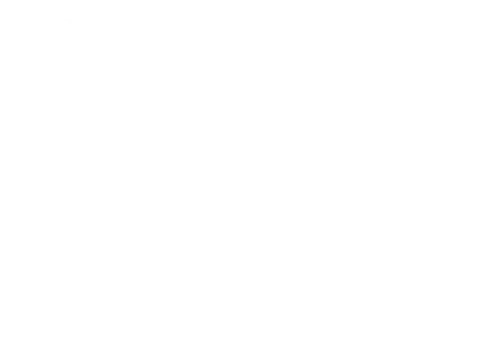 So you can kind of see it right there Drawn on the graph. And finally, today We're going to talk about The second Derivative Test. The second derivative test States the following: Suppose F double prime Of x. 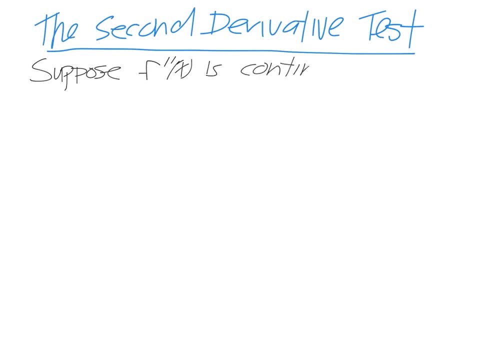 So the second derivative Is continuous Near the point c, Then we have two things. If F, prime Of c Is zero, So if the first derivative is zero, Meaning it's a critical point, Then we have two things. 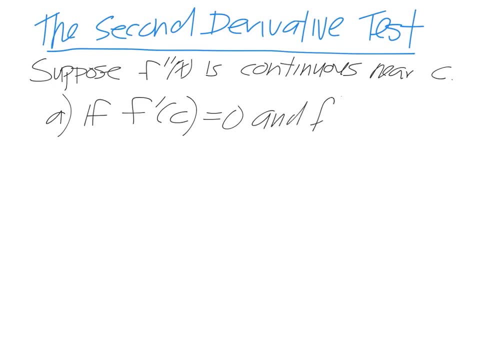 If The second derivative At the point c Is greater than zero, So meaning it's concave Up, Then F Has a Local Minimum At the point c, So And then b, If F prime of c. 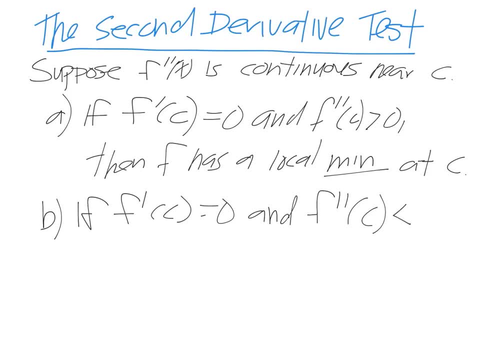 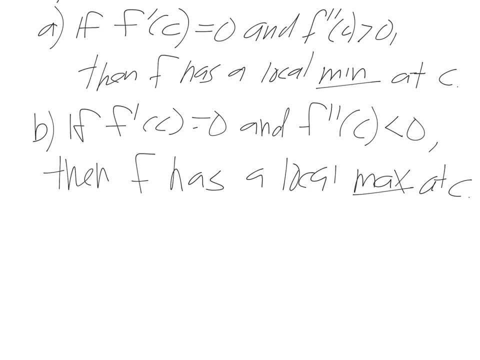 Is zero And f double prime of c Is less than zero, Then F has A local Maximum At c. So If we were to have a curve And say we have a curve That looks like this F prime. 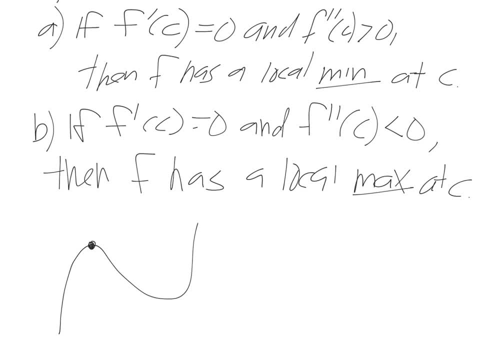 At c Is zero, So the derivative Is zero. These two points: we have derivatives And the derivatives are zero. Now we look at the second derivative. Is it concave up Or concave down? Well, right here it's concave. 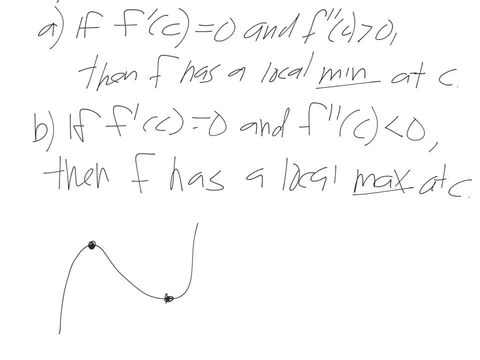 Down, Then it has a Maximum. Right here it's concave Up. So if it's concave up, Meaning second derivative is positive, Then it's a minimum And also you can notice, You may notice about right here: 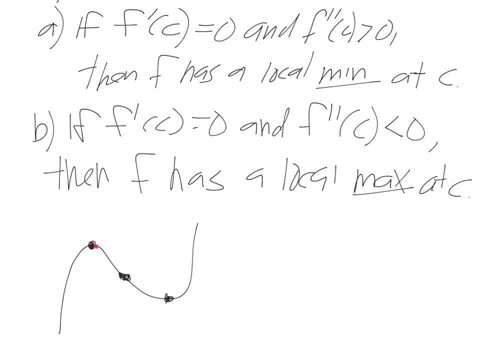 The concavity switches. That's the inflection point. It goes from Downward To upward And finally, If it's equal to zero, Well then this test doesn't really tell us anything. It could be a local max, It could be a local min. 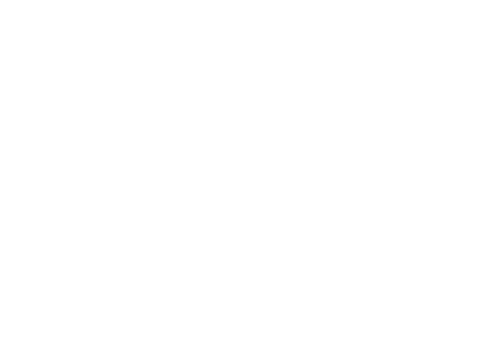 Or it could be neither, So we don't really know. So let's do an example. F of x is equal to X to the four Minus four, x cubed Plus ten. We'll take the first and second derivative. 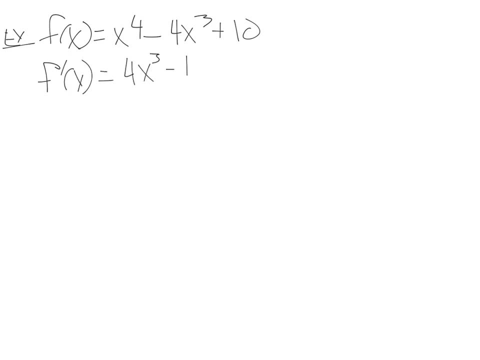 First derivative: X cubed Minus twelve X squared. The second derivative Is twelve x squared Minus twenty four X. To find the critical points, We want to set the first derivative equal to zero. We get four x cubed. 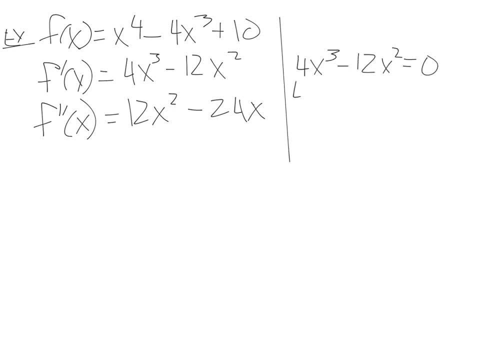 Minus twelve x squared Equals to zero. We can factor out four x squared And we're left with X. Three equals zero. So we have Critical points. are x equals zero And x equals three? Plugging these two points in. 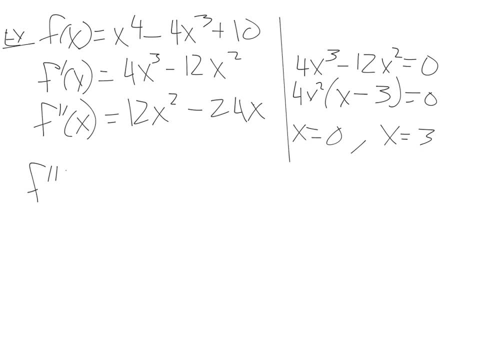 Into our second derivative, We get f double prime of x. We'll put in the first point zero. So f double prime of zero Is just going to be zero. Well, that doesn't really tell us anything, But that's alright. We plug the second point. 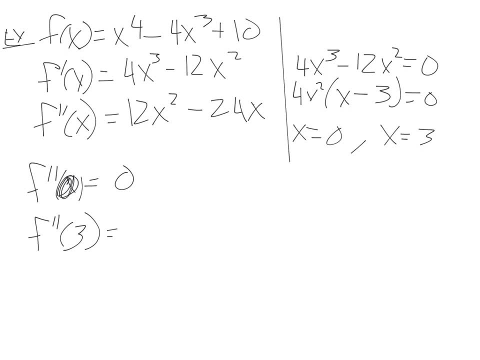 F, double prime of three In. And then what we get is We get twelve Times three, squared Minus twenty four Times three, We get thirty six, Which is positive. So if the second derivative Is greater than zero, 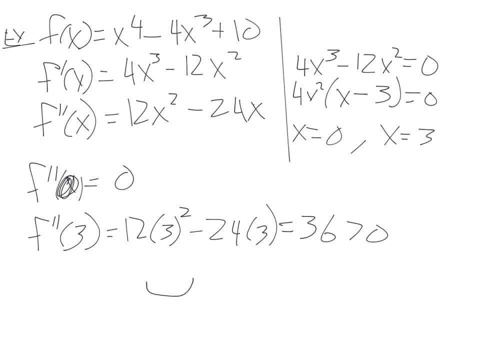 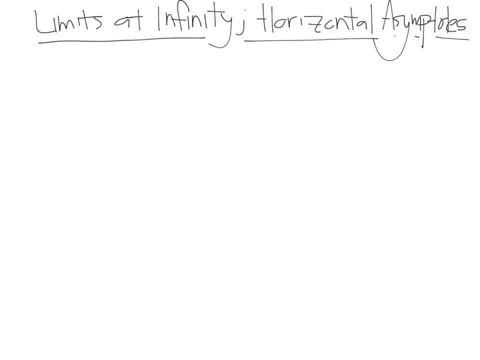 Meaning it's concave upward. So we have something like concave upward. That means it's a minimum. So x Equals three Is At The minimum. Today we're going to talk about The limits at infinity, As well as the horizontal asymptotes. 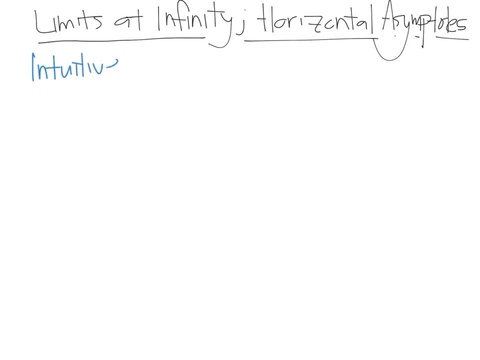 So we'll begin With an Intuitive definition Of A limit At infinity. Let f Be a function Defined On some interval. Let's call this interval A To infinity, Then The limit As x. 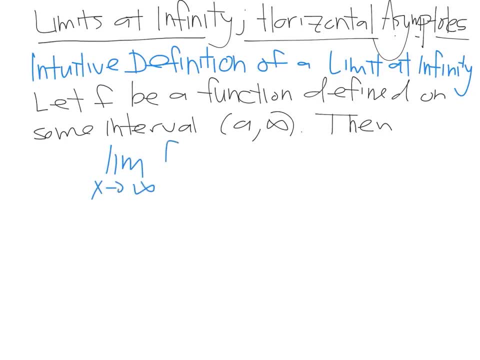 Goes to infinity, Of F of x Equals. l Means That F of x Is That The values Of F of x Can Be Made Arbitrarily Close To The Value. 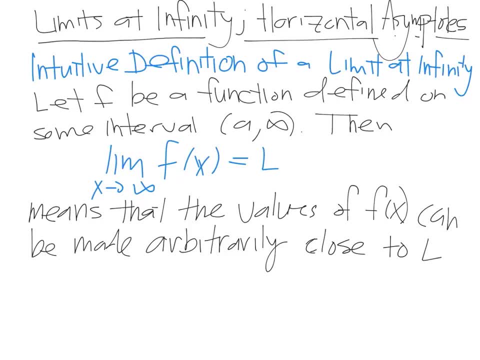 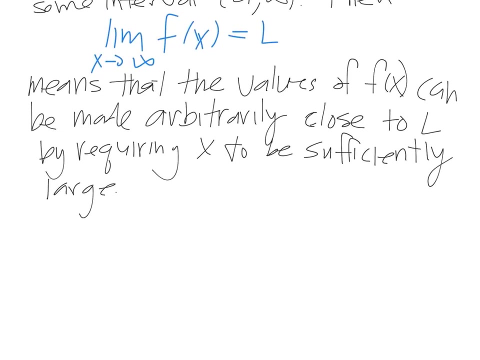 Of L At infinity By Requiring X To be Sufficiently Large. Now Another Notation For This You Might, As X Goes To Infinity Of F. 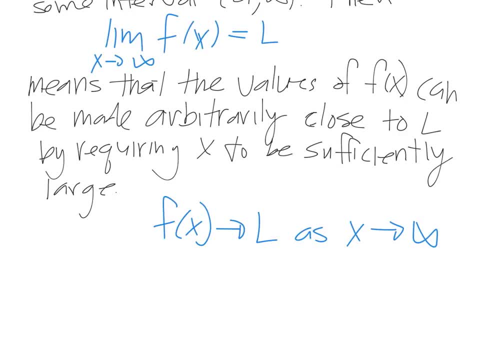 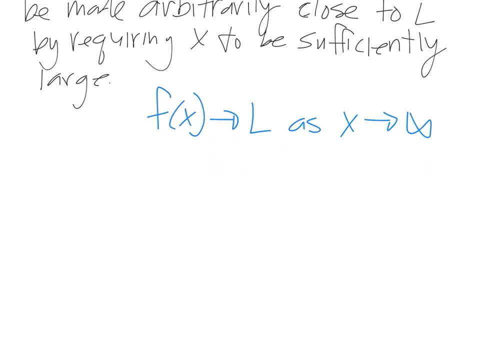 Of X Equals L. You Might Also See The Line Y Equals L. You May Have The Graph. Do Something Like This Is Something Else You. 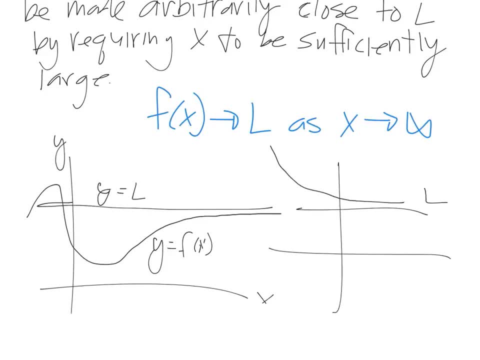 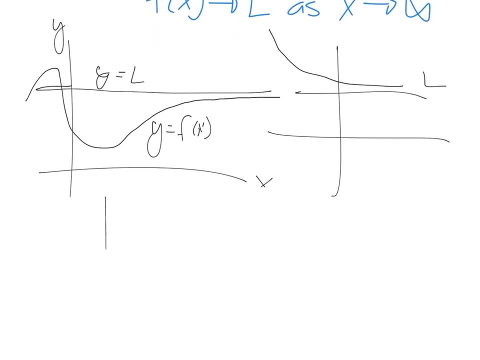 Might See Something Like: And Where. This Is L The Function Might Look Like That, Or Even Something That Oscillates. You Might Have Something Where. 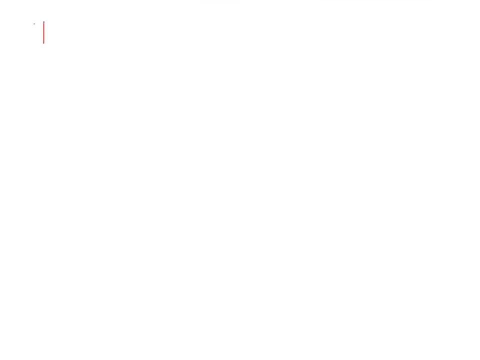 This Is Next. We Have A Definition. This Says That Let F Be A Function Defined On Some Interval Negative Infinity To A. Then We Write: 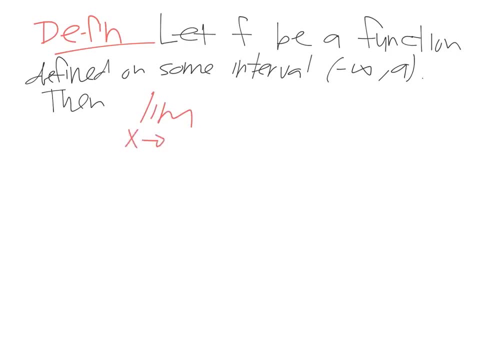 The Limit As X Goes To Negative. Infinity Of F Of X Is Equal To L, And Likewise This Means That The Values Of F Of 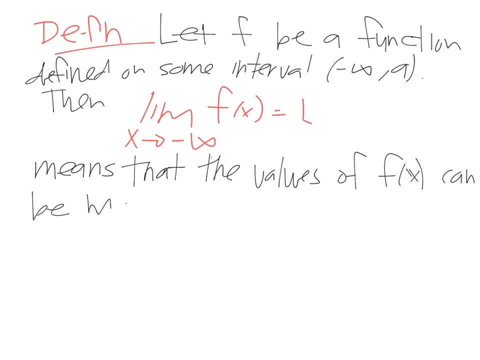 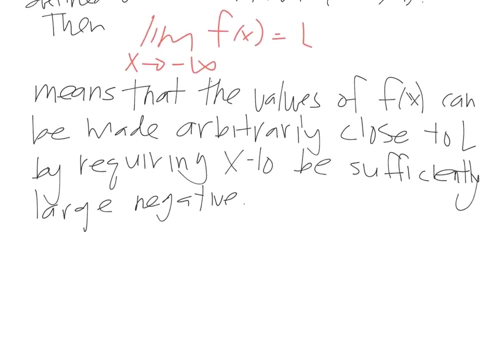 X Can Be Made Arbitrarily Close To L By Requiring X To Be Sufficiently Large In The Negative Sense, And So What That? 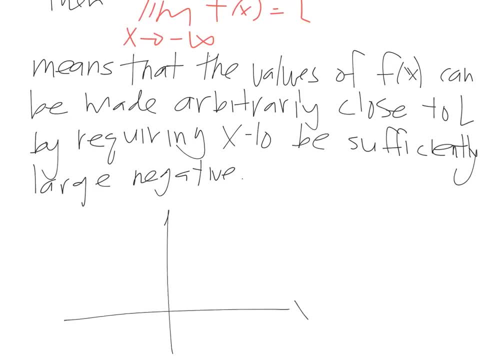 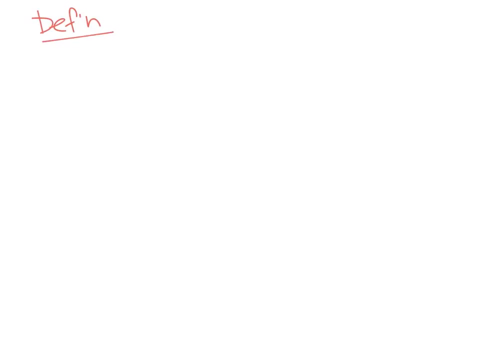 Could Look Like Graphically Would Be: We Have X And A Like That Going Towards L, All The Way Negative. Now We Have A Third. 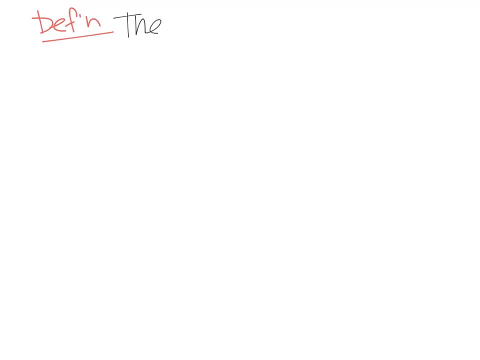 Definition And This Definition States: The Line Y Equals L Is Called A Horizontal Placental Of The Curve. Y Equals F Of X If Either 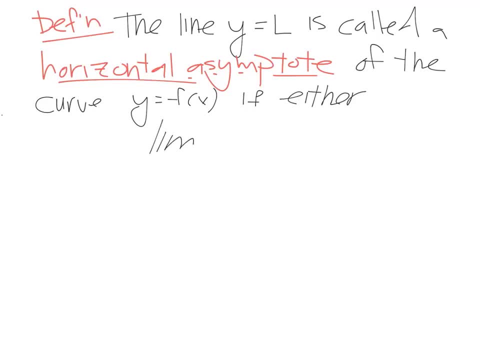 One: The Limit As X Approaches Infinity Of F Of X Equals L, Or The Limit As X Approaches Negative Infinity Of F Of X. 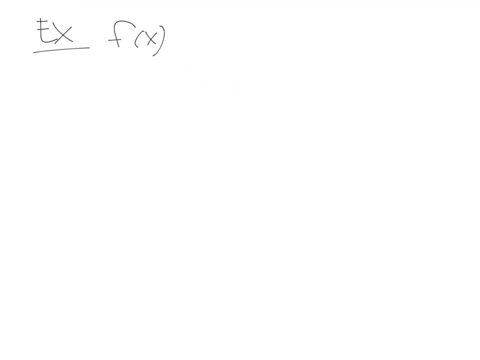 Is Equal Of X Is Equal To X Cubed Minus Two, Divided By The Absolute Value Of X Cubed Plus One. The Graph Of 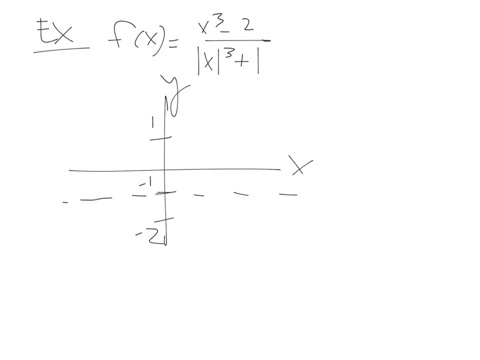 This Looks Something Like The Following, And So What We Can See Is That The Limit As X Goes To Infinity Of This Function As It. 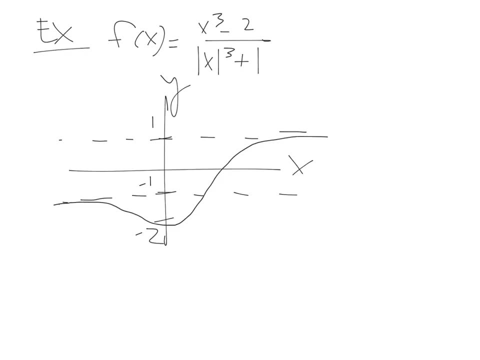 Goes To Infinity. We Approach One And The Limit. If R Is Greater Than Zero Is A Rational Number, Then The Following The Limit As X. 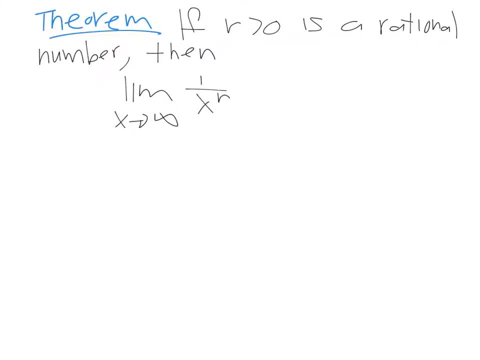 Goes To Infinity Of One Over. X To The R Is Greater Than Zero, And This Is A Rational Number, Such That X To The R 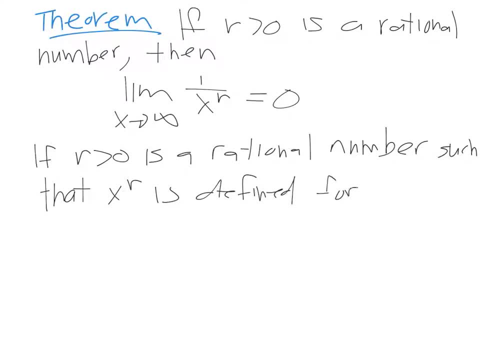 Power Is Defined For All X And The Limit As X Goes To Negative Infinity Of One Over X To The R Is Equal To Zero. 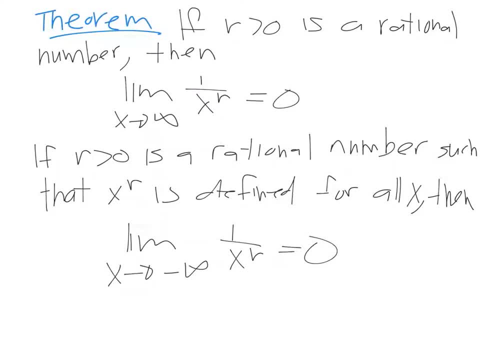 And So Thinking About This For A Moment, X Small. And So, As This Goes To Infinity, This Goes Towards Zero, And Similarly In This Case, 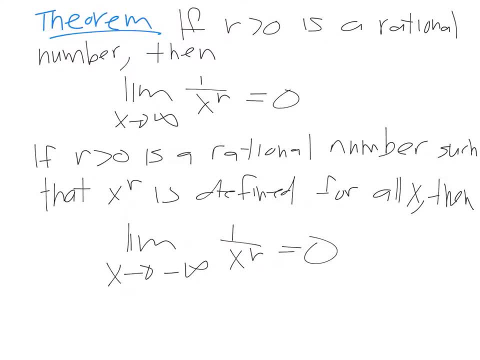 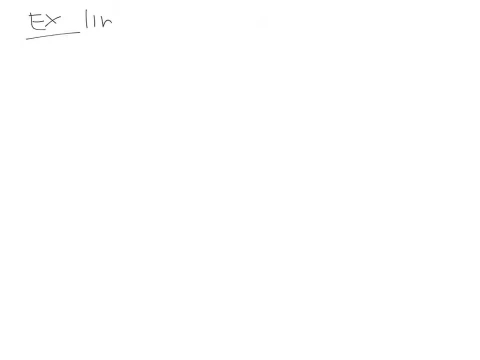 A Negative Number, Raised To A Very Of A Very Large Limit, As X Goes To Infinity, Of The Quantity Five X Squared Plus Eight. 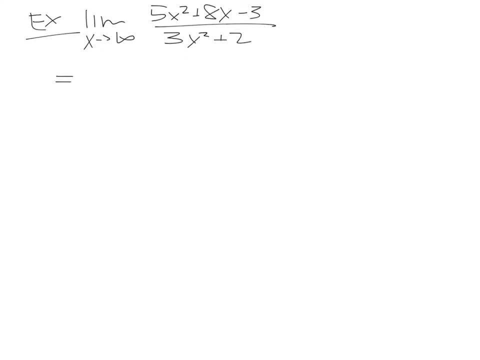 X Minus Three, All Over Three X Squared Plus Two. So What? We're Going To Divide Every Term By X Squared, So Five X. 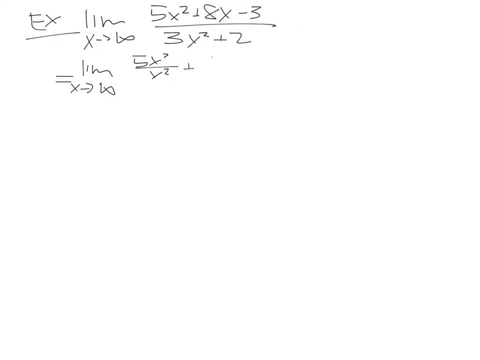 Squared, Divided By X, Squared Plus Eight X Divided By X, Squared Minus Three Over X. Squared All Over Three Over X. 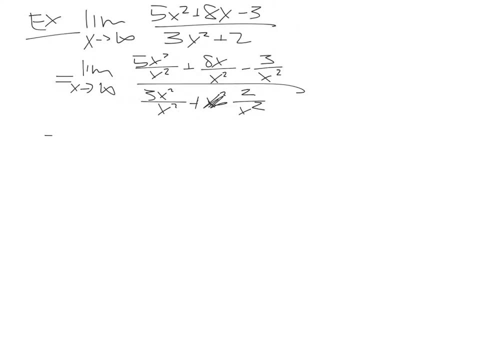 Squared, And Then This Will Equal The Limit, As X Goes To Infinity, Of Well, Five X Squared Over X Squared Is Just Going. 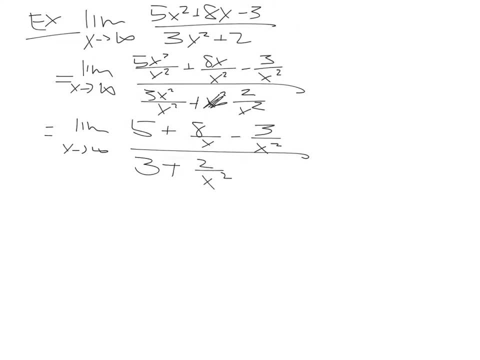 To Be Five. Now We Can Actually Take The Limit And Of Each Of These Individual Components, And So This Is Equivalent To The Limit, As 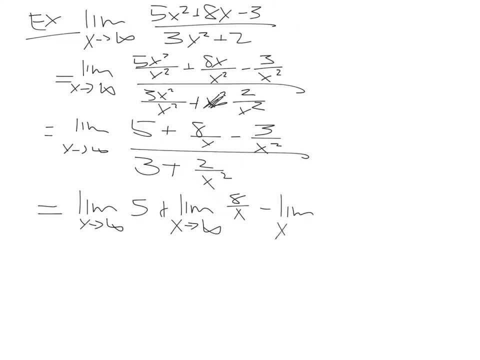 X Goes To Infinity Of Five Of Three Over X Squared Is All Divided By The Limit As X Goes To Infinity Of Three Plus. 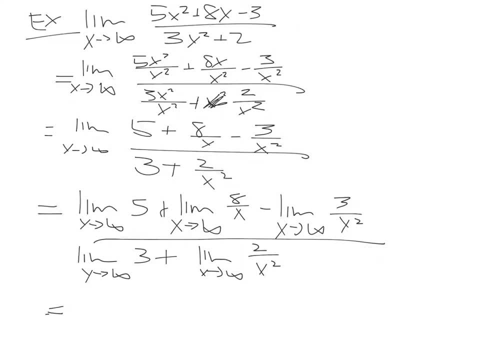 The Limit, As X Goes To Infinity, Of Two Over X Is Equivalent To The Limit Of X And The Limit Is Zero Of X Is. 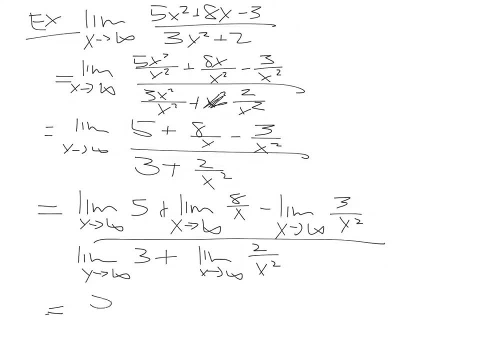 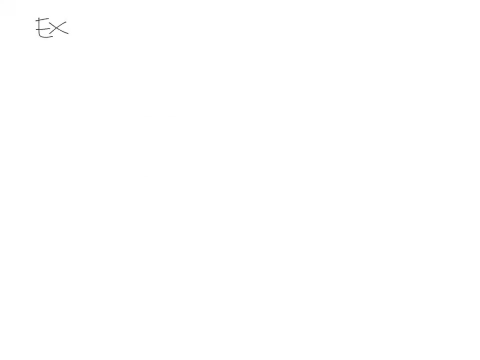 Five Plus Zero Plus Zero Divided By Three Plus Zero, And So Your Limit As X Goes To Infinity, Of The Quantity X Minus The 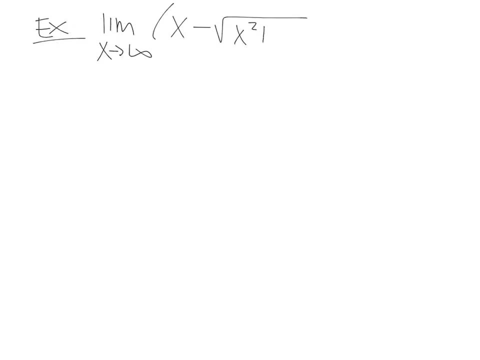 Square Root Of X, Squared Plus Sixteen. Well, What Do We Do Here? It May Not Be By The Conjugate Over Itself, So 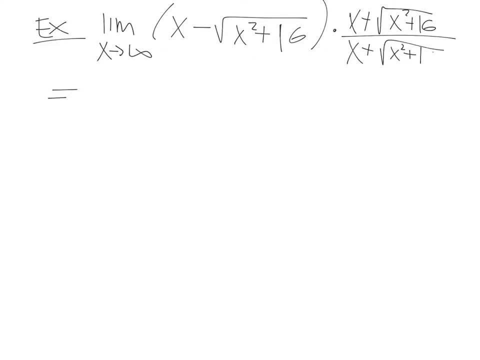 X Squared Plus Sixteen And Divided By X Plus The Square Root Of X Squared Plus Sixteen, And So This Becomes The Limit. 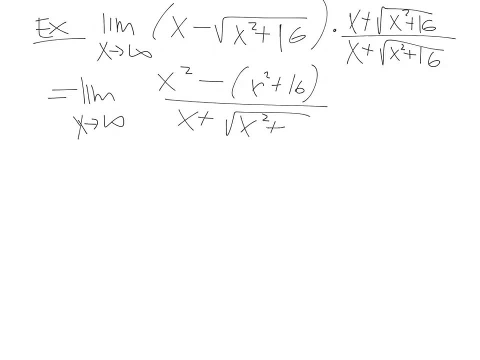 For X Plus The Square Root Of X Squared Plus Sixteen, And This Simplifies The Numerator, Simplifies Our X Squared Will Cancel And 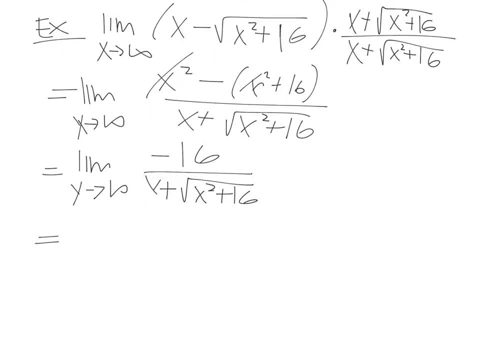 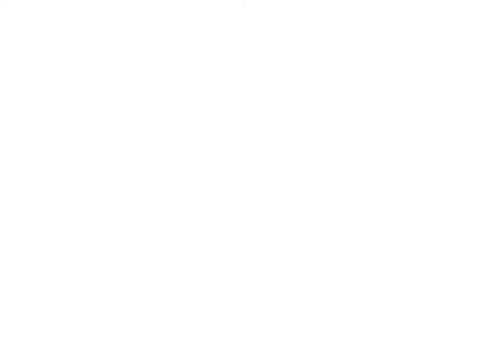 So This Is The Limit, As This Denominator Is, Of Some Power X Being Positive, And So This Is Just Going To Be Zero And 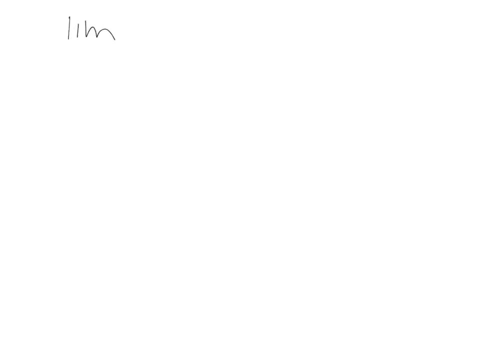 That's Your Limit. Now We're Going To Take A Look. And If This Equals Infinity. So This Is Used To Say That If Our Function 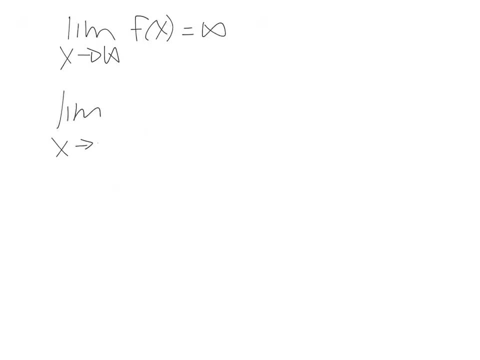 F Becomes Large As X Becomes Large. Similarly, We Might. We Might Also Have A Of F, Of X Is Negative, Infinity Or The Limit. 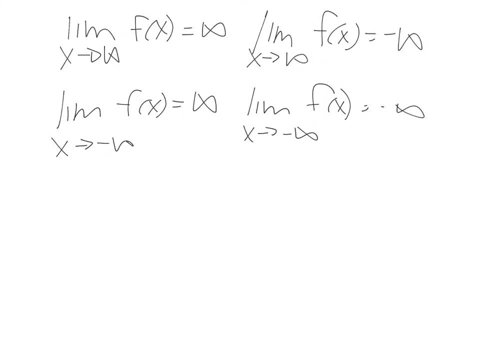 As X Goes To Negative Infinity Of F, Of X Is Negative Infinity. So An Example Of This Might Be: As X Goes To Infinity Of. 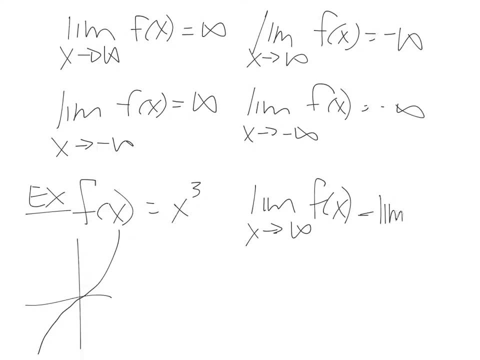 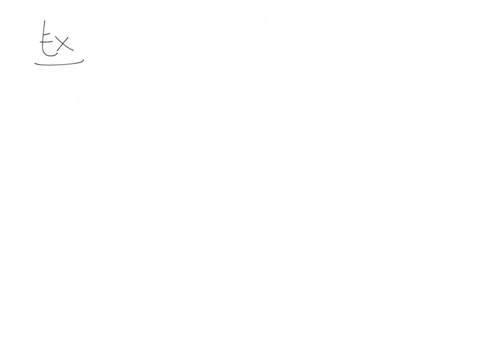 F Of X Or Of X Cubed Is Going To Be Positive Infinity, But The Limit As X Goes To Negative Infinity Of X Is: 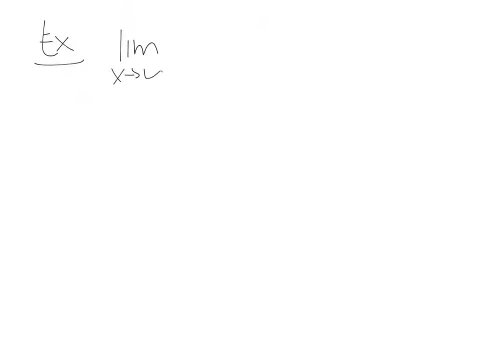 As X Goes To Infinity, Of The Quantity X Squared Minus X, If You, If We Were To Use The Law Of Limits- And I'm 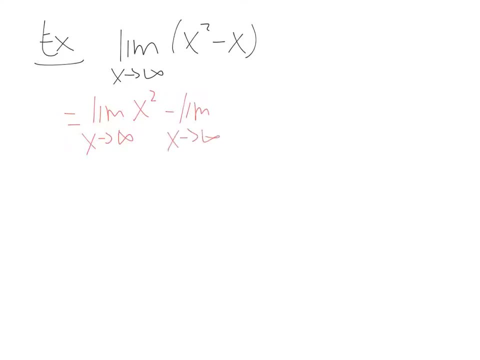 Actually Going As X Goes To Infinity Of X, And So This Is Infinity Minus Infinity. We Cannot Do This, Because Infinity Is Not A. 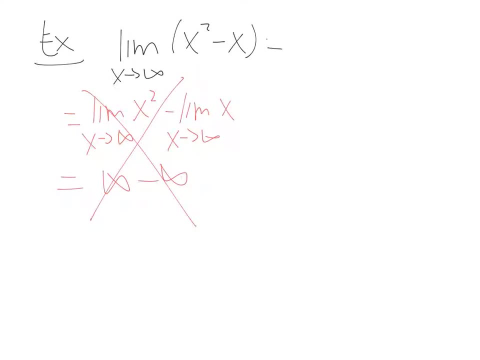 Number, There's No Number. Infinity, You, As X Goes To Infinity. Of The Quantity, X Times X Minus One. And Now, Because We're Multiplying, 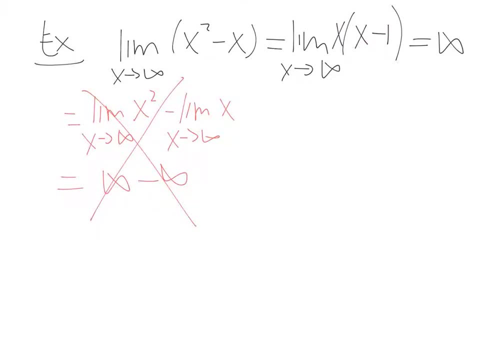 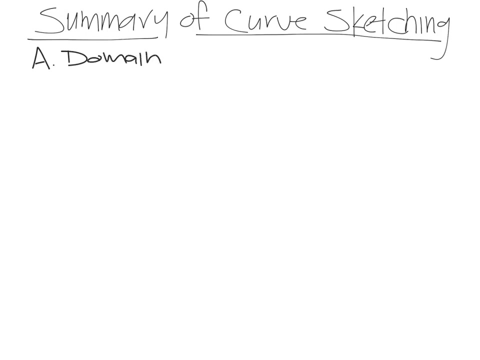 Two Things. This Limit Is Going To Be Infinity. Both Of Z. Everyone. No X X, One Z. I Have A Number Of X Times X. 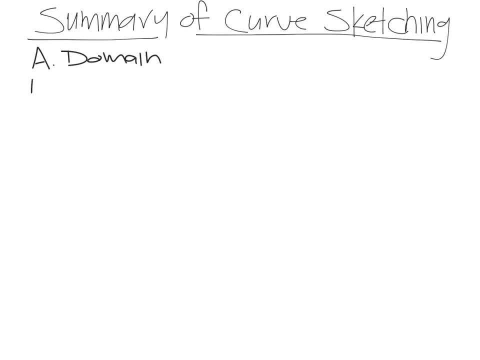 Minus Infinity, X, X, X, Minus X, X, Minus X, X, X, X, X, And they include both the x and the y-intercept. To find the x-intercept, that's when it crosses the x-axis, you set y equal to 0.. 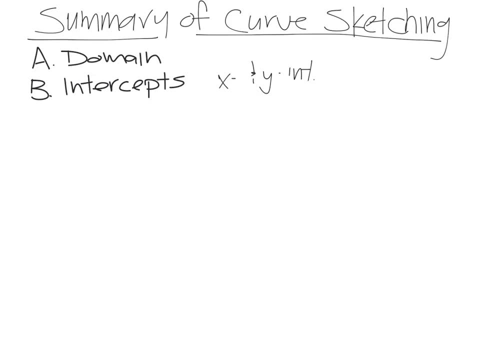 And to find the y-intercept, you set x equal to 0. The next thing we do is you check for symmetry. Checking for symmetry, we want to see if f of negative x equals f of x. If that's the case, then the function is going to be even. 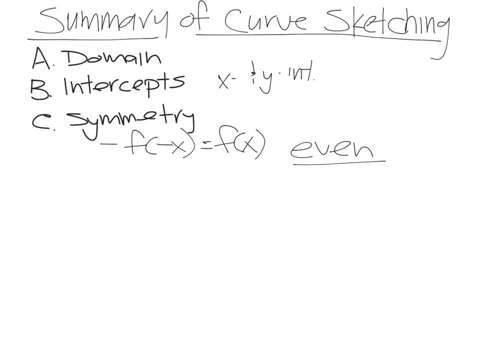 An even function is when it's symmetric. about the y-axis, For example, you might have something that looks like this and then it's symmetric like that. Okay, And so this is really: if f of negative x equals f of x, And then we check if f of negative x equals negative f of x. 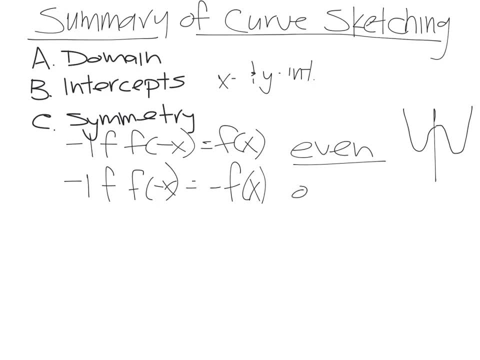 In this case, this would give us an odd function, An odd function. Okay. So f of an odd function looks like a reflected over the x-axis and then reflected again over the y-axis, like that. And the third type of symmetry we might get is a periodic function, that is, if we have 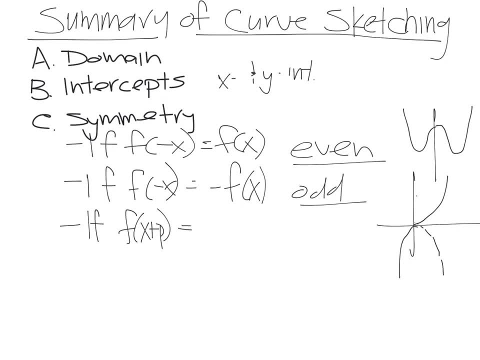 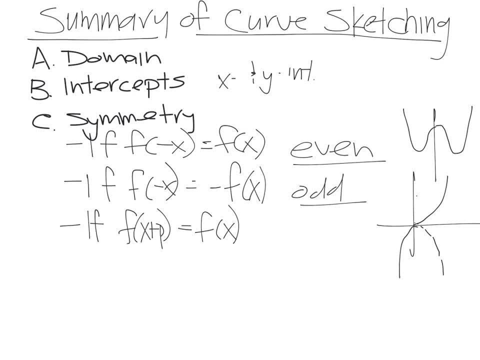 Okay, Okay, Okay. Okay. Here we have a period And we're going to look at f of x for some positive constant p. That's where we have our period. For example, trig functions. the graph of y cosine of x repeats forever. 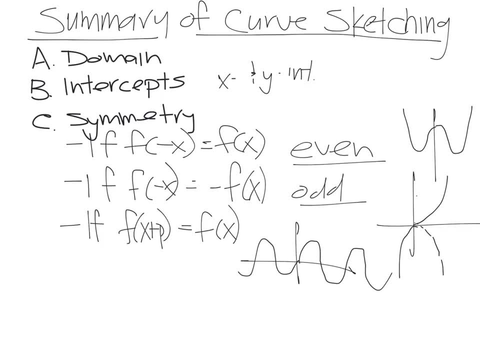 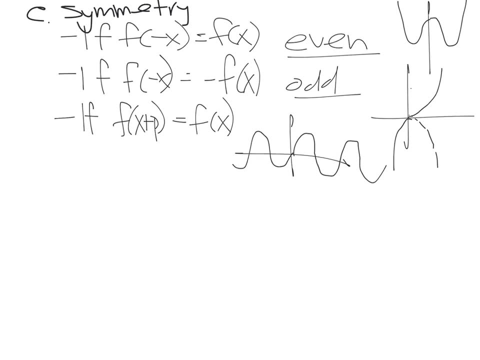 It's periodic, And now I'm going to move up a little bit. The next thing we're going to look at is asymptotes. So d equals f of x equals f of x, And d equals f of x equals f of x. 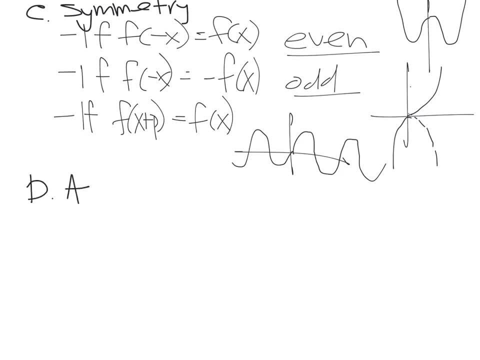 And d equals f of x, equals f of x, equals f of x would be asymptotes. We have different types of asymptotes. The first one we'll discuss is horizontal asymptotes. Horizontal asymptotes are found usually when we take the limit as x approaches. 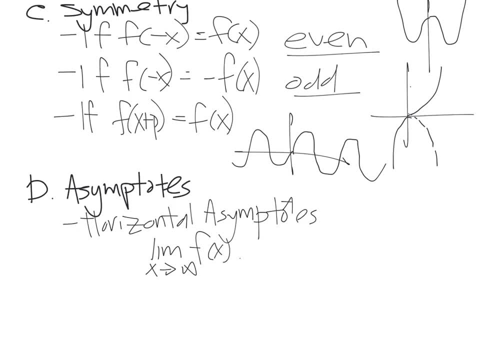 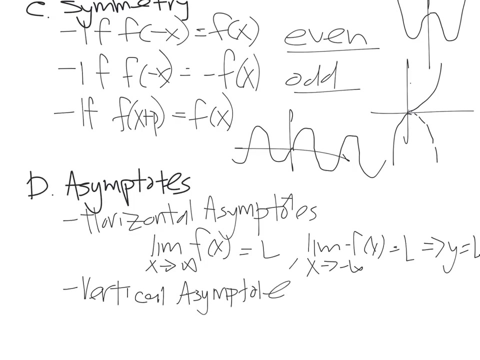 infinity of f of x. if that limit is some l, or if we take the limit as x approaches negative infinity of f of x and it equals some value of f of x, Then that implies the line y equals l is a horizontal asymptote. The next type of asymptote we have would be the vertical asymptote. 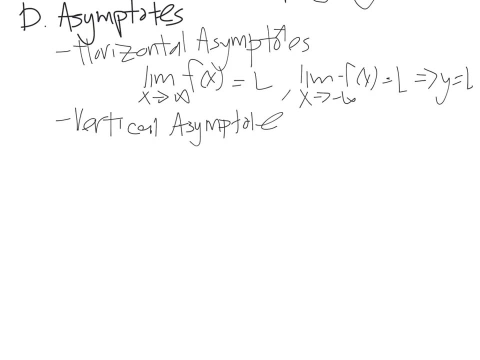 And the vertical asymptote is a horizontal asymptote And the vertical asymptote is a horizontal asymptote. And the vertical asymptote is: if we're taking the limit as x approaches some value, a from, say, the right of f of x, if that equals infinity, or if the limit as x approaches a from the 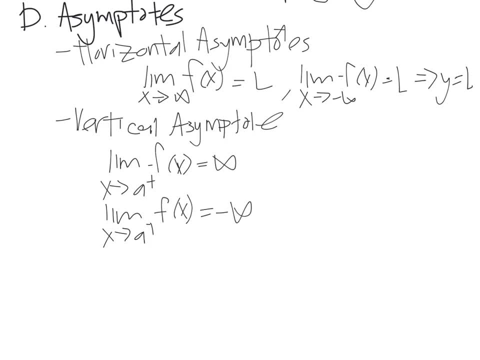 right of f of x is negative infinity, or the limit as x approaches a from the left of f of x is infinity, or the limit as x approaches a from the left of f of x is negative infinity. So any one of these, if the limit is going to be infinity as we approach a number from. 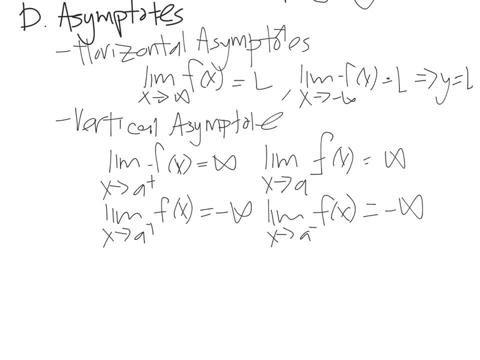 the left or right, then that means that the line- so this case we had the line- y equals l is horizontal asymptote. We get x equals a, It's the vertical asymptote. There's another type of asymptote that we have and this is called a slant asymptote. 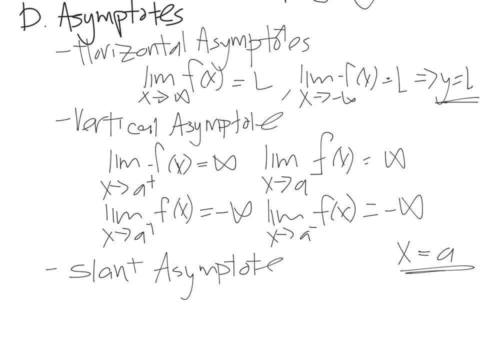 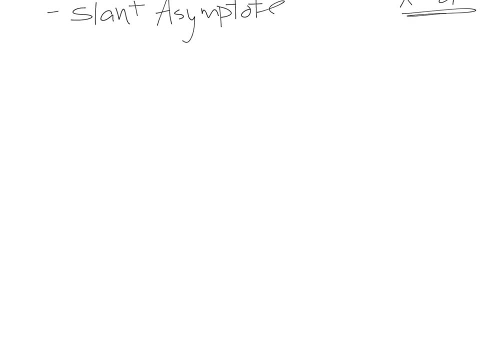 Another name for a slant asymptote is an oblique asymptote, but we'll discuss this another time. Now, the next thing that we look for would be: We're going to look at the intervals of increase or decrease, and this is where we take the. 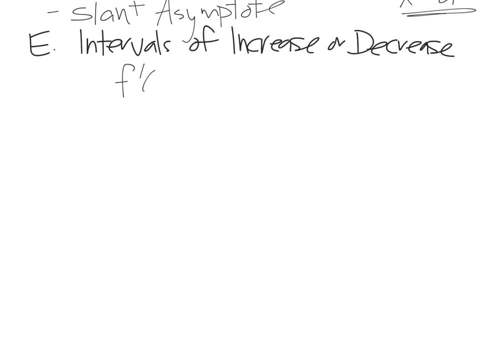 derivative we find f prime, and if f prime of x is positive it's increasing. and if the derivative f prime is negative, If f prime of x is negative, then we're decreasing. Then step f: you look for the local maximum and minimum values. To do this, first we find all the values of f that are critical numbers. 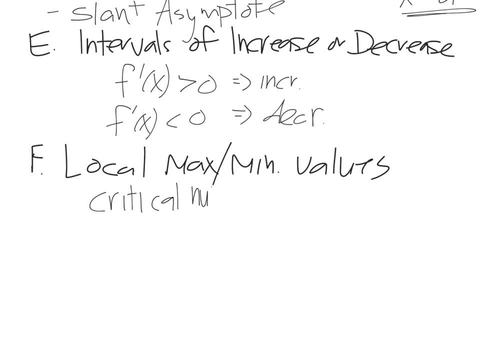 If you recall, critical numbers are when the derivative f prime of x equals zero or when the derivative f prime of x does not exist, And then to determine if it's a local max or a local minimum, you take the first derivative test And if your function is increasing before the critical number and then decreasing afterwards, 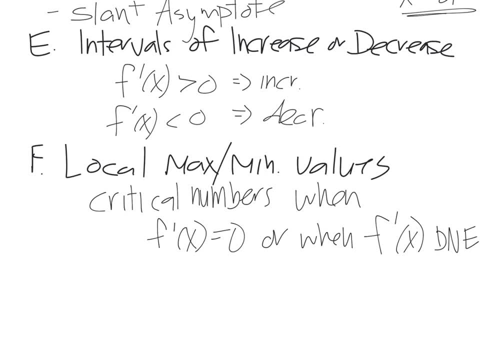 So if it's increasing before and then decreasing after, we have a local max. Or if it's decreasing and then increasing, we have a local min. And then step g, you check out the concavity And points Of inflection. So, concavity and the points of inflection, we're going to take a look at the second derivative. 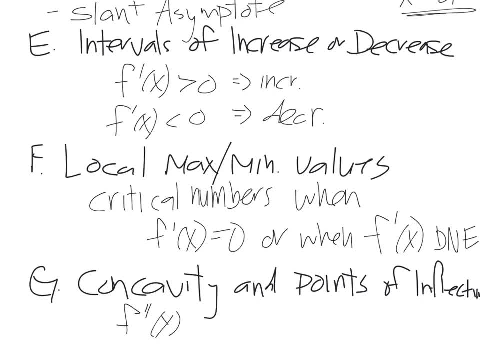 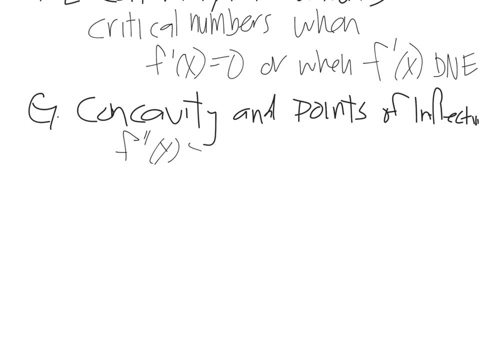 f, double prime of x. If your second derivative is greater than zero, Then it's. if it's greater than zero, Then it's going to be concave Up. If the second derivative Is less than zero, Is concave down. 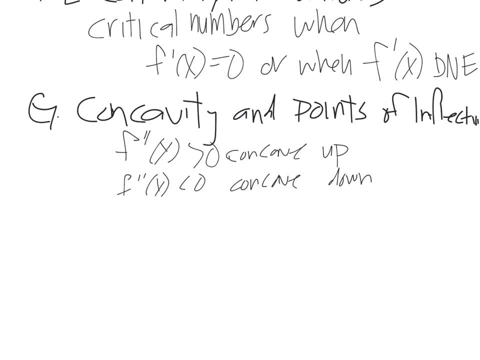 When it changes concavity. so, going from concave up to concave down, Or from concave down to concave up, That's our inflection point. And then the last thing, h, Now that we have all this information, We Are going to. 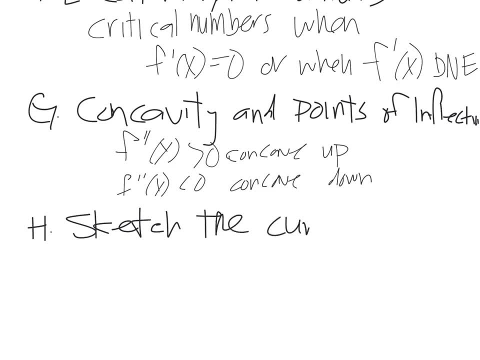 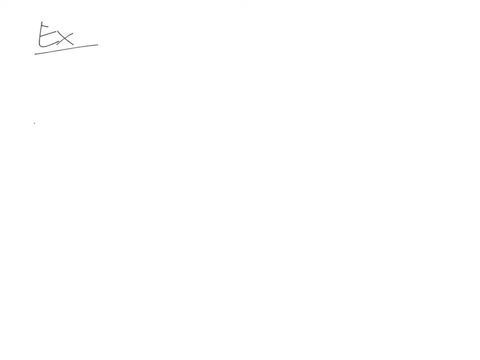 Sketch The curve. So now let's do an example Using all the steps that we have. Sketch the curve. Y Is equal to two x squared Divided by x squared Minus one. So, following our steps, Step a: 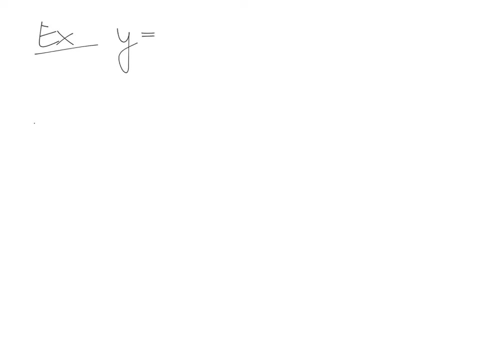 What's the domain? Well, the domain Is Already Concavated, So the domain Is Already Concavated. So the domain Is Already Concavated, So the domain Is Already Concavated. 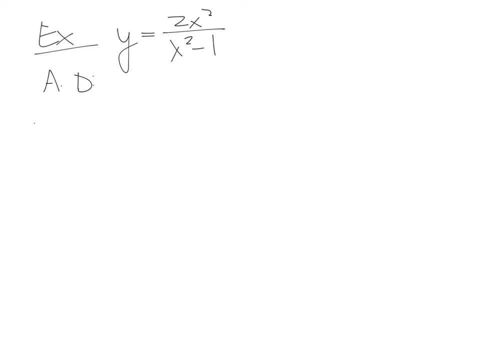 Concavated, So the domain Is Already Concavated. OK, Now let's write All the real numbers, And in fact I'll write it As all real numbers, Except for One Or negative one. 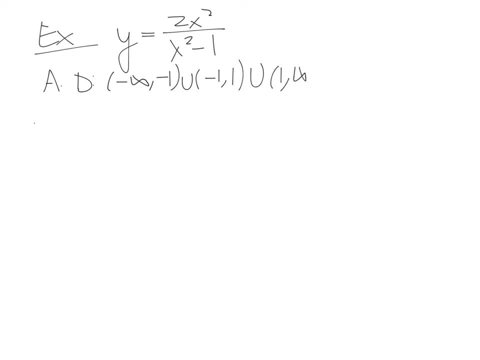 I'll write in interval notation: Negative infinity to negative, one Negative one to one, And then one To infinity. OK, Now Step B. Next, We find our intercepts, And so for the intercept To find the Y Intercept. 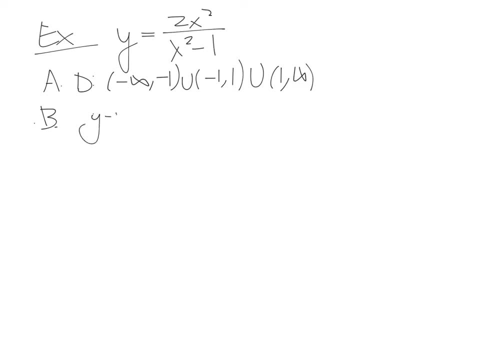 We set X, And then The power, we set X equal to 0, and if X is 0,, well, Y is also 0, so we get 0,, 0, and then to get the X intercept, well, for the X intercept, we'd set Y equal to 0, and in this case the X and Y intercept is the same. 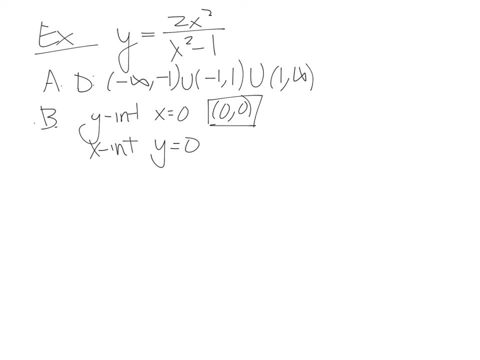 it's 0, 0.. Now we could check for symmetry in this case. if we put negative X into F of X, we get 2 times negative X quantity squared divided by negative X quantity squared minus 1.. Negative X quantity squared is just X squared, so this is 2X squared divided by X squared minus. 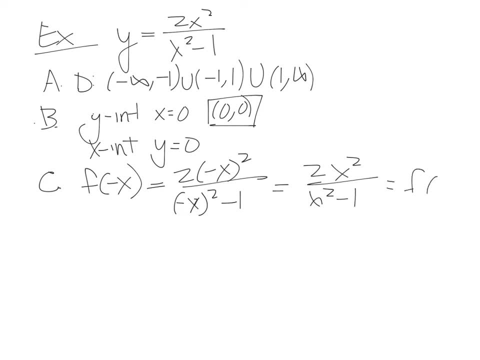 1.. 2X squared minus 1, which was our original function. this was F of X, so this is telling us that this function is even. Next, we'll check for the asymptotes. We'll check for vertical and horizontal asymptotes. 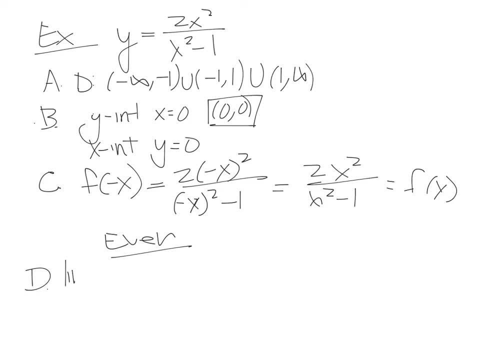 To check for the horizontal asymptote, we're going to take the limit as X goes to plus or minus infinity of our function 2F of X. and we're going to take the limit as X goes to plus or minus infinity of our function 2F of X. 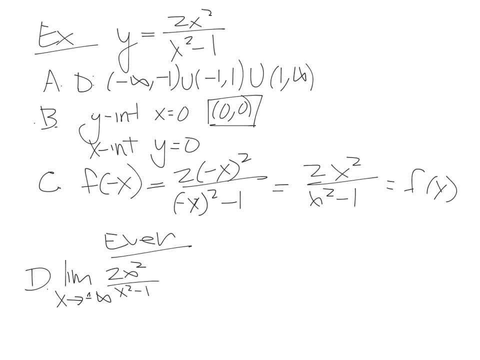 2F of X squared divided by X squared minus 1.. If we took this and we divided both the numerator and denominator by X squared, what we get is just 2 in the numerator and on the denominator dividing by X squared. well, X squared divided by X squared is 1, and then 1 divided by X squared is just going to be 1 over X squared. 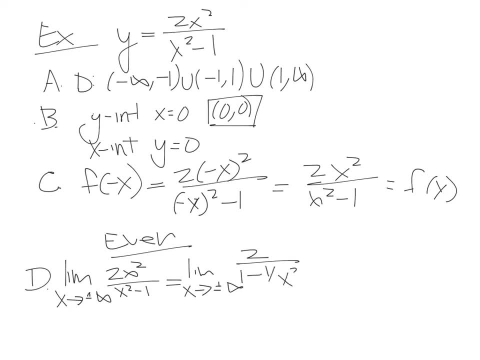 So this is 1 minus 1 over X squared. And now you can see: as X goes to infinity, this goes to 0, and so we're left with 2 over 1, or just 2.. So that tells us we have a horizontal asymptote at Y equals 2.. 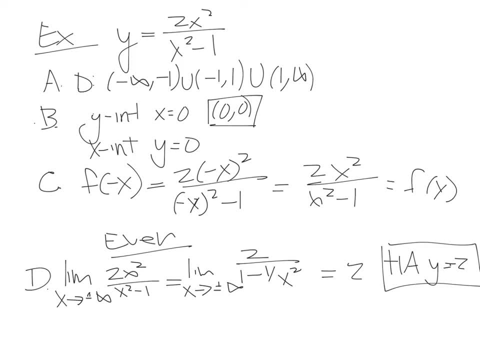 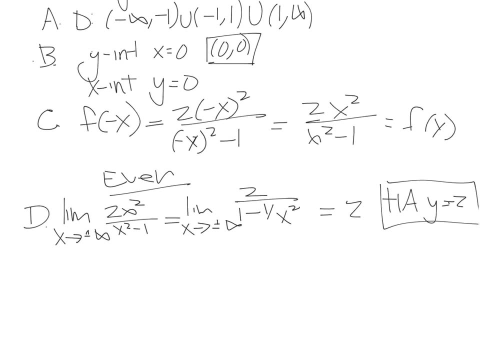 To find the vertical asymptotes, notice that the denominator is 0 when X is plus or minus 1, and this is also coming from our domain, where X couldn't be negative or positive 1.. And so if we looked at the limit, we get the limit as X approaches 1,. 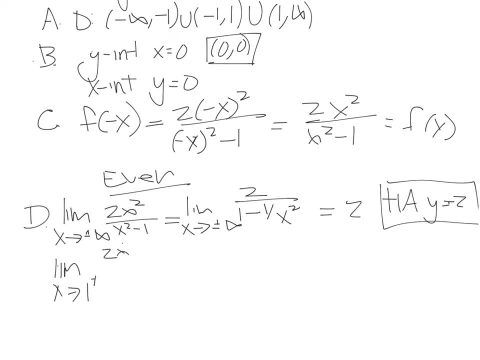 let's say, from the right side of our function, 2X squared divided by X squared minus 1.. Well, this is going to be infinity. And then if we also took the limit as X approaches 1, from the left side of 2X squared over X squared minus 1,. 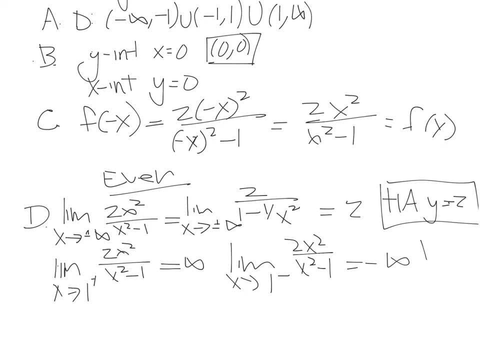 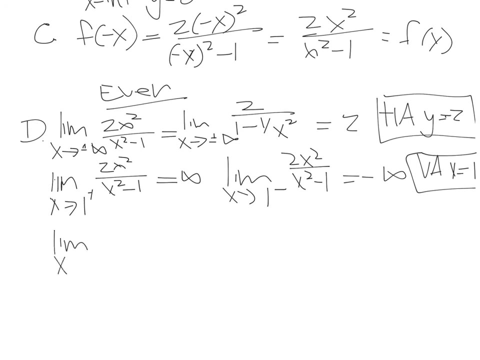 this is negative infinity. So this tells us we have a vertical asymptote at X equals 1.. And similarly, if we went for negative 1, we get the limit as X goes to negative 1 from the right of 2X squared over X squared minus 1.. 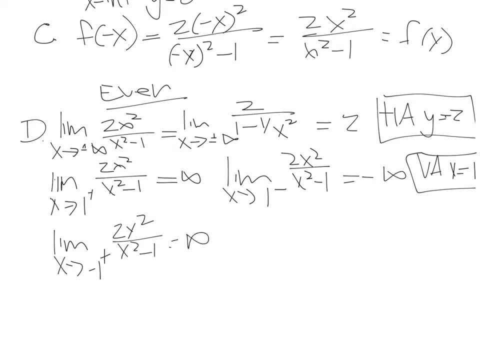 That's also going to be infinity. Excuse me, it should be a negative infinity rather. And then this limit as X goes to negative 1 from the left of 2X squared over X squared minus 1, that's positive infinity. 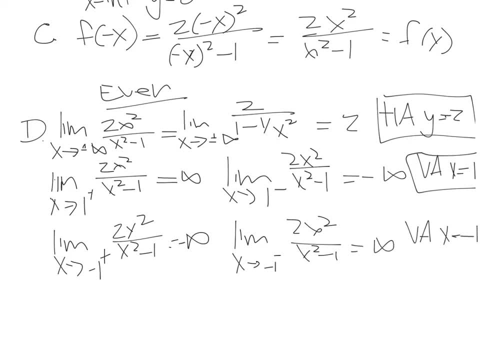 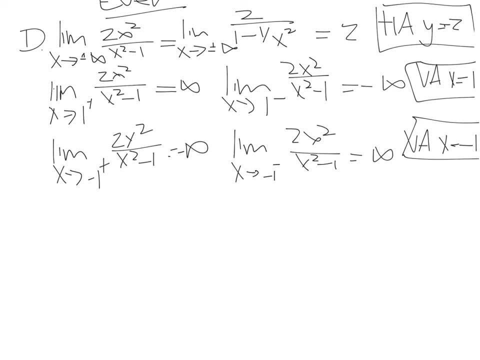 So we have a second vertical asymptote at negative 1.. Alright, we're almost there, Bear with me E. well, let's first take the derivative F prime of X, And here we're going to have to use the quotient rule. 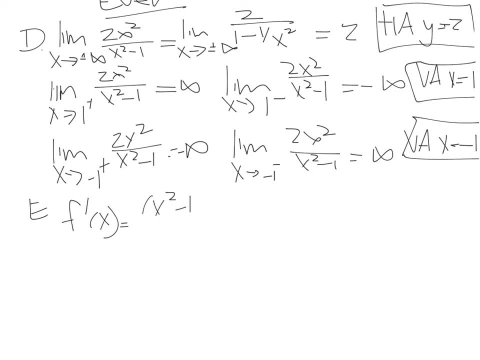 Okay, so the denominator X squared minus 1 times the derivative of the numerator 4X minus the numerator 2X squared times the derivative of the denominator times 2X divided by the denominator squared. This actually simplifies to negative 4X over X squared minus 1 quantity squared. 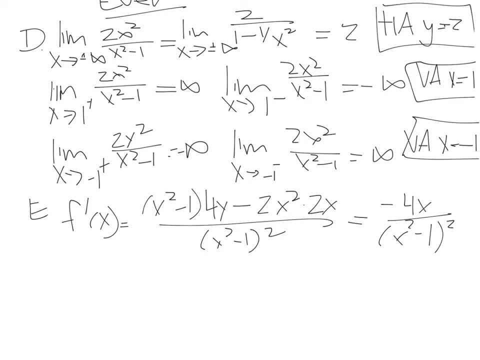 Now, since the denominator is always going to be positive because it's a derivative, we can just look at the numerator. When is this derivative positive And when is this derivative negative? Well, F prime of X is going to be positive when X is less than 0.. 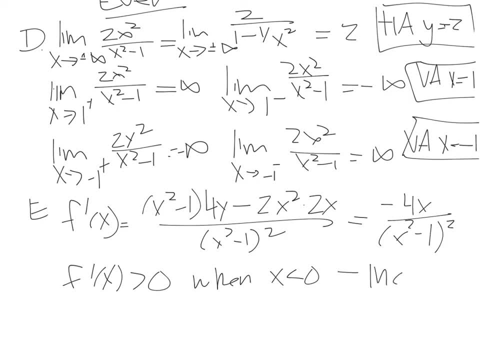 That means when X is less than 0, it'll be increasing, And F prime of X is negative when X is greater than 0, and when X is less than 0, it'll be increasing, And so that's where we're going to be decreasing. 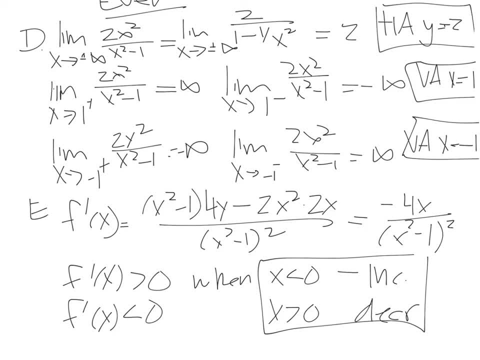 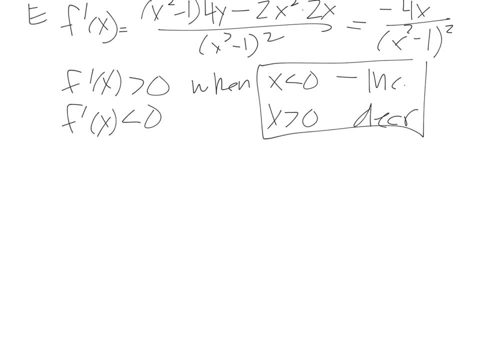 Of course, keep in mind that X can't be 1 or negative 1, because it's not in the domain. Now we're going to find F, which is our local max and minimum values, So we have our derivative over here. 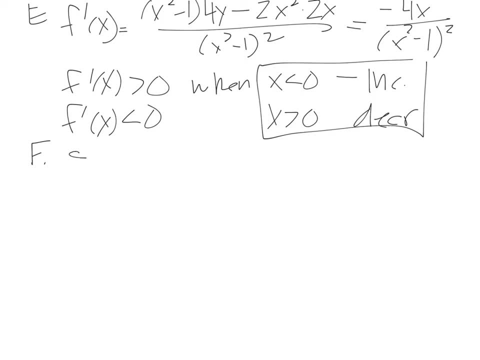 That will tell us our critical points. The critical points are: when the denominator is less than 0, and the derivative is 0. So that first one: the numerator is 0 when X is 0, so that's the first critical point. 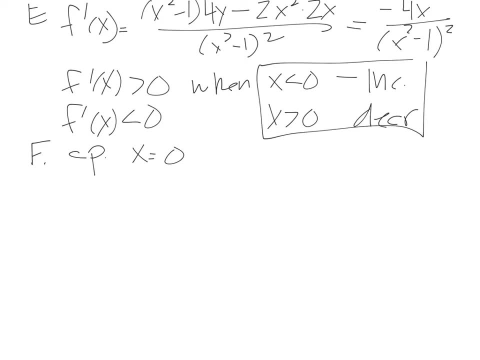 And the critical point also occurs when the derivative is not defined, So when our denominator is 0.. Our denominator is 0 of the derivative when X is 1, or when X is negative 1.. So that's the first one. Plugging in all these, we get F of 0,, F of 1, and F of negative 1.. 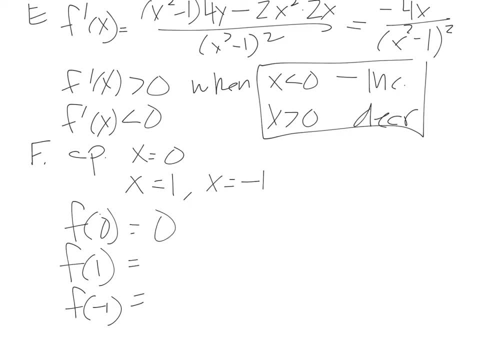 F of 0 is 0.. F of 1 and F of negative 1 is undefined, so they're not a local max or a local min, because it's not even in the domain. So we have just F of 0 equals 0.. 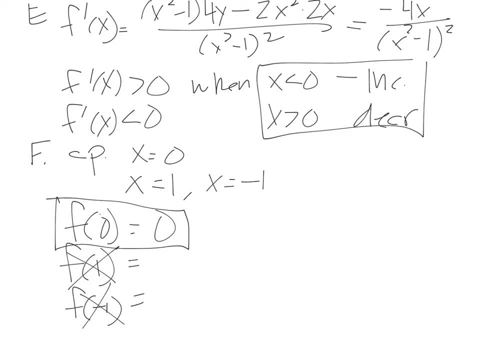 So now this could be a local max or a local min, and so we need to determine which one it is. Now we can use the first derivative test, So we'll pick a point. just to the left of it, We'll pick a point. let's say: 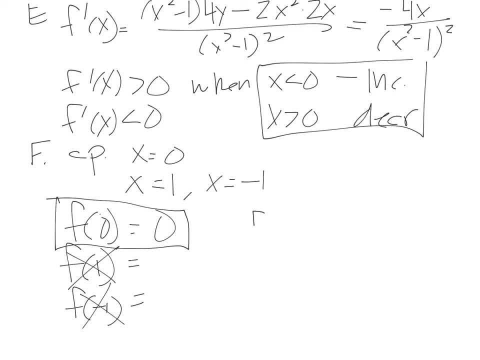 let's say 0.5, or negative 0.5.. So if we're on the number line, we're at negative 0.5,, 0, and then 0.5.. If putting these points into our derivative, 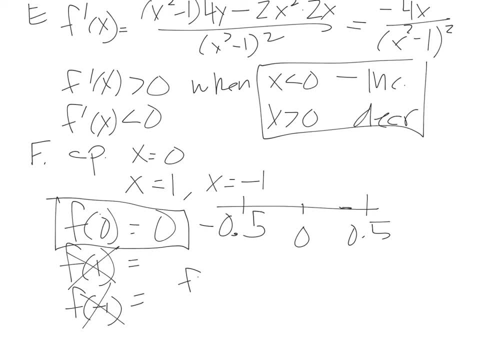 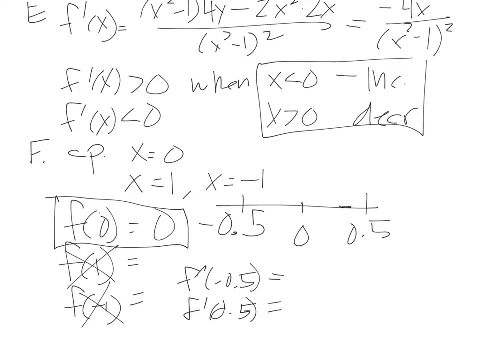 F prime of X, or rather F prime of negative 0.5,. so the derivative at negative 0.5, and the derivative at 0.5, and we're going to determine if the derivative goes from increasing to decreasing. 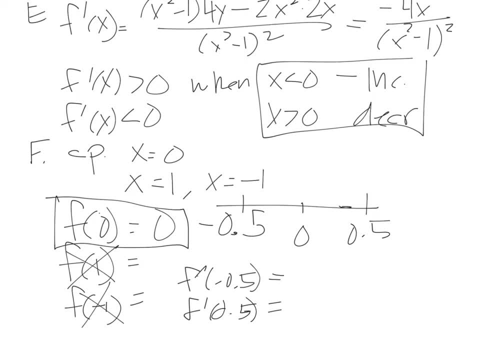 or decreasing to increasing. This gives us something like approximately 3.556, and negative 3.556.. And so if we're going before, our derivative is going to be positive and then after 0, our derivative is negative. So since we're changing, this tells us: 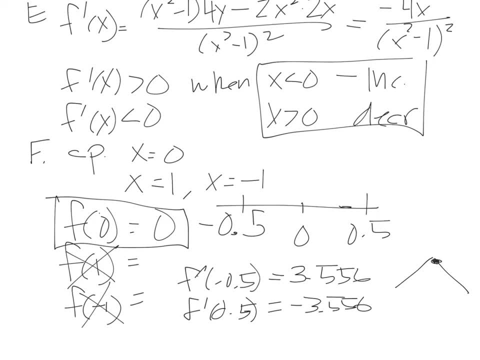 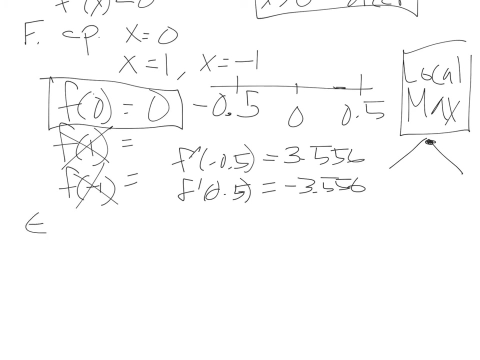 that we have a local maximum. So this is a local max. And the very last thing, last step that we got to do is take the derivative of the derivative, or the second derivative and, if you recall, so our first derivative. 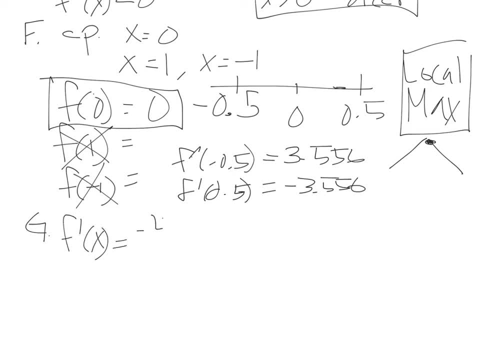 F, prime of X was equal to negative 4X over X squared minus one quantity squared Determining concavity. we need to have the second derivative, And so here we go. We're going to take the denominator, which is going to be: 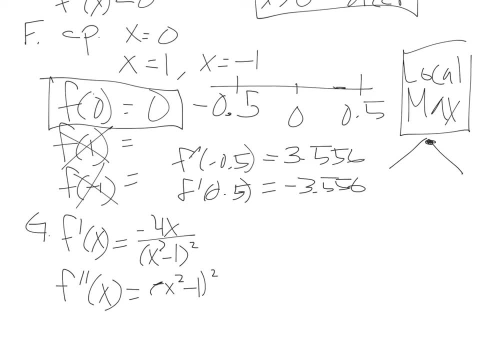 X squared minus one squared times the derivative of the numerator, times negative four minus the numerator. so minus a negative four is a plus 4X times the derivative of the denominator. And this is where it's going to get pretty ugly. 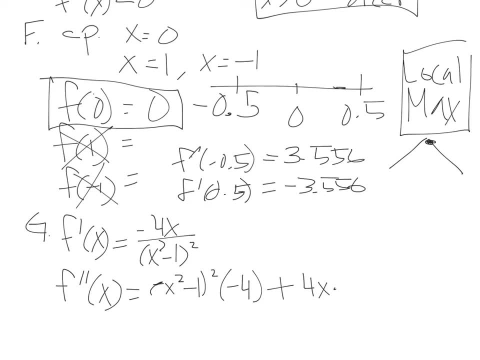 So we're going to have to use the chain rule. derivative of the denominator is going to be two times the quantity X squared minus one squared times the derivative of the inside 2X all over the denominator, which is X squared minus one quantity squared. 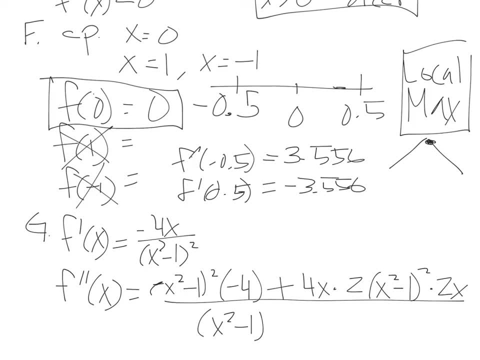 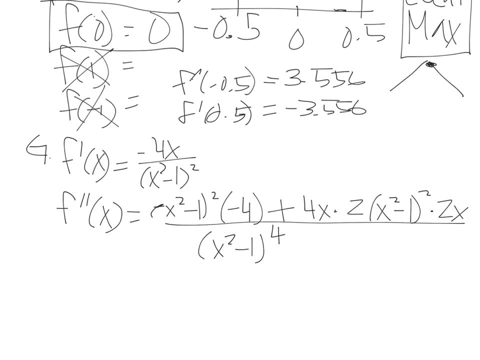 so if you have a squared squared, it'd be raised to the fourth power. Now, all this simplifies, and thankfully it simplifies, and what we end up with is the following: We end up with 12X squared plus four. 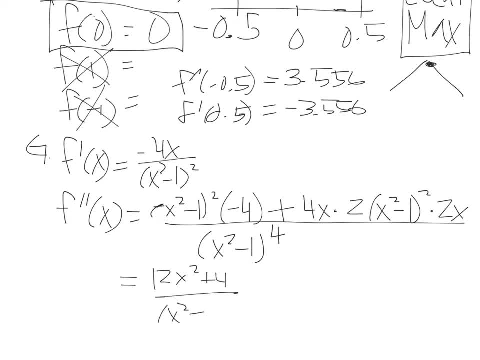 divided by X, squared minus one cubed. Oops, and I just realized this should be to the power one. Now, if we're determining concavity, if it's concave up or concave down, notice the numerator. 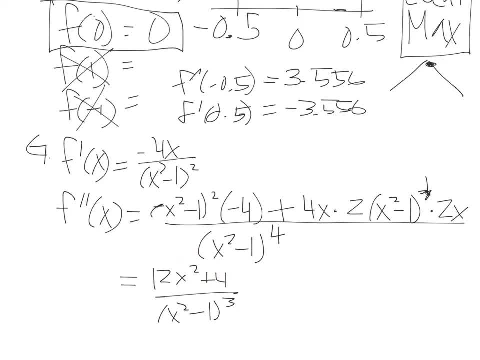 this is always going to be positive because X squared is positive. 12 times the positive number is positive, and if you add four, so this is always going to be positive. So we're only really concerned about this denominator, this X squared minus one. 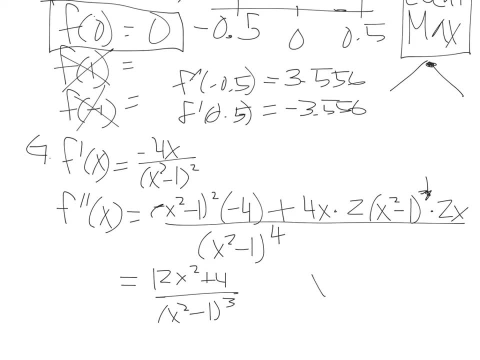 So we want to see X squared minus one. when is X squared minus one going to be positive? Well, X squared minus one is positive only if X is going to be greater than one or less than negative one. So if X is greater than one. 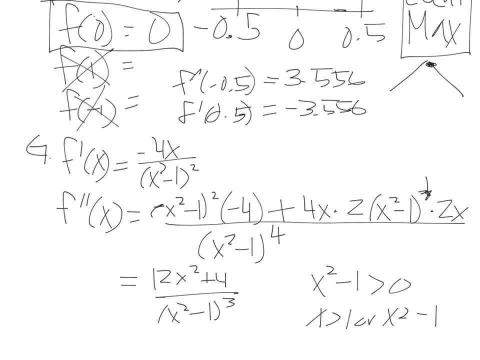 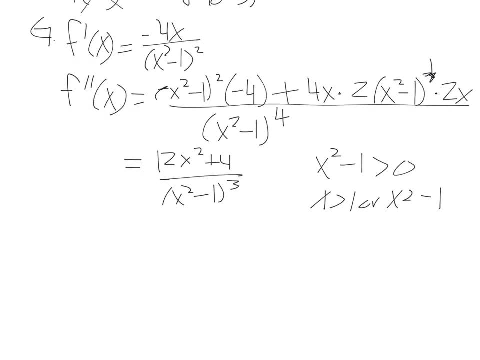 or X is less than negative one, it'll be concave up. well, it'll be positive. this is positive, which means this is positive, which means the second derivative is positive. so it's concave up for there, and this is a less than. 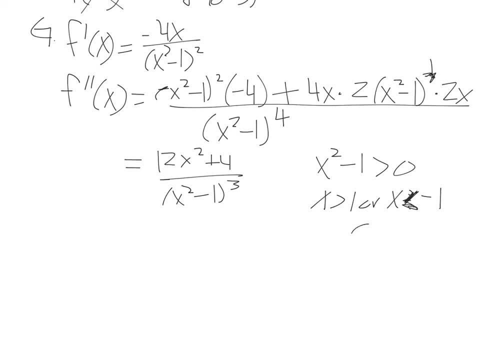 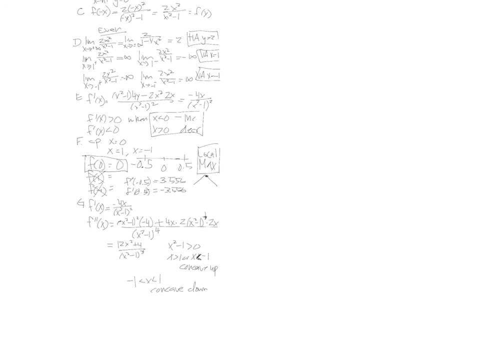 not a two. so that's where it's concave up, and when X is between negative one and one, it's concave down. All right, now we're going to have to try and put all of this together into a graph. 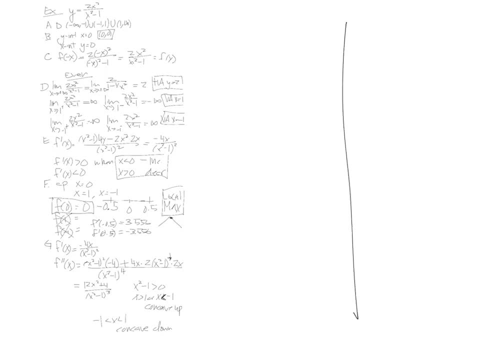 So I have everything right here. so let's see what we got Going through the steps, so we have right here: X cannot be one or negative one. we have an intercept right here at zero, zero, zero. the origin. 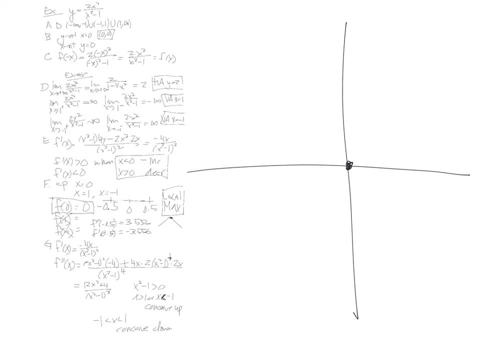 looking at C, it's going to be an even function, so we only need to draw half of it and the other half would be reflected. Now we have part D. these are telling us right here. these are telling us all the limits. 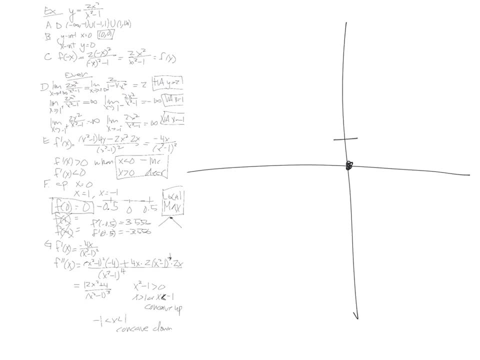 and that gives us a horizontal asymptote of two. these limits give us a vertical asymptote at negative one and positive one. but taking a look at these limits a little bit more careful, what we get is the following: we get: 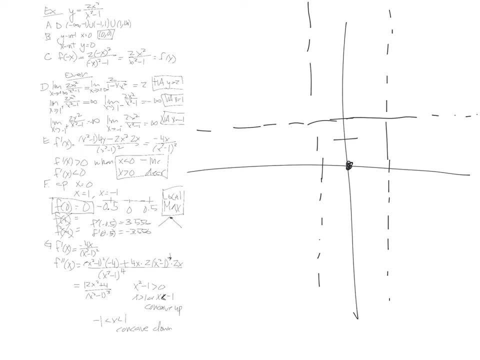 as we go to negative infinity, the limit is two. so as we go out to negative infinity, we're going to be at two, and as we go out to positive infinity, we're also going to be at two. and then we look at the vertical asymptote. 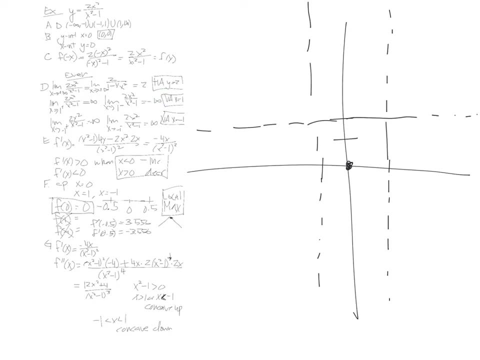 these vertical asymptotes say as we approach. so I'm just going to look at the negative one right now. so if we approach negative one from the left side, it's going to be infinity. so as we approach negative one. 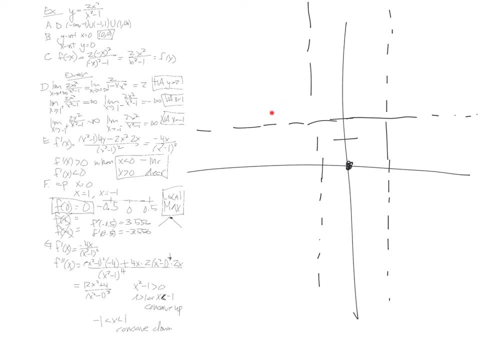 from the left side it'll be infinity and we're going towards two, so we can sort of fill in our gap like that, knowing that this is an even function. we would get the mirror image something to be like that, and then: 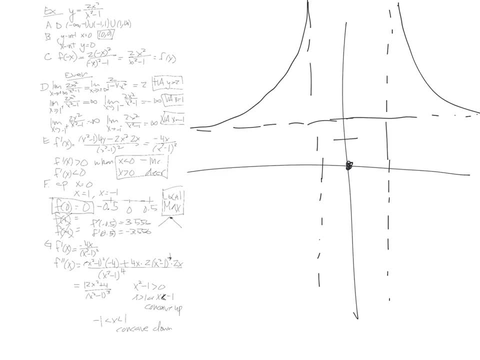 the limit as x approaches, negative one from the right side is negative infinity. so we'd be down here, negative infinity going upwards. and we'd be going upwards because right here step E says we're increasing as long as we're. 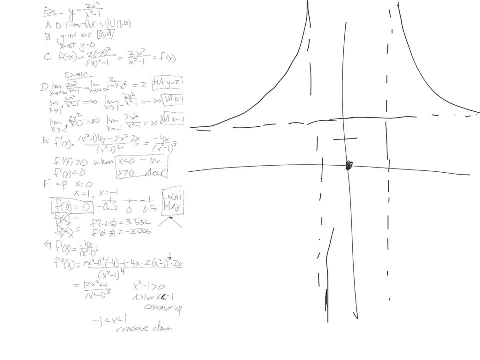 as long as x is negative. so we're increasing and we're going to keep increasing until we hit this local maximum zero, zero. so we're going to keep increasing until we hit the local maximum. local maximum means, then it goes around. 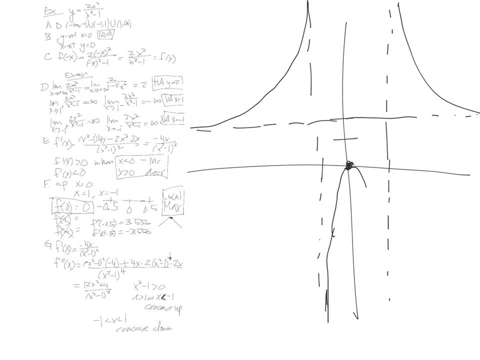 it turns back, heading downward, and we can see, taking a look at, at a, just a reflection, we get something like that and we can verify the way that we drew it, because as we draw these curves, instead of 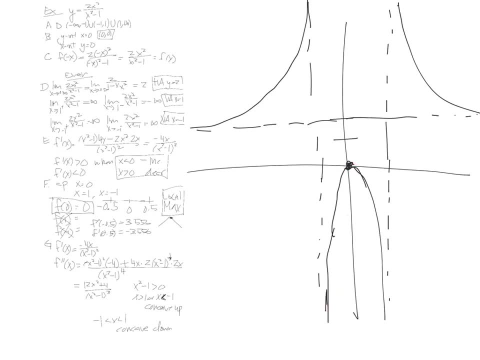 the curve looking like something funky. we know it's sort of smooth like this, meaning it's concave down when we're between negative one and one, and over here that's a concave up and that's also a concave up. 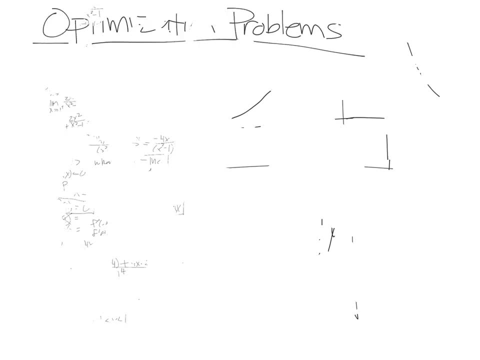 and that's how we draw our curves. today we're going to talk about optimization problems. there are a couple of steps to solving optimization problems. the first thing is to read the problem. read the problem and understand it. 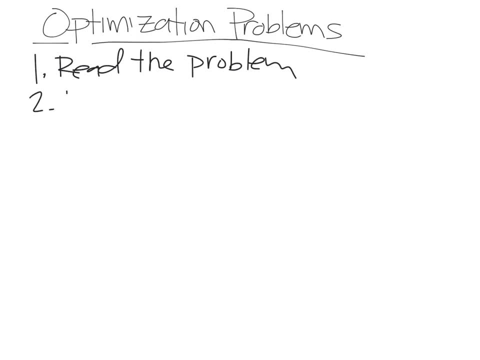 second thing you want to do is draw a diagram. so we're reading the problem. we're asking ourselves: what's the unknown, what are we given, what do we want to find those types of things? draw the diagram. these often help us. 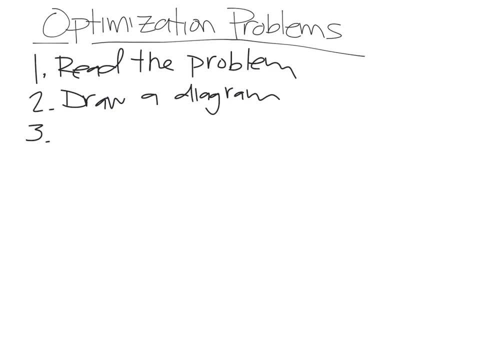 with these types of problems. and then the third thing: introduce notation or variables. for now, let's say what we're trying to optimize, trying to maximize or minimize. let's call that Q, then step four, what we want to do. 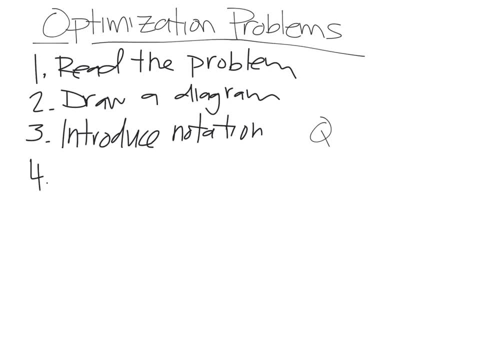 is we're going to express Q in terms of some other symbol or whatever unknown quantity or other quantity that we have, and we'll keep doing this until we only have just one variable. so let's say Q is just a function of X. 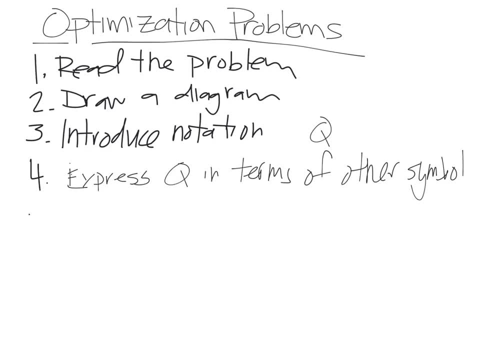 or something to that effect. and after we do that, the last step, step five, is to basically find the absolute maximum or minimum. I didn't finish my five right there, so step five would be find. 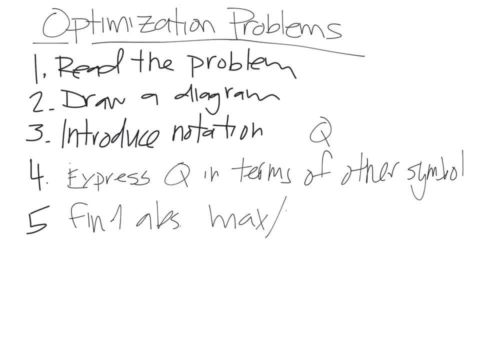 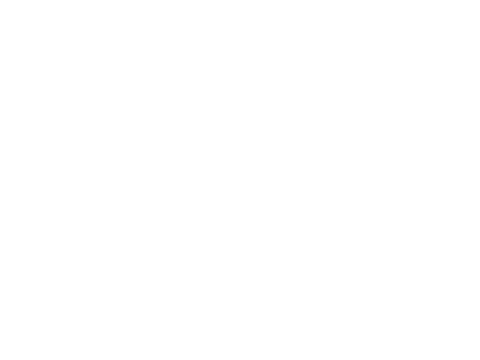 the absolute max or minimum, and we'll use one more test that will help us, and this is the first derivative test for absolute extreme values, meaning maximum and minimum, and what this says is that suppose 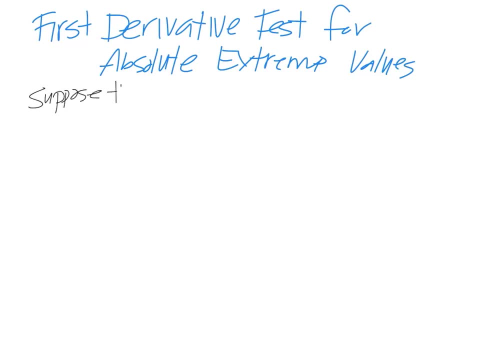 that that C is a critical number of a continuous function, F defined on an interval. A says that if the derivative F prime of X is greater than zero for all X, that's less than C. 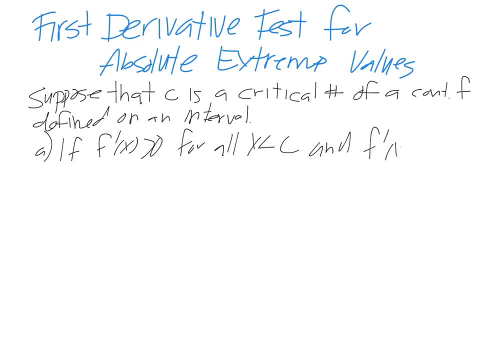 and the derivative F prime of X is less than zero for all, X greater than C, then we conclude that F of C is the absolute maximum value and B? well, let's just back up. 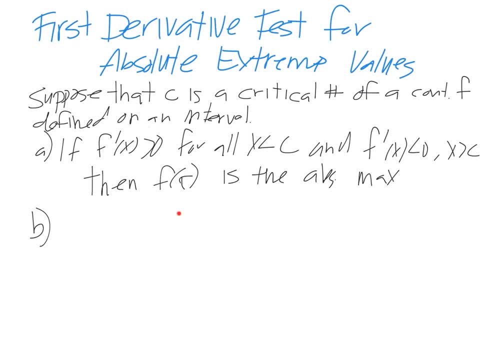 for a minute. so if the derivative is greater than zero, so we're increasing for all some values, and then the derivative is less than zero, we're decreasing, we have an absolute max, and then if the derivative 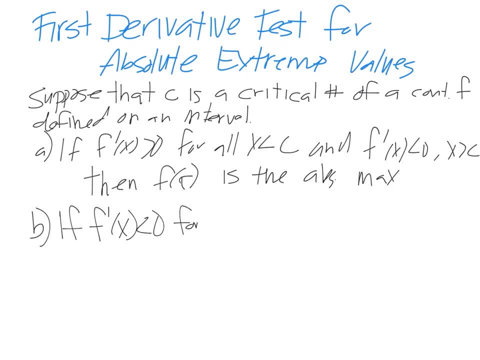 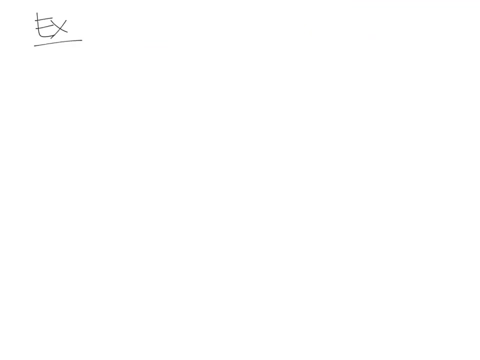 F prime of X is less than zero for all X less than C and F prime of X is greater than zero for all X greater than C, then F of C is the absolute minimum. let's do an example. 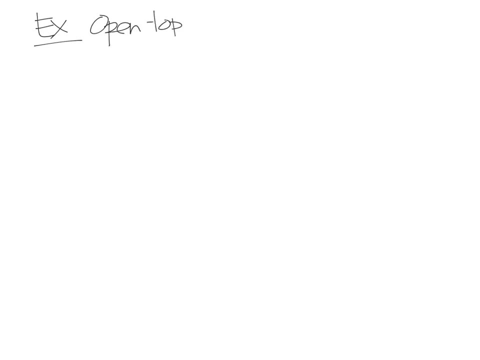 so we have an open top box and it's made by cutting small squares out of the corners of a 12 by 12 inch tin. okay, so if we have a square like this and it's 12 inches, 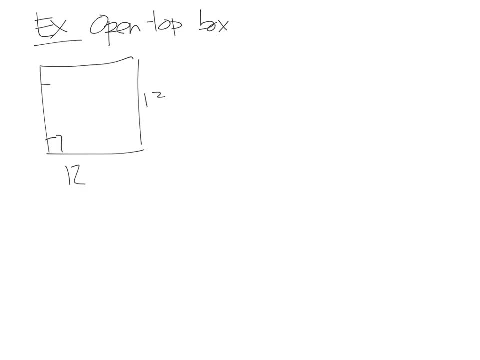 by 12 inches. but we cut off the corners like this and then we fold these tabs upwards. so we were to fold this tab up, this tab up, this tab up and this tab up. what we would get. 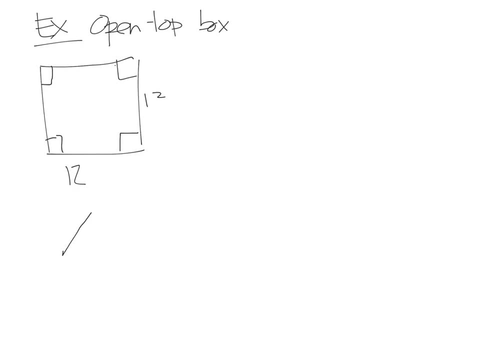 would be a box where the tabs will go up like that. those tabs will go up and so forth, the tabs that were once out here. they get brought up like this, and so we have our box. so what we have is: 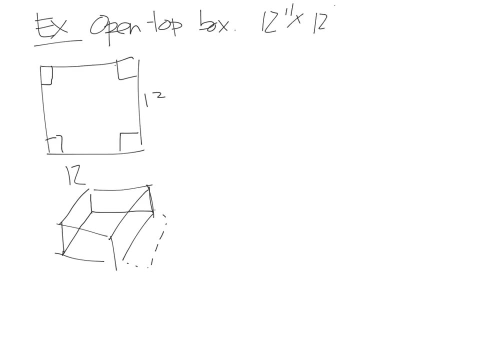 we have 12 inches by 12 inches and we cut. we cut small squares out of the corners. what I want to know is: how small should these squares be so the box holds as much as possible? 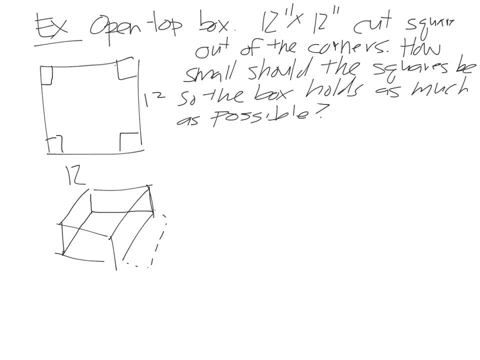 in other words, what we're trying to do is we're trying to maximize the volume of the box. now we're trying to figure out what these squares we're cutting out of, and so let's call these squares. 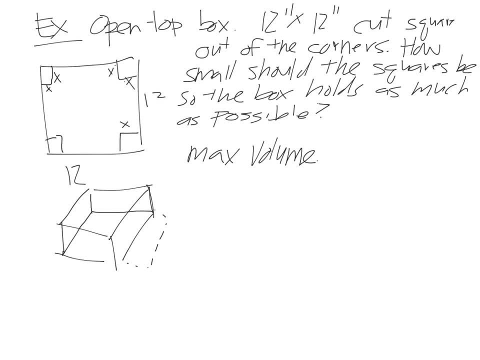 the length of these squares x, and so let's try and figure out the formula for the volume of this. so what is the volume? well, if this whole length is 12,, what is this length? that's really just. 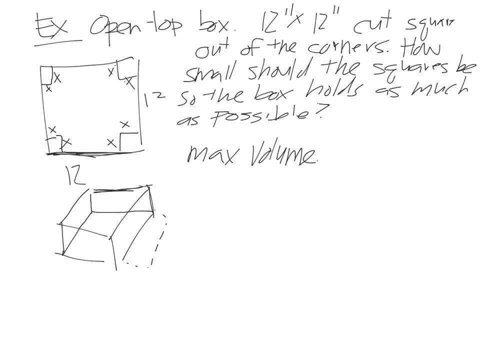 this smaller piece and we took aside x off and x off, so this new length is 12 minus 2x, and so this whole square is going to be 12 minus 2x by 12 minus 2x. 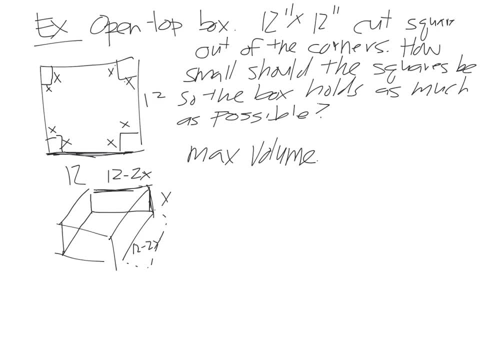 and how high is this? this height is going to be x, so the equation for volume as a function of our x is going to be our height x times 12 minus 2x. by 12 minus 2x. 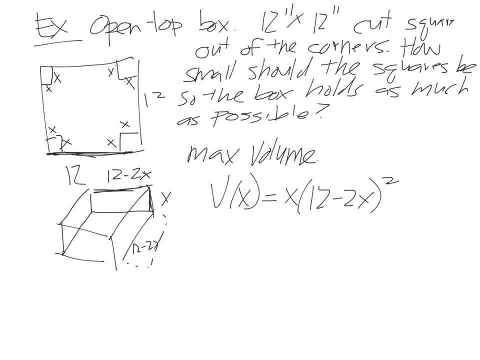 or 12 minus 2x quantity squared, and we can go ahead and write this all out. we'll expand this so we get 144, minus 48x plus 4x squared, or 144x minus 48x squared. 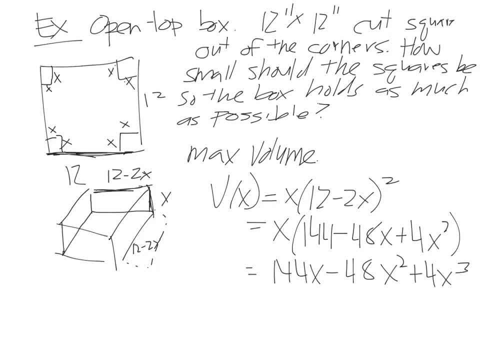 plus 4x cubed. so we're trying to maximize this, maximize the volume. so let's go ahead and take the derivative. and one thing to note before we take the derivative: remember this whole thing has a length of 12,. 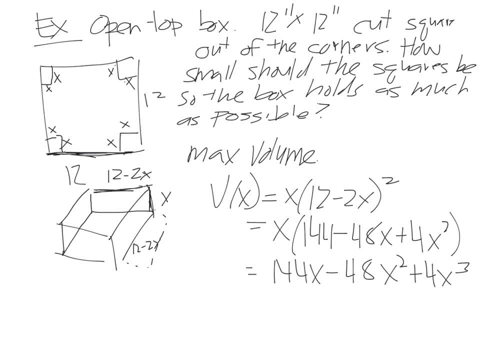 so if we have x and x, keep in mind that we can't have a negative length. so x can be at most 6, otherwise 12 minus 2x would be negative and you can't have a negative side. 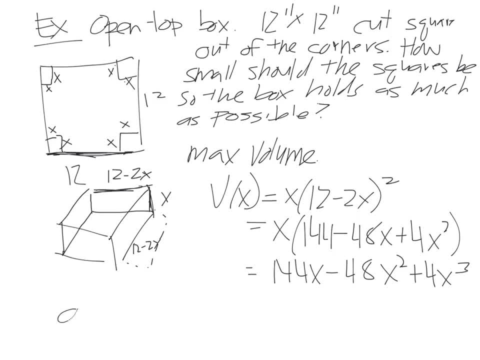 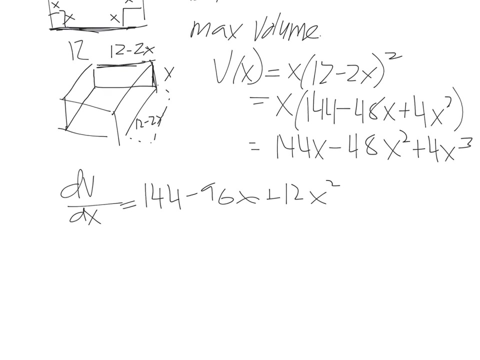 so, taking the derivative dv dx, we get 144, minus 96x plus 12x squared. if we want to maximize this, we're going to set this equal to zero and find the critical points. so we'll set this equal to zero. 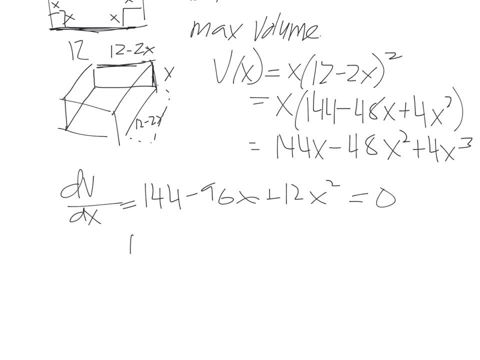 and what do we get? well, we can factor out 12, so we get 12 times the quantity. 12 minus 8x plus x, squared equals zero. we can factor this one more time, so this is 12 times the quantity. 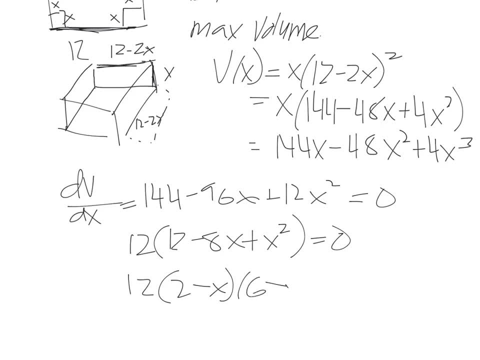 2 minus x times 6 minus x equals zero, and so, therefore, our critical points are: x equals 2, and x equals 6, but remember, if x equals 6, then we wouldn't have any length, so we can go ahead and disregard. 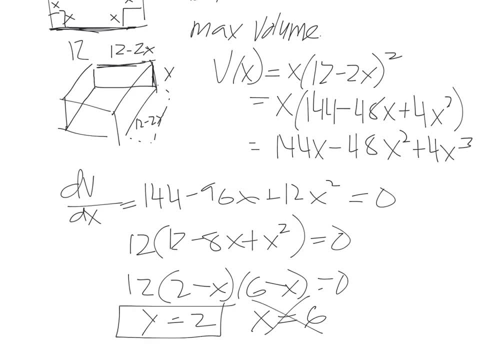 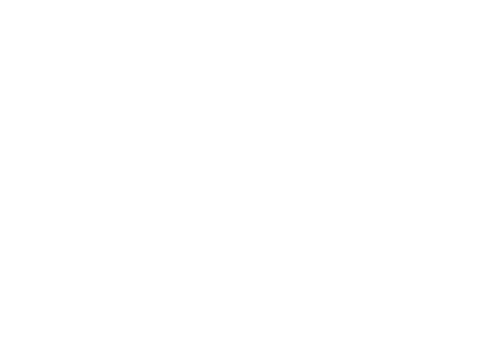 this one point- so x equals 2, is how much we'll have to cut off from each side 2 inches. now these optimization problems involve application in business and economics. so in these types of problems you might say: 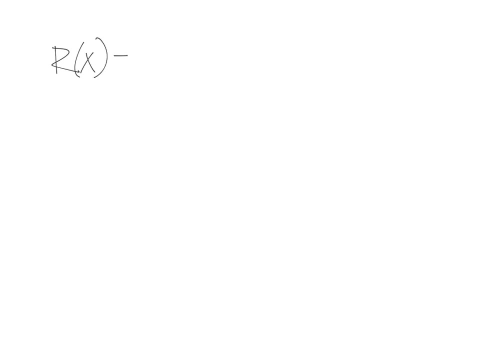 define some r of x to be the revenue. you might say c of x would be the cost, and then p of x would be your profit, and so we'd say p of x would be the revenue which you make. 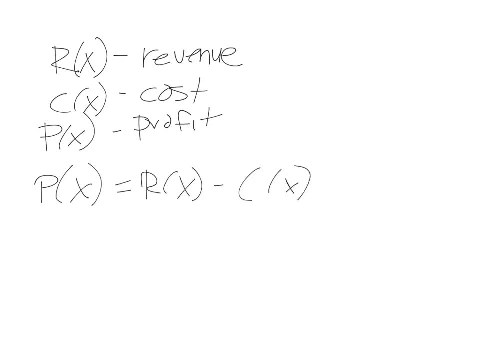 minus the cost, and if you want to maximize your profit, then you find this function and take its derivative now in economics, the derivative of r. economists tend to use the term marginal revenue, marginal cost for the derivative of the cost. 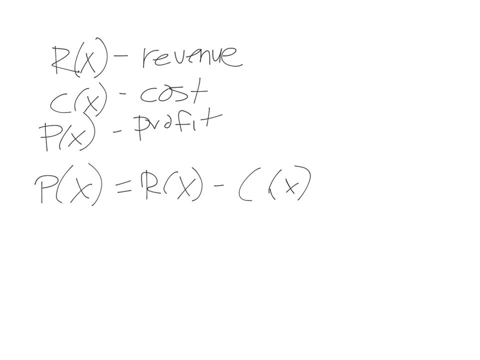 and marginal profit, for the derivative of the cost, for the derivative of the profit. today we're going to talk about Newton's method. the goal of Newton's method for estimating a solution for an equation is to write a sequence. 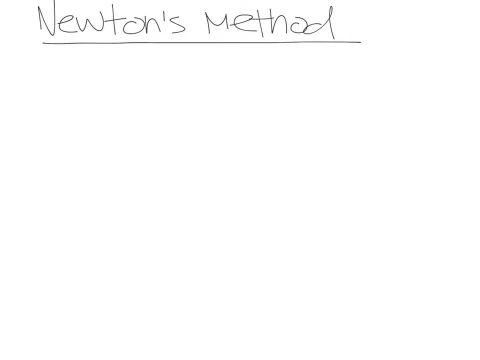 of approximations that approach the actual solution. this is what goes on inside a computer or a calculator when it tries to find the solution to an equation. in Newton's method we wish to solve some sort of equation. 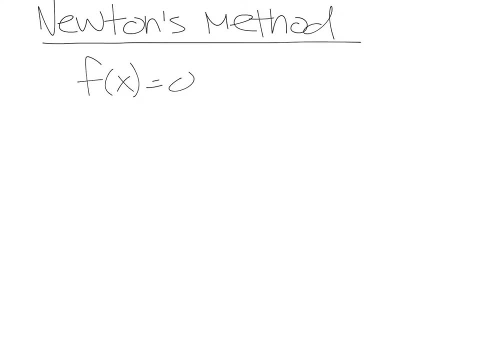 f of x equals zero, and so if we're to graph something like this, let's just say our function is x and y, this is our function f of x, right here, and we want to find when it's zero. 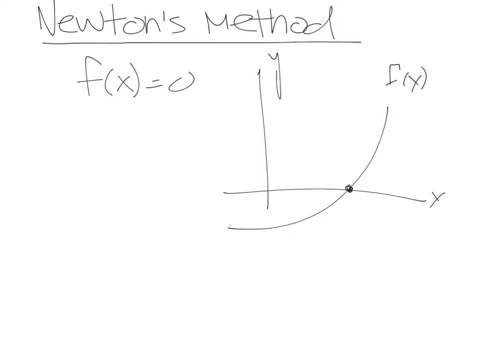 so basically the x intercept, what we do with Newton's method, we begin by just picking some point on this curve, and so let's say, this point is the point x, one comma and then our y value. 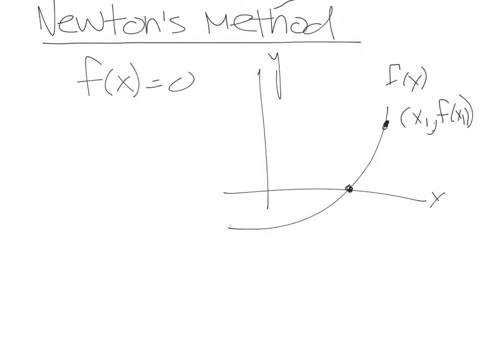 would be f of x one. so this is the point x one right here. that's straight down and we're trying to find this point right here. let's just call that point r now, if we consider the tangent line. 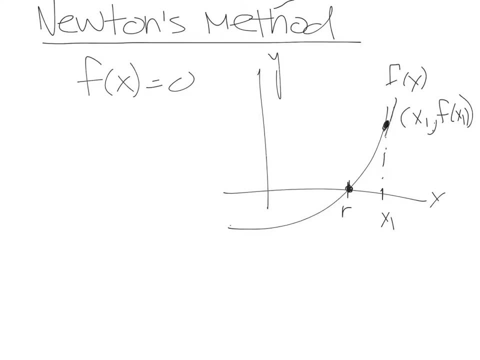 to this curve, at x one. that tangent line looks something like this: the tangent line will cross down and we'll say that point will be x two. so the tangent line of at this curve we'll call this: 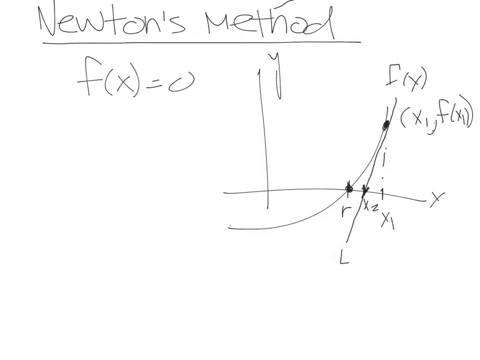 l one and it crosses the axis at x two or just l. to find the formula for the, for the tangent line l, we use the equation y minus our y, one value. and so this is our, this is our points that we're using. 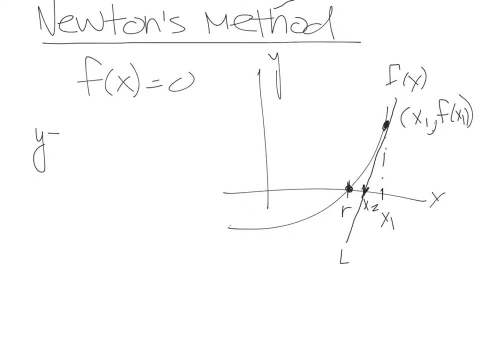 so the y one value is really f of x one is equal to the slope. so we're using the formula y minus y one equals m times x minus x one, where our slope is really our derivative. so that's. 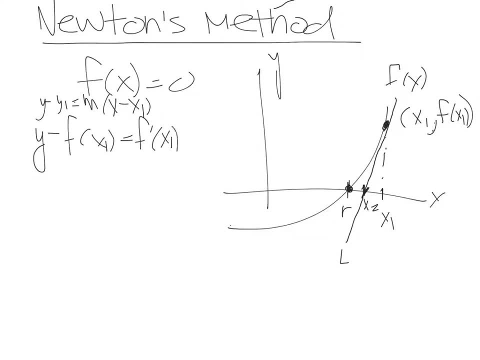 f prime at the point x, one times x minus x one. so this is the equation of that line. but we know that line when it crosses right here at that point, that's at the point x, two comma zero. 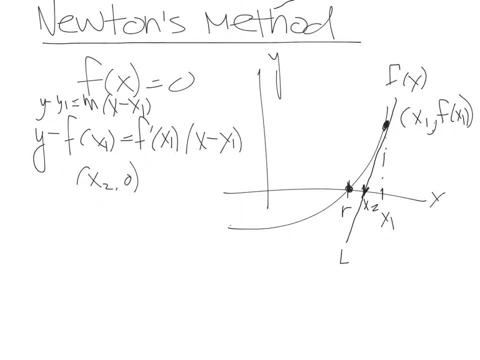 that's at the point x two comma zero. so we can plug x two comma zero into this equation. so what we get is zero minus f of x one. so we're plugging in x two in for x. 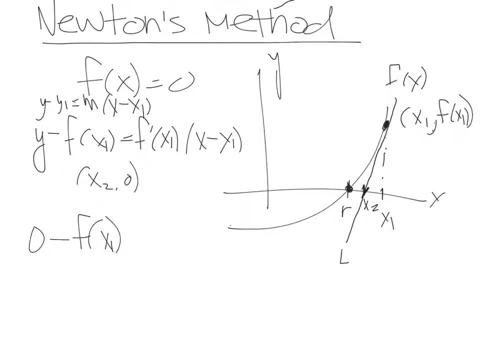 and zero in for y. so this is zero minus f of x one equals f prime of x one times x two minus x one and doing some rearranging of terms we can solve for x two. 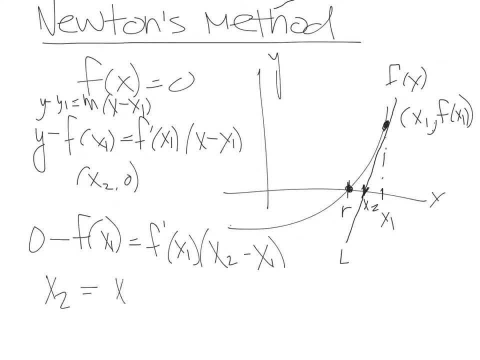 and we get that x two is going to be x one minus f of x one, divided by f prime of x one. so now, given just some initial point that we picked on this graph f of x. 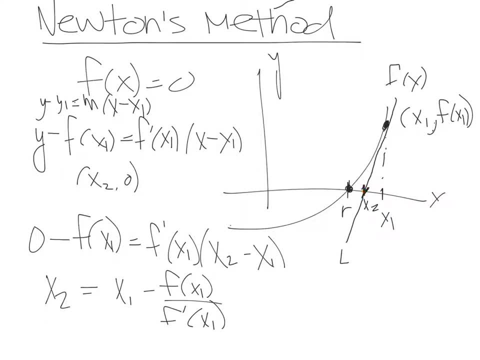 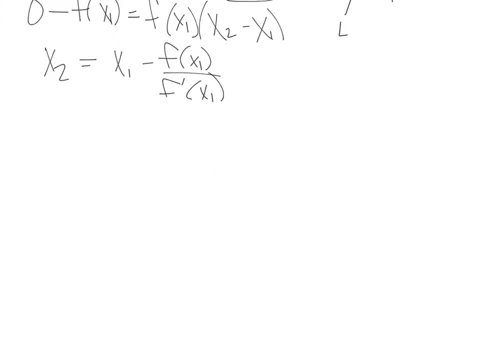 we can now get this point x two and notice this point x two is going to be closer than our original x one is to where it crosses the axis. now let's go ahead and draw another diagram. I'm going to make this one. 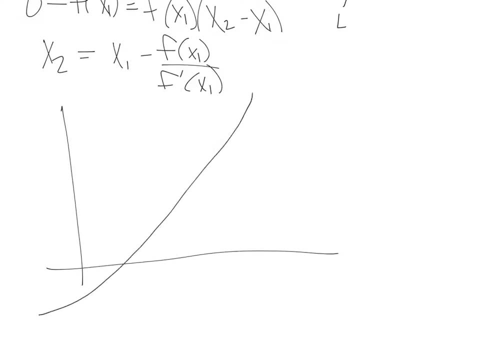 maybe a little bit bigger. so we had our point. this is the point x one comma. f of x one. this is x one right here. that's r over x and y. this is the graph of f of x. 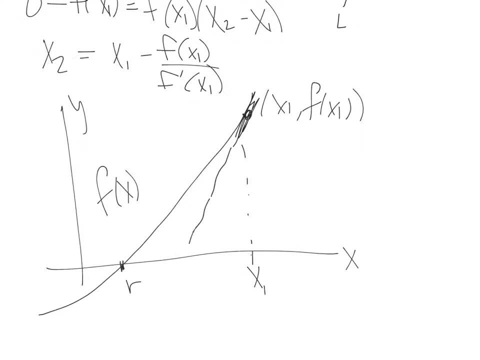 we found the tangent line right here. tangent line crossed at this point. this is our point x two. so now, if we move x two up to the line, we have another point x two, comma f of x two. 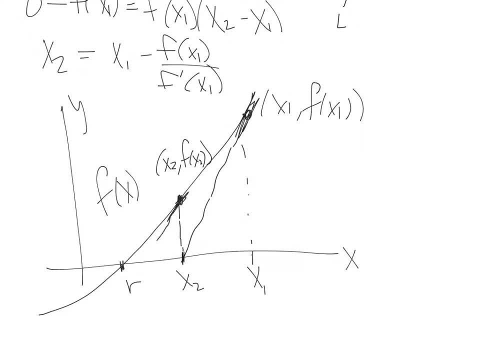 and we'll do the same thing. we'll find the tangent line right there and it crosses and we'll get another point, x three, each time we're getting closer and closer, and then from x three we'll move up. 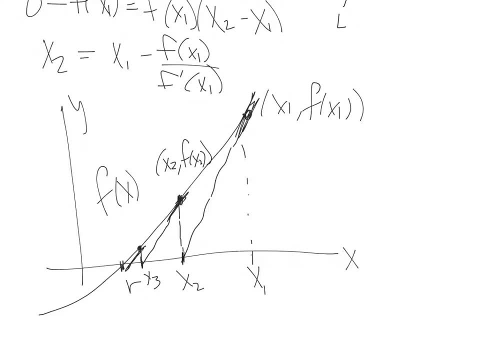 find that, and then they'll get closer and closer and closer. so what would x three be? well, using the exact same method we did, we would have found out that x three was equal to x two minus. 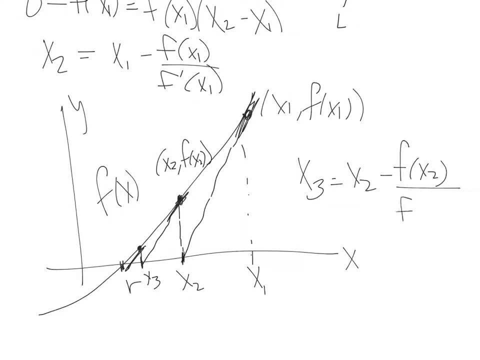 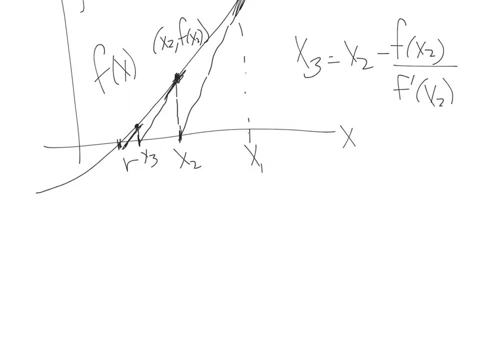 f of x two divided by f, prime of x two. so this leads us to the formula for Newton's method. if we have that the derivative does not equal to zero, we can find the nth approximation. so this one right here. 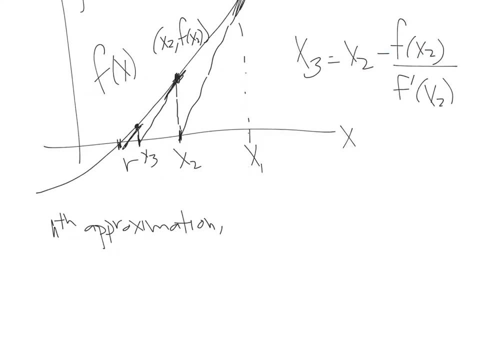 would be the second approximation, the one that we did above to find x. two would have been the first approximation, and so to find the nth approximation, what we would do is we assume that f prime of x of n. 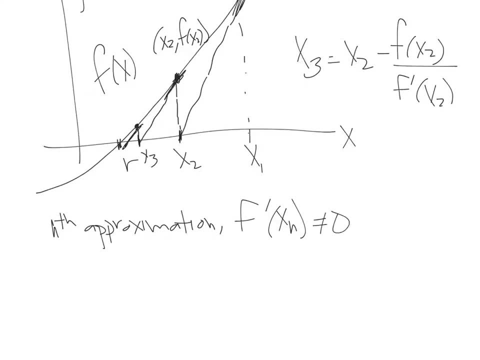 is not equal to zero, then we're given, and I'll go ahead and change my marker for this: we're given that x to the n plus one is equal to x to the n minus f of x to the n. 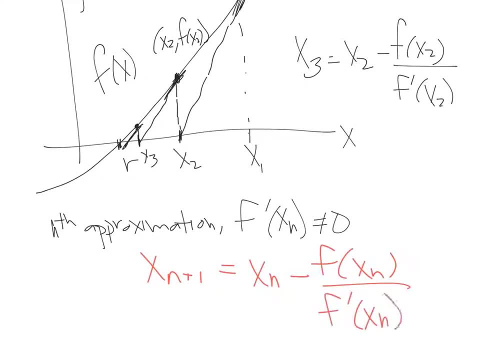 over f prime of x to the n. this is Newton's approximation, and we can do this to help us approximate our zeros, and if we do it more and more, we'll get closer and closer and closer. 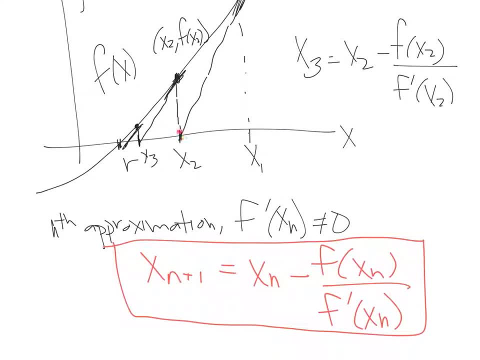 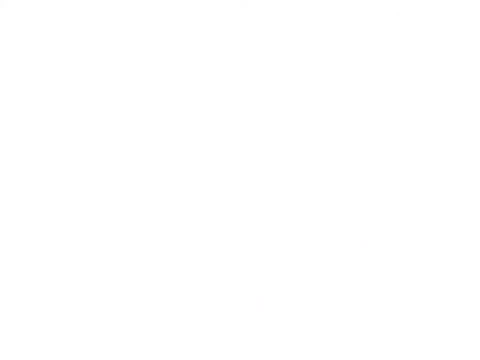 towards r. we started off way out here at x one, then we moved our x two, got a little bit closer, x three: we get closer, and we can get on and on and on. so let's do an example. 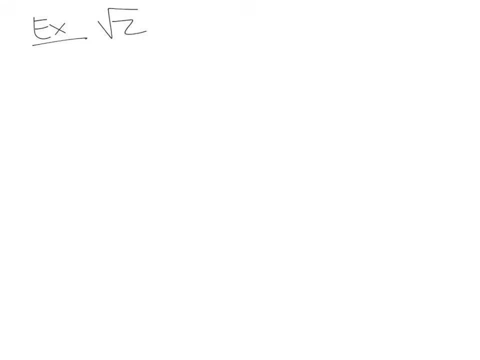 so if we wanted to find an approximation for the square root of two, what we would have to do would be to approximate. the zero of f of x is equal to x squared minus two. so if we wanted to find 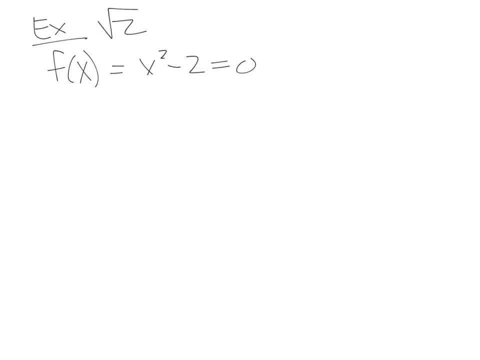 when this is equal to zero. you could see manipulating this. we found we would find that x is equal to zero or x- sorry- is equal to the square root of two. so this is the function we're going to deal with. 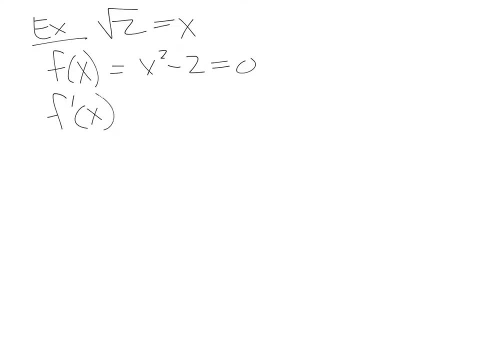 we need one piece of information, and that's the derivative. so f prime of x, and this is equal to two x. so now Newton's method will say that x to the n plus or x sub n plus one. 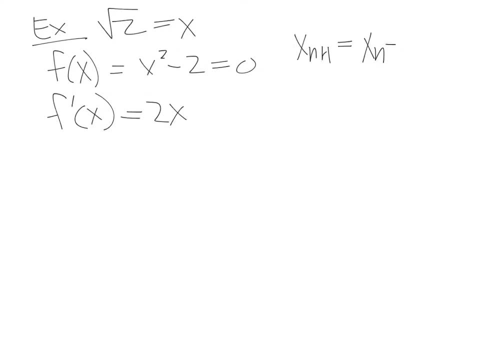 is equal to x sub n minus our f of x, which is x squared minus two. but remember we're dealing with x sub n instead of just x. so this is x sub n squared minus two over the derivative. 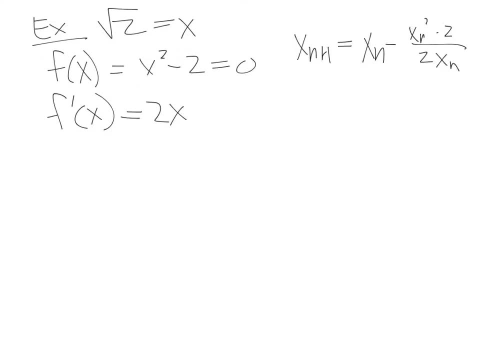 two x or two x sub n. now I'm going to go ahead and just simplify this. I'm going to break up this fraction into two fractions, so we're going to get x sub n squared over two x sub n. 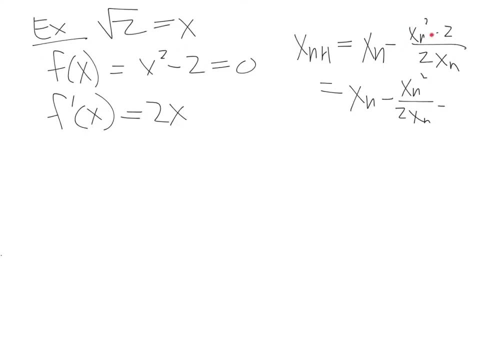 and now we're doing a minus, a minus two. so minus a minus gives us a plus two over two, two sub x n, and this simplifies. we get x sub n minus here. our x n cancels. 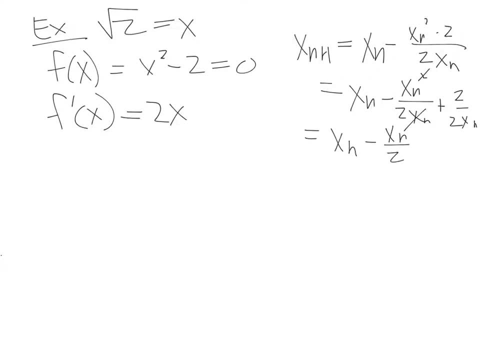 so we get x? n over two plus and then our twos cancel one over x sub n and we can combine the first two terms. one minus a half is just a half, so x sub n over two. 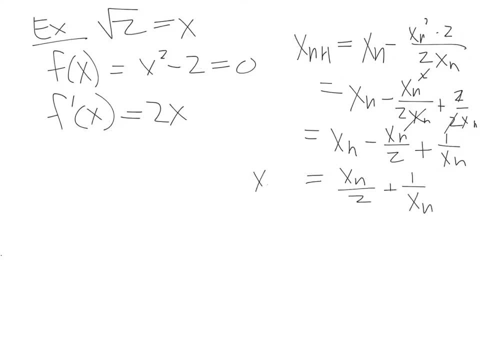 plus one over x sub n. this is our approximation that we'll be using in this example. now we do know, because we have calculators, what the exact value or a good approximation of the square root of two is. 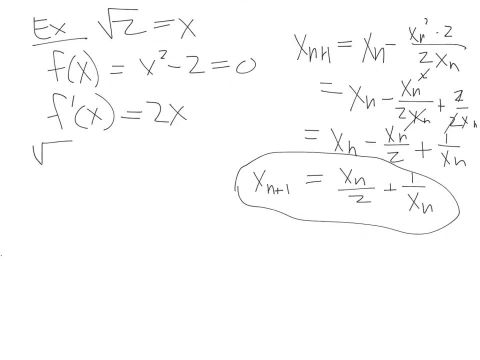 and so if we were to calculate square root of two to five decimal places, we get: the square root of two is equal to one point one, one point four, one four, two, one. so we're going to. 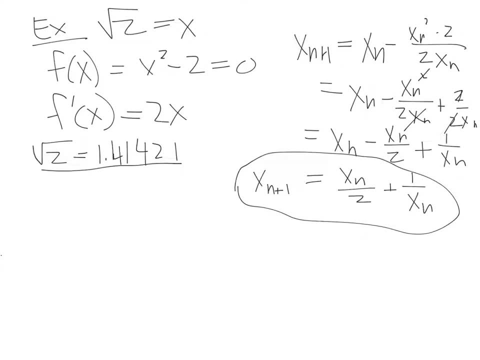 have this and now let's start computing. it would be nice if we kind of knew where to begin and we can sort of figure out that the square root of two is going to be between one and. 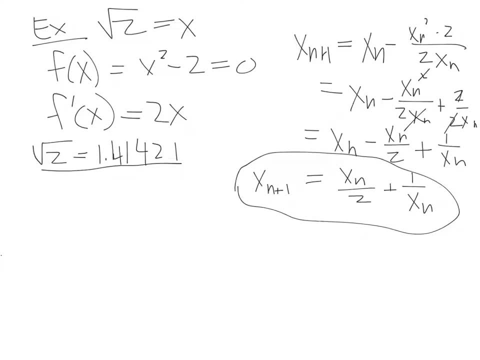 two, because we know that the square root of four is two and the square root of one is one. so we know this: the square root of two is between the square root of one and the square root of four. 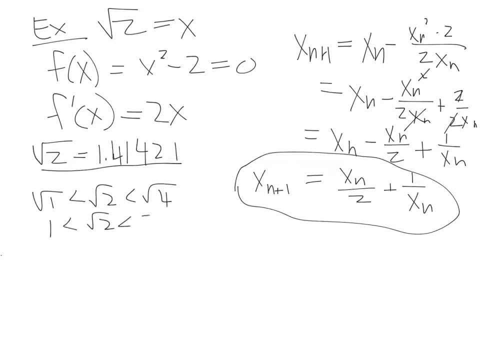 so we know the square root of two is between one and two, so we'll have to pick some number at least that gives us a ballpark area. we're not picking. the square root of two is approximately a hundred, so let's start off. 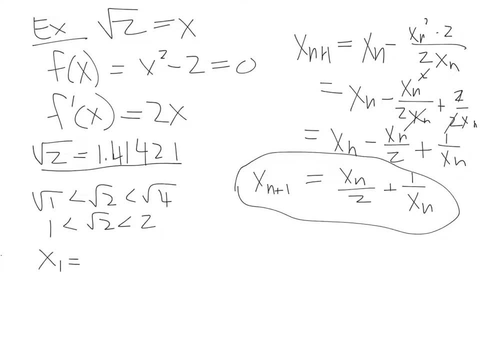 with x sub one is equal to, or x sub zero, or, very first thing, is equal to one. then plugging it in, what do we get into this equation? so, plugging this in, we get into our formula. 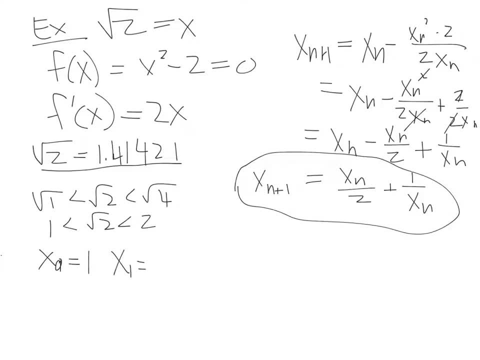 x sub one, which is x zero over two plus one over x zero, which is one half plus one over one. we get one point five. and then, for the next term, x sub one. well, x sub one we found is one point five. 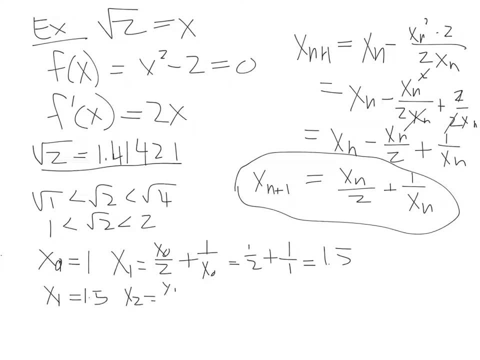 so we get x sub two is going to be x one over two plus one over x sub one, which is one point five over two plus one over one point five, and this gets one point four one. 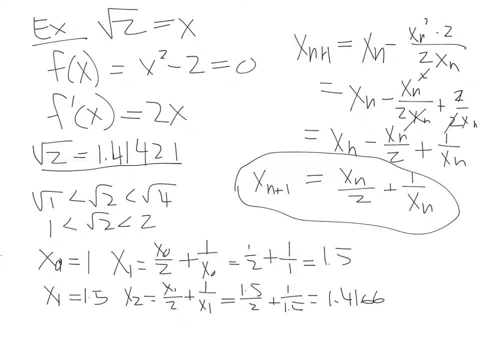 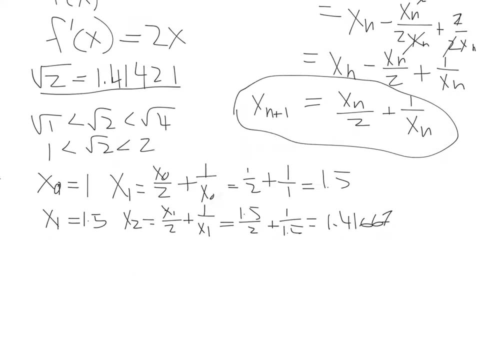 six, six, repeating forever, and we'll call this six, six, seven, and then we'll do x sub three would be x sub two over two plus one over x sub two, which is equal to one point four. 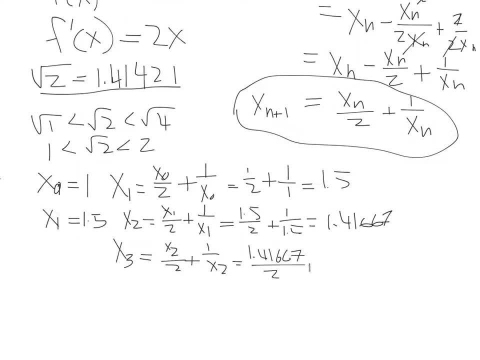 one six, six, seven over two plus one over one point four, one six, and this would give us one point four, one four, two, two. so we only did a couple of calculations. 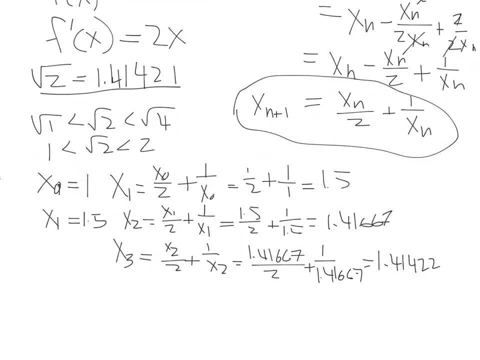 we started. when x is zero, when x is going to be one. then we got one point five, one point four, one, six, six, seven, and we got one point four, one, four, two, two, remember. 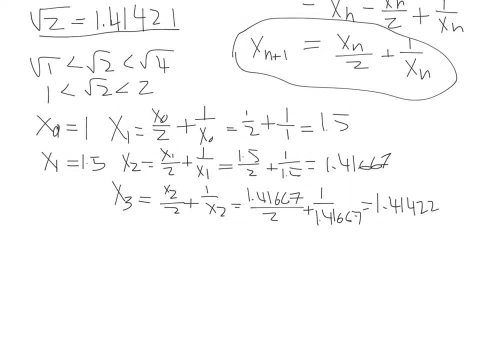 the square root of two. we could take a look at the error that we had, and so, if our value for x zero is one, x one is one point five, x two is one point four, one, six, six, seven. 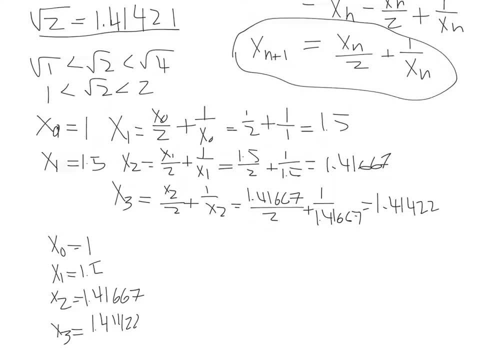 and x. three is one. point four: one, four, two, two. the error we get is going to be the first number off by point four, one four, two, one, and this is negative. then the next. 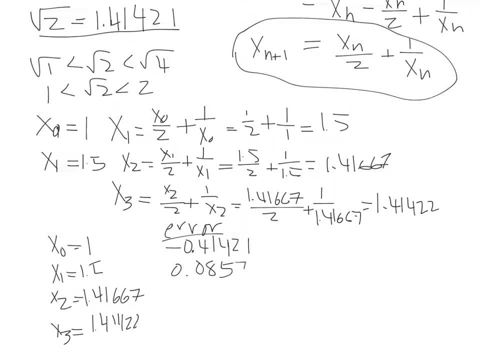 error. we got point zero, eight, five, seven, nine- we're getting better- and then we get point zero, zero, two, four, six, and then we get zero, zero, zero, zero, one. 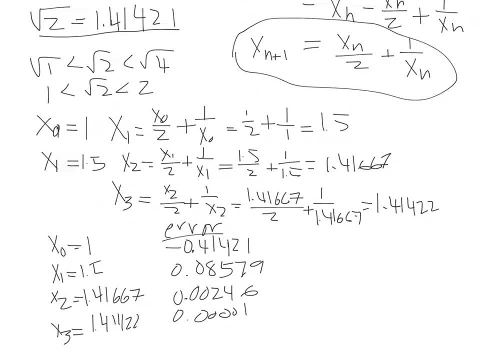 five digits of accuracy. so this is Newton's method, and we use it to get approximations, and sometimes- in this case, we get an approximation by just using a couple of calculations. today we're going to talk about 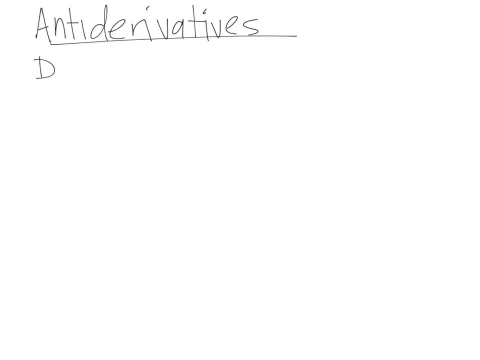 anti derivatives. we'll begin with a definition. a function, capital F, is called an anti derivative of the function little f on an interval i, if we have capital F, prime of x, the derivative of that. 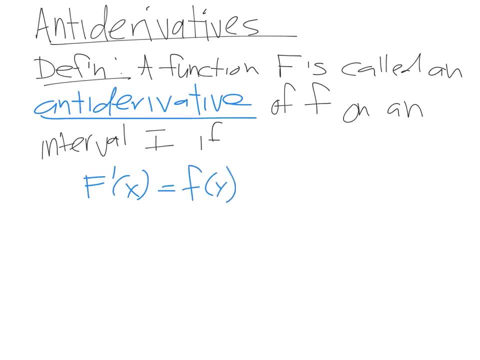 is equal to little f, and this is going to be for all x in the interval i. so what this is saying is before, if we had some function little f and we took the derivative f prime, that would be its derivative. 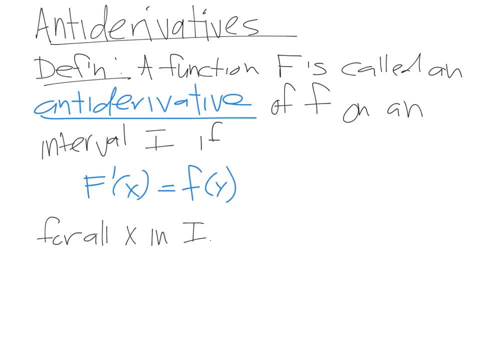 now we're going the other way. we're taking the anti derivative, and this often, often happens when we have some function, little f, or we're going to call it capital F, prime, and we we don't know. 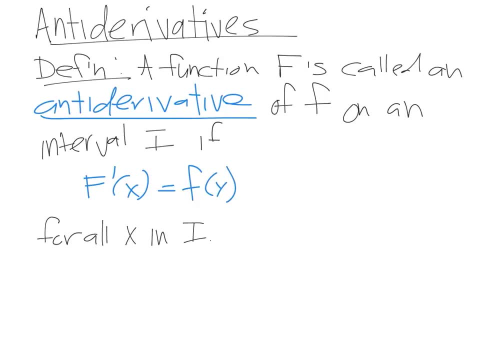 we know the derivative, but we don't know what the original function was. so we take the anti derivative and that's what we would get, capital F. so let's do an example: if our function f of x is equal to two x, 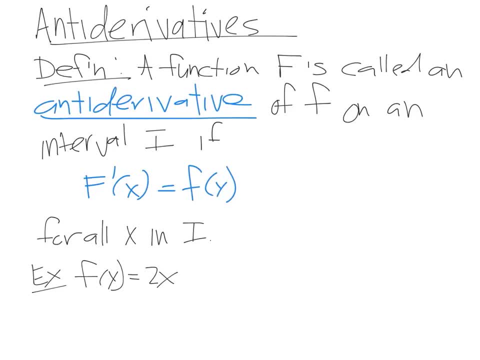 what's the anti derivative? well, in this case we need to think about what function whose derivative is equal to two x. well, if you remember, our original function would be x squared. the derivative of x squared is two x. 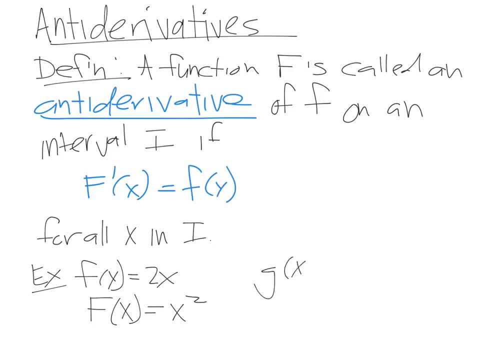 similarly, if we have a function g of x is equal to cosine of x, what would its anti derivative be? the derivative of what is cosine? well, the derivative of sine is cosine, so in this case, sine of x. 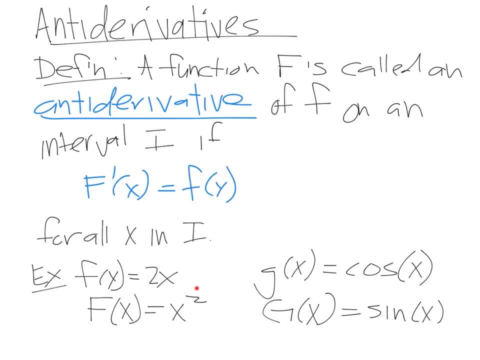 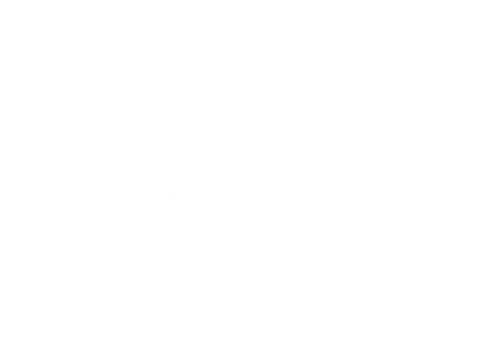 is the anti derivative of cosine and x squared is the anti derivative of two x, in the same way that two x is the derivative of x squared or cosine is the derivative of sine. but let's say we have functions. 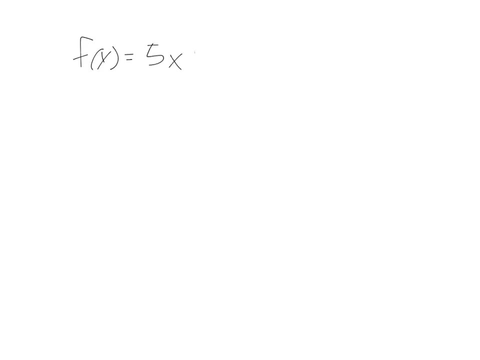 f of x is, let's say, five x plus four. the derivative of this is five. but if we also had another function, g of x, who was five x plus 80, the derivative of g is still five. 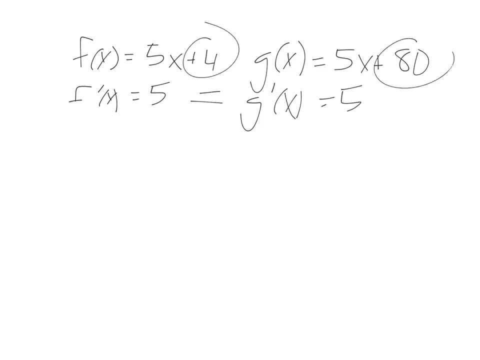 so they're both going to be the same. the derivatives are the same as long as we have some, as long as the constants can be different, and then the rest of the terms are going to be the same. so the five x's. 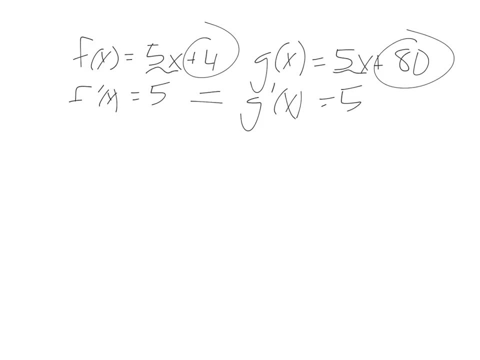 are the same, it's just the constants would be different. so this leads us to a theorem: if capital F is an anti derivative of F on an interval, i then the most general anti derivative of F. 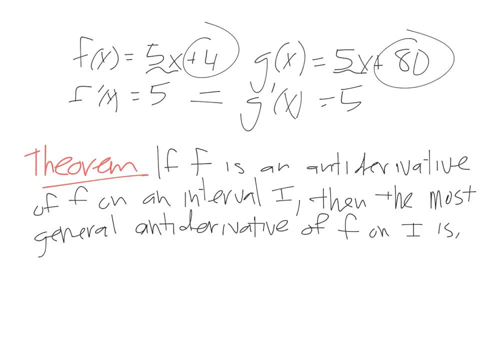 on. i is the following is going to be capital F of x, but we're just going to add some c plus c, because it doesn't really matter as long as c is a constant. so 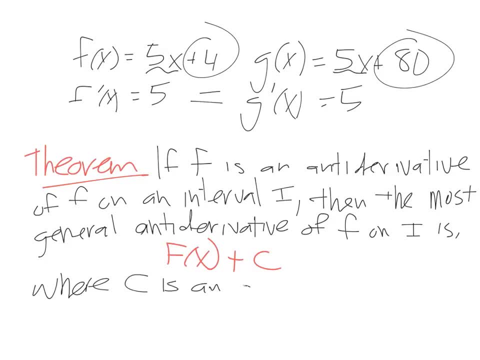 where c is an arbitrary constant, because if we took the derivative of capital F, or rather of this whole thing, the derivative of all of this, the derivative of capital F becomes F prime, which is the anti derivative and the derivative. 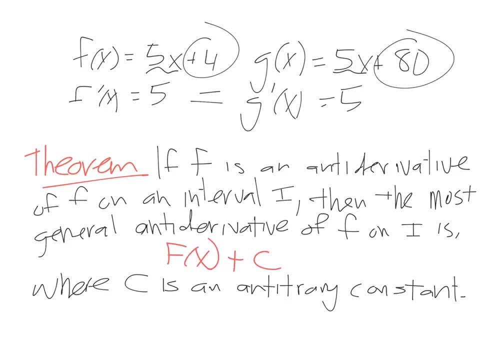 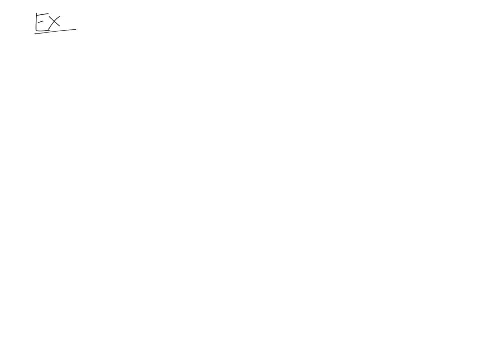 of c is zero. now let's do another example: find the most general derivative- or anti derivative, excuse me, of F of x equaling x to the n. well, we're doing the power rule, and if we're taking the derivative, 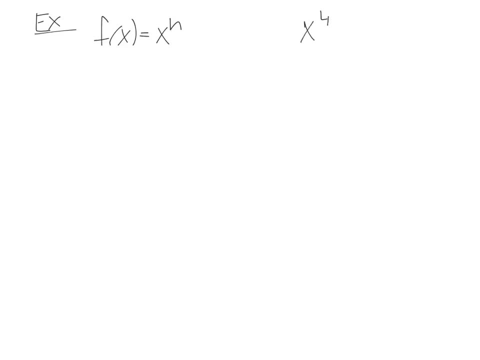 of, say, x to the fourth power, that would be four times x to the four, or, excuse, x to the four minus one. so if we're going this way, taking the derivative, we're subtracting one. 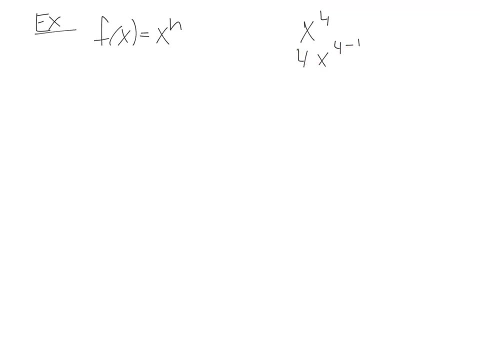 and multiplying by that power. if we're going to go the other way, what we would do is we would, instead of multiply, we would divide, and instead of subtracting one, we would add one, so we would. 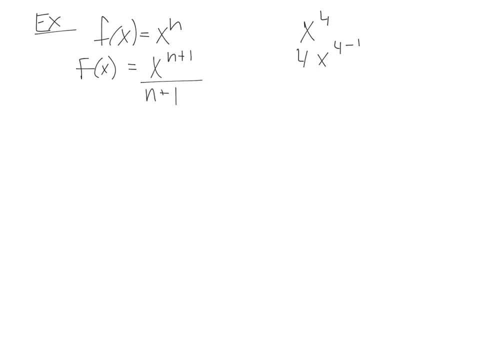 add one up here and divide by that power and we can test this. what's the derivative of this? well, the derivative capital, F, prime is going to be the power times, our power, our function to the. 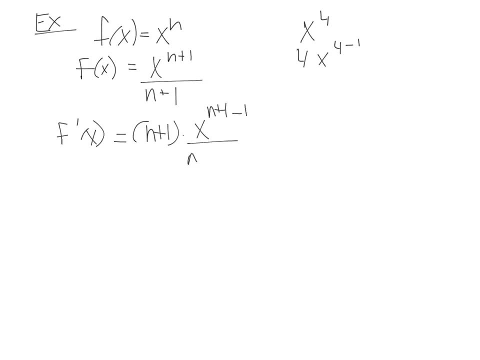 n plus one minus one power. so n plus ones cancel, and we're left with just x to the n, which is what we started with. so this leads us to a series of anti-derivative formulas. but before we do that, 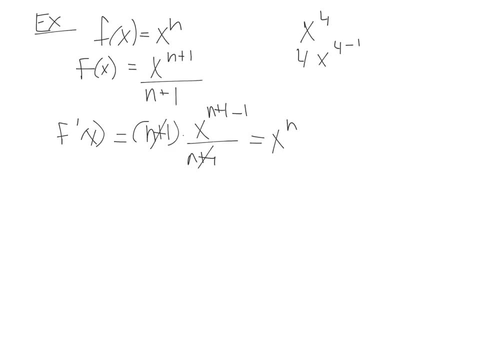 I forgot that I was asking for the most general anti-derivative, and so that would be a plus C, and so we'll have a function, and then we'll have the particular anti derivative. so if our function 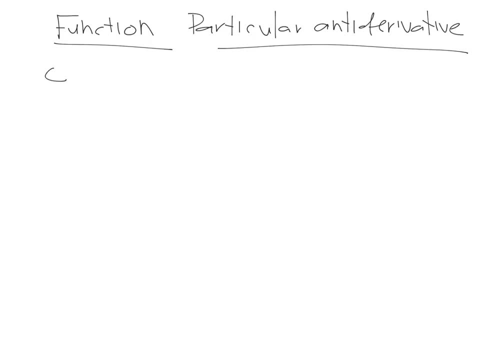 is some constant C little case: C times our function F of x and the particular anti-derivative is still C times F of times our capital F of x. if we're adding two functions F plus. 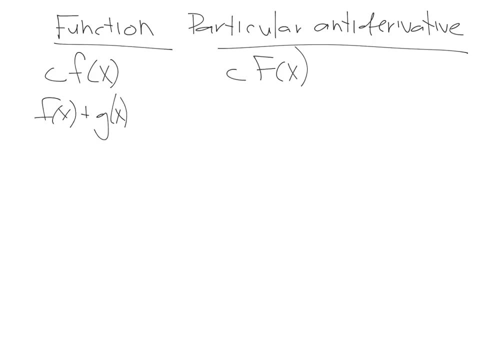 G of x, then what we get would be the sum of two anti-derivatives: capital F of x plus capital G of x. if we have the power, rule n to some power, and we're gonna assume in this case, 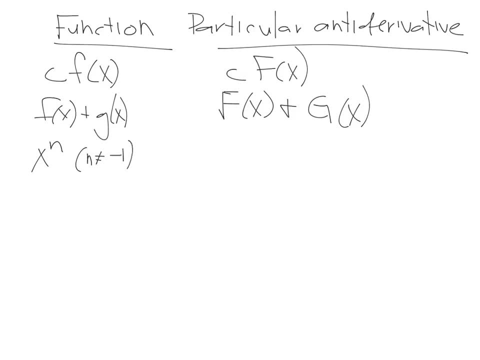 n is not equal to negative one. if we have this, then we get x to the n plus one over n plus one. that's our anti-derivative. if our function is cosine of x, then the anti-derivative. 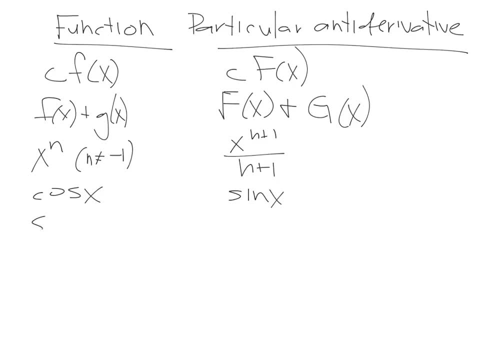 is sine of x. but what about sine of x, derivative of what would be sine of x? well, derivative of cosine is sine. so, really, using this first formula, so derivative of cosine is negative sine, so we would take the negative. 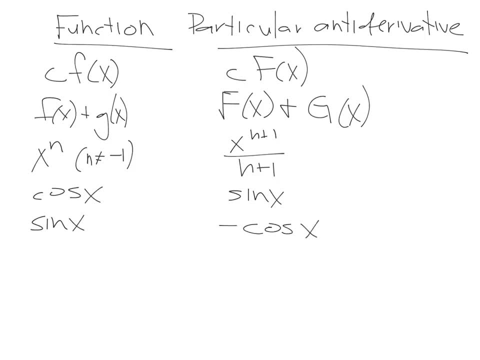 and this would be negative of cosine of x. if secant squared of x is our function, the anti-derivative, the derivative of what would be secant squared. well, if you recall, the derivative of tangent is secant squared. 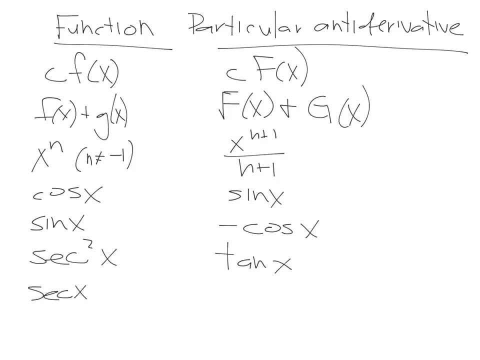 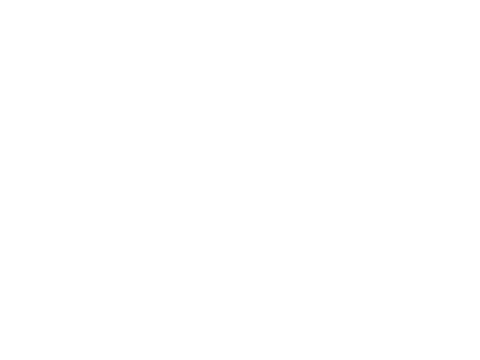 and then the derivative or the anti-derivative of secant times tangent of x. well, that anti-derivative is secant because the derivative of secant of x is secant tangent. so let's do an example. 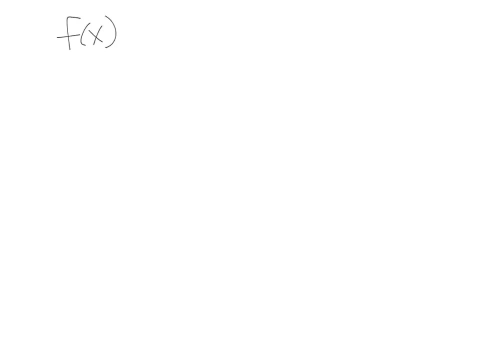 find the general anti-derivative of the function f of x is equal to three times the square root of x plus, let's say, sine of x. well, we can rewrite this. so this would be, instead of writing it. 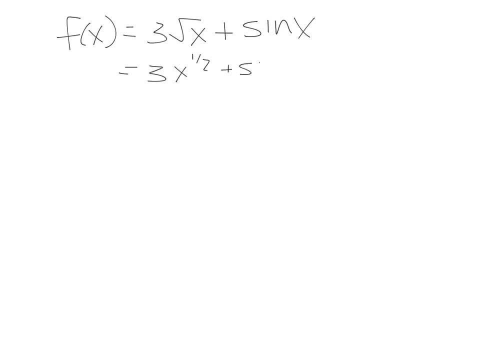 as the square root of x, we'll write it as x to the one half power plus sine of x, and so the anti-derivative of this is: we have two different things, so we can take the anti-derivative. 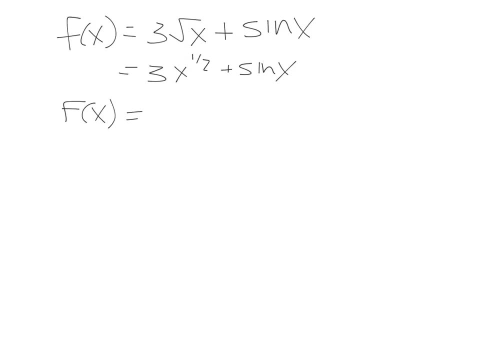 of each one separately, and so the anti-derivative of three to the x, three times x to the one half, would be three times the anti-derivative of x to the one half. the anti-derivative of x to the one half. 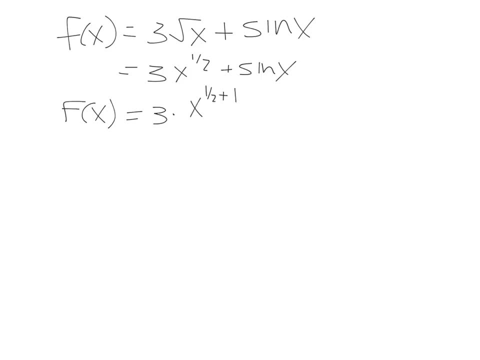 would be x to the one half plus one divided by one half plus one, plus the anti-derivative of sine. well, anti-derivative of sine is negative cosine of x and since we're taking the general, 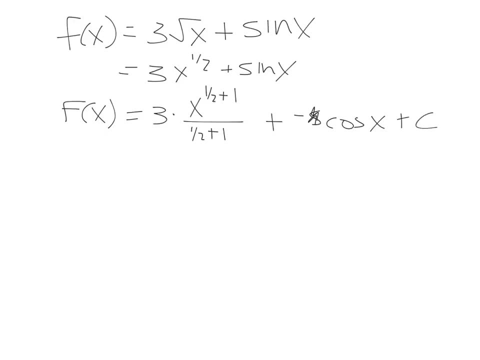 anti-derivative, we're gonna add plus c. so here we get three times x to the three halves divided by three halves, minus cosine of x plus c, but this three and three halves. well, we can simplify. 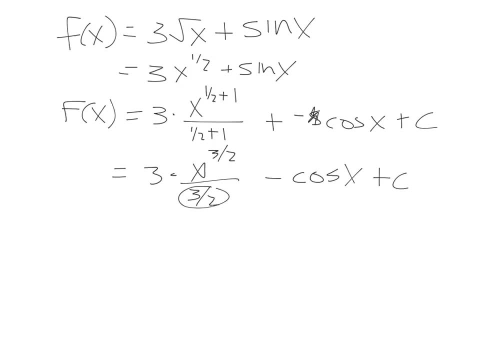 if we're dividing by a fraction, it's the same as multiplying by the reciprocal. so now we multiply by the reciprocal, our threes cancel. so this is just two x to the three halves minus cosine, x plus c. 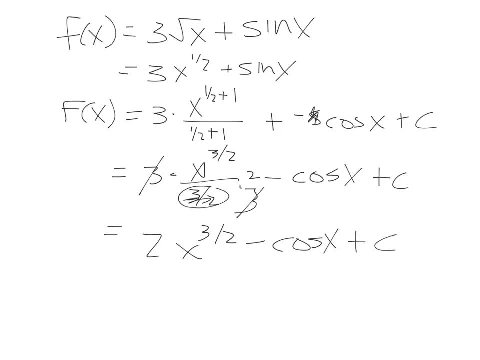 now, an equation that involves derivatives in the original function is an equation that we call a differential equation, because they have differentials in them, and usually these differential equations will have some sort of initial condition so that we can figure out. 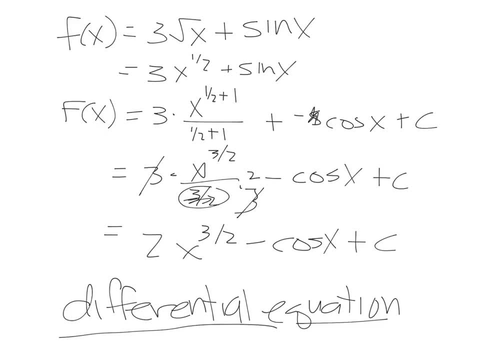 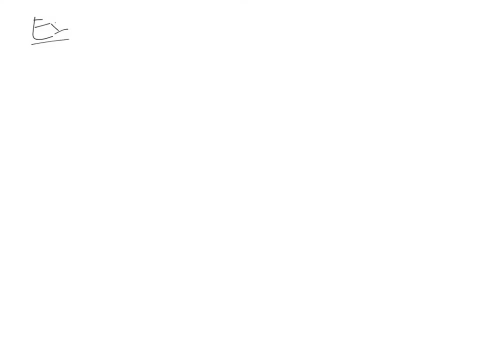 what that c value is that constant we get? so let's do an example now. recall that if we're dealing with something like s of t and that's the position, then the derivative of your position s prime of t 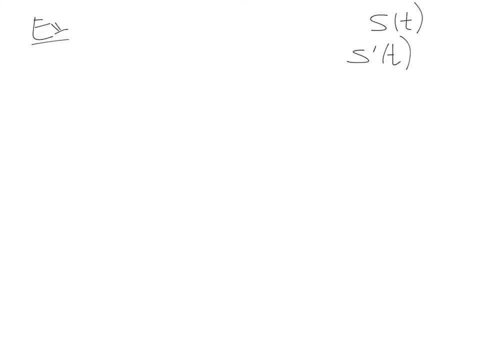 is gonna be your velocity and the derivative of the velocity or the second derivative of position. so the second derivative is the derivative of the velocity, which is acceleration, and so if we were to work backwards, the anti-derivative of acceleration. 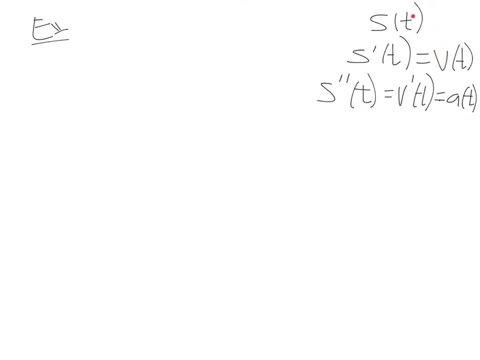 would be velocity, and the anti-derivative of velocity is position. alright, so now let's do this example. we have a hot air balloon is ascending at a rate of 12 feet per second. 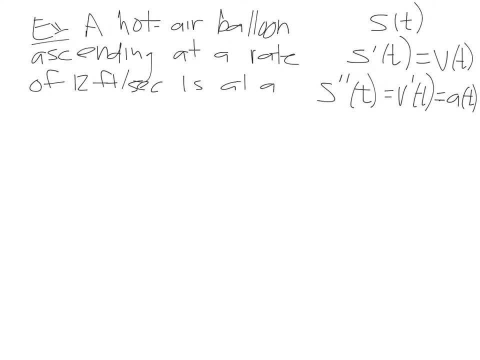 and is at a height 80 feet above the ground, and when it's at 80 feet above the ground, this is when a package is dropped. what I wanna know is: how long does the balloon? 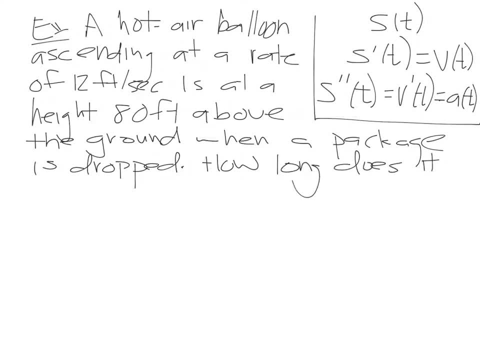 does it take the package to reach the ground? so in this case, we're gonna start with the velocity, and so we're gonna call the velocity v of t, and I'm gonna change my color to: 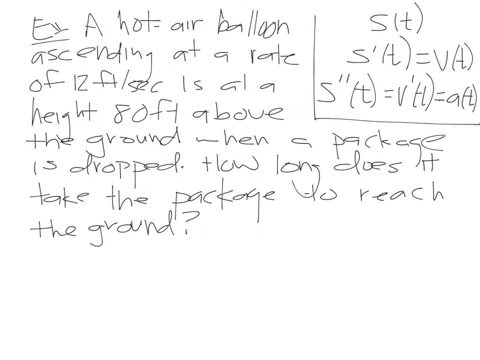 blue for the solution, just so that we don't get confused, cause there's a lot of words here now. the acceleration due to gravity is 32 feet per second squared, and this is for acceleration on earth. 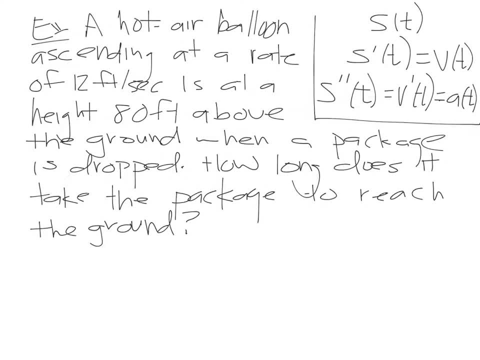 the gravity on some other planet is gonna be different. okay, so the acceleration due to gravity is 32, feet per second squared. so we have a of t equals 32,. now, if you're. 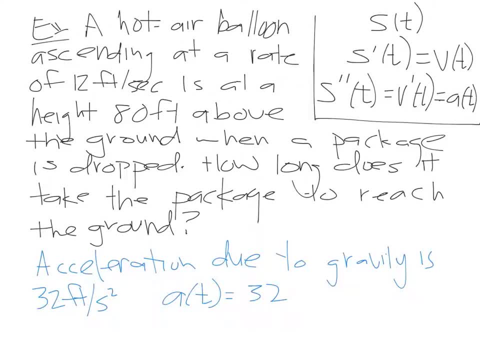 going up, then gravity is pulling you down, and so we'd write negative 32, and I'm just gonna drop the units. so that's our acceleration, now acceleration, and we're gonna refer to all these right here. 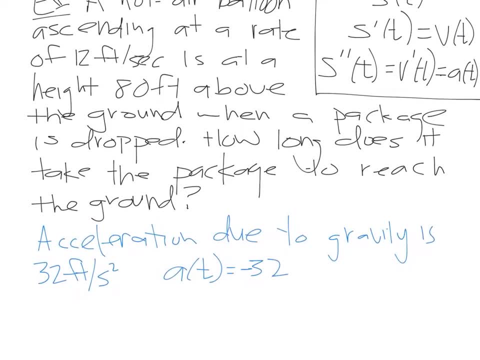 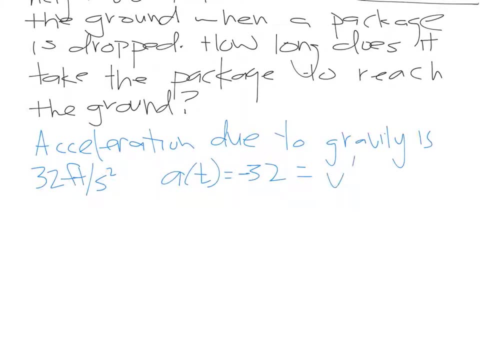 but I'm not gonna have it on the screen. so acceleration is really the derivative of velocity, so that's really v prime of t. so let's figure out what v of t is we wanna find. 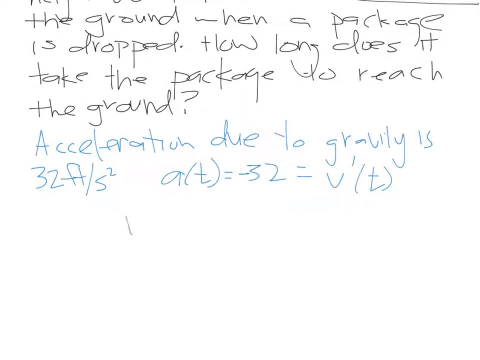 the anti-derivative so v of t, the velocity, is the anti-derivative of negative 32,. well, it's just negative 32, and so the anti-derivative negative 32, would be negative 32 t. 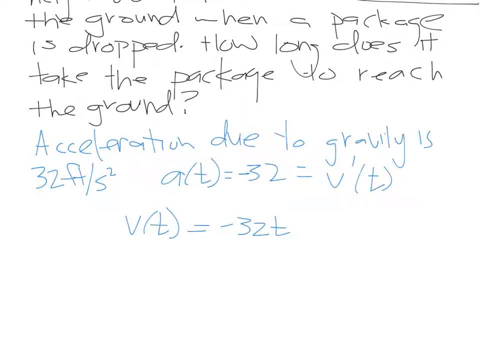 because taking the derivative of negative 32, t is just negative 32, now when we take the anti-derivative, we're gonna add a plus c. we get this constant. so here we have our velocity in terms of time. 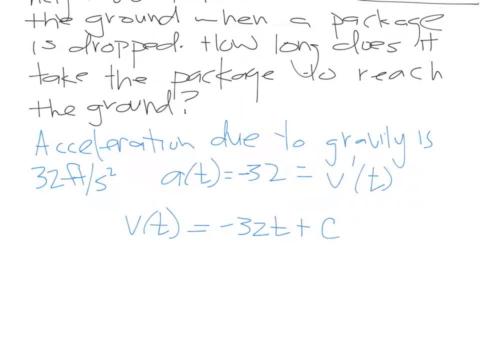 is negative 32 t plus c. now we think about our initial condition. so this right here, initial condition, initially, when time was zero, what is our velocity? so our velocity was negative 32, times zero plus c. 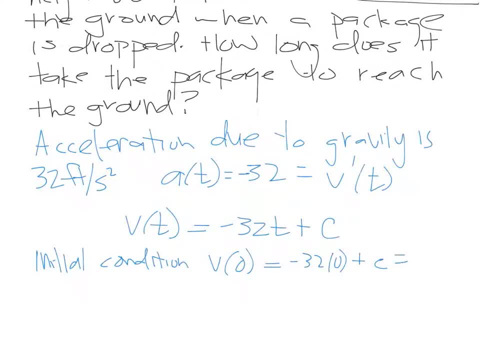 but we were in a balloon that was going up in the air. the initial velocity of the balloon was 12, because we're moving up, we are ascending at 12 feet per second, so this allows us to be able to figure out. 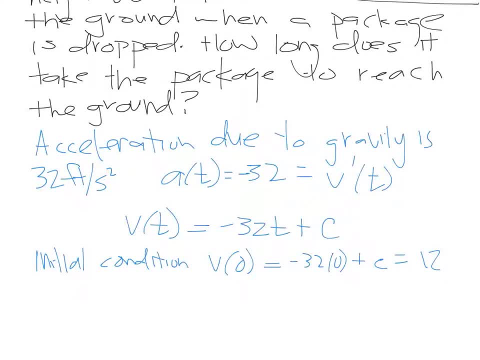 what c is. so we can evaluate c at c, and so our constant is 12,. so our new- and let me just change colors for this- so our velocity equation for that is gonna be v of t. 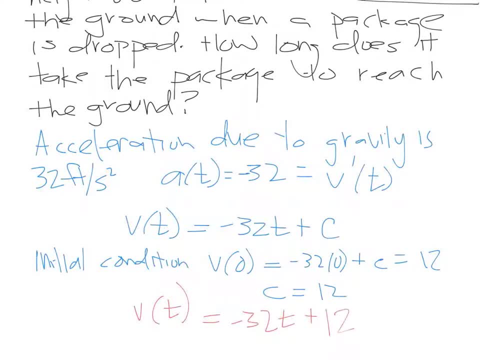 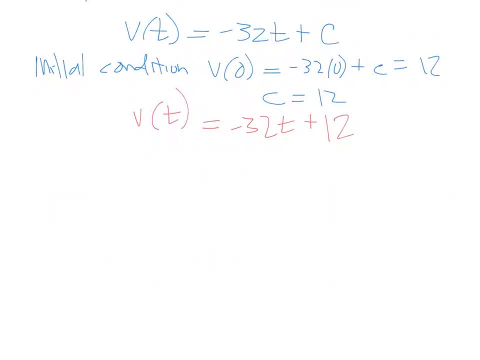 is negative, 32 t plus 12, so that's our velocity. now we're trying to find the position because we want to figure out what's the position function, so to find that we know that the position. 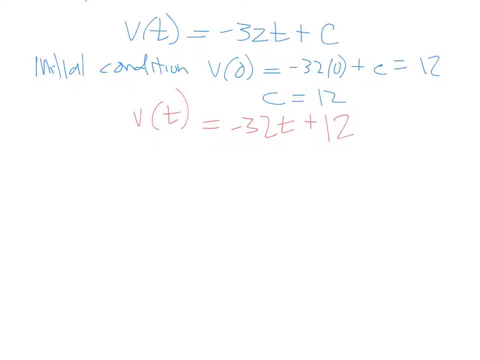 well, before I do that, let me just back up one more step. velocity is the same as the derivative of the position. so velocity is the derivative of the position. so we can figure out what's the position s of t. 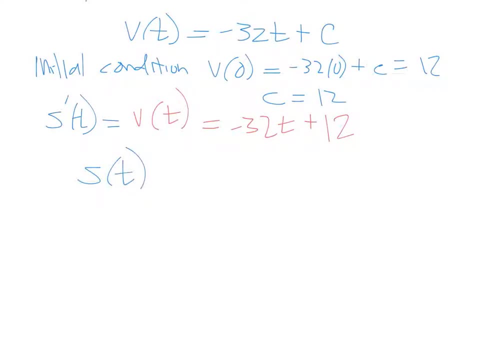 we take s of t by taking the anti-derivative of the velocity. so the anti-derivative of negative 32 t is negative 32,. anti-derivative of t using the, the formula we have, you add. 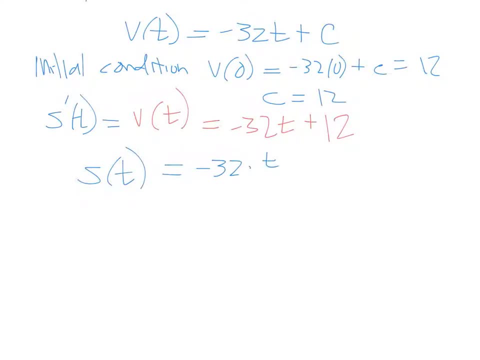 t to the power. this is already really t to the power of one, so you do t to the power of one plus one, which is two over two plus now we're going to have 12, the anti-derivative of 12 would be: 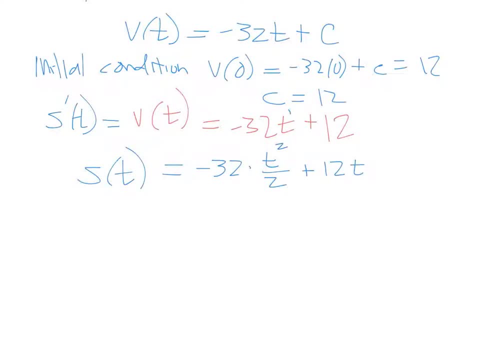 12t. and now we're going to have another constant when we take the anti-derivative, so let's call this constant. since we've already used c, we'll call this constant d. so now we have an equation. 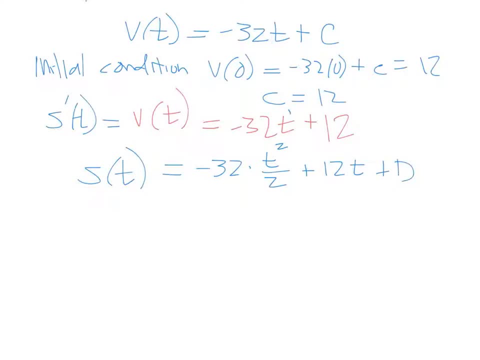 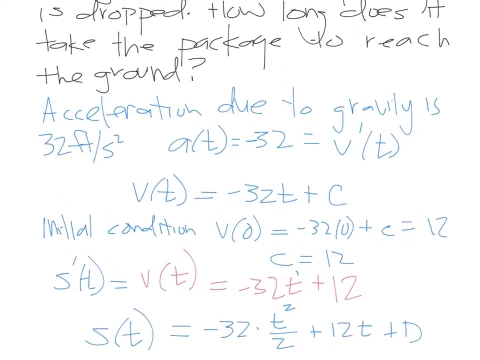 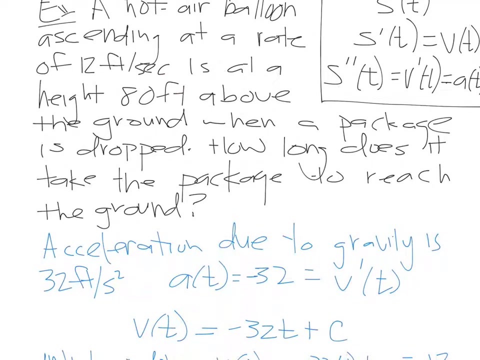 for s of t, but we still have a constant. now we again, we use our initial condition, and so, if we remember back from the equation, initially the package was dropped at a height of 80 feet. so, moving back down to here, 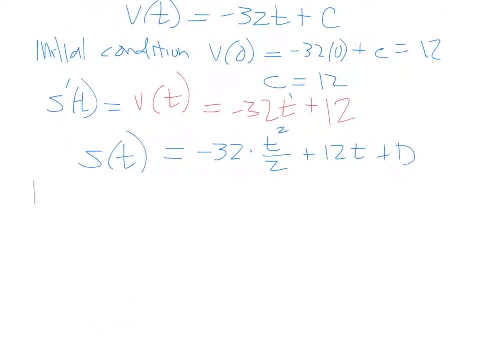 initial condition we're going to have: initial height s of zero is going to be 80 feet above the ground. in fact, we can simplify this because we have negative 32, divided by two. so let me just write it down here. 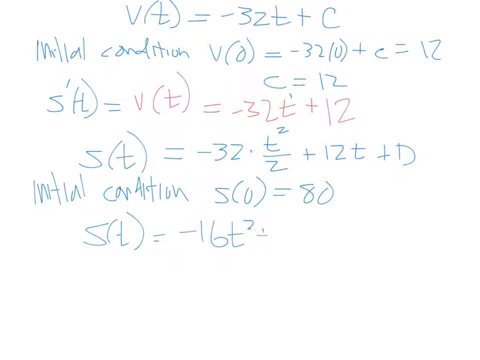 s of t is going to be negative: 16, t squared plus 12t plus d, and so, plugging in our initial condition s of zero, we get zero plus zero plus d is equal to 80,. 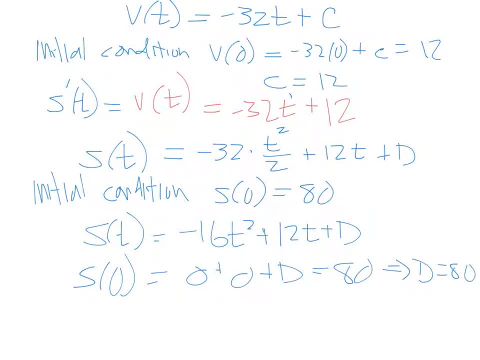 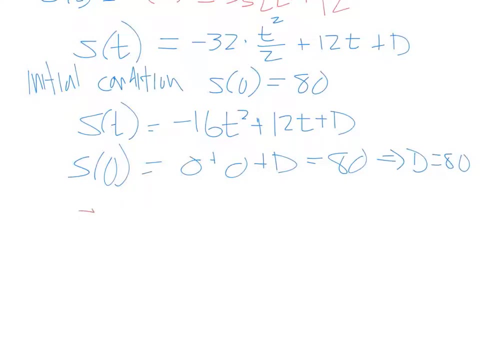 so we know d is 80, and now we can figure out what's the formula for height. so the formula for the height is going to be negative, 16, t squared plus 12d, and we had plus d before. 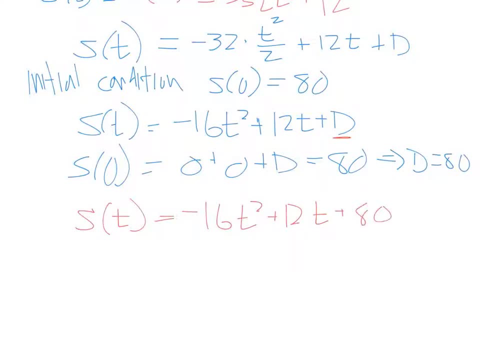 but now we know d is going to be 80, so this is the equation for the height. what we wanted to do is we wanted to find what's the time when the package hits the ground. so what we want to do, 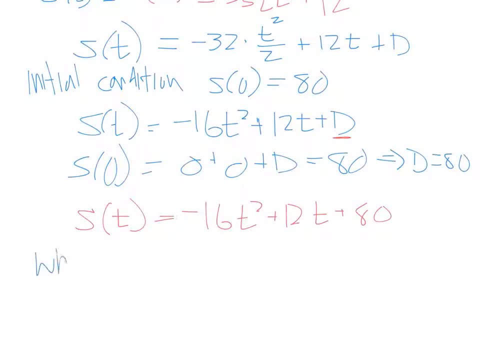 is. we want to find what is t when your height is equal to zero. so we're going to set zero equals to negative 16, t squared plus 12t plus 80, and so we can solve this. 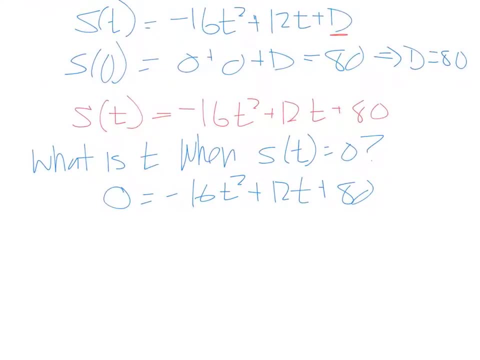 maybe say using the quadratic formula or your graphing or however you like to solve equations, and we get that t is going to be negative, 12, plus or minus the square root of 12 squared minus 4,. 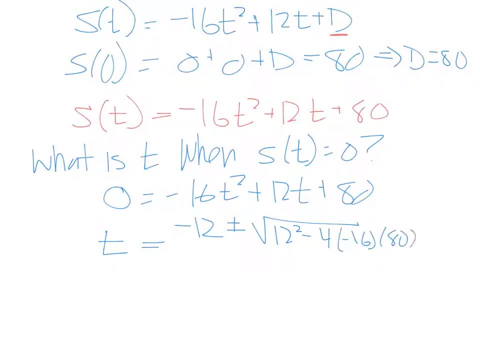 times negative: 16, times 80, divided by 2 times negative 16,, and so this would give us that t is approximately negative 1.89, or t is approximately 2.64 seconds. now we can't have a negative time. 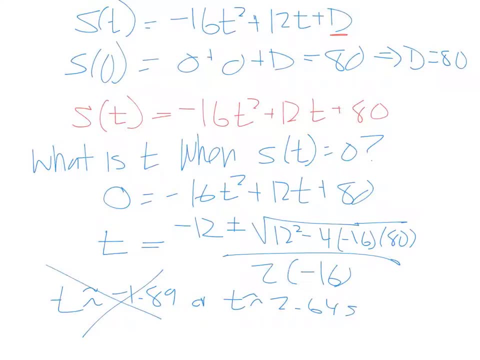 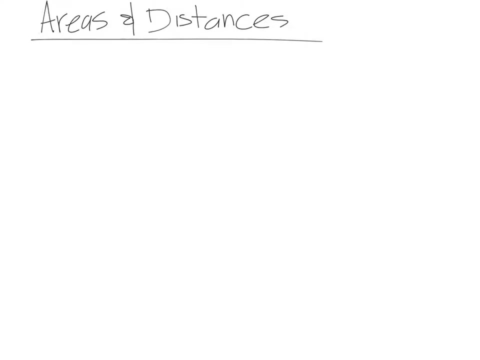 so we rule that out, and so we get for our answer. it takes about 2.64 seconds to hit the ground. today we're going to talk about areas and distances, so let's first take a look at the curve. 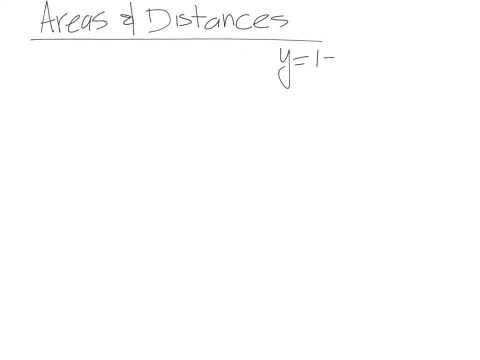 y is equal to 1 minus x squared. if we were to plot that, what that graph looks like is something like this: so this is 0.5, and we have 1, and so 1 minus x squared. 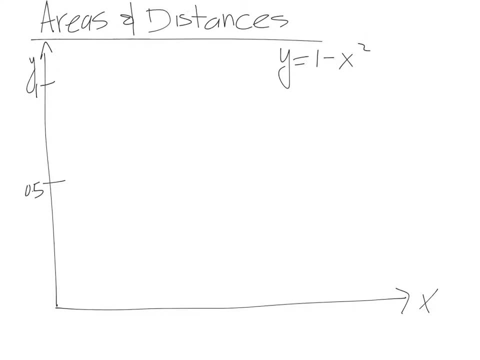 that is a parabola facing down whose vertex is up at 1, so we have this something like this: it crosses down here at the point 1, so now, given this, how can we figure out? 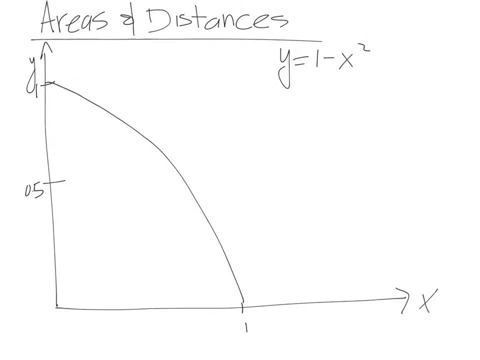 what's the area under this curve? what is this area? now, we know how to find areas of nice geometric shapes like a rectangle or a triangle, but this is neither of those shapes. what we can do is we can make an approximation. 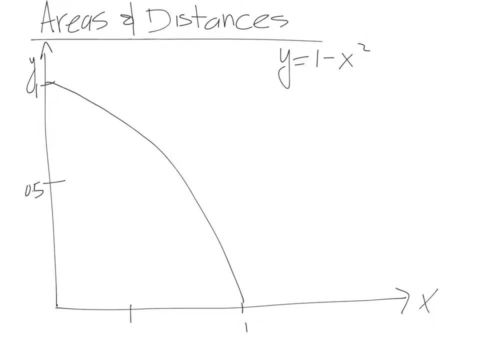 and we can say, well, let's sort of break this off into two different rectangles, and so we'll pick the point right here and we'll go across. we have something like this, and then again at this point right here: 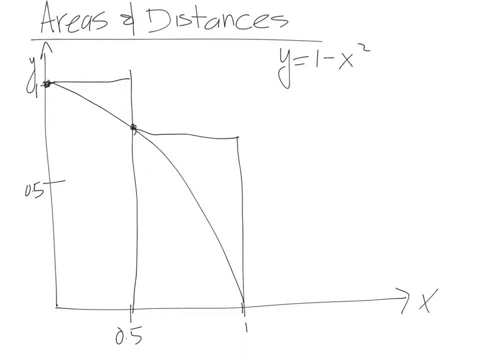 we'll go across and we'll go back down and so, shading, what we'll get is we'll have two rectangles. but the thing is, this is an approximation, but it's a bigger approximation because this area right here, 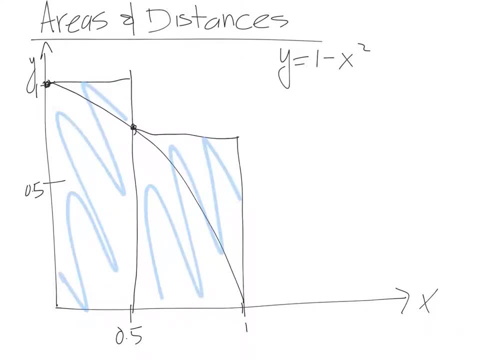 and this right here we're counting that in our approximation and that doesn't fall in there. so in fact maybe I should have colored this a different color. so this is all the extra shading and that shouldn't belong there. 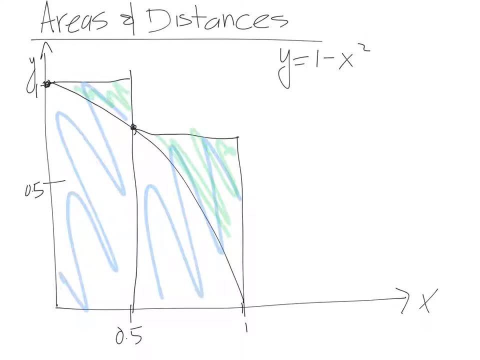 can we do a better approximation? sure, so let's try. so, instead of using two different rectangles, let's make four rectangles, and each of these rectangles is going to be equidistant, so this is going to be 0.25,. 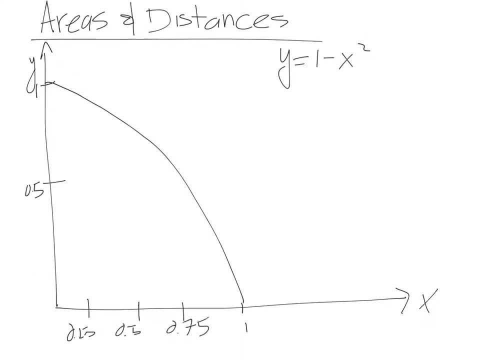 0.5,, 0.75, and 1,, and so we're going to go ahead, start up here, go across, we hit that, and then each time, I'm going to start at the left, wherever this line. 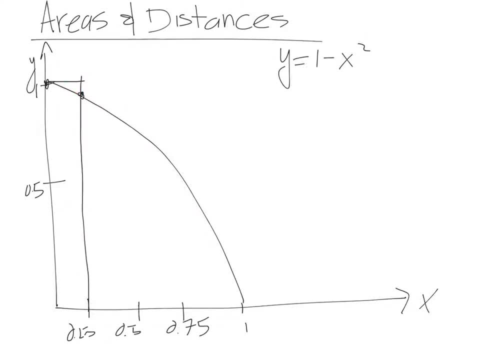 touches our curve. I'm going to start right there. so we go ahead, go across, then we go up, take that point, go across, up and then go across and up. so now we have four rectangles. that's approximating this. 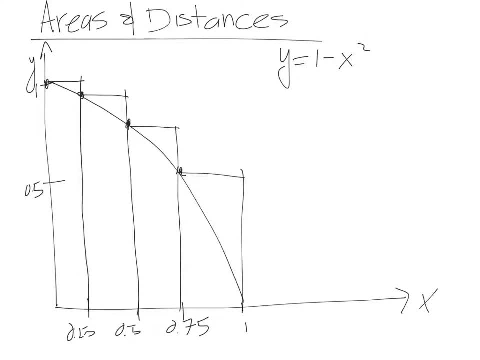 and this is getting a little bit better. so you see, the error is better, it's not as much, and I'm going to draw our first approximation. so our first approximation actually went all the way up here and went all the way over here. 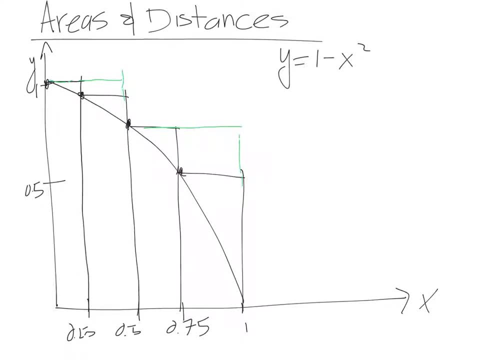 and if we were to shade that, that first approximation had a much larger error, all of this area, so that's a pretty big area. our second approximation, the error, the error is just these areas. so we got a little bit better. 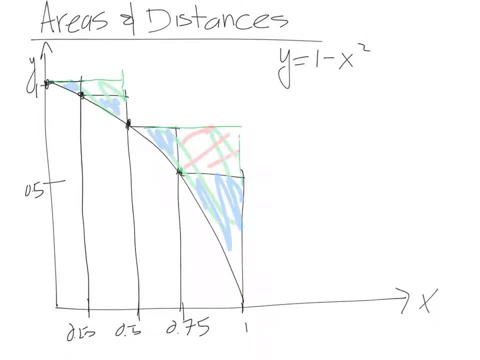 we no longer had this as our error. so we're improving. could we do better? sure, let's just make more rectangles. so if we made more rectangles, so each of these rectangles would have a distance of .125,. 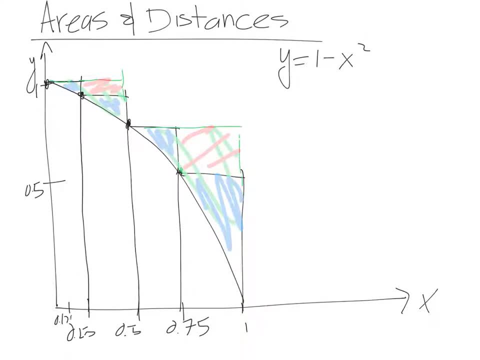 instead of .25,, so 0.125,. then what that would be is we'd have this first one and now we'd go over here and then, following this, we go up and actually I'm going to change my color. 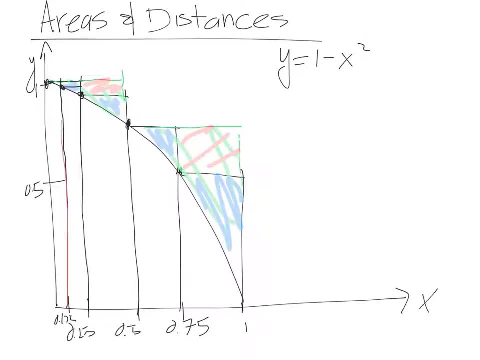 for these lines. okay, we have that. go right here and then keep having each of these, and so again, you're going to see our error is getting better and better and better. so now the error that we get. 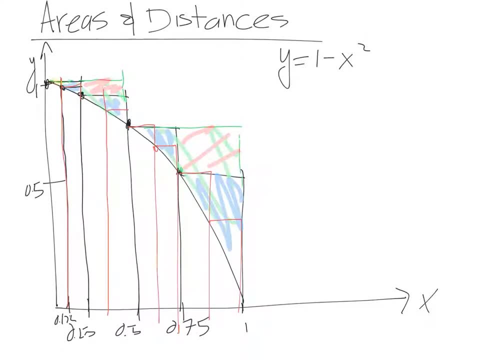 is far better than ever before. let me use a darker shade. so each of these errors is smaller and smaller, so we are getting more and more accurate. so, compared to our first approximation, where we used two rectangles, 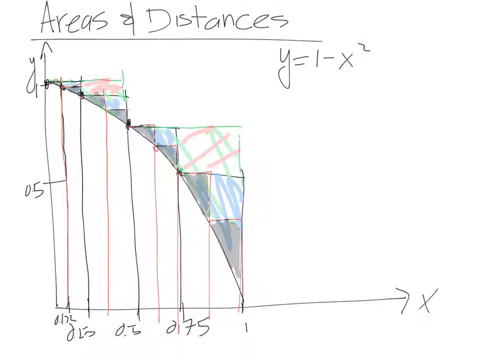 this is much better. and then we used four rectangles. it got better. now we're using eight rectangles and we can use more and more and more, and we get better and better and better each time. 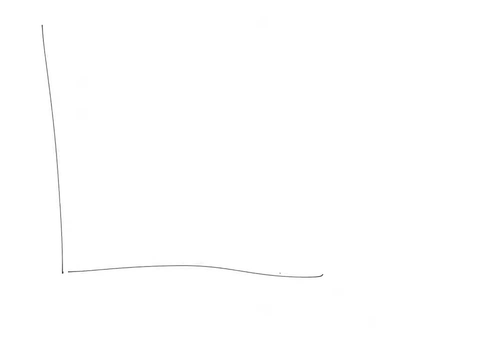 so just redrawing this on a clean slate so we get: y is equal to one minus x. squared this point right. here is the point one, comma one. and if we had split this up and let's say: 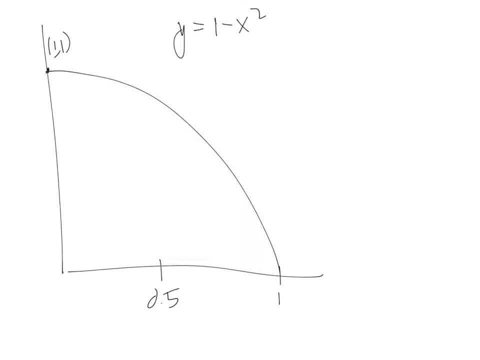 let's just do four approximations. so we have one or four rectangles, rather we have two, three and then four approximations. now this approximation we're going over, so we're we're missing over two large of an area. 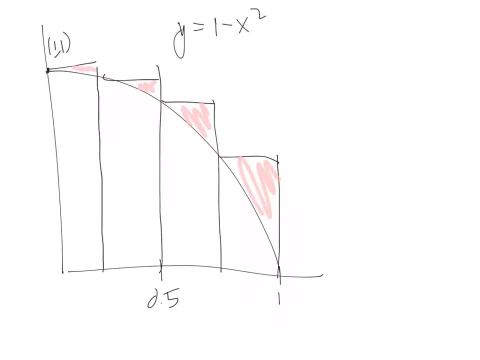 by that. now, this approximation we're going to be using for each of these rectangles, we're using the left hand end point and we're using four of these, so we're going to call this l four for the left hand approximation. 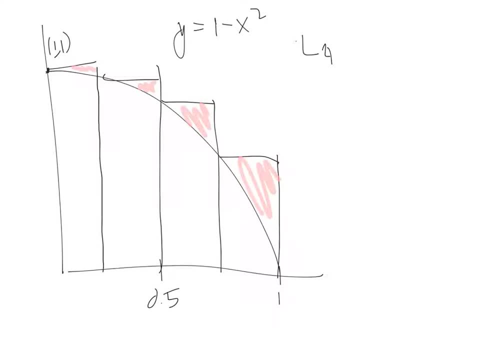 left point, left end point, approximation using four rectangles. so let's calculate what l four is. we're going to approximate, or we want to calculate the area of each of these rectangles. well, the width. so if our total distance was, 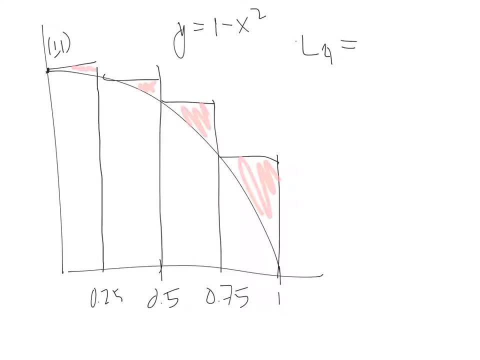 zero to one for the x values and we split it up into four pieces, then we know that each of these right here, each rectangle, has a width of point two, five, point two, five, point two, five and point two five. 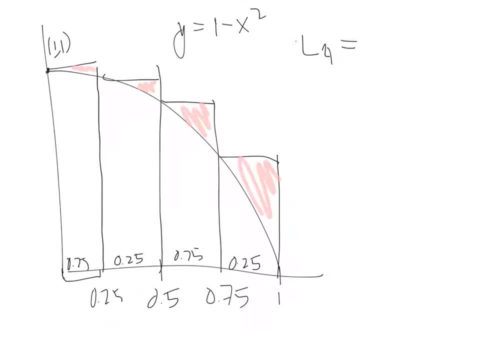 so now we need to figure out what's the height. well, if our function f of x is one minus two x, we're going to figure out, go all the way up and we just plug in your left end point. 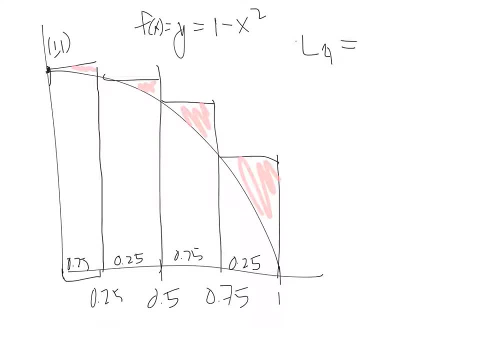 so this one is one one. we knew that this was, or you could have thought of it as one comma f of one. this point right here is going to be point two five, comma f of point two five. 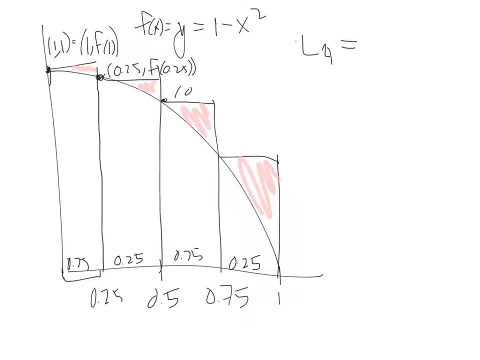 this point right here is going to be zero point five, comma f of zero point five. and then this point is going to be zero point seven five, comma f of zero point seven five, and so the area of a rectangle. 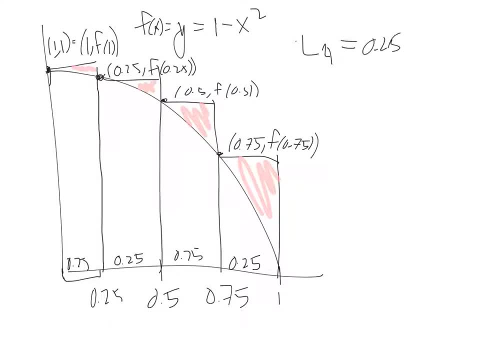 is base times height. so we're going to have point two five times f of zero and excuse me, this is not one one, this is zero one. so f of zero plus another base times height for our second rectangle. 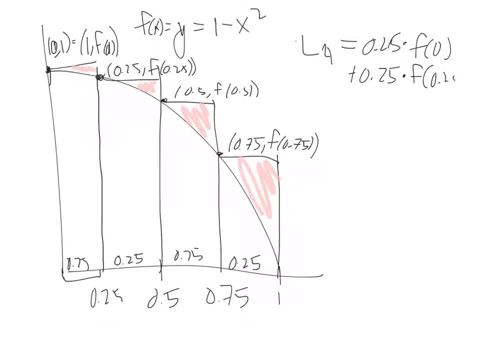 is point two, five times f of point two, five, plus point two, five times f of a half and finally, plus point two, five times f of point seven, five. so I'm going to 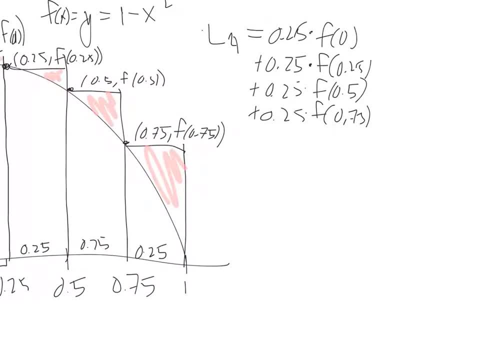 sort of move this over a little bit and what we get is we get point two five times. well, this first value would be one plus- let me going to use fractions- point two, five is one. fourth, 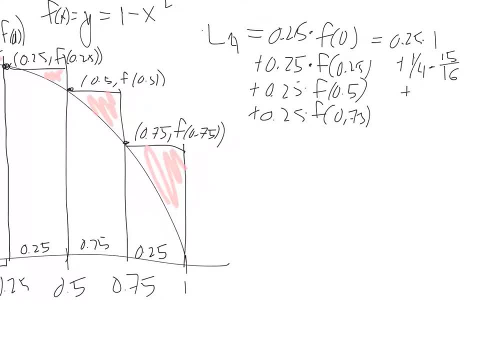 times fifteen over sixteen. that's the times and the minus plus one fourth times three, fourths, and then plus one fourth times seven, sixteenths. I got each of these numbers by evaluating f of those values. 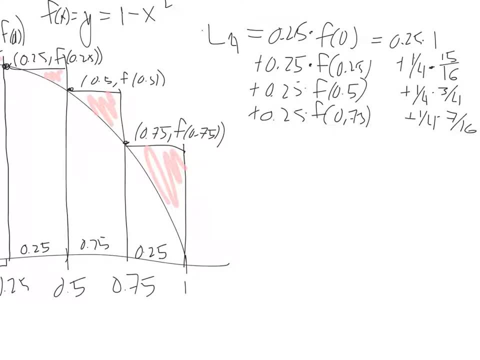 f of point seven five is one minus point seven. five squared and we end up with point or seven sixteenths. so adding this all together, we're going to get that the area is equal to zero. 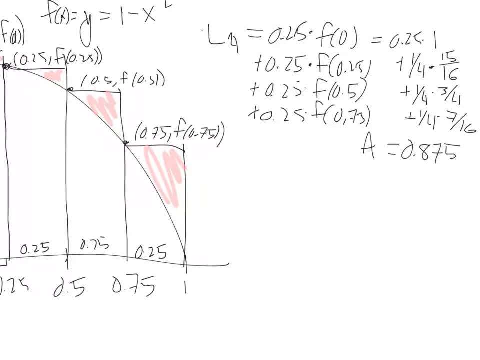 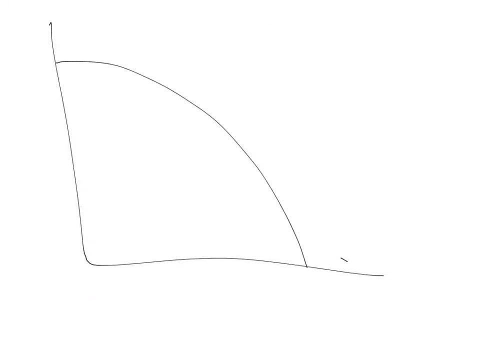 point eight, seven, five, or rather this should be the L four. well, we took the left hand approximation. we can do the same thing. we can do a right hand approximation we have. our f of x is equal to. 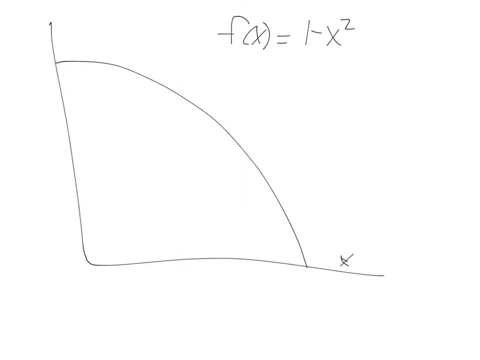 one minus x squared, we have x and y. this is our point one. we got another point one right here, so we can still split it up into four segments, but instead of starting at the left and then going across, 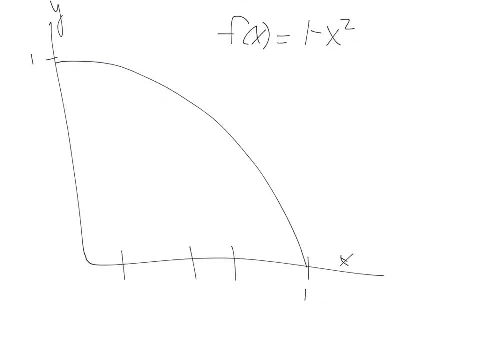 we would start at the right, so each of these intervals, each of these rectangles would go up, and then we'd go across, and here we'd go up and across, up and across. and well, right here, 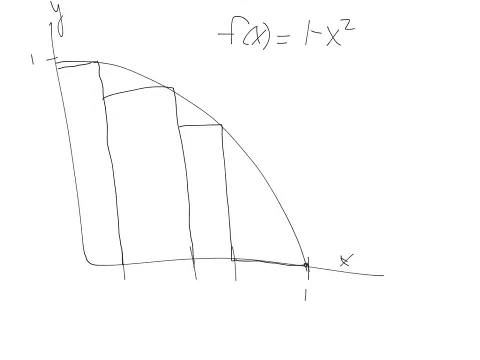 it that's already touching, so we don't need to go up at all and we go across. but you may notice, by doing the right hand approximation we're missing out on some areas right here. in fact, this is a pretty big area. 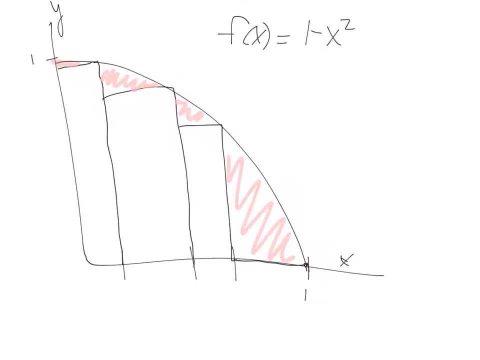 so the left hand approximation we had overestimated, now we're underestimating, but that's alright. I mean, these are our approximations, and so this would be our R4 approximation: four rectangles using the right hand approximation. 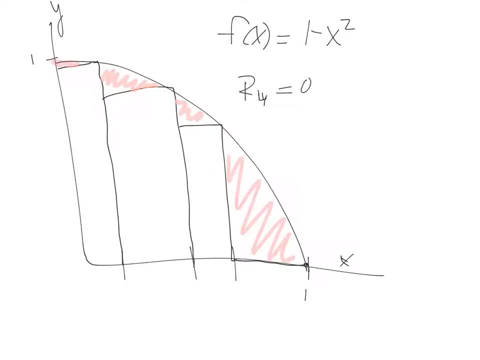 or the right end point, and so each of these is going to be a width of 0.25, just like the last screen, so our first rectangle is going to be: width is 0.25 times the height is going to be. 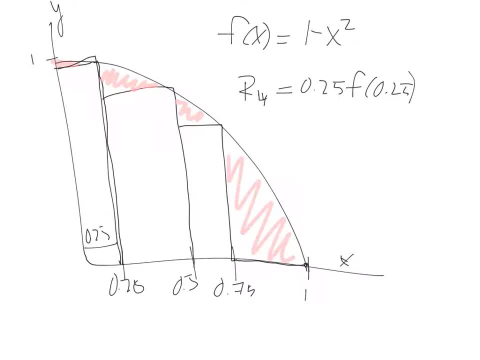 f of 0.25,. since we're using the right part of this end point, then we're going to use this next one plus 0.25, times f of 0.5,. this mid, this second rectangle, the right hand is going to be. 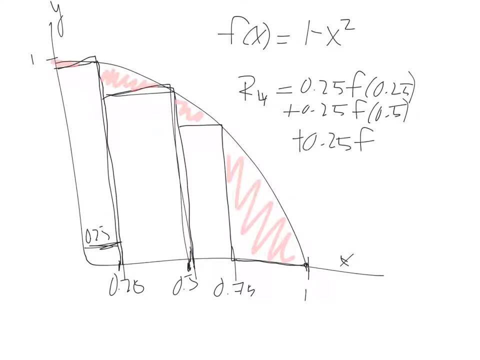 right there, plus 0.25 times f of 0.7, times f of 0.75, and then, finally, this last rectangle is 0.25 times f of 1, but in this case f of 1 is 0,. 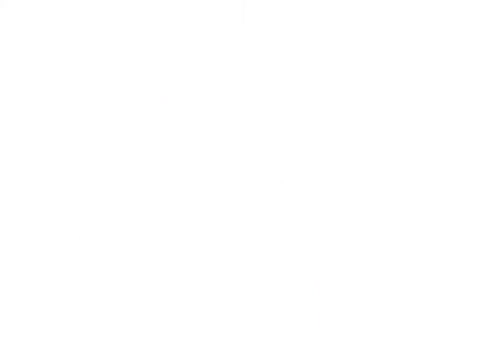 so that would have gone away. now we could do another approximation, and this is: f of x is 1 minus x squared. now, instead of doing a left or right approximation, what we could have done is, at each interval, use the midpoint. 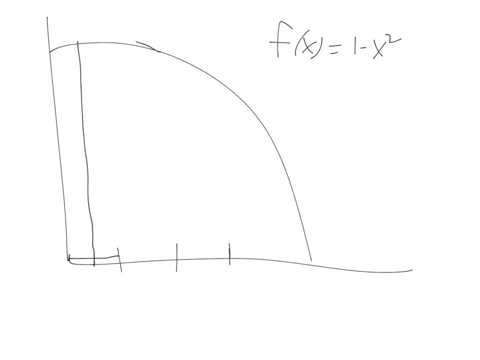 go half way up, and so I guess this graph was that shouldn't be there. it's a little sloppy, but we go about half way up, alright, what we do. that's going to be our interval. we take the midpoint. 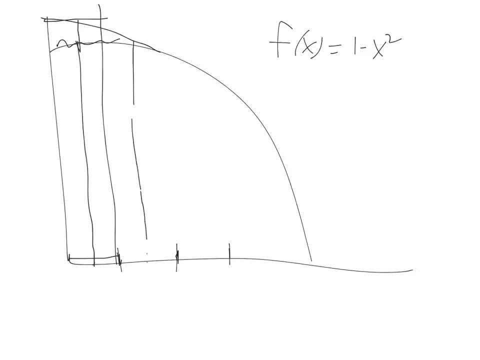 from here to here and then we go up again. take the midpoint, go up and, as you can see, by doing this, we're going to have some areas where we're overestimating, but we also have some areas where 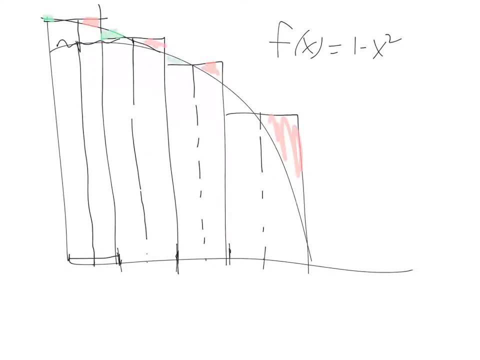 we underestimate, and so this midpoint approximation cancels it out. this would be the midpoint approximation. we'll call it m4, each of these still has a width of 0.25, so they both have, they all have a width of 0.25,. 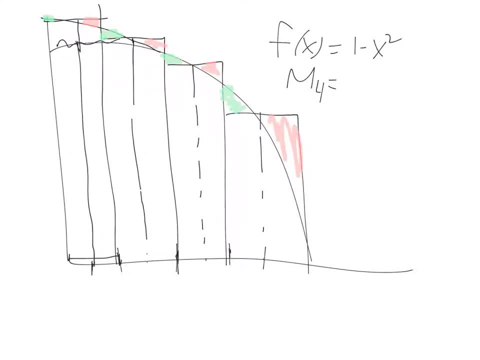 but these midpoints is now going to be the midpoint that's 0.125,, this midpoint right here is going to be 0.375,. this midpoint is 0.625, and then this midpoint is 0.875,. 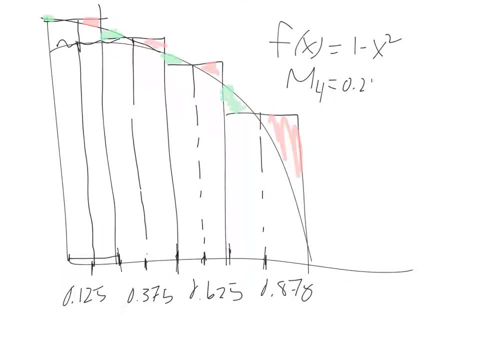 so we would have midpoint approximation. we get for our first rectangle, plus our second rectangle and then our third rectangle. we'd get this and plus 0.25, times f 0.878,. so these would be. 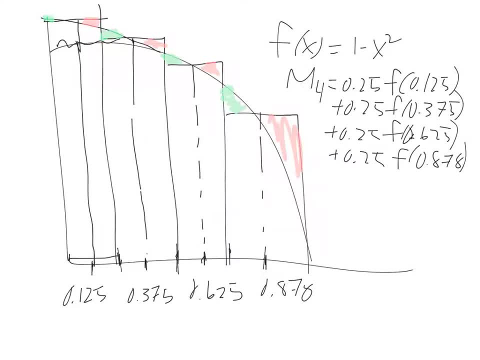 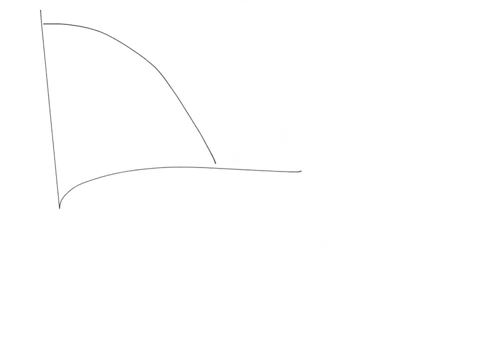 the approximations we get for our midpoint. so if you're trying to approximate the area under this curve, this is: y is equal to one minus x squared. you can use- well, that's a pretty bad axis. 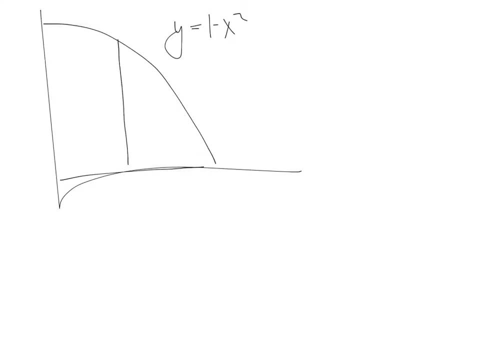 we can use rectangles and let's say we're just going to use the right rectangle. using two, we got a pretty bad area. we're missing a lot. using four rectangles, we're getting a little bit better. 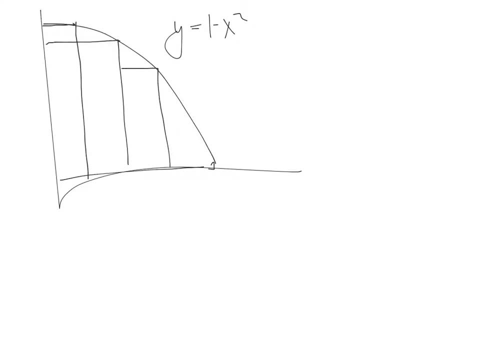 but we still have quite a bit of error. if we use eight, rectangles- getting better. if we use 16, we're getting even better. we're getting closer and closer and closer the more rectangles we get. 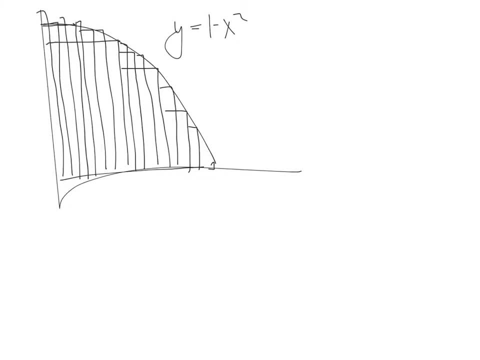 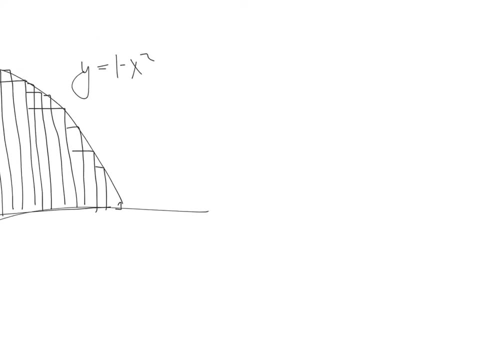 so if we we then use more, we use, say, 32, and so the more and more intervals we use, the better our accuracy. so now let's create a table. so the first column on the table: 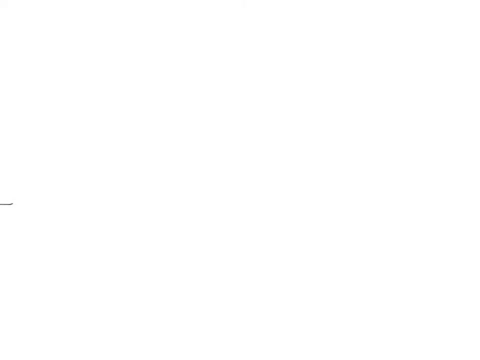 is going to be. I'm just going to clear this all the way out. the first column on the table is going to be the number of sub intervals that we have, the number of sub intervals, and then 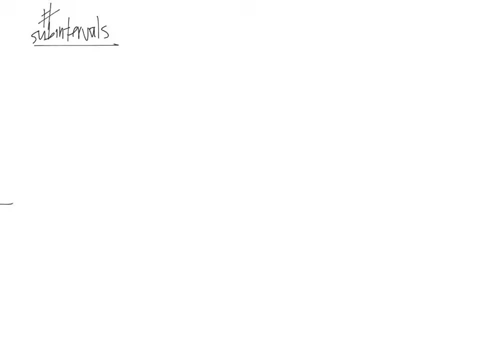 if we use, say, the left hand or the right hand or the midpoint, so so we'll have our right approximation. so the number of sub intervals, we'll say that that's going to be our n. 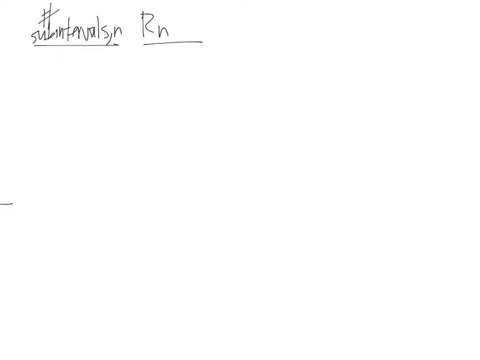 and then we have our right approximation, and then we have our midpoint approximation and we have our left hand approximation- L sub n- and if you remember, I'll sketch it right here: if we're doing the left hand approximation, 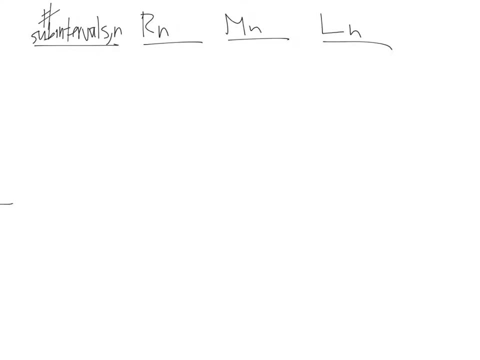 that's going to be over guessing, because we have all this extra right here and then if we do the right hand approximation we're under guessing, so and then the midpoint might balance it out. you have a little bit more. 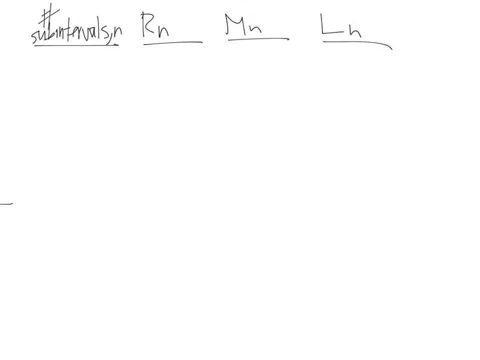 in some spots you'll have a little less in other spots. so, like this interval right here you overestimate it, but then you underestimate it so that might cancel out. so if we have just two sub intervals, the lower sum is going to be. 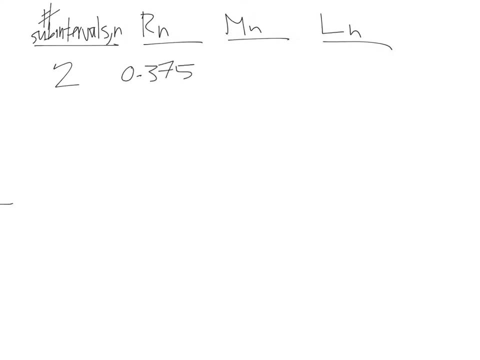 0.375,, or the right hand, the midpoint is going to be 0.6875, and then the left hand sum is 0.875,. if we have four sub intervals, we're going to get 0.53125,. 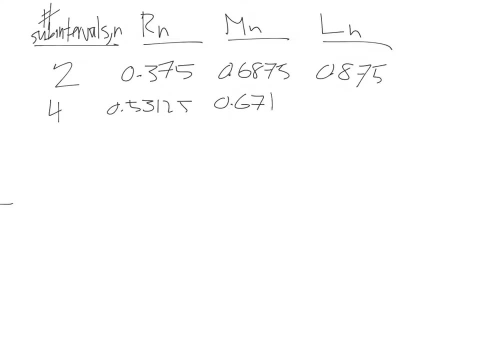 we're going to get 0.671875, and then 0.78125, and so, if you notice, the left hand is going to be a larger number than the right hand, and then the midpoint should fall somewhere in between. 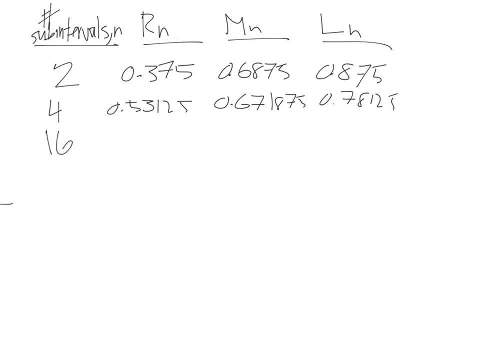 let's go up to 16 intervals, and so the right hand approximation is going to be 0.63476,. we'll stop. we'll do one more six. the midpoint is going to be 0.66699,. 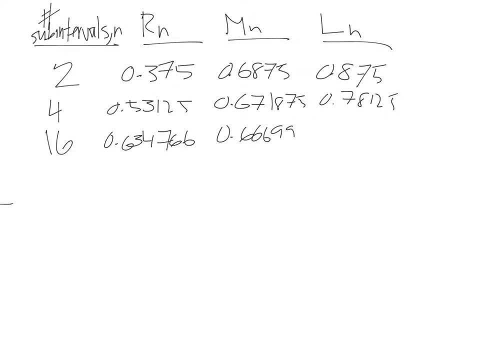 and then the left hand approximation is 0.697,. I'm going to stop it at three, alright, so these numbers are getting closer to each other. if we went up to, let's say, 50, sub intervals, then we'd get. 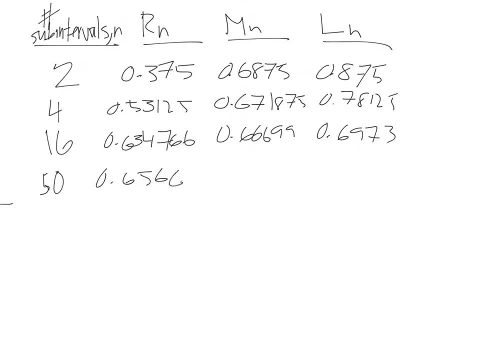 0.6566,, we'd get 0.6667, and then 0.6766,. you might be able to see that these numbers are approaching something, but if not, we'll do a little bit more. 100 intervals. 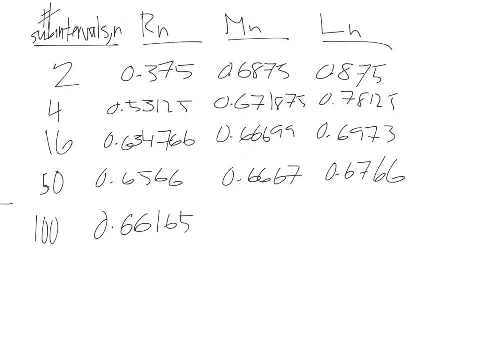 we'll get 0.66165,, 0.666675, and then 0.6716, and if we say went up to 1000, we would get 0.6661665, 0.66666675,. 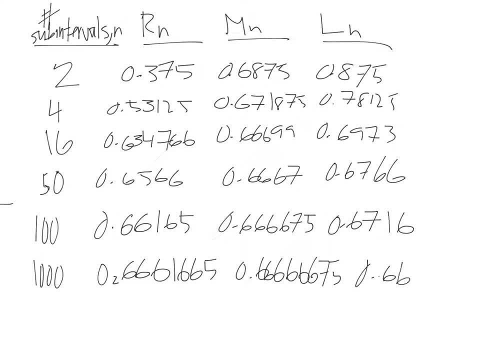 and then 0.6671665,, 0.666665,, alright, and again, each of these would. each of these values would have been computed rather by multiplying the width of each sub interval times the height. 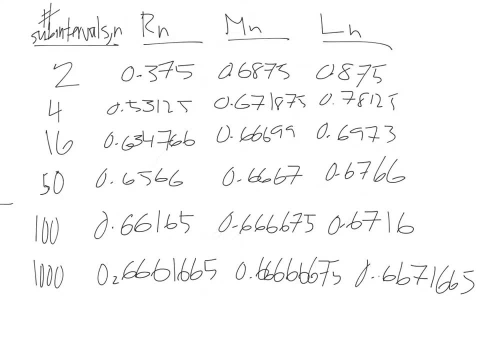 which would have been our function, at either the left midpoint or right hand side of that interval and then taking the sum of all those. so this last one would have been the sum of 1000 rectangles. so we notice. 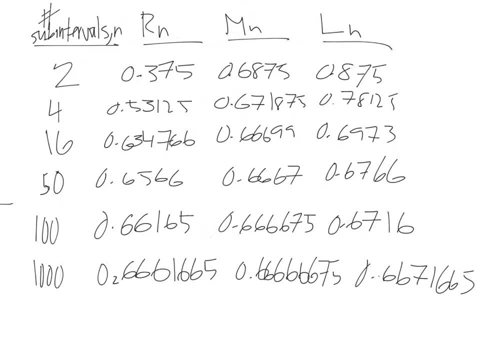 that this is approaching. if we took infinite, one is going to be approaching 2 thirds, and so what we would say is: the area is equal to the limit as n approaches infinity of r sub n. the right hand approximation. 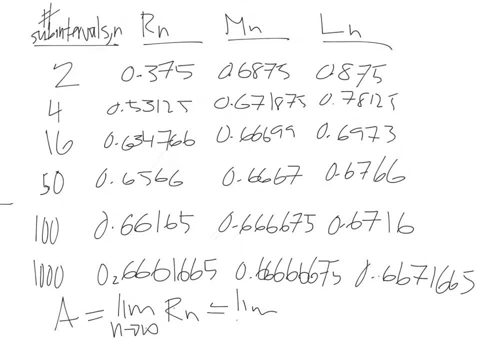 but this is also equal to the limit as n approaches infinity of the midpoint approximation, mn, and the limit as n approaches infinity of ln. so we can get our area by taking the infinite limit, but this would mean we'd have to. 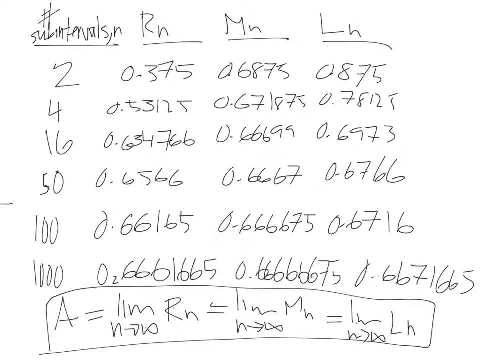 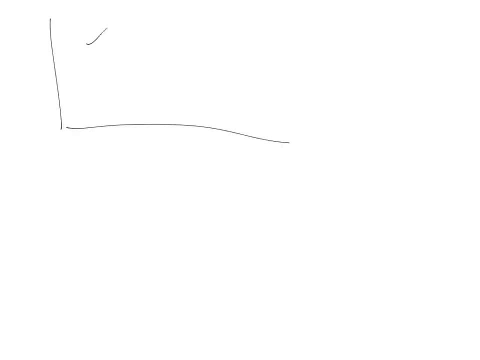 take the infinite sum of infinite rectangles. now let's just study some arbitrary curve like this. so this is: y is equal to f of x, and let's find the area under this curve. so x and y. 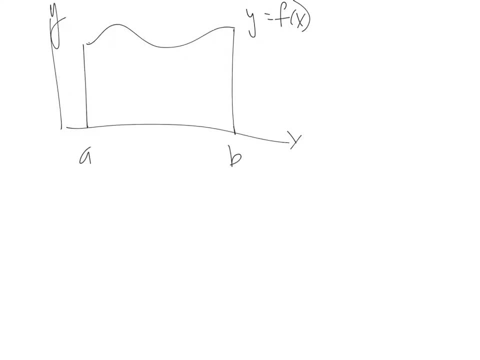 and let's just start from some point a. let's divide this up into n intervals, and so we'd have- we'll call this s one, s two, s three, and we'd have a bunch of ones in between. 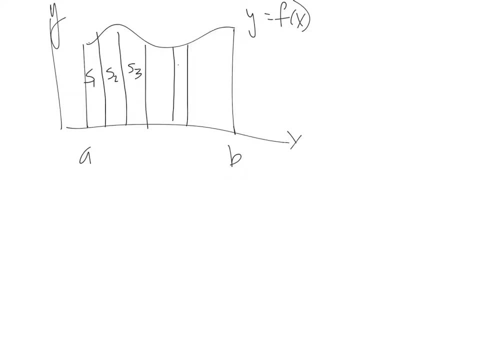 we'll have some arbitrary interval in the middle. call this s sub i, and then a very last interval would be s sub n. so in between we have a bunch of stuff. so we start off. our first point would be a. 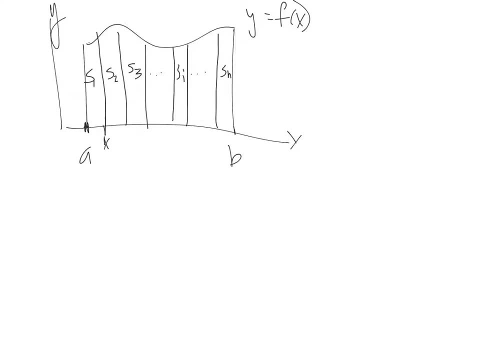 and then we're gonna start labeling each of these values. we'll call that x one, then we'll call this one x two, call this x three, so at the end of each section. so s i, the end of s i would be. 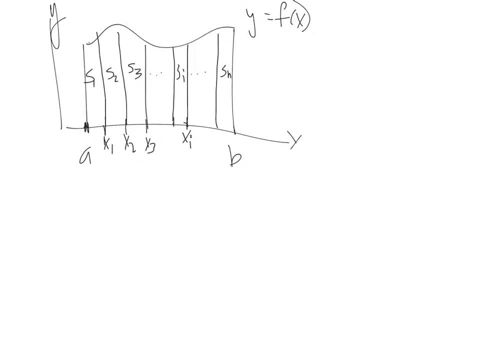 x, sub i. what about at the beginning of s? i? well, that's just the one before it, so that'd be x of x or x i minus one, and then, finally, the beginning of our s n would be x. 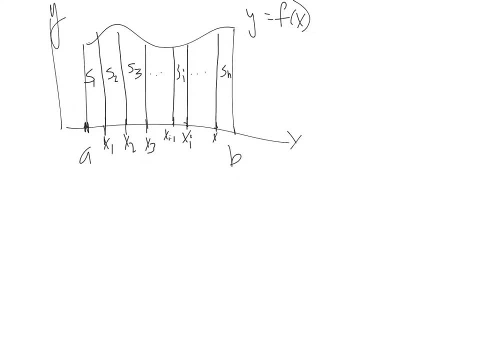 sub. well, if this is the nth one, the start of it would be x of n minus one, and I'm just gonna put a couple of dots in between here, so we know that there is maybe some arbitrary space. 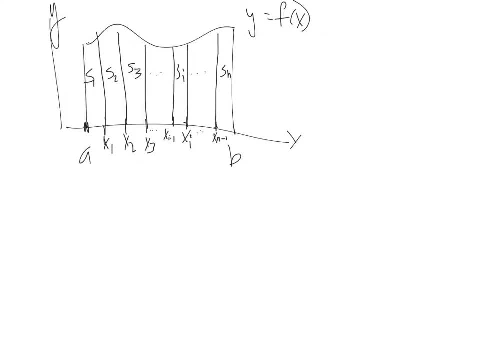 well, what's the interval, what's the gap or the width of each of these rectangles? we'll call it delta x. well, delta x is gonna be. well, how far is the whole thing? the distance is gonna be, or the length is b minus a. 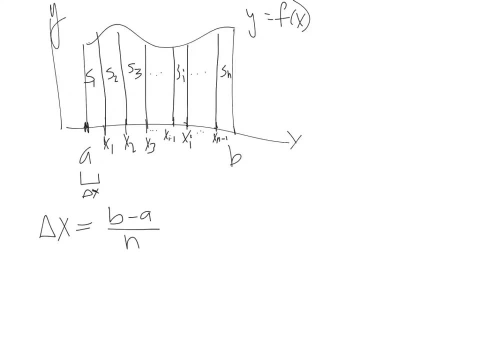 and if we're breaking it up into n intervals, then that length b minus a, divided by n, is how long each of these intervals would be. so now, how do you figure out what's the value of x one? well, x one. 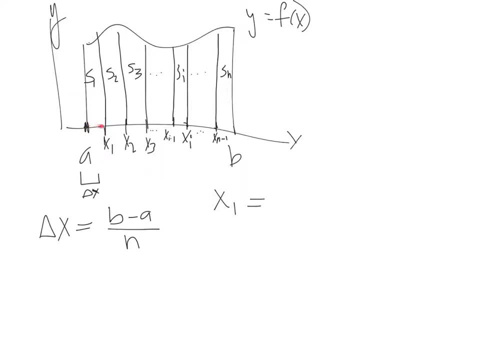 if we started off at a and this interval has a length of delta x. x one is a plus delta x, but what about x two? well, x two. we started off at a, we added a delta x and then we added another delta x. 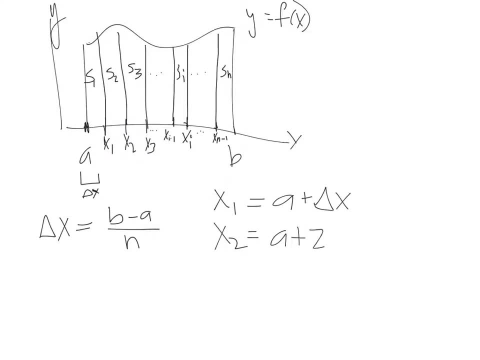 so x two is gonna be a plus two times delta x, x three would be a plus three times delta x, and so forth. and so now what we can do is we can figure out the approximation, the right hand approximation. 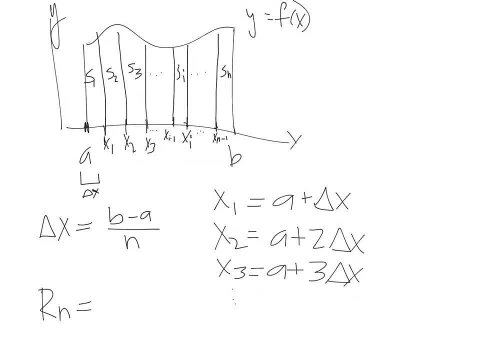 r sub n for this would be. the of each rectangle is length times height, or length times width, delta x times our height, and so the height would be f of whatever x one you know. 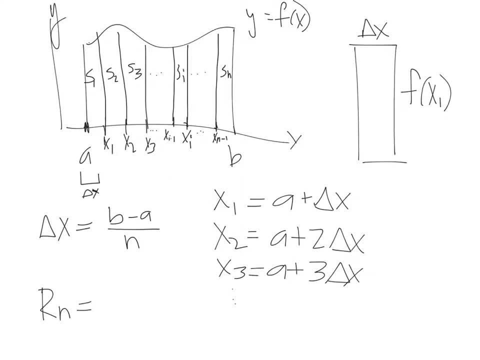 x one or x two and so forth, and we have our x one, x two right here. so r sub n would be f of x one times delta x. and remember we're using the right hand approximation. 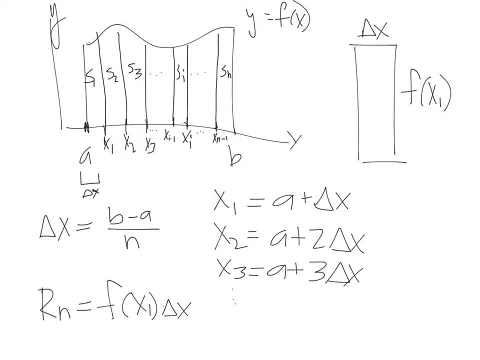 so for our first rectangle we're using the right hand. the second approximation we're gonna use that right hand. so, plus f of x, two times delta x, plus f of x, three times delta x, plus so forth. 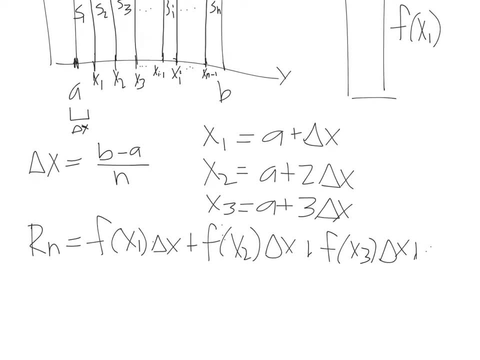 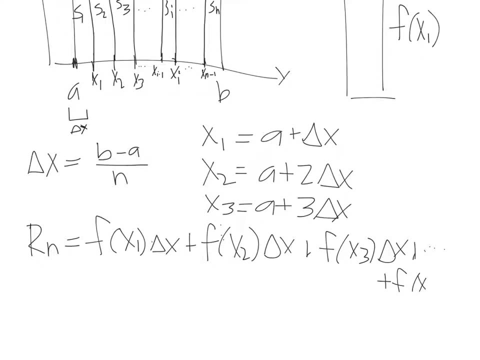 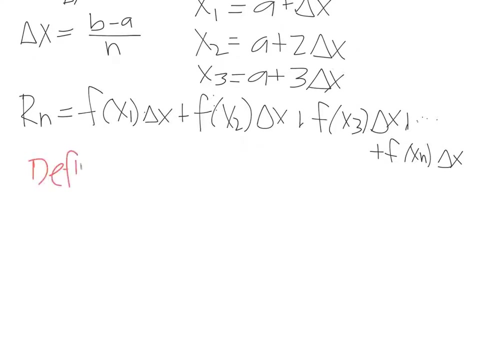 and I sort of ran out of space and let me go up one more line: plus dot, dot, dot, plus f of x, n times delta x. so this leads us to our first definition and the definition says the area. 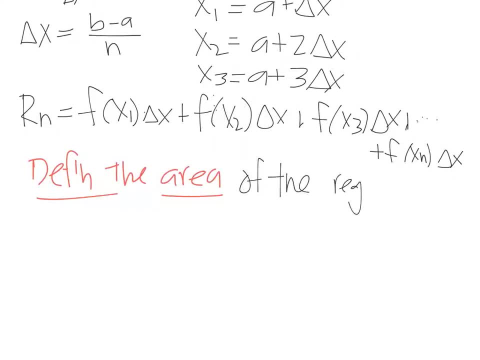 of the region, and we'll call that region s, and this is the region that lies under the curve or under the graph of the continuous function. f is the limit of the sum of areas. 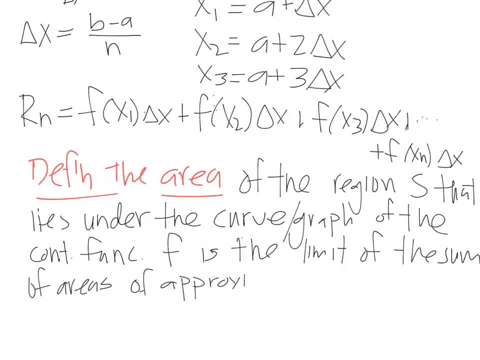 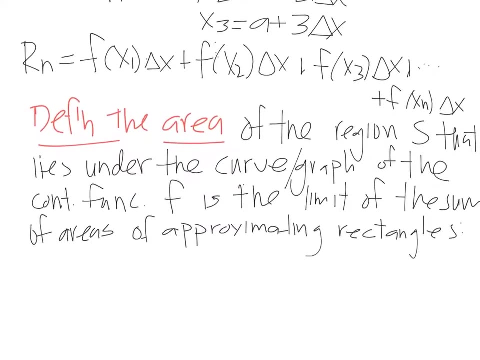 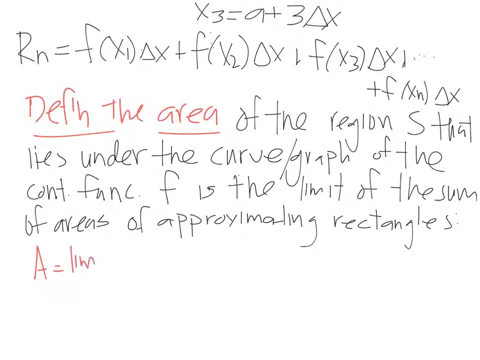 of approximating rectangles. and here we go. here's the formula it's gonna be: area is equal to the limit as n approaches infinity of r sub n, and so if r sub n is what's written above, 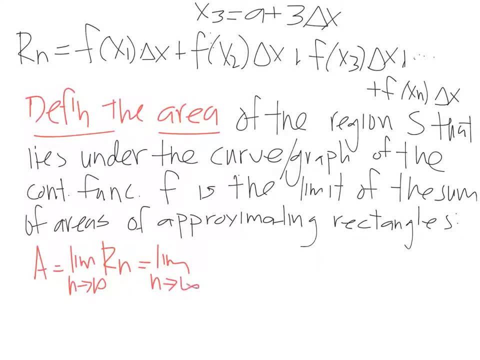 then this is really the limit, as n approaches infinity, of the following: f of x sub one times delta x plus. f of x sub two times delta x plus, so forth, all the way to our last term. 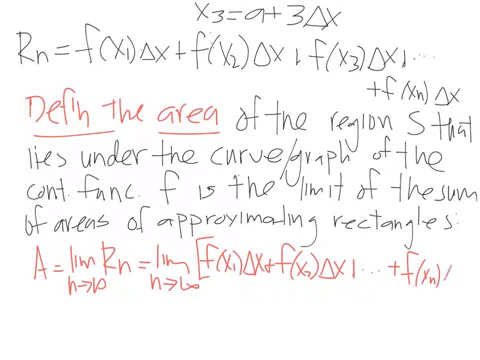 f of x sub n times delta x, and that's how we find the area of the curve. now, another way to write this, this infinite sum, is using something that we call sigma notation. sigma notation is gonna be as follows: 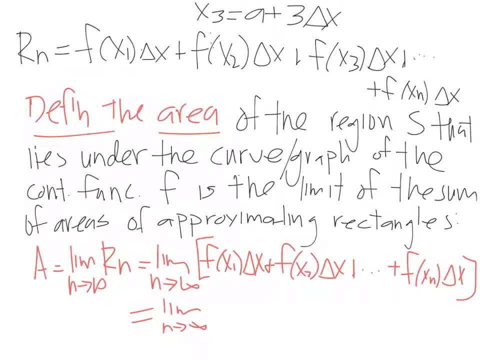 if we're taking the sum, and we're taking the sum of f of x one plus f of x two plus f of x three, and so forth. instead of writing it all out, what we can do is write: 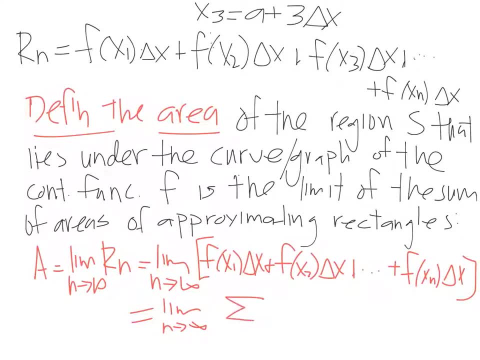 sigma, like this sigma, and we'll say some index number, some. i goes from one to n and we'd say f of x sub i times delta x, and what this means is that i is gonna go from one. 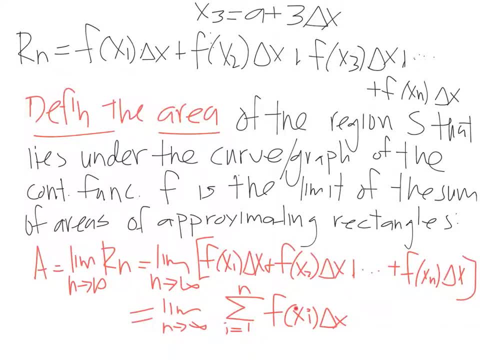 all the way up to n, and so when i is one, this is f of x one times delta x plus. and then you move up in number. this now becomes i, becomes two, and so this is f of x two. 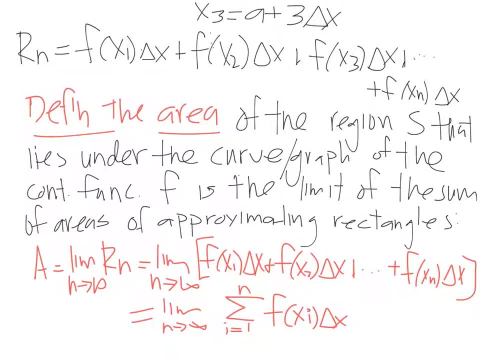 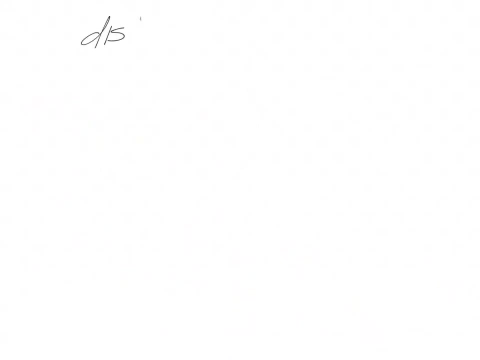 times delta x plus f of x, three times delta x, all the way up to n. now let's take a look at something called the distance problem. we know that distance is equal to velocity times time. 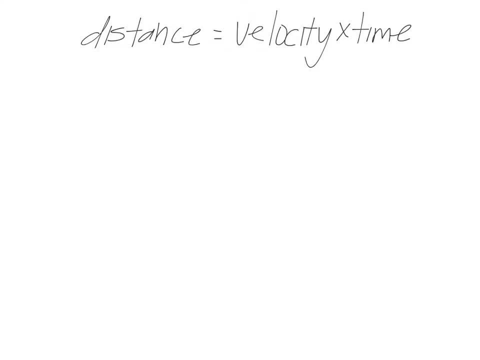 because velocity is distance over time. so if you multiply both sides by time, distance is velocity multiplied by time. so let's say we're driving in a car and we don't know the odometer reading, but we do know. 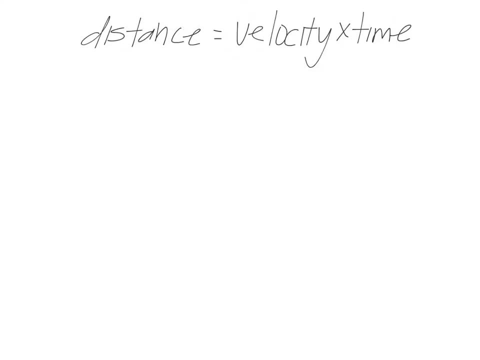 how fast we're going. we do know our velocity, and so if, if we knew our velocity at certain time, we could figure out how far we've traveled. so let's say, we have time and the unit for time. 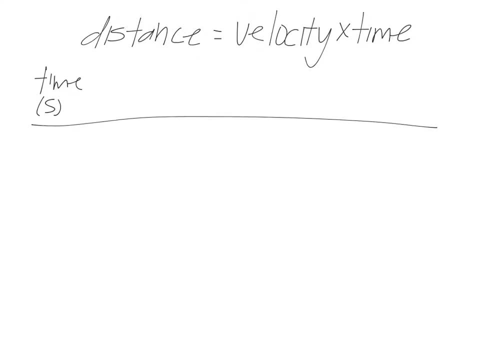 is gonna be in seconds and then we're gonna have our velocity and the unit for velocity is gonna be feet per second. so we start off when, when we start our taking a look, look at our recordings. 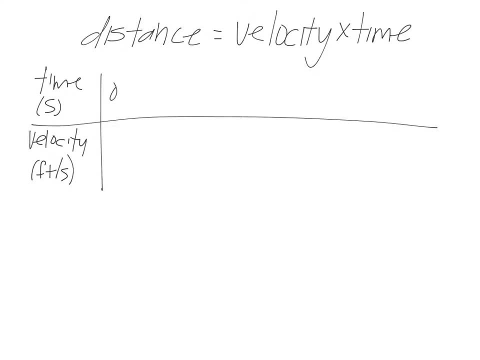 at time is zero. so we're moving. we start the timer times zero, we're going 25 feet per second and then, after five more seconds, we take a look and we're traveling 31 feet per second. 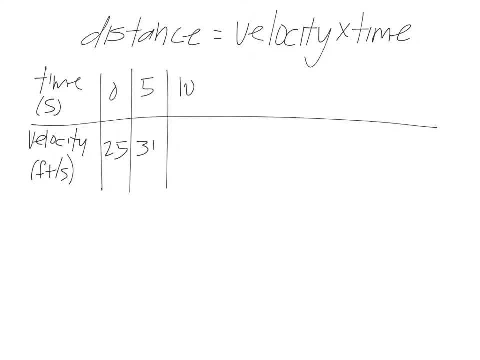 and then after 10 seconds, we're traveling at a speed of 35 feet per second- 15 minutes. then we're gonna travel 43 feet per second- 20 seconds. we'll travel 47, 25 seconds. 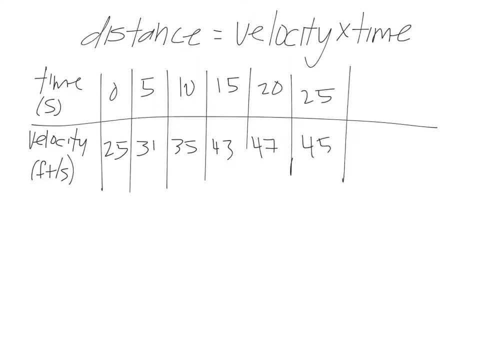 it'll be 45, and then at 30 seconds, we're traveling at 41 feet per second. how far have we traveled? well, if we were to plot this, it would look something like we have. 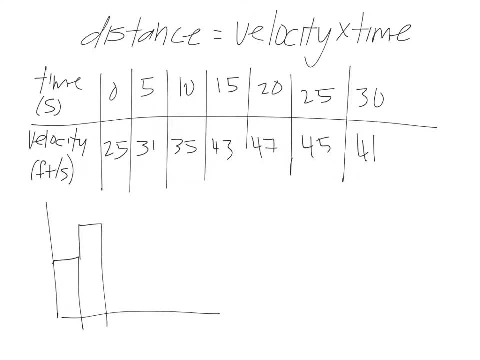 a bunch of rectangles and it starts to look like what we had before when we're finding the areas. so it goes up. for the first five intervals we're counting 25,, 31,, 35,, 43,. 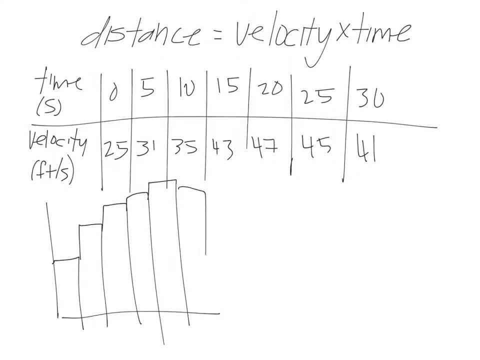 47, and then it starts to go back down a little bit: 45, and then 41,. this is not my. this graph is not entirely accurate, but close enough so to figure out. 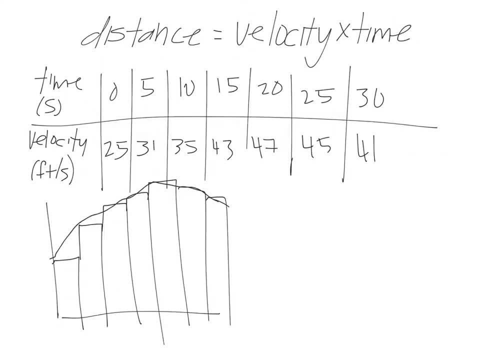 how far we've traveled. distance is velocity, times, time, and so if we're using, say, the left hand approximation, which is kind of what I drew right here, the distance traveled is going to be so for the distance, 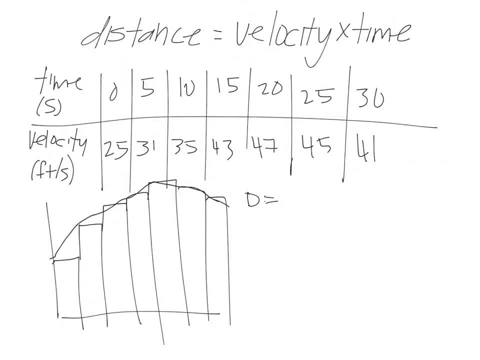 that's going to be. we're using the left hand approximation, so that's our delta x is five times our height, which in this case we didn't need to figure it out because it's already given, as opposed to: 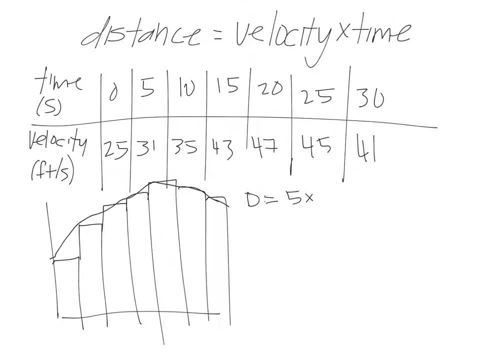 figuring out what f of x sub one is, or so forth. so five times 25, plus five times 31, plus five times 35, plus five times 43,, plus five times 47, plus five. 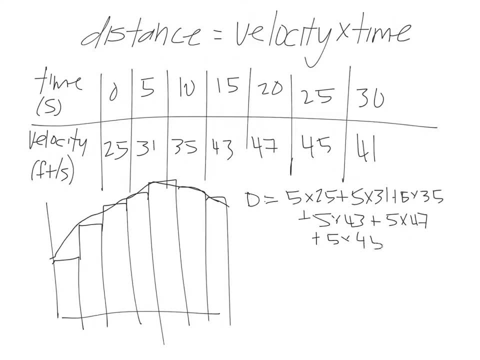 times 45, and so, calculating all this, we get 1000, 130 feet now if we were to instead use the right hand approximation. so in this case, the left hand approximation leaves us, we're. 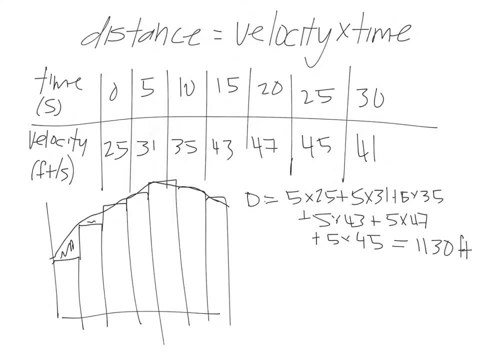 doing. we're underestimating. if we did the right hand approximation, we would overestimate. so let's just do that, the right hand approximation. so it'll be five times our first rectangle using the right hand approximation. we're going to start off. 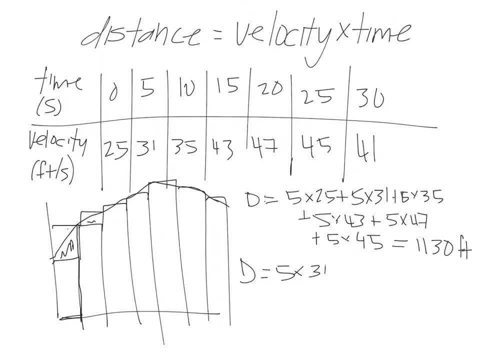 with the second value, so five times 31,, plus five times 35,, plus five times 43,, plus five times 47,, plus five times 45, and then the last point, plus five times 41,. 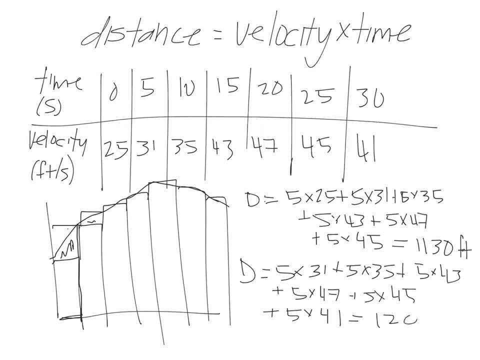 and what we get here is we get 1210, feet. so we knew that we were a little bit over, but this is sort of an approximation. we don't. we don't know exactly how far we went. 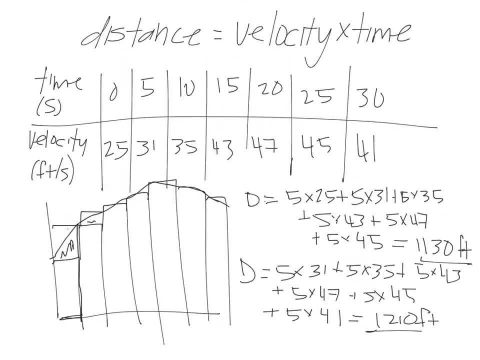 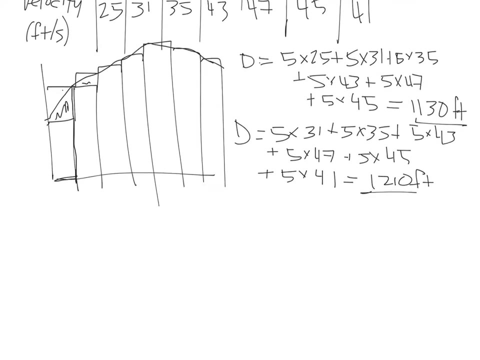 in general. you know, we in between, we could have sped up at the very end or sped up early, but we don't know. but this leads us to the equation for distance, and that is distance. 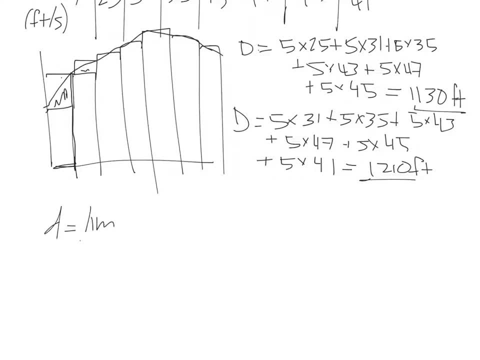 is equal to the limit, as n goes to infinity of- and we're going to use sigma notation- the sum where i goes from one to n, of f, of t, and this is sub i minus one. so 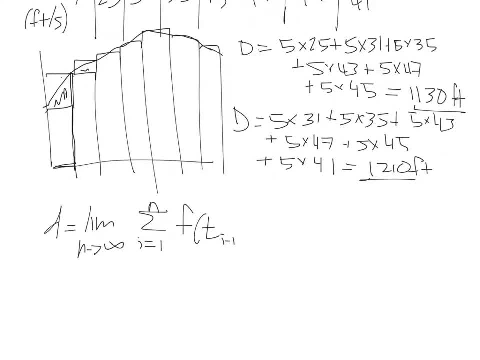 we're doing the left hand approximation times, delta t, or if we did the right hand approximation, this would have been the limit, as n goes to infinity, of the sum where i goes from one to n of f. 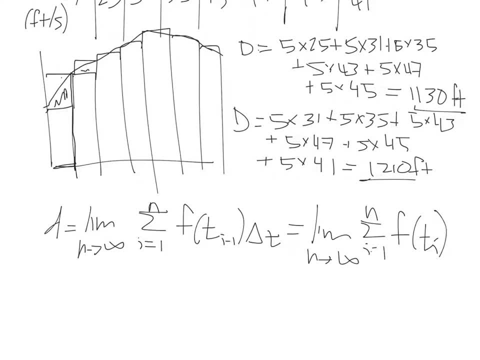 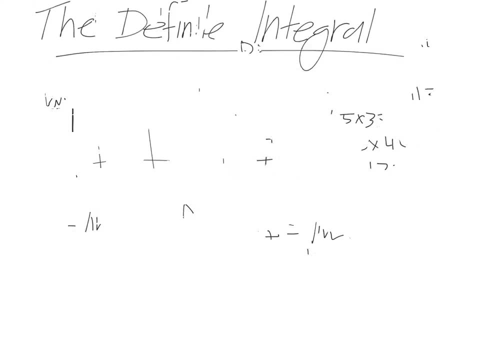 of t sub i times delta t plus what one. so let's go back and look at it now. your friends, today we're gonna talk about the definite integral, so we'll begin defining what is the definite integral. 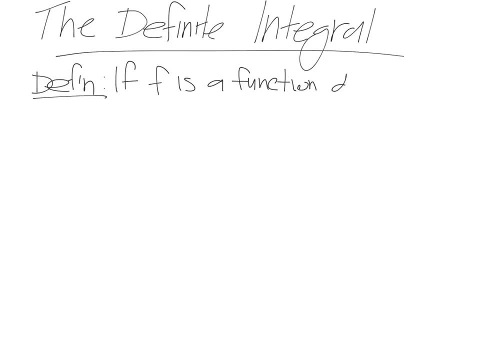 if f is a function defined for x being between and including on the endpoints, then we divide the interval a to b into n subintervals And each of these subintervals are going to be of equal width, And we'll say that equal width is going to be called delta x. 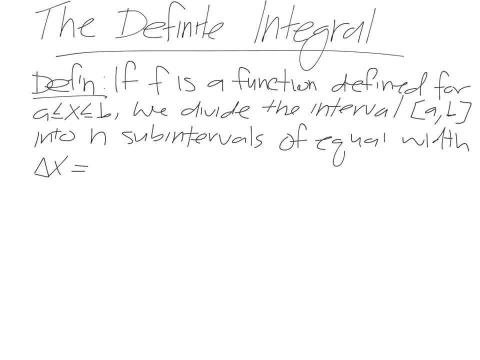 And, if you remember from before, delta x is going to be b minus a divided by n. Now, if we let x zero be our first point a, and then we have x one, x two, so forth all the way to the last point, x sub n. 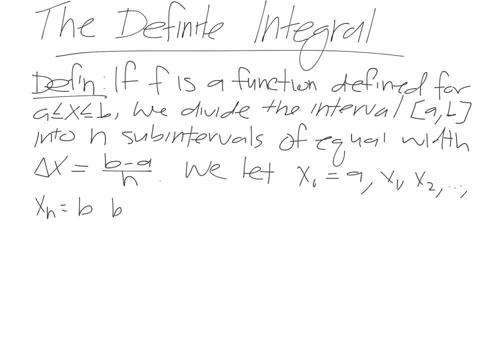 and that's going to be equal to our b, And so b the endpoints. so each of these are the endpoints of the subintervals. Now, if we divide the interval a by b, So each of these are the endpoints of the subintervals. 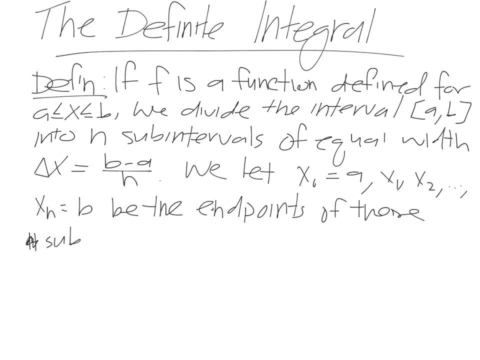 Not intervals but rather subintervals, And we let these points x one star, x two star, and so forth, all the way to x n star, And we're going to say these are going to be any samples And we're going to say these are going to be any sample points. 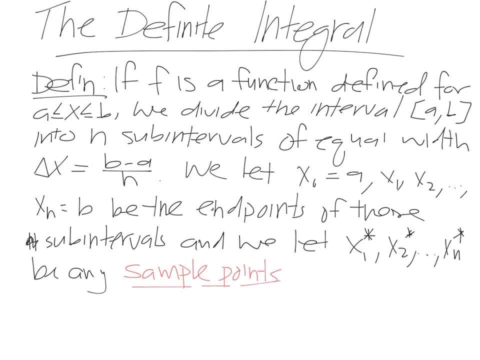 And so sample points really are just the points that can be the left endpoint or the right endpoint, And so we might want to pick sample points. that would make sure that we're getting a pretty good approximation. Half of that is going to be above and half of it's going to be below. 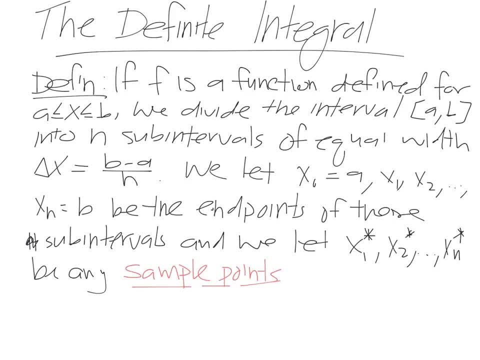 and half of it's going to be below. If you notice, sometimes before, if we just did the left approximation we might overestimate everything or underestimate. So sample points are something that allows flexibility. So if these are sample points in the subintervals, 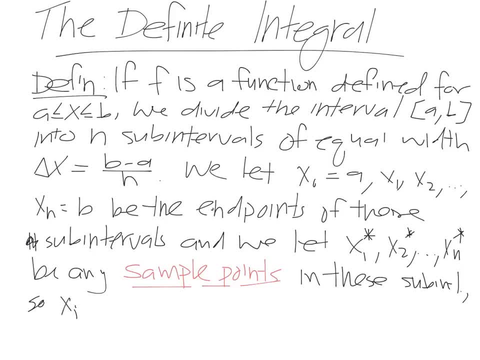 so that x sub i star. so for some arbitrary i, this lies. so for some arbitrary i, this lies in the i'th subinterval from x sub i minus one to x sub i. So we're not done just yet. 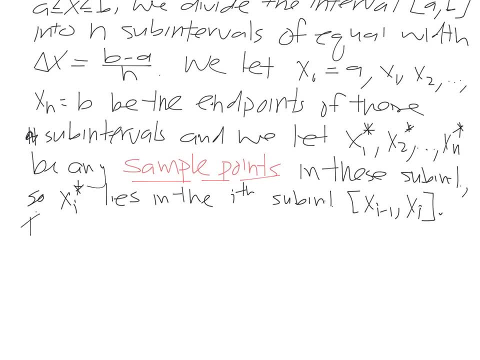 And then we say then, And then we say, then, we say that the definite integral, we say that the definite integral, The definite integral of f from a, The definite integral of f from a, from a, from a to b, this definite integral is going to be defined to be the following: 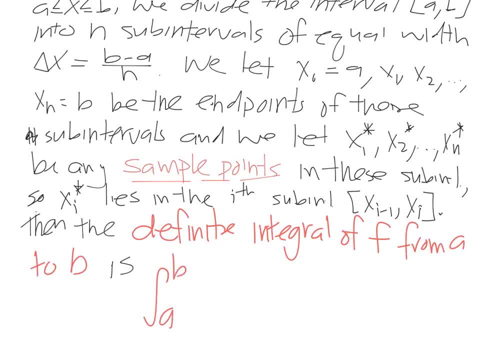 So this is not an s, this is an integral sign, the integral from a to b of f, of x times dx, and this is the limit, as n goes to infinity, of the sum where i goes from 1 to n of f. 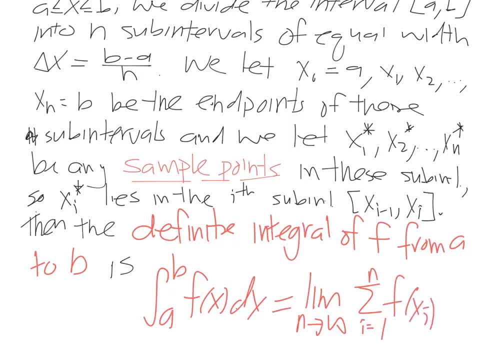 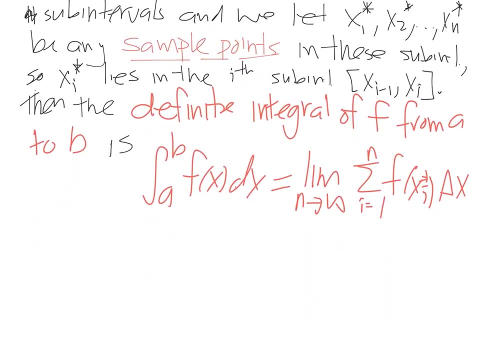 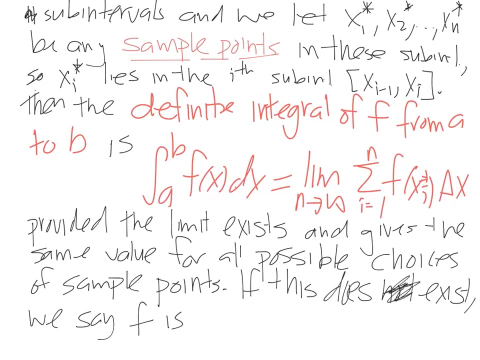 of x, sub i, star times, delta x. So we have all this, And this is provided the limit exists and gives the same value for all possible choices of sample points. If this does not exist, then we say that f is going to be and the definition here is integrable. 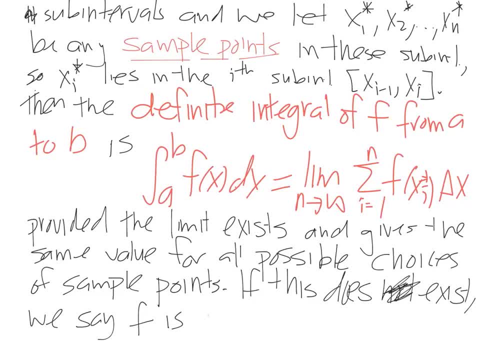 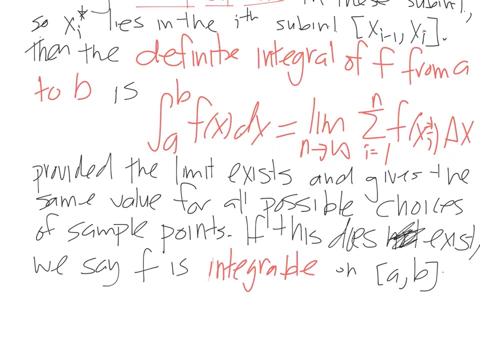 And then we say that f is going to be and the definition here is integrable, And it will be integrable on the interval a to b. This definition is something that we call a Riemann sum, And Riemann sum is spelt R-I-E-M-A-N-N. 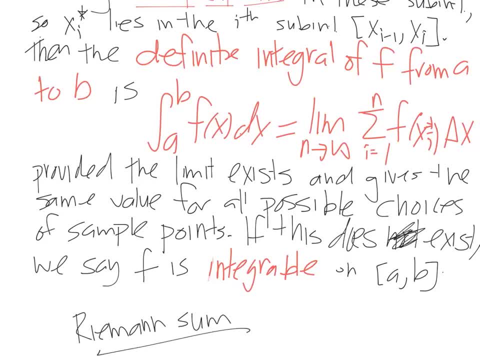 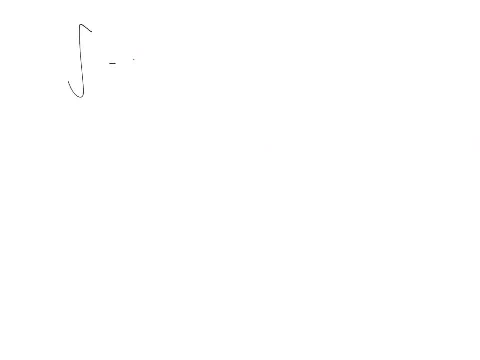 This is Riemann sum. So just to note this right here, this is the integral sign. And then if we have, For dealing with something like this, if we have something like this, if we have something like this, the integral from a to b of f, of x, dx, we're going to say that f of x is the 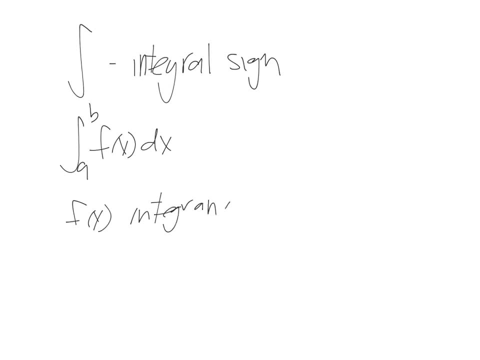 integrand a and b are the limits of integration. a is the limit, b is the lower limit, b is the upper limit, And then we're always going to have this dx. It just simply indicates that the independent variable that we're dealing with is x. 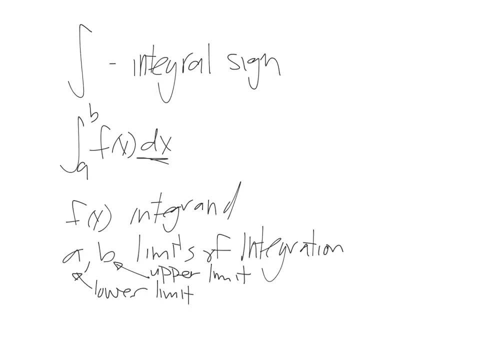 And so the whole procedure is to break down this line, And so the whole procedure is to break down this line, And so the whole procedure is to break down this line procedure of calculating an integral. this is what we call integration. and again this DX just tells us that that's the variable we're dealing with. we could 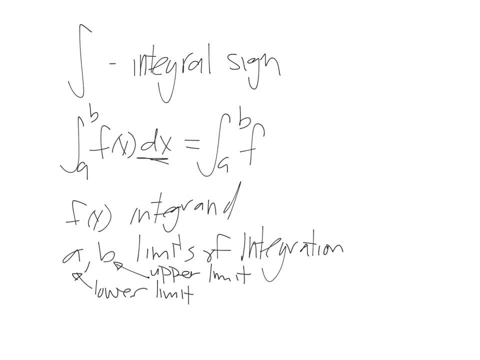 have been dealing with another variable, say like the integral from A to B of F, of T. and if T is our variable then we would say DT, or if it's R, it would be DR. so we have a couple of theorems. the first theorem state says: if F is, 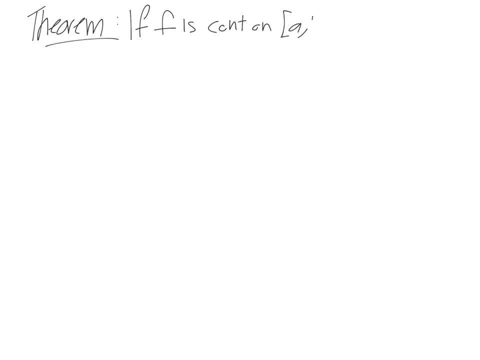 continuous on the interval A to B, or if F has only a finite number of а jump discontinuities, then the function f is integrable on a to b. What this means is so that is the definite integral, the integral from a to b of f, of. 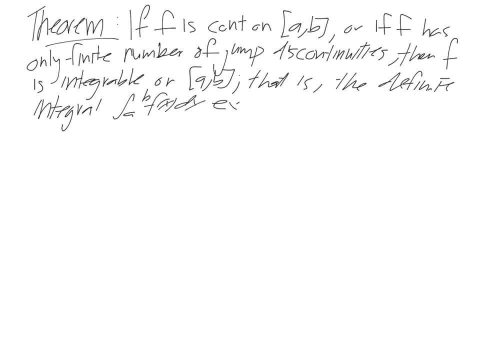 x, dx exists, Okay, Okay. So the next theorem states: if f is integrable, alright, and now we know how to find if it's integrable from the previous theorem. if it's integrable on the interval a to b, then we: 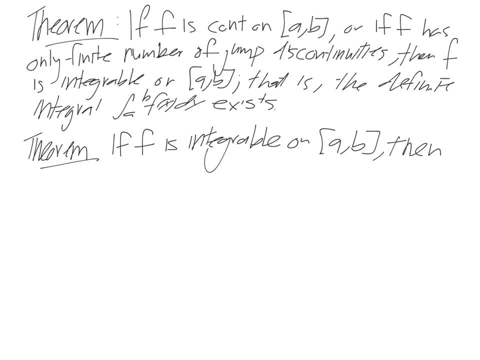 have- I'm going to change my pen for this. We have the integral from a to b, of f, of x, dx, which is equal to the sum or n or, excuse me, the limit. not the sum, but the limit. so it's equal to the limit where n. 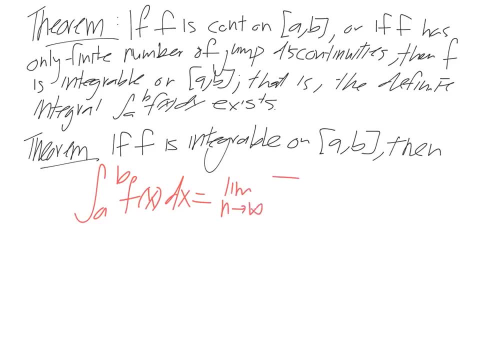 goes to infinity Of the sum, where i goes from 1 to n, of f, of x sub i times delta x, and this is where we have that delta x is b minus a over n and our x sub i is really our starting point. 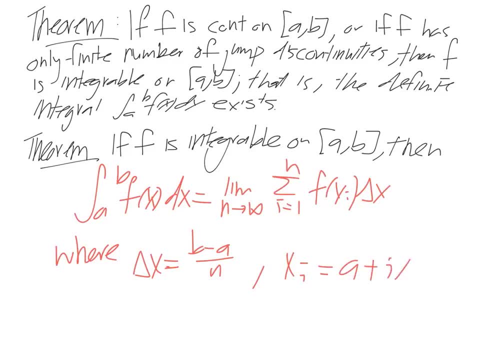 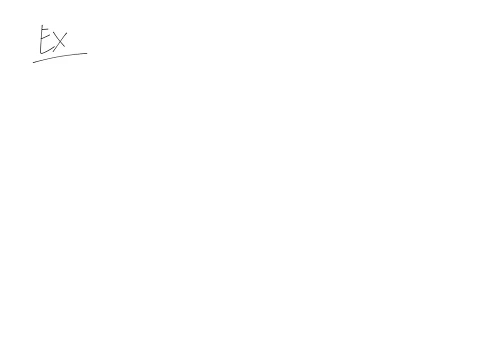 a plus i times delta x. Okay, Okay, Okay. So we have this del f of x, depending on which rectangle or which sub interval we're dealing with. Alright, let's do an example. If I'm given the limit as x- excuse me, not as x, but as n- goes to infinity of the sum. 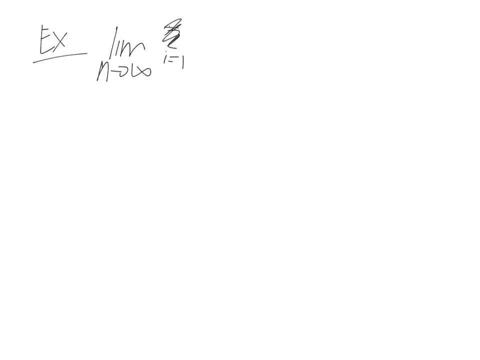 where I goes from 1 to n and the sum that is equal to n, because this is the denominator. This is a terrible sum. Let me rewrite that: The sum where i goes from 1 to n of the quantity x sub i cubed plus x sub i times sine, of x sub i times delta x. 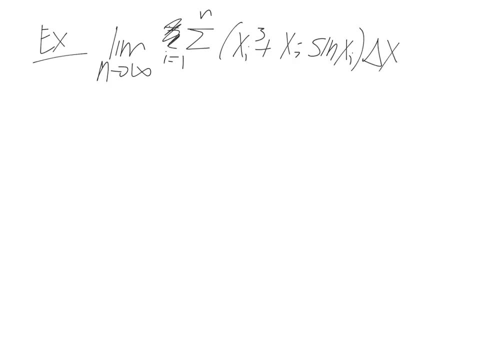 Write this as an integral on the interval 0 to pi. Well, if we wrote this as the integral, this would be the integral from 0 to pi of the inside stays the same, so it's still going to be the same function. 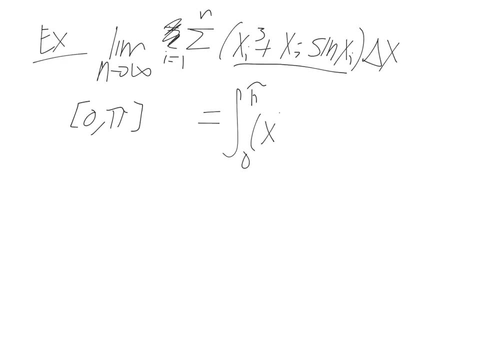 Except x. sub i is just going to be replaced with x. So x cubed is the integral from 0 to pi. So x cubed is the integral from 0 to pi. So x cubed plus x times sine of x. And then, when we finish this, we want to make sure we're integrating with respect to our variable x. 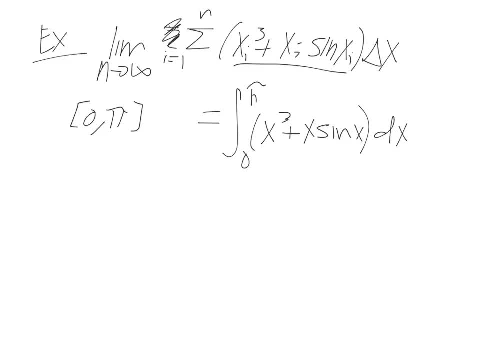 So we put times dx. Now I'm going to go over some formulas and rules to help evaluate integrals. Now I'm going to go over some formulas and rules to help evaluate integrals. The first one is the sum where i goes from 1 to n of just i, meaning we're taking 1 plus 2 plus 3 plus 4, so forth, all the way to n. 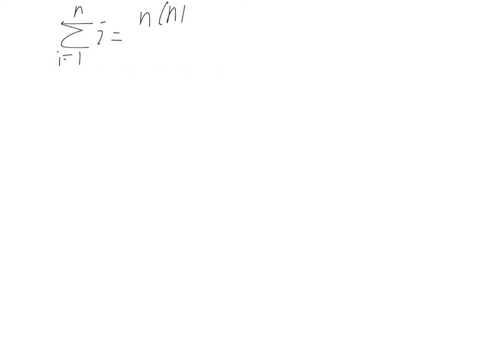 This actually can be written as n times n plus 1 over 2.. The next thing is the sum where i goes from 1 to n Of i squared. So again, this is 1 squared plus 2 squared plus 3 squared, all the way to n squared. 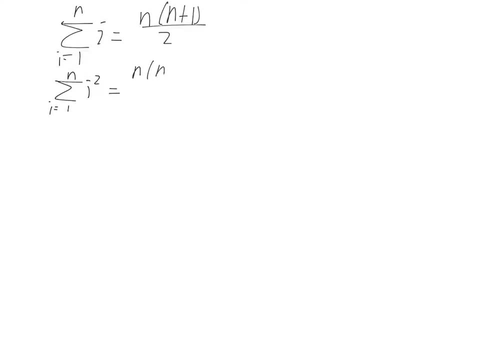 This is n times n plus 1 times 2n plus 1.. This is all over 6.. The next formula we have is the sum where i goes from 1 to n, Of i cubed, And this is the quantity n times n plus 1, all over 2.. 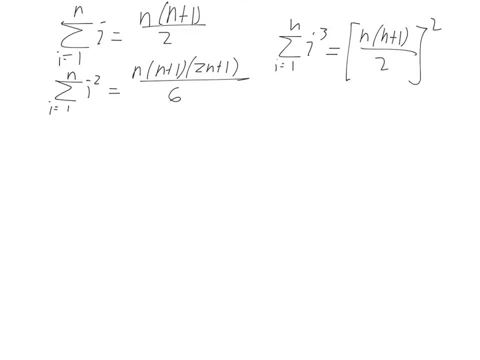 This whole quantity squared. Now here are some rules that would help us when working with sigma notation. And that is the sum where i goes from 1 to n of c. Well, c doesn't relate to i, So it's basically: we're adding c n times. 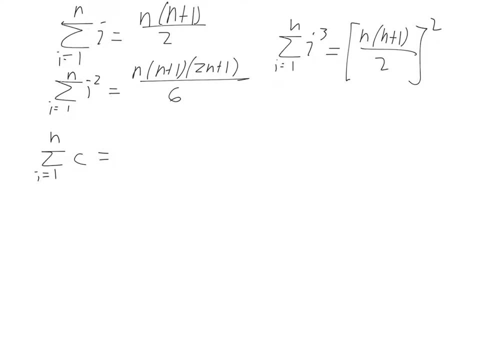 We're adding c plus c plus c, Whereas before so, like in this case, this number changed. It went from whatever i was changing to, But there's no i, So it's just c plus c plus c n times. So in other words, this is just n times c. 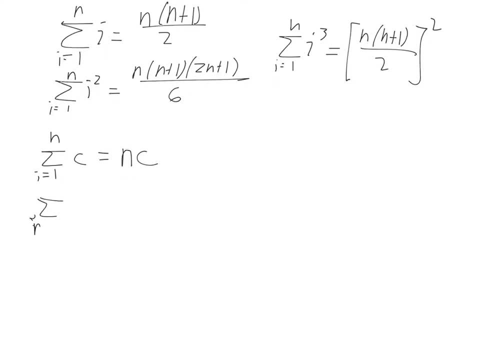 If we have the sum where i goes from 1 to n of c times some a sub i, Well, that c is a constant, So we can just say it's c times that whole sum. Let me rewrite my sigma notation: Times the sum where i goes from 1 to n of a sub i. 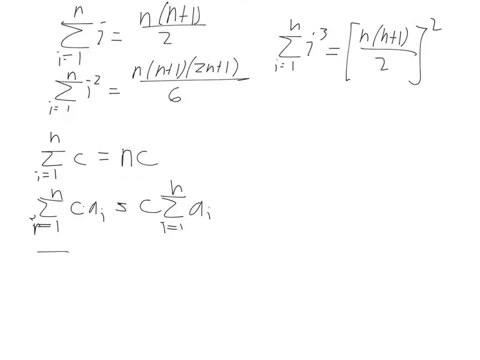 Now we can do another one, So the sum where i goes from 1 to n of the quantity a sub i plus b sub i. We can split this up into two different sums: The sum where i goes from 1 to n of a sub i, plus the sum where i goes from 1 to n of b sub i. 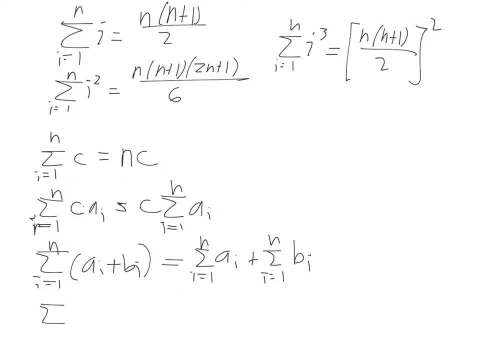 And similarly, if we're subtracting The sum where i goes from 1 to n of a sub i minus b sub i Is going to be the sum where i goes from 1 to n of a sub i minus the sum where i goes from 1 to n of b sub i. 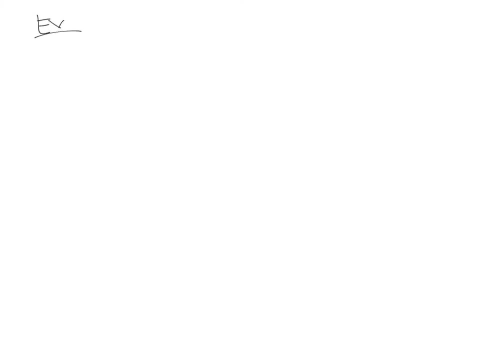 Now let's do an example: Evaluate the Riemann sum for f of x equals x cubed minus 6x, And we'll use our endpoints a to be 0,, b to be 3.. And then we're going to pick: n is going to be 6.. 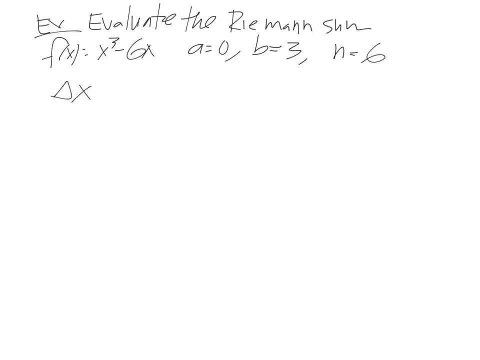 So if n is 6, what's our delta x? So this is all what's given. Delta x is going to be our b minus a over n, Which is 3 minus 0 over 6.. Or it's going to be 1 half. 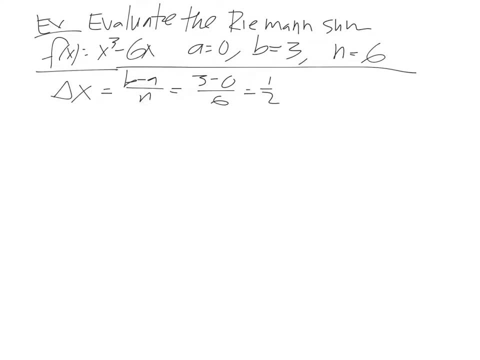 So if our right endpoint is a, 0.. So our x sub 0, which is a, is 0. Then the next point, x1 is going to be- So we're going by a half, It's going to be 0.5. 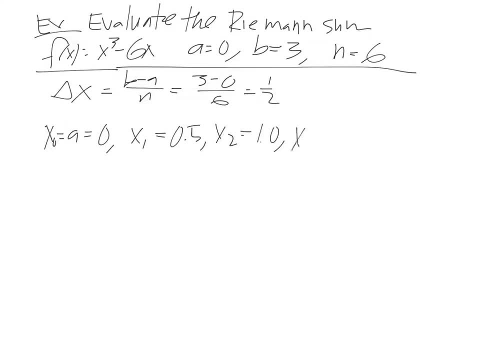 x2 is 1.0.. x3 is 1.5.. x4 is 2.0.. x5 is 2.5.. And then x6 was our endpoint b. x6, which is b, is really 3.0.. 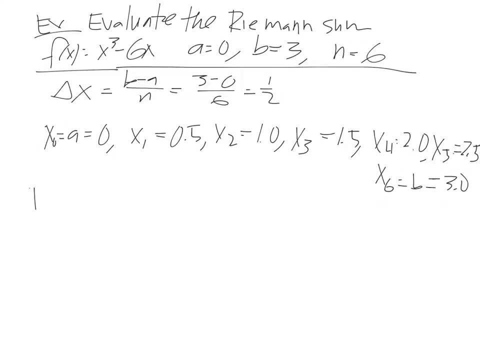 So the Riemann sum R6 is going to be the sum Where i goes from 1 to n, Or 1 to 6, rather Of f, of x, sub i Times delta x. So we're going to get: 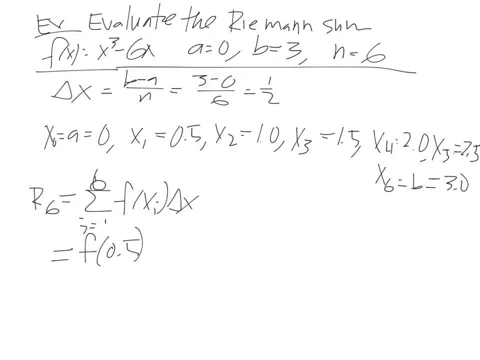 Our first will be f of 0.5. Times delta x Plus f of 1.0. Times delta x Plus f of 1.5. Times delta x Plus f of 2.0. Times delta x. 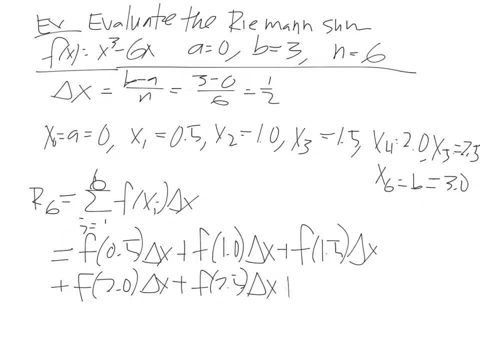 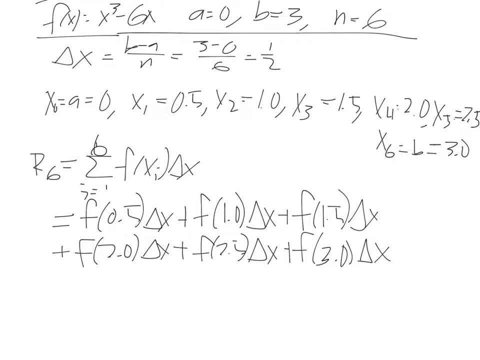 Plus f of 2.5. Times delta x, Plus f of 3.0. Times delta x, And so Give me a little bit more space. And remembering our function, f of x is x cubed minus 6x. 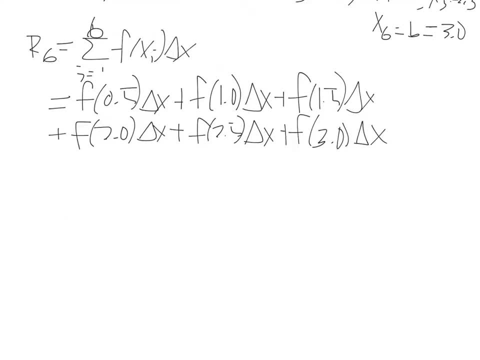 And so this all Can be simplified. Since delta x is really 1 half, I'm going to factor out delta x from everything, And so we get f of 0.5.. Ends up being Negative 2.875.. 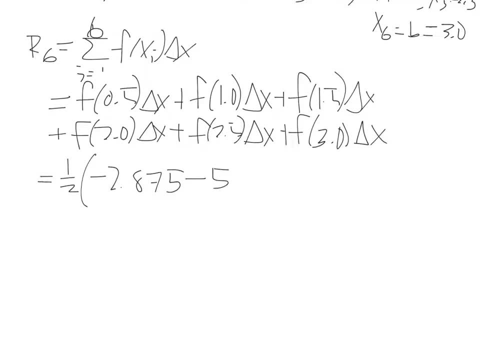 f of 1 is Negative. 5. f of 1.5 is negative: 5.625.. f of 2 is negative, 4. f of 2.5.. So now we're getting to positive numbers And that's 0.625.. 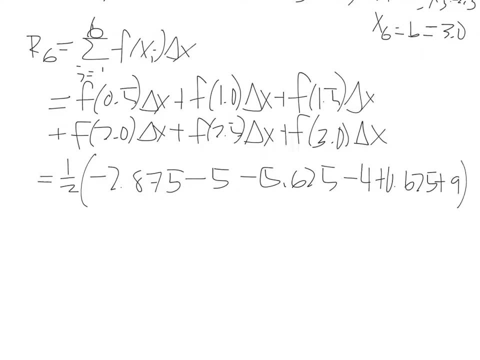 And then f of 3 ends up being 9.. So This whole thing, We get Negative 3.9375.. And what you notice is This is actually a negative number. Well, if we were to have graphed this. 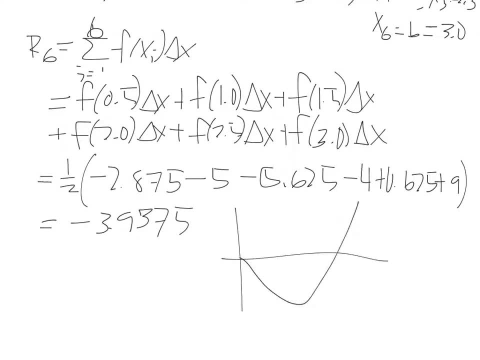 What this would have looked like, Something Like that. And so we did pick A couple of Points right here: Our first Rectangle, Second rectangle, Our third rectangle, Fourth rectangle And then Our fifth rectangle Comes- Positive. 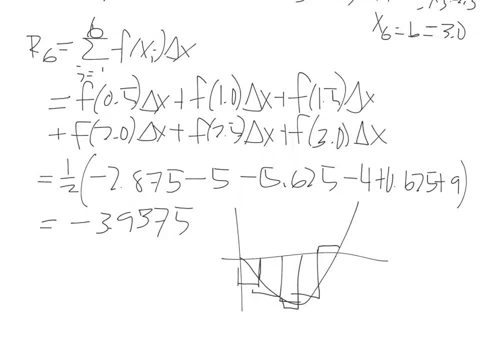 And then Our sixth rectangle Is also going to be positive, But If we're below the axis, Then It's a negative value, And so that's why Most of this is going to be below, And so we end up with a negative. 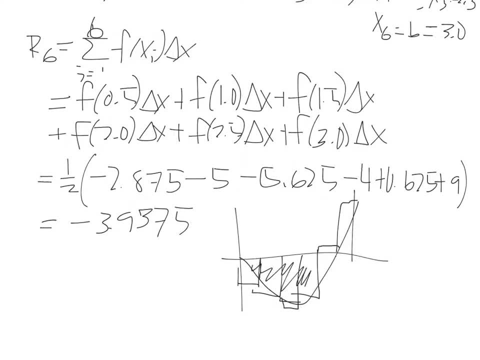 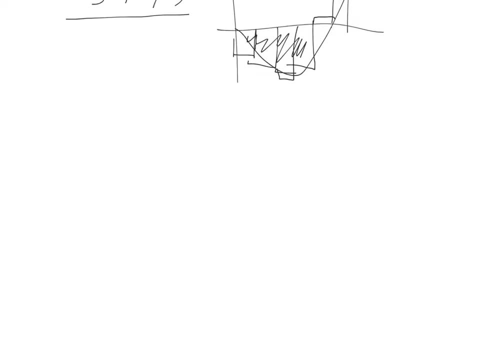 At the bottom, At the bottom, At the bottom. Now, Continuing on This Example, Calculate The Integral From 0.. To 3.. Of X Cubed Minus 6x dx, 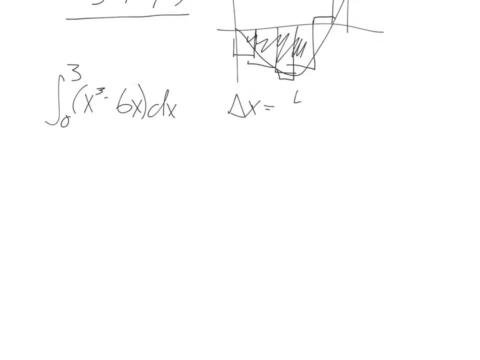 Well, What's our delta X Going to be? Delta X Is B Minus a. a over n is 3 over n. We started off. our x0 was 0.. Our x1, if we're going at intervals. 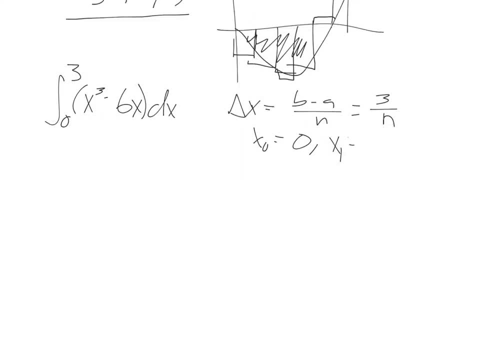 of 3 over n is 0 plus 3 over n, or just 3 over n, Our x2, we add another 3 over n, so it's going to be 6 over n, and so forth. x3 would be 9 over n. So in general we'd get: 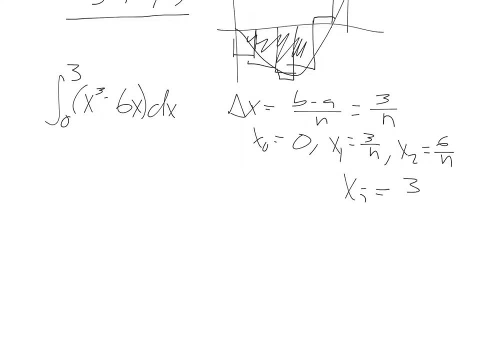 x of i is equal to 3i over n, And this is since we're using the right endpoints. Well, since we're using the right endpoints, rather, we can write that this integral is equal to the limit- as n goes to infinity- of the sum where i goes from 1 to n. 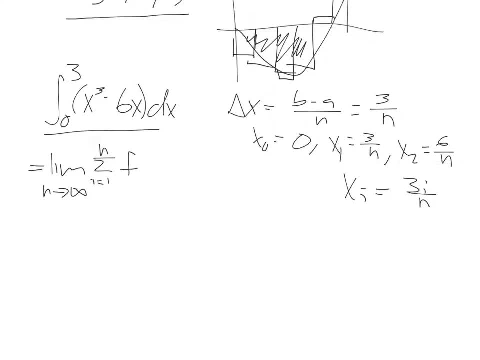 which is the limit of the sum where i goes from: 1 to n Of f of x of i times delta x. And now we can fill in: we know what x of i is and we know what delta x is. so this is the limit, as n goes to infinity, of the sum where i goes from. 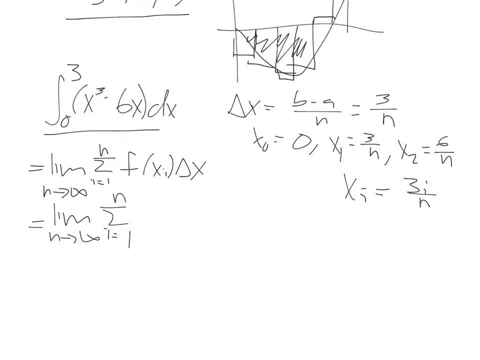 1 to n of x of i is going to be 3i over n times delta x. Our delta x is going to be 6 over n, And so now we know we can start filling some things out. Excuse me, not 6. 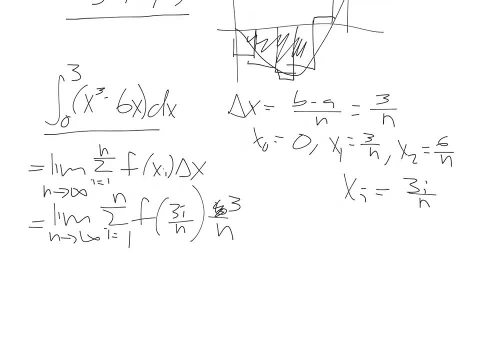 over n, 3 over n. So, using what we know, 3 over n does not relate to i, so we can pull this whole thing in front of the sigma, in front of the sum, so we get the limit as n. 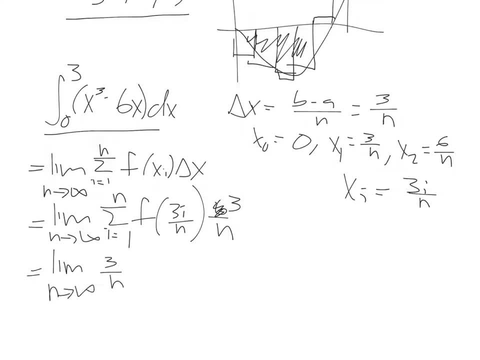 goes to infinity, of 3 over n times the sum where i goes from 1 to n, And what's f of 3i over n, Where our function was x cubed minus 6x. So this is going to be the quantity 3i over n cubed minus. 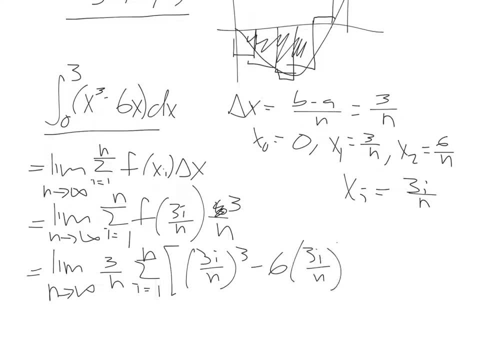 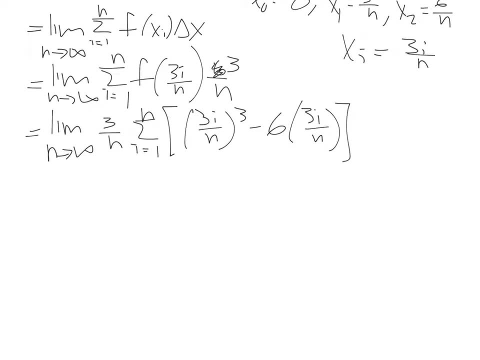 6 times. Now you're probably thinking this is not the nicest thing, and you're probably right: it's not that nice. So this is going to be the limit, as n goes to infinity of 3 over n times. now we'll go ahead and factor out inside here or multiply, so this becomes: 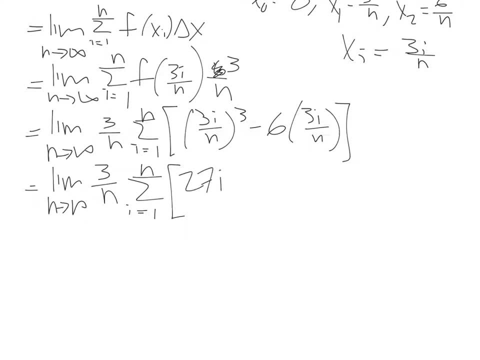 3i over n cubed 27.. And this is i cubed over n cubed minus 18i over n. Now we're subtracting to sums, So we're taking the sum of the subtractive And so, because of this difference, we can split this up into two summations. 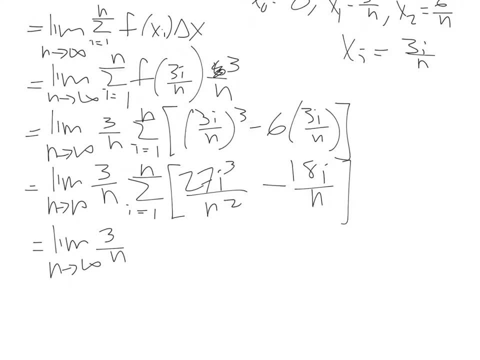 And when we split this up, this 27 over n squared, minus 18i over n, equals 28i over n wheel. There we go squared and this 18 over n, they don't deal with i, so we can pull them out. so this is going to be. 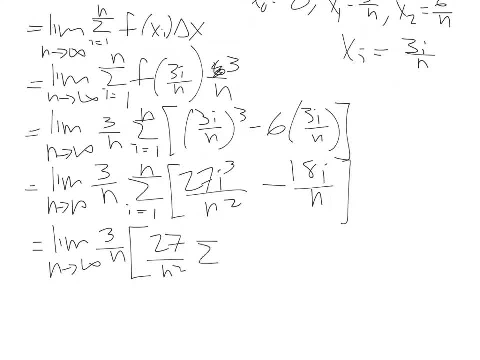 27 over n squared times the sum where i goes from 1 to n of i cubed minus 18 over n times the sum where i goes from 1 to n of just i. now we know what the sum, we know this sum and we know this sum. 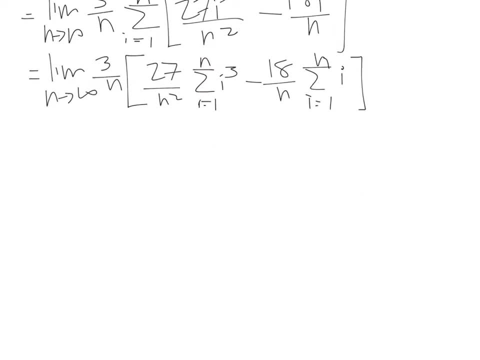 so let's keep forging ahead. this is the limit, where n goes to infinity, of 3 over n times the quantity 27 over n squared times. now this we know to be n times n plus 1 over 2 quantity squared. oops, uh, this should have been an n cubed way up here. 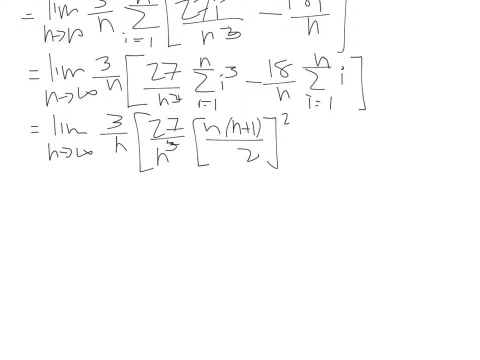 that should be an n cubed. then that should be an n cubed because that was 3, 3 i over n quantity cubed, so sorry about that. and then minus 18 over n times and then the sum where i goes from 1 to n of i. 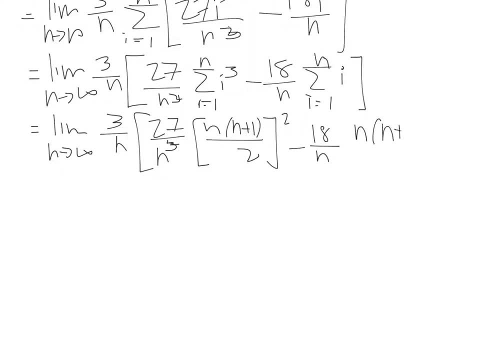 this is n times n plus 1 over 2, and i'm going to go ahead and i'm going to multiply this times this, and there's 3n times that. right there, so we get the limit, as n goes to infinity, of we have 81 over n to the fourth times. 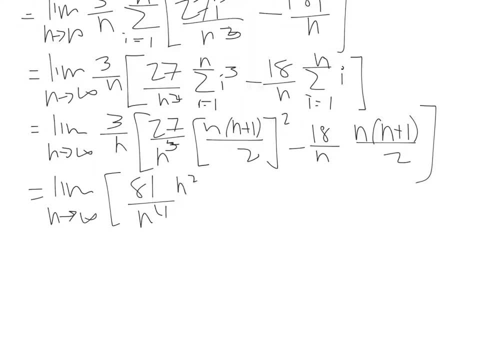 squaring this, we also have an n squared, n plus 1 squared, and this is going to be divided by 4 minus and we get 54 over. let's see we have n out here. so 3 times 18 is 54, and n times n would be n squared, and then we still have 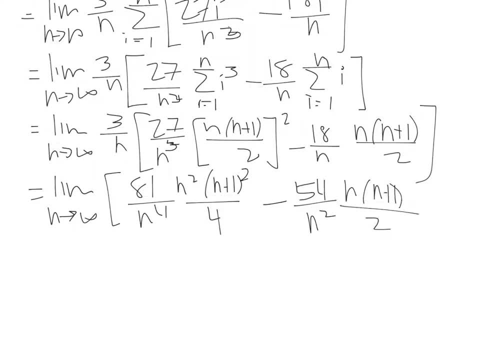 times n, n plus 1 over 2, so we can still simplify some more. so doing that, we get the limit, as n goes to infinity, of we get from this first term. we can pull out the constants 81 over 4. and now let's see. 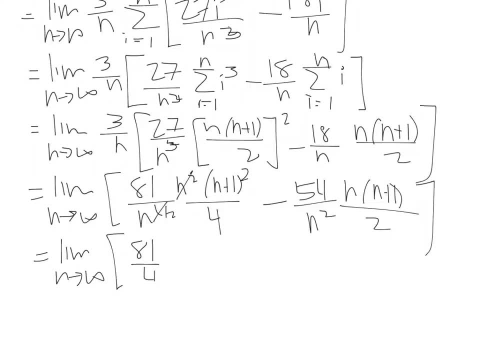 this n squared and this n to the fourth cancel. so it'll be n over over n squared, and so that's going to be n plus 1 over n squared, and in fact we could do a little simplification. yes, so we get n plus 1 squared over n squared minus 54 times. 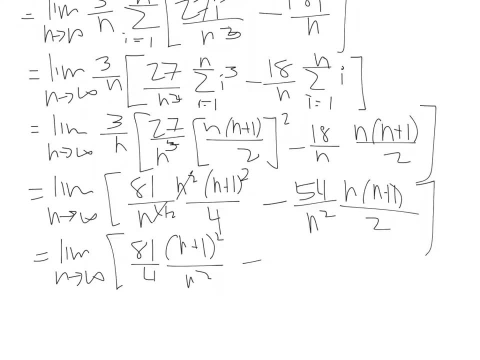 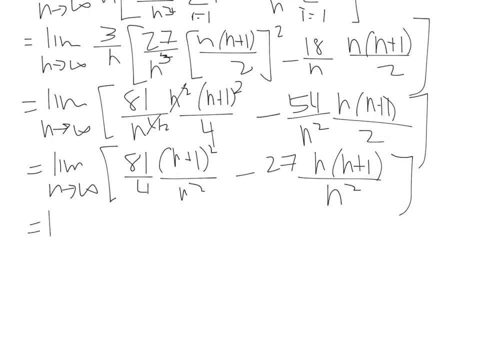 well, 54 over 2 rather, so back that up. sorry, we get 27 times n times n plus 1 over n squared. still not the nicest thing. but remember we're taking the limit as n goes to infinity, so we're almost there. this is gonna be the limit n goes to infinity of. 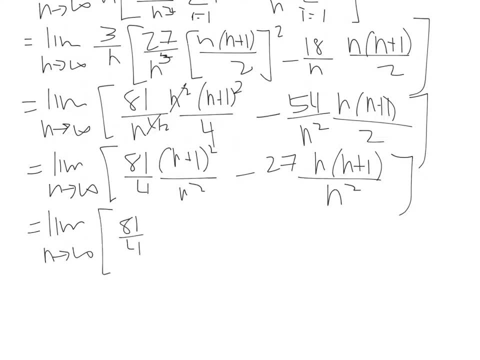 the quantity 81 over 4, and this factors n squared plus 2n plus 1 over n squared minus, and this is 27 times the quantity n squared plus n over n squared. and so this all becomes the limit, as n goes to infinity, of 81 over 4 times the quantity and. 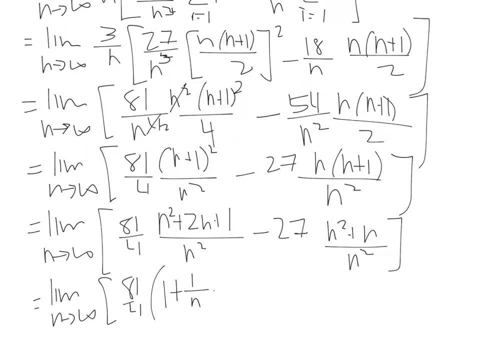 this is going to be 1 plus 1 over n, excuse me, 2 over n plus 1 over n, squared minus 27 times, and then we get 1 plus 1 over n. all right, almost there the limit as n goes to infinity. well, if n goes to. 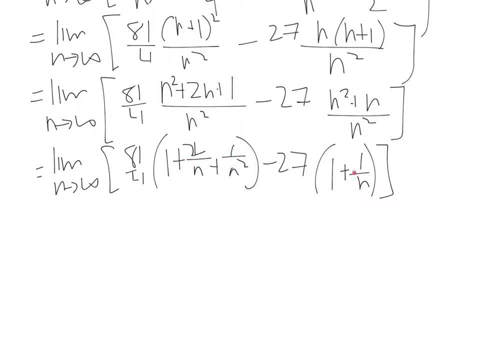 infinity. this term goes to 0, this term goes to 0 and this term goes to 0, and we're almost there. so this is going to be 81 over 4 minus 27, which is negative six point seven five. so this is what that area is. 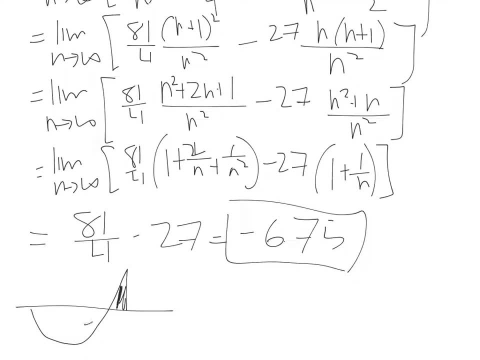 through the curve. that looks something like this: we have that area and this area more negative than positive. but that's what we got now. it's way better than our estimate using the Riemann sum, where we got negative three point nine, three, seven, five. I'm sure if we did the Riemann sum, where we found a lot more, 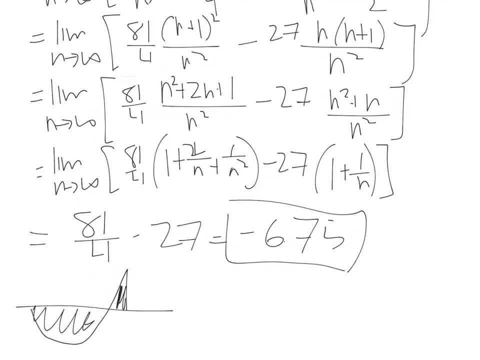 it would be a lot better. so if we did Riemann sum for 40, we get negative six point three, nine, nine, nine, eight. if we did with n is five thousand, we'd get pretty close negative six point seven, four, seven, three. so you think about this. this was a very long. 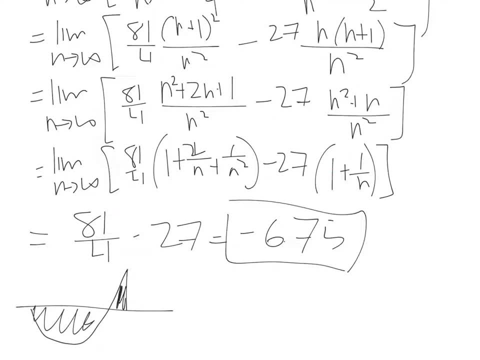 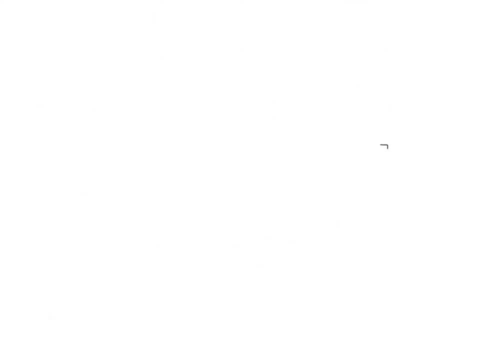 method to do this problem. but it sure beats calculating when n is five thousand, doing five thousand summations. let's do an example. remember: calculating the area or calculating the integral of something is basically finding the area under that curve. so if we're trying to calculate the area under the curve of 1 minus x, 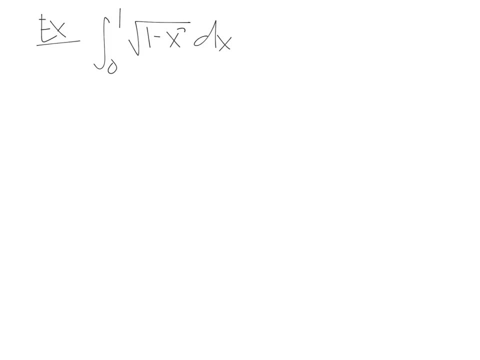 squared dx, and we're going from 0 to 1, or in other words, the integral from 0 to 1, the square root of 1 minus x squared. that is the same as finding the area. so rather than actually going through and trying to calculate this, sometimes it's. 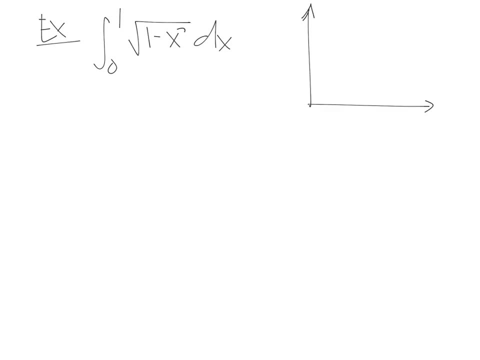 just useful to draw what that looks like. well, what is this? if we had, y is the square root of 1 minus x squared. if we squared both sides, we get y squared 1 minus x squared, or x squared plus y squared is 1, so it's a circle centered at. 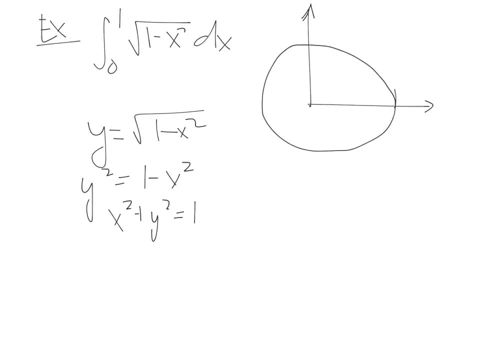 the origin with radius 1 and since this is the square root, meaning our y value is only going to be positive, so we can ignore this stuff below the axis. and then our x is going from 0 to 1, so really we're just going to be going from 0 to 1, so we're just concerned with this right here. this is: 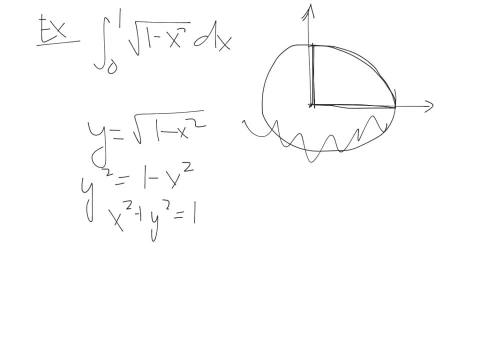 one-fourth the area of a circle, so the area is one-fourth pi r squared plus r, and since r is 1, this is just pi over 4. so we can calculate the error or the integral from 0 to 1 of the square root of 1 minus x squared dx is pi over 4. 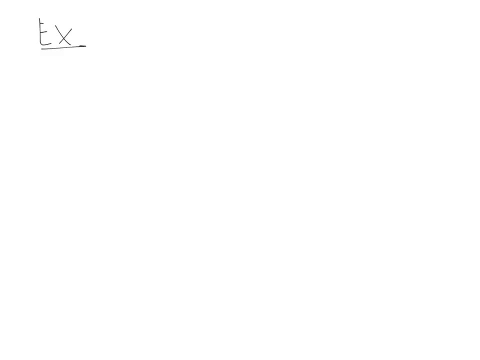 let's do another example. what about the integral from 0 to 3 of the quantity x minus 1 DX? hello again, we're just trying to find the under curve. so if we were to graph this this, it's going to get negative 1 at 0. 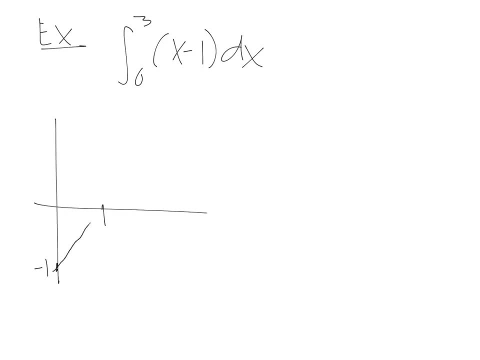 it crosses the axis at 1 and it goes up, and when X is 3, your y value is going to be 2. well, we have here are two triangles, or call these two triangles, because they triangles A1 and A2.. If it's below the axis, it's negative. 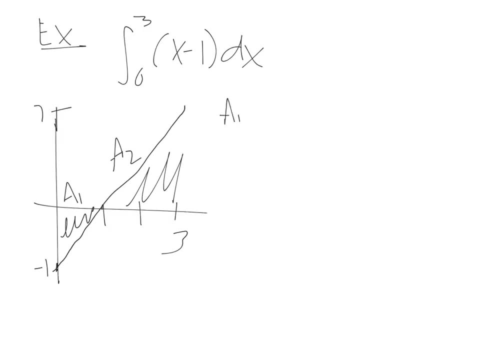 If it's above the axis, it's positive. Well, A1 is going to be, it's negative. but what is the area of the triangle? 1 half base times height. So 1 half 1 times 1.. 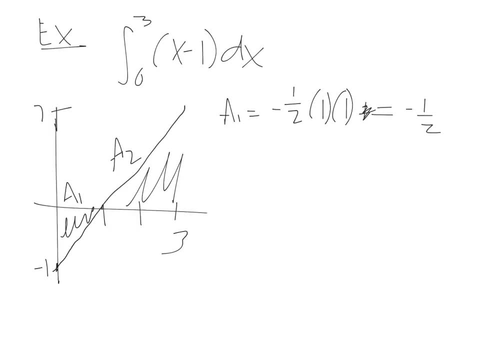 So that's A1, and this is going to be just negative 1 half. A2 is 1 half base times height, So this is 2 by 2, and so this is going to be 2.. So the integral is just this negative 1 half plus 2,. 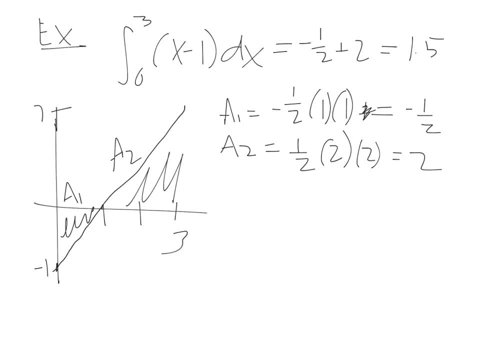 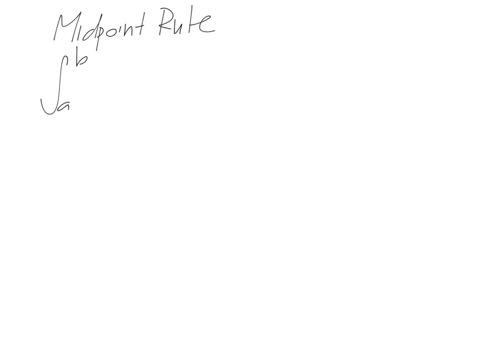 and we get this is going to be 1.5.. So sometimes calculating the areas or the integrals not as bad as the last example we did Now calculating the integral using the midpoint rule. the midpoint rule says the integral from A to B. 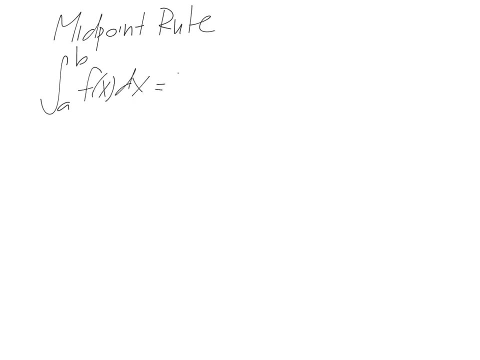 of f of x, dx is equal to the sum where i goes from 1 to n of f of x sub i, and we're going to use bar x sub i, bar times delta x, And what this is is this is delta x times f of x1 bar plus so forth. 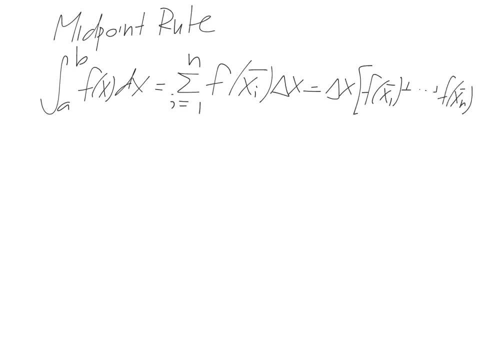 all the way to f of xn bar. So this is: we're going to say our delta x is the same, B minus A over n and our x sub i bar. that's the average or the midpoint. So we're going to it's going to be 1, half of the left part. 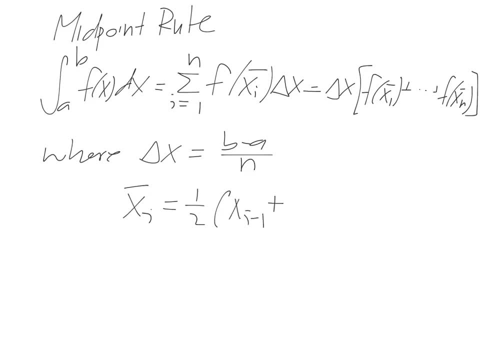 of the subinterval, so x sub i minus 1, plus x sub i, taking the averages of this. So in other words, midpoint of the interval x sub i minus 1 to x sub i. Now we're going to go over some properties. 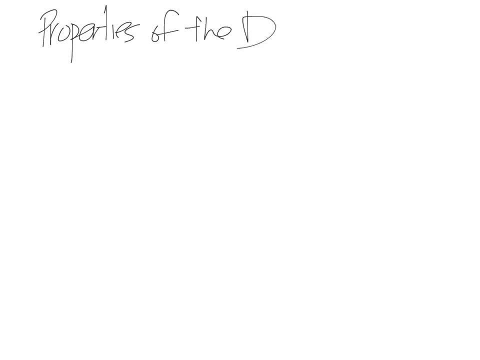 of the definite integral. The first property says that, and let me change my ink right here. So the first property says the integral From. normally we go from A to B, So the integral from B to A of f, of x, dx. 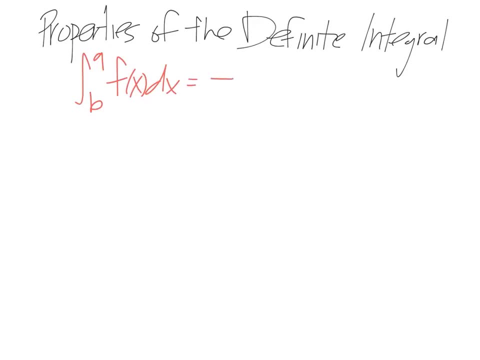 So if we're going backwards, this is negative. the integral A to B of f of x dx. So if we go backwards, then it changes. What about if your A and B are equal? So this is the integral from A to A of f of x dx. 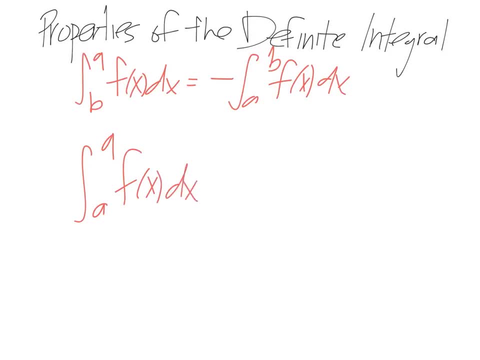 x, dx. well, you don't have any area. there's nothing to go under, since it's just a single point. so the integral is 0, all right, so here's more properties: the integral from a to B of just some constant C, DX. well, that's just C times B minus a. yeah, this is where C is a. 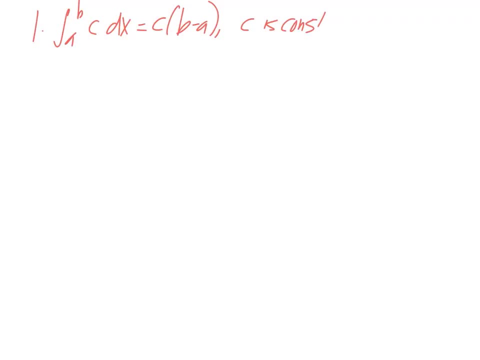 constant. so if you think about that constant, if we looked at the picture, the constant is just a horizontal line. so if you're from A to B of a horizontal line, we have a rectangle. area of the rectangle is base times height. the next property: we have the integral, from a to B, of the sum f of X plus G of X- DX. well, this is really. 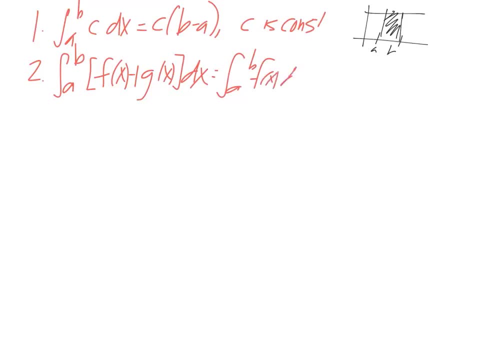 the integral from a to B of f of X DX, plus the integral from a to B, G of X DX. if we have an integral from a to B of some constant times, your function f of X DX. this is just the constant times. the integral from a to B of f of X DX. again, C is a constant if we have the integral from a. 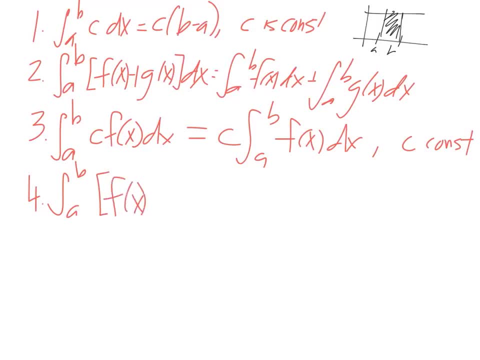 to B of the difference f of X minus g of x DX. this is the integral from a to B of a wave of x dx. yes, let's work that dex. so the assemble the내 monedice f of x dx minus the integral from a to b, g of x dx. now the fifth one, if we have. 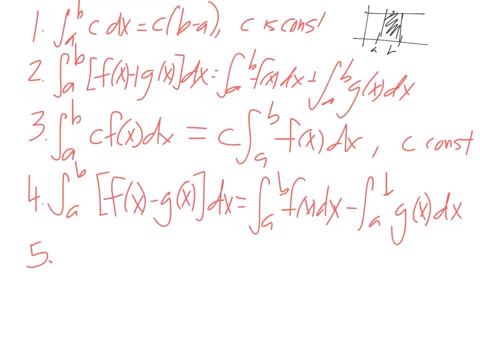 some, let's say, looking on like a number line, if a is over here, B is over here and C is in between, and you go a to C and C to, so you go from a to C and then C to B. it's the same as going all the way. in fact, this works where C doesn't. 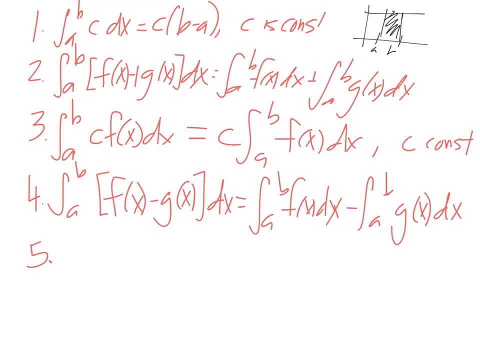 even need to be between a and B. C could be on the outside, but we get. we get the following: the integral from a to C of f of x? dx plus the integral from C to B of f of x? dx is equal to the integral from a to B of f of x. 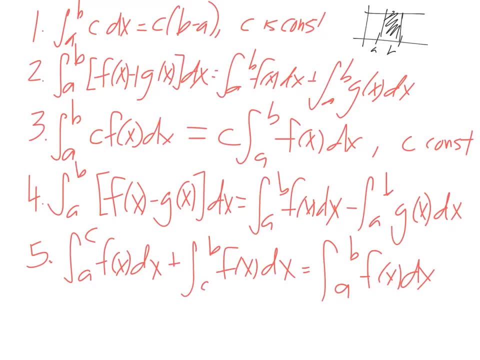 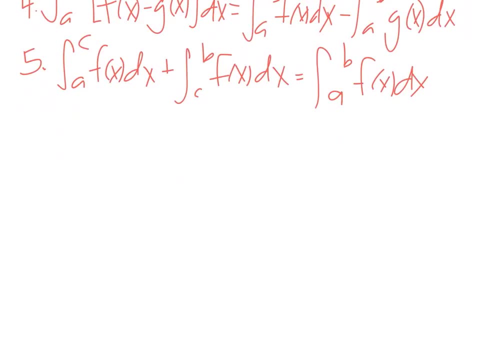 dx, and now we have a couple of properties where we compare the integrals, and so this first property says that if f of X is greater than or equal to zero- this is for a being less than or equal to X being less than or equal to B- then the 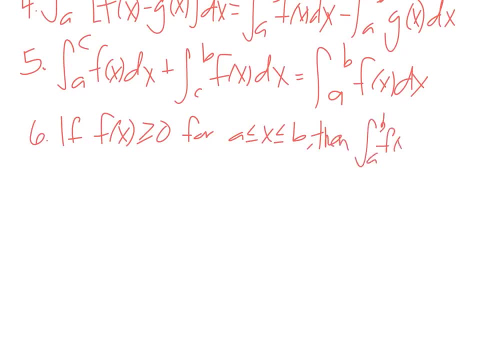 integral from a to b of f, of x, dx. so if our function is always going to be a positive, then the integral will be positive. if we have f of x is greater than or equal to another function, g of x for a less than, equal to x, less than or equal to b, then we have the integral from a to b of f of x, dx will be greater. 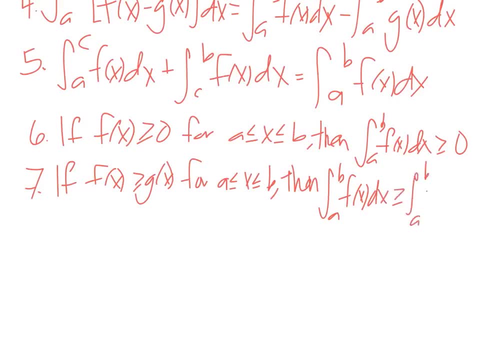 than or equal to the integral from a to b, of g, of x, dx. and then if m is less than or equal to f of x, which is less than or equal to capital, M for a is less than or equal to, x is less than or equal to b, then we have that m times b minus a. 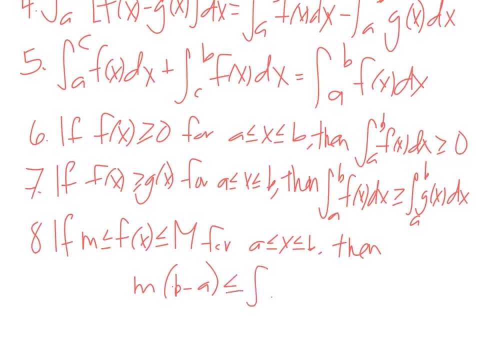 is less than or equal to the integral from a to b of f of x dx is less than or equal to capital M times b minus a. and really what we did right here was we took the integral from a to b of f of x dx times b minus a. and really what we did right here was we took the integral from a to b of x dx. 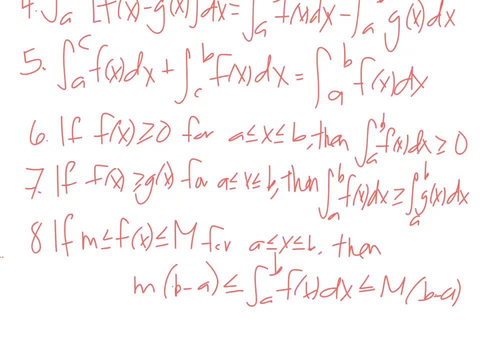 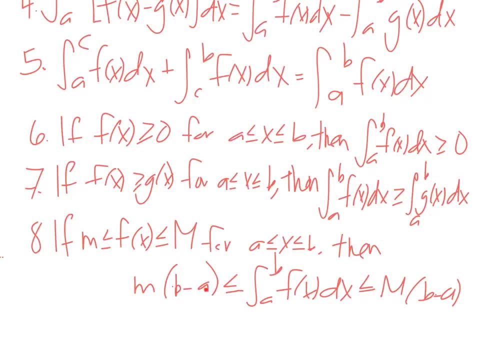 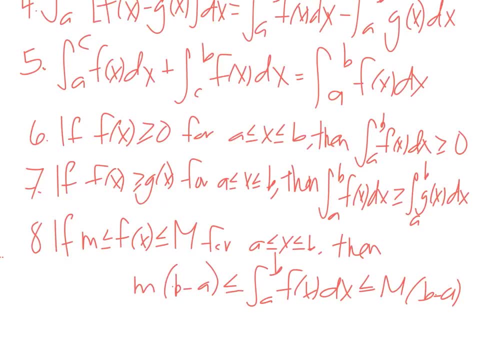 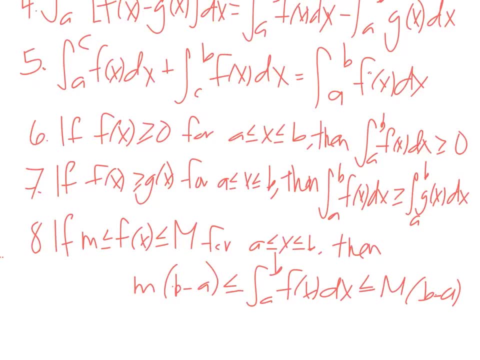 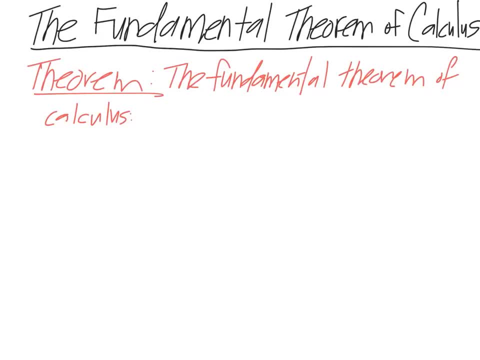 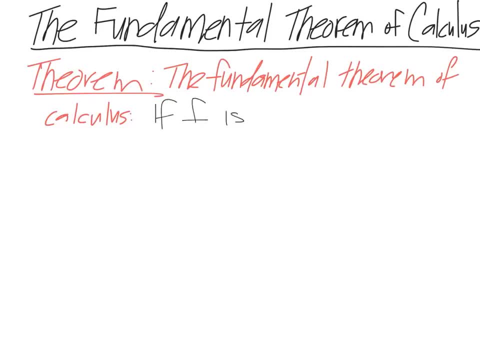 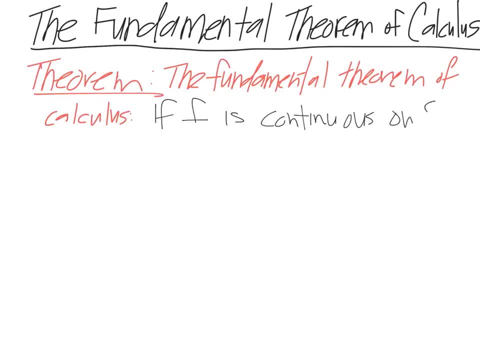 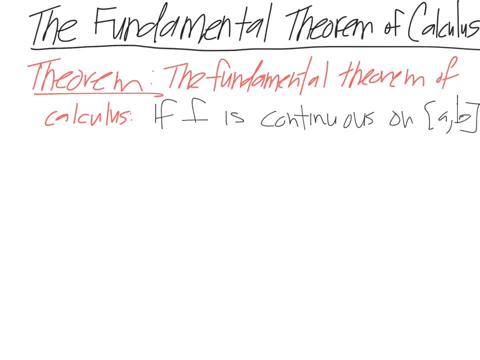 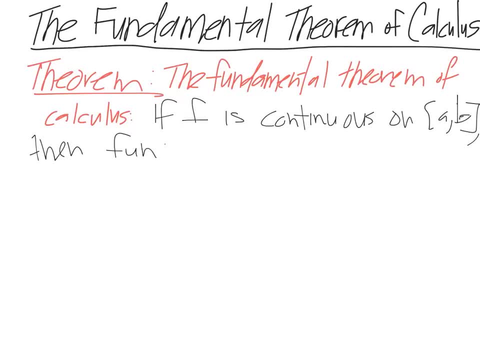 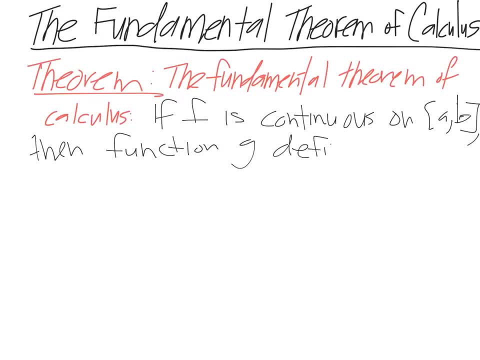 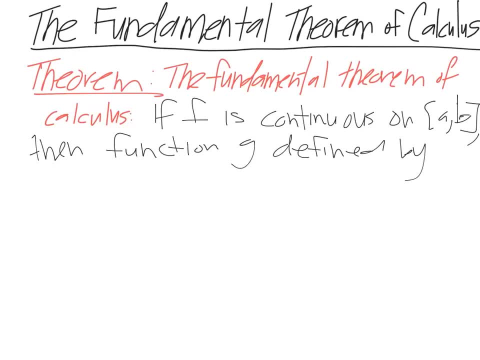 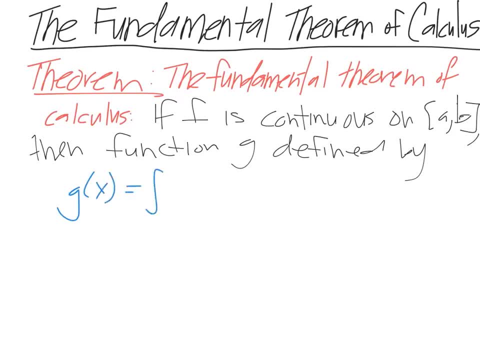 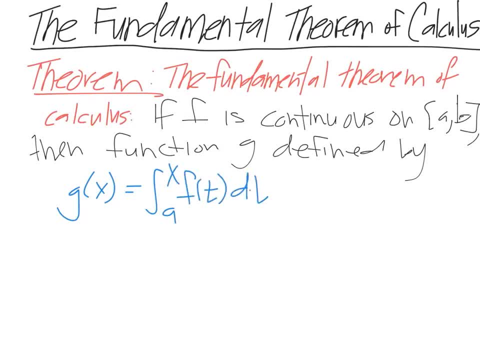 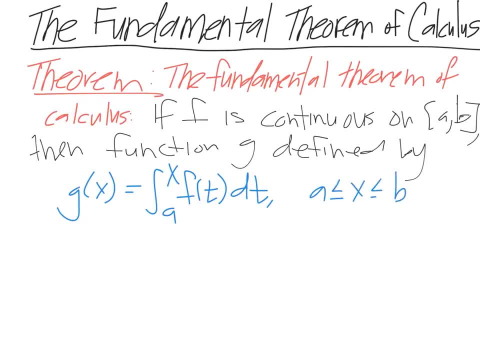 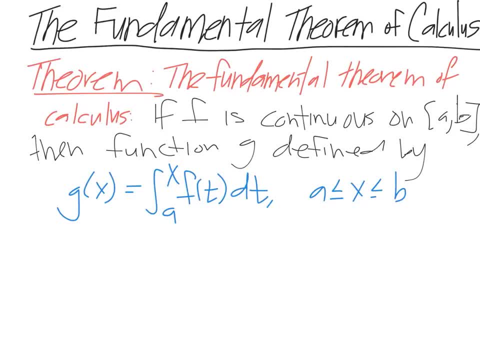 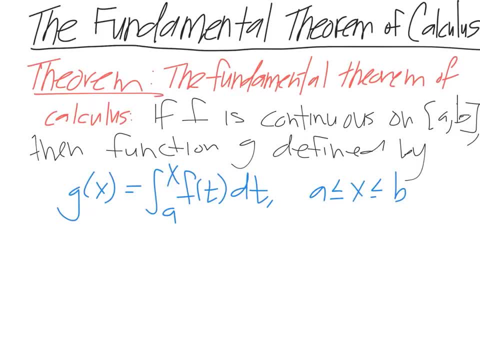 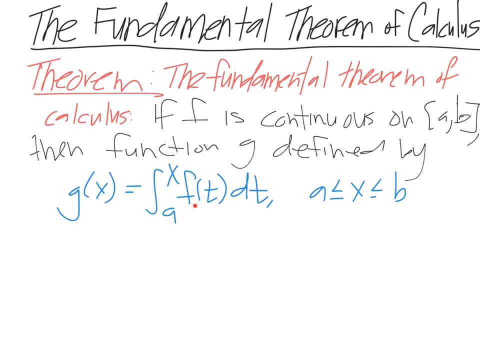 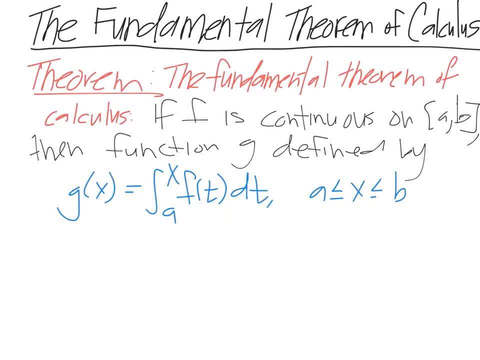 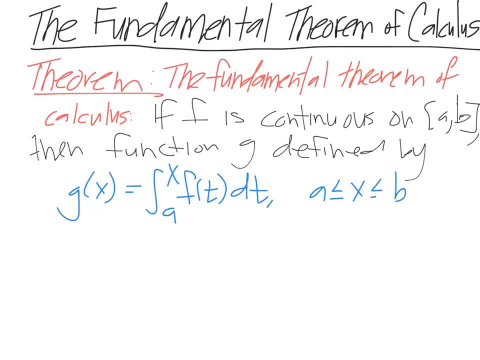 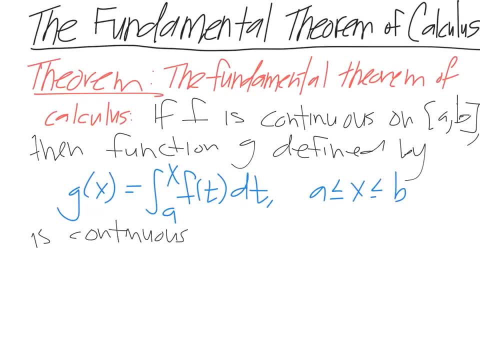 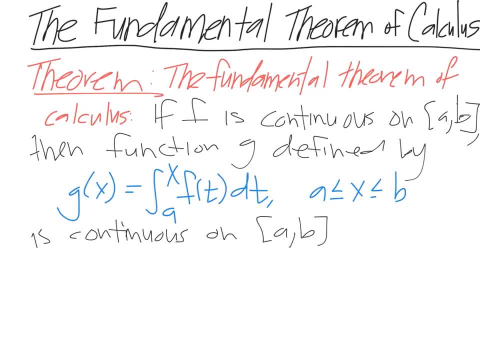 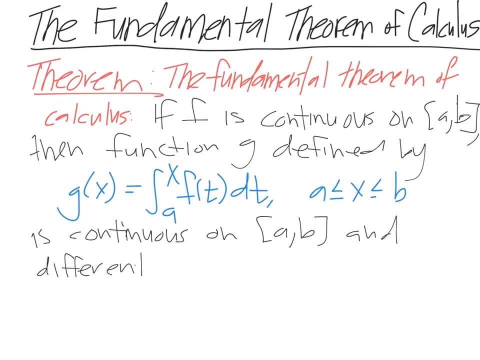 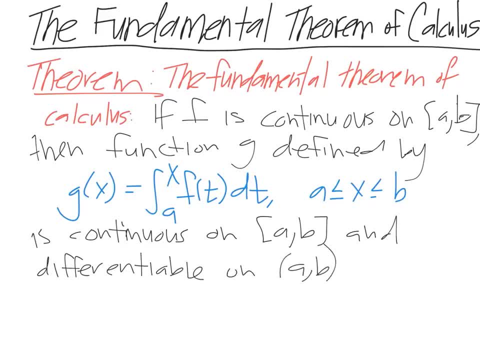 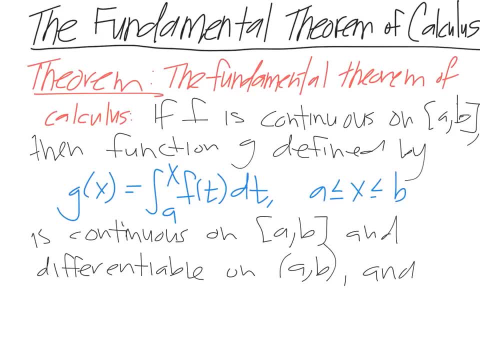 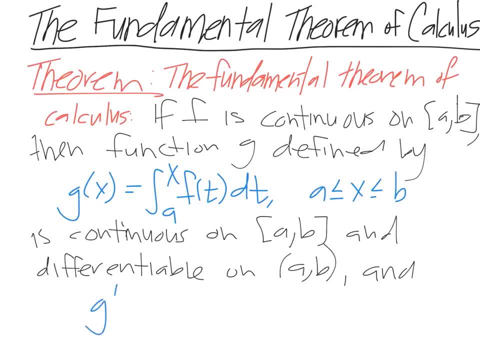 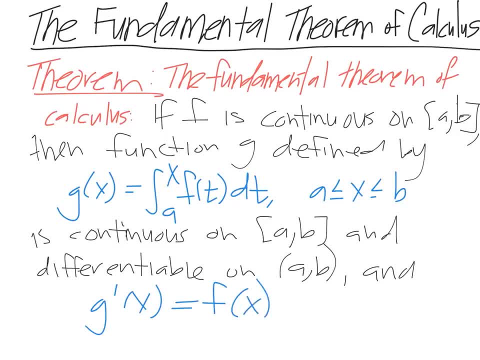 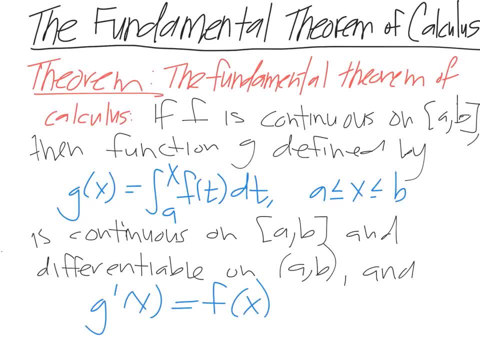 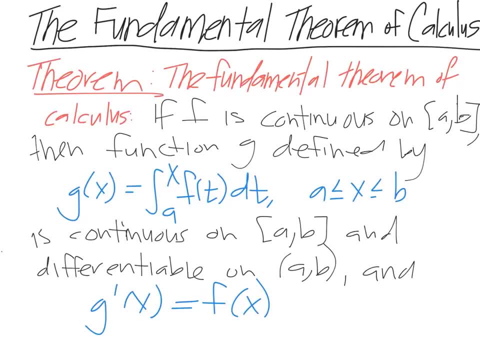 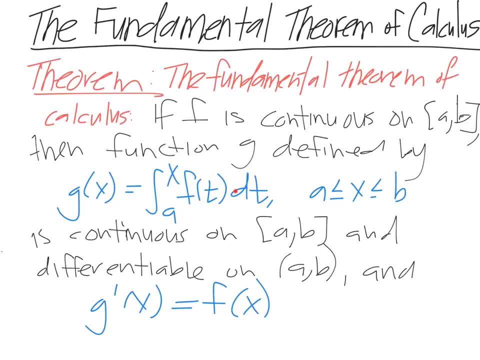 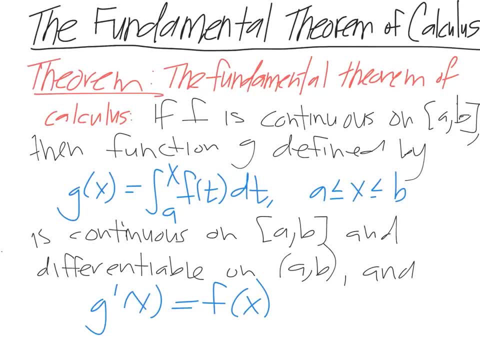 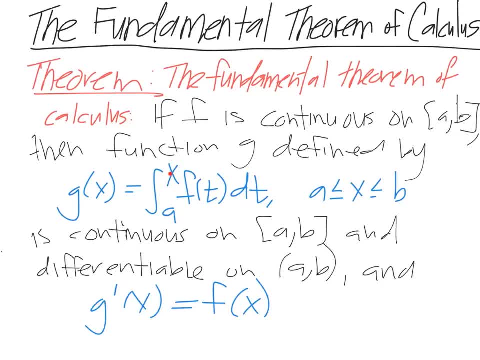 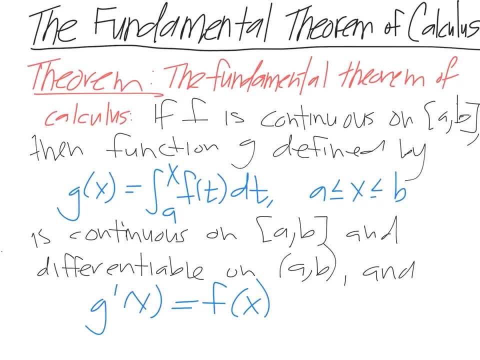 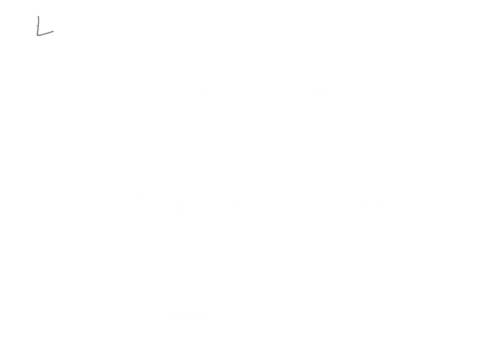 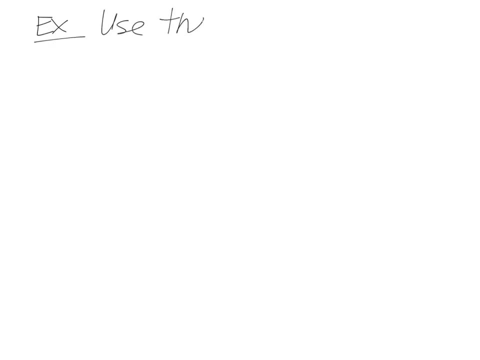 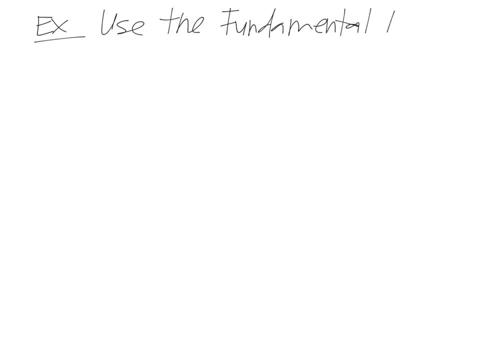 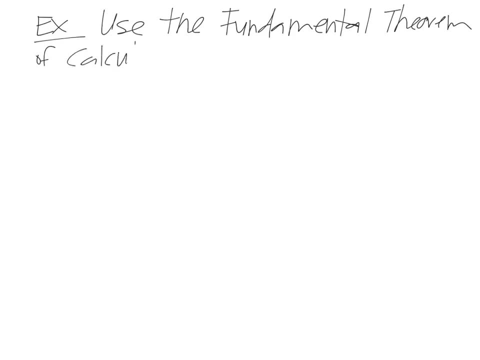 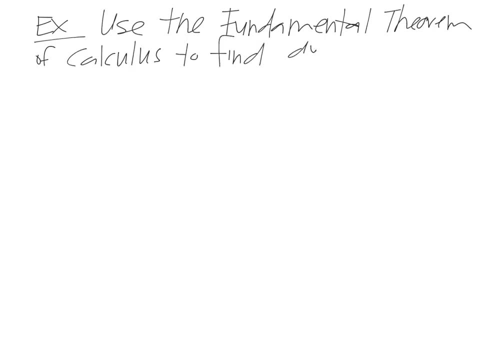 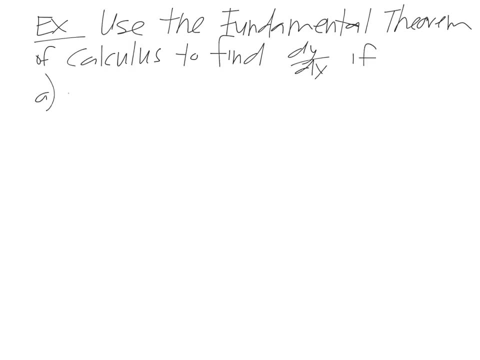 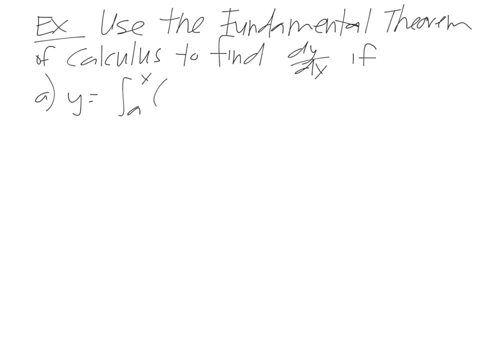 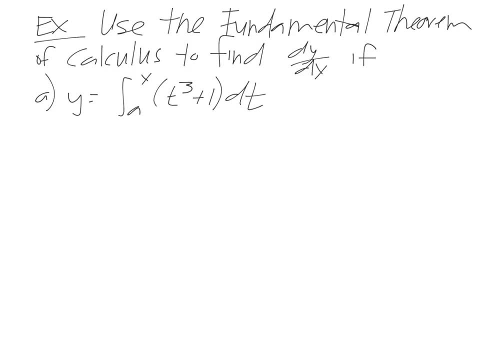 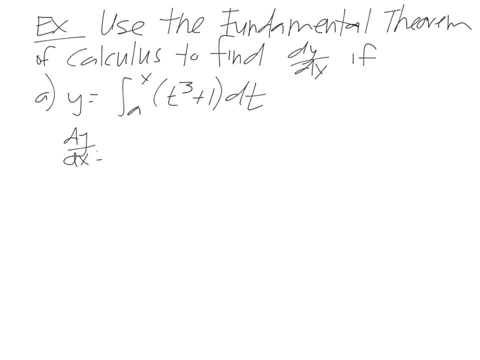 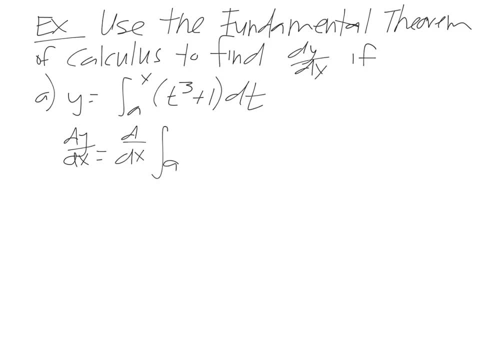 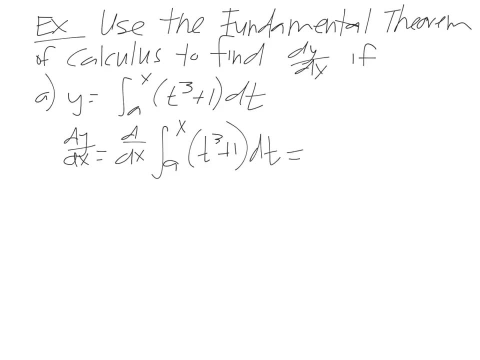 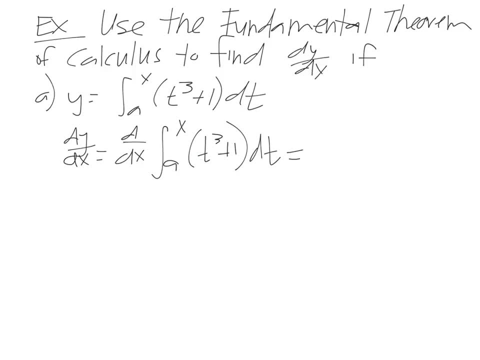 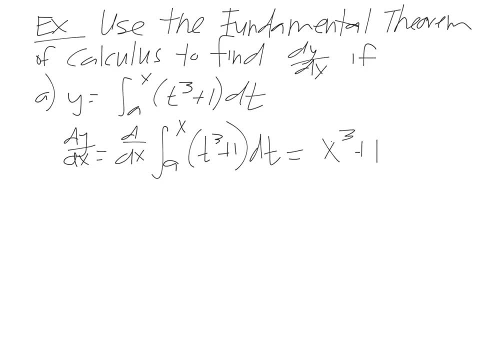 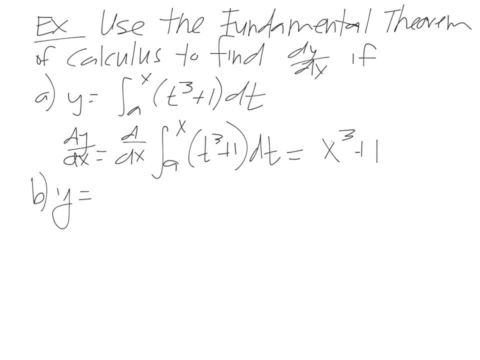 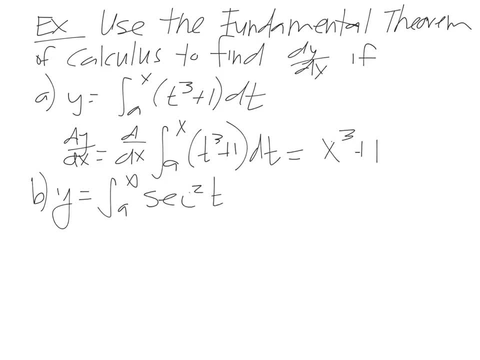 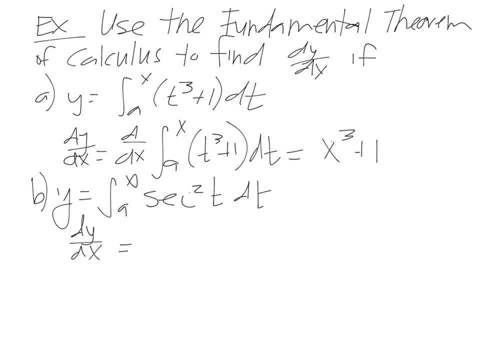 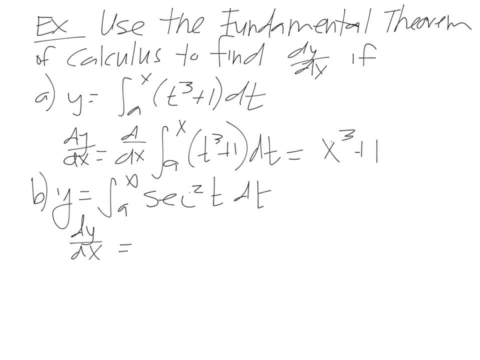 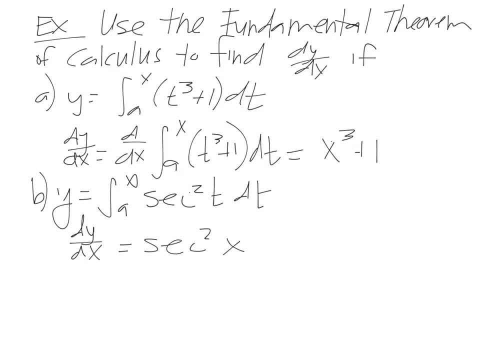 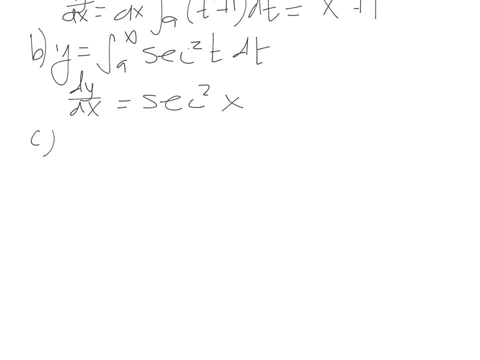 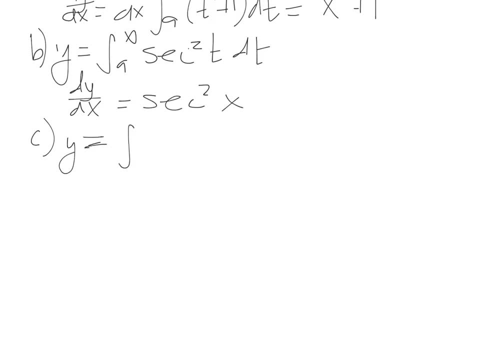 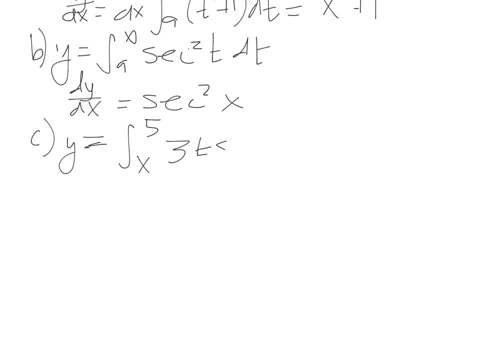 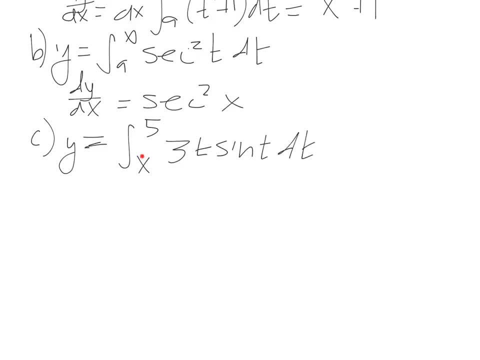 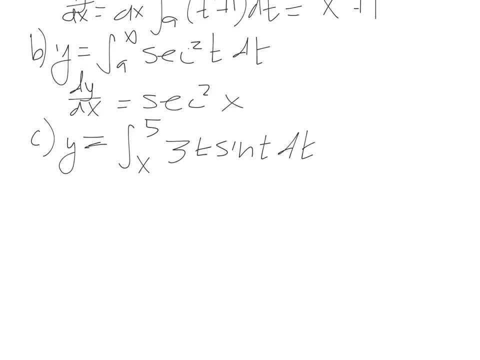 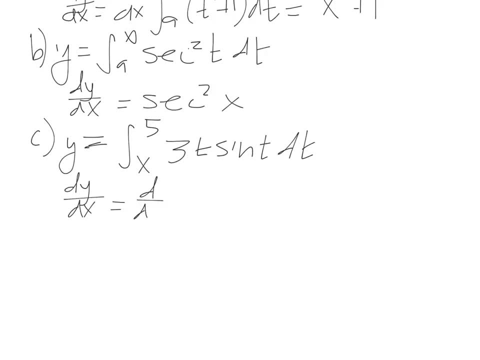 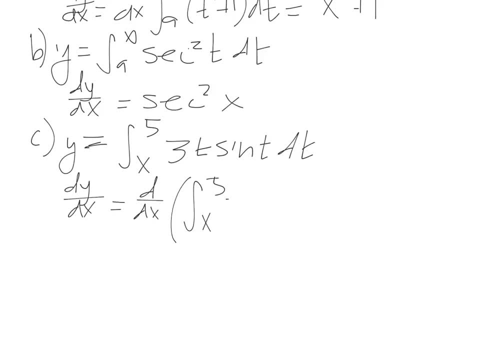 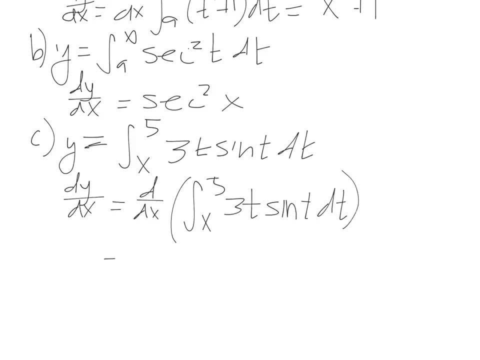 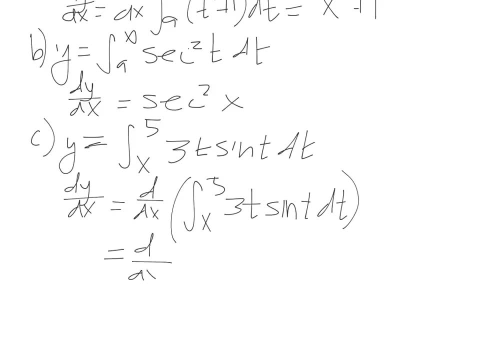 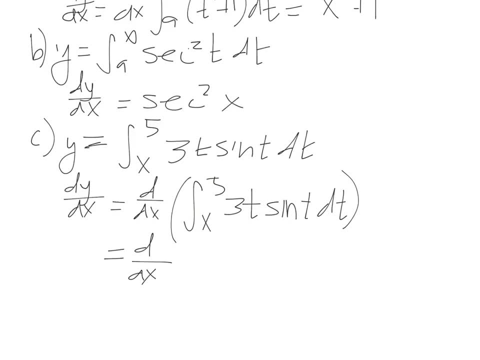 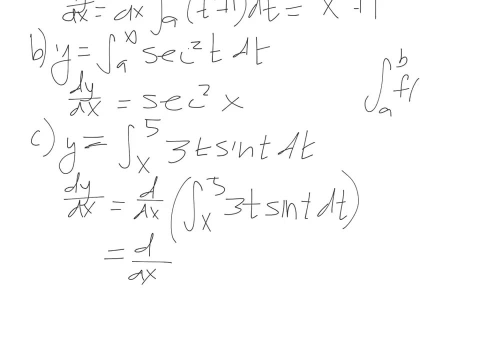 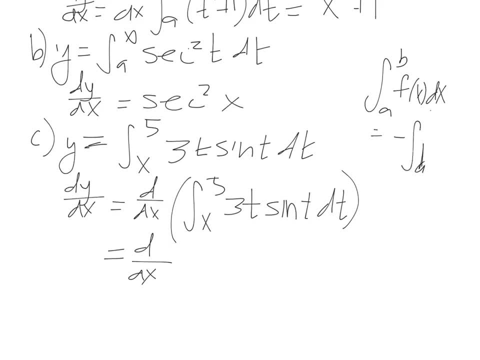 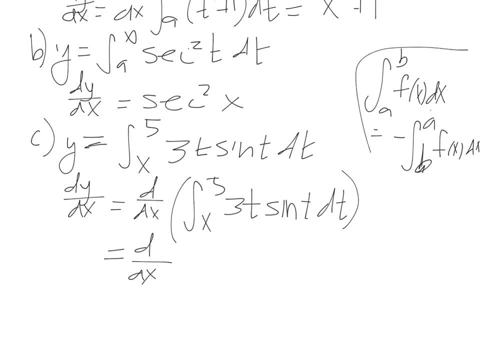 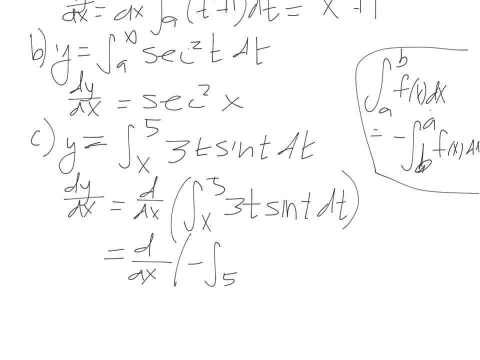 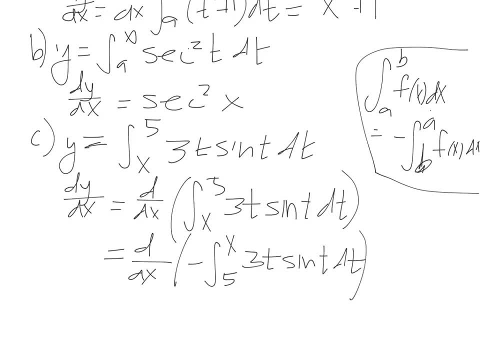 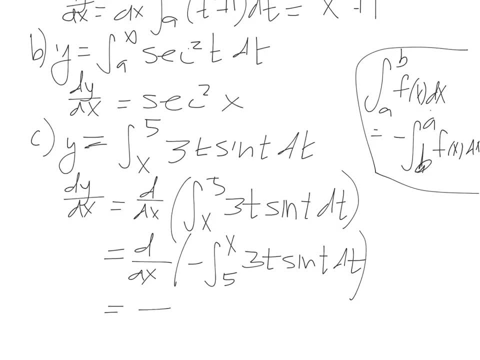 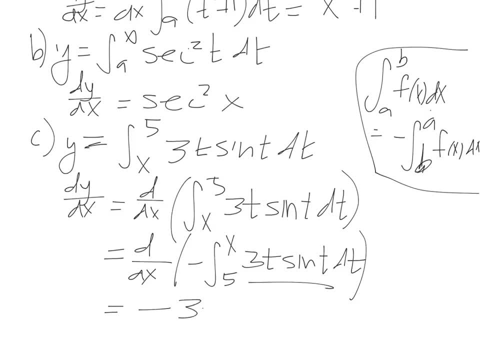 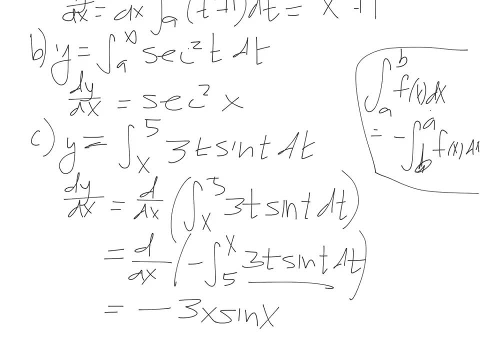 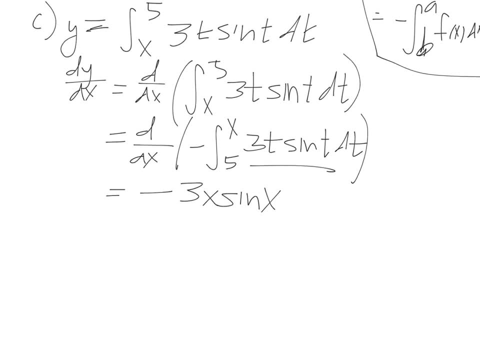 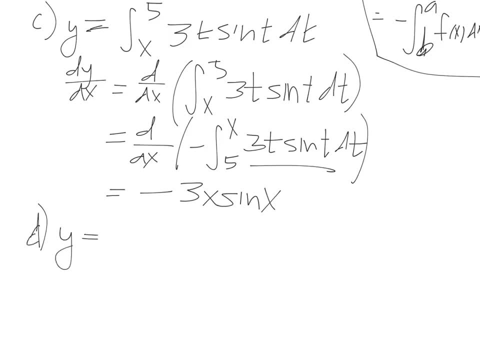 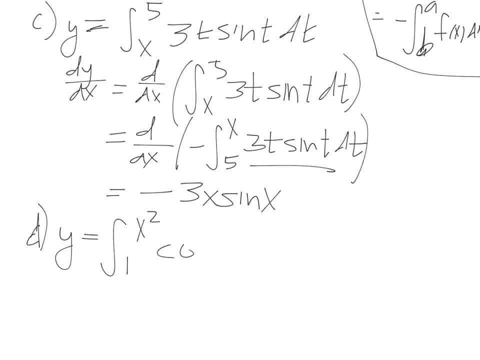 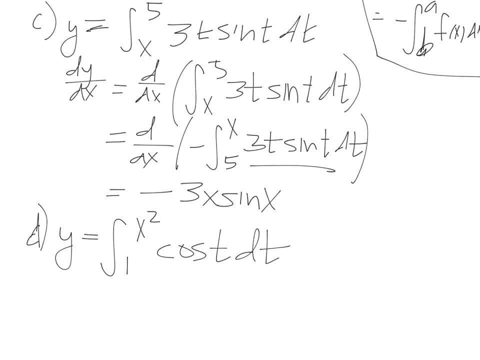 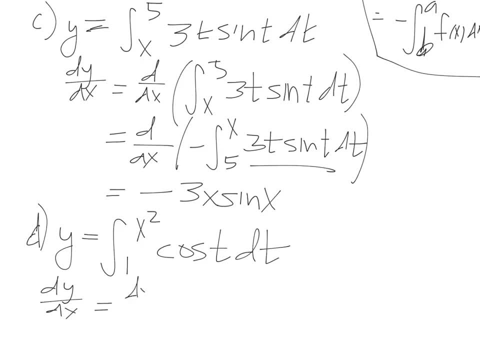 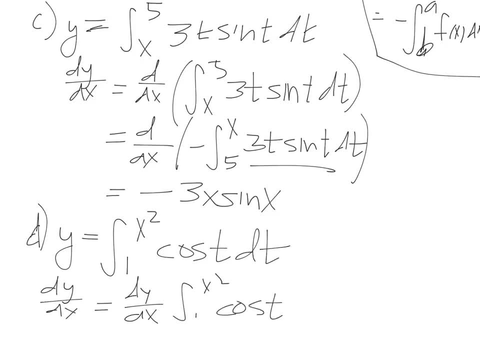 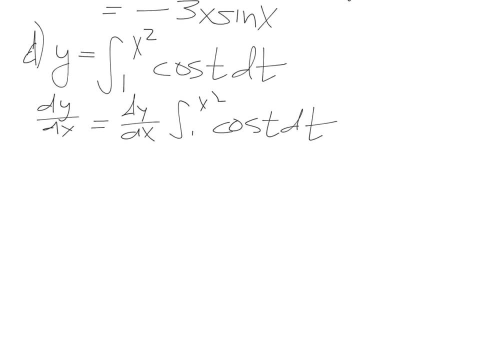 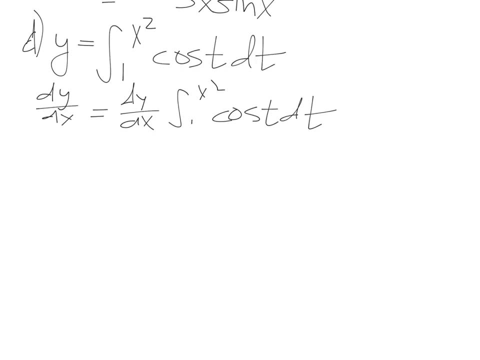 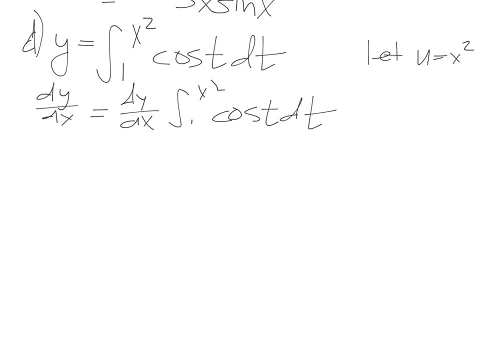 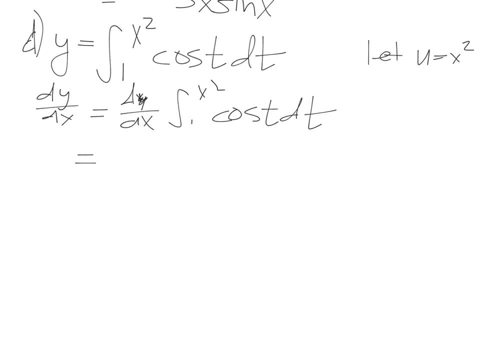 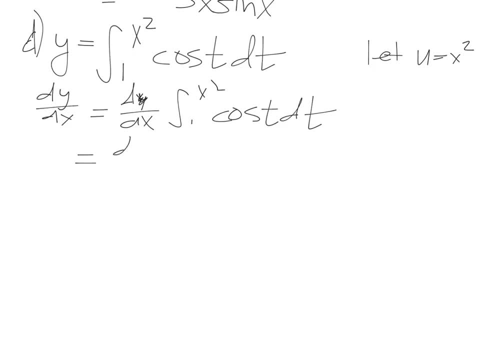 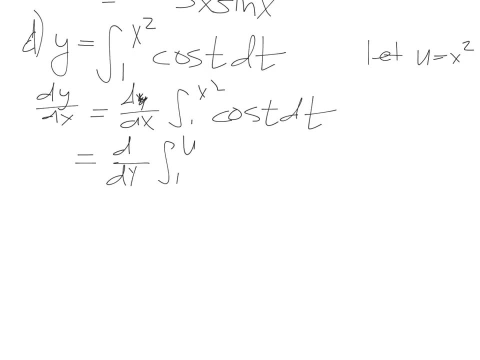 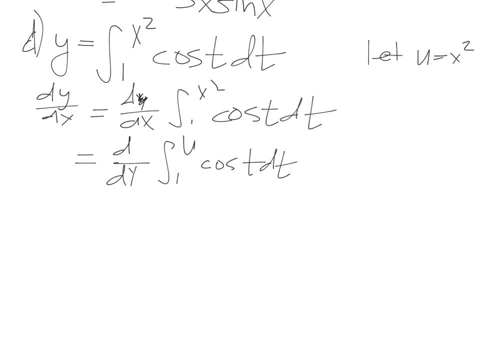 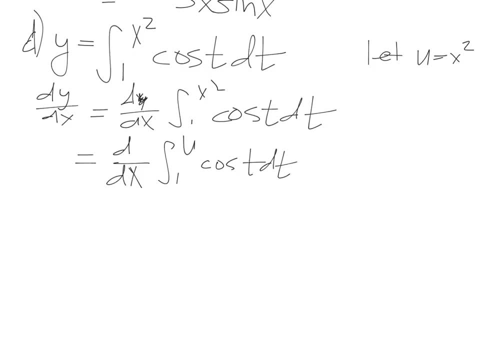 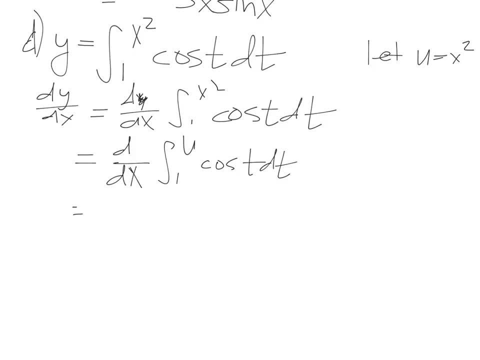 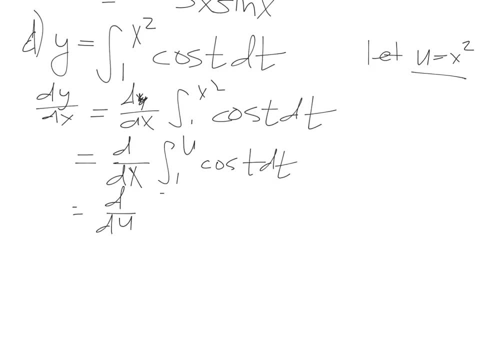 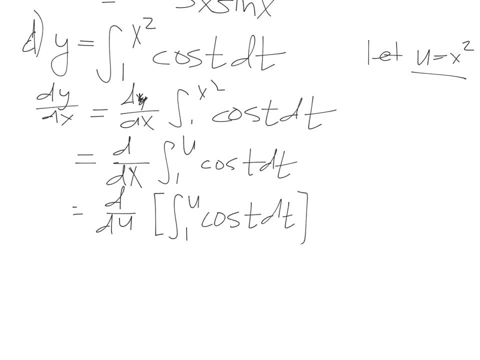 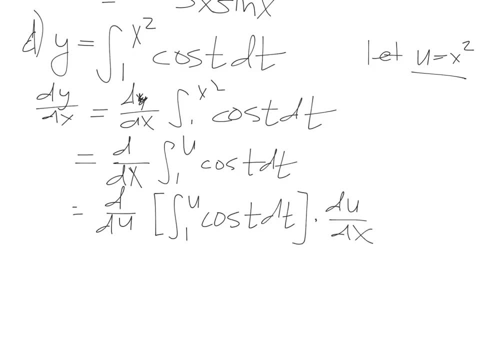 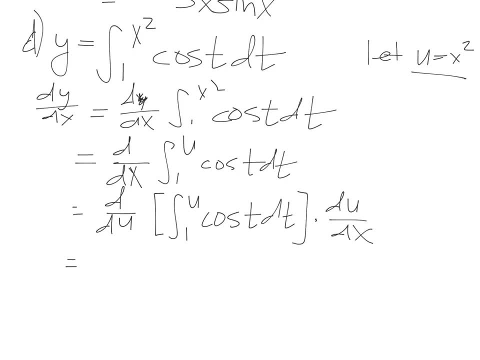 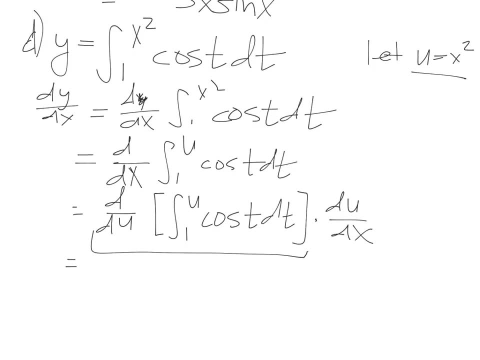 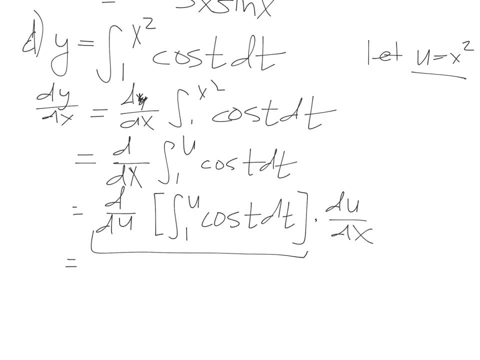 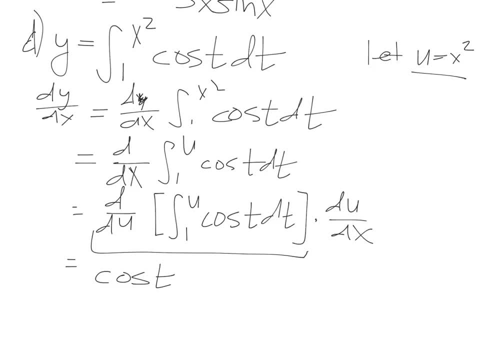 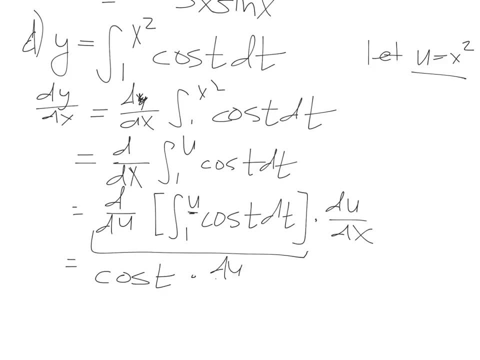 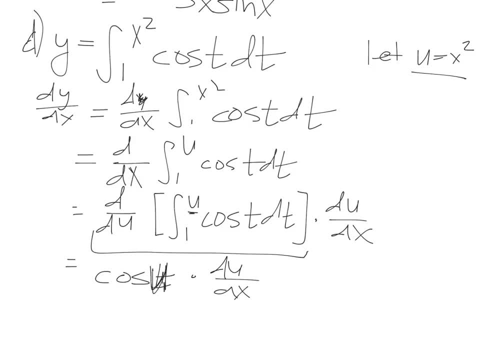 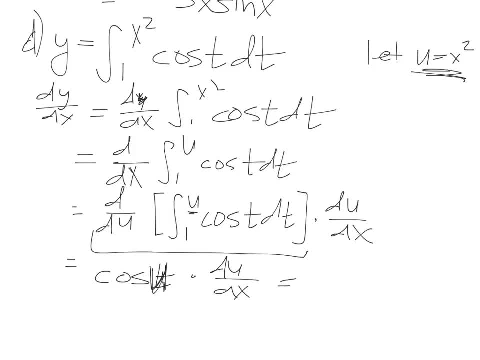 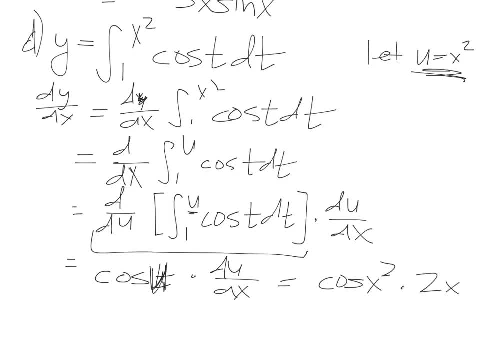 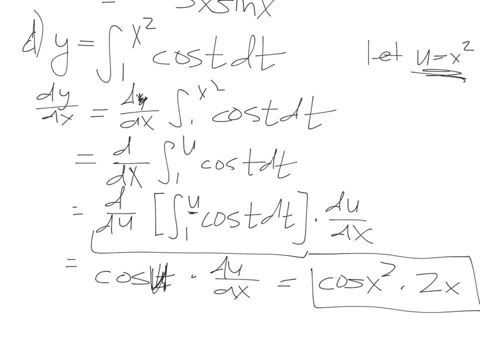 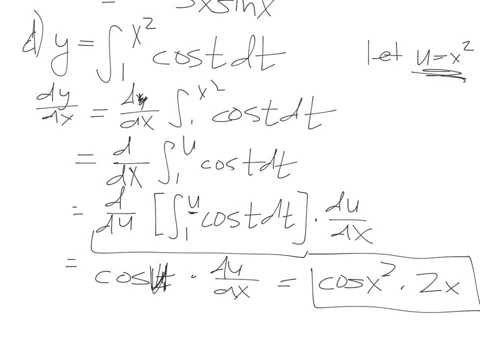 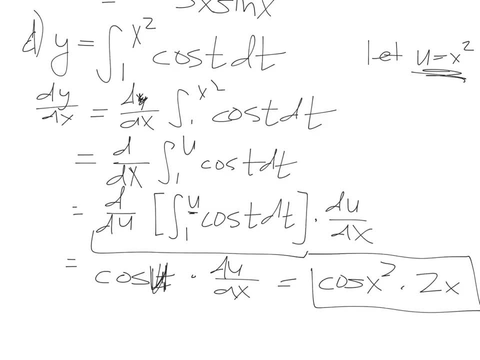 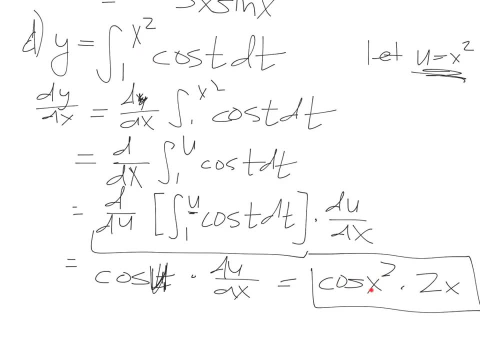 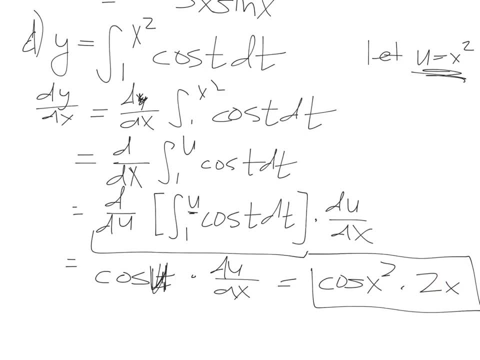 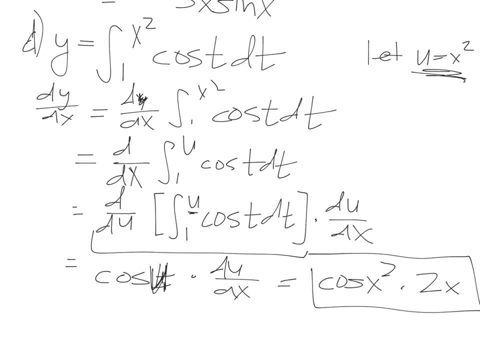 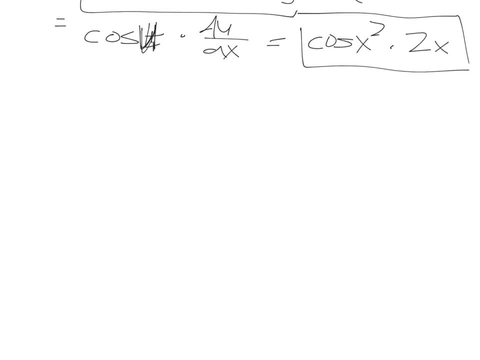 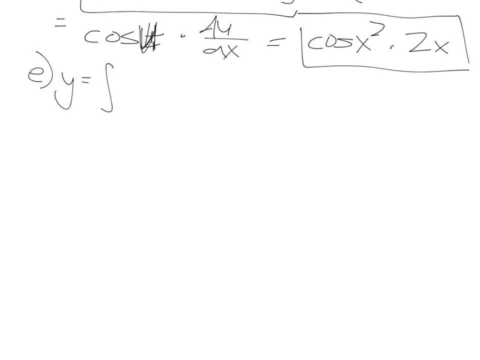 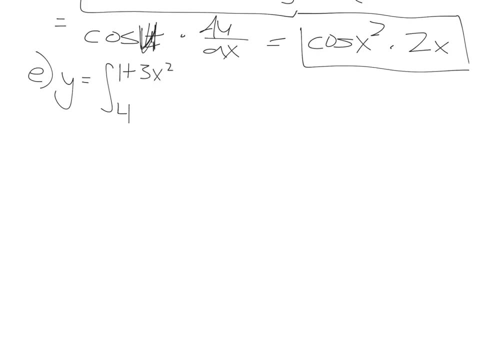 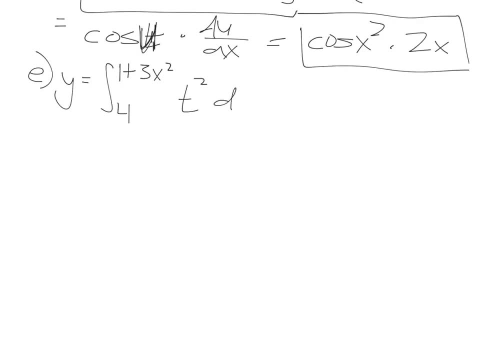 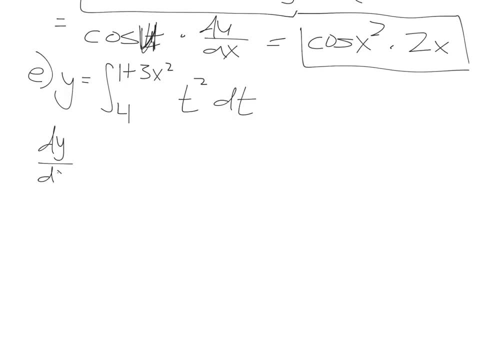 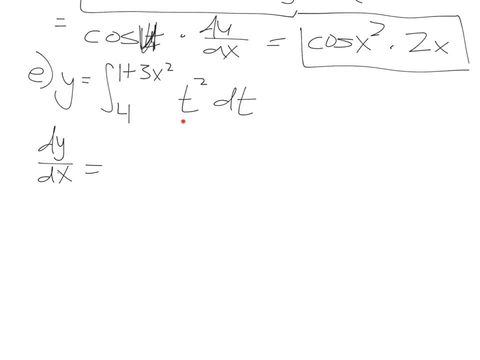 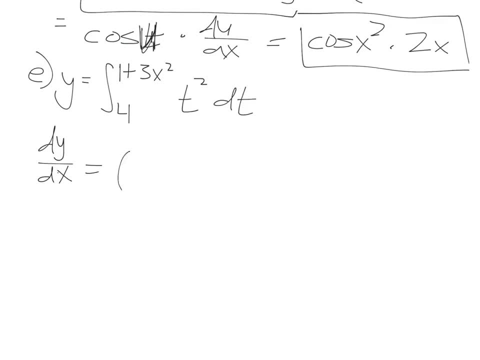 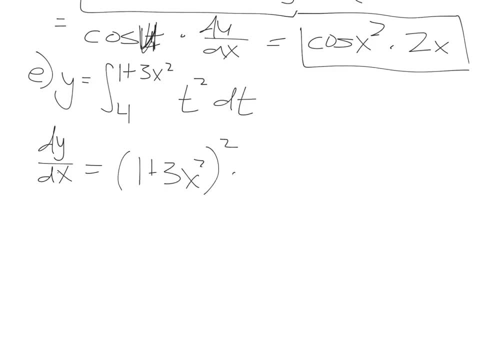 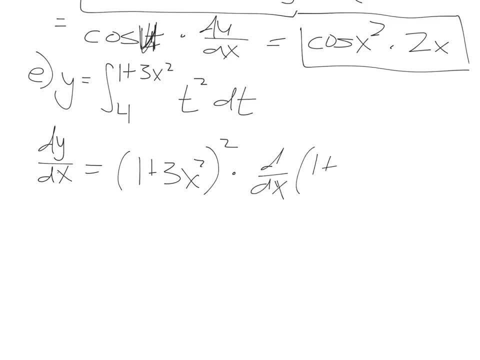 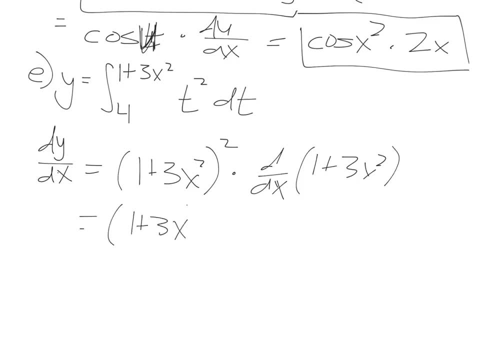 And so we get: this is one plus 3x squared quantity squared times the derivative here is 6x. And so we get: this is one plus 3x squared quantity squared times the derivative here is 6x. Now we have the second part of the Fundamental Theorem of Calculus. 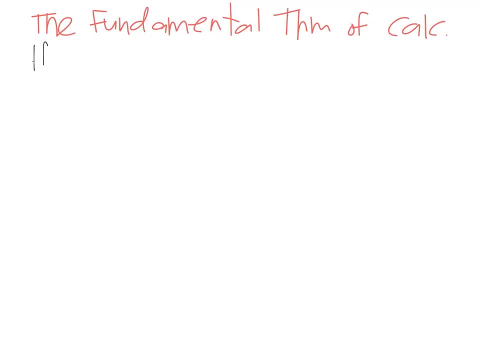 And this says the following. And this says the following: If f is continuous on the interval a to b, then the integral from a to b of f dx is equal to capital F of b minus capital F of a, where we define capital F to be any antiderivative. 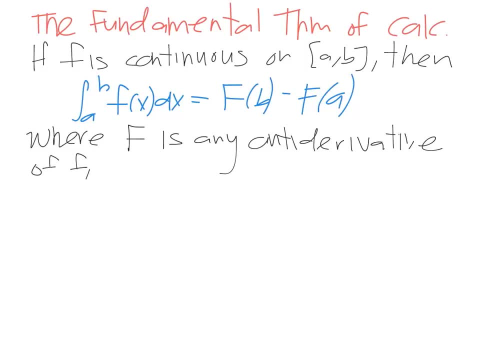 of our little f. So that is a function, capital F, such that capital F prime the derivative of that is little f. So the second part of the Fundamental Theorem of Calculus states that: 1. The integral of this is really the antiderivative at this point, minus the antiderivative at this. 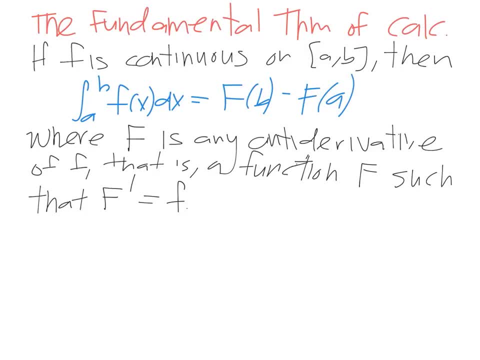 point, And sometimes, instead of writing F of b minus F of a, we'll use the shorthand notation F of x, and this means we're going to evaluate this f from a to b, And sometimes you'll see it with just a straight line, and that just means f of x is evaluated from a to b. Now 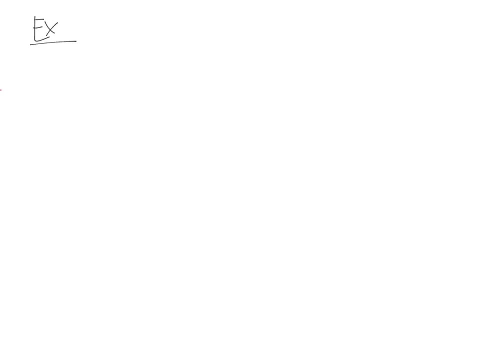 let's do some examples: The integral from 0 to pi of cosine of x, dx. Well, what is this going to be? Well, the antiderivative of cosine of x is sine of x. If you remember that the antiderivative of cosine of x is sine of x, 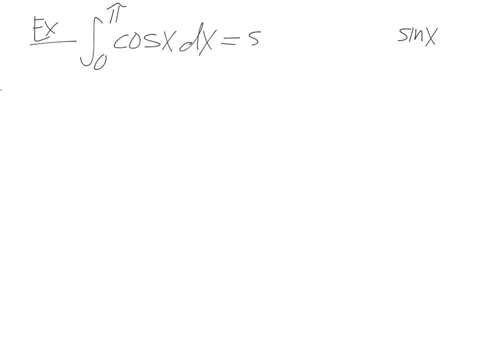 And so this is just going to be sine of x, evaluated from 0 to pi, Meaning this is going to be sine of pi minus sine of 0. Because the fundamental theorem of calculus says the integral from a to b, of f, of x, dx is the antiderivative evaluated at the second endpoint. 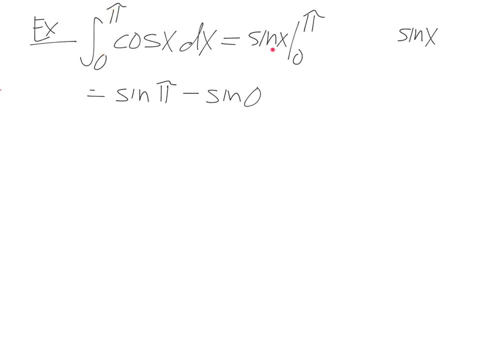 pi minus evaluated at the first endpoint. So let's do another example. So let's call this example a and we'll look at b. So now let's evaluate the integral from negative pi over 4 to 0 of secant of x times tangent of x dx. Now, if you remember the antiderivative, 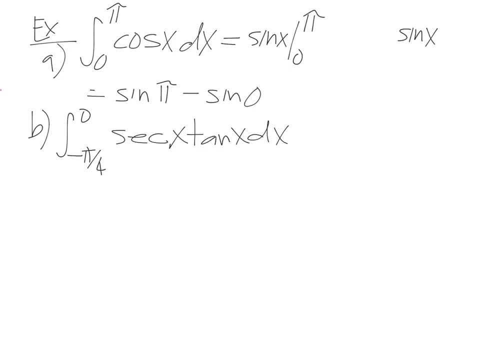 of secant times tangent of x. that's just going to be. that's just secant of x. So what we have here is this is going to be secant of x, evaluated from negative pi over 4 to 0.. And I'm sorry We didn't really finish this first one, because we know what sine of 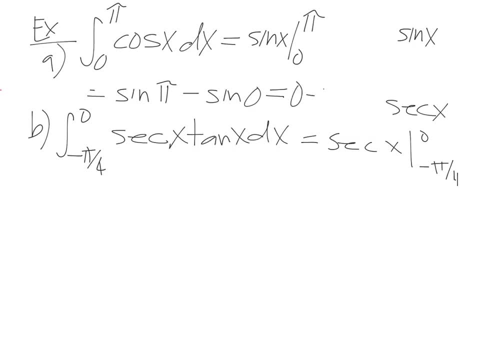 pi is, and then sine of 0 is also 0, so this is just going to be 0. and so now we evaluated this integral without actually having to compute any, any areas of rectangles and what not. so same thing here. so now this is going to be: 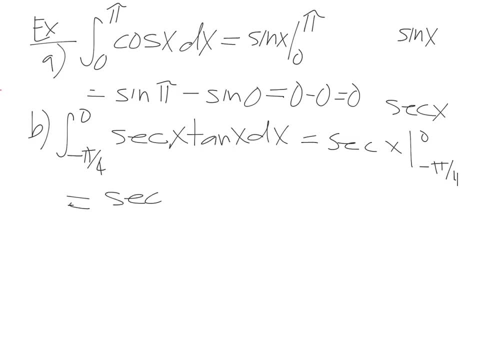 secant of, not secant of x, secant of 0 minus secant of negative pi over 4. well, secant of 0 is going to be 1 minus secant of negative pi over 4. if you remember from trigonometry, that's just root 2. 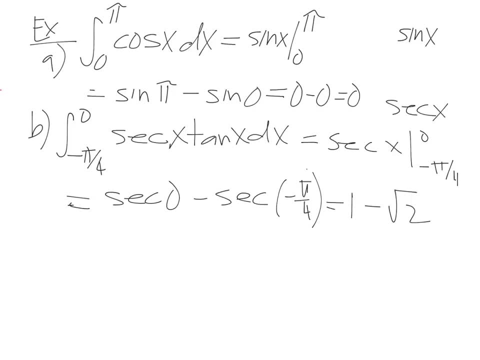 so we get 1 minus root 2. now let's do another example: evaluate the integral from 1 to 4 and we get 1 minus root 2 of the quantity 3, halves times the square root of x minus 4 over x squared dx. 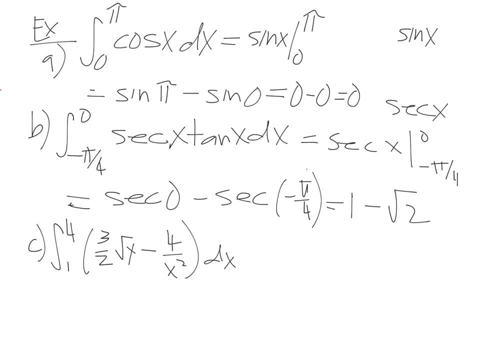 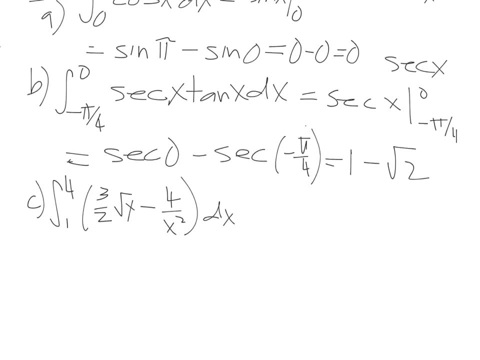 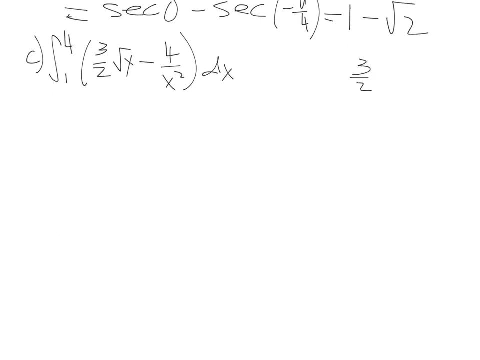 so now we need to figure out what's the antiderivative of all of this. well, let's actually give ourselves a little bit more space so we can work with right here. so what's the antiderivative of 3 halves square root of x, or 3 halves x to the 1 half power? 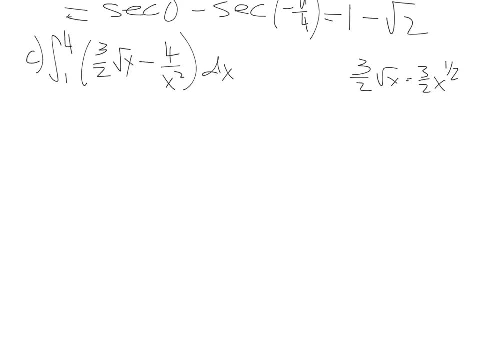 well, the antiderivative of that is x to the 3 halves. so this is just going to be x to the 3 halves minus. and what's the antiderivative? and this is our little scratch work right here: what's the antiderivative of 4 over x squared? 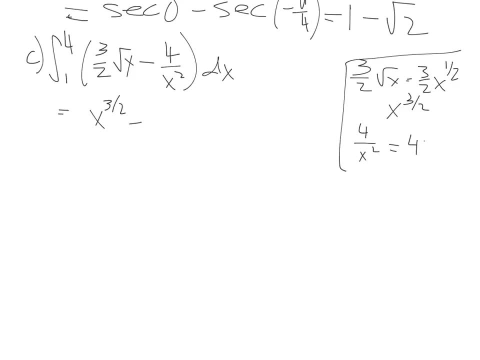 well, it might be easier if we looked at it as 4 times x to the negative pi over x squared, or x to the negative 2 power, and so the antiderivative of this is going to be negative 4 times x to the negative 1. 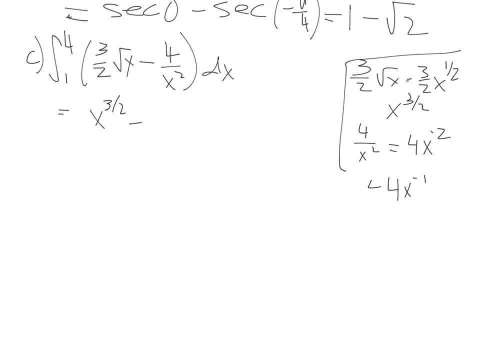 and you can double check this by taking the derivative of this term and seeing that the derivative of this term and seeing that it's equal to that one. right there. now another way of writing this is going to be negative 4 over x. x to the negative 1 is really the same as saying: 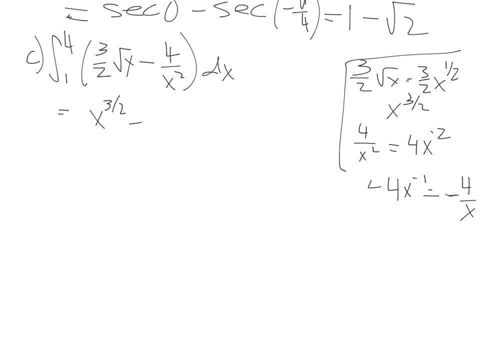 dividing by x to the 1 power. so now what we have is we're subtracting right here, subtracting the negative. so really we're going to add 4 over x and this is evaluated from 1 to 4. so, plugging this in, we're first going to go through this evaluating. 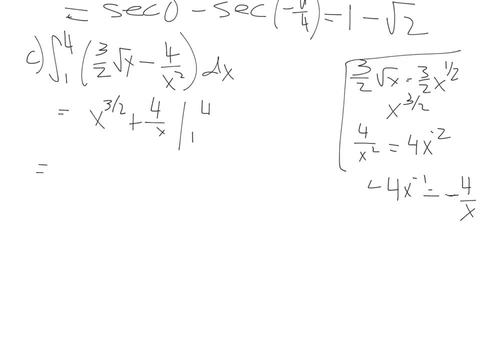 at 4, and then we're going to subtract this evaluating at 1, so, evaluated at 4, we get not x but rather 4 to the 3 halves, plus 4 over 4, and then we're going to evaluate it at 1: 1 to the 3 halves. 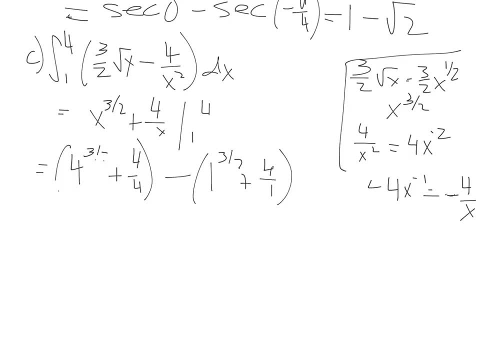 plus 4 over 1. oops, 3 halves right there, and so we get this should be 8 plus 1 minus 1 plus 4, and so this is going to be equal to 4. so now we can use the fundamental theorem of calculus. 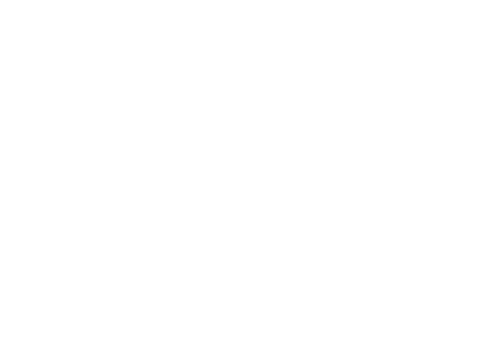 to find a lot of things if given, let's say, velocity. so if we know that v of t is the velocity of something and we also know that s of t is the position, and if we're given that the velocity is the derivative of the position, then we could calculate. 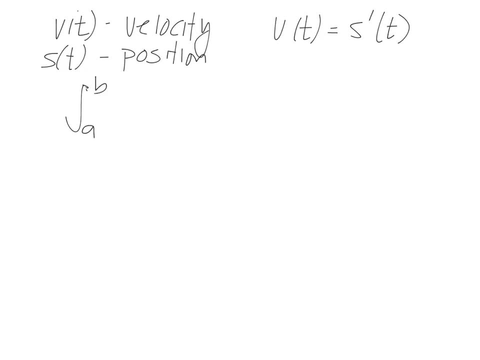 the integral of the velocity from a to b. that's going to be minus d t, that's really s of b minus s of a. this is done using the fundamental theorem of calculus. and what is this if we're subtracting our position from this end point? 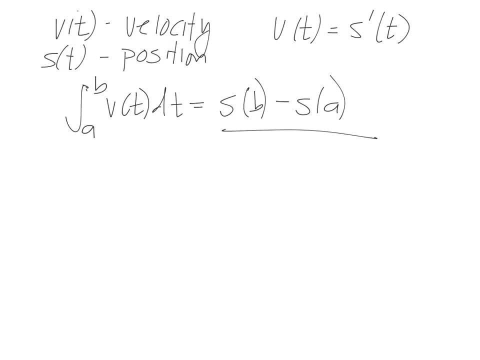 minus the position of our start point, that's the distance traveled. and so when we get this, we have to get the distance traveled. that's the distance traveled, and then we're going to get the distance traveled. So if you just need to know what's the distance you traveled, you just take the fundamental. 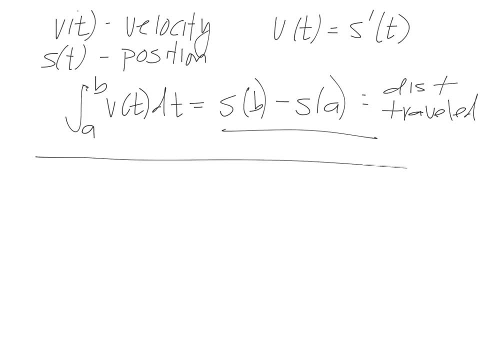 theorem of calculus, of this antiderivative or of this integral. We could also use this in applying, say, finding the area under a curve. So find the area under the parabola, and this is y is equal to x squared from 0 to 1.. 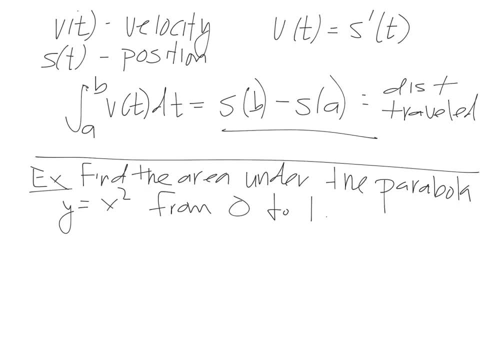 So the solution to this is going to be well, if our f of x is equal to x squared, then because x squared, what's the antiderivative? What would capital F of x be? Well, the antiderivative of x squared is 1 third x cubed. 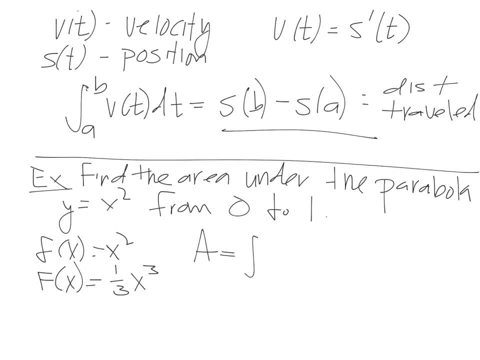 And so the area is going to be the integral from 0 to 1, because that's where we're going, from 0 to 1, of our function x squared dx. That's the area, And now, using the fundamental theorem of calculus, we're going to find the area under: 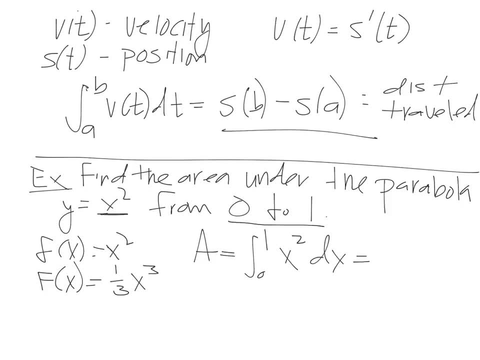 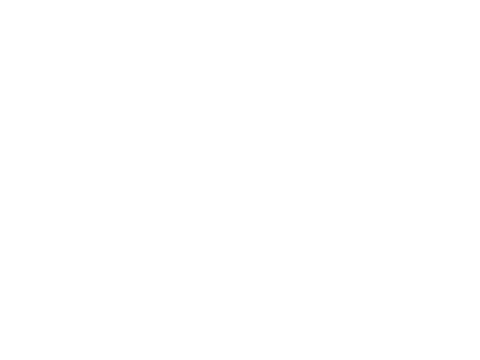 calculus. We're going to say this is the antiderivative 1 third, x cubed or x cubed over 3, evaluated from 0 to 1.. So this is going to be 1 cubed over 3 minus 0 cubed over 3, which is just 1 third. 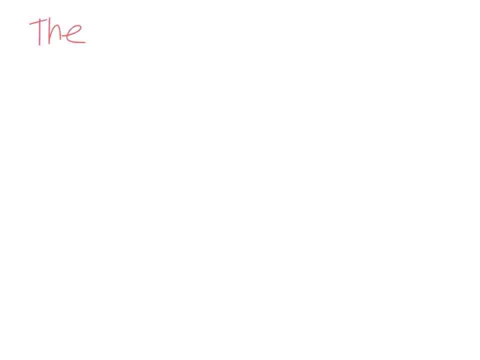 So let's just combine everything and rewrite the fundamental theorem. So for producing ну we can use is equal to 1 squared x squared, And we'll just say we're going to use a constant. so since it's 0, we're going toeffective. 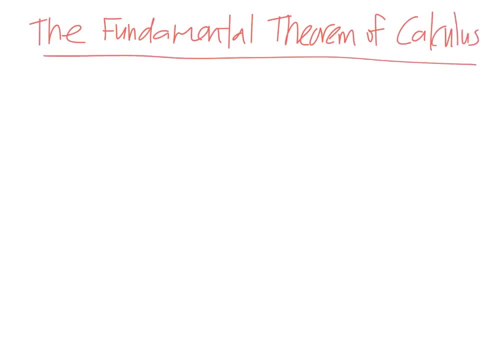 rid of f times the int convention as x squared And we're going to put our to the rest of our function. So the int convention is equal to F squared, x squared, all the way against f to the int combination in the denominator. And if we were going to give this and this in function, we might know that we're simply 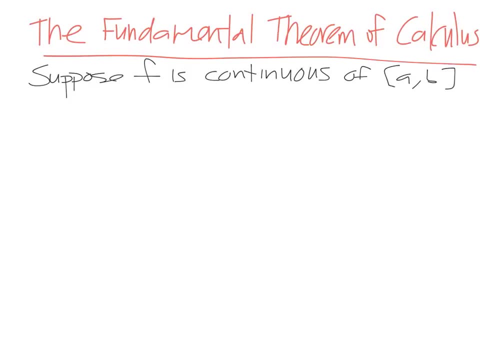 closed interval a to b, then we're going to have two things: One, if g of x is equal to the integral from a to x of f of t dt, then g prime of x is equal to f of x. And then two: the integral from a to b of f of x dx is equal to capital F of b. 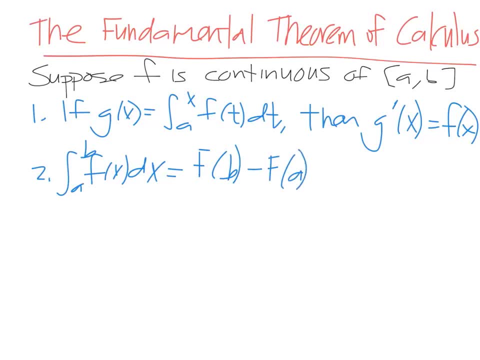 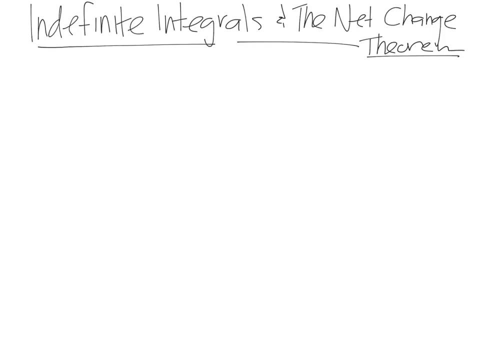 minus capital F of a, And this is going to be where capital F is. any anti-derivative of little f, That is, capital F, is equal to little f. Today we're going to talk about indefinite integrals and the net change theorem. 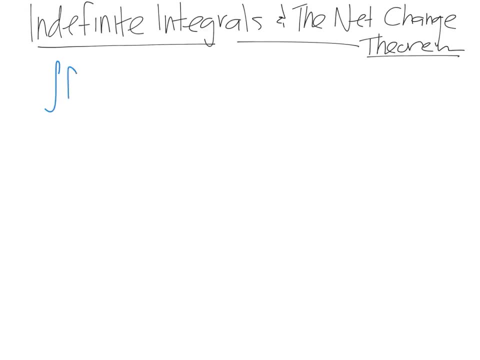 Now the notation: if you write the integral of f of x- dx, this is traditionally used for an anti-derivative of f, And if you write the integral of f of x- dx, this is traditionally used for an anti-derivative of f, And what this is called is the indefinite integral. And so if we wrote the indefinite, 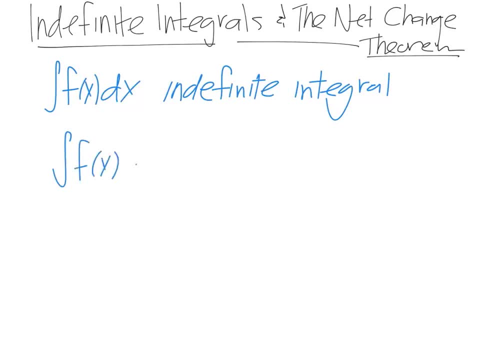 integral and we said this is equal to capital F of x. this means that the derivative of capital F of x- dx is equal to capital F of x- dx, And so if we wrote the indefinite integral, we'll see how much capital F of x is equal to capital F of x- x- dx. 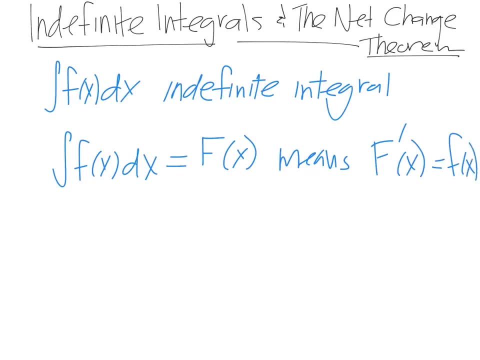 Now again, if you write the integral of f of x, dx and this is used to get into the interval right in, and then the integral won't be equal to x, which we get, and the integral f is equal to capital. F of x, dx isn't equal to. 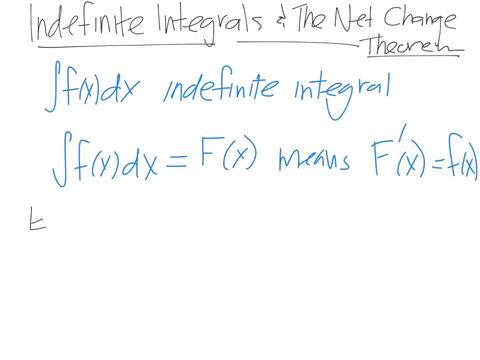 x And I'm going to write here capital F of x, So f of x, the indefinite integral of x squared dx. who are the variably X squared is x cubed over 3. it's X squared over 3 plus c. 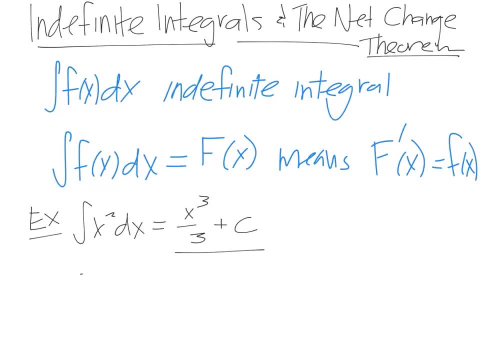 So if we took the derivative of x squared dx and we thought we're supposed to write you took the derivative of x cubed over 3 plus C. well, the derivative of x cubed is 3x squared over 3, and the derivative of C? well, C is a constant, so the 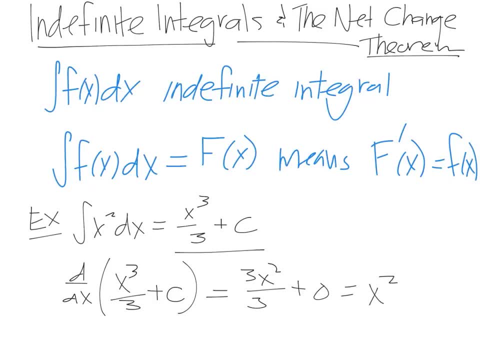 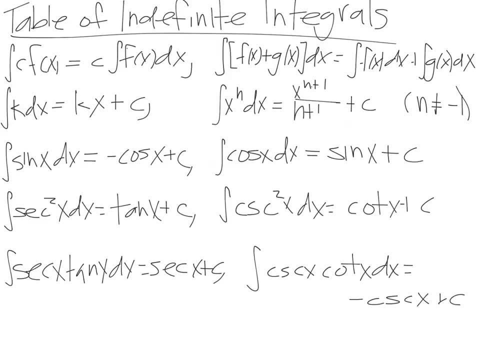 derivative constant is 0. so this is just x squared, which was that function on the inside. now let's take a look at this table of indefinite integrals. so the integral, the indefinite integral of some constant C times f, of X, DX, is you just pull this, the constant, out, and that's. 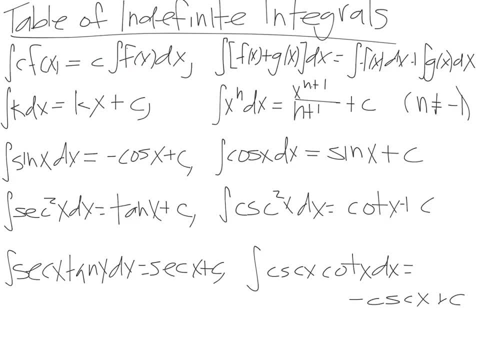 just C times the integral of f of X DX. same thing. if we're adding two functions, the indefinite integral of f plus G of X DX becomes the indefinite integral of F of X DX. the indefinite integral of of g of x dx, the indefinite integral of just a constant k times dx is going to be kx plus c. 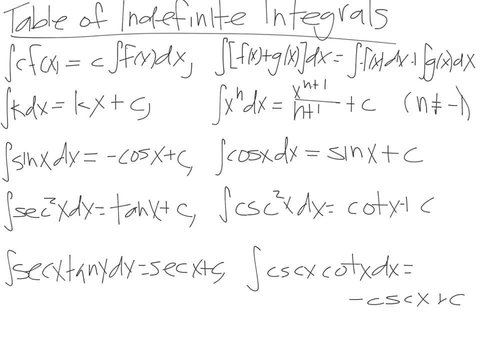 remember, when we take the indefinite integral, we would be adding a, an integrating constant c. the indefinite integral of x to the n becomes x to the n plus 1, over n plus 1, again plus c, the indefinite integral of sine of x. well, the antiderivative of sine is negative cosine. 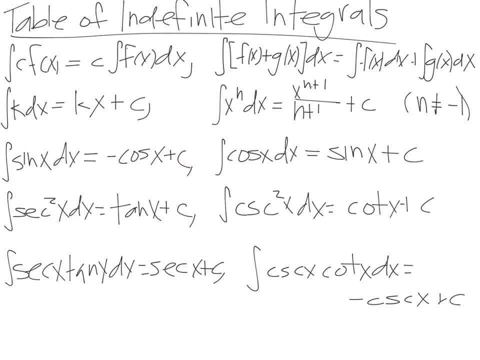 plus c. of course the indefinite integral of cosine is going to be sine, since the antiderivative of cosine is sine. and then we again add plus c. the indefinite integral of secant squared of x, dx, becomes tangent of x plus c. the indefinite integral of cosecant squared of x is cotangent plus c and the indefinite 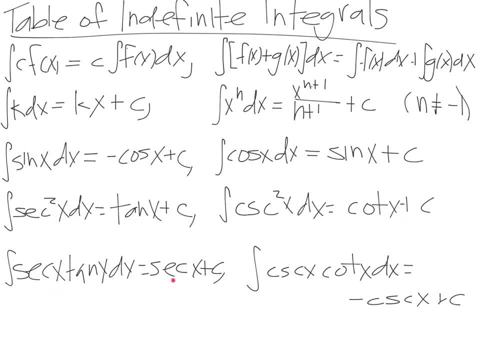 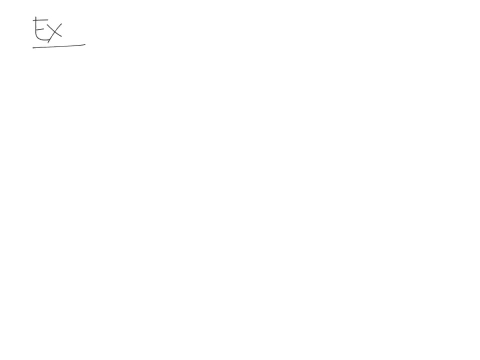 integral of secant of x times tangent of x is secant of x plus c. and then finally, the indefinite integral of cosecant of x times cotangent of x is negative cosecant of x plus c. so let's do some examples. find the general indefinite integral of: 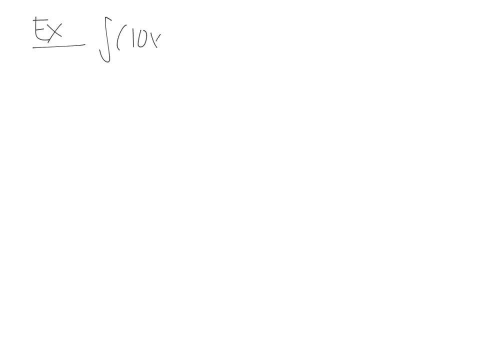 10 x to the 4 minus 2 times secant squared of x- dx. so you can just use this and you're going to be able to solve theerweisequaire of x- dx, x, 65 plus c Using that table. we have two different things, so we can break it up into two integrals. we're subtracting. 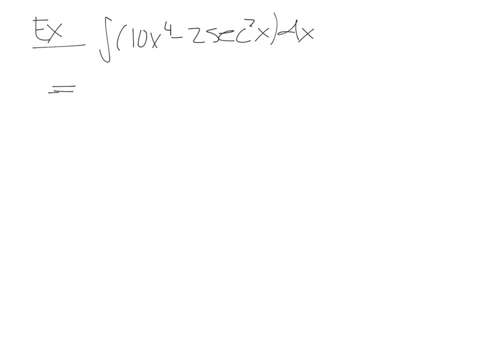 And then also we have a constant in front, so we can pull these constants in front, This 10 and this 2.. So we get first off: we get 10 times the integral of x to the 4 dx, minus 2 times the integral secant squared x- dx. 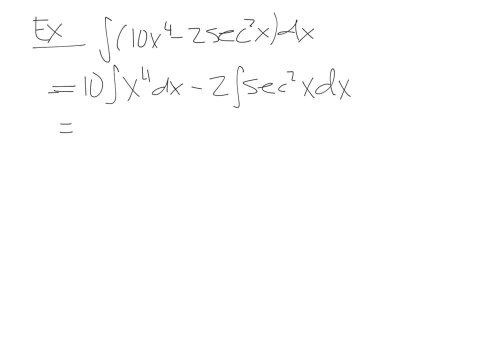 So this becomes the integral of x to the 4.. The 4 dx becomes x to the 5th over 5.. And so if we were to add the plus c over here, we'll call it a c1 minus, And then we have 2 times. 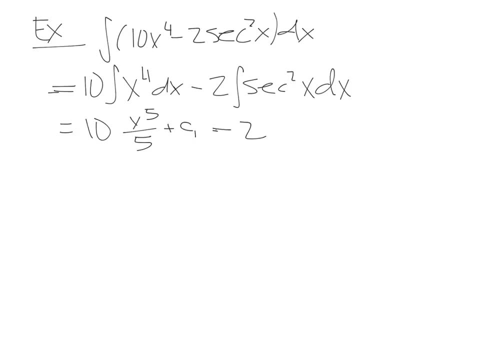 And then the antiderivative or the indefinite integral of secant squared of x dx becomes tangent of x Plus. we'll call this a c2. But we have a constant and we have plus another constant. So really what we can just do is just write it as one big constant. 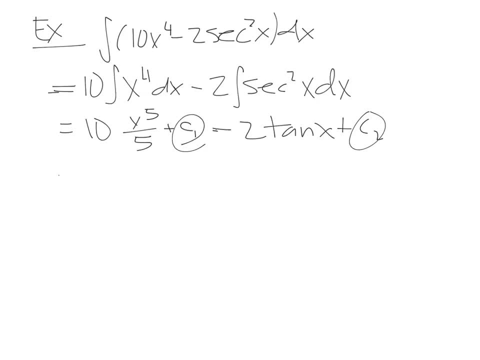 Because it doesn't really matter as long as it's a constant. So simplifying this: 10 over 5 gives you 2x to the 5th minus 2 tangent of x, And then we just call it plus c, So really you don't need to add a c. 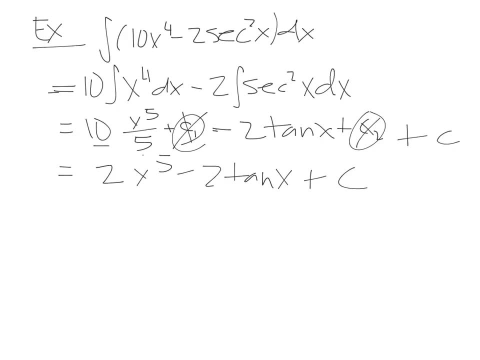 1 and a c2. here We could have just said plus c. Now if we do another example and we take the integral from 0 to 3 of x cubed minus 6x dx, This is a definite integral. 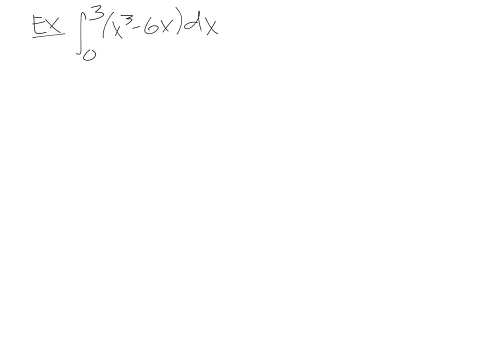 And so we're going to use the fundamental theorem of calculus as well as a table earlier in this video. This equals: and now we have two things, And then we look at each one: x to the 3rd and 6 times x. 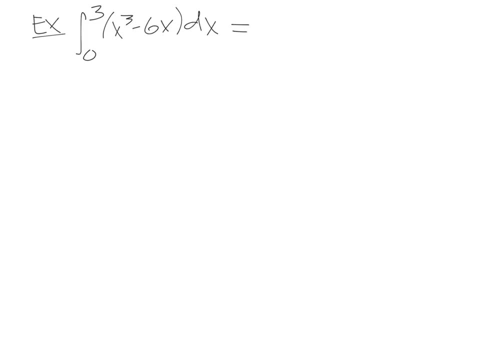 And so what we get is the x to the 3rd becomes x to the 4th over 4 minus, and then 6x is 6 times, and then x is x squared over 2.. And then this is all going to be evaluated from 0 to 3.. 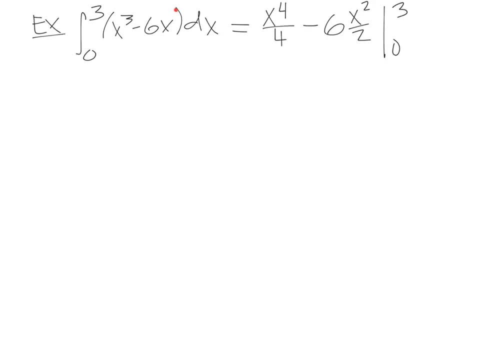 Okay. so again, we took this and split it up into two things: x to the 3rd becomes x to the 4th plus 4.. 6x is 6 times x squared over 2. And we don't have a plus c, because it's a definite integral. 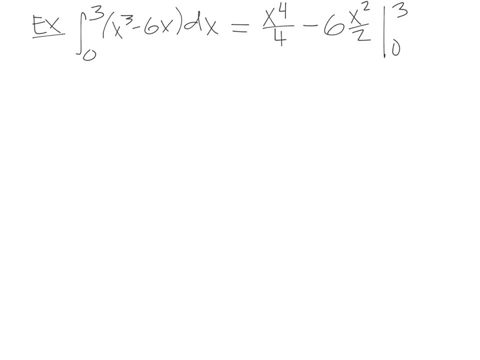 So we know exactly the values 3 and 0, the bounds. So this becomes 3 to the 4 over 4 minus 6.. Well, 6 over 2 is really this? 6 over 2 really should just be a 3x squared. 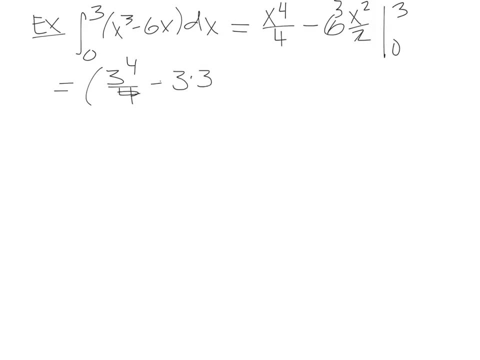 So minus 3 times 3, squared minus, and then we get 0 to the 4th, So we get 8 times 4 over 4, minus 3 times 0 squared. So we're left with it's going to be 81 over 4 minus 27.. 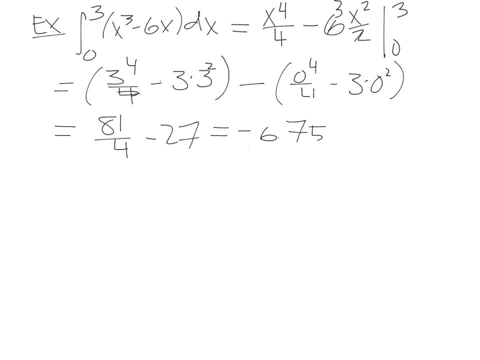 And well, that's just 6.75.. Now if we did another example and we were to find the integral from 0 to 12.. Of x minus 12 times sine of x, dx, what we get here is, well, the integral of x gives you x squared over 2. 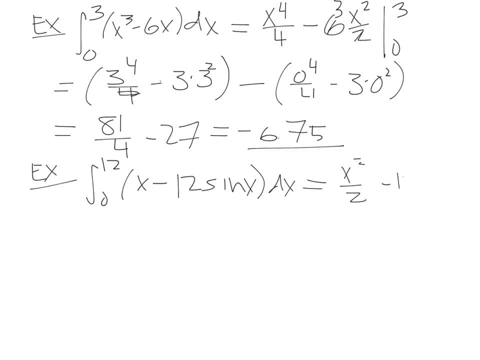 minus 12 times the integral of sine of x. well, the integral of sine of x is going to be negative cosine of x, and then this is going to be evaluated from 0 to 12. so what we get is the following: we get 12 squared over 2 minus 12 times cosine or negative cosine. 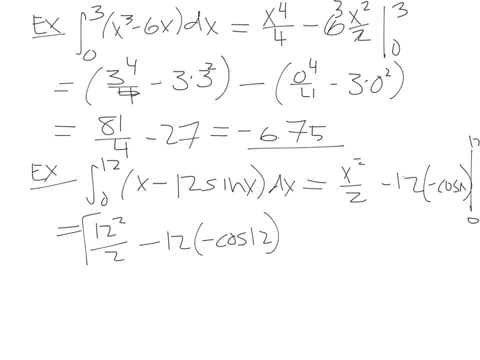 of 12 minus 0 squared over 2 minus 12 times negative cosine of 0, and I guess these minus negatives can cancel and they can just be become a plus cosine of 0. well, that's just 1, so this becomes 12 squared over 2. we get 72 plus 12 times cosine of 12, and then we get minus. well, 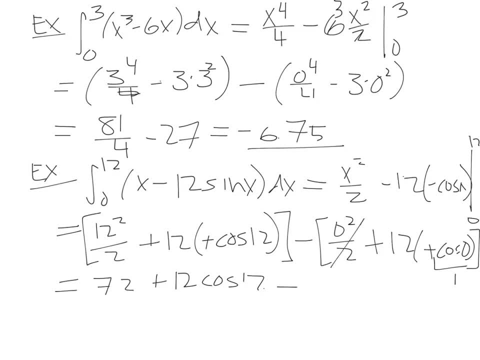 that's just 0, that cancels out, and so we get minus 12, and so we're left with 60 plus 12 times cosine of 12, so this becomes 12 squared over 2. we get 72 plus 12 times cosine of 12, and then we get: 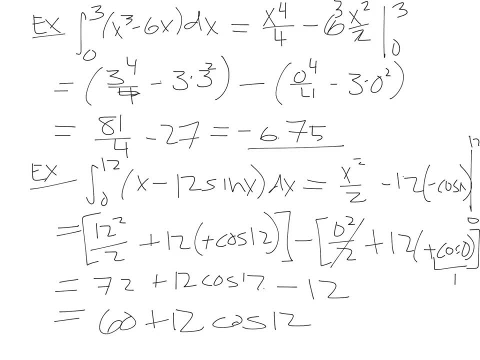 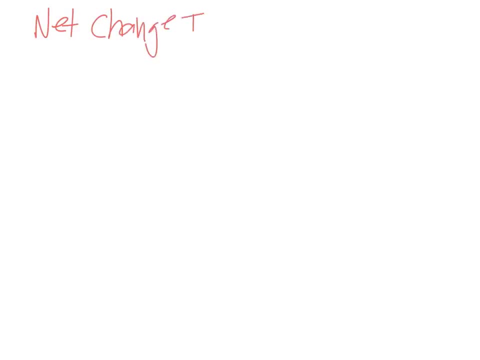 cosine of 12. the last thing we're going to do today is something called the net change theorem, and this says that the integral of a rate of change is the net change of meaning, the integral from a to b of f, prime of x, dx, and this is f of b minus f of a. 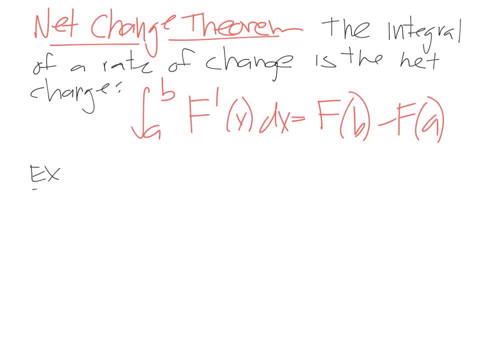 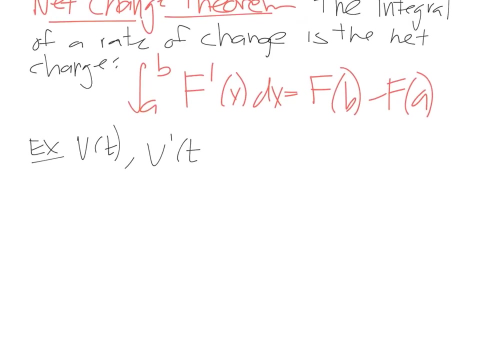 and so an example of this might be: if we're dealing with the volume in a tank with respect to some time t and we say that vt, vt is the volume coming in or it's the rate that water moves in, water flows in then the change in amount of water. 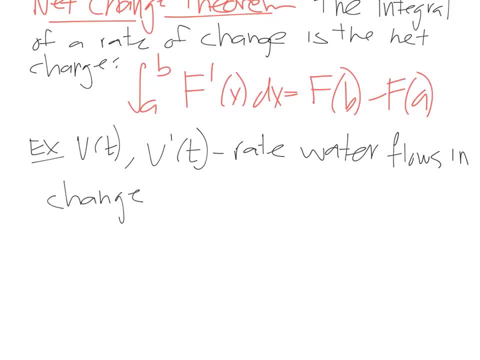 of water in the tank is going to be the integral, from some time 1 to time 2, of the derivative of v dt, and that's really just vt – v. this works for a bunch of different things. for example, if we have velocity versus position, the change in position s of t 2 minus s of t 2, which means that we're responsible. for more of the change of Russian velocity and in that sense it looks like we have K- cooling possible because it contains a lot of water. but when we say a constant an our temperature, blah, blah, blah, blah, blah, blah, blah. that way the long crossed scale is used up for the number of Bi44?. then to the K- coordinate range: 4wwww, 35villeb0?, süol&m clos, pm22?, sab2 and sto2?. question 7: please don't forget it. 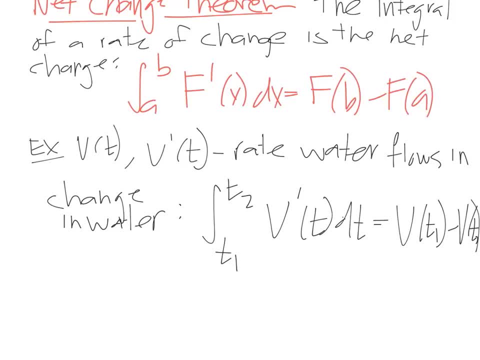 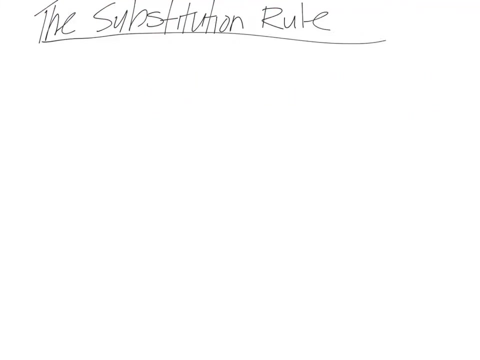 T1 is just the integral of the velocity. Today we're going to talk about the substitution rule. Now, because of the fundamental theorem of calculus, it's important to know the antiderivatives. But sometimes the antiderivatives we don't really know. 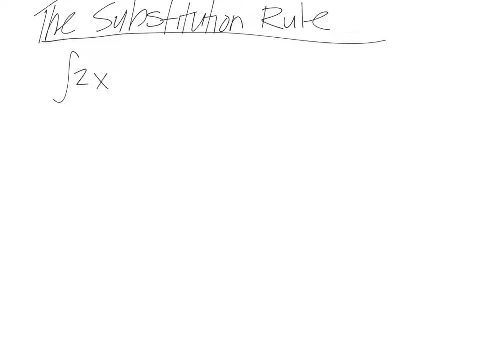 For example, if we have the integral of 2x times the square root of 1, plus x squared dx, what's the antiderivative of this? Well, we don't know that antiderivative just yet, but we can look at this and look at. 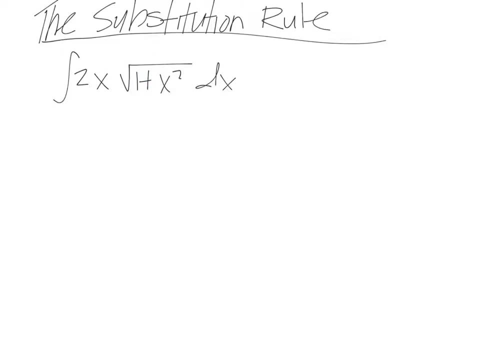 this 2x and then this square root of 1 plus x squared and we can make a little substitution. What if we introduce this new variable u, and let u be what's inside the square root of 1 plus x squared? 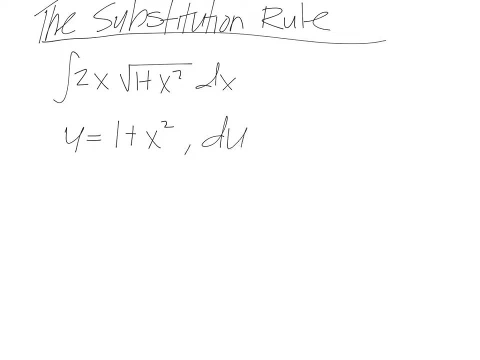 Well, what's the derivative of u? du is going to be 2x times dx, And so this original integral. I'm going to move it down here. if I rearranged it and I moved this 2x After the square root, we get the integral of the square root of 1 plus x squared times. 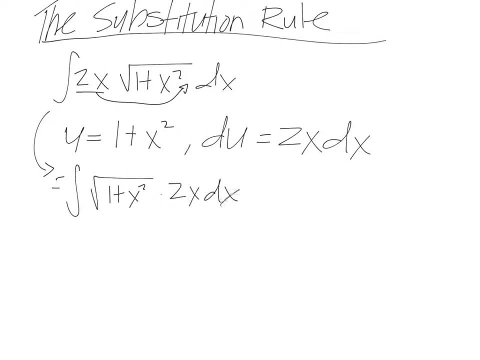 2x dx, and now we can make some substitutions. This is the integral, the square root of 1 plus x squared – well, we know, 1 plus x squared from right, here is going to be u – and then 2x d x, right here is du. 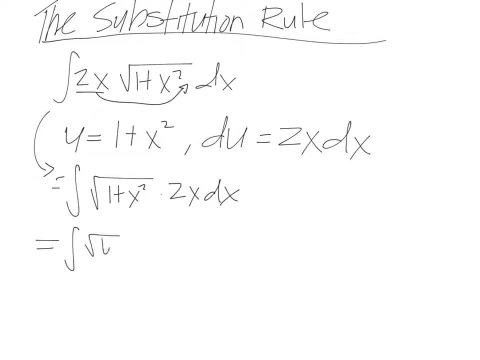 So this becomes the square root of u times du Or, if you prefer as an exponent, u to the one half du. And now we know what this antiderivative is. The antiderivative of this is two thirds u to the three halves plus c. 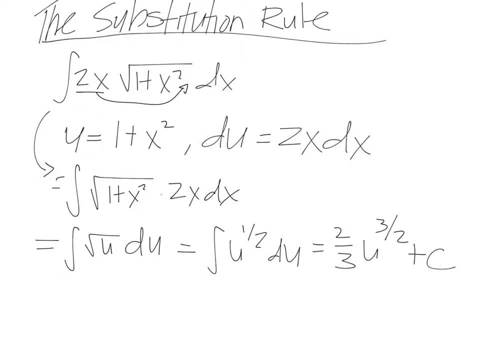 But remember u, we made that substitution. we defined u to be one plus x squared, So really putting it back into x because our original actually, I'll just write it up here. So this is going to be two thirds u times du. 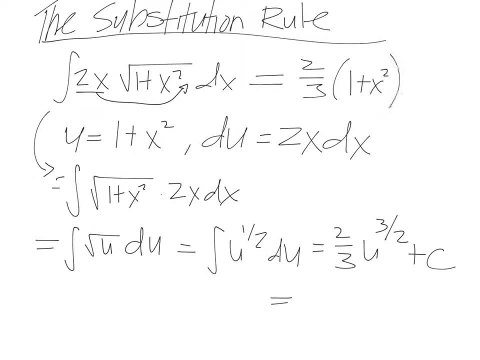 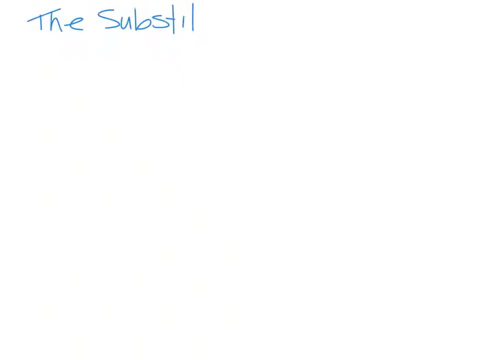 u was one plus x, squared raised to the three halves plus c. That is our answer. So this method that we did right here is using substitution. So we have something called the substitution rule And this says that if u is equal to some, g of x is a differentiable function. 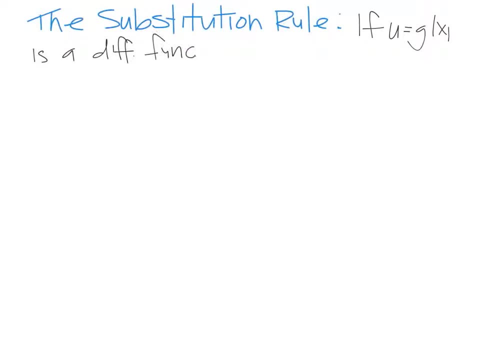 Whose range is an interval. I'm going to write this into a problem. So u times g of x, This is going to be one plus x squared. So we're going to write this down: This is going to be one plus x squared. 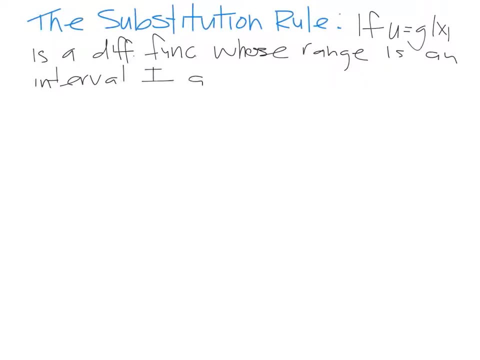 We'll say this interval, call it i, and f is continuous on i. Okay, then the integral of f of g of x times g, prime of x, dx, is equal to the integral of f of u du. So basically, what this is saying is, if we're taking the integral of some function, f, that of some variable times, the derivative of that, 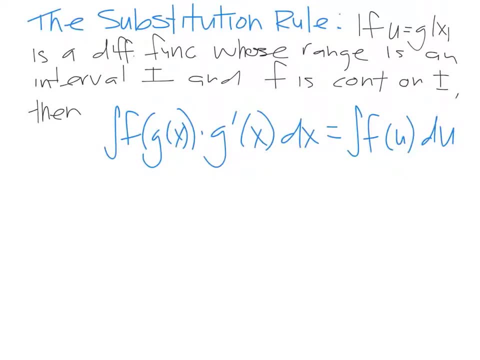 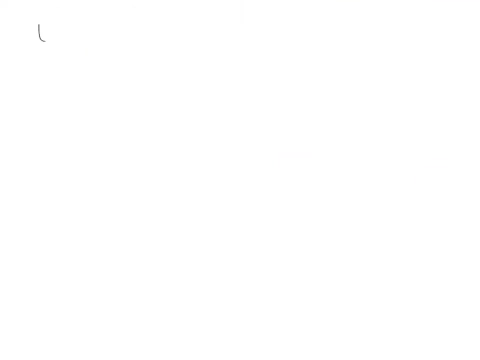 that could be written as the integral of f of u, du. So instead of writing it as g of x, we're writing it as u, And this all becomes that. So let's do Example. Let's evaluate the integral of x squared times. cosine of x, cubed dx. 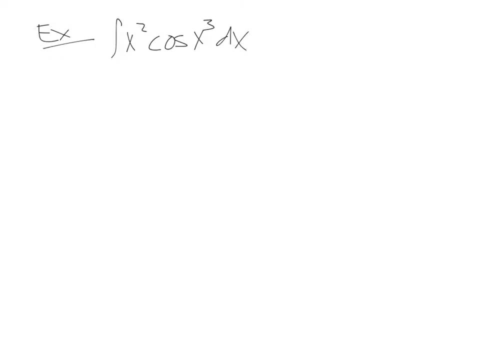 If we rewrote this and we move these x squared after the cosine, so this would be the integral of cosine of x cubed times, x squared dx. Now this x cubed inside the cosine, that might be causing a little problems. So that's probably what we're going to want: to let our u equal. 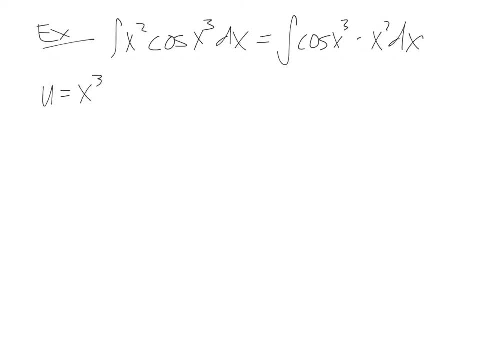 So let u be x cubed, And that means that du is going to be 3 times x, squared times dx, And so, making this Substitution, we get the integral of cosine. instead of x cubed, We're going to use u. 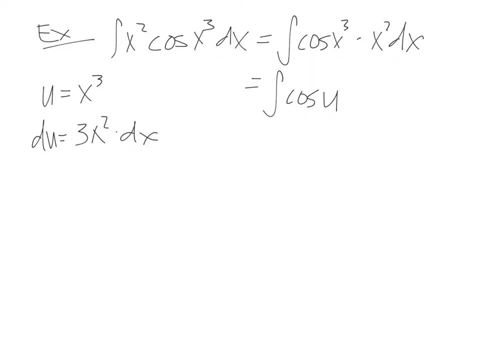 But now we run into a problem. This is x squared dx And this is not quite x squared dx. It's 3 times x squared dx. Well, how do we make it like x squared dx? We can divide both sides by 3.. 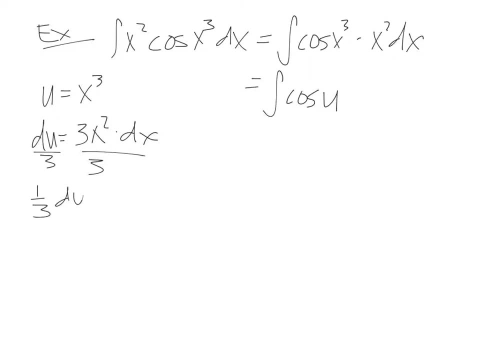 And so 1 third du is equal to x squared. So this is going to be multiplied by 1 third du. So to evaluate this, this 1 third, we can pull it in front. And so this is 1 third the integral of cosine of u du. 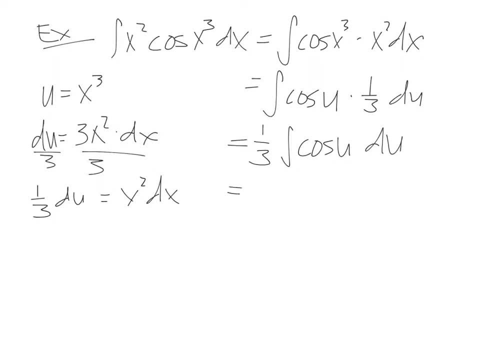 And we know this. So we get 1 third times sine of u. The antiderivative of cosine Is sine. And then we add plus c, But we're not done Because the initial problem had x's in it. we cannot leave our answer with u. 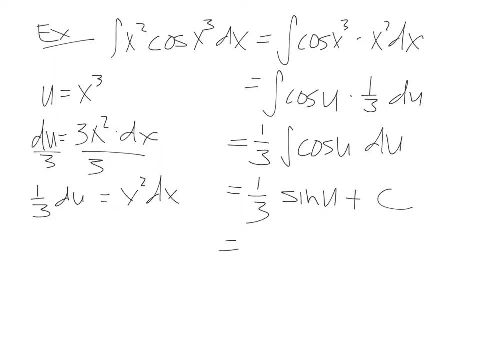 We have to always write back Or convert back. So this is going to be 1 third sine. Our u was x cubed plus c. That's our answer. Now let's do another one. Let's do another example. Let's evaluate the integral. 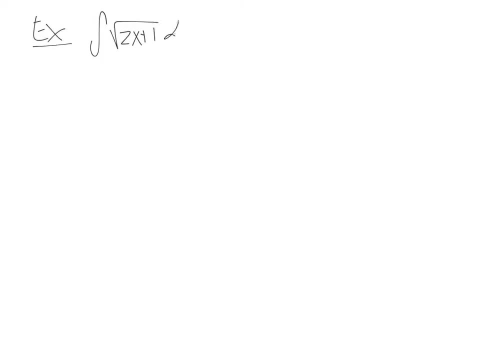 The square root of 2x plus 1 dx. So here we look inside the square root And because it has more than just x, we're going to have a problem. So that's what we're going to: let our substitution be. 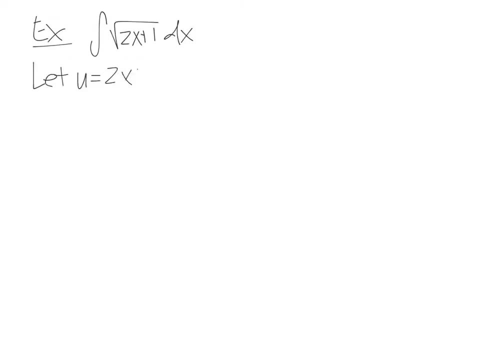 Let u equal 2x plus 1.. Then our derivative du, The derivative of 2x plus 1., Is just 2 times dx, Because the derivative of 2x is just 2.. The derivative of 1 is 0.. 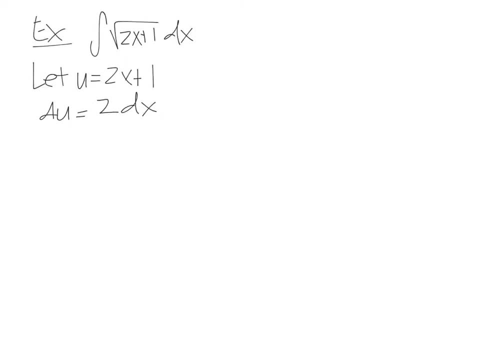 So it's just 2 and then times dx. So going ahead and making the substitution, This is the integral of the square root of u, But again we only have just dx. So to get just dx, we divide both sides By 2.. 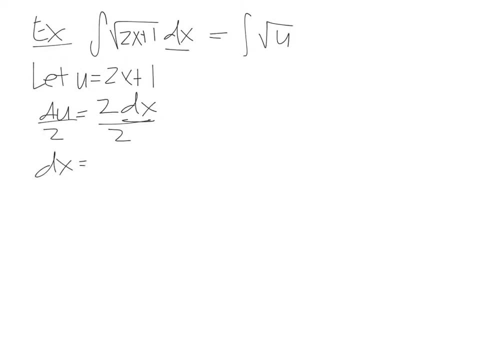 So we get 2x, And so dx is just 1 half du. So times 1 half du, So we get 1 half times the integral of square root of u, Or rather u, to the 1 half du. I'm going to write it as an exponent. 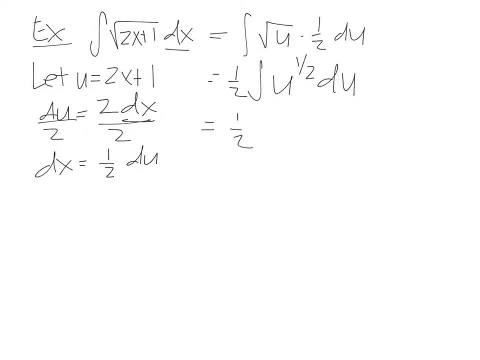 And so the antiderivative or the integral of u to the 1 half du Is going to be 2 thirds u to the 3 halves plus c, And so this becomes 1 third u to the 3 halves plus c. 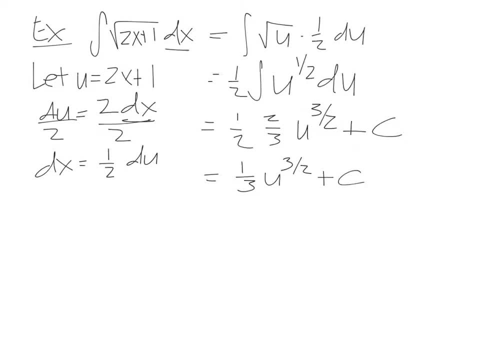 And u we said was 2x plus 1.. So this is 1, third times 2x plus 1.. All raised to the 3 halves plus c. That's your answer. Now let's do another example, But very similar. 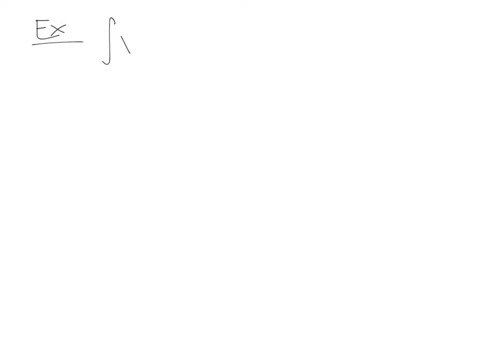 Evaluate the integral of x times the square root of 2x plus 1 dx. So this is similar to the last problem, Except now we have an x in front, So we'll make this. the substitution u is equal to 2x plus 1.. 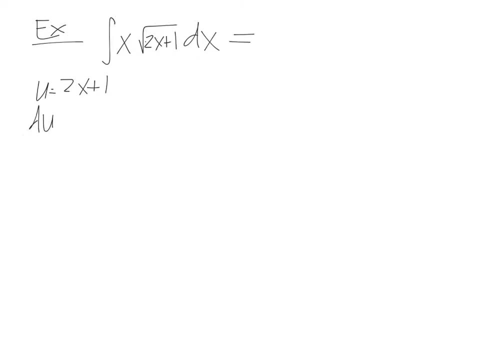 Just like we did before, And du is going to be 2 dx, Which means that our dx is really 1 half du, So this becomes the integral of- I'll leave that x for now- The square root of u times 1 half du. 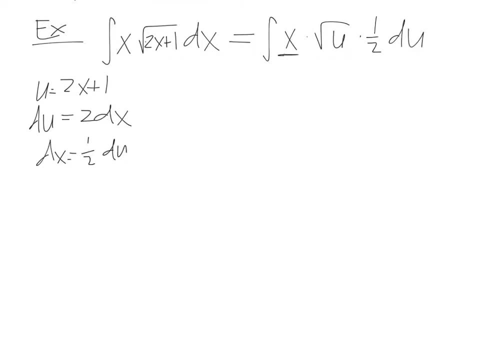 So we're stuck with this x. What can we do with this x? Well, take a look at what we said over here. u is 2x minus 1.. So if we rearrange that term, So if we rearrange this, 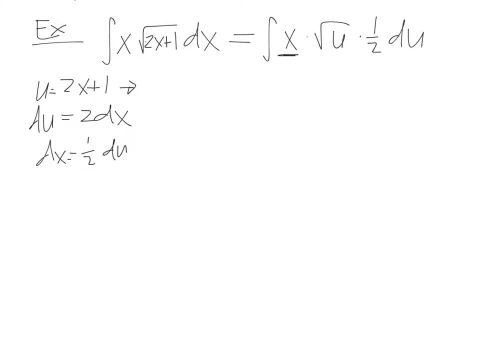 We could solve for x, And so if we subtracted 1 from both sides, We could get: u minus 1 is 2x, Or divide by 2, we get x, Which is u minus 1 over 2.. So making that substitution, 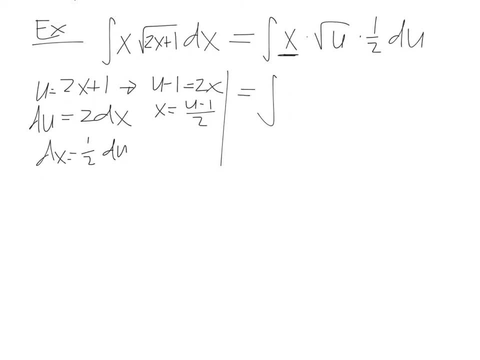 We now get the integral And rather than having it u minus 1 over 2. I'll write it as 1 half times u minus 1.. So we get 1 half u minus 1.. The square root of u is u to the 1 half. 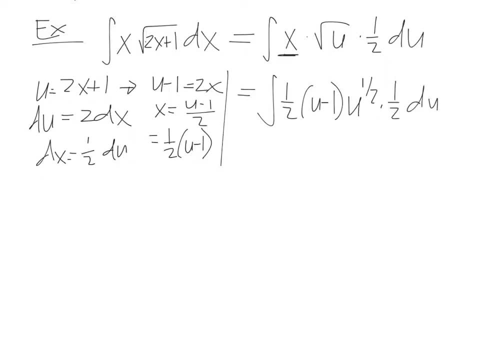 And then times 1 half du, We have 1 half and 1 half. You can pull that in front, So we'll get 1 fourth times the integral And I'm going to go ahead and just distribute this u times u to the 1 half. 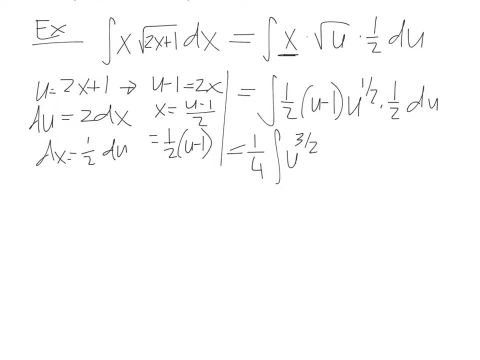 Becomes: u to the 3 halves Minus 1 times u to the 1 half is just u to the 1 half And then times du. So this is something that we'll be able to solve. So this is going to be. 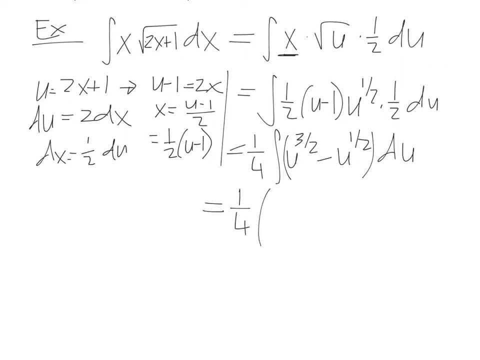 1 fourth times the antiderivative of u to the 3 halves. Well, that's going to be 2 fifths u to the 5 halves, Minus 2 thirds u to the 3 halves Plus c, And again we know that u was 2x plus 1.. 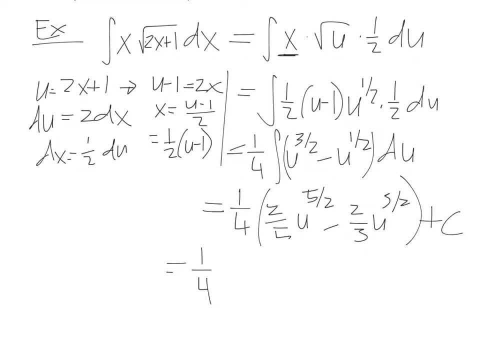 So this is going to be 1 fourth times the quantity, 2 fifths times 2x plus 1. to the 5 halves Minus 2 thirds Times 2x plus 1.. To the 3 halves: 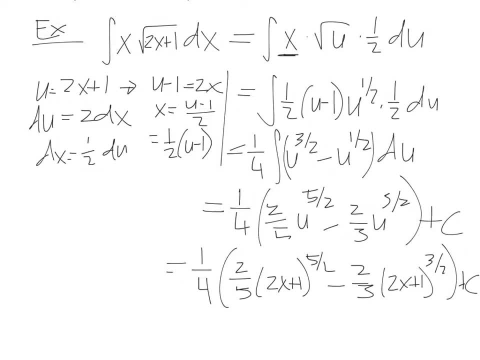 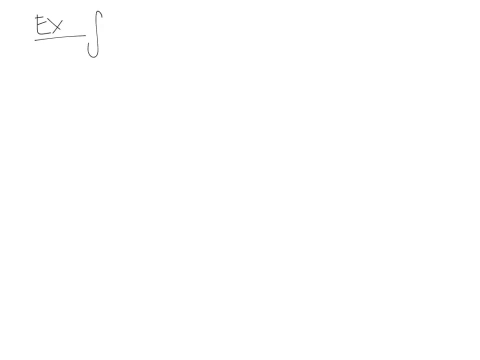 Plus c. Now let's do an example: Evaluate the integral Of cosine of 5x, dx. So we let u equal 5x, Then du is going to be 5. Dx. So this is going to be The integral. 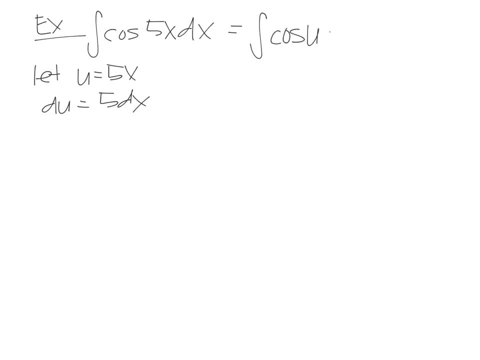 Of Cosine of u Times, And so if we just have a dx, Then We can Write: dx Is going to be 1 fifth du, So times 1 fifth du. We have 1 fifth. 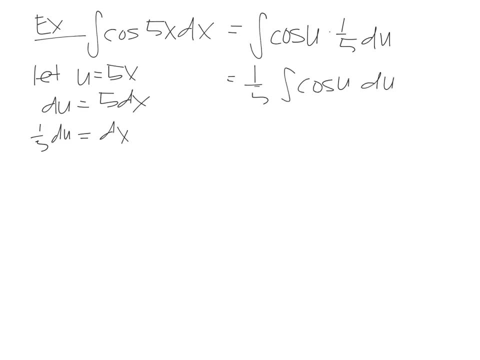 The integral Cosine of u du, Which is 1. fifth, The integral Of cosine of u du Is just Sine of u Plus C, And so Substituting u Is equal to 5x. 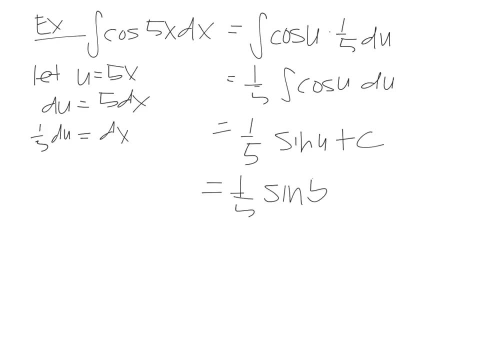 This is 1 fifth Sine Of 5x plus c. Let's do another example. Evaluate the integral Of the square root of 1 plus 1 plus x, Squared All times X to the 5th. 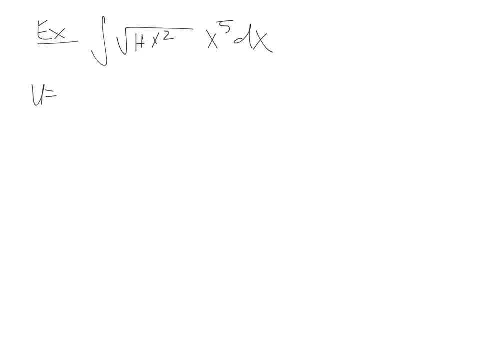 Dx. So we make u equal 1 plus x squared, Then du is 2x Dx, And so we get. This is The integral Of the square root of u, And now we have X to the 5th. 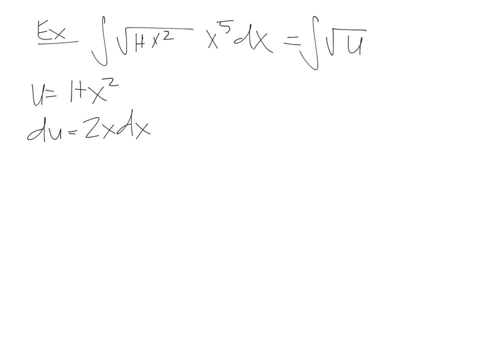 Dx. Well, Going back to this du, If we divide Both sides By u Or by 2. We get 1 half. du Is x Dx, And so X to the 5th. 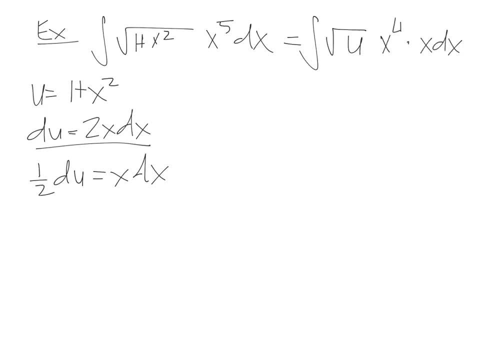 Can be rewritten as X to the 4. Times, x Dx. X to the 4. Dx Is x to the 5th, And so We get The integral Of the square root of u Times. 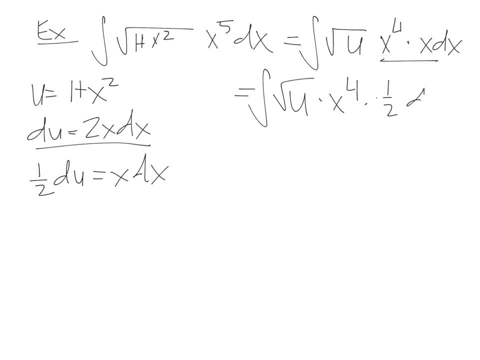 x to the 4.. x Dx Is 1 half du, But we're still left with x to the 4.. But remember That we Let u Be 1 plus x squared. So. 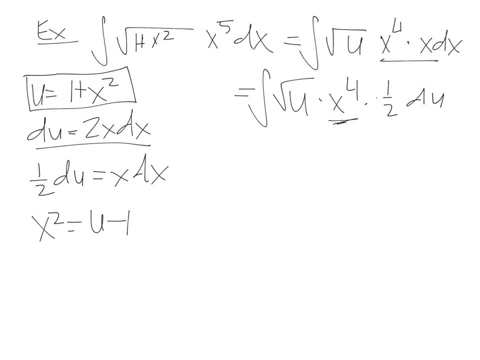 x squared Is going to be u minus 1.. We just Moved The other side. If x squared, Is u minus 1.. x to the 4. Is x squared Squared? So 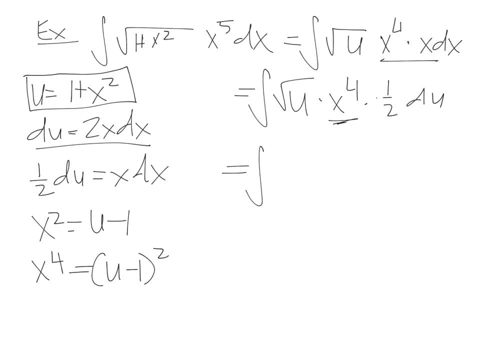 u minus 1.. Quantity Squared Is x to the 4. And so Now This Is Going To Be- And I'm Going To The Front- We Get. 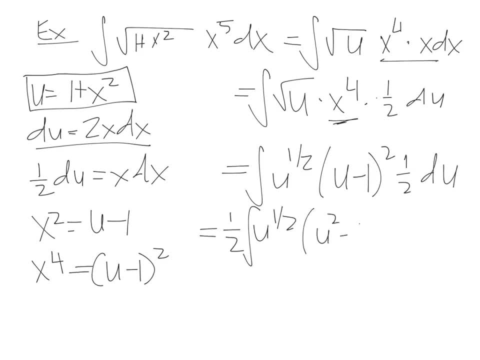 The Integral Of u to the 1 half. I'm Going To Expand u minus 1 squared. Is u squared Minus 2u Plus 1.. du This: 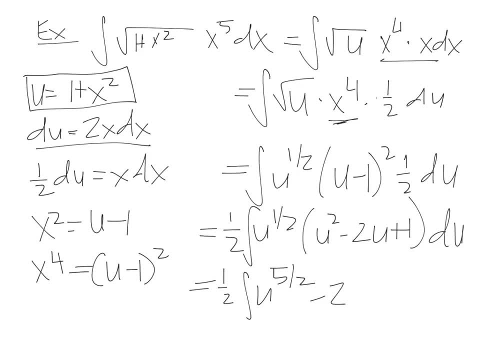 Becomes u to the 1 half Times 2. Is 3. 3 halves Plus u to the 1 half du, And So Now We Can Actually Start. 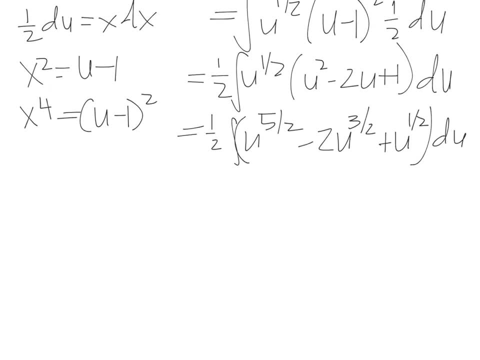 Taking The Anti Derivative Or Integrating. So This Is 1 half Times. This Is Going To 2. 7ths U To The 7 halves. 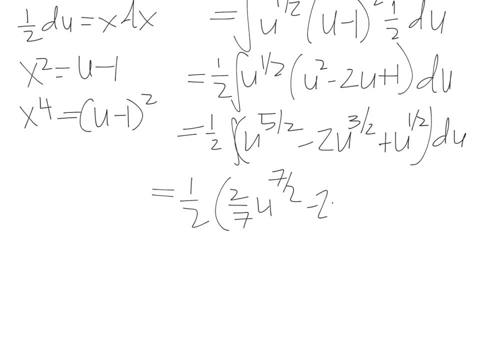 Minus 2. Times: 2. 5ths U To The 5 halves, Plus 2 thirds U To The 3 halves, All Plus C And So 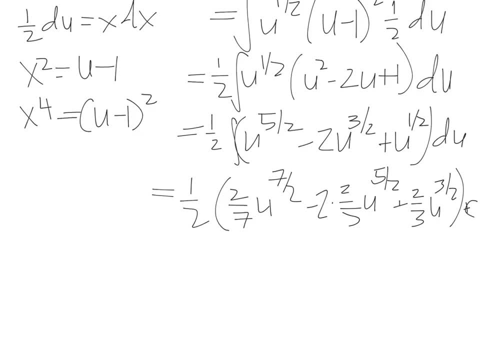 Writing This Out, Remember U Was Up Here, Got To Go Back Up A Little Bit. U Is 1. Plus X Squared, So This Is: 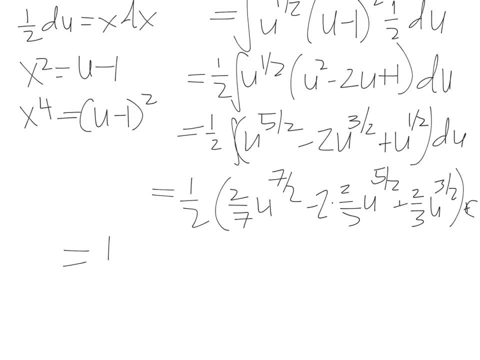 Going To Times 2. 7ths Is Going To Be In Fact. This: 1. Half Will Cancel That. 2. Cancels This: 2. And 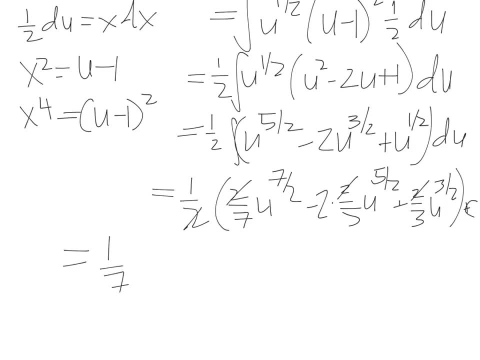 It Cancels This 2., So That Be 1. 7ths. This 2. Is Equal To 1. Plus X Squared, So 1. Plus. 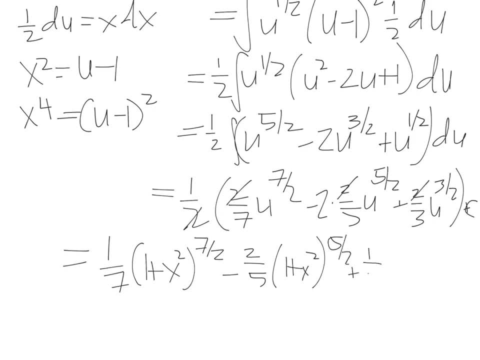 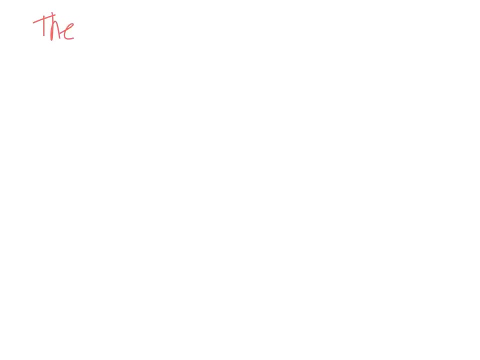 X Squared Raised To The 7. Halfs Minus 2. 5ths 1. Plus X Squared Raised To The 5. Halfs, This: 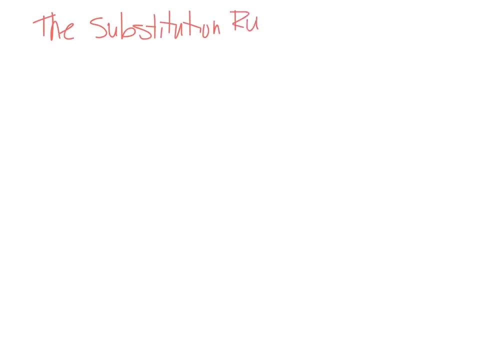 Time In The ícia As A оде The De S For The Definite Integrals. This Says The Following: If G Prime Is Continuous On, 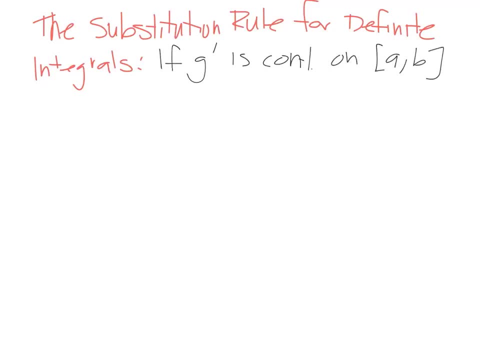 A To B. This and f is continuous on the range of u equaling g of X. then the integral from a to b, of f, of g, of x times g, prime of x, dx, is equal to the integral. and now here's where we're going to. 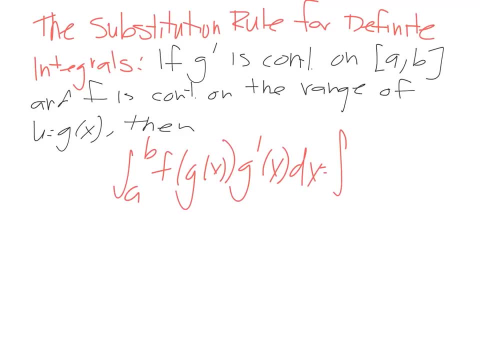 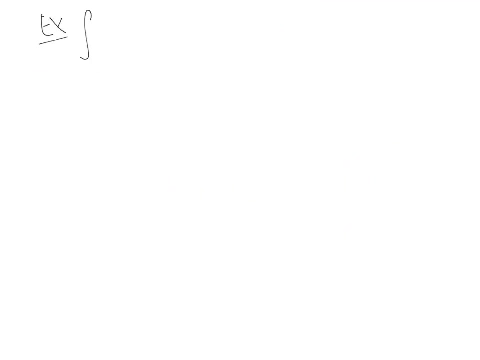 make a change. if we're going to be changing from to u, our bounds from a to b also have to change. so our a, instead of going from a, it's going to go from g of a. instead of going to b, it goes to g of b, and then we have f of u, du. so we'll do an example. evaluate the integral from 0 to 4 of the square. 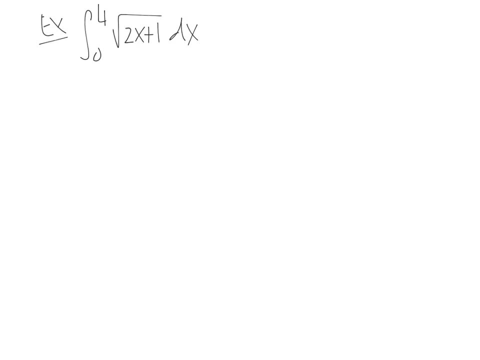 root of 2x plus 1 DX. so we're going to make the substitution, we're going to let u equal 2x plus 1 and du is equal to 2 DX. and then now, when we had initially that X was going from 0 and X went to 4, what we're going to do is we're going to plug in those values into our u. 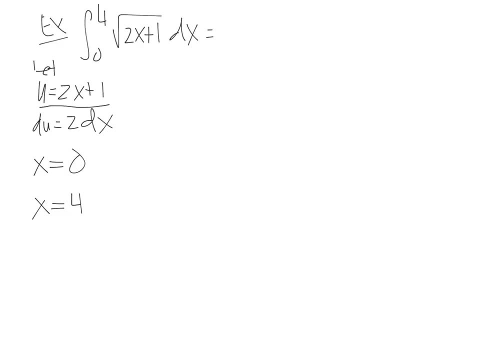 so if it went from 0, the new value is going to go 2 times 0 plus 1, which is equal to 1, and then it would go to 2 times 4 plus 1, which would be 9. so instead of going from 0 to 4, that goes from 0 to. 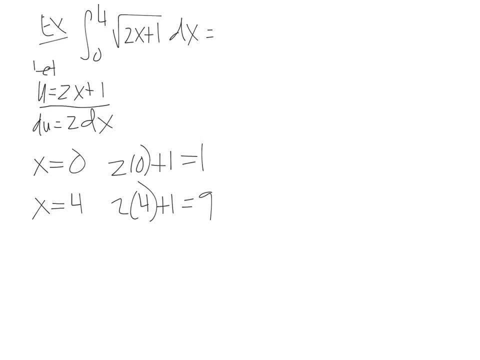 4. it'll go from 1 to 9. so now we have this is the integral from 1 to 9 of the square root of u, and then DX. well, we knew from the other video: 2 du equals 2x. that means that DX is 1 half du. so 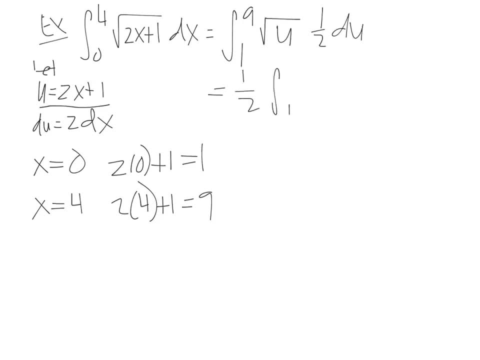 here we have 1 half, the integral from 1 to 9, of u to the 1 half du, and so this becomes 1 half times. the antiderivative of u to the 1 half is 2 thirds u to the 3 halves evaluated from 1 to 9 for 1 half. 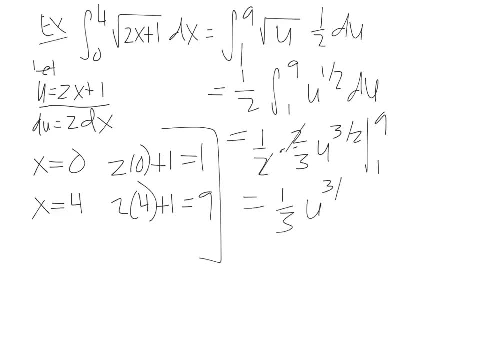 and 2 cancel. so this is 1 third? u to the 3 halves, evaluated from 1 to 9, which becomes 1 third 9 to the 3 halves minus 1 to the 3 halves, so this is 1 third. 9 to the 3 halves is going to be 27 minus 1, and so this is 26 over 3. so this is: 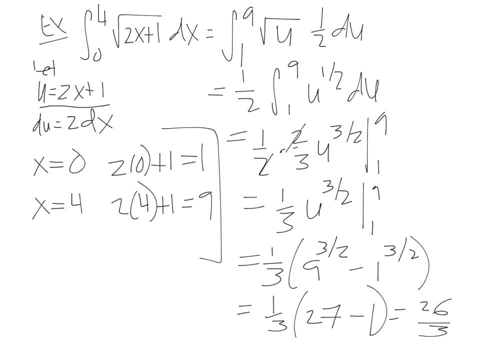 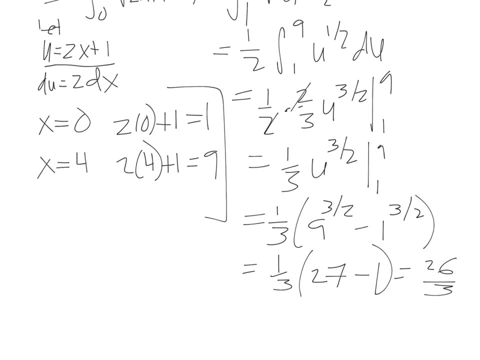 one way of solving these definite integrals- and some of you may find this confusing, having to change from 0 to 4 to 1 to 9. there is an alternate way of solving this, so the way I'm going to solve this is going to be: 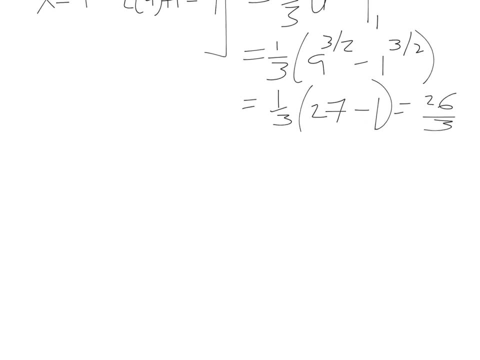 the following: we have the integral from 0 to 4 of the square root of 2x plus 1 DX, and then we made the substitution for u, so this is the integral of the square root of u times 1 half. du now notice I'm not putting our bounds in. okay, and this is the same substitution. 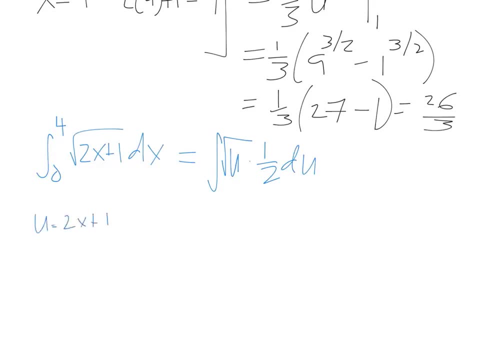 we had before, where u was 2x plus 1 and then du is 2 DX. so that's the same substitution we did before and now. so this is the integral of u to the 1 half and actually I can bring it 1 half integral u to the 1 half du, which is 1 half times 2 thirds u to the 3 halves. 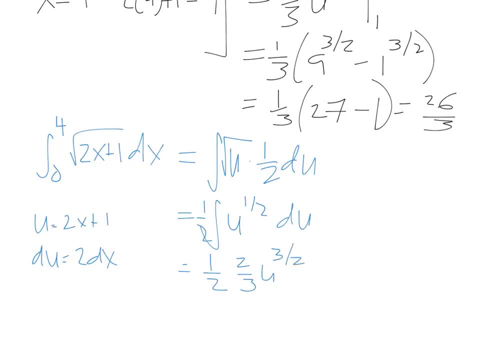 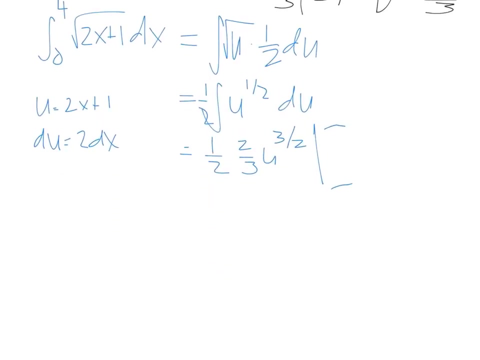 right here and we're supposed to evaluate it from something to something and we didn't. we didn't make that change, but this is because we're dealing with u. now if we, instead of dealing with u, we converted back to x, so we have it says one-third instead of u to the 3 halves we have. 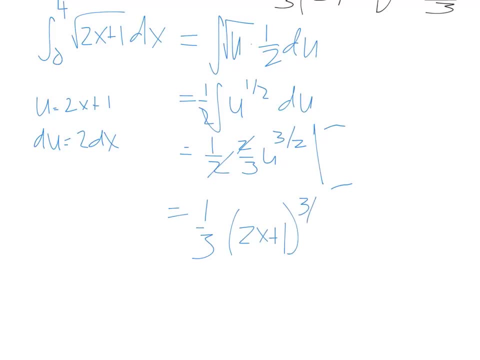 2x plus 1 to the 3 halves. we can evaluate it back to our original thing, which was 0 to 4. original value was 0 to 4, so we don't have to convert it, like how we did before, from 1 to 9. we can leave it. 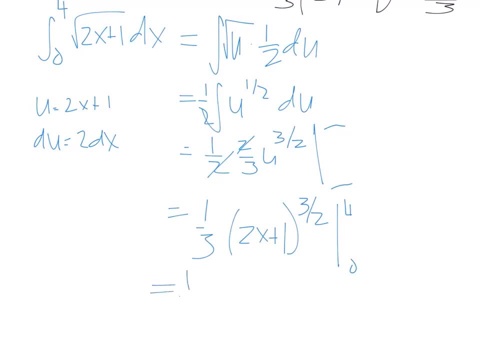 and so now This becomes 1 3rd times 2 times 4 is 8,. well, 2 times 4 plus 1 raised to the 3 halves, minus 1 3rd times 2 times 0 plus 1 raised to the 3 halves. 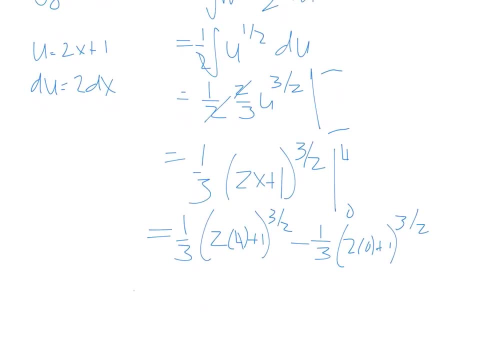 And this is going to be 1, 3rd. 9 to the 3 halves minus 1 3rd times 1 to the 3 halves, And so this should give us 9 to the 3 halves is going to be 27 times 1, 3rd. 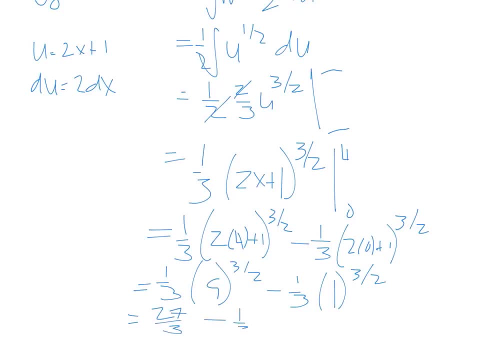 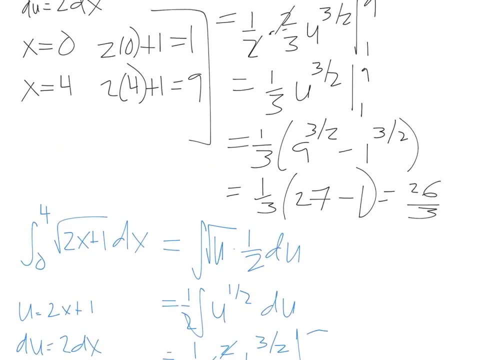 So 27 over 3 minus 1 3rd, which is 26 over 3, and that's exactly the same answer we got from up here. You can see 26 over 3.. So there are two different ways of doing it. 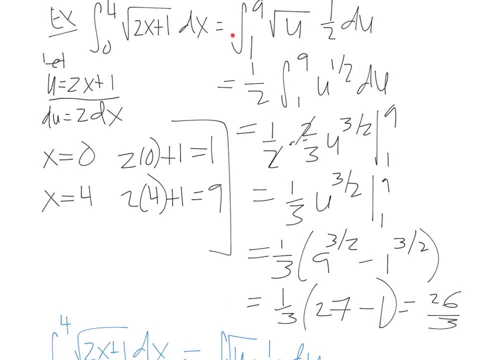 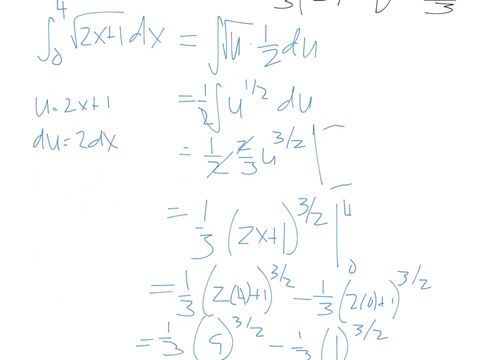 This first way, we had to convert from 0 to 4 to 1 to 9. And we just made that substitution by plugging in for u. A second way of doing this is instead of having to change your variables- we just went back, so instead of changing the limits of integration. 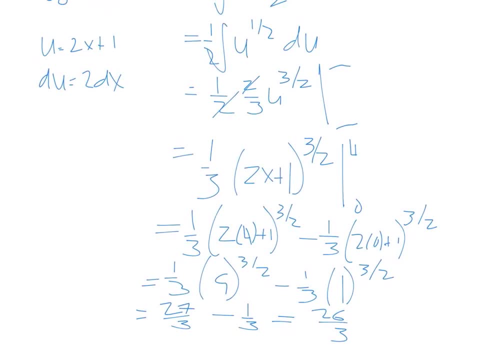 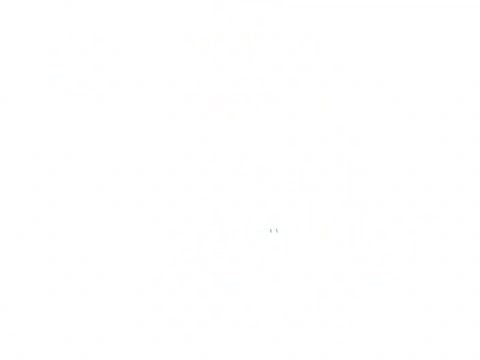 we went back and writing it instead of u, we put it back in terms of x, and then we could keep our original limits of integration. So now let's do another example with a definite integral. So let's evaluate the integral from 1 to 2 of dx over 3 minus 5x squared. 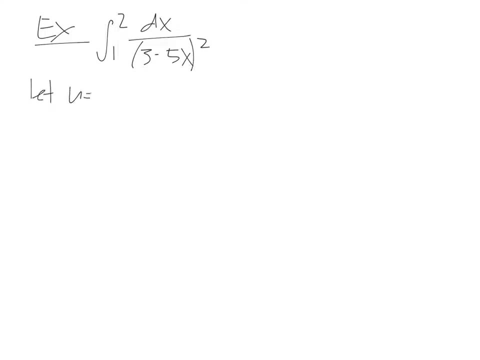 Well, we're probably going to want to let u equal 3 minus 5x, And that means that du is going to be negative 5 dx, And so this becomes the integral of: Well, dx should be negative 1 5th du. 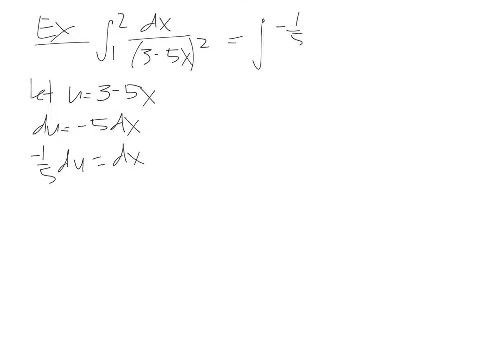 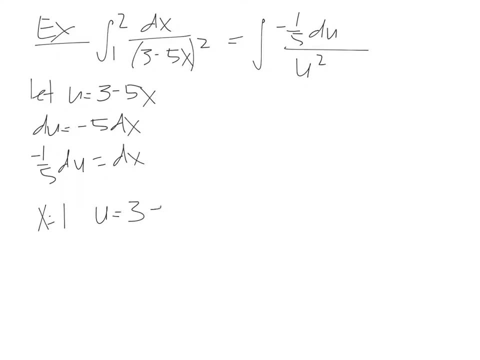 our new limit would be 3 minus 5 times 1,, which is 3 minus 5 or negative 2.. So we're going to be at negative 2.. And then if x was 2, so we're going from 1 to 2,. 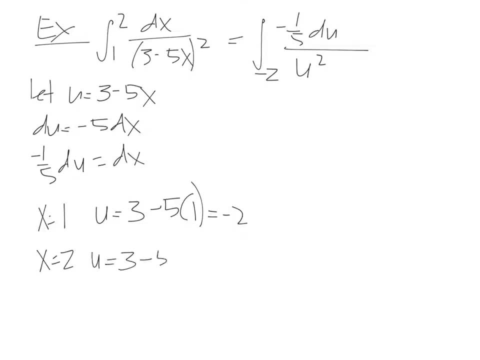 the? u would become 3 minus 5 times 2. Which is going to be negative 7.. So we're going to have the integral from negative 2 to negative 7 of negative 1. 5th du over u squared. 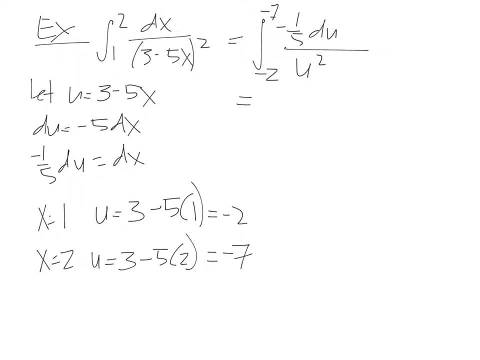 So it doesn't really look too pretty the way it is. So let's pull out the negative 1- 5th, Negative 1- 5th integral from negative 2 to negative 7 and dividing by u- squared, let's write it as u to the negative 2 du. 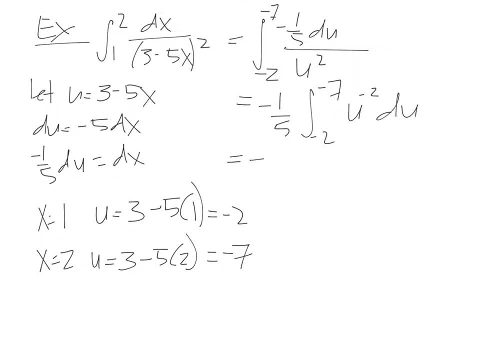 Now this looks a little cleaner. This becomes negative 1- 5th, The integral of u to the negative 2 is going to be negative 1.. Well, negative u to the negative 1.. And then we're going to evaluate that from negative 2 to negative 1.. 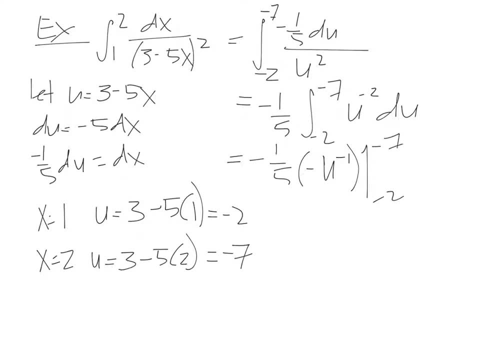 So we're going to have u to the negative, 2 to negative 7.. So we have this is going to be negative. well, negative, negative will cancel. So this is going to be just positive. 1, 5th of negative. 7 to the negative 1. 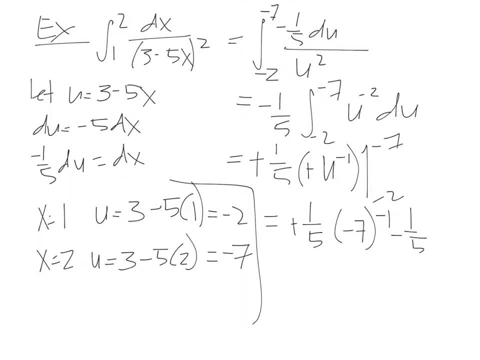 minus 1 5th of negative 2 to the negative 1.. So here we have 1 5th Times negative 1 over 7.. And then plus because again another negative negative: 1 5th times 1 over 2.. 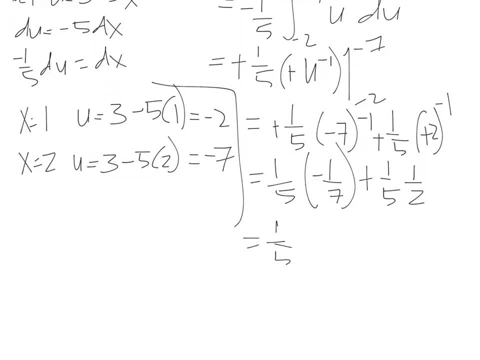 They both have a 1: 5th, so we'll factor out 1: 5th. Then we have negative 1 7th Plus 1 half, So we get 1: 5th times. common denominator would be 14.. 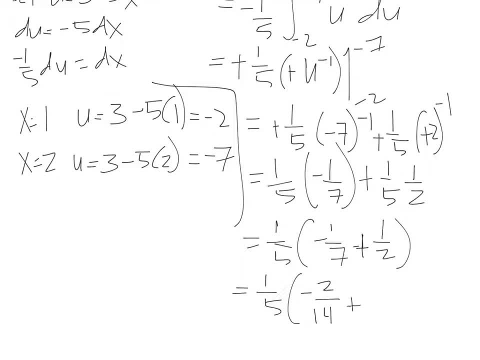 So this would be 2 over 14 plus 7 over 14. Negative 2 over 14 plus 7 over 14 gives us 5 over 14. Negative 2 over 14. So we get 1 5th. 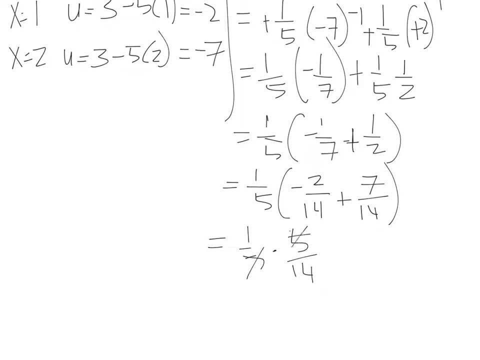 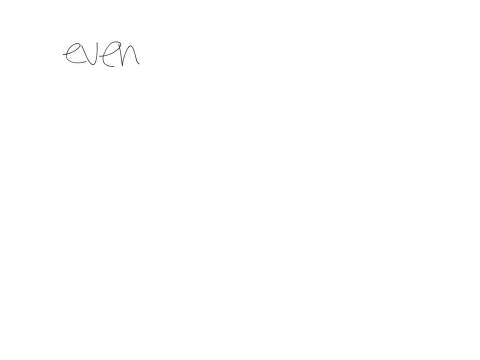 Times 5 over 14.. Our 5s cancel And we finally end up with our answer 1 over 14.. Now recall what it means if a function is even. So you might recall from algebra or precalculus that an even function is something that's symmetric. about the y-axis: 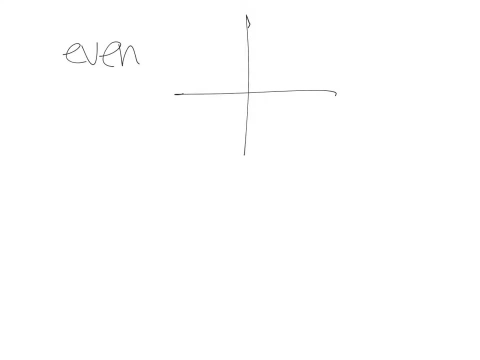 So it might be something that looks like this, Something like that, And pretend that's symmetric, Or even let's just say, a simple parabola That's going to be symmetric about the axis. A function that's odd is something that might look like this: 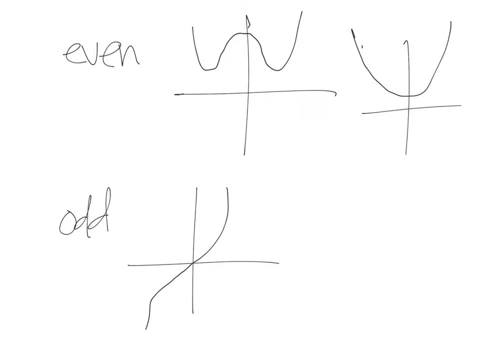 And remember, we can graph an odd function by taking one of these, These quadrants, reflecting it over the x-axis and then reflecting it again over the y-axis to get that. Now, the definition for something to be even versus odd is that if we plug in negative x into our function, f of x, 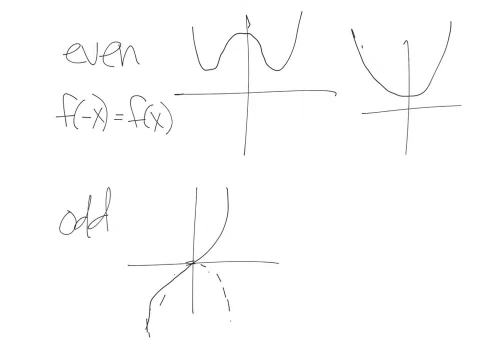 it comes out to just being the same thing, And it's odd if we plugged in negative x And we ended up with negative of our function. So this is what it means to be odd. and even In the context of integration, this becomes useful if you're integrating an even function. 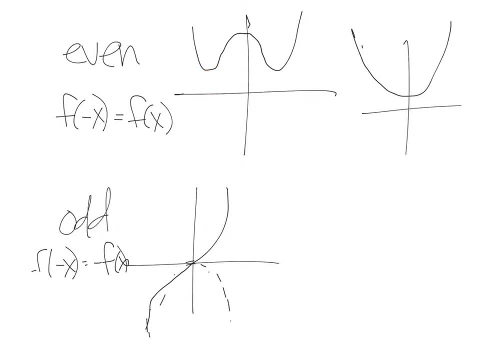 And instead of going from say like negative this part to this part, you only need to calculate half of this, half of that, and then multiply it by 2.. And then, And then, for an odd function, if we're calculating something and the width is even, or it's like: 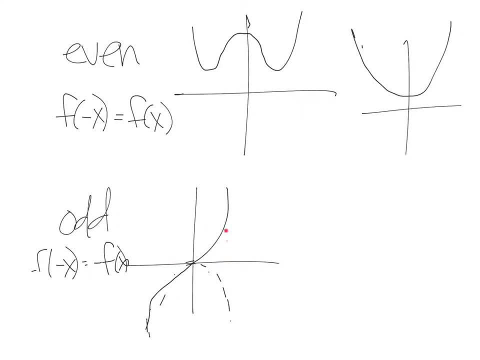 negative one value to another. the area under here is going to be positive, but then you go down here, that area would be negative and it cancels out. That's only for evaluating from the exact same value, So from like negative two to positive two or negative 10 to positive 10.. 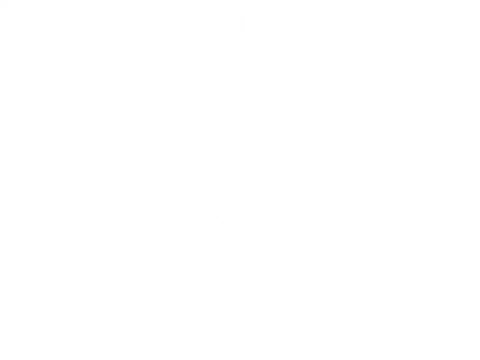 So let's actually write this up formally. So integrals of symmetric functions. and this would say the following: Suppose f is continuous on the interval negative a to a, And then, first thing, if f is even, then we have the integral from negative a to a. 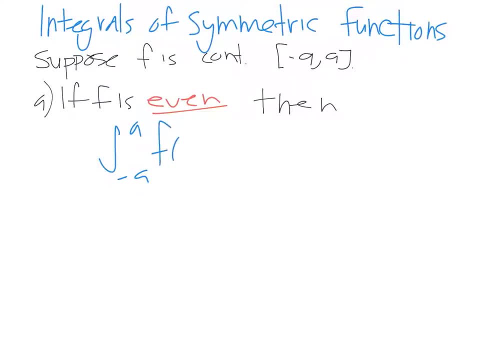 of f, of x, dx, dx, dx, dx, dx, dx. This is just twice the integral from zero to a, of f, of x, dx And even functions. so we only need to do half of it and then multiply it by two. 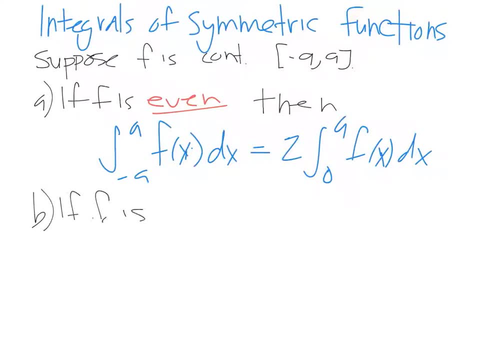 And if f is odd, then we have the integral from negative a to a, of f, of x, dx. that is equal to zero. And just a reminder what it means to be. even f is equal to zero. And then you're flooded with some otherوا. 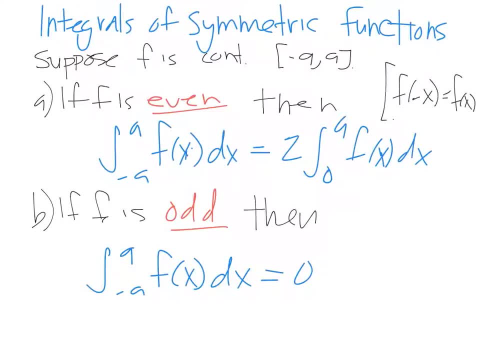 f of negative x is f of x. And what it means to be odd is f of x, fucking odd Done. and next, if you multiply along these following, you're going to notice that x is equal to minus f over x times x가는 value, which means that x bar of a is equal to 1.. 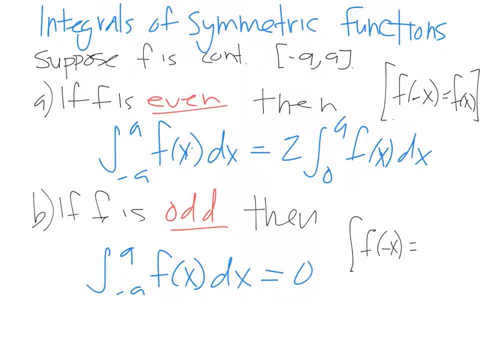 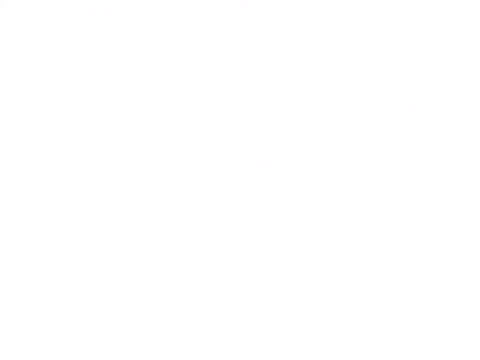 is f of negative x equals negative f of x. so an example is: since the function f of x equals x to the 6 is even- and we can test that, test it- so f of negative x is going to be negative x to the 6, which is just x to the 6, which is f of x. so since this is, 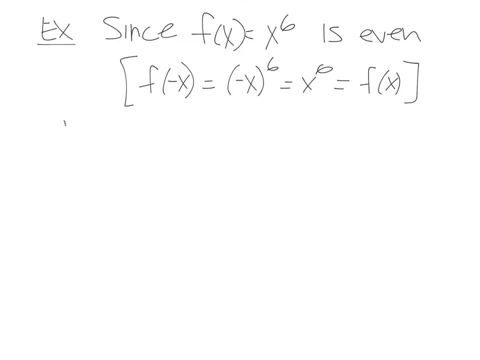 even we have that the integral from negative 2 to 2 of x to the 6 dx is going to be twice the integral from 0 to 2 of x to the 6 dx, which is going to be twice the antiderivative of x to the 6, or the integral of x to the 6 dx becomes 1 over 7.. 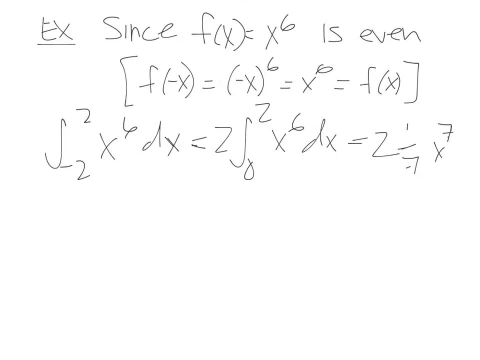 x to the 7, evaluated from 0 to 2, and so this is going to be 256 over 7 minus 0, so it's just 256 over 7.. and then another example: Since f of x is equal to: 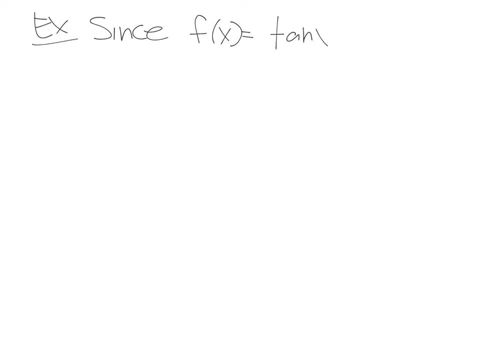 f of x is equal to x to the 7. is equal to tangent of x divided by 1 plus x squared plus x to the 4.. This is going to be odd. And why is it odd? Well, f of negative x is going to be tangent of negative x divided by 1 plus negative x. 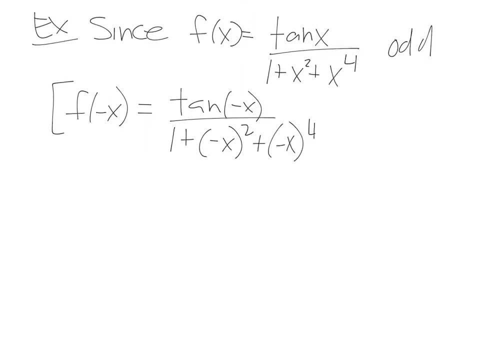 divided by 1 plus negative x Quantity. squared plus negative x quantity to the 4.. Now tangent, we know is already odd. If you recall, from the graph of the tangent, Tangent looks like that. In fact it repeats on and on. 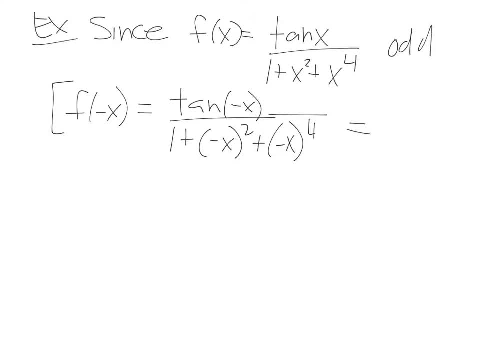 But now, since tangent is odd, Then what we have is This is equal to negative tangent of x divided by 1 plus x, squared plus x to the 4, and this is negative of this whole thing. So this is just negative f of x. 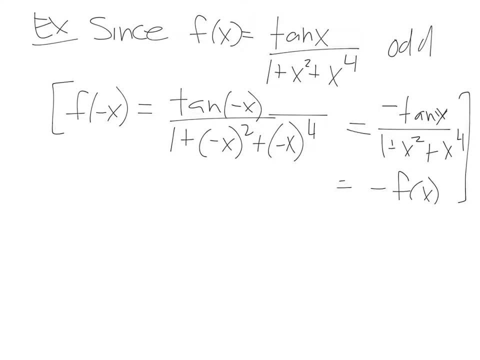 So now we know it's odd. So We have that the integral from negative 1 to 1, of tangent of x divided by 1 plus x, squared plus x to the 4 dx. Because it's an odd function, This integral is just 0.. 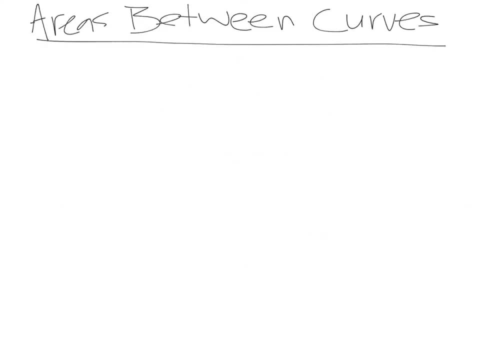 So remember what a tangent center function looks like. Today we gonna talk about the areas between curves. So let's say we have a curve that might look like this. We'll call this curve F. This is our function f of x. and let's say we have another curve that lies below the. 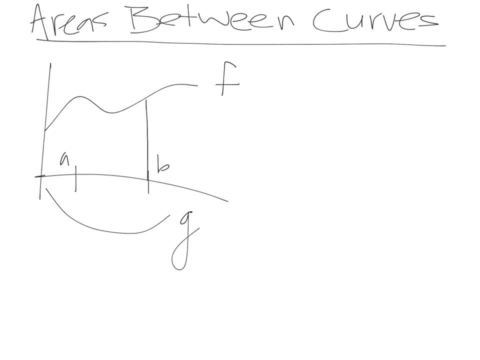 axis And that's our curve G. Now, Well, to find this area, we already know how to find that and if we do approximations, we can approximate by using rectangles. or when we take the limit as it goes to infinity, we can use integration. 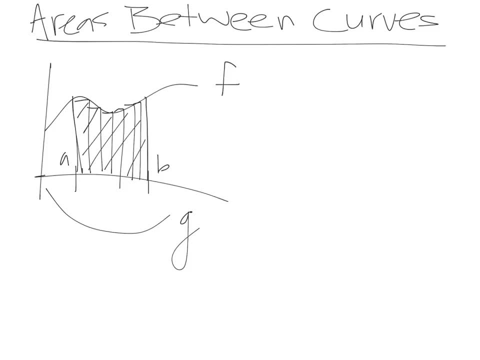 same thing. if it lies below the axis, down here we can use a bunch of rectangles and when it's below the axis, the area is going to be negative. or we can also use integration. so finding the total area between these two regions. we really want to find the difference. we want to find 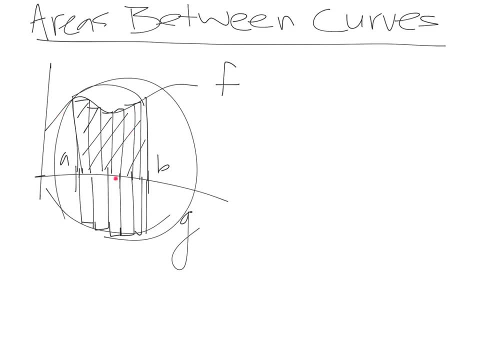 this area above, and remember, if this is below it's going to be negative. so we want to add these two and so, if we're adding a positive number and a negative number, really what we're finding is f minus g. so the formula for the area will be given by the following: 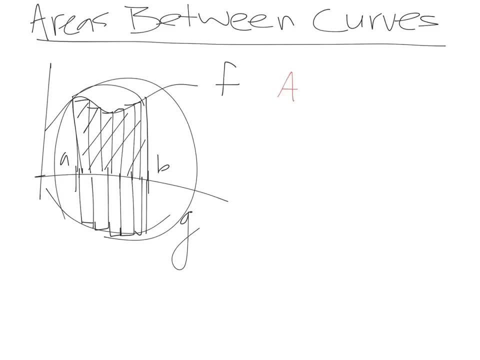 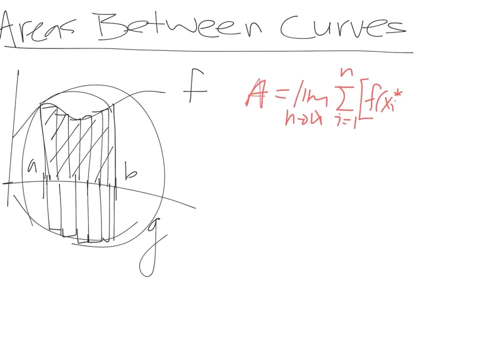 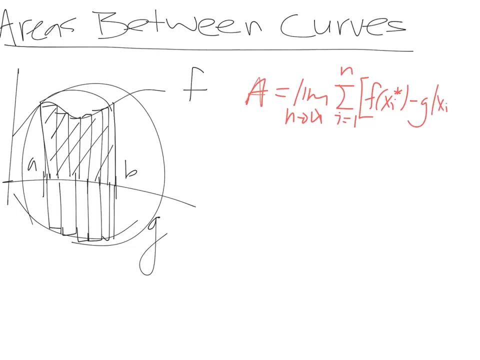 so area is equal to- let me make this a little bit bigger: font area is equal to the limit, as n goes to infinity, of the sum, where i goes from 1 to n, of the difference of f of x sub i star minus g of x sub i star. 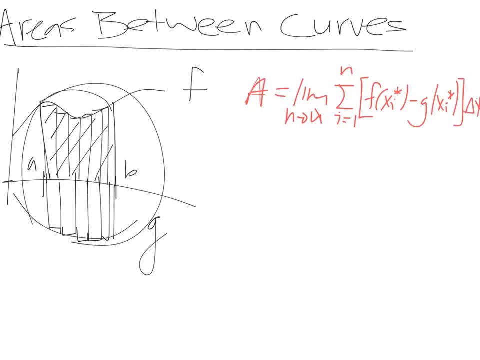 all times our delta x. alright, delta x. there we go. ok, so this looks familiar if we didn't have this minus g, but this looks familiar. the limit n-th constant is equal to f of x, less than xx-th formula of the sum of f of x sub i star times delta x. 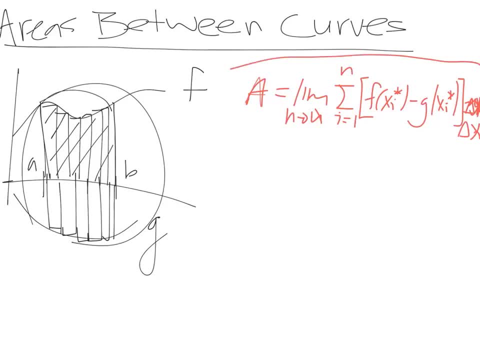 Now. so this is one equation for the area, and another equation is going to be given with the following: The area, we'll call this A of the region bounded by the curves, y equals f of x and y is equal to g of x. 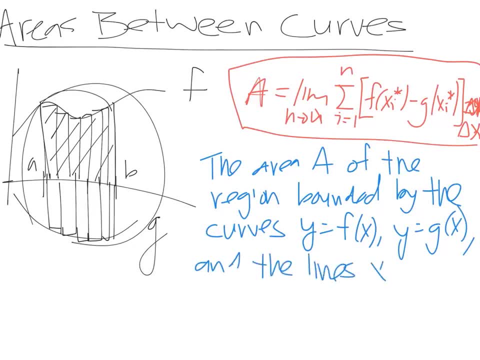 and the lines x equals A and x equals B. So we're going to be between this curve and this curve down here and between the vertical line and this vertical line. This is going to be where f and g are continuous and we're going to have 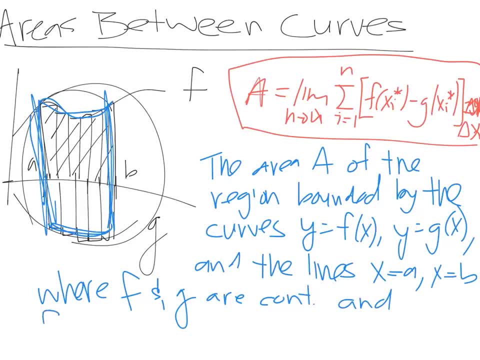 to assume that the f of x function is going to be the top function, So that's going to be greater than or equal to g of x. So in this case order matters: The top number has to be greater than the bottom number. 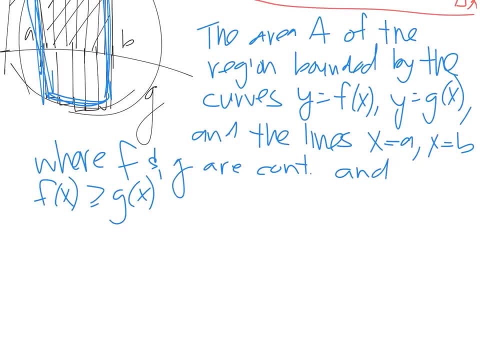 So f of x is greater than g of x and this is going to be for all x in the interval from A to B. So this is given by the function. formula a equals the integral from a to b of f of x minus g of x times dx. So 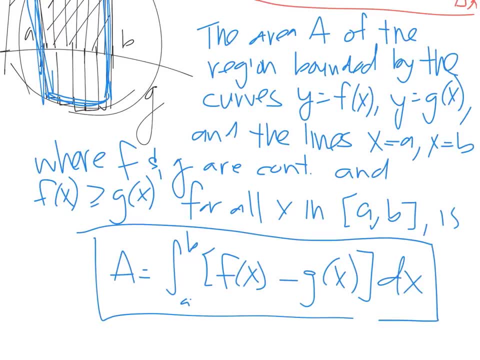 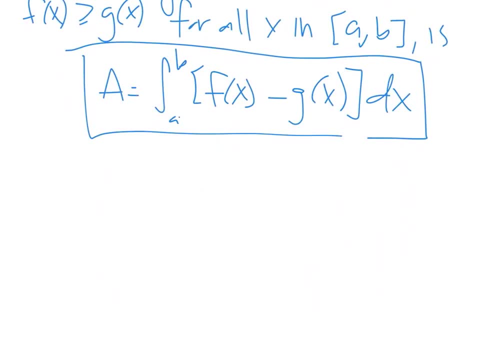 this is what we're going to use and it doesn't have to always be above or below, but you might have your two functions. let's say this is the function f and the function g looks like this: f and g are both going to be above the axis if we're. 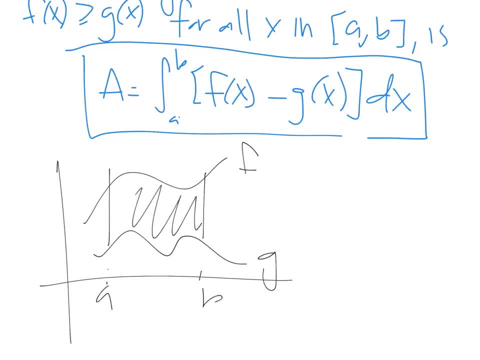 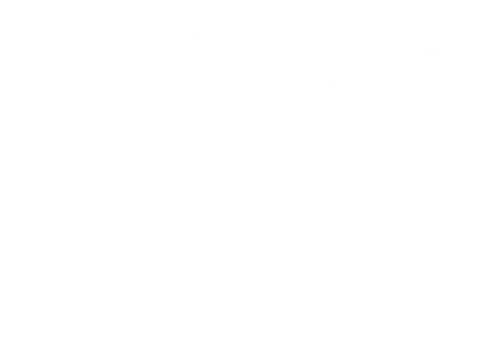 going from a to b. this is the area underneath, and you can find that area using this formula. Now let's do an example: Find the area bounded by the two curves. let's just call it. say: between the two curves, y equals 2 minus x squared, and that's a parabola. and the line y equals: 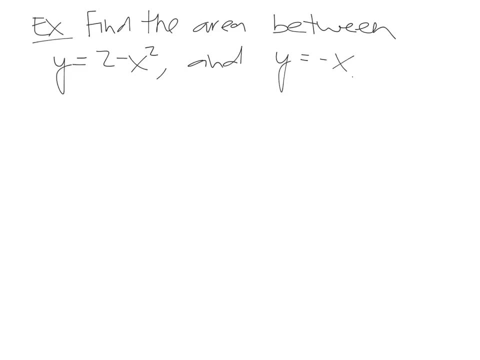 negative x. So here I didn't give you where, what function to go, from where to where. so we actually have to figure that out. So let's go ahead and plot what we have. This first function is going to be a parabola, and it's a parabola that goes up here at 2. 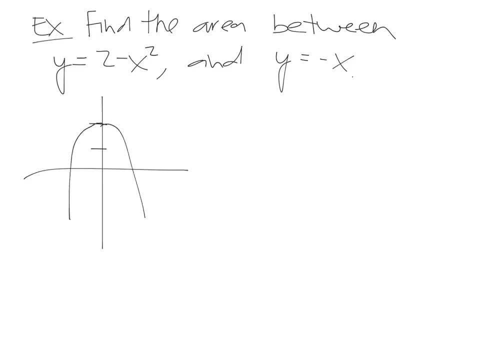 and it's facing downwards, so something like that. then we have a straight line with a negative slope, slope of negative 1. And so we have that and it crosses at the origin. So we want to find the area between these two curves, which is going to be this region. 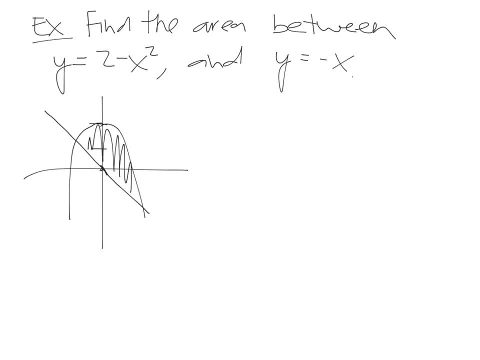 right here. So this is going to tell us that this top curve, that's going to be the function we'll call f. So that's the parabola. so our f is going to be 2 minus x squared, and then this straight line is going to be our g function and that's going to be negative x. 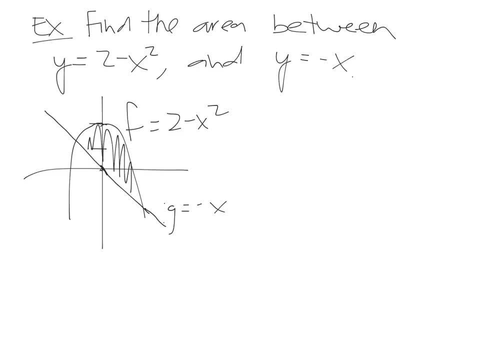 So now we know our curve, which one is going to be f and which one is g, but we still don't know the regions. But we can figure that out. So when are these two functions equal to each other? So you get 2 minus x squared equals negative x. you set them equal to each other. you can. 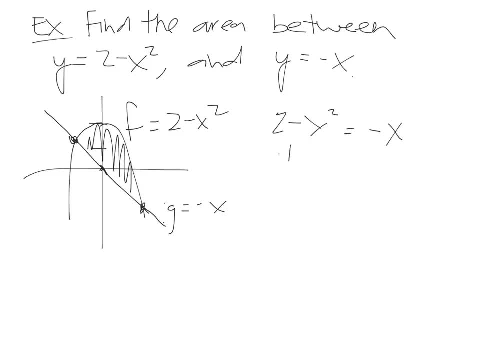 solve. I'm going to move everything to the right side. so if I add x squared, Add x squared, and then I also subtract 2 and subtract 2, we get zeros on the left, x squared minus x minus 2, and we can now factor x minus 2 times x plus 1, and so we get x is equal to negative 1 and x is equal. 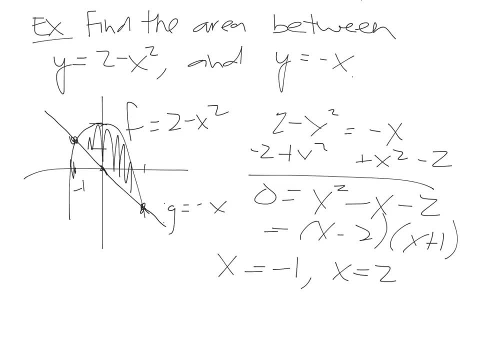 to 2, and so that's the points negative 1 and 2.. So the area is going to be the integral, from negative 1 to 2, of your f function, your top function, which is 2 minus x, squared minus your bottom function, which is negative x. So the integral of 2 minus x, squared minus negative x. 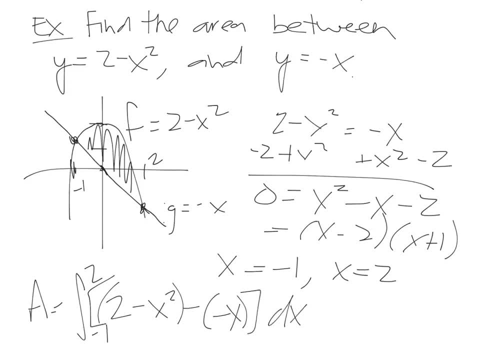 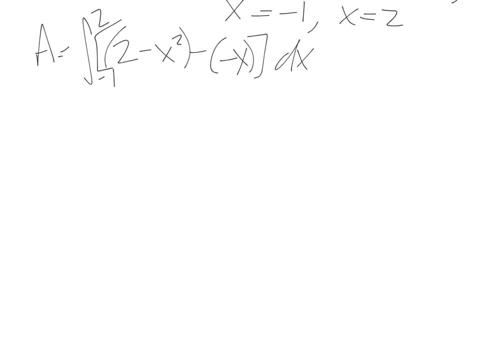 and this is going to be all times dx. So now we can solve this definite integral and we can solve this integral. This is going to be the integral from negative 1 to 2 of, let's say, 2 minus x squared and minus a negative x gives you plus x and all dx. So go ahead and finding the integral of this, the. 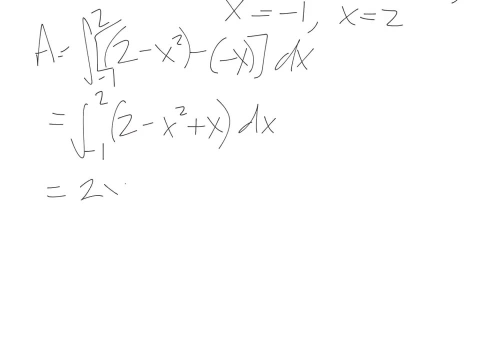 antiderivative of 2 is just 2x. the antiderivative of x squared is one third x cubed and the antiderivative of x is one half x squared, and we're going to evaluate it from negative 1 to 2.. 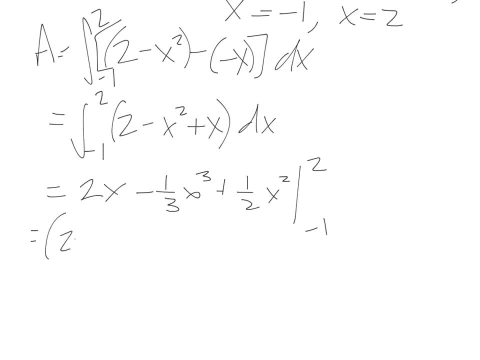 So we get evaluating that 2, we get 2 times 2 minus one third times 2 cubed, plus one half times 2 squared, minus 2 times negative 1, minus one third times negative 2.. So that's going to be the integral. 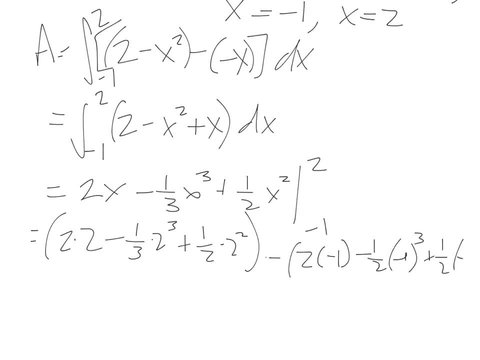 times negative 1 cubed plus one half times negative 1 squared, So we get 4 minus 8 thirds and then one half times 2 squared, so one half times 4 or just plus 2, and then we get minus and negative. so 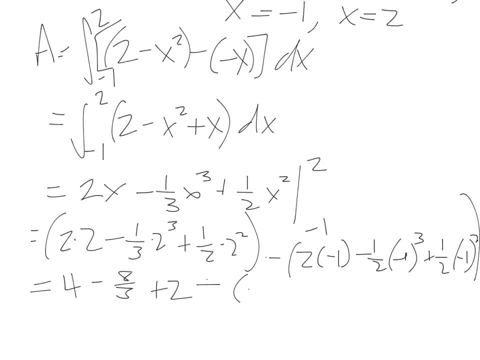 we get- oh, we'll just do this. so 2 times negative 1, negative 2, and then negative 1. cubed is still negative 1, but minus one half comes plus one half and then plus another one half. so we get 6 minus 8 thirds, and in fact this should have been a 3, so sorry about that. that should be a 3.. 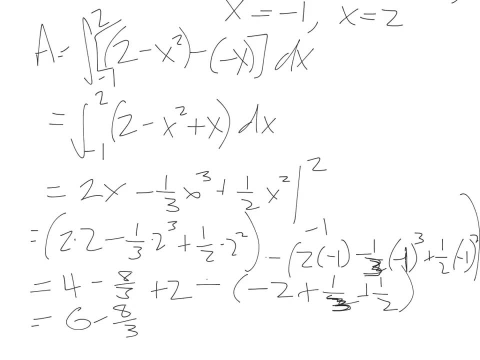 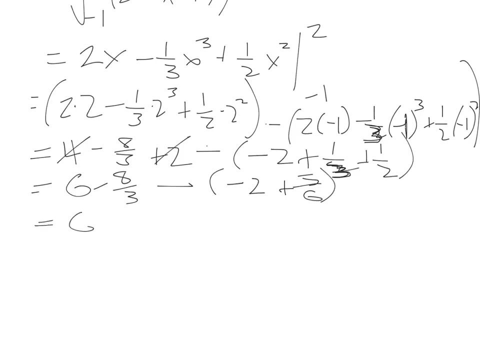 So 6 minus 8 thirds is a combined those to make 6, and then we're going to subtract and then we'll have negative 2 plus one third plus one half 5 over 6, and so we get is gonna be 6 minus 8 over 3. in fact I'm instead of writing 8 over 3, I'm gonna 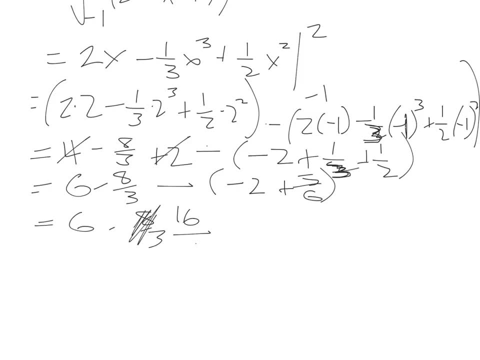 write 16 over 6. I just multiplied it by 2 over 2 so we can have a common denominator: plus 2 minus 5 over 6. so now we are 6 plus 2 will give us 8 minus. we get 21 over 6, and that 21 over 6 they both have a 3 in it, so we can reduce and 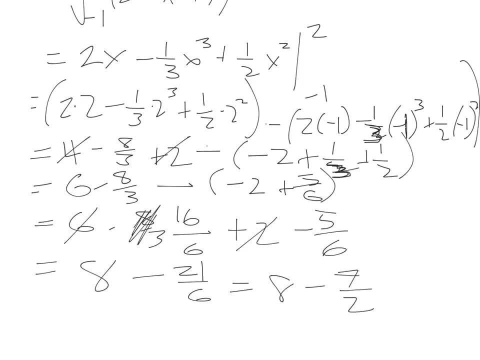 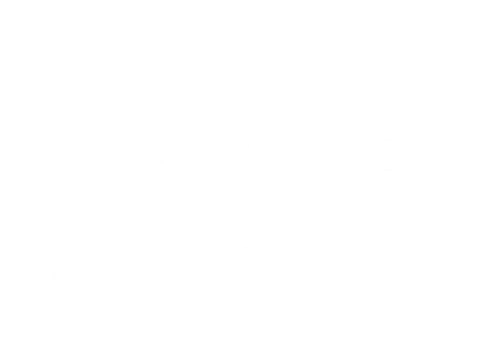 that becomes 7 over 2, and if we want to combine that into just a single fraction it would be 9 halves. so that's the area between the two curves. we'll do another example. find the area bounded between the two curves. y equals the square root of x, and y is equal to x minus 2. so again, we're not really. 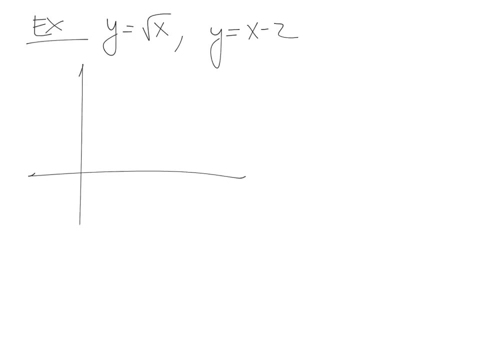 given much here, so we're gonna have to figure out what this region looks like. so the first graph- y equals the square root of x- looks something like this: this is: y is equal to the square root of x. and then the straight line, y Zurich, is equal to x minus 2, that's going to be a straight line at negative 2, with a slope. 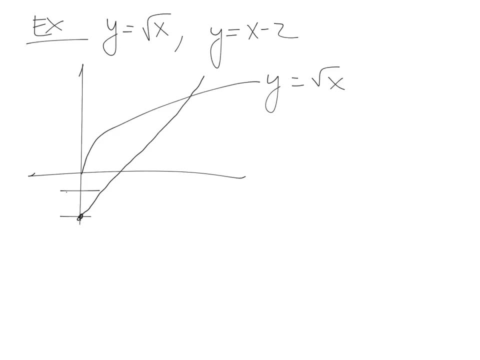 maybe something like that. And just for sake, let's also add another stipulation: and this region will also be bounded below by the x axis. So now, we're not going to look at this part below. we're going to be restricted by the 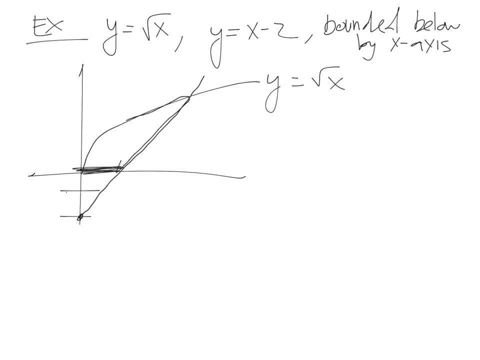 x axis. this line, and then y, equals square root of x, And so this right here was: y is equal to x minus 2.. So this problem is a little different From the other one, because we're actually going to break this up into two separate pieces. 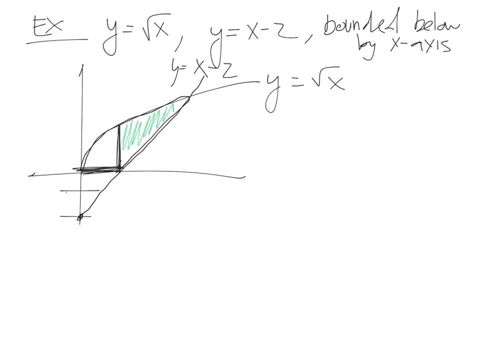 The first piece is going to be right here and this is going to be between two curves. It's going to be between this upper curve and this lower curve. Then the other piece is just going to be this little piece right here and this is bounded. 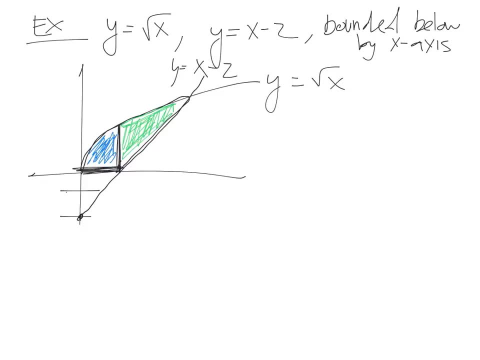 above by the square root of x, And that's it. When you just take the integral of the square root, or just the integral, it's just the area below that curve and above the axis. So all we need to do is figure out. what are these points? where does it cross? 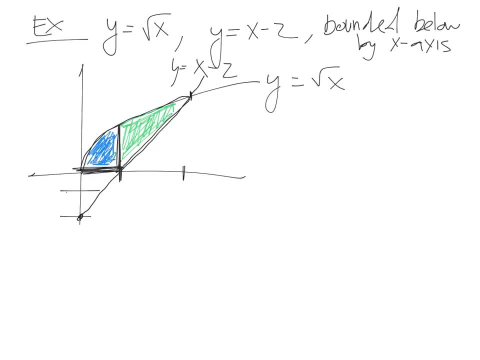 Well, the graph: y equals negative or x minus 2, excuse me, it crosses the axis right here when x is equal to 2.. So we know that point, but then to find this other point, that's when we're going to have. 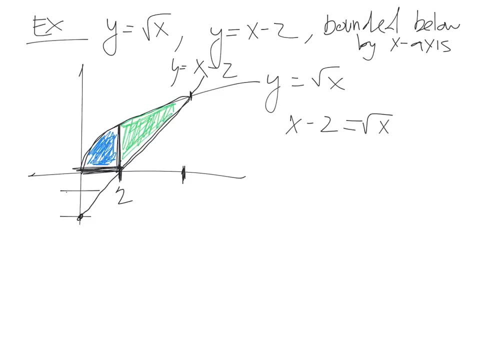 x minus 2 equals the square root of x. So we need to figure out when they're going to be equal. Well, we have a square root of x. that's really not something we like, so let's actually square both sides. So we get x squared minus 4x plus 4 equals x. 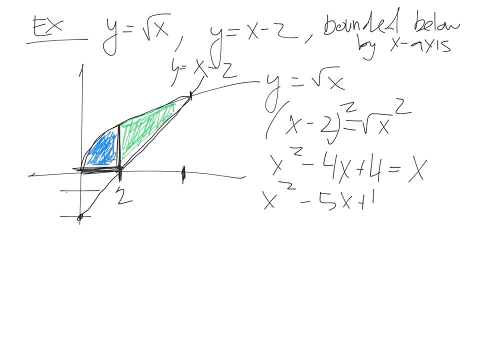 Moving x to the other side, we get x squared minus 5x plus 4 equals 0, or x minus 4 times x minus 1 equals 0. And so we're going to get two values. We're going to get x is equal to 1, or x is equal to 4.. 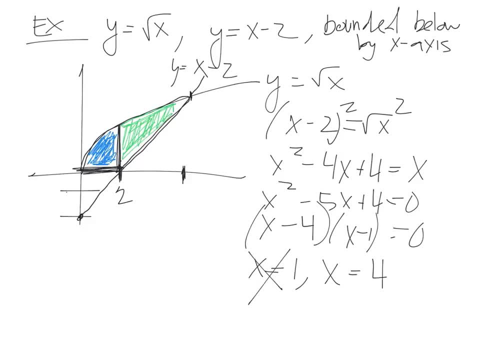 This value, x equals 1, is an extra root that comes out when we end up squaring it And you can just look at the graph. 1 does not work, So we ignore that and then we look at this point. So this is going to be right there. 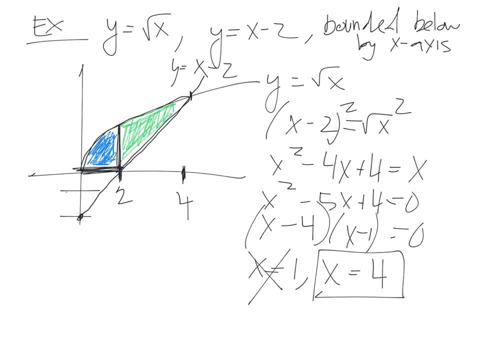 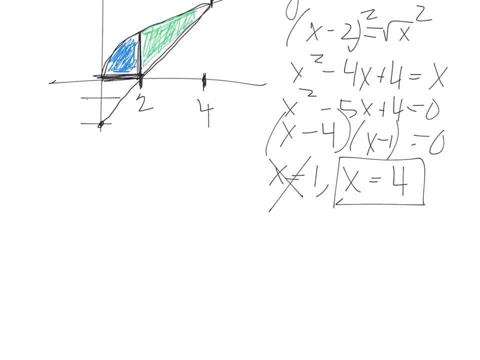 For the green region, we're going to have an integral between the two points 2 and 4.. And then for the blue region, we'll have just an integral from 0 to 2.. Alright, so area for the blue is just the area under the curve. 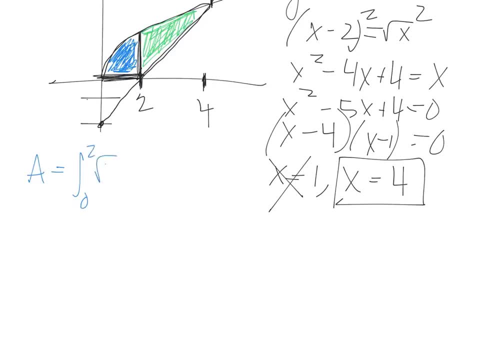 So that's the integral from 0 to 2 of the square root of x- dx. Or the integral from 0 to 2 of x to the 1 half dx, Which is 2 thirds x to the 3 half dx. So that's the integral from 0 to 2 of x to the 1 half dx. 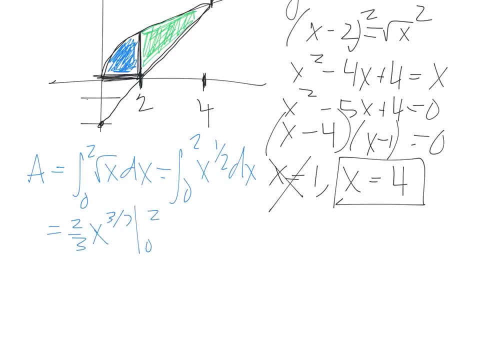 Evaluated from 0 to 2.. This comes up to just being 2 thirds x 2 to the 3 halves, minus 2 thirds x 0 to the 3 halves, or 2 thirds x 8.. The green region, our area, is going to be the integral from 2 to 4 of the 3 half dx. 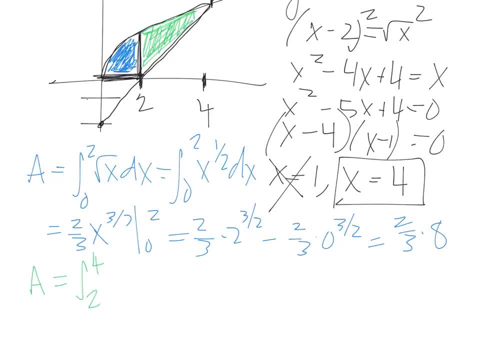 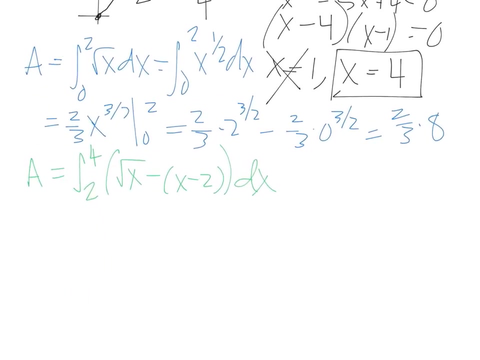 So that's the integral Of the top function, which is the square root of x, minus the bottom function, which is x minus 2 dx. And so we're going to go ahead and we'll rewrite this. This is the integral from 2 to 4 of x, to the 1 half minus x plus 2 dx. 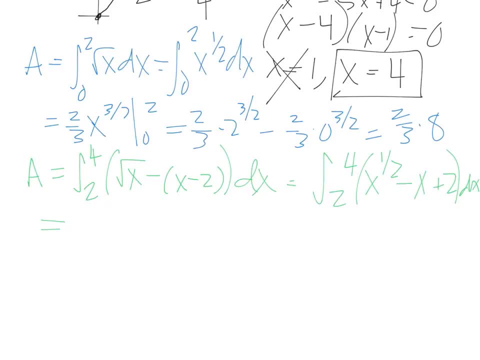 Alright. So we're going to get 2 thirds x to the 3 halves minus 1 half x squared plus 2 x evaluated from 2 to 4.. And so we get 2 thirds times 4 to the 3 halves minus 1 half times 4 squared plus 2 times. 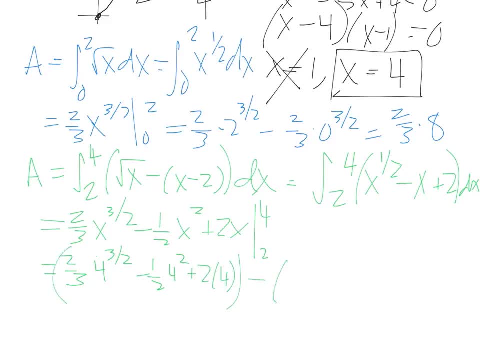 4. Subtracted by 2 thirds times 2 to the 3, halves minus 1 half times 2, squared plus 2 times 2.. And then, if we were to go ahead and simplify this, I'll tell you right now that that is. 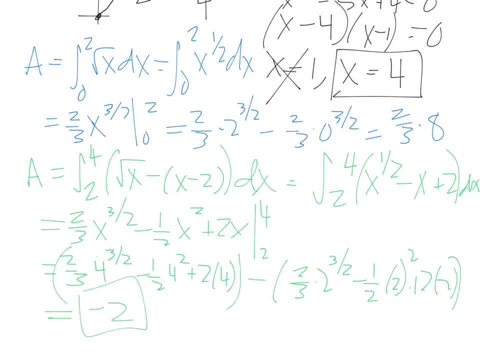 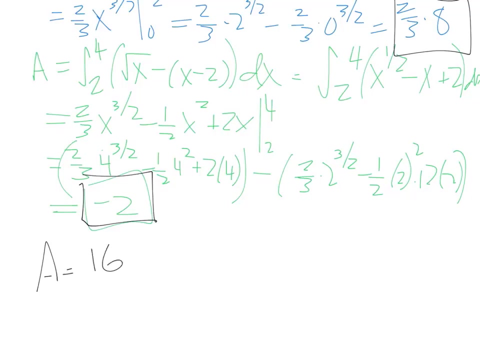 equal to negative 2.. So the total area is going to be the area plus blue, Or of the blue plus the area of the green. So our total area between the two curves is going to be 16 thirds plus negative 2, which. 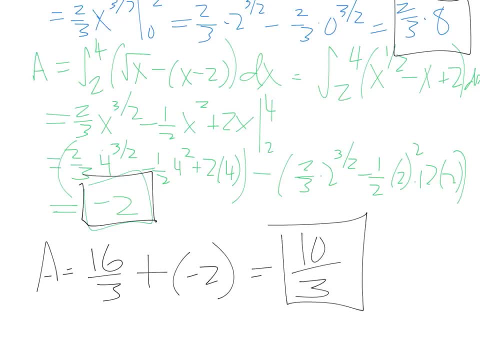 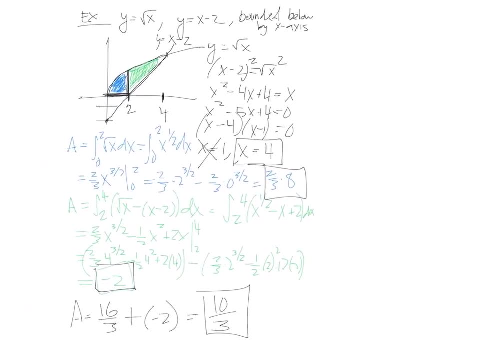 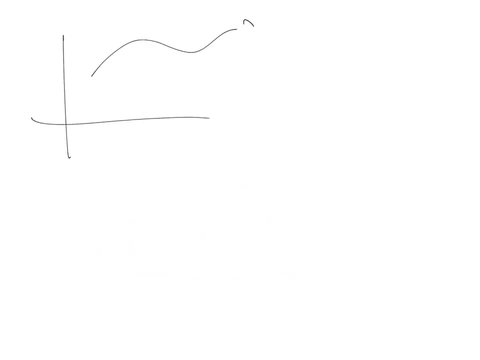 is 10 thirds. That is the area between the two curves Right here. So now we know how to find the area between two curves When you have one curve f and that's above another, curve g. But now what if we have, say, our curve f looks like this: 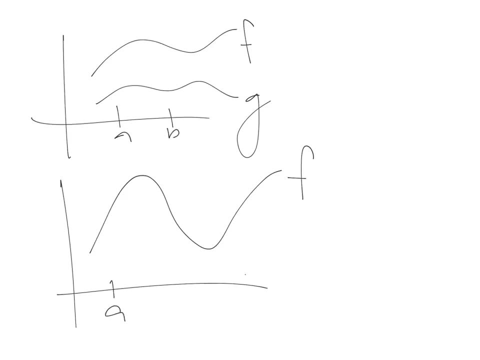 If we're going between two points, say a and b, a and b, And we have a curve g that starts off below and then it goes above and then maybe even below again, And notice, if we're going between two points, which is 10 thirds, then our total area is: 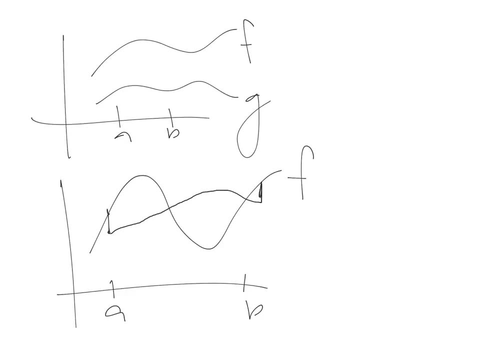 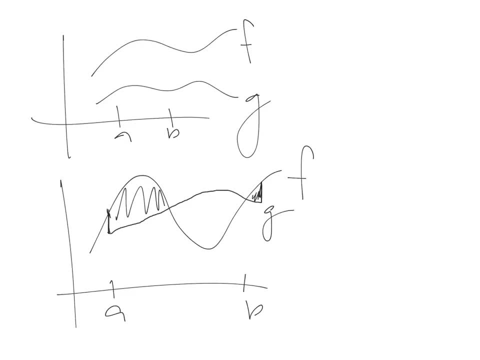 is above, so we call that's our g function and another region where f is above, but in this region down here where g is above. so how do we really do something like this when you have when it switches? so in this case we knew what happened when f was above g, but when they alternate, what we're going? 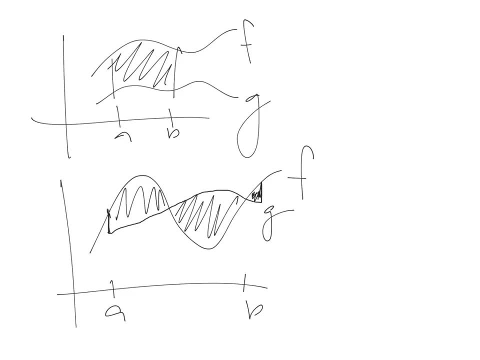 to do is the following: just simply break it up into different pieces. we'll have this one red piece right here, and maybe i'll make this other one over here red as well, and then we'll have make this one blue, okay, and then you just figure out where these points are and you do three sec, you figure out. 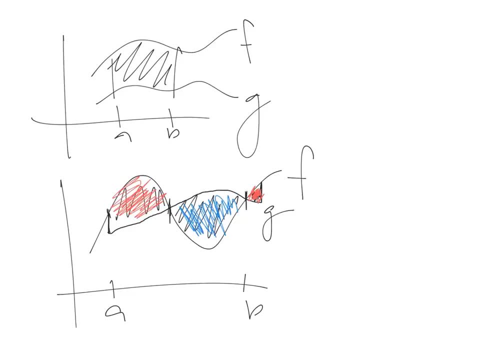 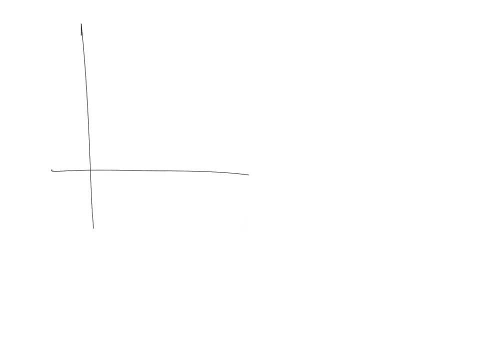 where each of these intersections are, and you just calculate three separate integrals. each integral the. you're going to make sure you got to figure out the top function versus the bottom function, the top function versus the bottom, and so forth. now we might also have some sort of curve. that's instead of Y. 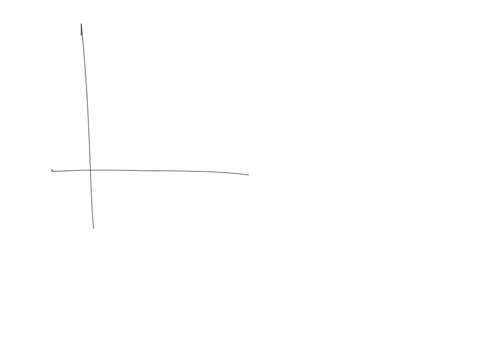 equaling a function of X. we'll have the other way around: X is a function of Y. so what that might look like would be we might have something like this, and then this would be the curve: X is equal to G of X, excuse me, X is equal to G of Y, and 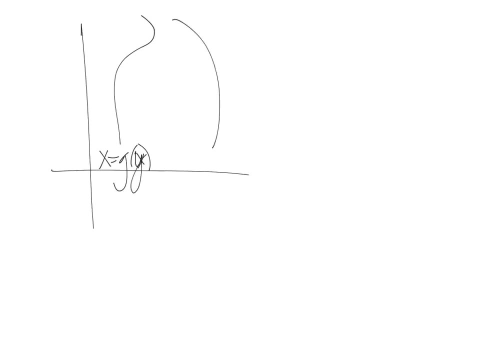 maybe something that looks like this, and this is going to be: X is F of Y. these are functions in terms of Y and if you want to find the area between these two curves, let's say between some point C and some point D, so you want to find this area we're going to integrate. so area would be the: 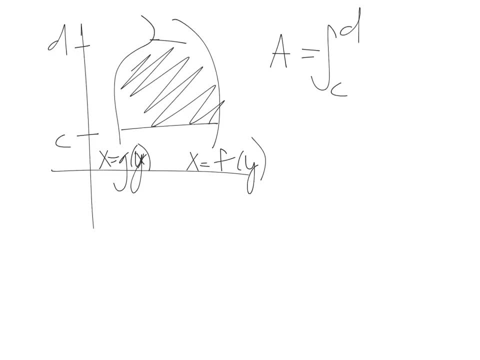 integral from C to D, but instead of it being a function of X, it would be a function of Y F, of Y minus G, of Y dy, and so we'll do an example to illustrate that why this might be useful. find the area enclosed by the line Y is equal to X minus 1, and the parabola Y squared is: 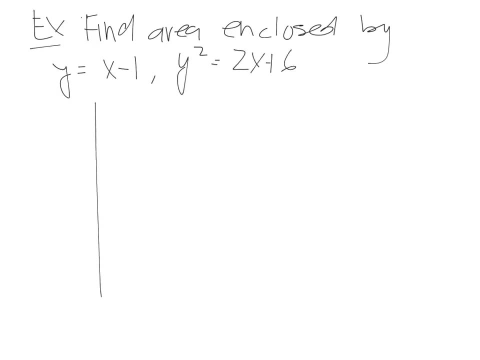 equal to 2x plus 6. what does this look like? well, we have a parabola: Y, squared, equals 2x plus 6. that's a problem that faces. that opens to the right something like this: and then y equals x minus one. that's. 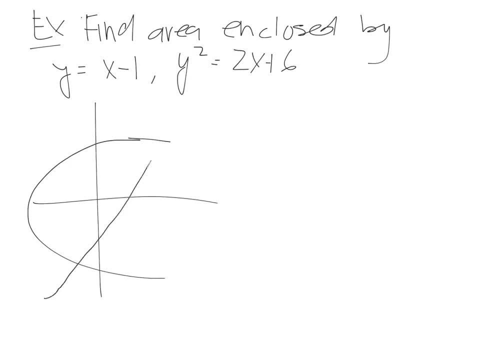 a line that go something like that. so now to find the area in between here, what we would have to do would be to figure out these points of interception, these points of integration you have to deal with. do these things have different y components, intersections? so we're going to have this equation: y squared equals 2x plus 6, and then, using the, 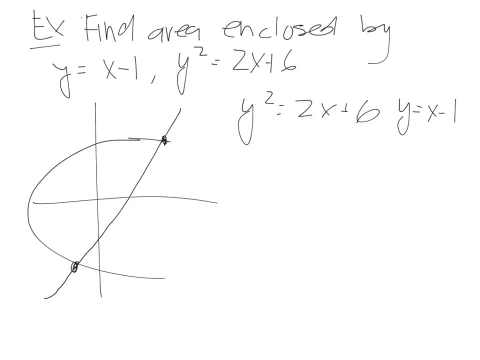 first equation, that said y is equal to x minus 1. solving for x, we get x is y plus 1. we'll solve, we'll substitute. so we get y squared is 2 times y plus 1 plus 6, or y squared is 2y. 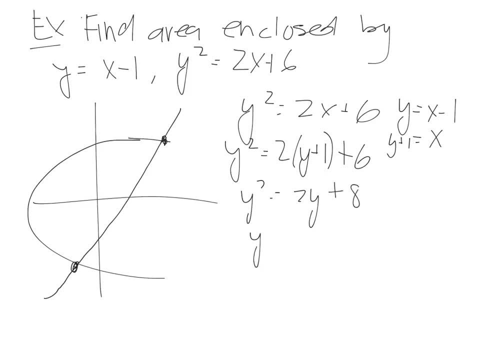 plus 2 plus 6, so 2y plus 8 or y squared minus 2y minus 8 equals 0. then you get y minus 4 and y plus 2 equals 0, and so we know that it goes from down here where y. 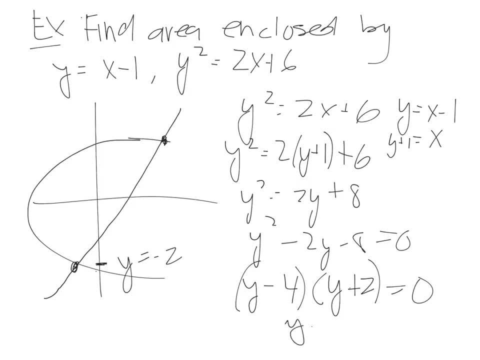 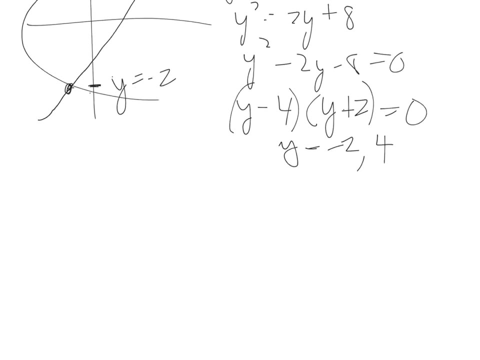 is negative 2.. so we get our answers: y is negative 2 and y is four, all the way up to up here where y is four. so now to find this area, we're going to get that the area is equal to the integral where y goes from negative 2 to 4 of our upper function. so now, looking here, we need to figure out up here. 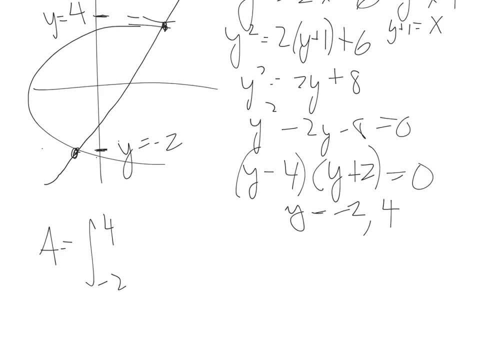 click the square for y to find out what the area of our number is, what's the upper function. so, if you can sort of like tilt your head sideways, this is the y-axis, so the upper function goes out this way. so this is our upper function and then this is our lower. 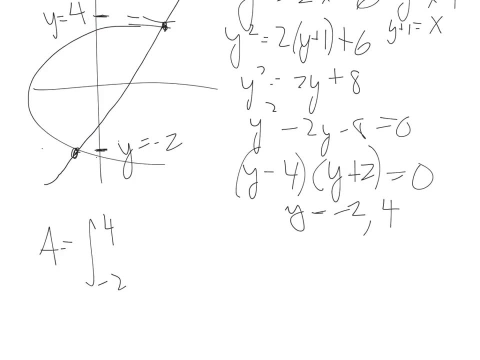 function. so it's just like how we did with a regular function, but just sideways. so we get our upper function is the straight line, and the equation for the straight line is going to be: well, it's what we need to do because, remember, we're we're writing it as x. 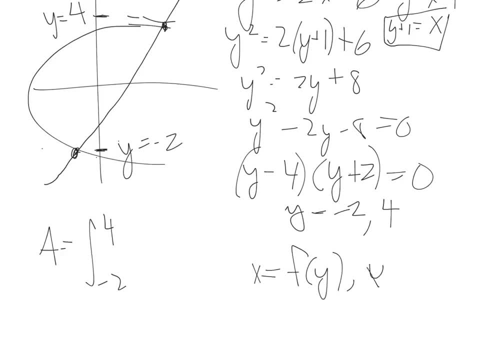 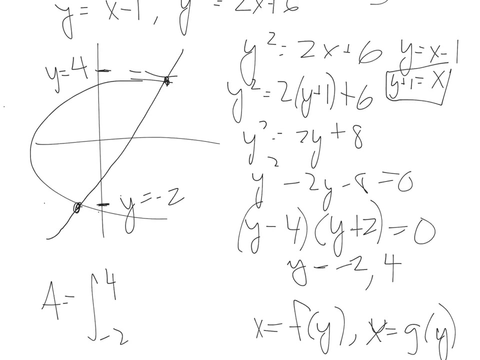 is like a function of y, and then x was like a function g of y. so what we need to do is we need to write them in terms of x, of just y's. so actually i'm going to move up a little bit more so we could see the initials. 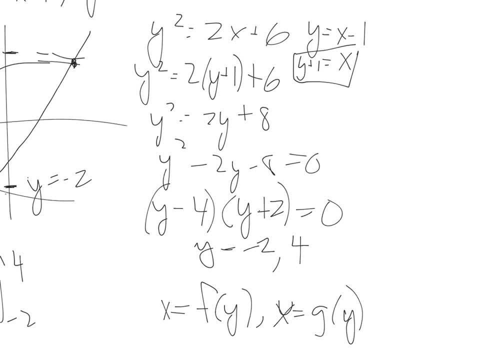 equations. we had them right here so i had written this first one, the straight line, but the parabola that needs to be rewritten. let's move that over here. so we want to just solve it. for x, we're going to get: 2x is equal to y squared minus 6. i move 6 over and then, if i divide, 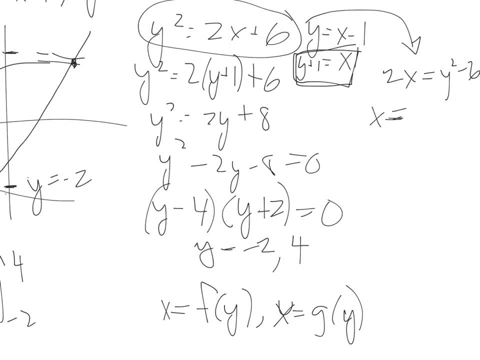 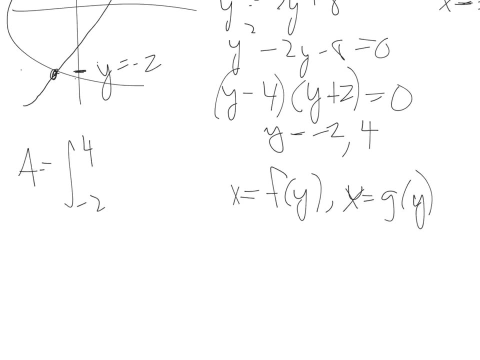 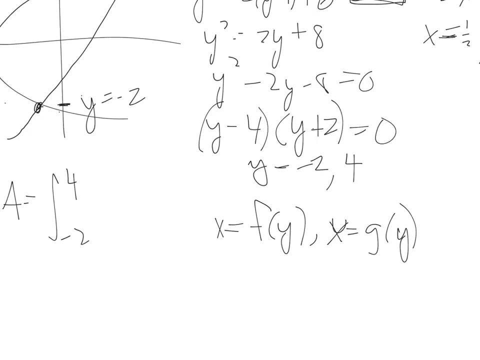 everything by 2, we get. x is equal to one half y squared minus 3. that's what we're going to substitute back into here. so a is going to be. well, the straight line comes first. so the straight line is going to be y plus 1, minus the parabola, which is one half y squared minus 3 times dy. 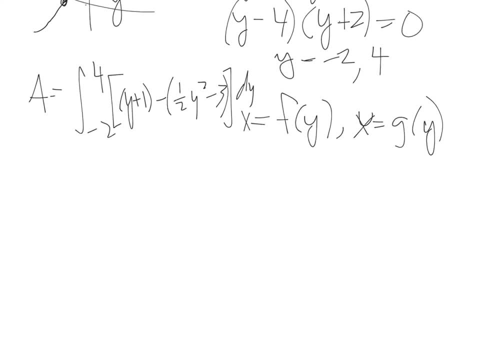 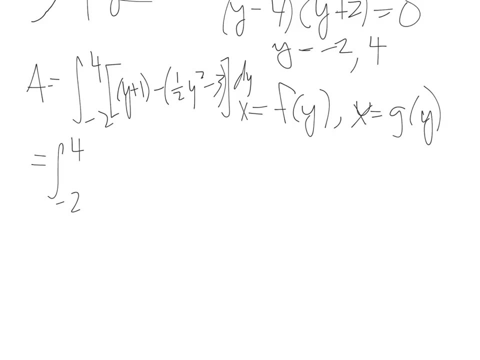 giving myself a little bit more room. go ahead, and this is going to be the straight line. so we're going to is going to be the integral from negative 2 to 4 of y, and then you can combine the 1 and 3 minus the negative 3, so that would give us plus 4 minus 1, half y squared all times. 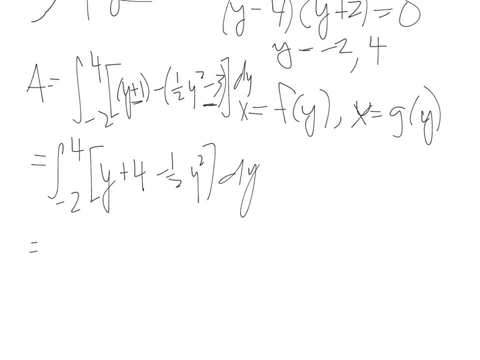 dy. and so now, integrating, we get 1 half y squared plus 4y minus 1, 6 y cubed, evaluated from negative 2 to 4.. Plugging in the limits of integration, we get 1 half times 4 squared plus 4 times 4 minus. 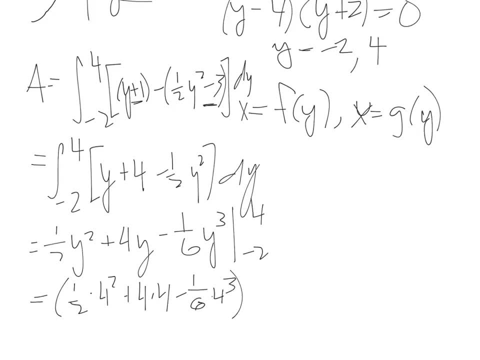 1, 6 times 4 cubed Cubed minus 1 half times negative: 2 squared plus 4 times negative 2 minus 1, 6 times negative 2 cubed. Simplifying this, we end up with 18, and that's the area. 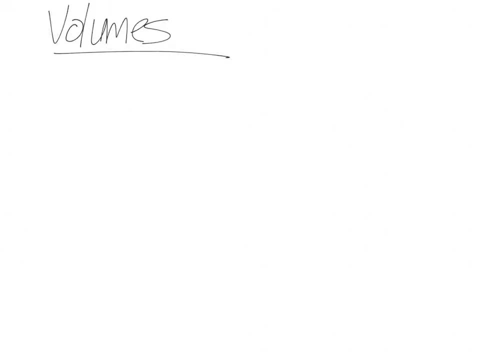 Today we're going to talk about volumes. Now we already know how to find the area between two curves. let's say we have a curve like this and we have another curve like that. so this first curve we'll call that f, the second curve we'll call it g. so we can find this area between those two curves by calculating. 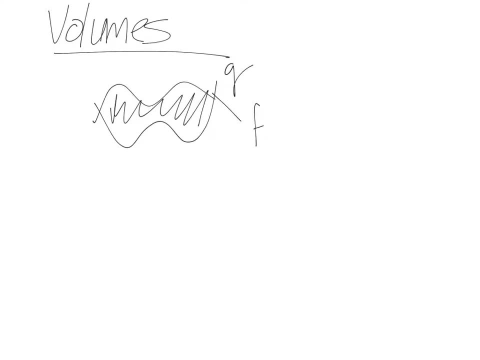 the integral of f minus g between those two points. But now what about if we had something? We'll start off with a shape like this: a cylinder. How would you find the volume of the cylinder? Well, the volume of the cylinder is just going to be base times height, just like the volume. 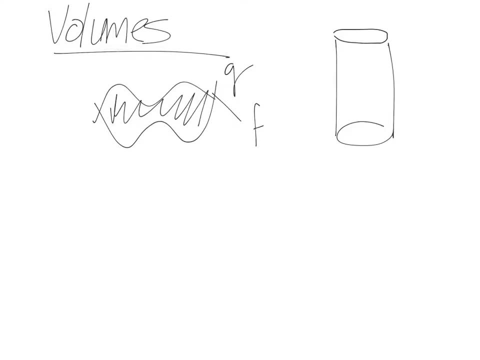 of a box. You take the volume. if this is your height and the cylinder has a radius r, the volume is going to be the base pi r squared times your height, And so we can do that. even if we don't have a circle as a base, you can have some kind. 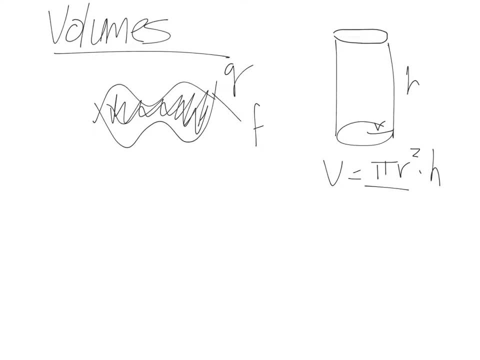 of weird shape like this. We can figure that out. we can figure out that volume. In fact, let's say, we had some sort of volume that kind of got bigger like this and bigger like that and cut one end like this and then the end is circular-ish, but maybe not. 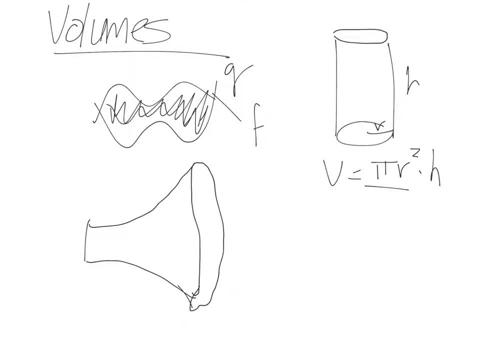 necessarily circular-ish, A little bit off, because it doesn't have to be an exact circle. Well, what we can do is we keep taking slices across, so we'll sort of like slice it with a little plane, and when we slice it across we'll see there's a cross section and that. 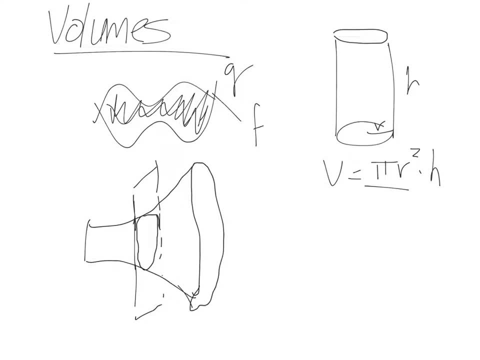 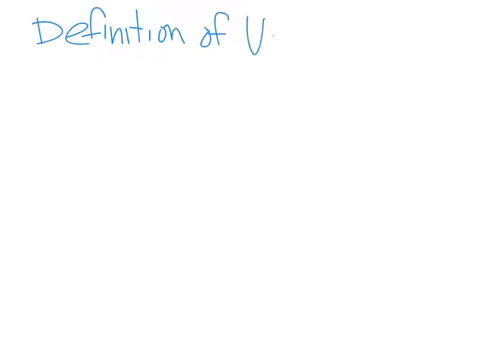 would be what our base is, and so we just go through this, and so we'll have the following definition: So definition of the volume based off of this. So definition of the volume, We'll say: let S be this is a capital S, so let capital S be a solid, and then we'll 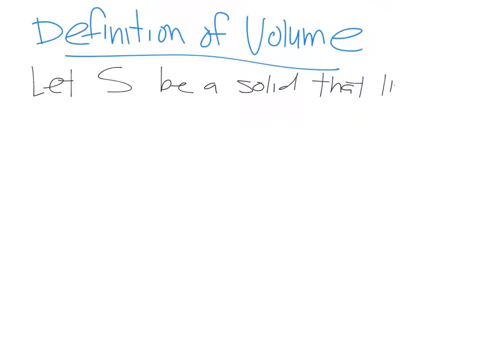 say solid, so not something that's hollow, but solid that lies between x equals a and x equals b, if the cross section, the cross sectional area for S mod A times A. Now, of course, if we don't use the same equation, I'm going toieren this particular formula. 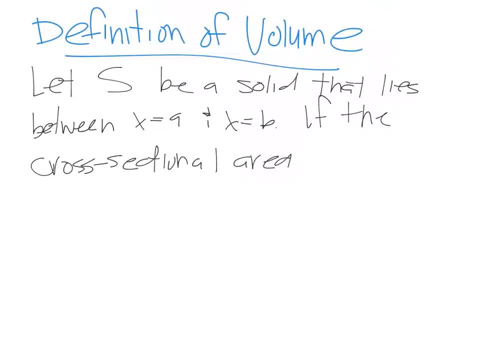 So S, the sum of x, then and, of course, b, the sum of the terms of q with respect to your Plan B. So let S be, let S bedock common and black and solid. So this is solid. so not something that's hollow, but solid that lies between X equals movies. 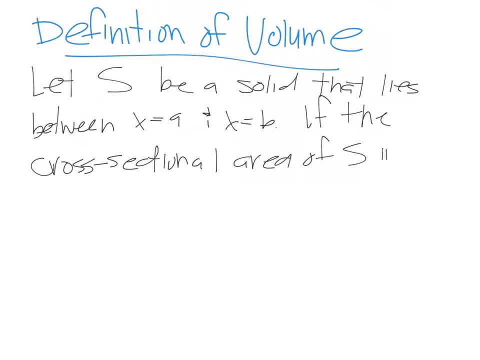 of s in the plane we'll say p sub x. so in the plane of the x-direction this means it goes through x and perpendicular. perpendicular to the x-axis is a of x, where a is a continuous function. so we have this then: the volume of s. 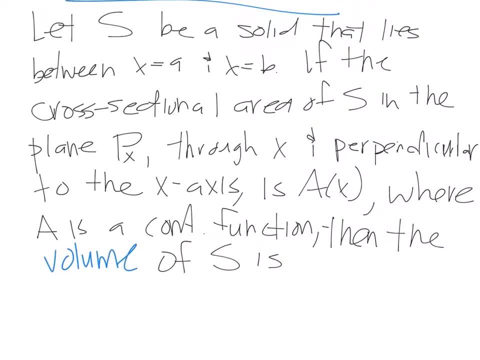 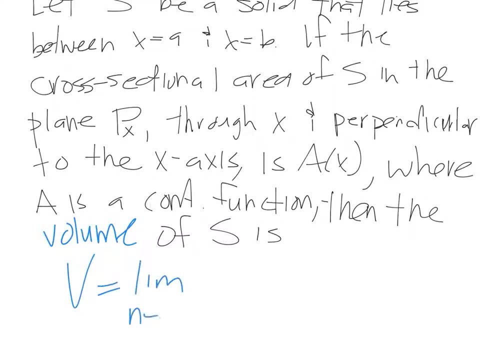 is the following: we have: v is equal to, and so, just like before, we would have the limit, as n goes to infinity, of the sum where i goes from 1 to n. i goes from 1 to n of a, of X, of I, star times, Delta X, which is 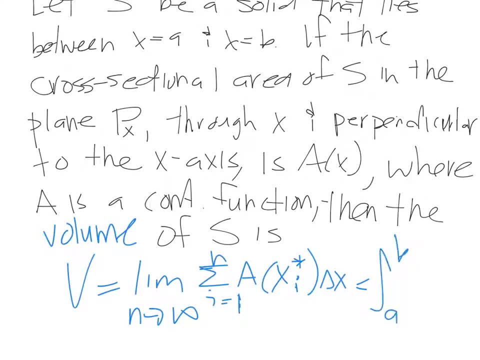 equal to the integral from a to B of your cross-sectional area, a of X, DX. so basically what we're doing, each of these a of X is like a slice, that's the area of a slice, and so we're gonna add up all these areas of the slices, and so when 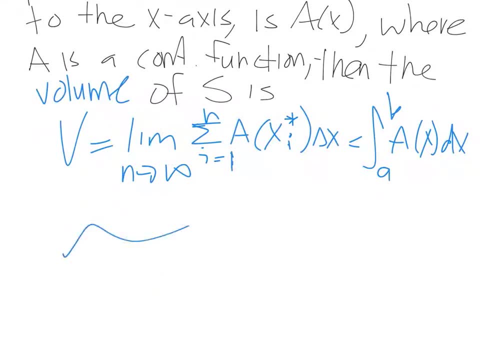 whereas before, when we found the area under a curve and we added up all these straight lines because we started off with, you know, the area of the rectangle and the square, and then we added up all the straight lines because we started off with, you know, the area- blue rectangle and the 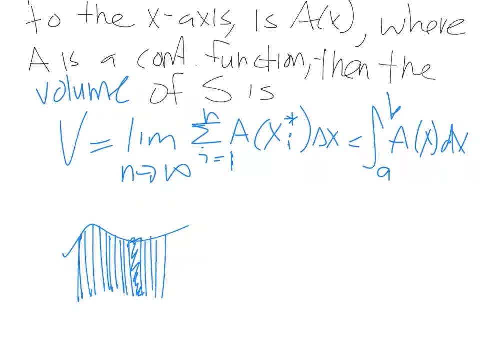 as it got smaller and smaller. we got these areas like this Same thing. let's just say, if it was like a cylinder, maybe not, maybe just something getting bigger- we add up one slice, we'll add up another slice, another, another, and so adding up all these slices. 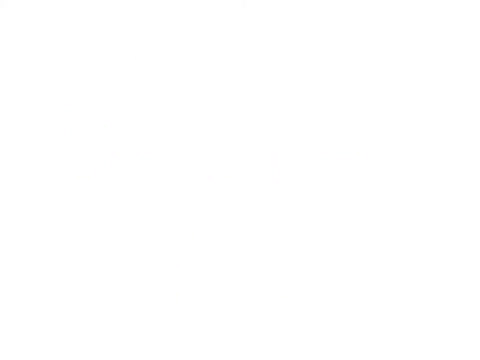 that's what we have. So now let's do an example. We're actually gonna prove right now that the volume of a sphere is equal to 4 3rds pi r cubed. You might remember this formula before, but now we're gonna show how we got this formula. 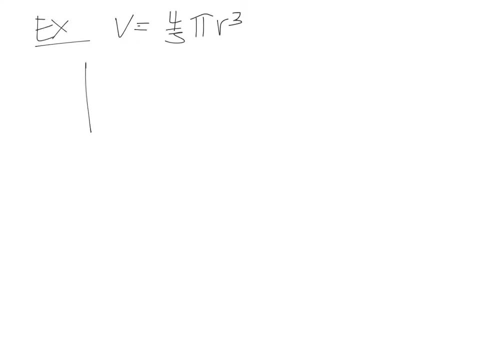 So if you look at a sphere, we have, so this is a three-dimensional axes, x, y, and then this would be z. The sphere comes up like that, but then if we looked at each little cross section, what we have is we have circles, circles, circles. 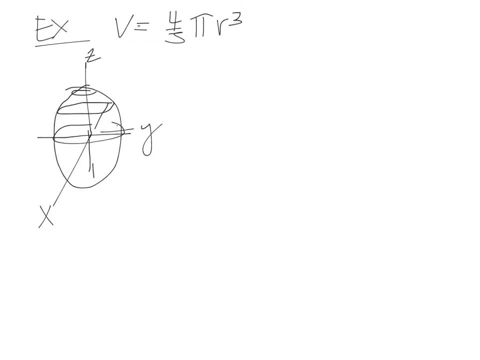 and so forth, And so the equation of each of these circles is: x squared plus y squared is equal to r squared. If we rearrange this, solving for y, we have: y is equal to, to the square root of r squared minus x squared. 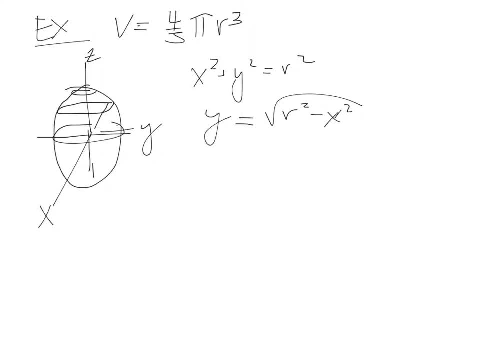 So we're really looking at one of these circles right here and then if these were our axes, so that was the x one and that was the y one, If we want to find the area of this circle, what we know area is pi r squared. 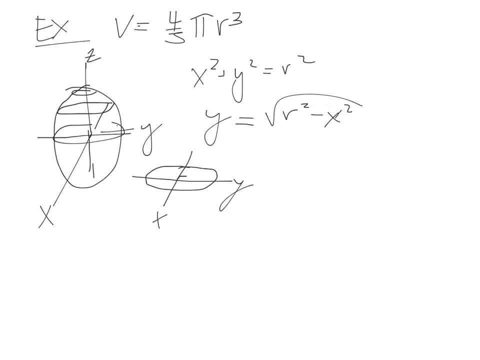 So just by looking at this right here, the radius is this length, This length, y. So your radius is really equal to y, which is the y that we're writing up here. So the area a of x is pi times y squared. 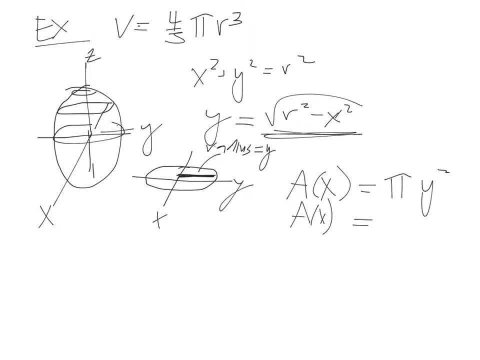 or a of x is going to be pi times the square root of r minus x squared squared. So the square root squared just gives you, you know, just gives you r squared minus x squared. Now we have a function just in terms of x. 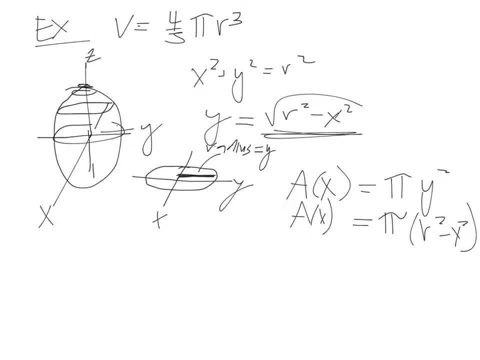 Okay. so now we're looking at here and remember this big sphere had a radius of r, so it went from negative r to positive r, went down here from negative r to positive r and even on this axis, negative r to positive r. 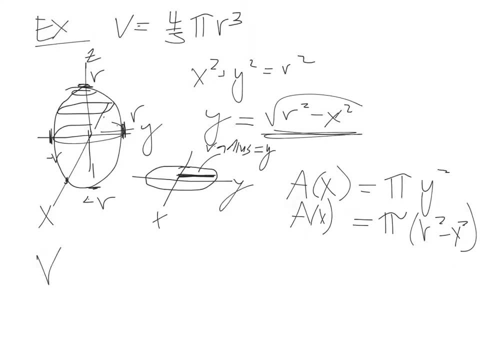 So, if we're computing the volume, the volume is equal to the integral and since we're dealing with x, because our function is going to be in terms of x, it's going to be the integral of a of x, dx. Now, what values did x go from? 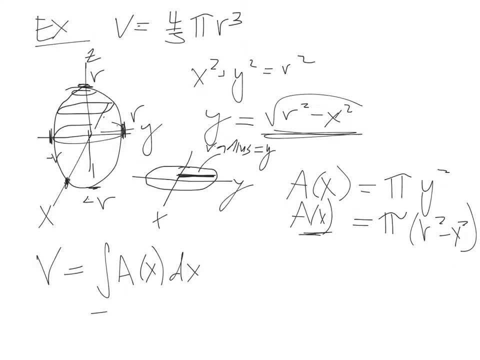 x went from negative r to positive r, So we're going to be integrating throughout all of that. Making the substitution for a of x. we get the integral from negative r to positive r of pi times r squared minus x squared times dx, And so integrating what we get. 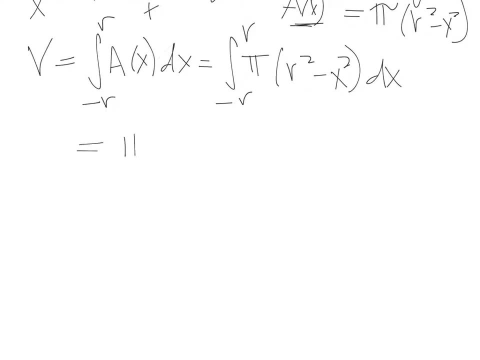 since pi is a constant, we can pull that in front, so that'll be pi times the integral from negative r to r, of the quantity r squared minus x squared dx. and now you may notice this function right here is even: And if you did notice that, 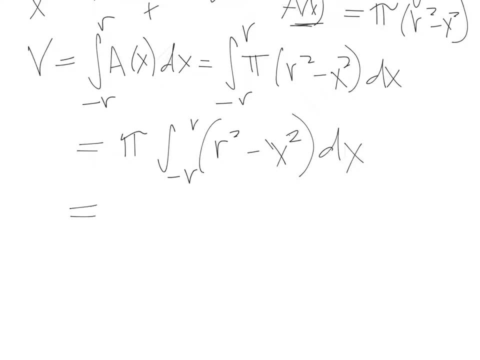 then we can use the property that this: since we're going from negative r to r, it's just going to be twice the integral from 0 to r of r squared minus x squared dx. If you didn't notice that, you can still integrate it normally. 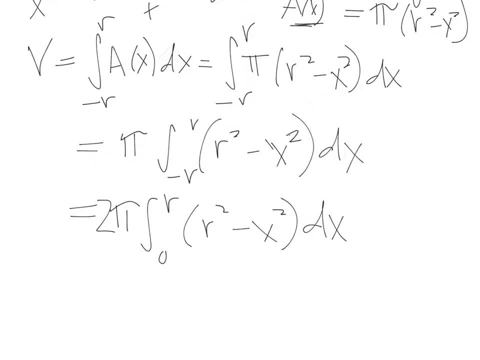 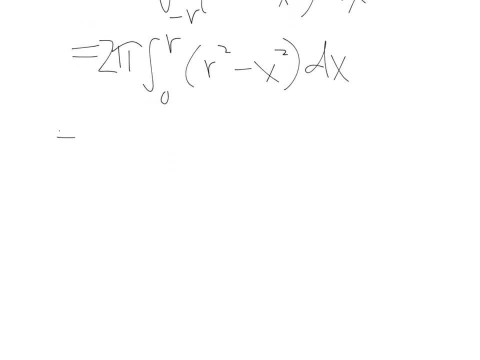 but sometimes integrating with 0 as one of the limits can be a little easier. So integrating we get this is going to be 2 pi times. the antiderivative of r squared is x times r squared and the antiderivative of x squared is 1 third x cubed. 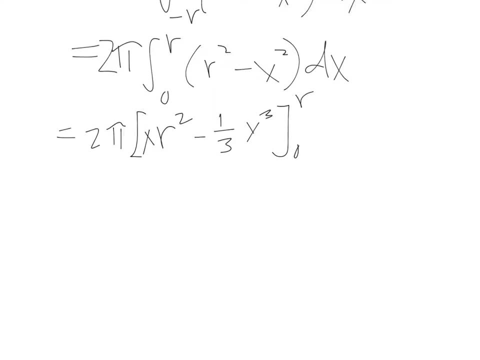 and we're going to go from 0 to r. So we get this is 2 pi times. when we evaluate it at r, it's going to be x times r squared, or r times r squared, gives you r cubed minus 1 third r cubed. 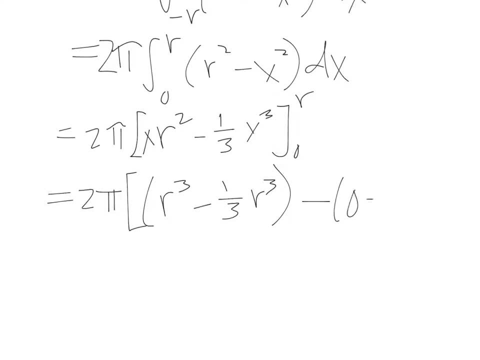 and then when we put 0 in, it'll be 0 minus 0. So this is going to be 2 pi times r cubed minus 1 third r cubed, gives you 2 thirds r cubed, and so this finally gives you: 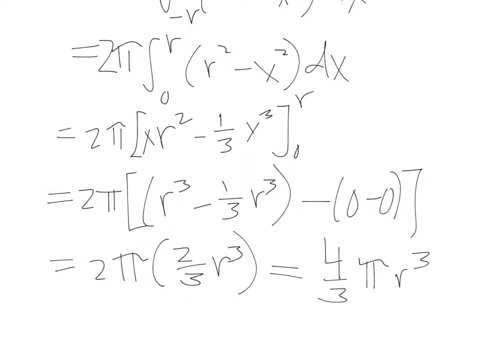 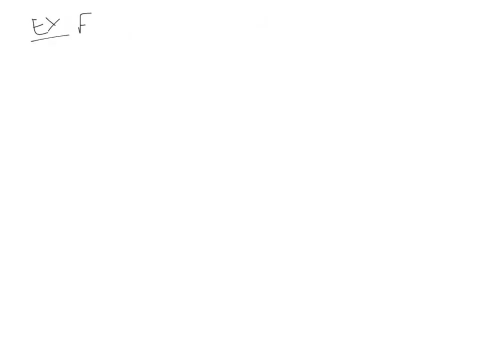 4 thirds pi r cubed. And this is the formula that we know for the volume of a sphere. Now let's do another example. Say we want to find the volume created or that's bounded by the lines y equals x cubed. 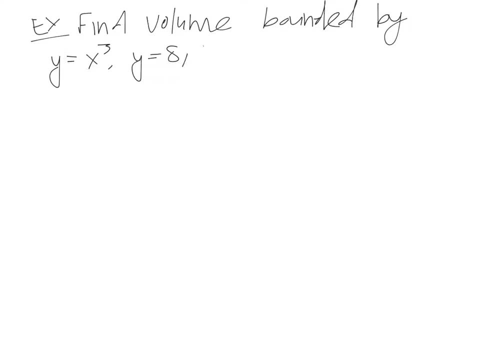 y equals 8, and x equals 0, and then we're going to revolve this or rotate it about the y axis. So first of all, let's draw what this figure looks like. So we have y equals x cubed. 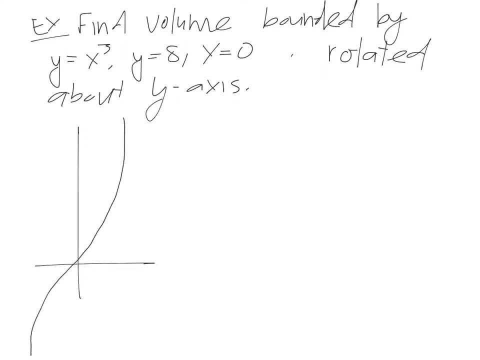 that's a cubic function, something like that. We have y equals 8, so we have something like this, and then we have x equals 0, which is that right there? So we have this right here, and then think about rotating it about. 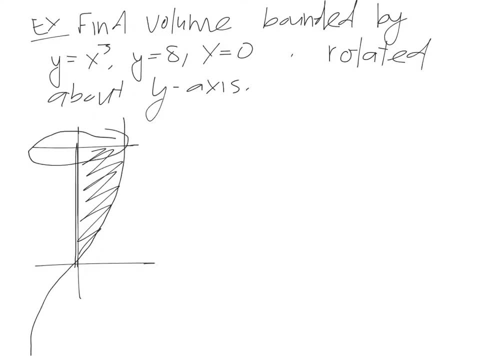 so we'll have something like that: bunch of circles rotate it about and the object looks something like this. So each of these circles that we're going to have, each of these circles, has its own radius, If this is the line. 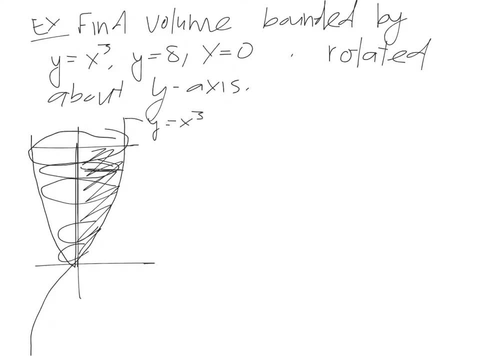 y equals x cubed the radius. here each of these radiuses are going to be the x value. So from this equation above, y equals x cubed, we can get that x is equal to y to the one third power. 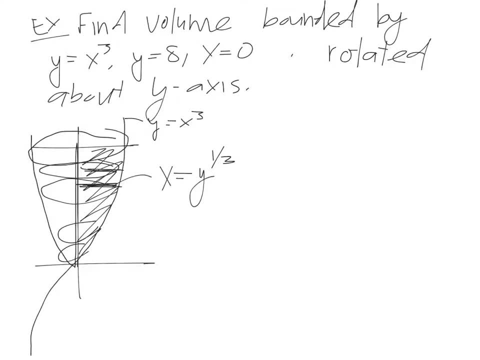 or the cube root of y. So now we're dealing with something in terms of y. So our area, our cross sectional area, is going to be a of y and we know that's going to be pi times the radius squared. 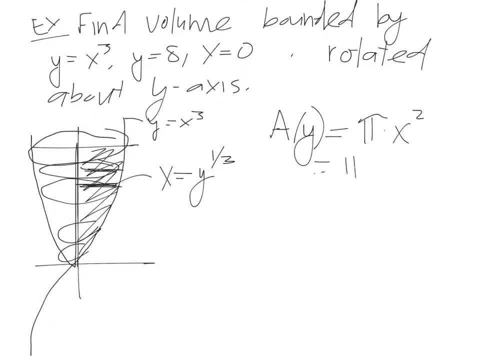 or pi times x squared or pi times, since we know x is from here y to the one third. this is going to be y to the one third squared, or pi times y to the two thirds. So that's the formula. 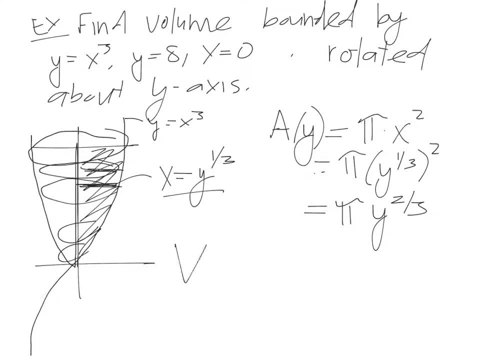 for a of y. therefore we get for our volume. volume is going to be the integral from well, what we're going to have it a of y times dy. So the limits of integration. your y goes from zero. 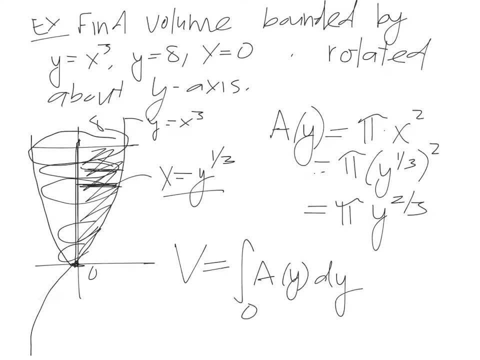 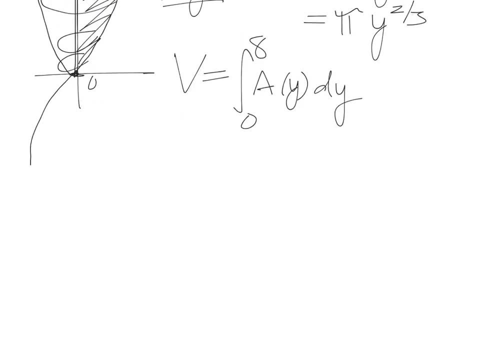 all the way up to eight. So we're taking the integral from zero to eight. therefore, substituting our a in, we get. volume is the integral from zero to eight of pi times y to the two thirds dy, And now we can integrate this. 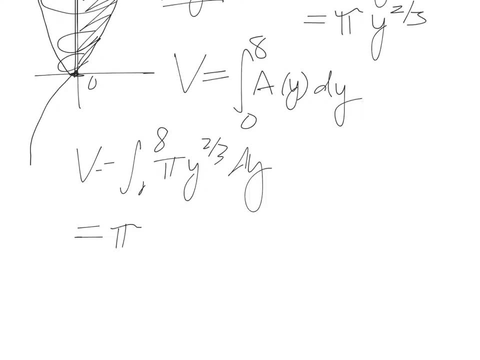 we get y times the anti, sorry pi times the antiderivative of y to the two thirds, which is going to be three fifths, y to the five thirds, evaluated from zero to eight. So we get.